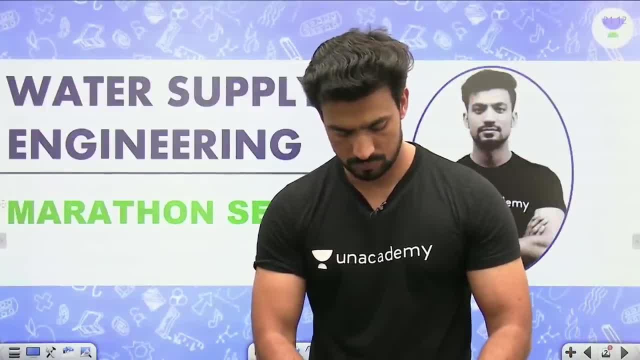 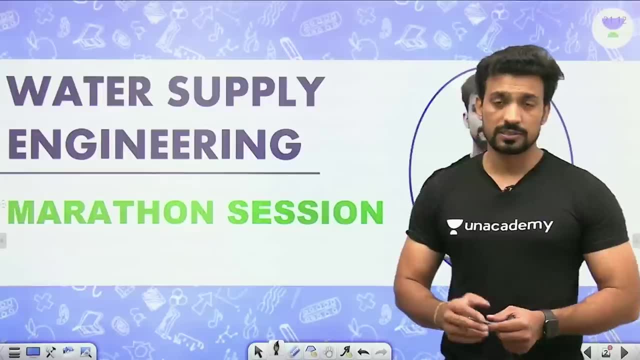 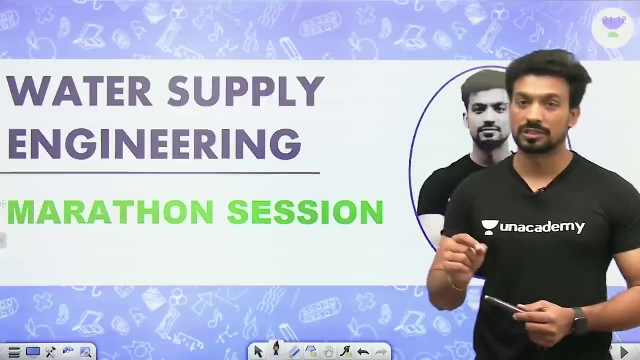 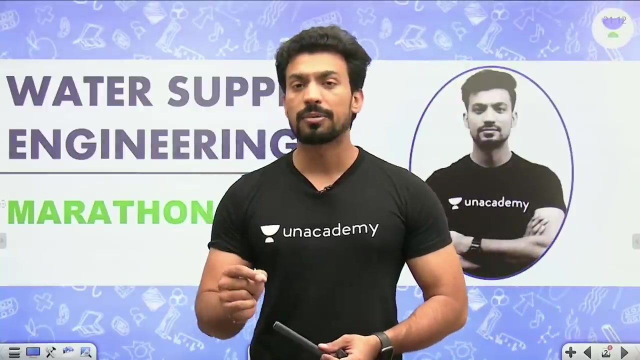 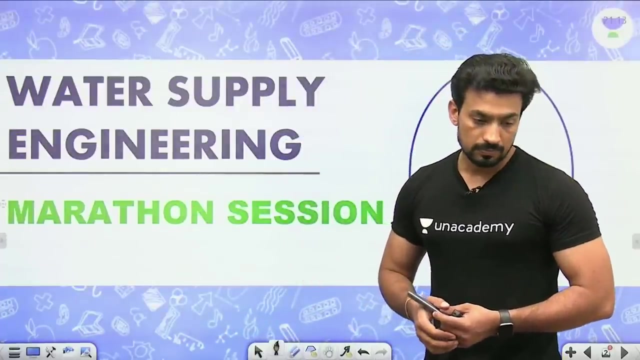 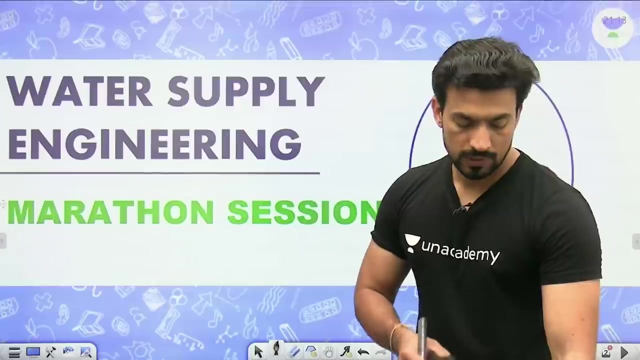 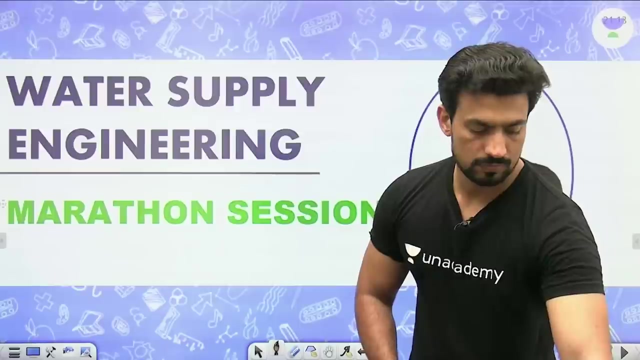 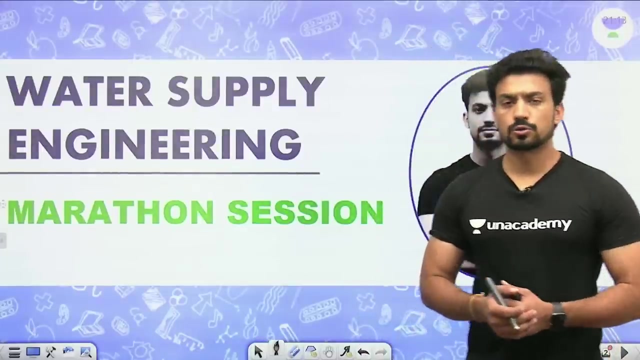 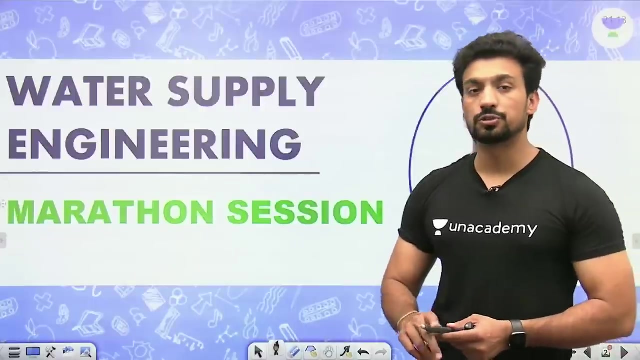 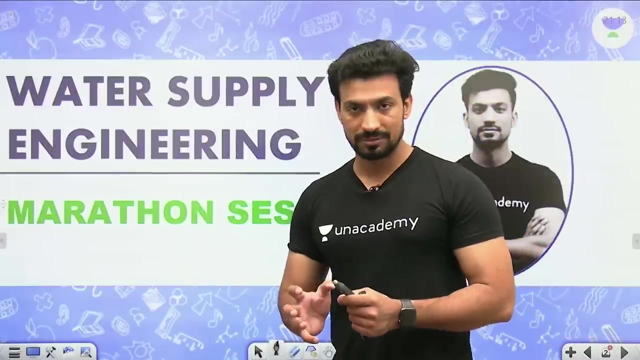 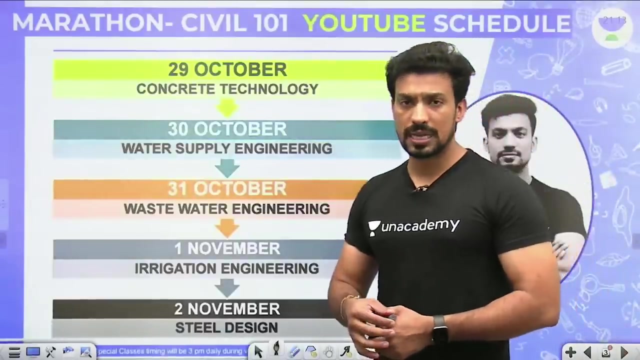 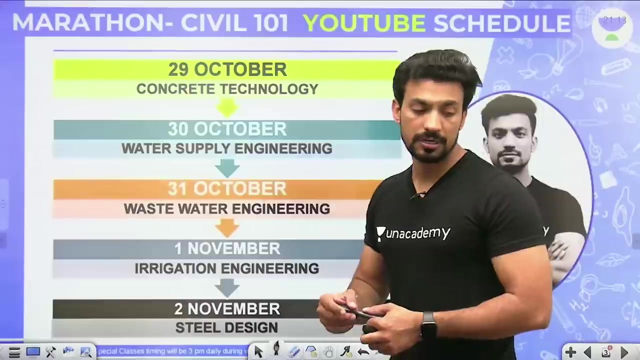 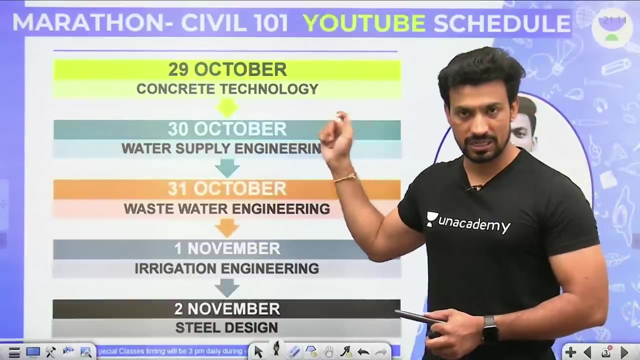 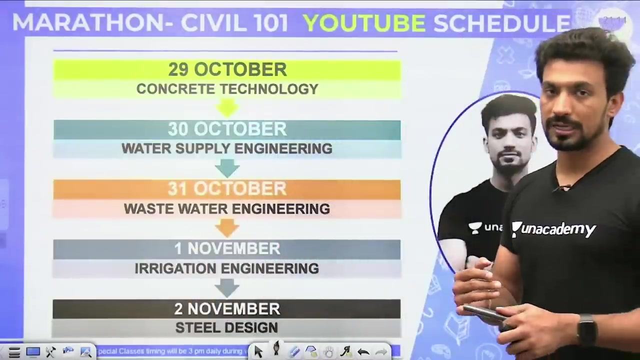 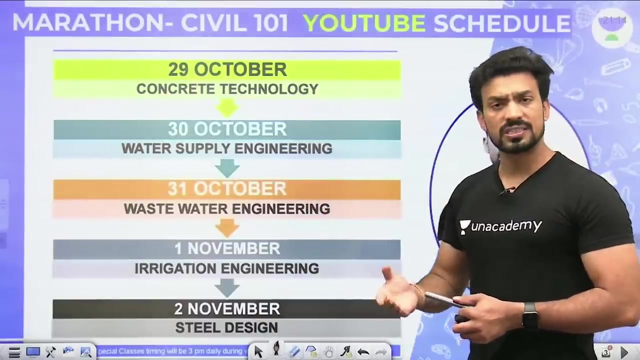 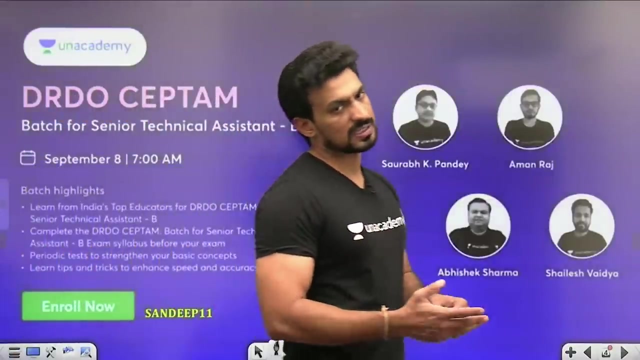 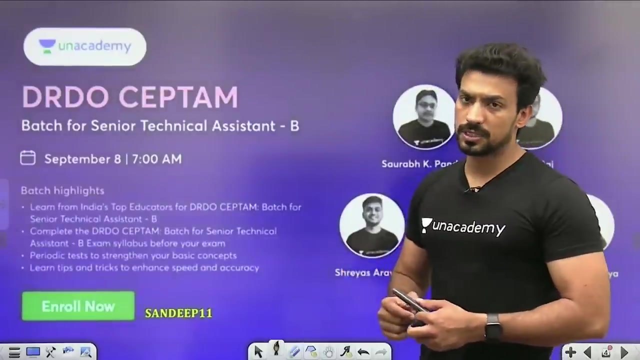 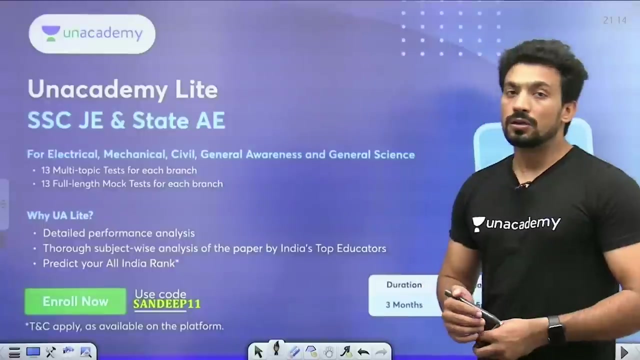 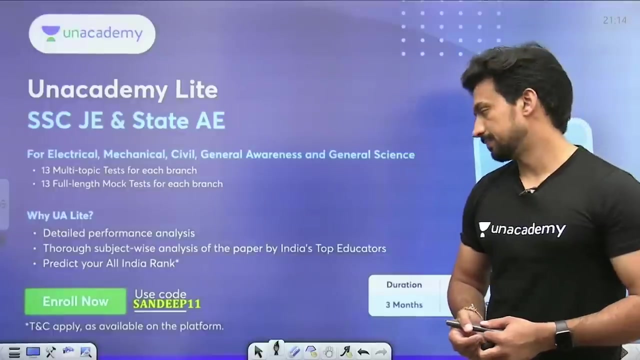 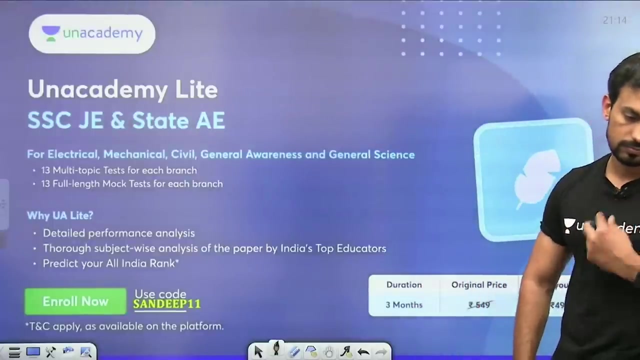 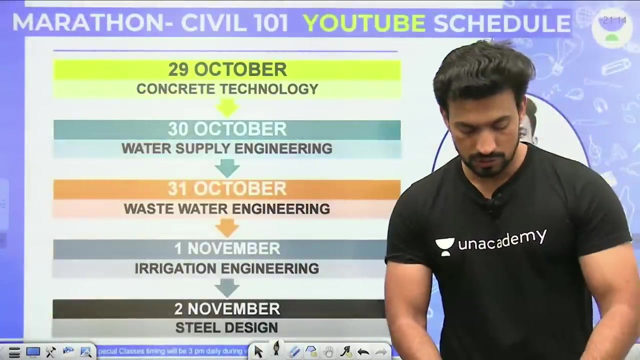 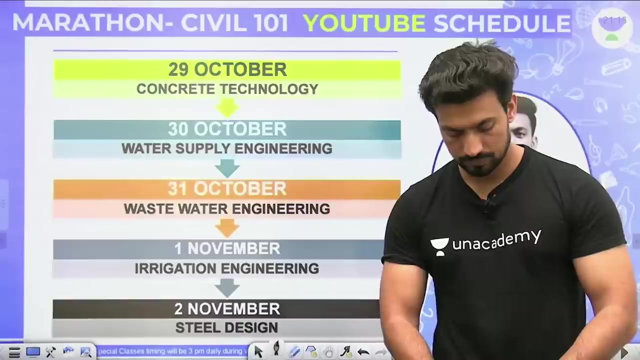 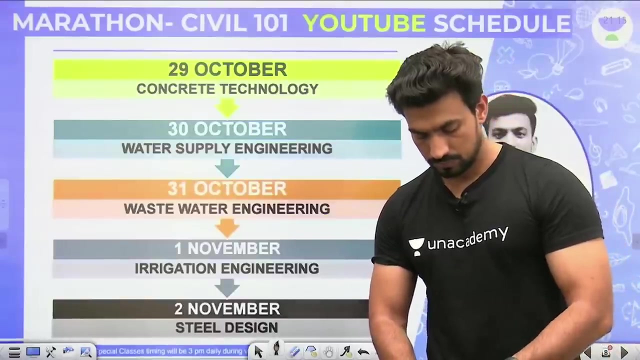 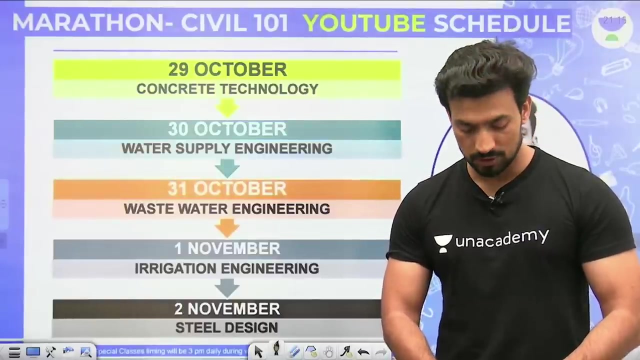 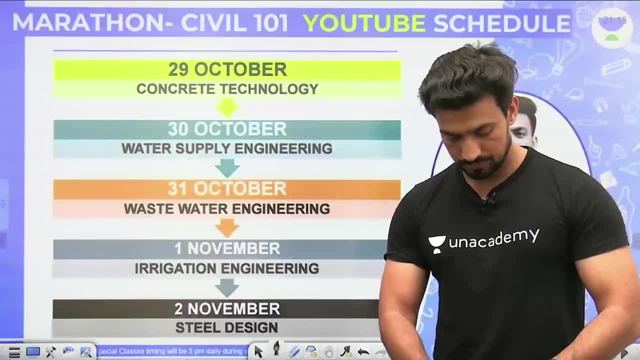 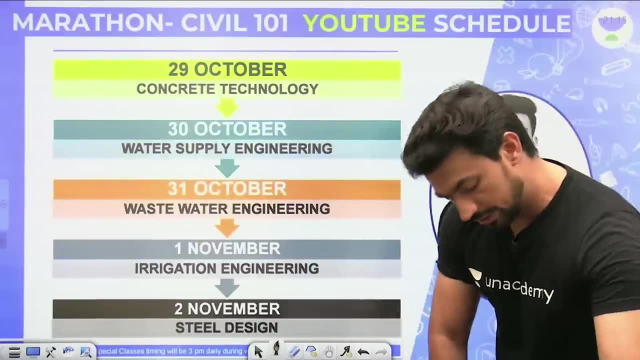 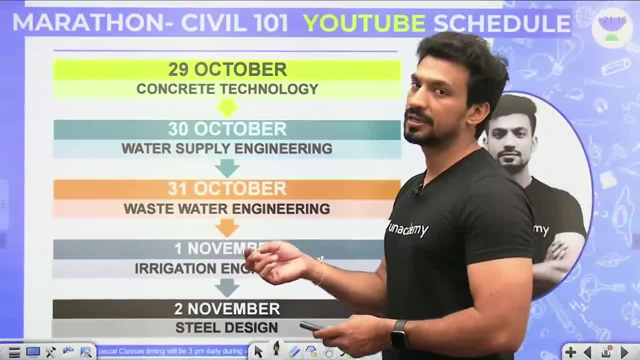 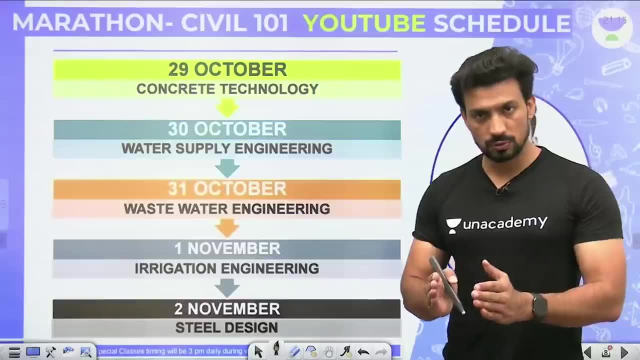 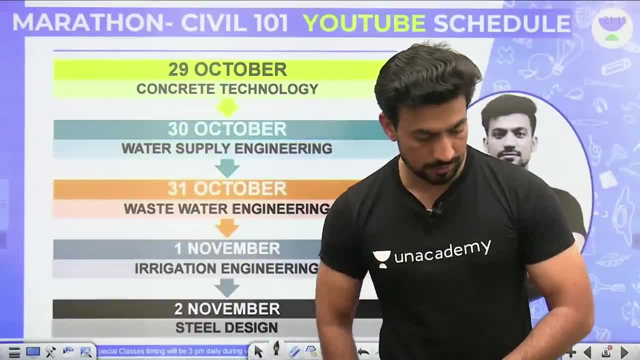 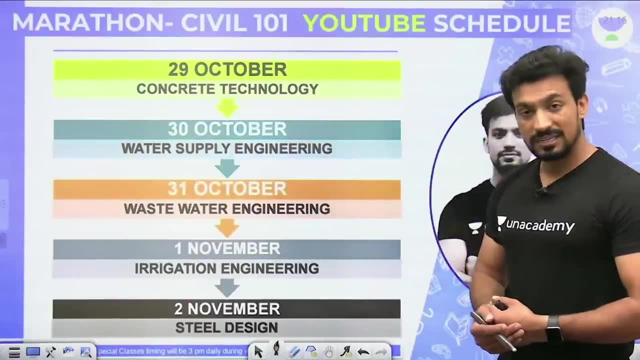 And this one is just itself. This is one of 6 slash schools. It is 5 to 5 grade schools. For 1 class school, we will have 2 like schools. We will have them French class 다면 hutim senior П conc 얼�ع❤️. 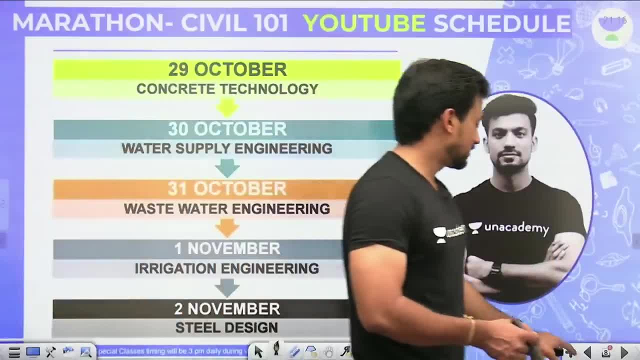 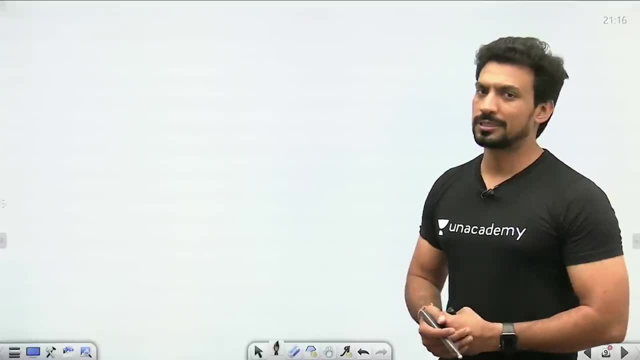 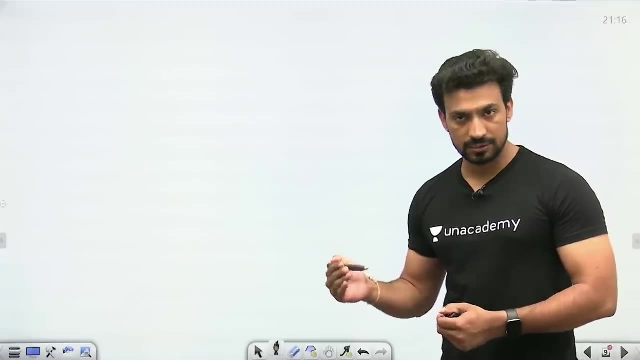 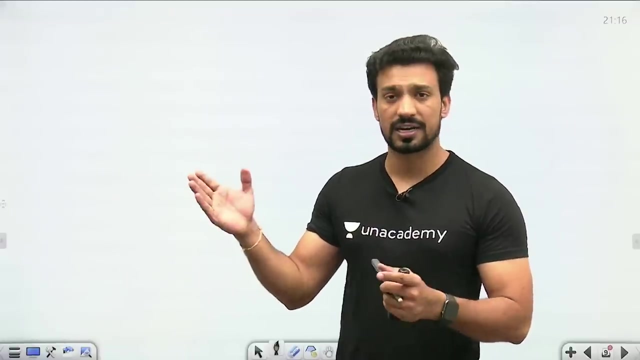 This is such a beautiful subject that everyone likes it and examiner also asks it from every aspect. There are many specifications and data in this subject that what are the properties related to water? that should be there. Now, if you talk about the same thing, for you, that the water is good, if you can see the water clearly. 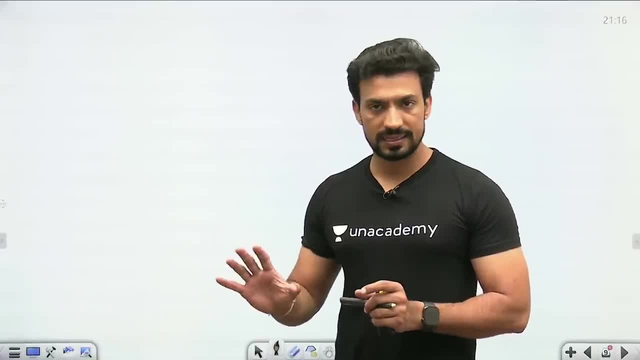 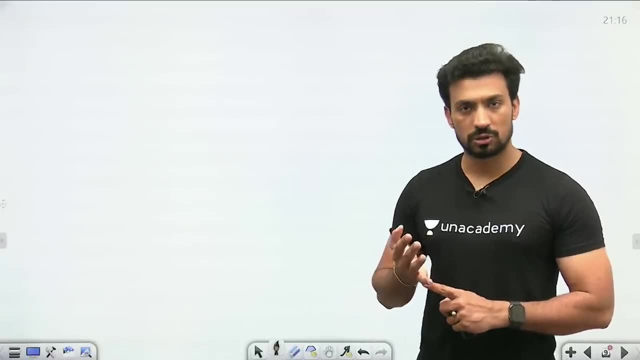 if you can see it only in the visibility, then can we say that the water is good, safe and drinkable? We will not be able to say. we will have to define many parameters so that water is physically, chemically and biologically safe for our drinking purposes. 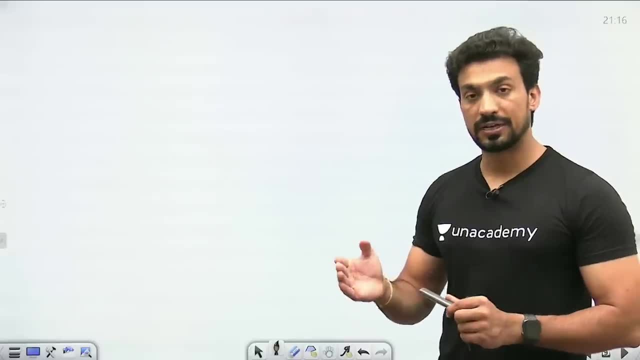 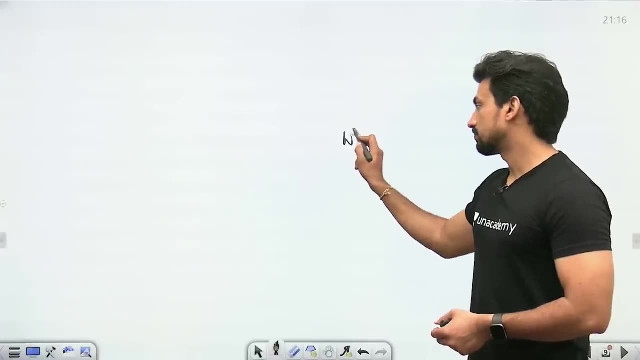 Now, who will tell if it is safe or not? or if it is safe, then to what parameter it is safe? who will tell this? These are some organizations that tell us. as we talk about WHO, as we talk about the Indian Standard Code, we have IS codes. 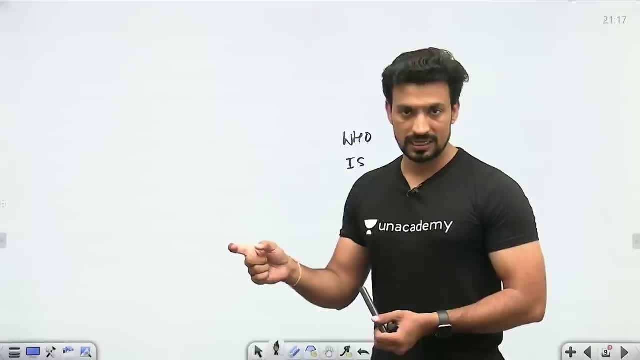 Or if we talk about the Indian Standard Code, we have IS codes. Or if we talk about the Indian Standard Code, we will talk about the Indian Standard Code. we have IS codes. Now, if we talk about water, then we have the Government of India Manual water supply, engineering or related to water supply. 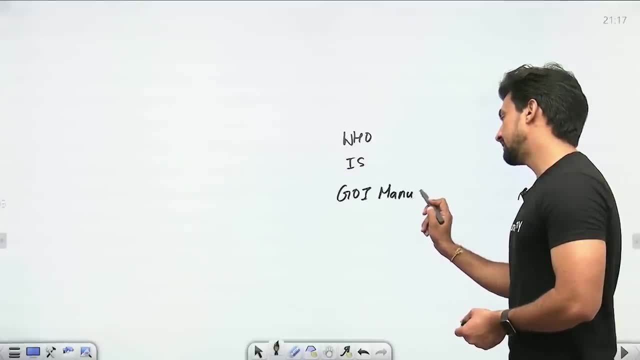 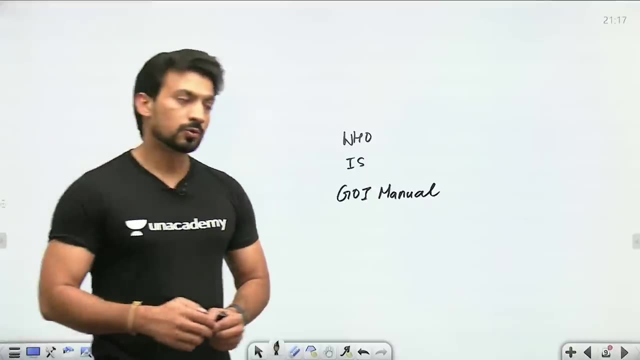 so we will talk about it, so we will have the Government of India Manual. Now again, let's come back to that topic. this subject is like your friend. this subject is also like your friend. So when you face any trouble in this subject, do you leave your friend, do not leave him. 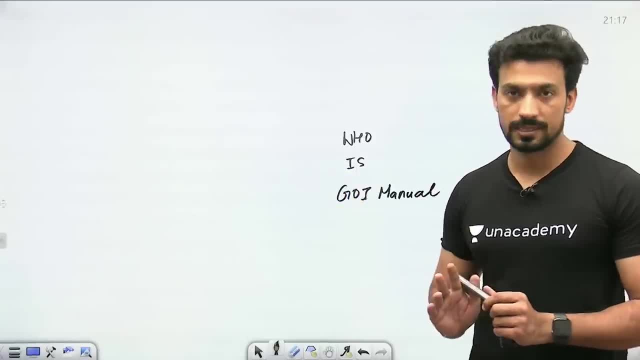 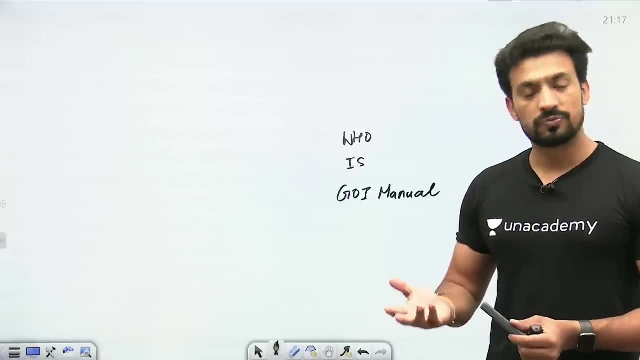 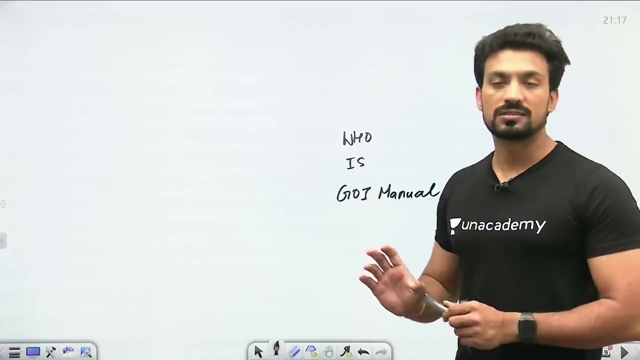 anyway. this subject has to be left in the course of the problem or the exam. But do you take your friend as seriously as he actually means or wants? No, you have to do the same thing here. Whatever data you see, whatever dangerous things you find, you don't have to take them that seriously. 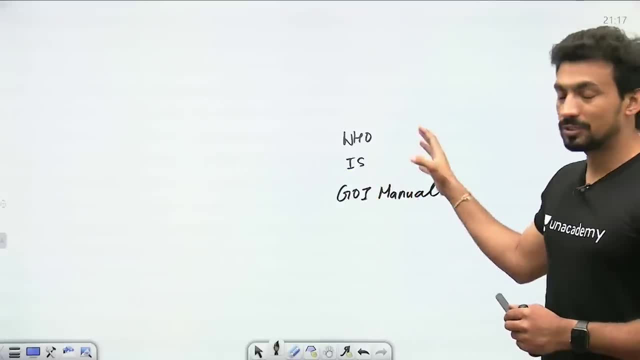 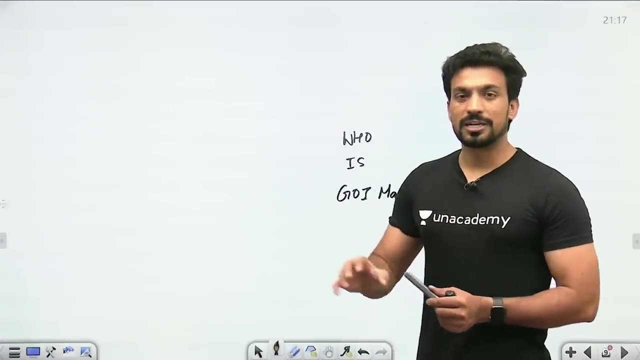 Just listen to the knowledge that is told, the data that is shown to you for reference, that, yes, this is to refer that if there is any need to see any data, then you can see it from here. Sometimes it happens that if we want to see any data, then what is it? according to WHO, 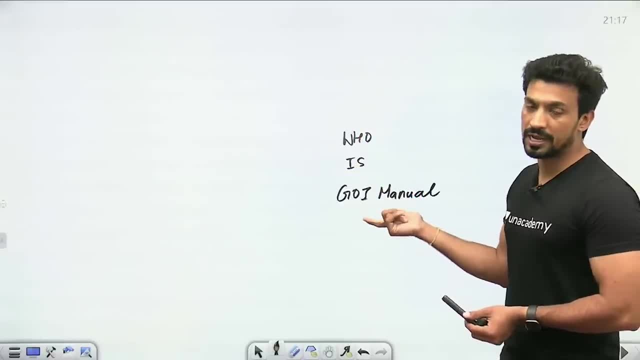 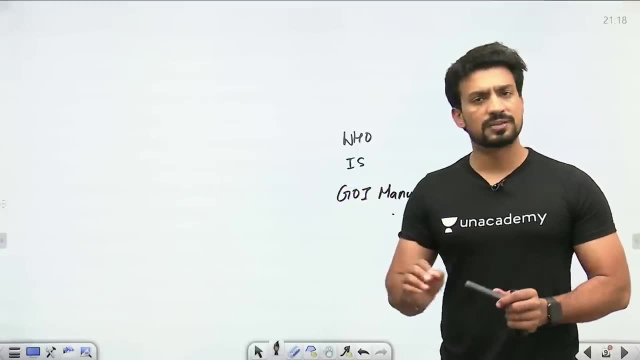 what is it according to the Indian Standard Code and what is it according to the Government of India Manual? If you want to see this, then you don't have to work hard. All this data will be given to you in this session, along with the PDF that you will get on telegram. 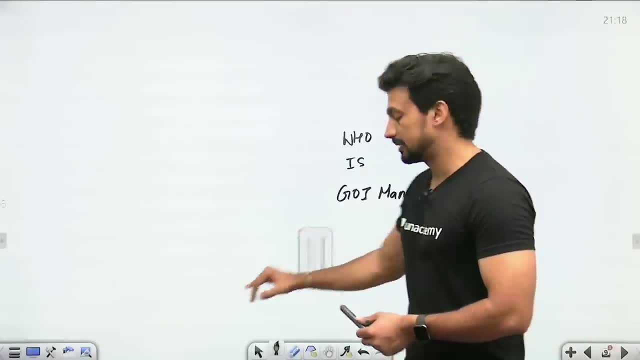 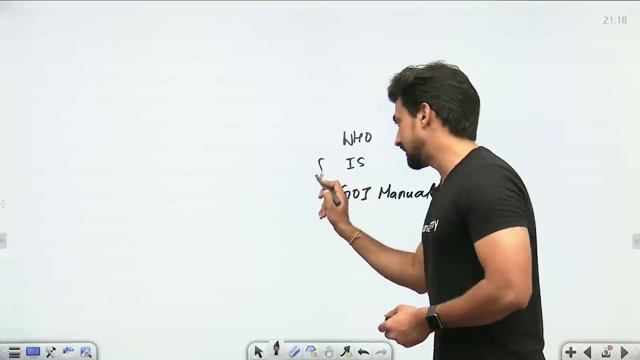 You can search by the name of Sandeep Jani after this live stream is over. So let's start our friends. whatever data will be related to WHO, although I would prefer more data- which is ours, or our exam centric, which is our exam centric. 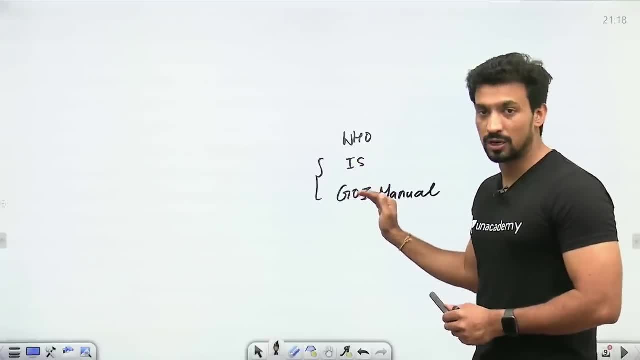 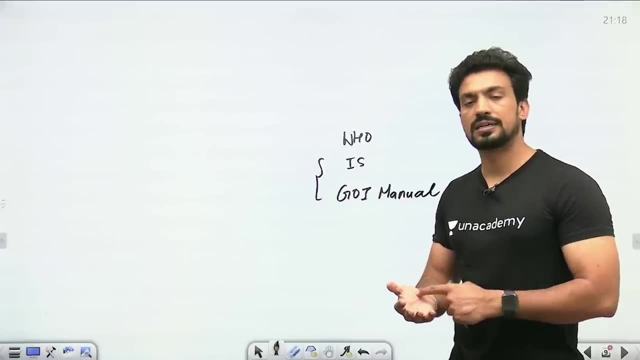 we will go near the Indian standards: Indian Standard or Government of India Manual. Now there are some variations in the data of these three, Somewhere in some exam, whether it is of the state, whether it is of ESC, whether it is of SSC. 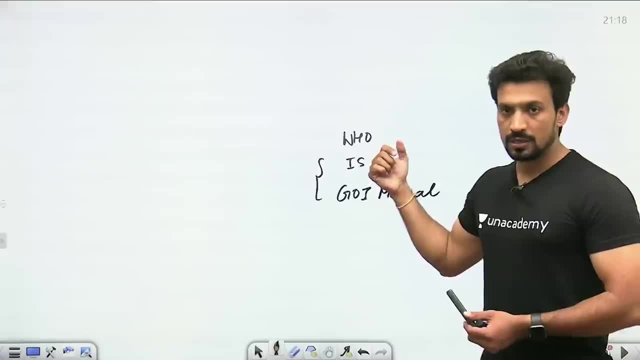 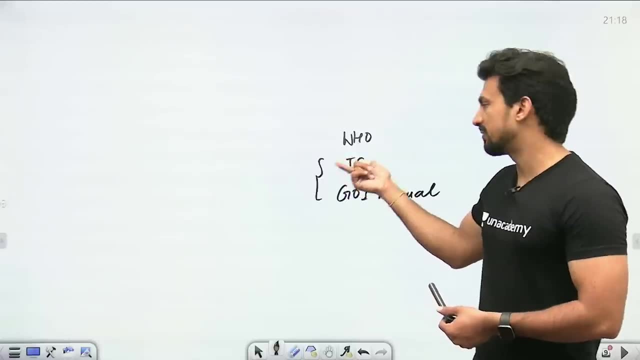 such a question was asked that tell this value according to WHO, Then you must have seen that we have written something else in the notes in the class. So what we have written in the class, in the notes, it is mostly according to the Government of India Manual or the Indian Standard Code. 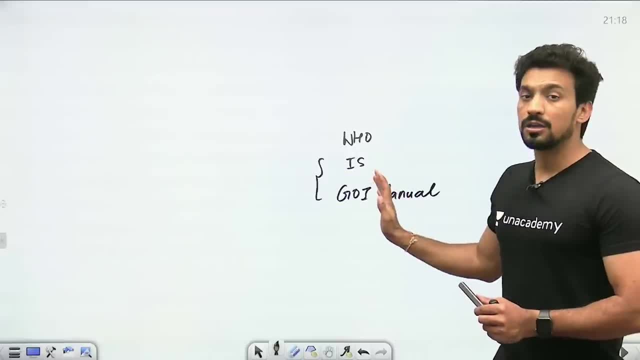 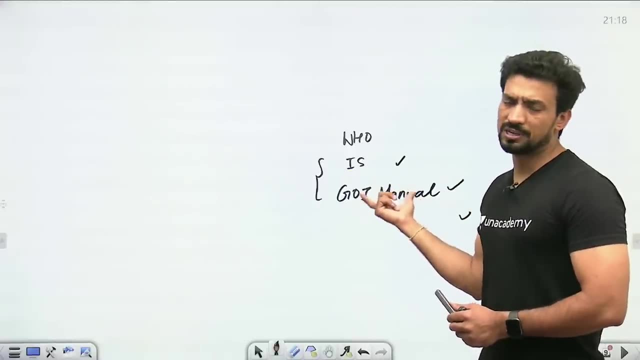 So you don't have to worry, you will get all the values here today, But keep in mind that we have to focus on these two values, on these two And the majority of the things that were taken in the Government of India Manual. 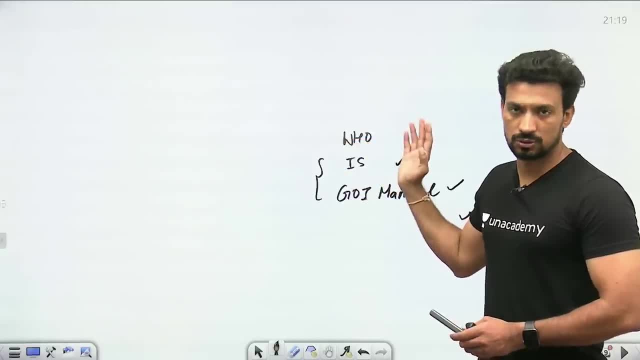 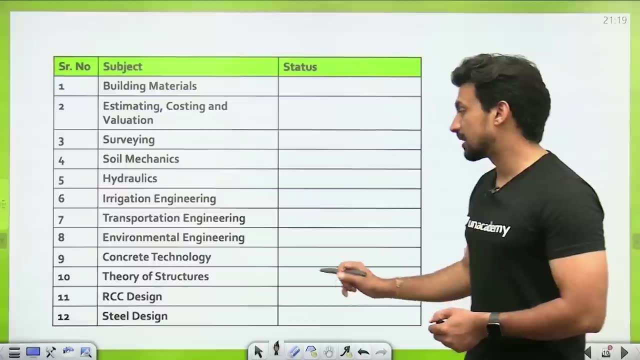 they were either taken by the Indian Standard Code or something was taken by WHO. We will talk about them too, If we talk about the subjects so far in the series of marathon sessions, one of our subjects has been covered, which is concrete technology. 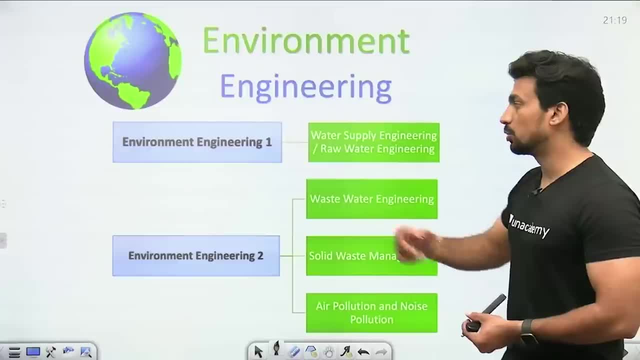 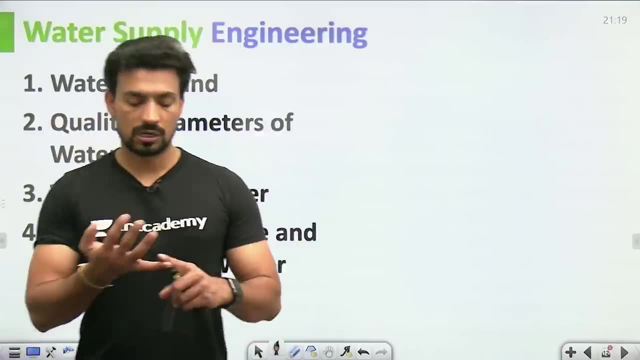 This has been done and now we have gone towards environment engineering, which has two parts: part 1 and part 2.. In part 1, we are studying water supply engineering. today, If we talk about water supply engineering, then first of all we have to understand what is the demand of water. 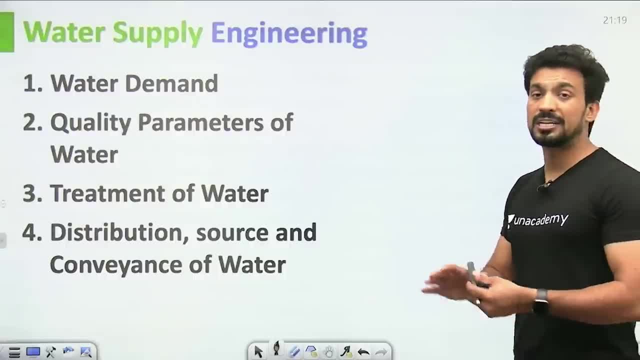 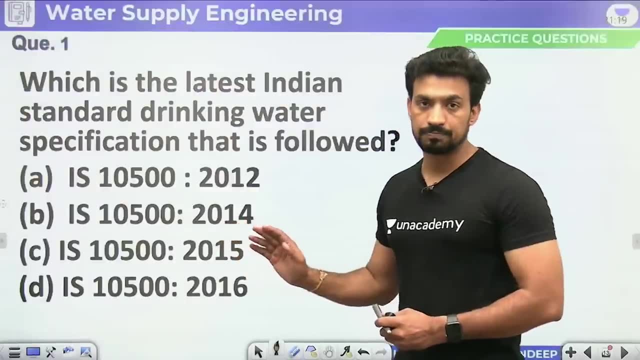 then what are its quality parameters? If those quality parameters are not meeting in the water, if it is impure, then in that case we will treat it. After treating it, we will distribute it. Now comes the most important thing, which is such a code, which is the latest standard. 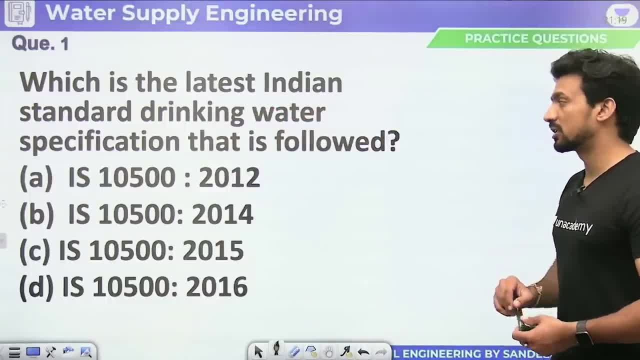 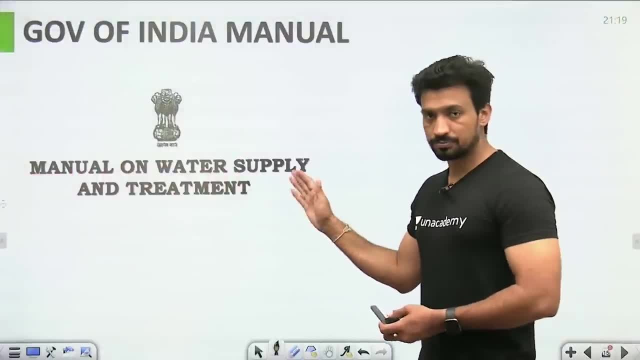 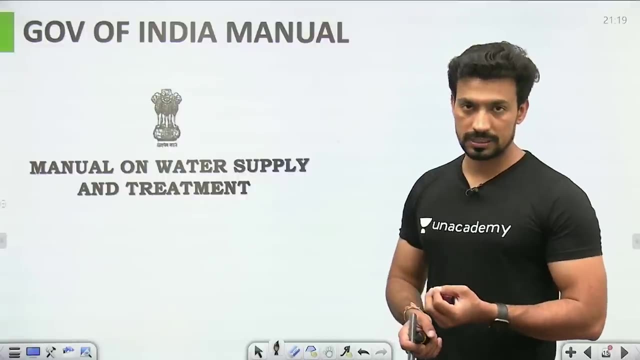 which is the Indian Standard Code for drinking water specification that is followed. So its correct answer is 105 00 2012.. Option A will be our correct answer. We will also get questions And I have one more request from all of you, dear friends. 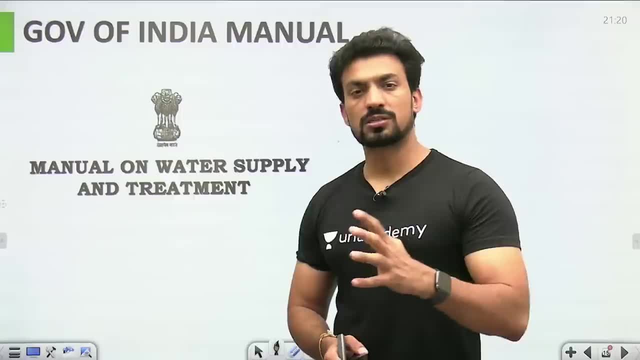 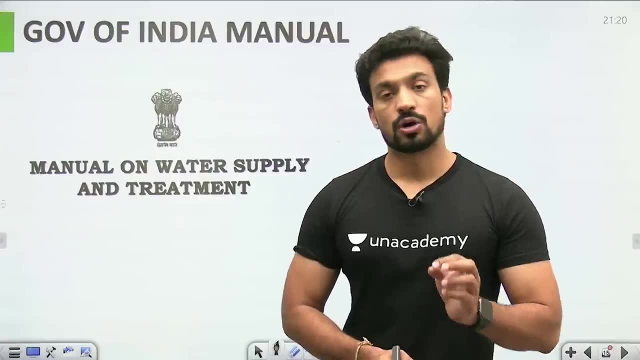 If you think there is a lot of data happening, Sir. so many tables, so much data, how will we remember? how will we remember then? just keep listening, Focus on whatever is important to be told And do all the questions well in the class. 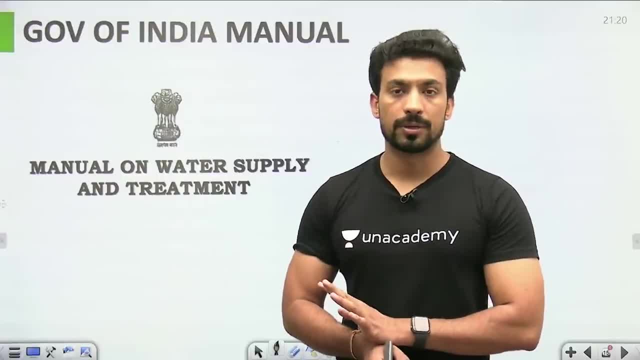 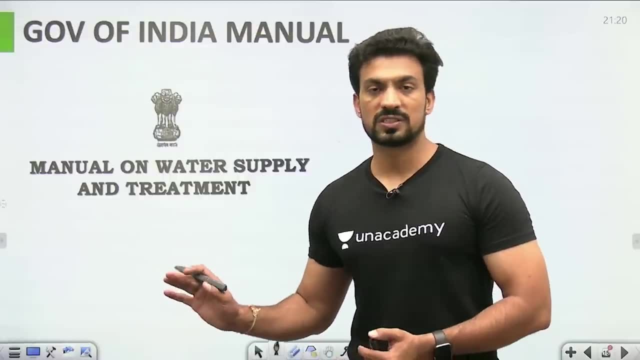 You will get to see the majority of the questions around them in the exam. So right now, at the last moment, don't say that I don't have this subject. I will leave it. Just do these questions once. All the questions in today's session. 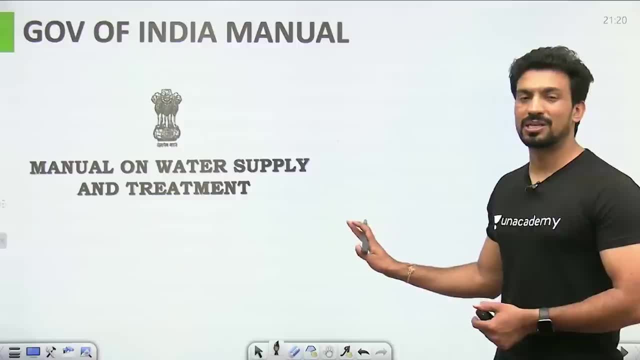 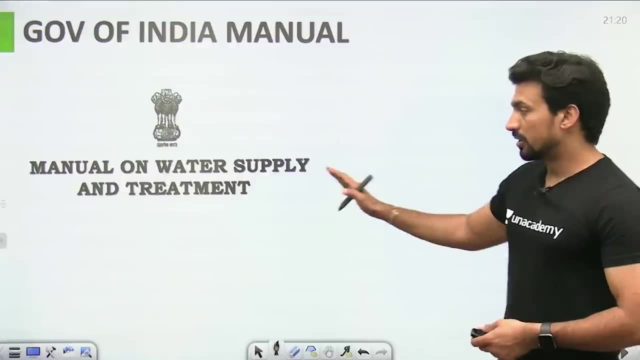 there will be almost 135 questions. So just look at all those questions. So your part of this- Environment Engineering 1, that will be covered by 90%. Government of India Manual. Now I am showing you, for reference only, what kind of data is given in it. 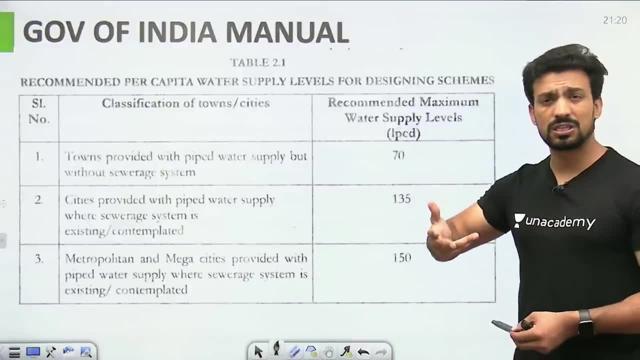 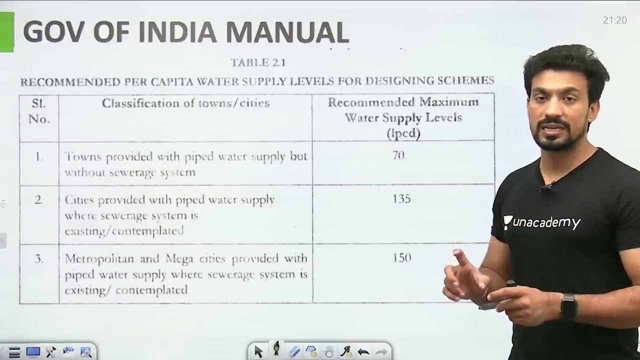 Okay, you have data in it. Like many times you see questions like this: that in someone's answer how much water demand is there? 135 has been given, in someone 270 has been given. So how was all that data answered? 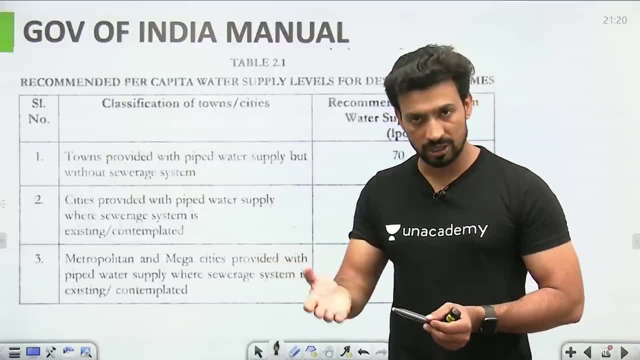 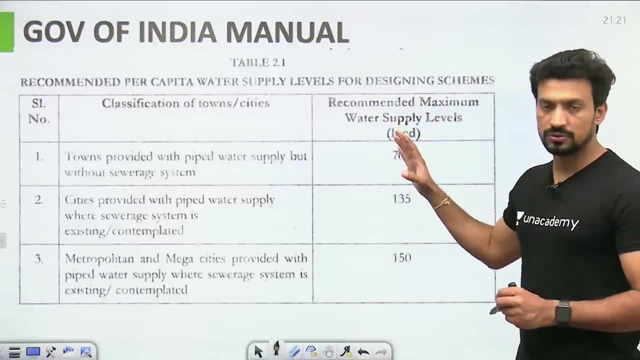 What did the examiner want? The first thing is that the examiner should say that tell the Government of India according to the manual, or particularly according to the code, or according to the WHO. Still, to avoid all the confusions, to just clear the cloud. 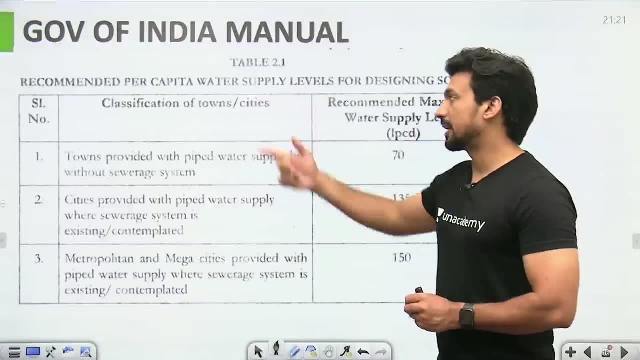 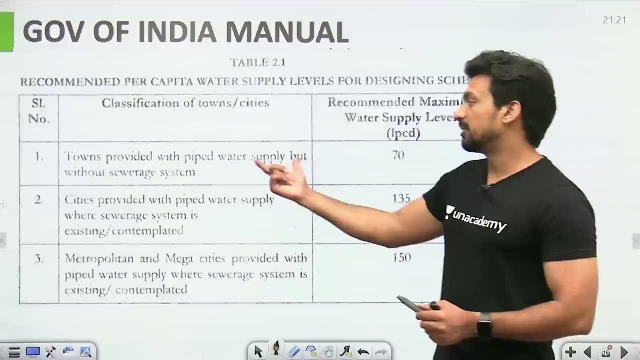 in front of you all the exact data, as it is Recommended per capita water supply levels. Now we will not go towards them, towards remembering them. I am just showing you this for reference: Towns provided with piped water supply but without sewerage system. 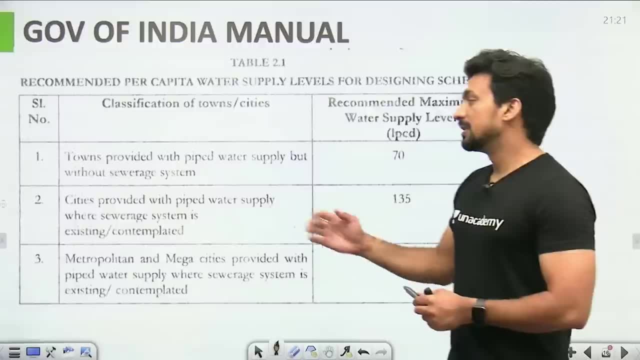 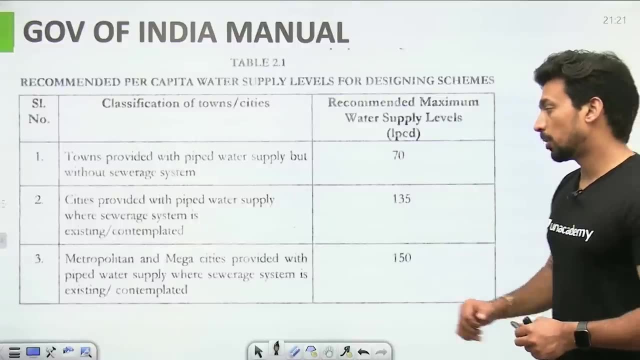 So in that case 70 liters per capita per day will be considered. Cities provided with piped water supply, where sewerage system is provided: 135.. Then metropolitan and mega cities provided with piped water supply, where sewerage system is existing. 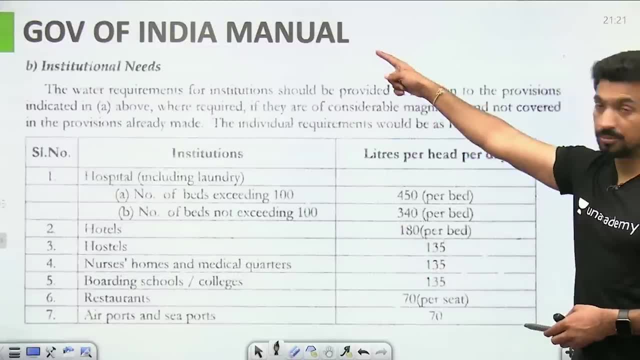 or contemplated. So in that case, 150.. Who is telling this? This is the Government of India telling us manually. Then, after that, if it comes to institutional needs, then how much water should hospitals need? How much should hotels need? 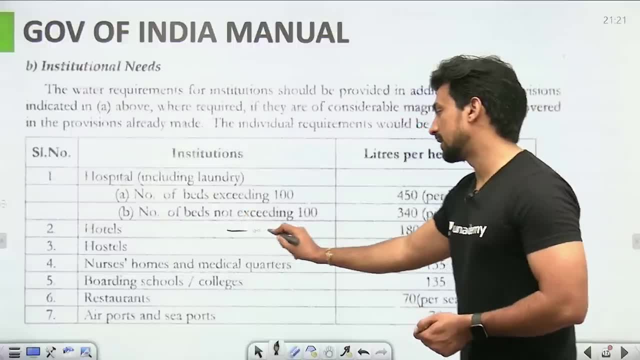 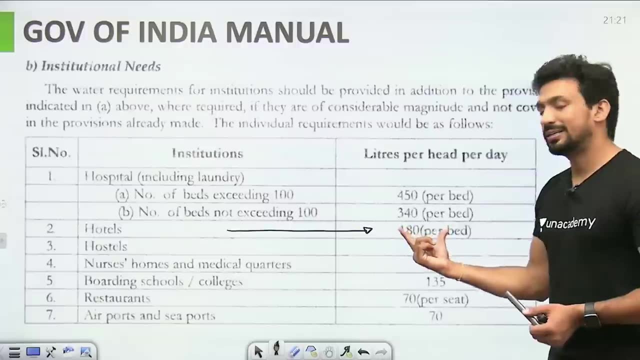 How much should hostels need? Now let's focus on a small point here, which is our hotels. Okay, For hotels, what did the Government of India manual tell us? 180 liters per bed, it told you here For hostels. 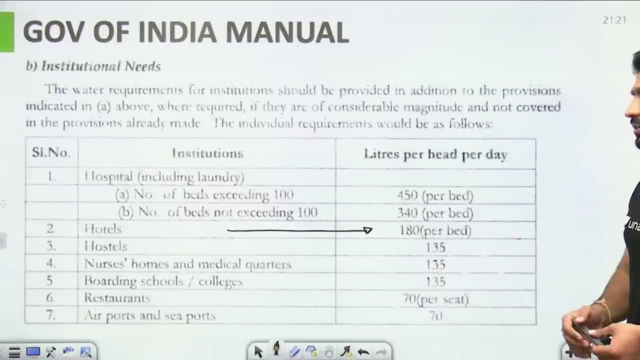 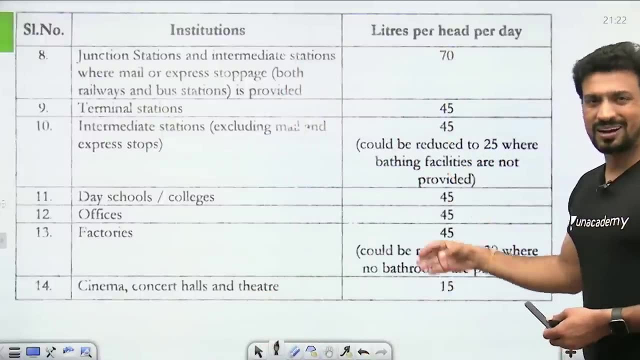 if we talk about 135, nurses' homes, medical quarters 135, and so on. all this data as it is. who gave this data? This is what the Government of India manual gave us. Then a lot more data according to different institutions. 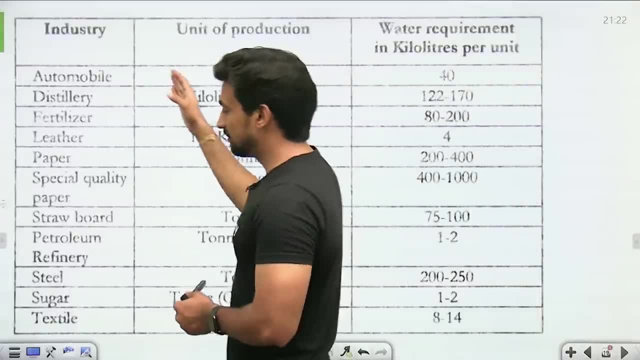 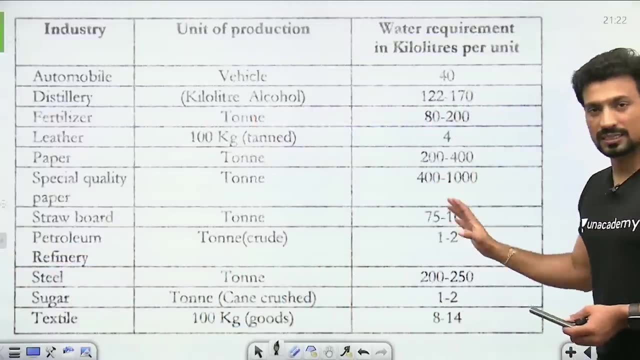 or if we talk according to industries, then this industry to industry varies. what kind of industry is there? what kind of? how much amount of water is going to be utilized? You don't have to take this data so much on your mind. 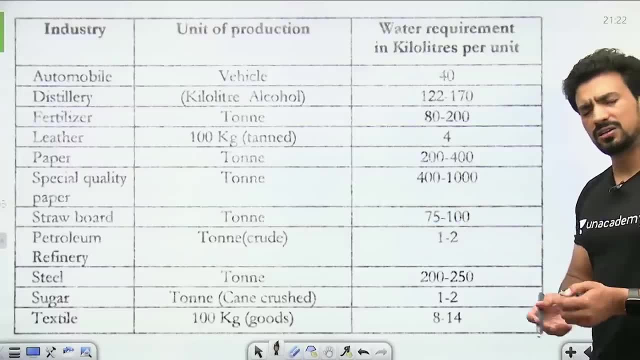 that. what is this? do I have to remember all this? No, don't remember. Somewhere in some one or two exams, someone must have been asked. even in that, you will be able to answer it with your mind. if you compare that. 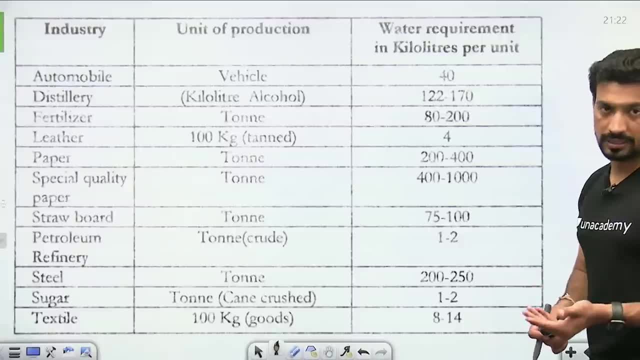 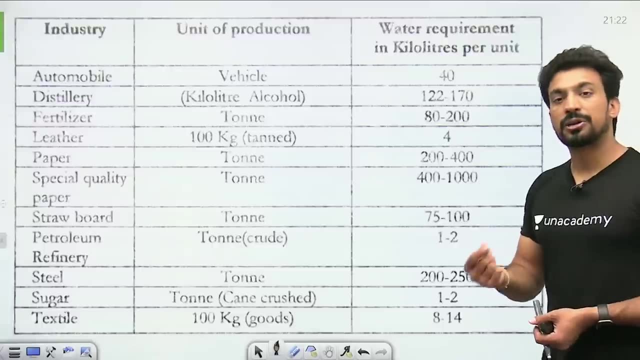 yes, which industry is such in which more water will be needed, Like if you talk about the paper industry, paper and pulp industry, then a lot of quantity of water is used in it. If you talk about the petroleum industry, then very. 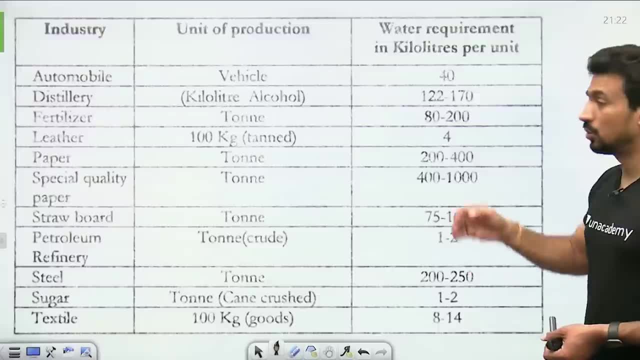 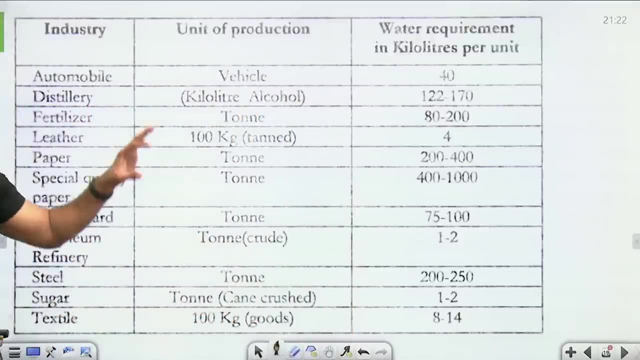 very little, very little. one or two kilo liters per unit. kilo liters: we are talking in terms of 1000 liters. So just by looking at the comparison you will be able to tell If you want to compare further for reference. 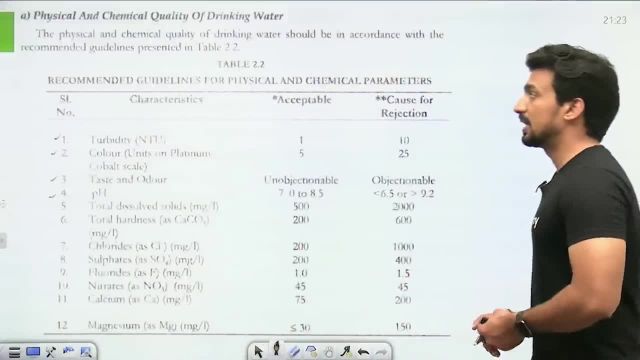 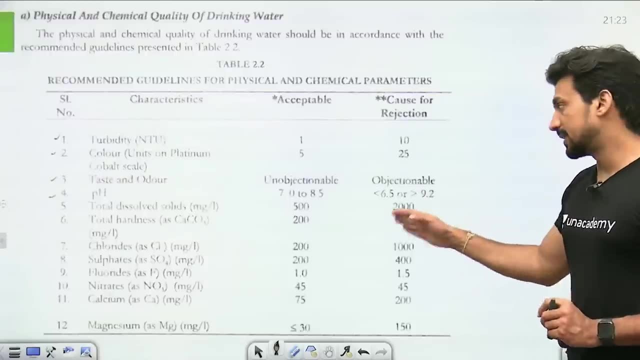 then you have this data here as it is. you will get it Then after that: physical and chemical quantity of drinking water. I will not make you remember all these values right now because we will go according to IS code. Most of the values have been made. 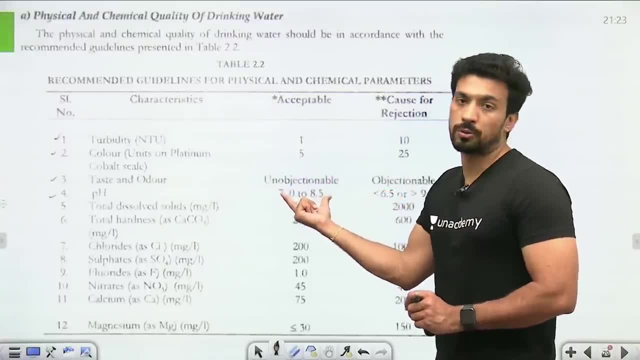 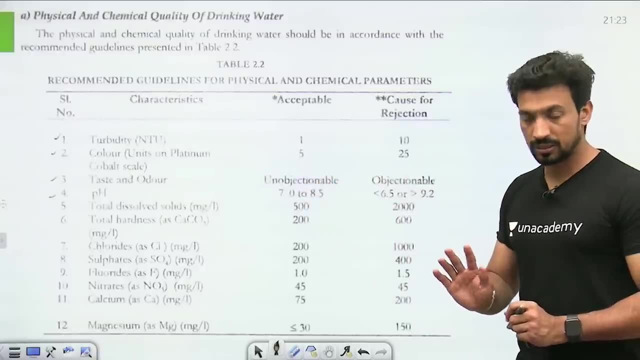 just one value, like in this case. the document of India manual has given us 7 to 8.5.. But if you look at this in IS code then it is between 6.5 to 8.5.. So 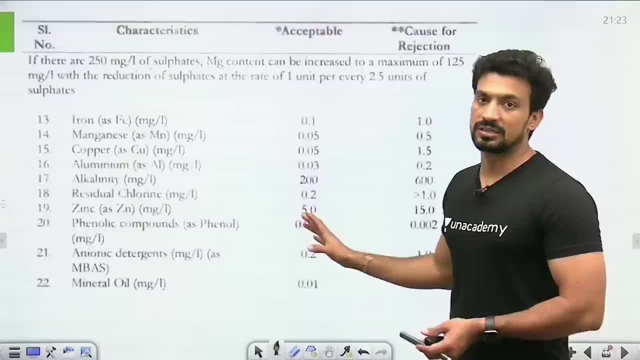 this is just for your reference, that in future, if there is any confusion, then you can refer from here. Now the thing that is to be remembered: it has not come here, So if you talk about physical and chemical quantities, 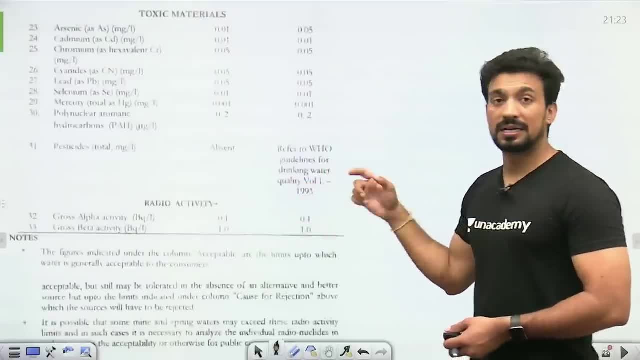 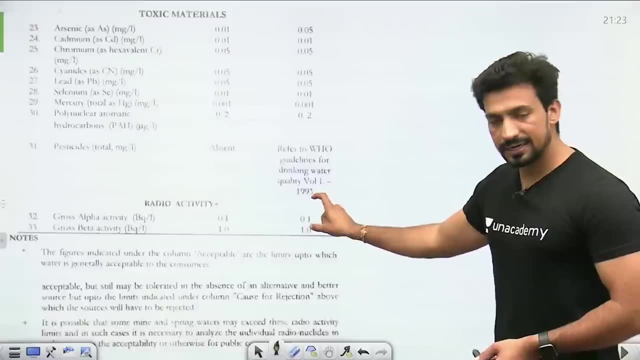 then all the data has been given to you here And after that, if we talk about toxic materials, then it will also be here. If we talk about radioactive materials, then it will also be mentioned here. There have not been any questions related to these. 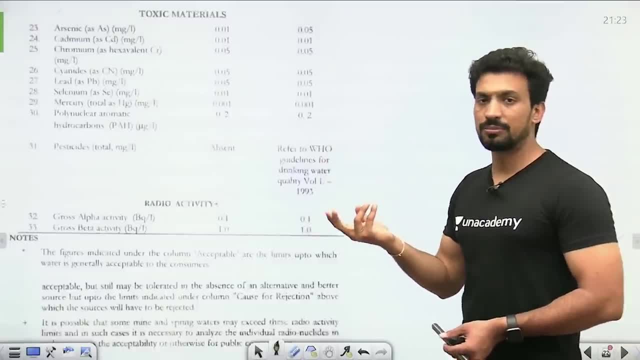 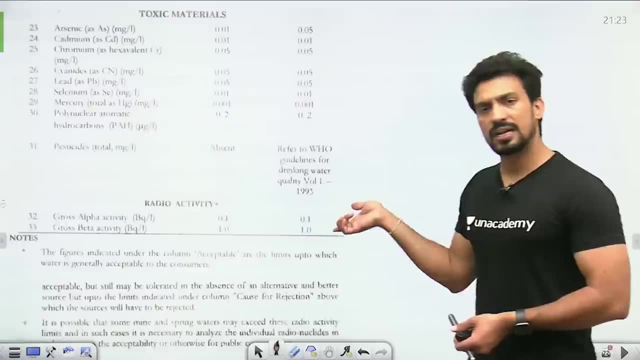 related to radioactive materials. So there are chances that the examiner may think that, yes, now something new should be asked. So if something new is asked, then he asks from such a portion sometimes. So the portions that are seen separately from the individual. 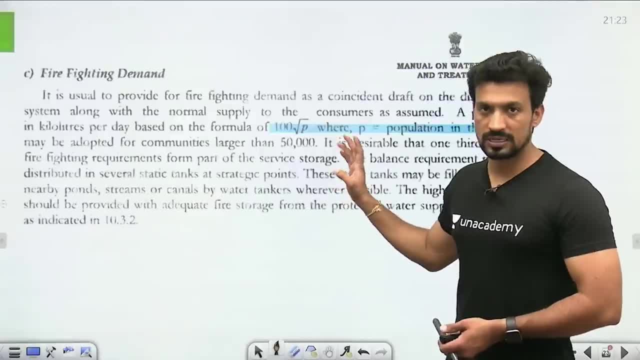 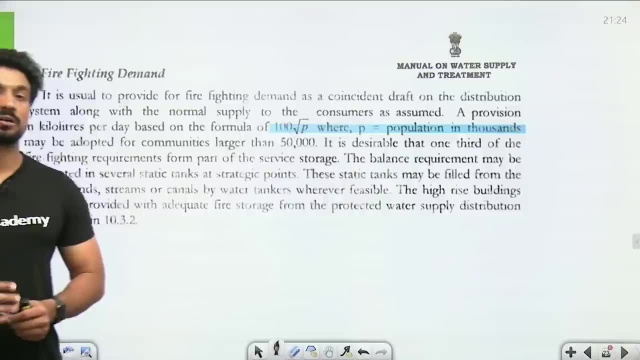 they should also pay a little attention to them. For now, we will go on this according to the code. This is the data of the entire Government of India manual. Another data has been given related to firefighting demand. By the way, 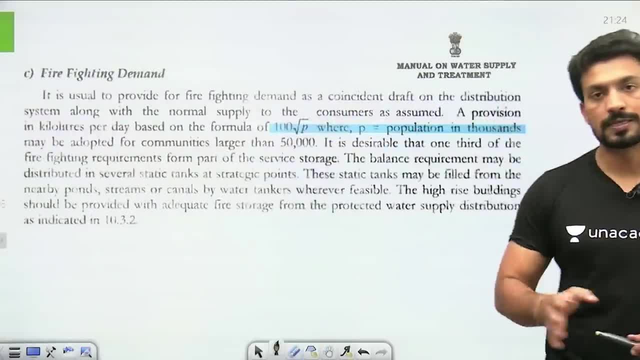 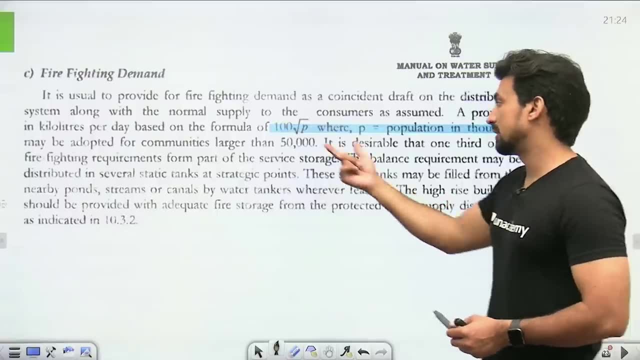 we read Buston's formula, Cushling's formula, Freeman's formula, all these formulas, But if we talk about the entire fighting demand, then the Indian Standard Code tells you the formula related to this, which is 100 root P. 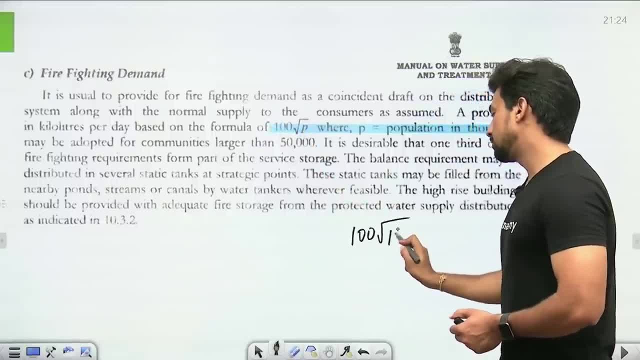 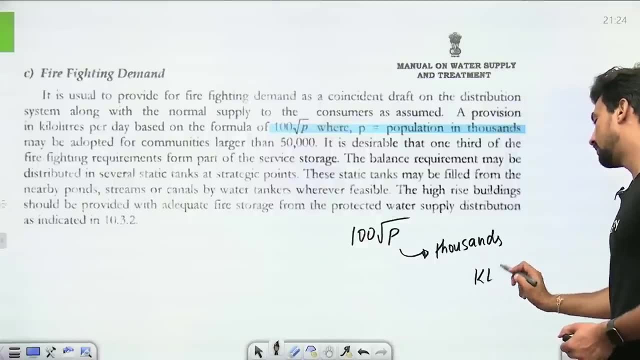 The formula is very simple. The formula is 100 root P. P is your population. This population will be put in the thousands And the answer will come to you. that will come in kilo liters per day. This fire demand will come. 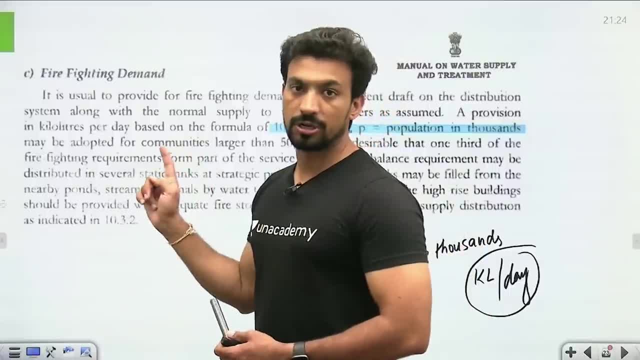 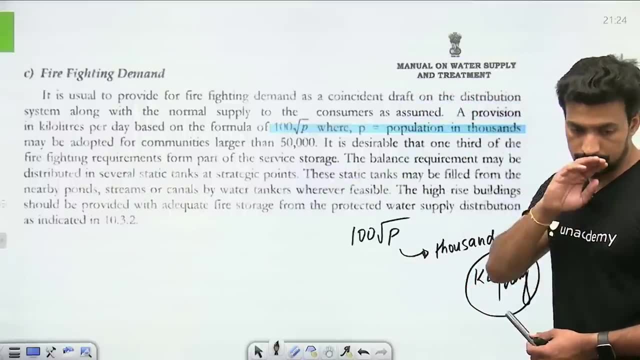 how many kilo liters of water should be obtained per day. So this is what the Government of India manual is telling Clear. Sorry, If you can't see this, then no problem, You don't have to read all these details. 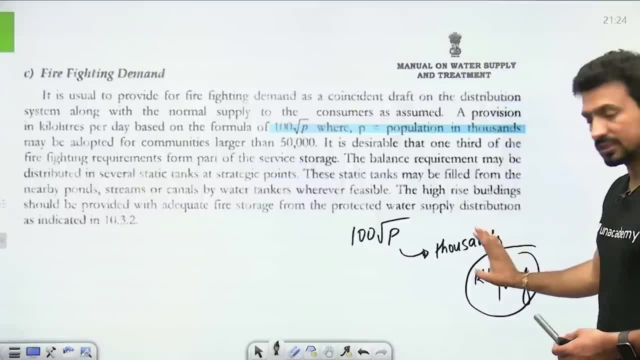 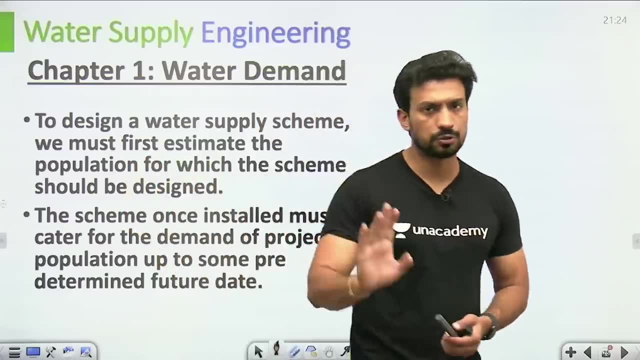 You just have to remember this. The firefighting demand as per the Government of India manual is 100 root P. Then after that the bacteriological guidelines were given. These are mostly the same guidelines which are of the Indian Standard Code. 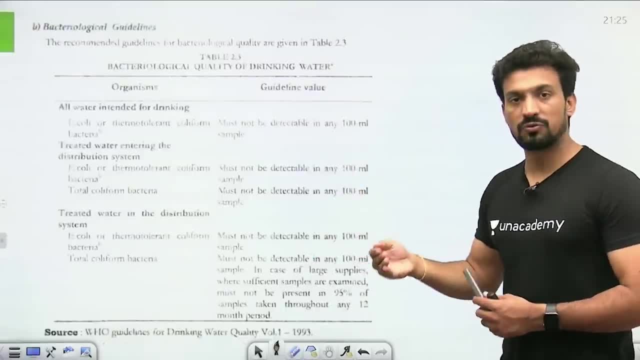 You may not be able to see this data clearly, Because what is given in the manual is the as it is of the manual. This is a screen grab. This screenshot is given to you as it is So, even in the manual. 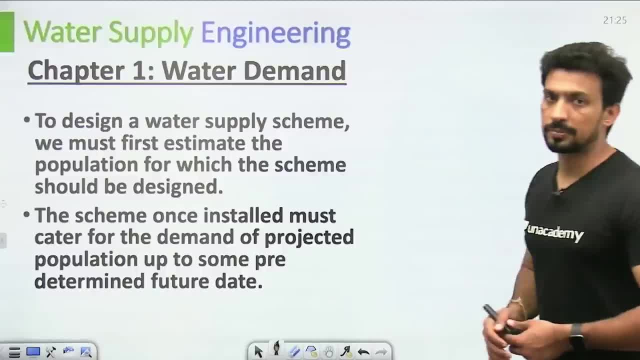 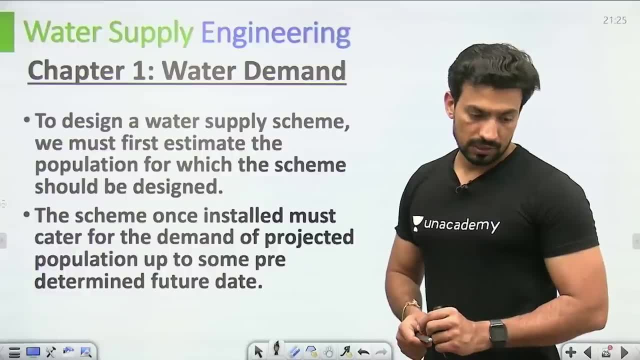 it looks a bit like this, But when you get it in the PDF, then you will be able to read it clearly. Let's start our subject And, wherever you need it, all the data will be given to you In this session. 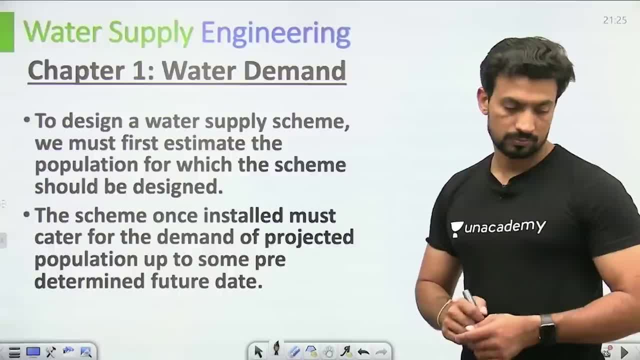 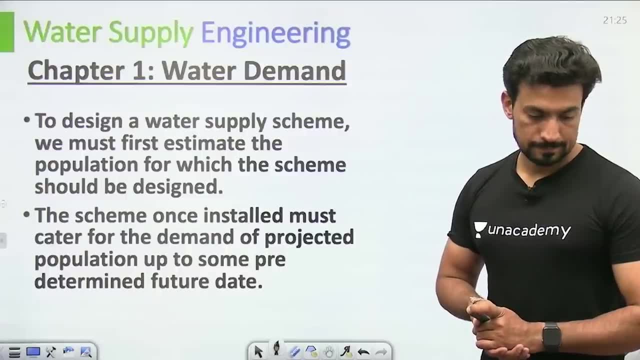 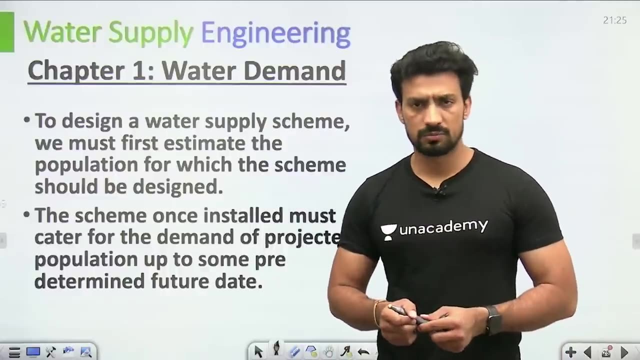 you will get the correct sound. Tell me quickly: can you hear the sound clearly? Can you see the video clearly? All clear? no sound, Ok, perfect, Let's start. This session will be a bit long, So keep patience. 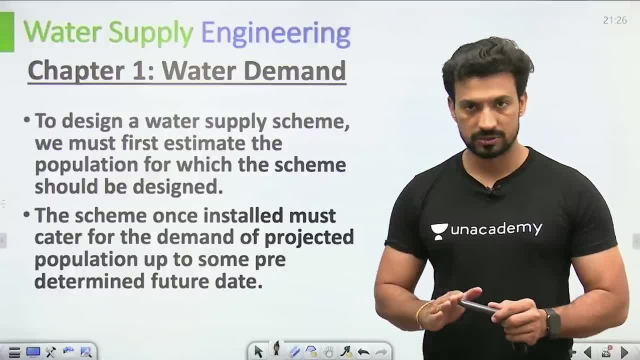 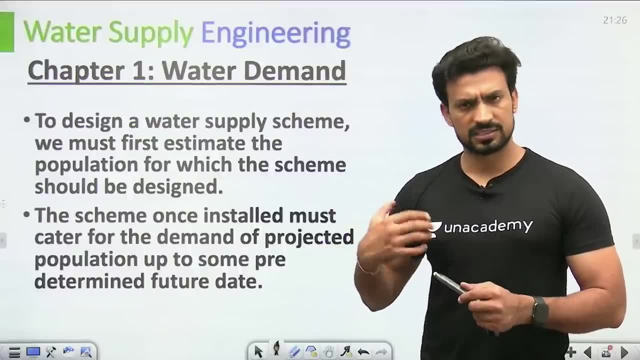 keep courage, keep energy. Close your eyes every 15 seconds so that your eyes get rest. Half an hour, 45 minutes or one hour. then stand up from your seat, walk a little. The class will continue. you have to walk. 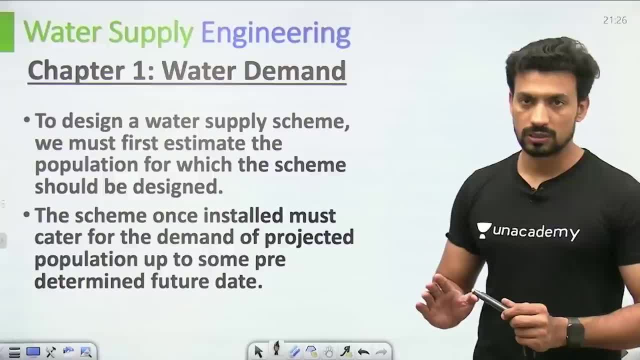 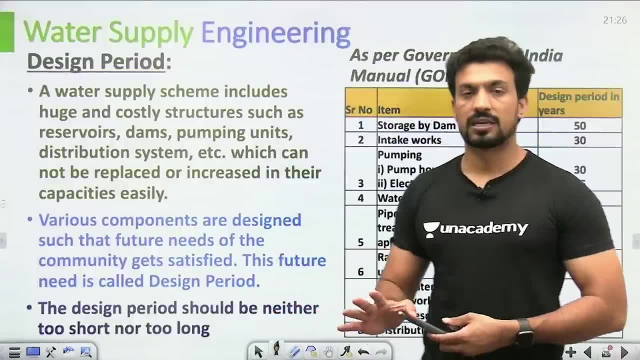 drink water in between, whenever you need it. Let's talk about water demand. Water demand means how much water is required for which particular purpose. In short, water demand comes to you. So first of all, we will find out the water demand. 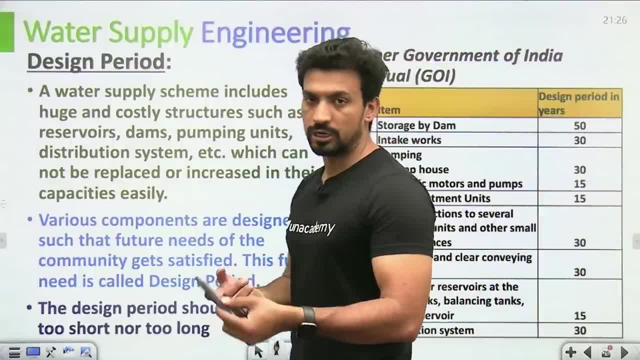 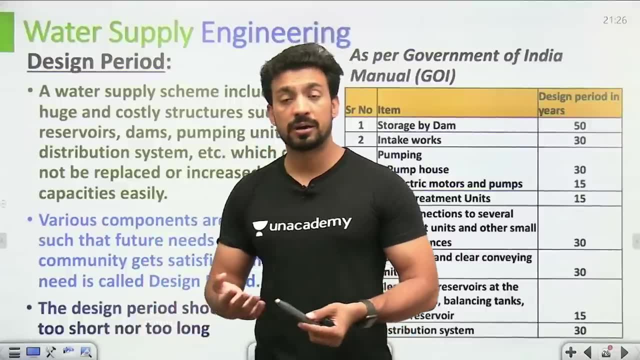 how much water is required if it is for any individual, for domestic purpose. if you need it for industrial purpose, for institutional purpose, for commercial purpose, for fire, demand for what work how much water is required. first of all, 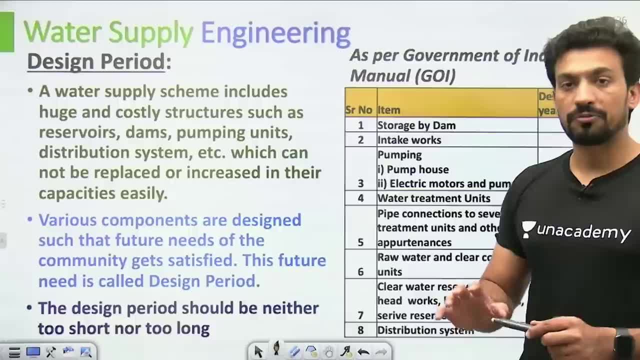 let's find out this And then for that we will find out how many people are required. what is the population? then the project will be designed. how long will it serve people? then we will talk about the design period. 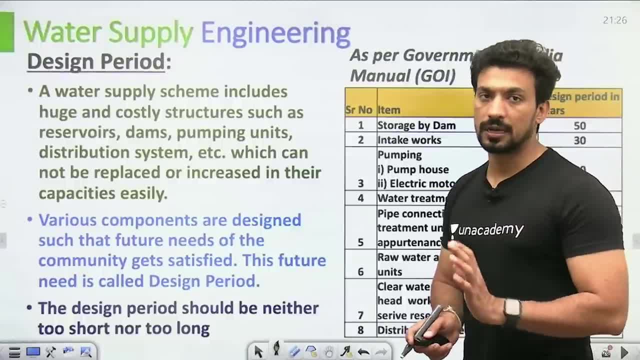 Now the design period, because we are executing such big projects or there is so much investment in the project, then it is not like we made it this year. next year Diwali comes, then we do something new on Diwali. 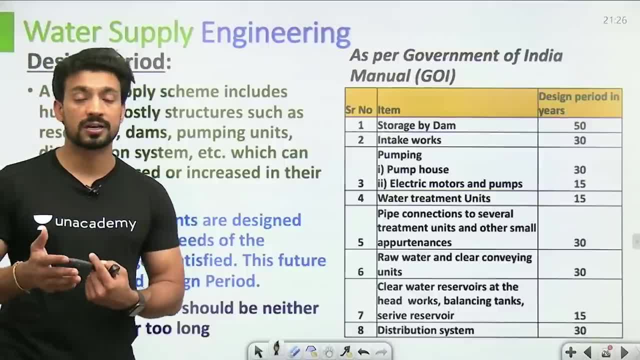 made it again. it will not be possible because a lot of money is spent, a lot of huge investments are made. So we will have to tell the design period. If we talk about the design period, then we will talk about. 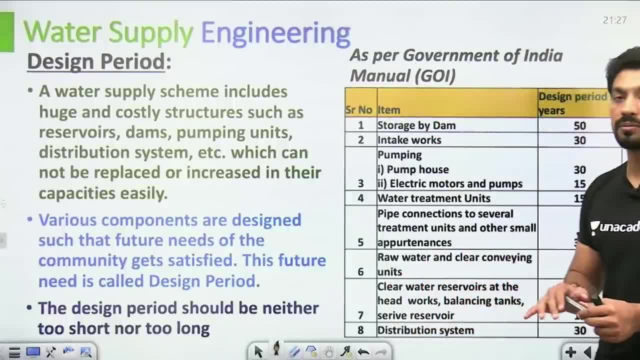 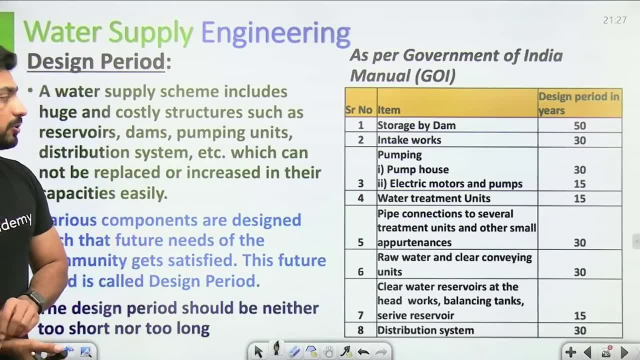 how much water is required. how much water is required. how much water is required. if we talk about the design period for the dams, 50 years are considered. whatever the intake works are, 30 years are left for them in the pumping units. 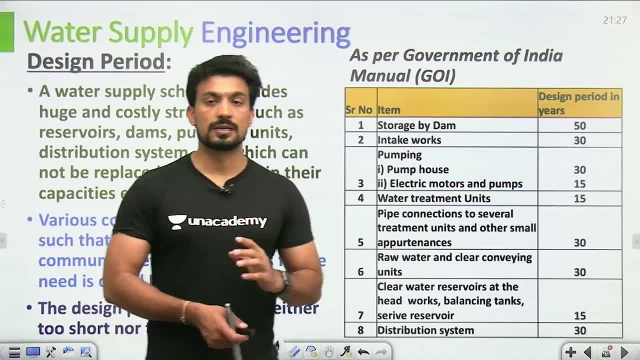 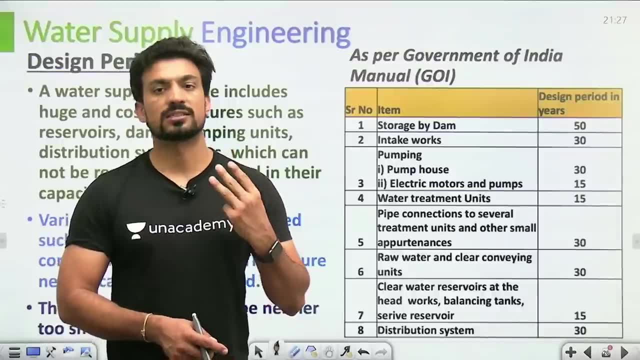 the pump house is 30, and the electric motors are for 15 years. Generally, if you are asked how many decades is the distribution system designed? for 3 decades, or 3 decades, or for 30 years it is designed. 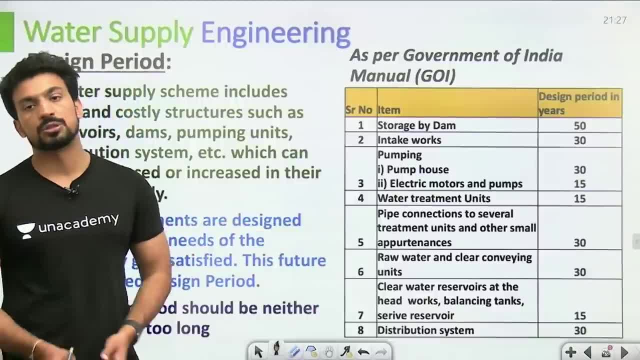 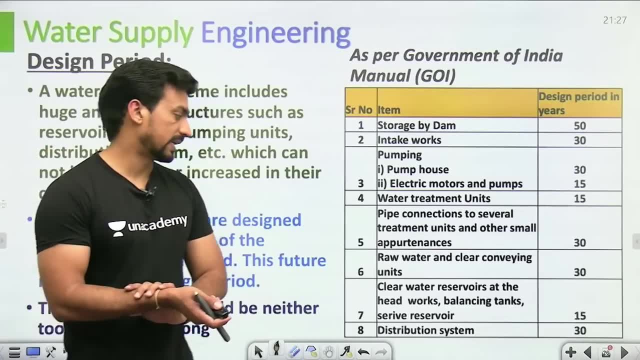 This kind of question is asked from you here. If we talk about pipe connections, then for 30 years the units that convey raw water or clear water units are there. They will be designed for 30 years- Clear water reservoirs or tanks. 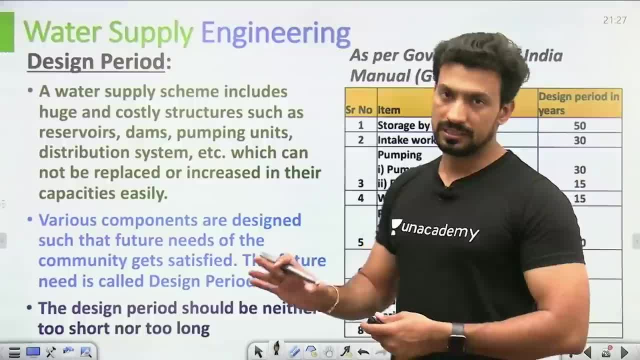 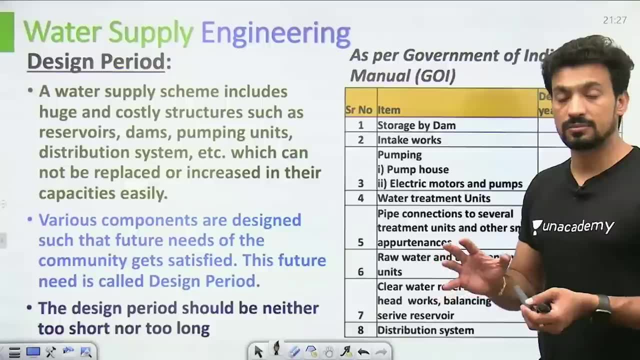 will be designed for 15 years. This period should not be so small that we have to do construction again and again. All these water supply schemes should not be so big that we will go later and invest so much money here today and tomorrow we will not be able. 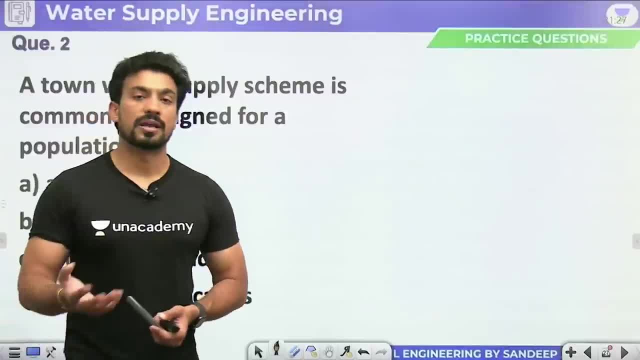 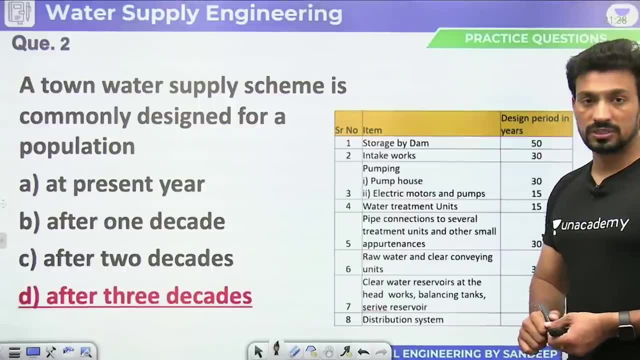 to refine it or bring changes in it as per the requirements. So there should be an optimum time. A town water supply scheme is commonly designed for a population, for a population. For how long do we design a population? The day when your construction? 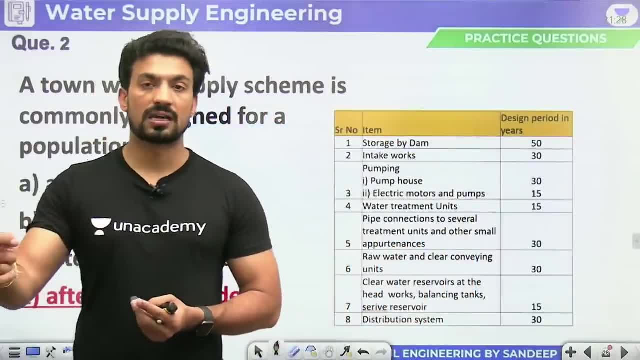 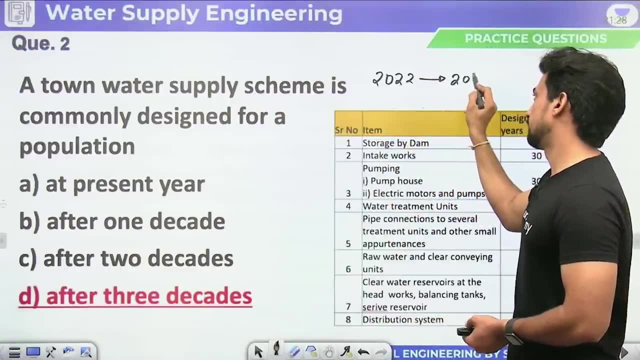 will be completed. the project will be completed from that day to 30 years. If it is currently 2022 and your project will be completed by 2025, then in 2025, when it starts to serve. from then you will add. 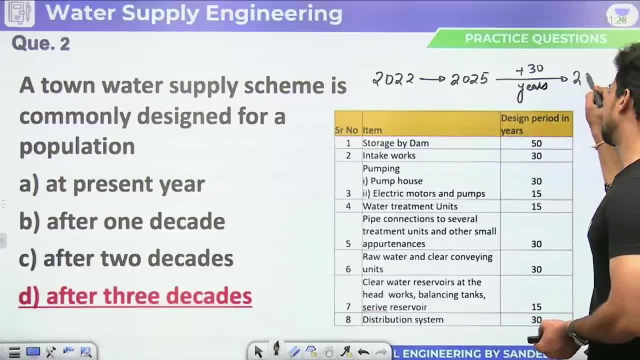 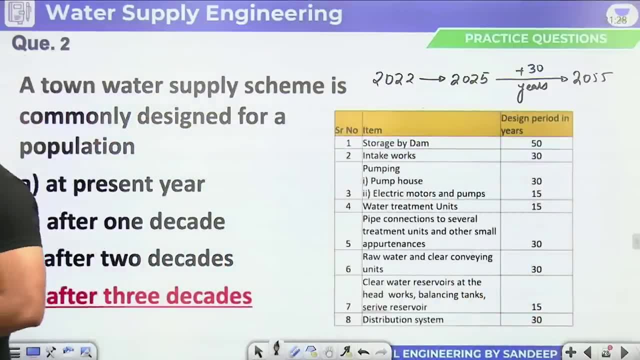 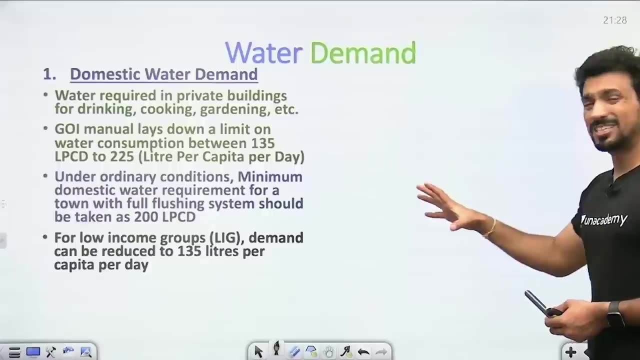 30 years in it. So if you add 30 years from then, it should serve up to 3 decades. Next, if we talk about domestic water supply, then domestic water supply is the water requirement that we need for our household work. 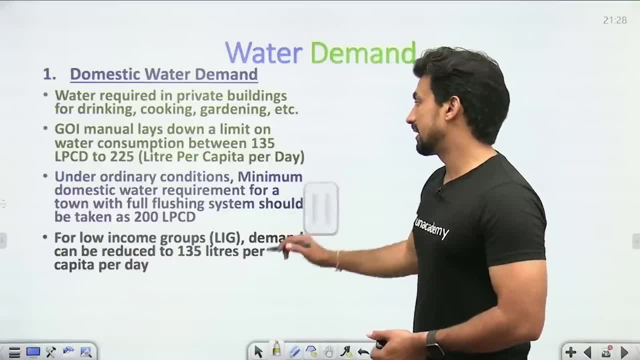 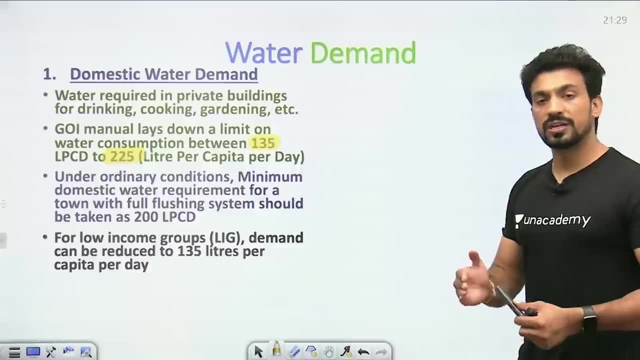 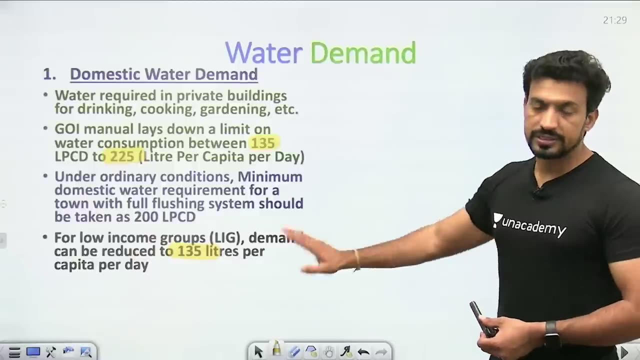 For this. if we talk about the Government of India, manual tells you that this value can be from 135 to 225.. If we talk about lower income groups, then it goes up to 235 liters per capita per day. These values have to be. 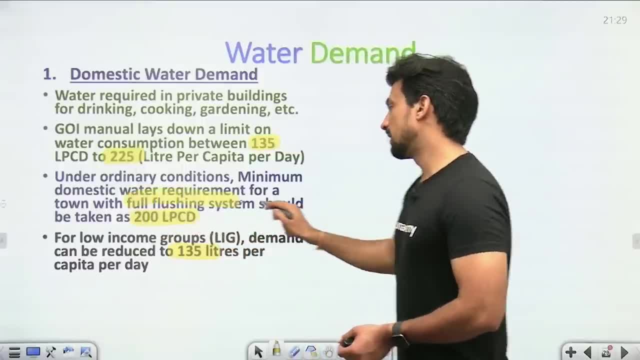 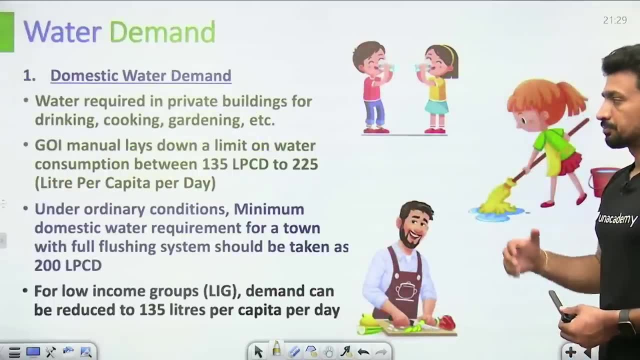 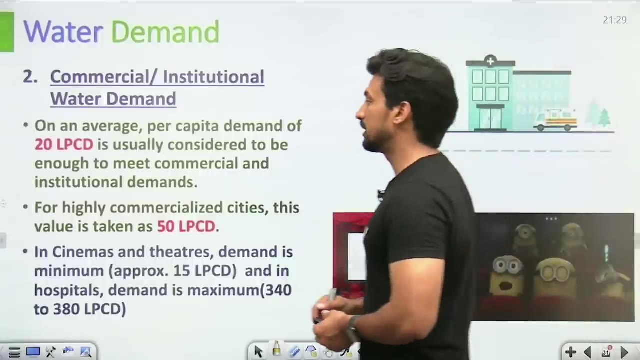 remembered Under ordinary condition minimum domestic water requirement for a town with full flushing system. If there is a full flushing system there, then 200 liters per capita per day. So water required in private buildings. these values we have already discussed for commercial. 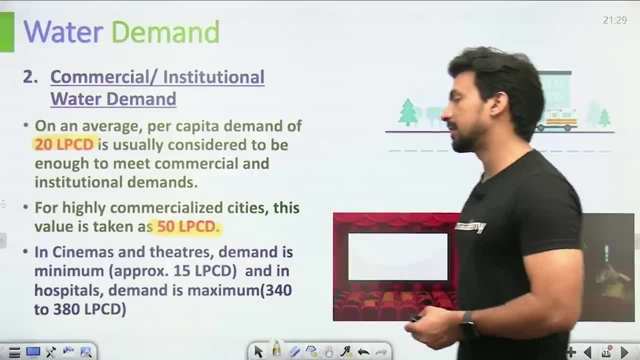 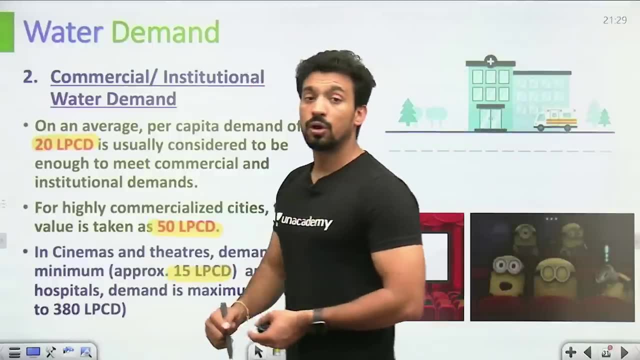 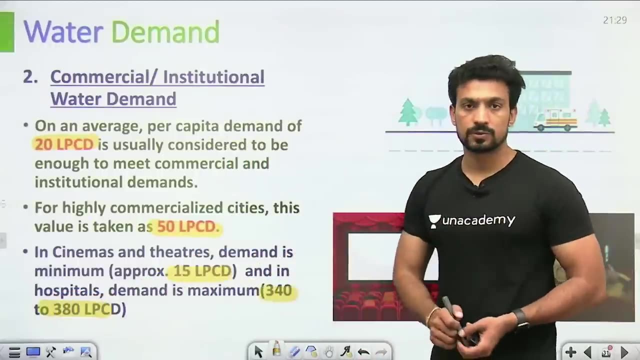 and institutional demand. If it is a very commercialized city, then 50 liters per capita per day can be considered. In cinemas and theatres this value is 15 liters per capita per day, And in hospitals this value can go from 350 to. 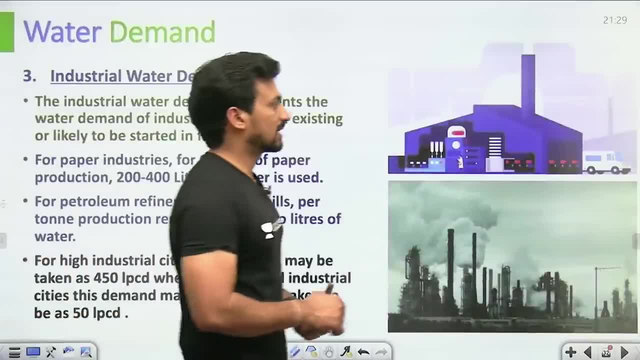 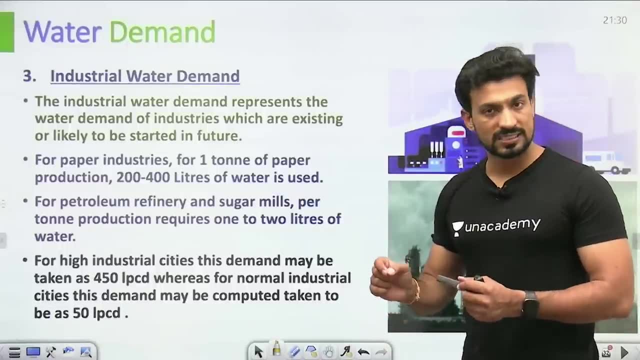 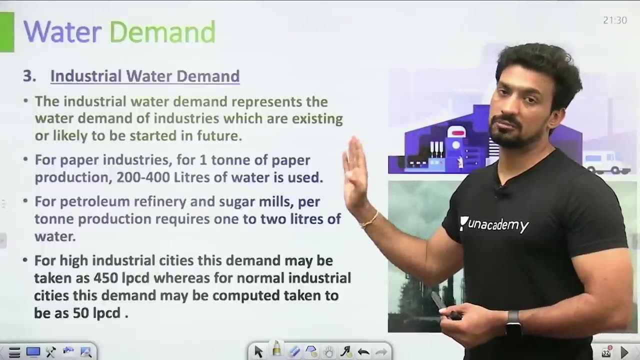 380 liters per capita per day. So, for all these purposes, industrial water demand is the highest for any city. If any water supply scheme has to be designed, then the biggest influence it will create will be the industrial water demand of that city. 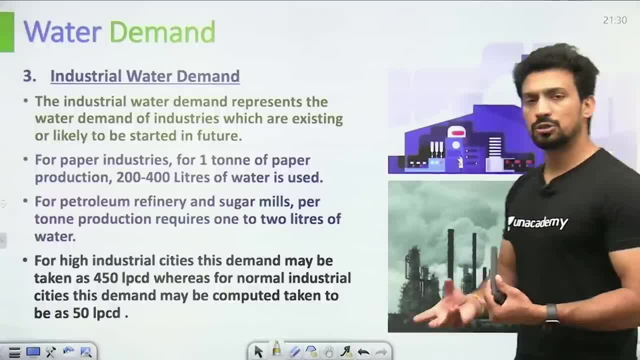 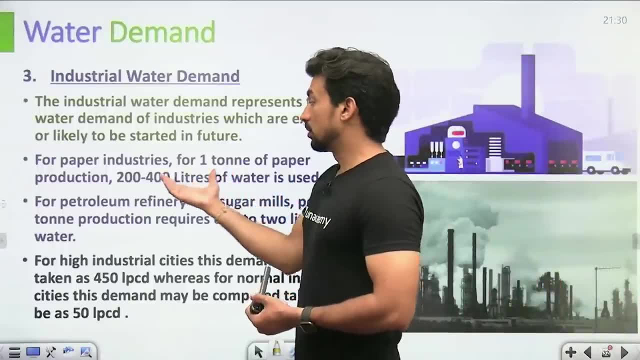 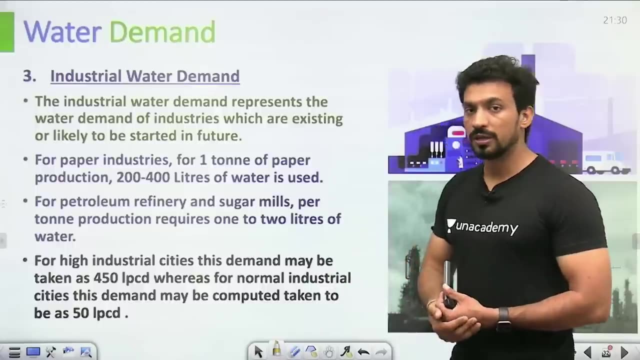 You have to remember this. So industrial water demand represents the water demand of industries which are existing or likely to be in demand for the next 10 years. If we talk about petroleum industries, it will be very less If we talk about the whole day. 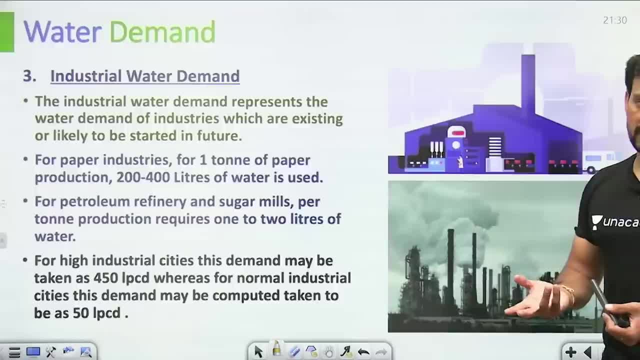 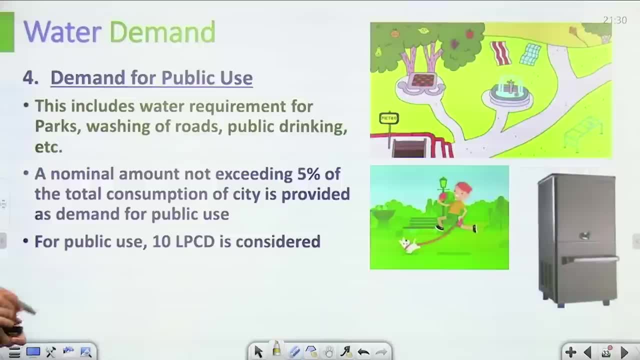 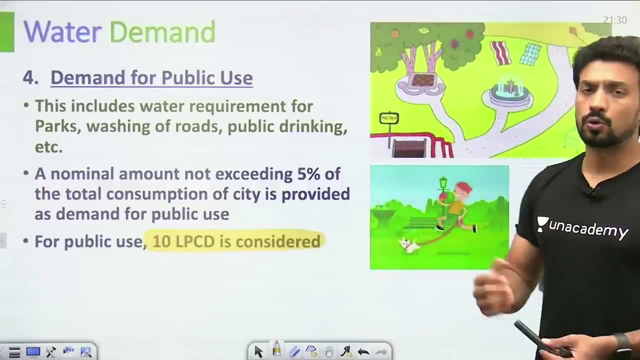 we will need around 1 kilo liters of water in petroleum refinery units. For high industrial cities it depends on the industries and the city. Then for public use, 10 liters per capita per day is required. All these are 10 liters. 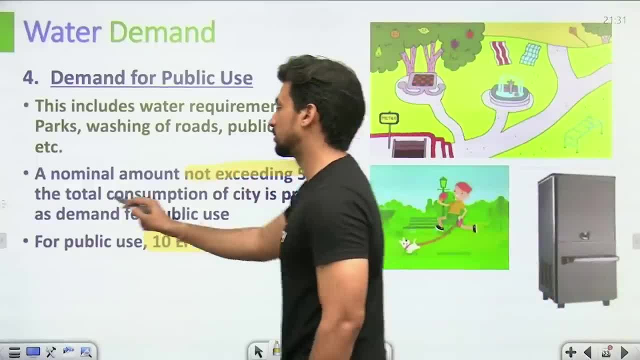 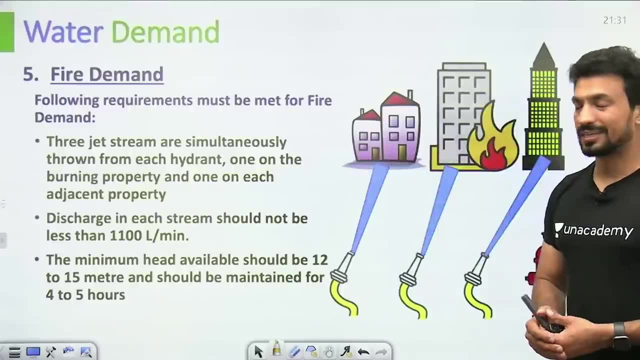 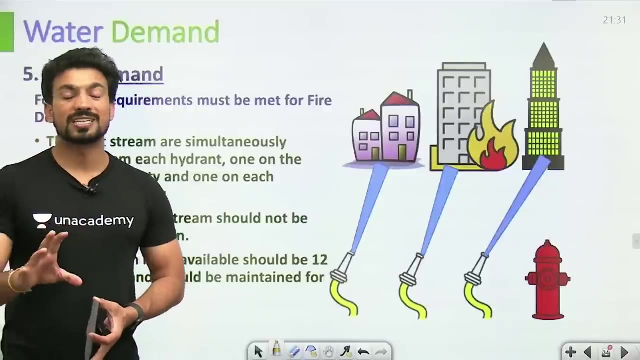 per capita per day. Nominal amount not exceeding 5% of the total consumption. Don't exceed more than 5%. Next, let's talk about fire demand Wherever there is a fire, if there is a fire in a building. 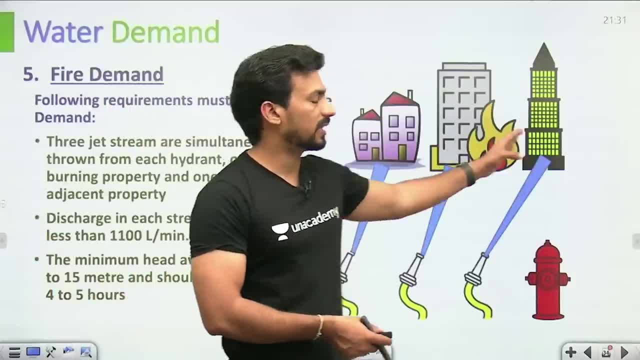 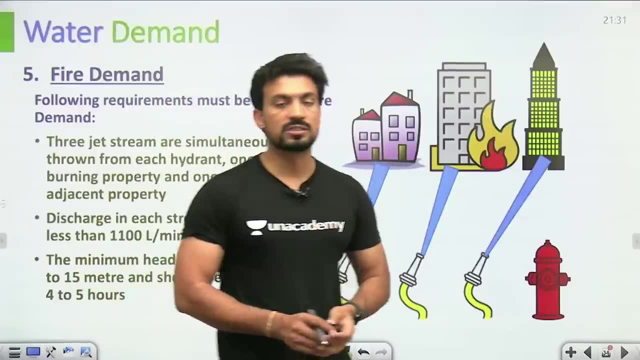 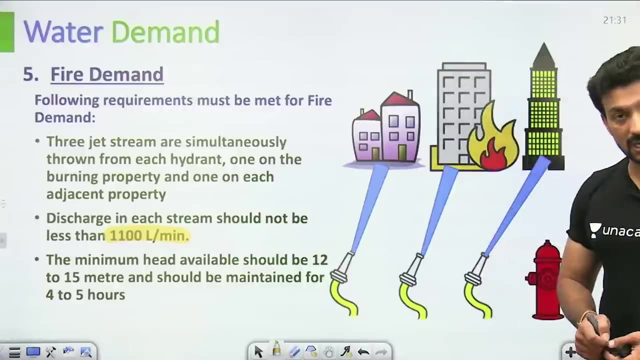 then in that case you have to put out the fire of that building. If the temperature does not increase, then there is no chance of fire. That's why we will throw three streams, and each stream should have at least 1100 liters per minute. 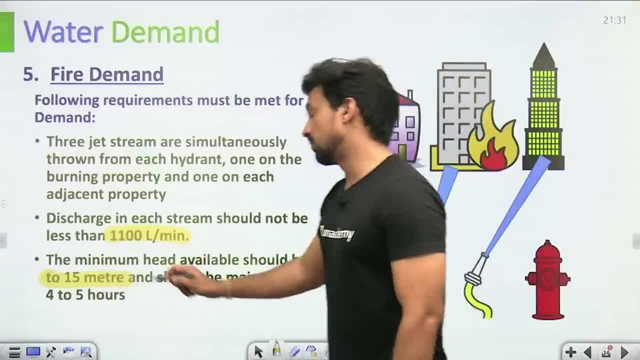 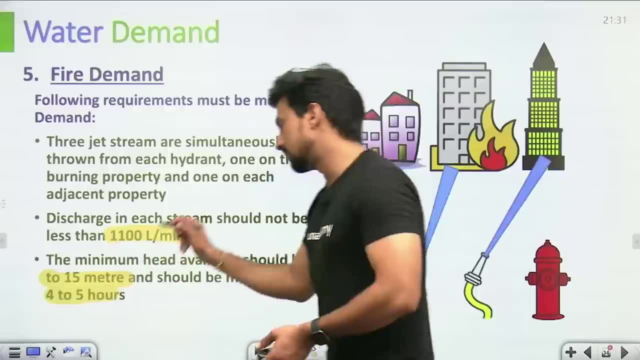 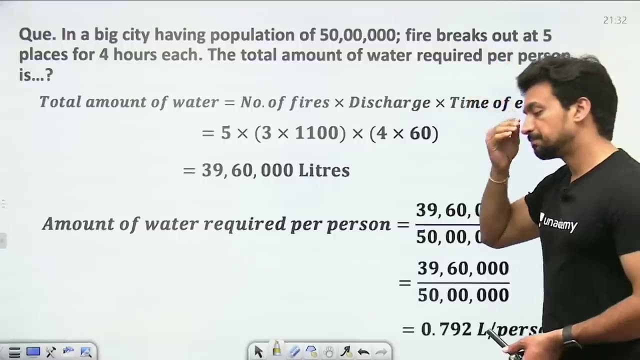 of discharge. The head that should be available should be 12 to 15 meters of water, potential, energy or head, and it should be 1100 liters of water per minute. Then the next question. we had seen this question in a class as well. 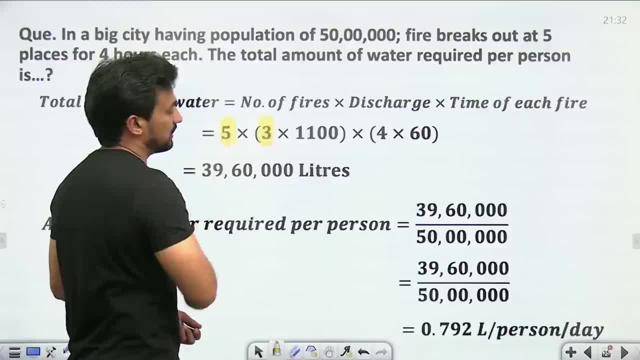 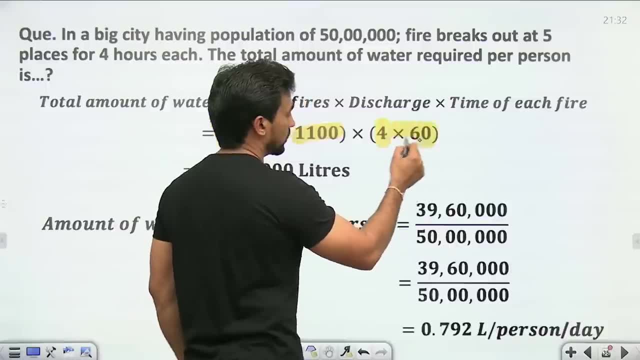 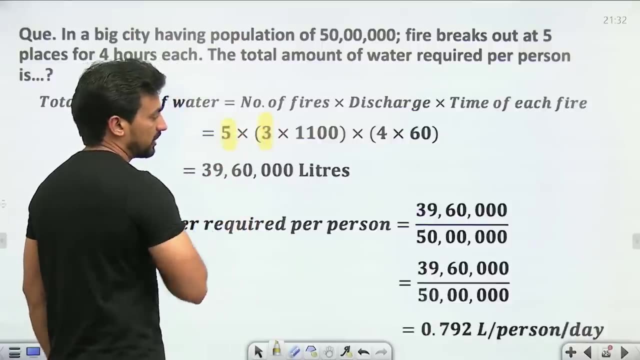 What was this question? If there is a fire, how many places does it take? 5 places takes 4 hours. So there was a fire at 5 places. there were 3 streams everywhere for every stream. you need at least. 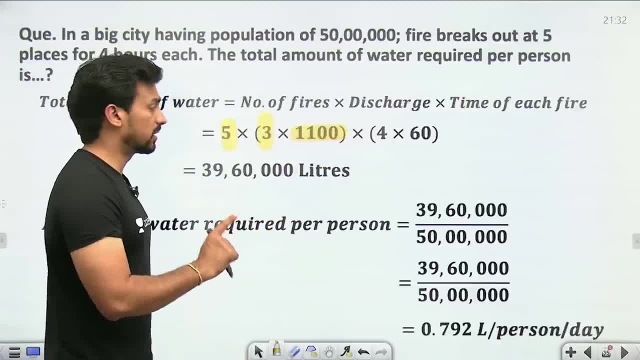 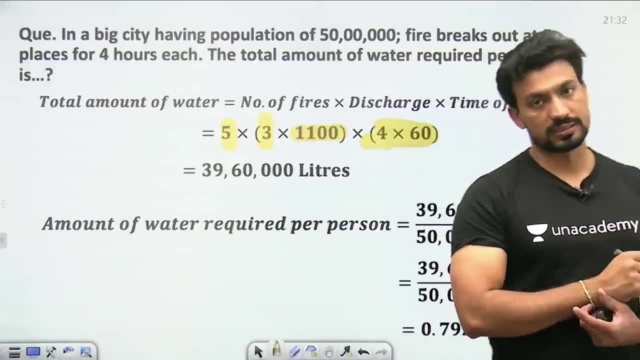 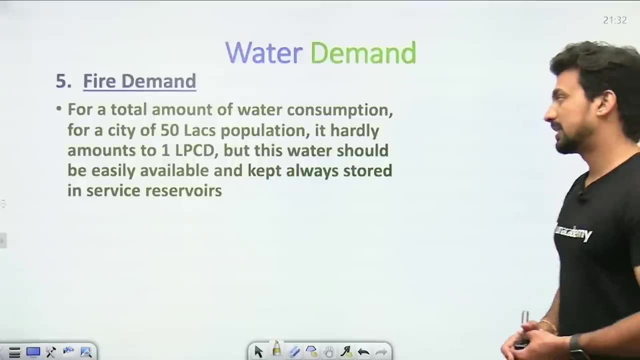 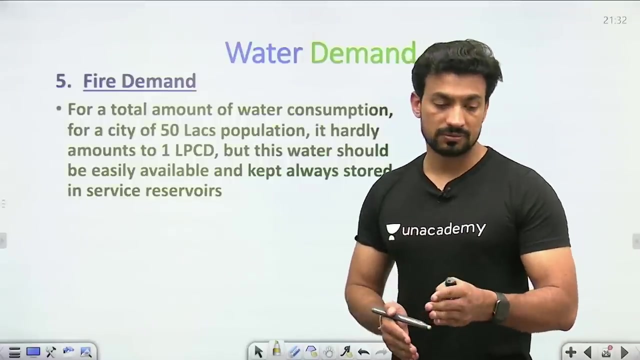 1100 liters of discharge per stream. For how long? For 4 into 60 minutes. So from here you will get the total amount of water. If we want to check per person, we have divided it from the population. Next question: 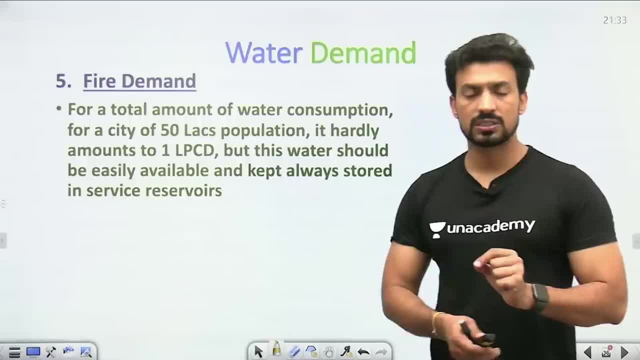 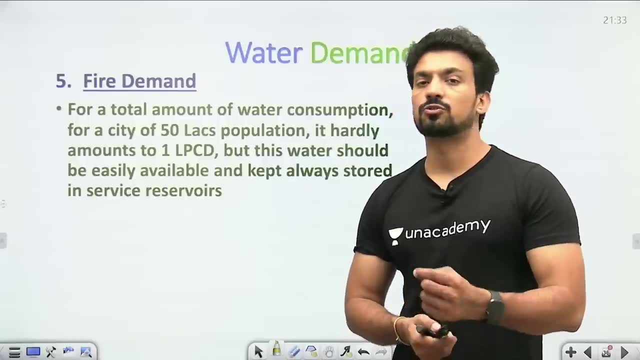 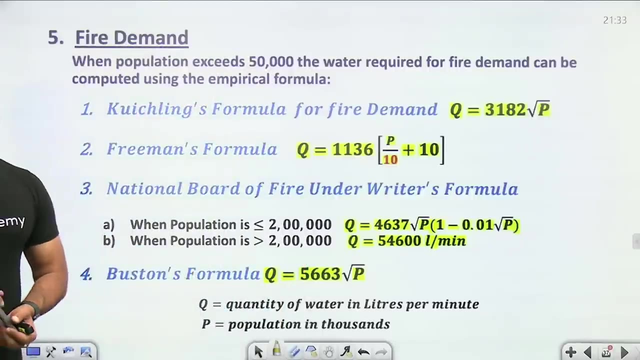 is, if we talk about overall city and take an average, then it may be less than 1 liter per capita, but if there is a need for a place where there is a fire, then we will need a lot of water Now for this. 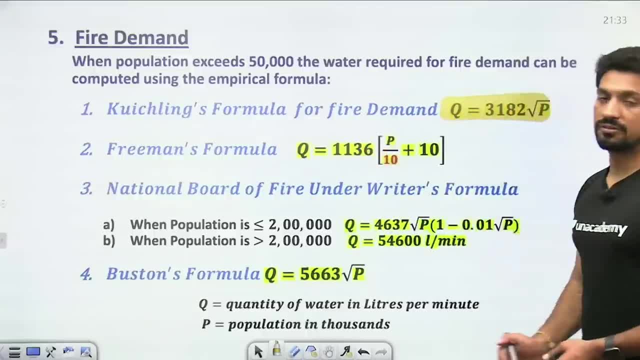 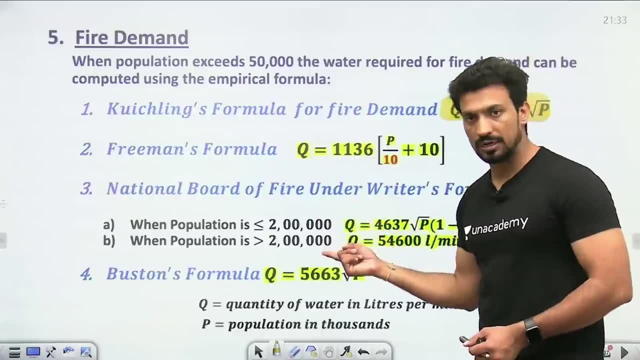 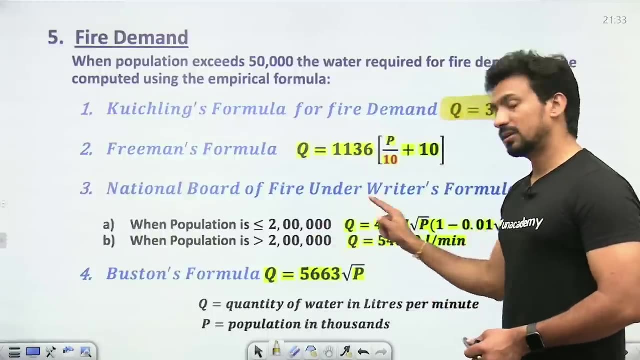 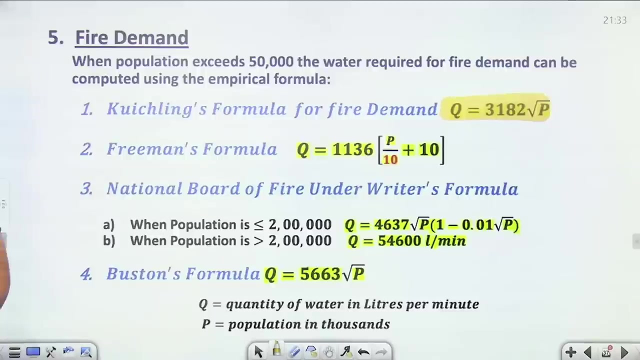 we have a formula: 1136p by 10 plus 10.. National Board of Fire Underwriters formula: if the population is less than 2 lakhs, then 4, 6, 3, 7 root p: 1 minus 0.01 root. 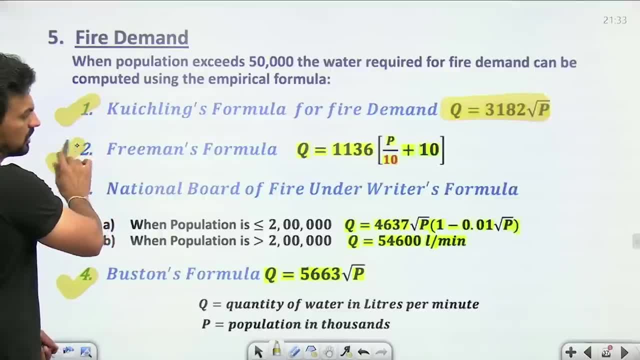 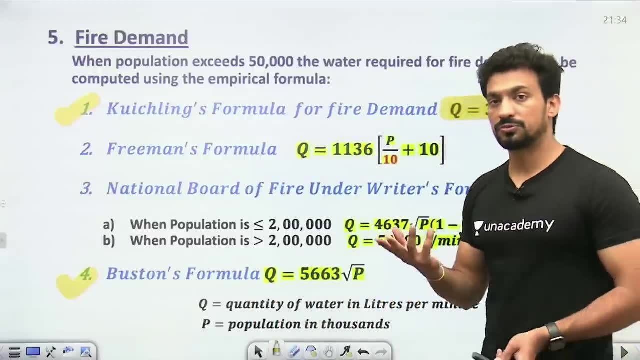 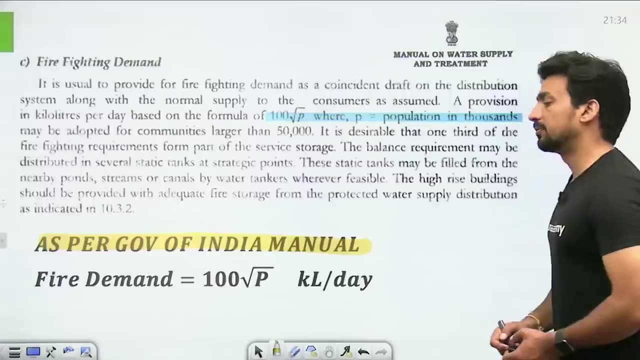 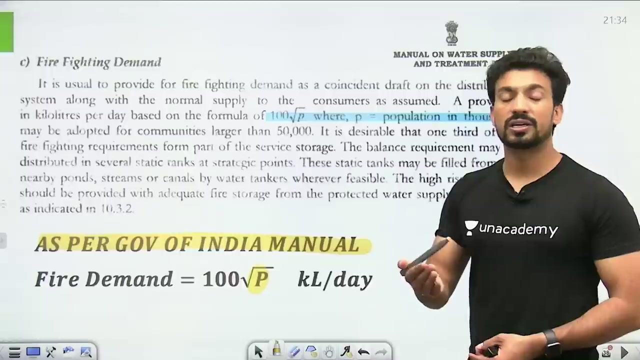 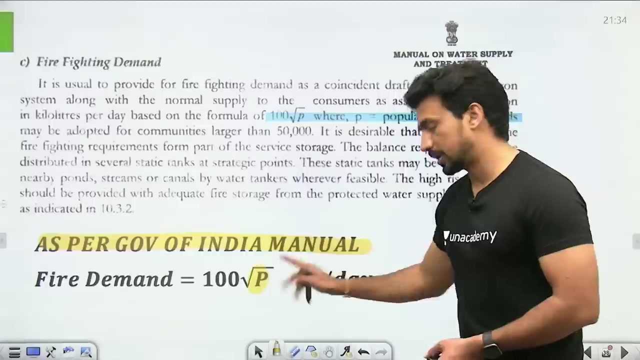 p. if the population is less than 1 lakh, then you have to calculate it according to the government of India. manual fire demand 100 root p, in which p will be put in kilo litre per day. the answer will come in kilo litre per day. 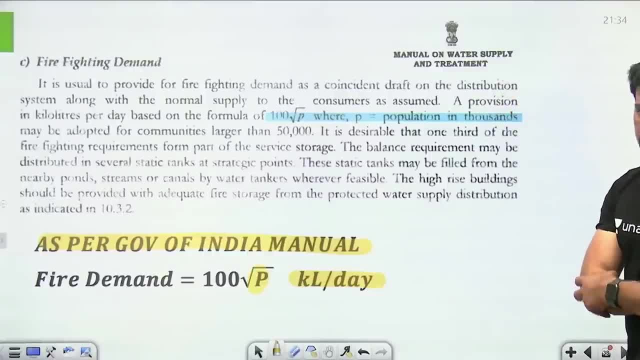 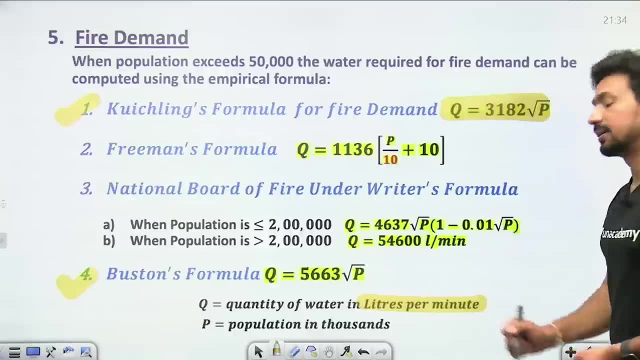 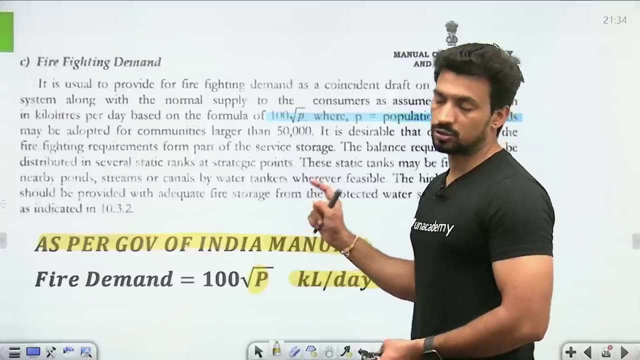 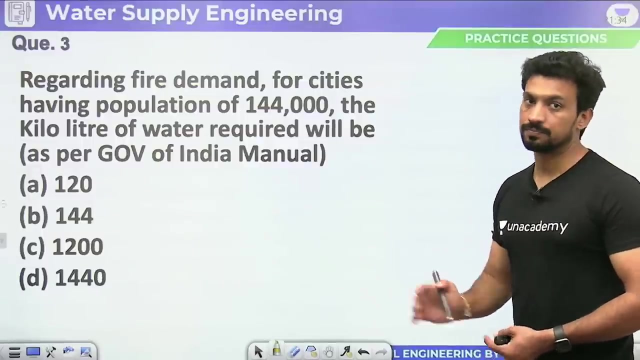 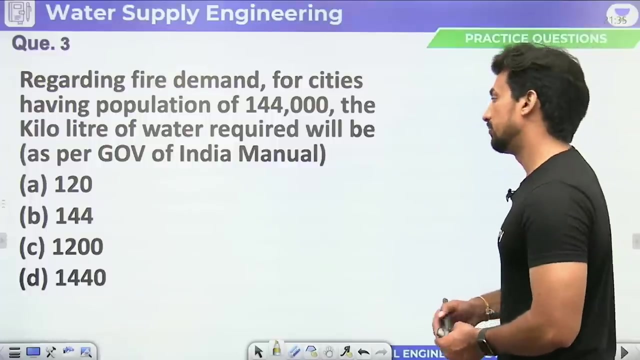 the answer will come in kilo litre per day. if we talk about the previous discharges, which come in liters per minute. these all values are in liters per minute. if the population is less than 1 lakh, then we have to calculate the fire demand for cities. 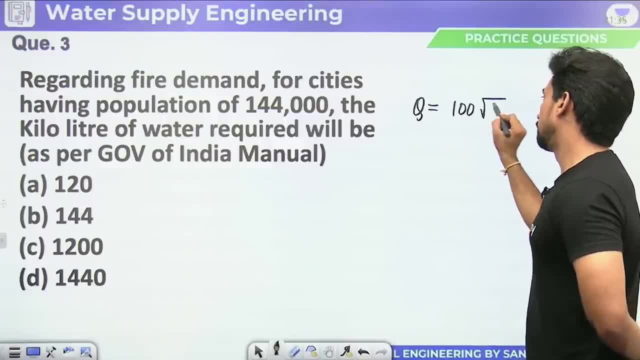 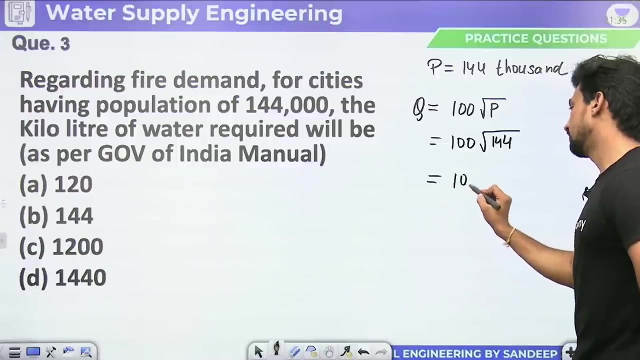 having population 144,000, the kilo litre of water required will be, according to the government of India, that is 100 into 12, 1200 kilo liters per day. so the answer will be 100 into 12, 1200 kilo. 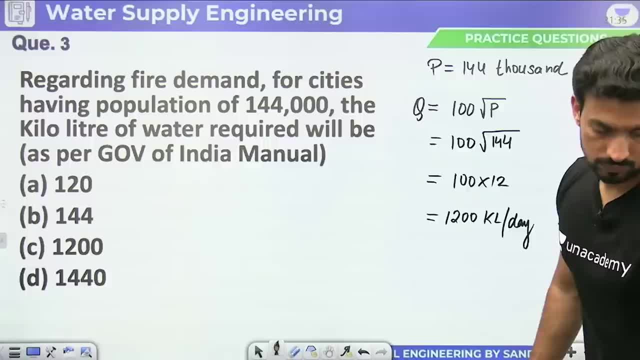 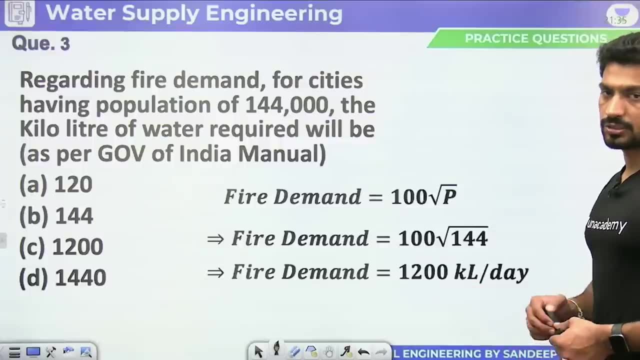 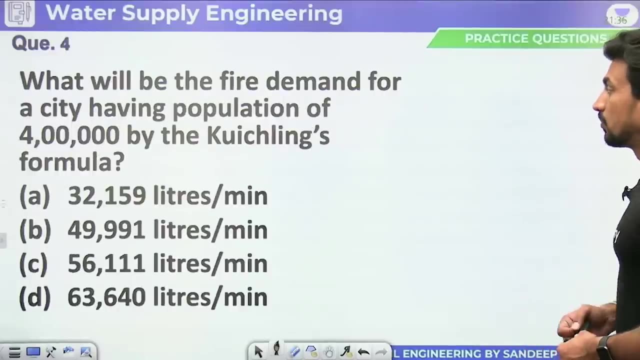 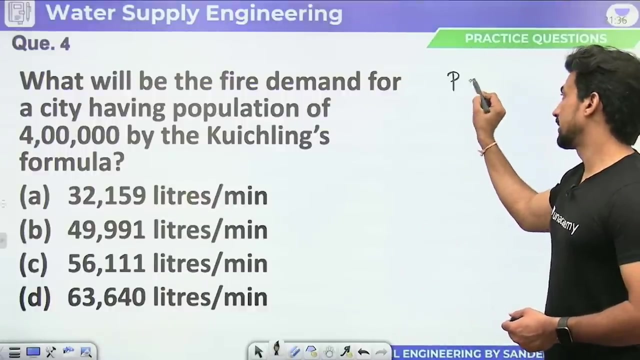 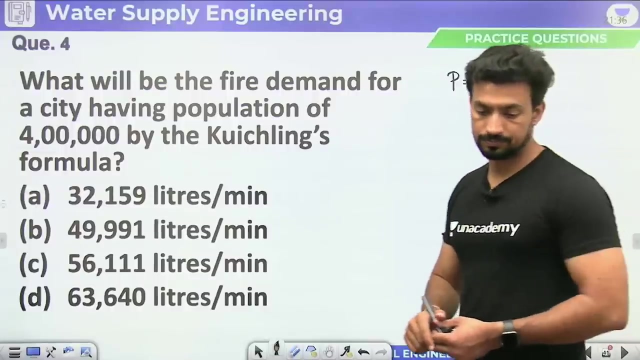 liters per day. so the answer will be 100. so what is the fire demand for a city having a population of 400,000? so what is the population value in a city in thousands? so you have to put 400 according to kushlings formula. 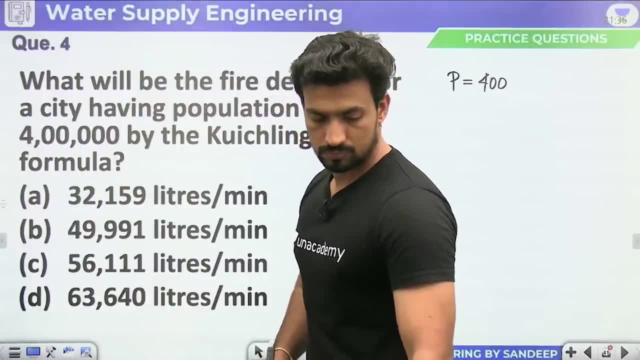 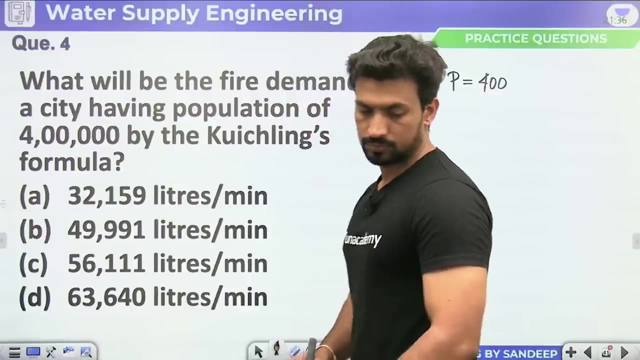 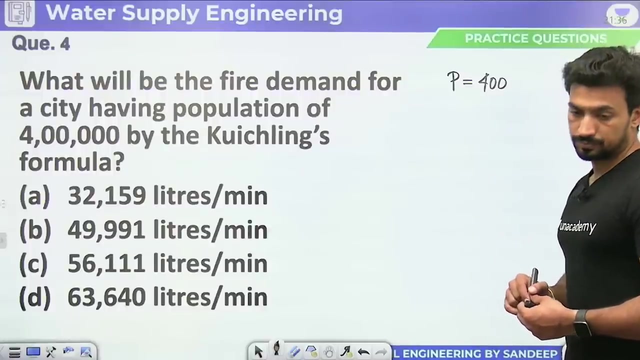 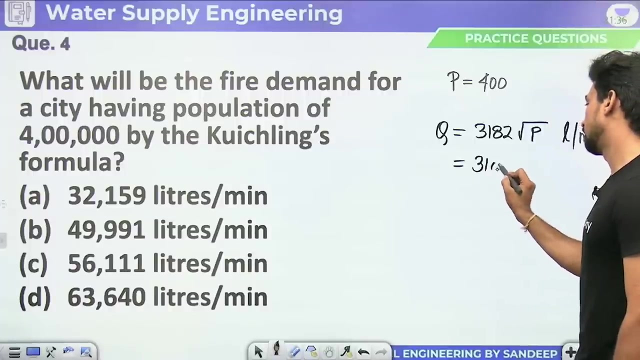 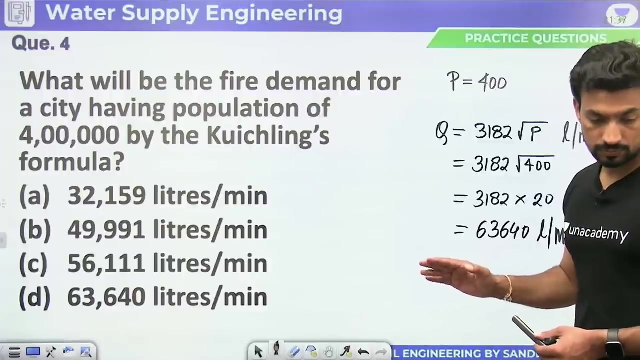 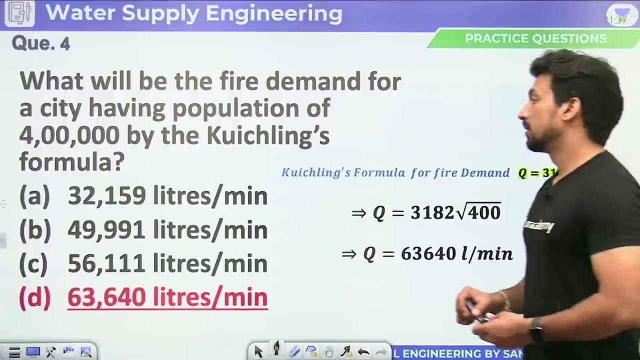 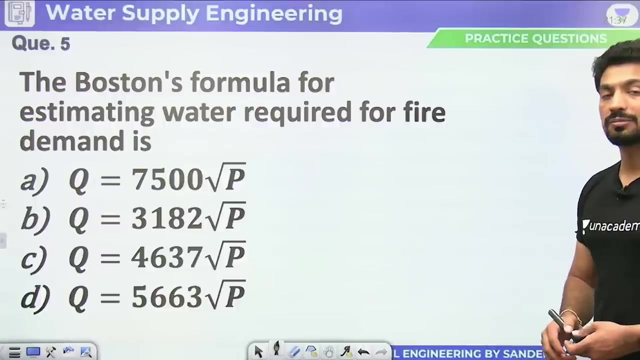 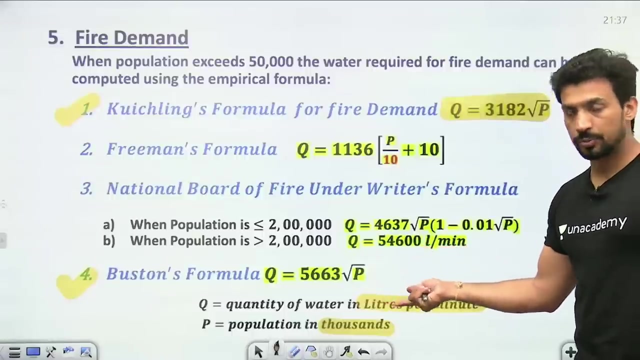 so if, Thank you, This will come in liters per minute: 63640. Next, the Bustons formula for estimating water required for fire demand is 5663 root p, First formula and last formula. from objective point of view, It is easy to ask in exam. 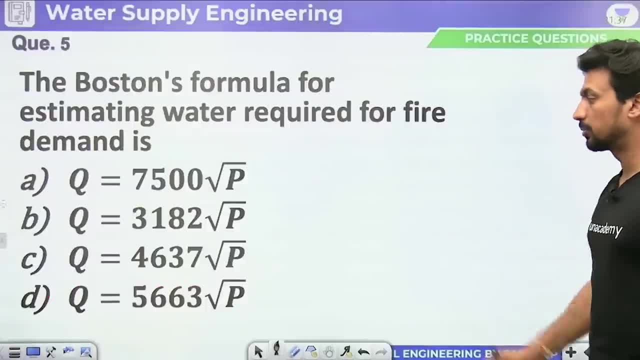 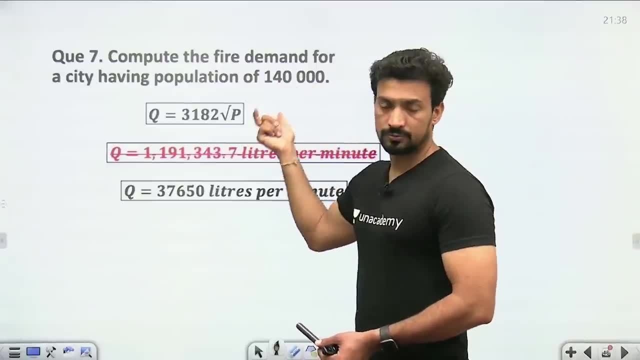 So you can ask. Ask according to Government of India manual, So you should know that too. Next, let's move ahead. Mistakes are here and there. If we put all the data as it is, Put 140,000 instead of it. 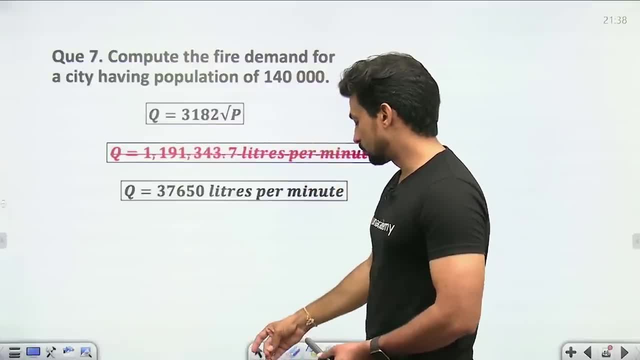 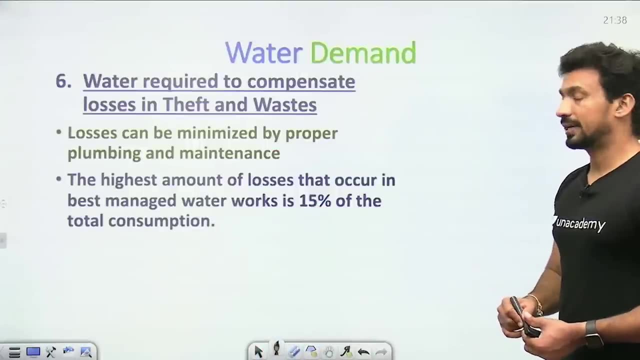 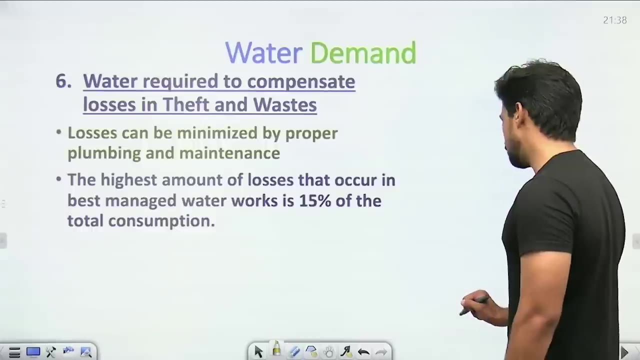 If the value given in the question is not written in thousands, You have to express it in thousands. Next, water required to compensate losses in thefts and wastes. How much water is considered in loss or thefts? You can consider that the water is stolen or the water is lost. 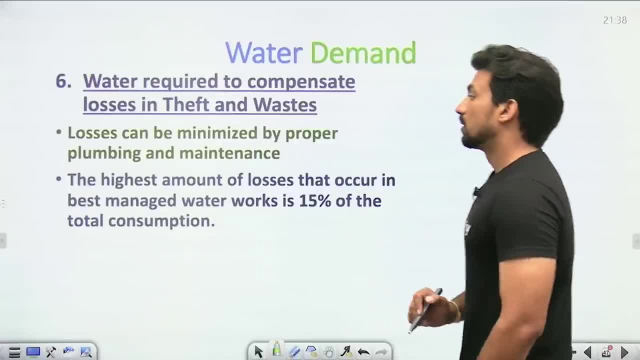 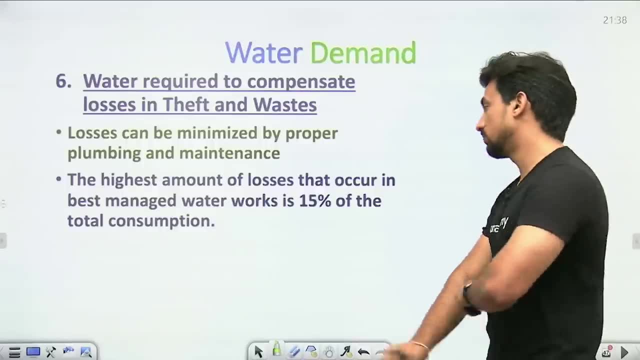 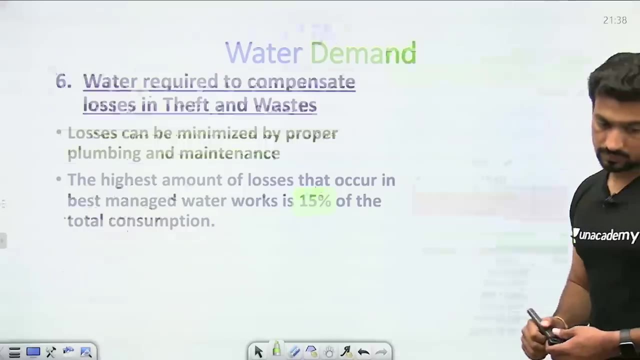 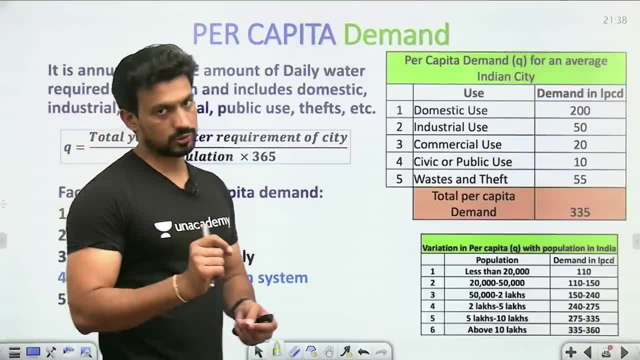 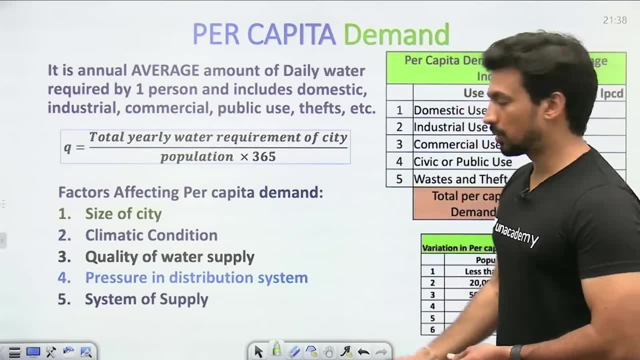 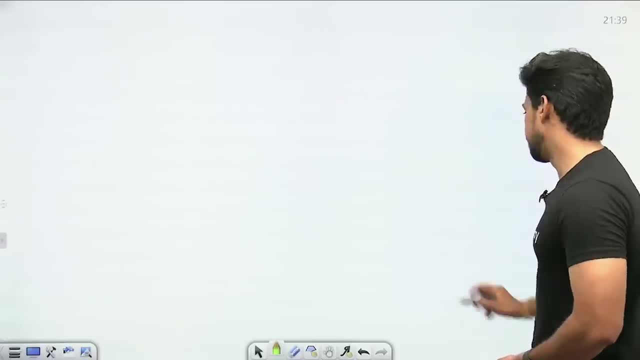 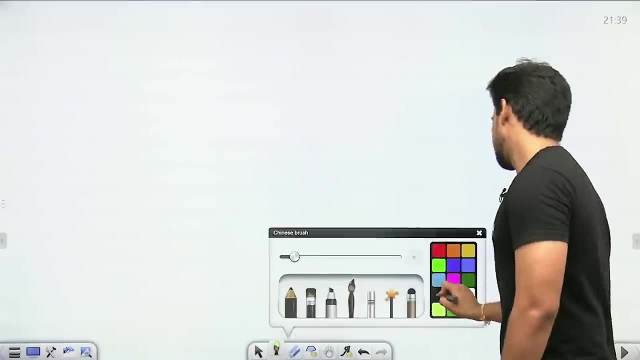 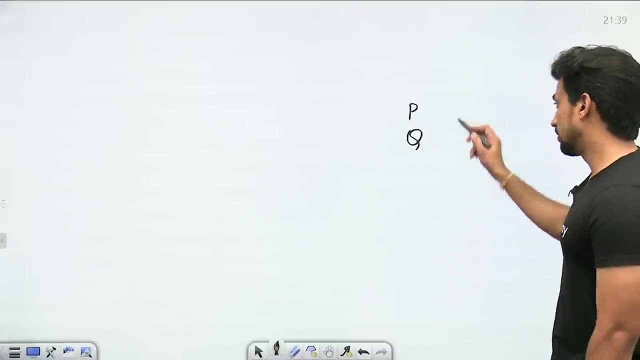 In some city the population is P. In some city the population is P, Capital Q. total water is being used there. So what will be the average demand? So what will we say to calculate the average demand? What we will say to calculate the average demand. 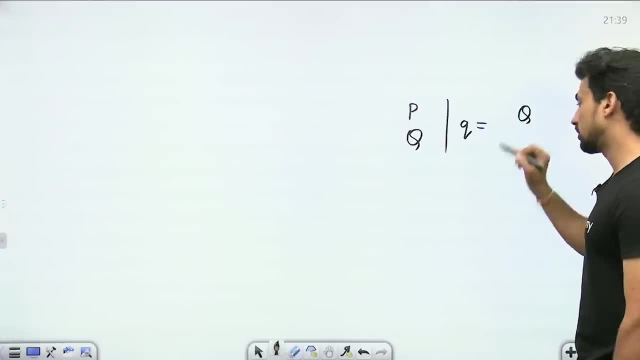 So what we will say here is that how much water was used in total whole year, Why water was utilized in the whole year, How many people utilized. People used P. We put Q by P, So how much total water was used in the whole year in that city? 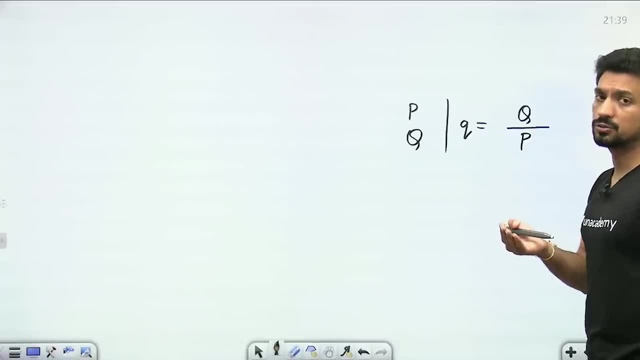 Divided by population, So how much water was used in the whole year for one person. If I divide this again from 365, then this will tell us that how much water was used per day. So a simple object like this. Please stay tuned. 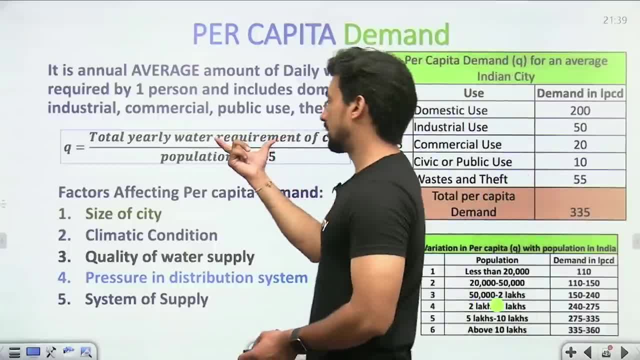 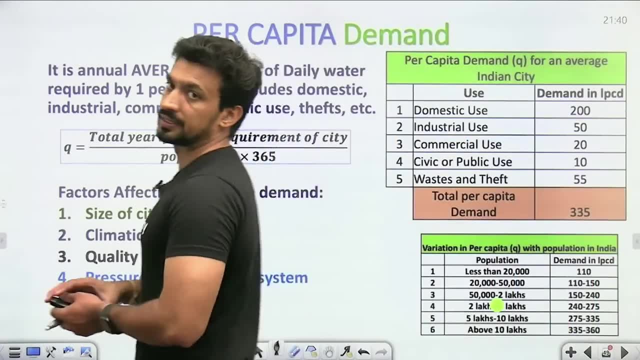 So I asked such a simple, objective question that total yearly water requirement of city, divided by population into 365, you have to do. Now comes some small data in it. The water that can be considered for domestic use can be used per capita: 200 liters per day. 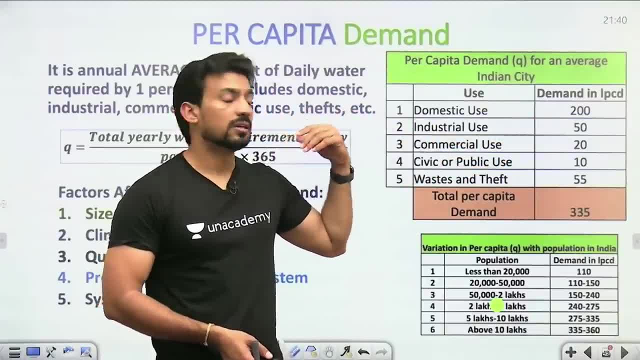 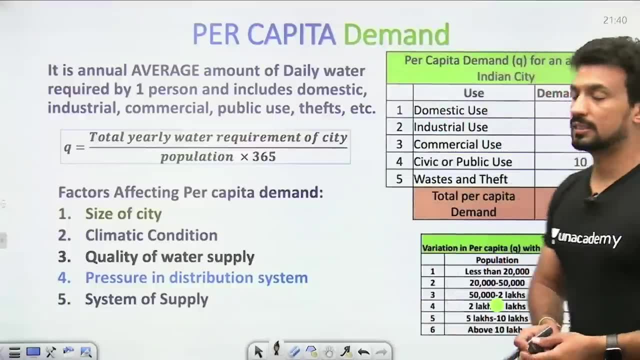 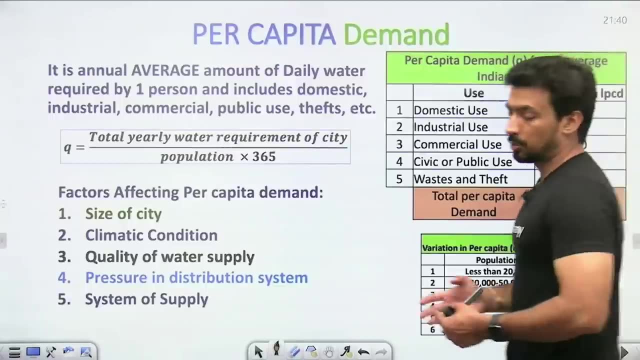 Consider 50 liters for industrial use, 20 liters for commercial use, 10 liters for civil use, 55 liters for waste and theft. According to this, the total per capita demand that comes is 335 liters per day. If you have to go according to the population, then how much will the population be? 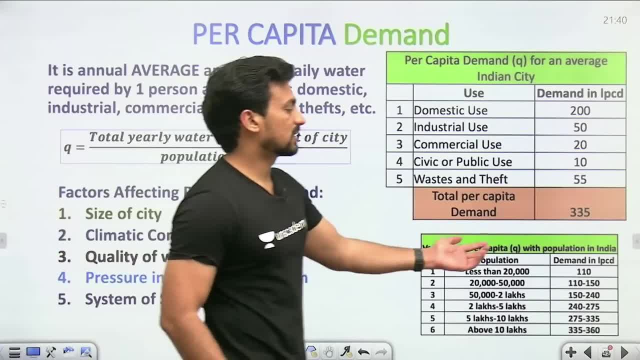 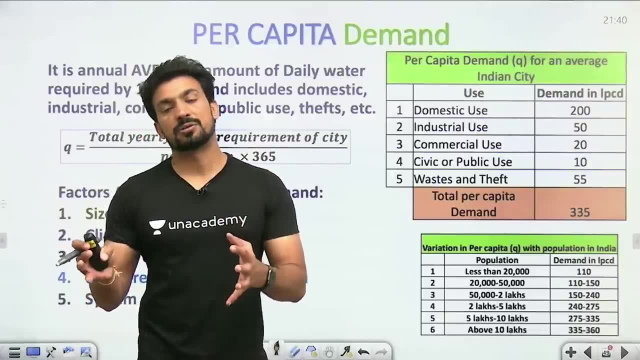 According to the population. we have data that if it is less than 20,000, then it is 110 liters per capita per day. As the population increases, the size of the city is increasing. If the size of the city is increasing, then the facilities and requirements of the city also increase. 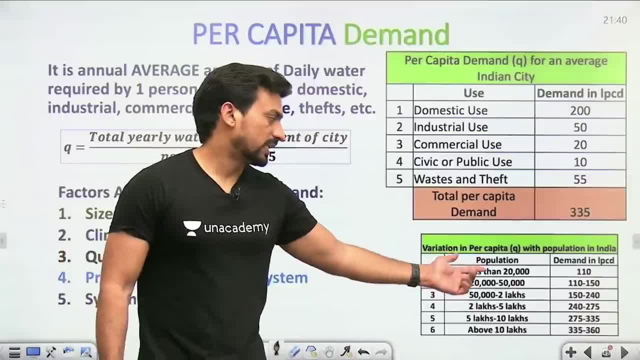 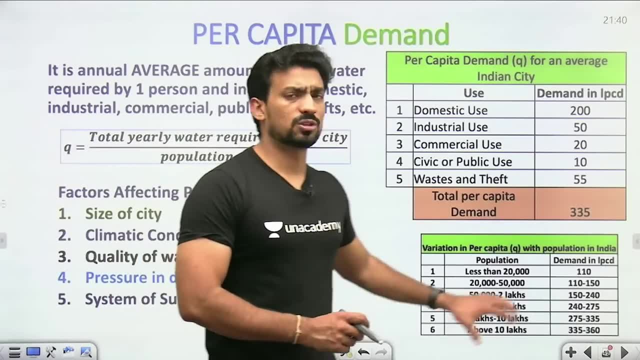 That's why the requirement comes out more, So less than 20000 liters per day. In 2010, it was only 110 liters per day. If we go to a population of more than 10 lakhs, then it comes between 335 and 360 liters per day. 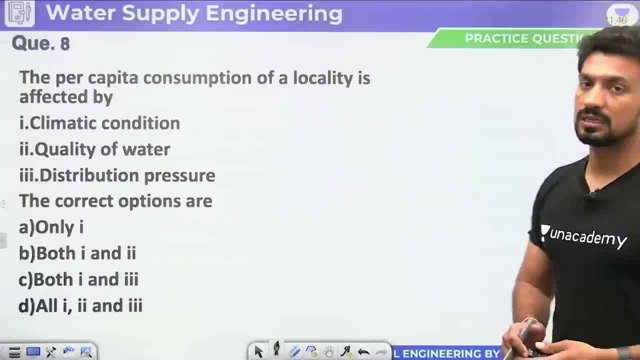 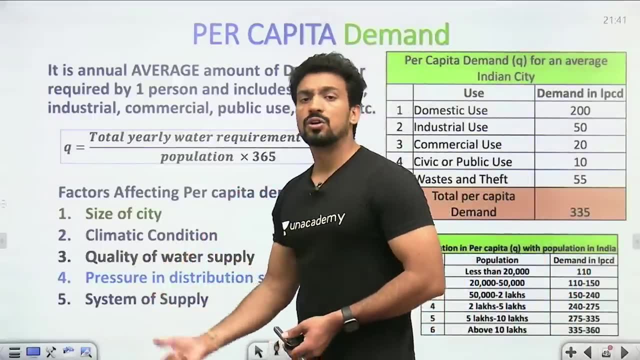 So you don't have to remember these values. You just have to understand one pattern of what it is The per capita consumption of a locality is affected by. What is the size of the city, What is the climatic condition? What is the quality of water supply? 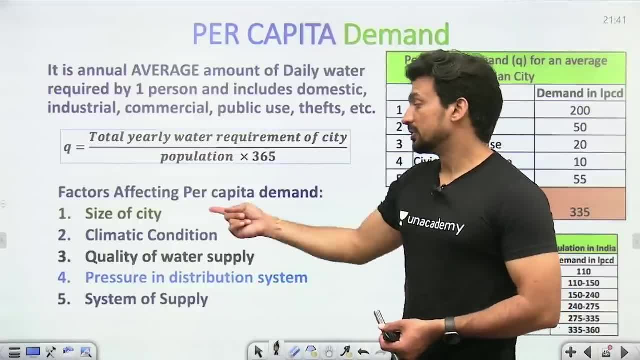 How much is the pressure in the distribution system? How much is the system of supply? The bigger the city, the more water it will require, And if the facilities will be more there, then the per capita demand will increase. Climatic condition. 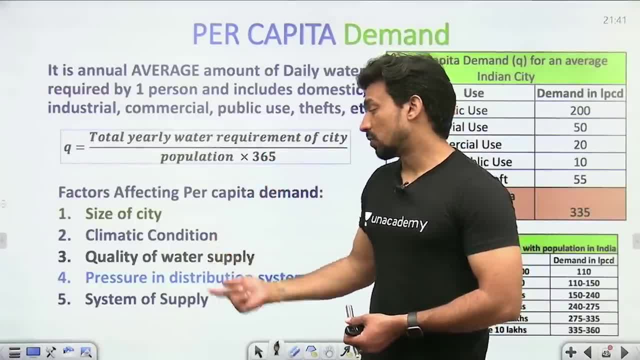 Hot conditions. If there is a hot climate, then the need for water will be more. Quality of water supply: If good water is available, then people will use it more. If the water is bad, if there is hard water, then it will be used less. 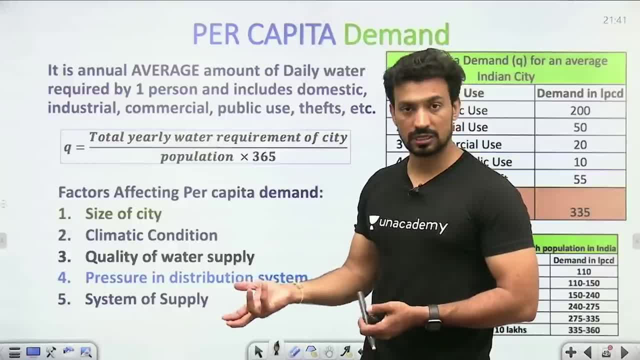 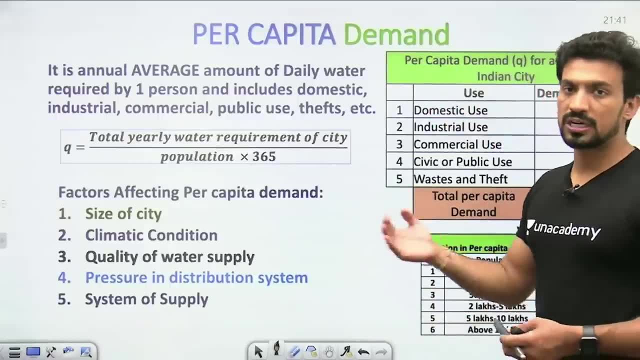 Pressure of distribution system: If there is more pressure, then more water will be utilized. System of supply: If 24 hours of water is available, then more will be used. Intermittent: If 2 hours are coming in the morning and 2 hours are coming in the evening, then less will be used. 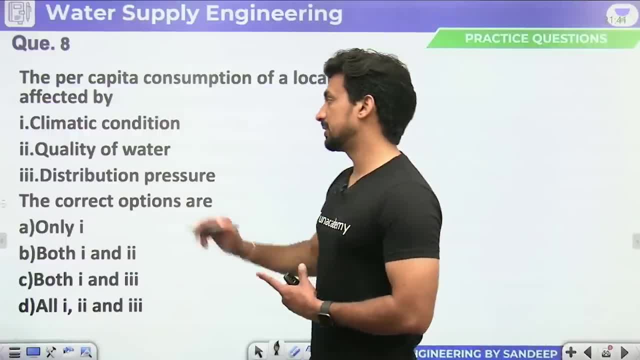 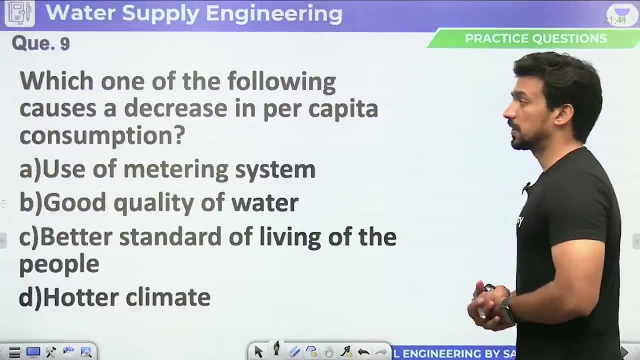 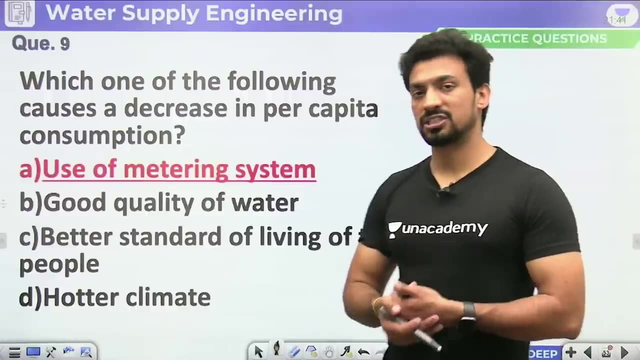 The per capita consumption of a locality is affected by climatic condition, Quality of water supply, Distribution, pressure. This is affecting everyone. Next, Which one of the following causes a decrease in per capita consumption? If you start taking money and start charging, because the more water you use, the more money you have to pay. 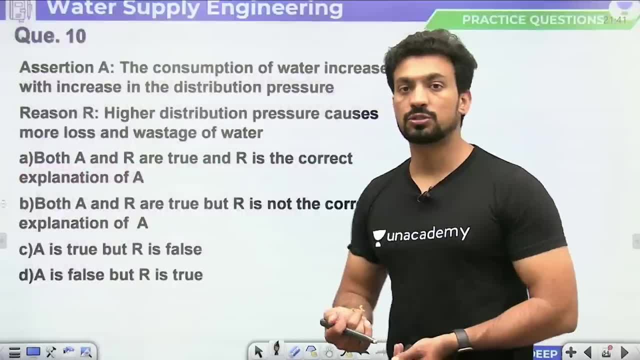 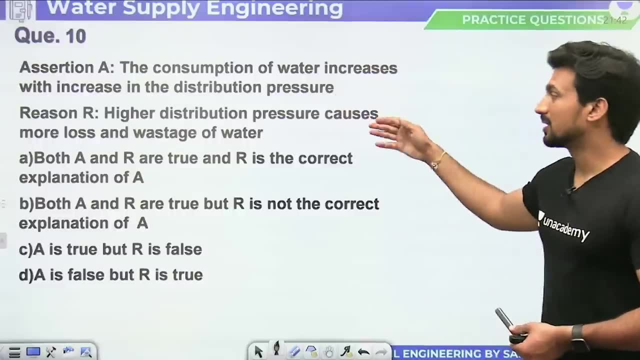 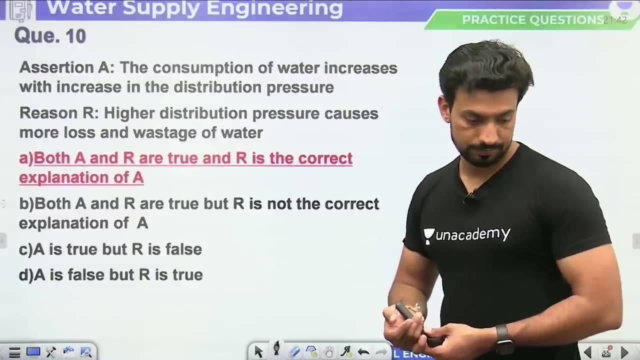 If you do the metering system, then obviously less water will be used. Next, The consumption of water increases with the increase in distribution pressure, Because higher distribution pressure causes more loss and wastage of water, Which is right. This is what the system is discussing and explaining. 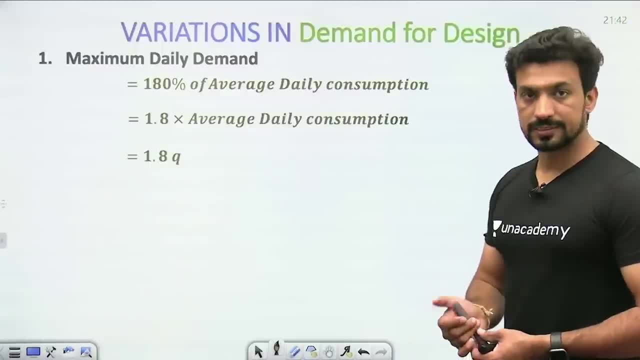 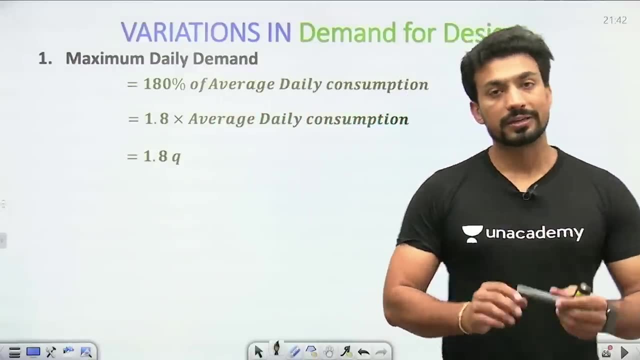 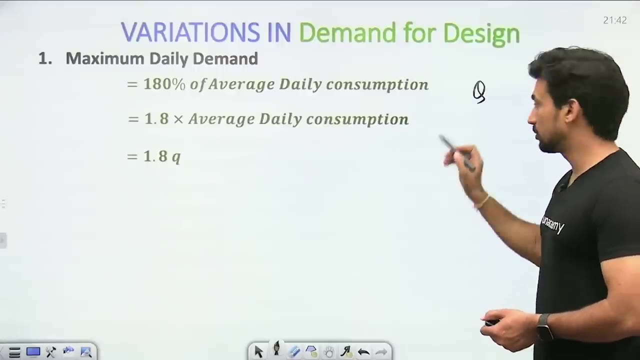 Next Let's see some demands. The first demand is the maximum daily demand. Maximum daily demand tells you how much you should get day by day to be the average. Why did we calculate that? Why does the entire city need water during the whole year? 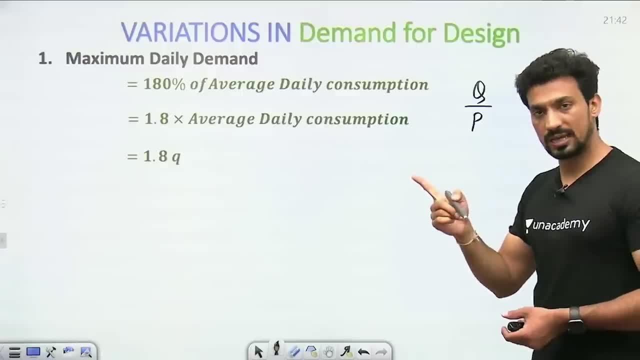 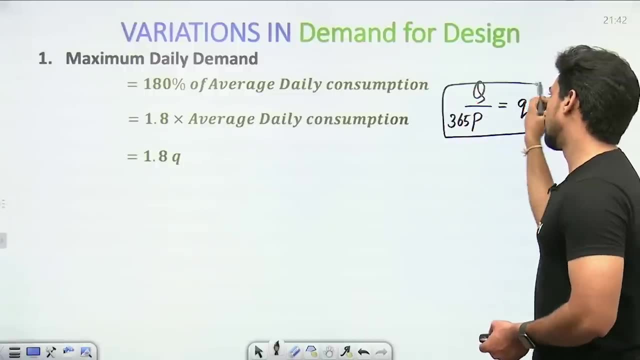 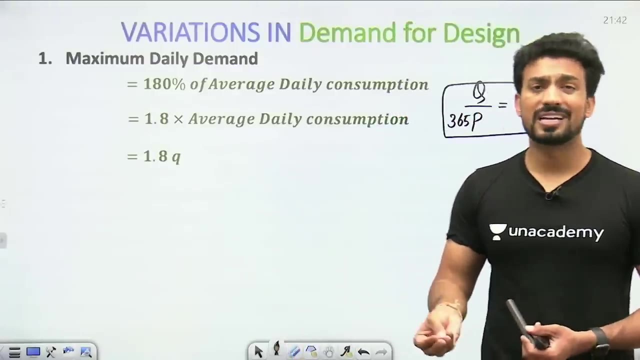 If you divide that by population, you will get that how much water a person should get in a whole year. If you divide that by 365, then how much water should be used in a day on an average, How much water should we get in a day? why did our average daily demand come now? if there is a day when we want more water than the average day, then we will say that if we increase it by 80%, then why do we mention it as 1.8 to calculate the maximum daily demand? 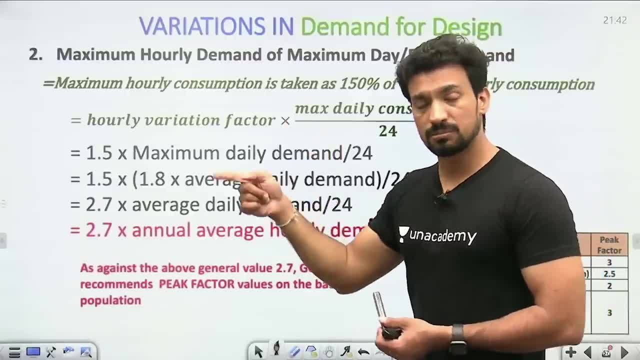 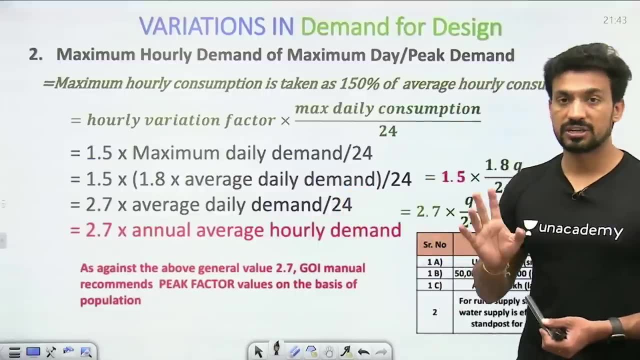 Then after that, friends, if the maximum day had to use more water in a particular hour, then what will we do for that? then we will use the hourly variation factor for that. We said that the maximum daily demand you had was 1.8 times of Q. 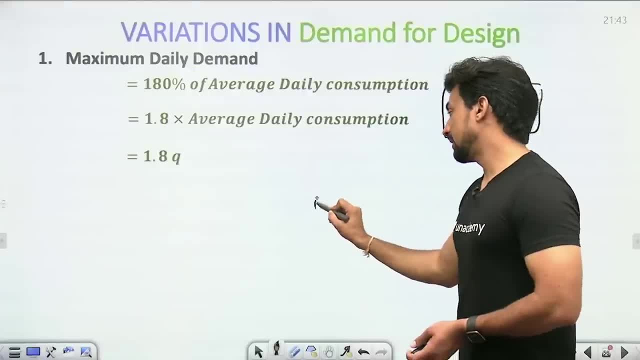 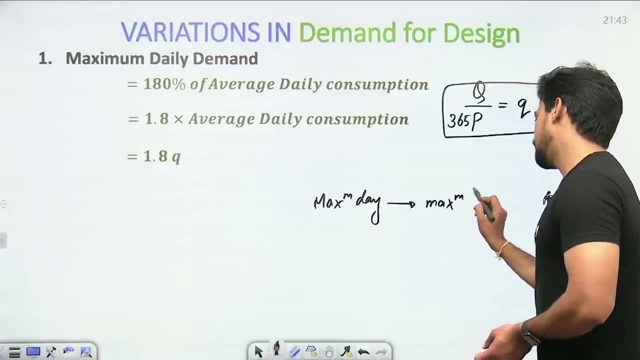 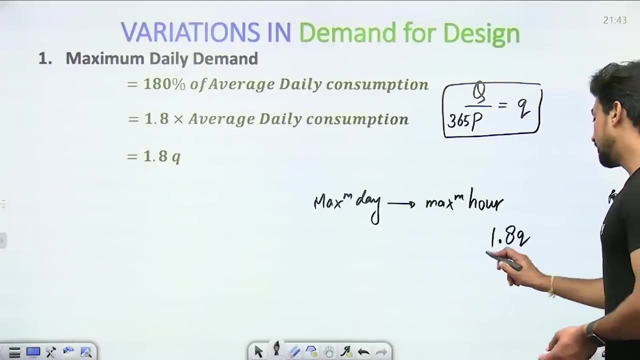 We said that 1.8x of Q is then on the maximum day. if we talk about any maximum hour or peak hour, then how much water was being used on the maximum day? 1.8Q and divide 1.8Q, so at an average, divide 1.8Q by 24 in one hour. 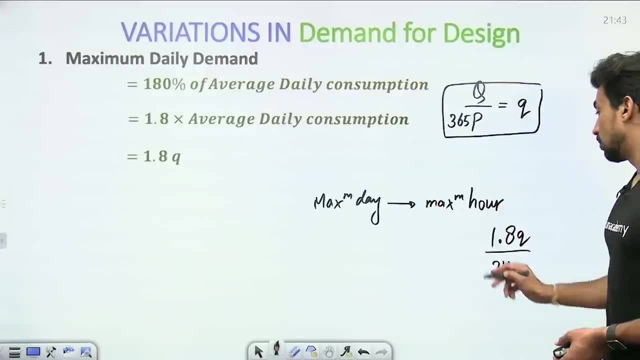 So on the maximum day at an average, divide 1.8Q by 24 in one hour At an average how much water was being utilized. so this is the maximum day at an average, how much water was being utilized every hour. 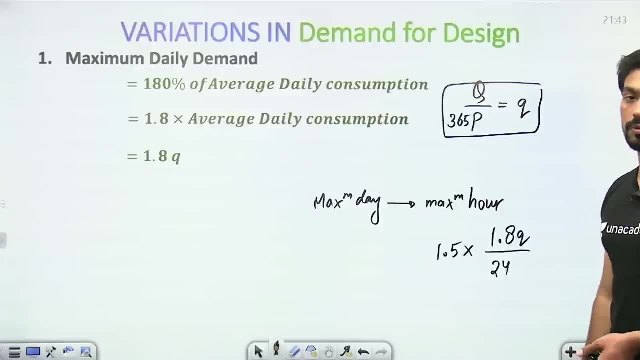 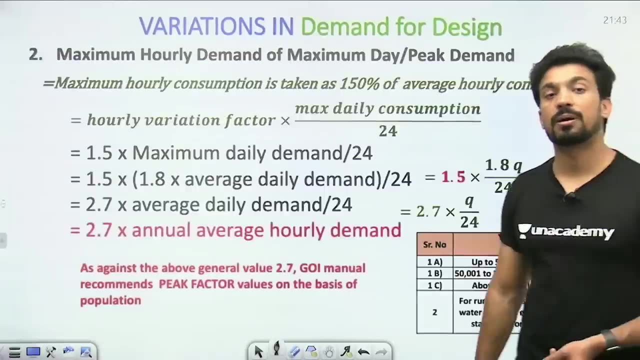 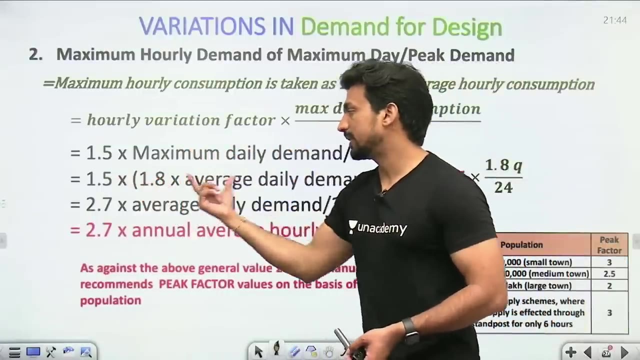 Let's multiply this with an hourly variation factor, which is 1.5. So we come to know what is the peak hour demand, or how much water we will need on that maximum day at a maximum hour. So do 1.5 times of maximum daily demand divided by 24. or you do 1.5 times of 1.8 average which you had divided by 24.. 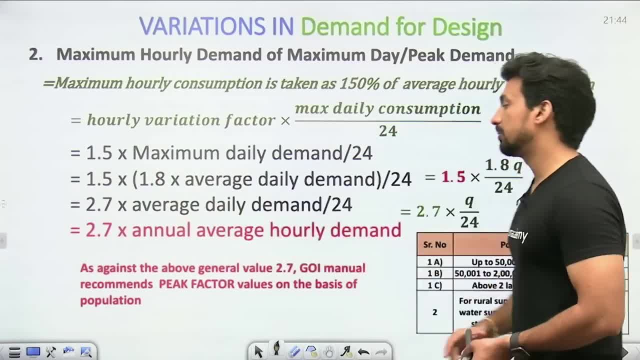 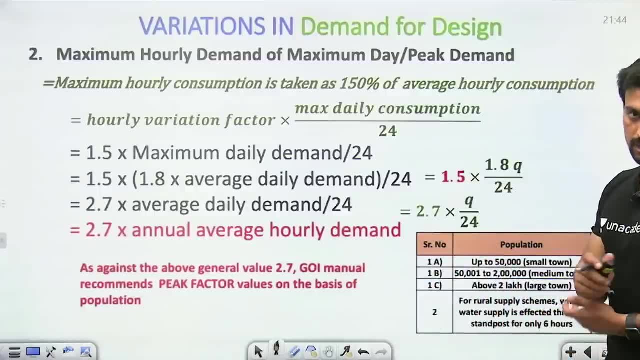 If we multiply these two then it becomes 2.7 average daily demand by 24, or you can say 2.7 times of annual average daily, annual average hourly demand. Now this is the factor that we have. Government of India manual says that it is not necessary to use it as it is. 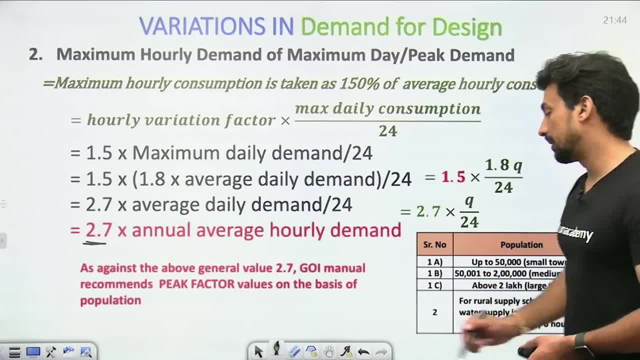 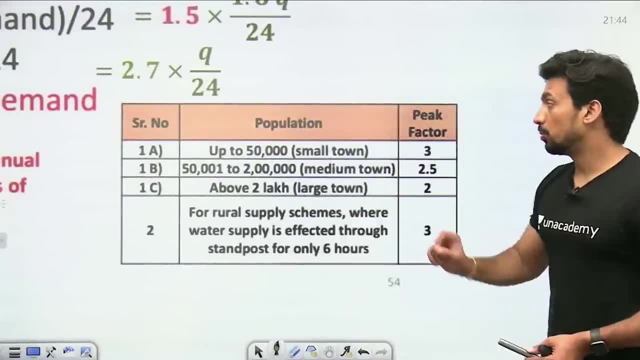 These peak factor values depend on the population, So you can use it according to the population. So what questions were asked related to this? A question related to this was asked: that if there is a population of a city, If it is a city. 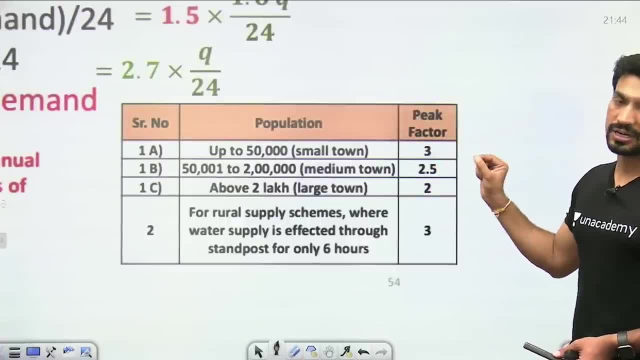 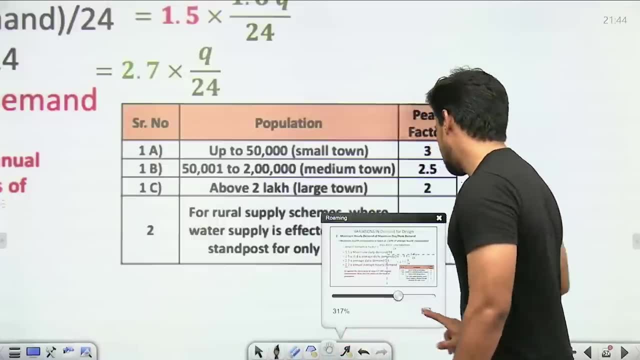 If there is a population of 70,000, then how much peak factor should be used for that? So for that we will use the peak factor 2.5.. Questions like this have been asked to you in the exam, So I hope you understood this. 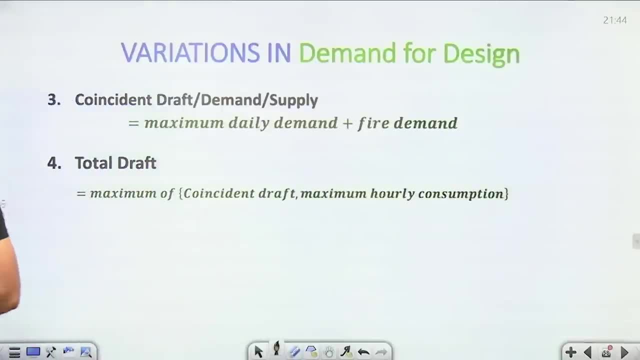 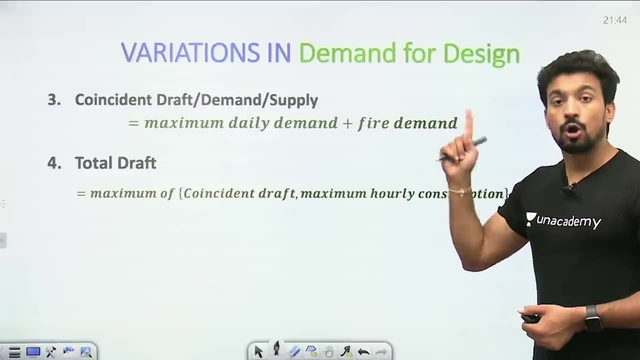 Now it has been revised through this session. Let's move ahead quickly How questions are made. If we talk about coincident draft or supply, then it is maximum daily demand plus fire demand. In the objective question you will see such options. 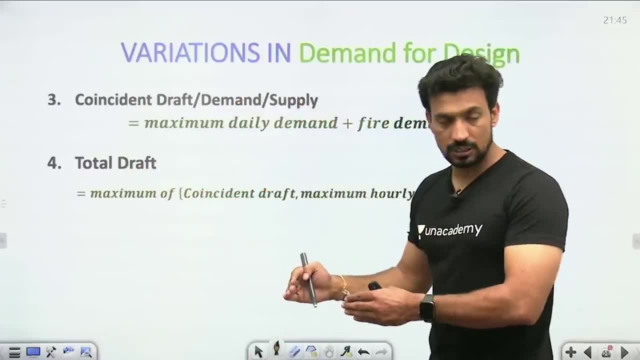 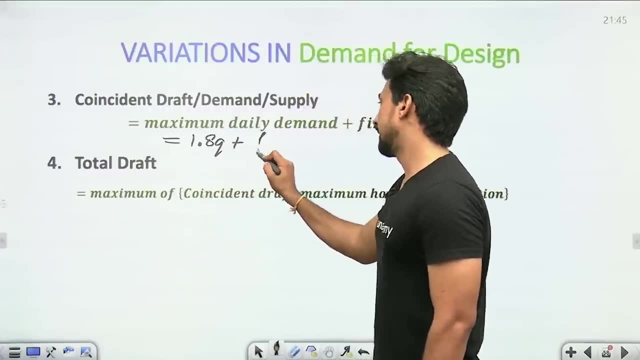 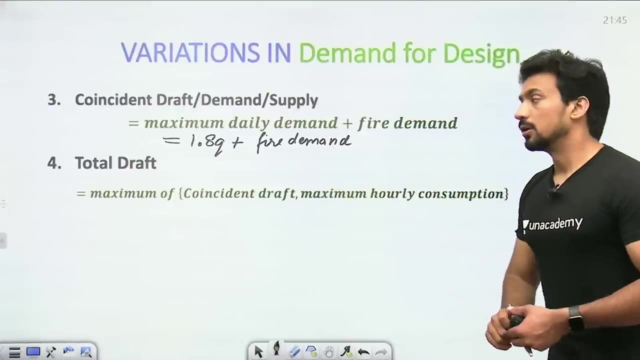 Coincident draft is represented by. Then there will be four options given In it. you can also see written that 1.8q plus fire demand. So the point is the same. Maximum daily demand is written as 1.8 times of average demand. 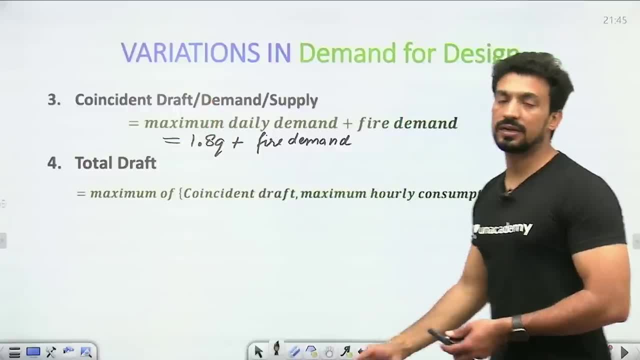 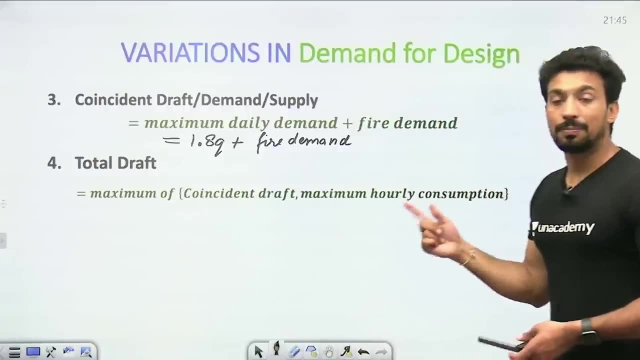 So if 1.8q plus fire demand is written like this, then it means that it is talking about coincident draft. If we talk about total demand or total draft, then it will be the maximum of coincident or peak demand. All statements are objective questions in themselves. 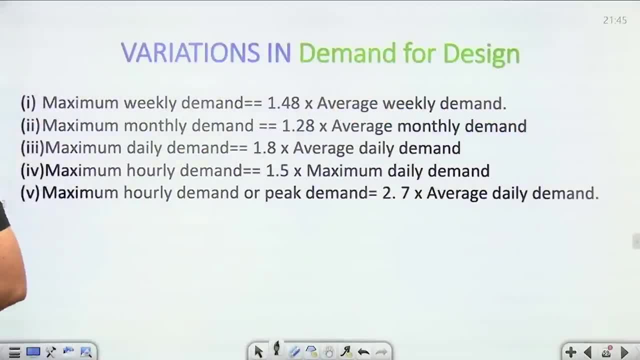 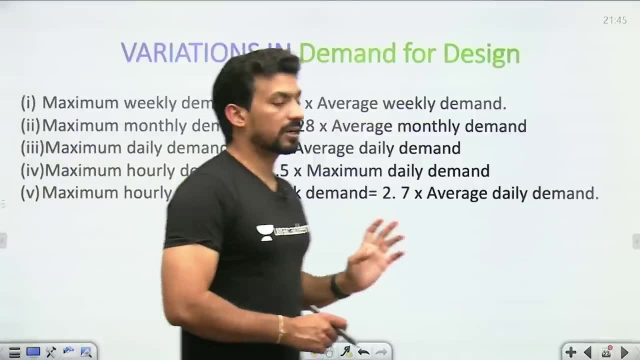 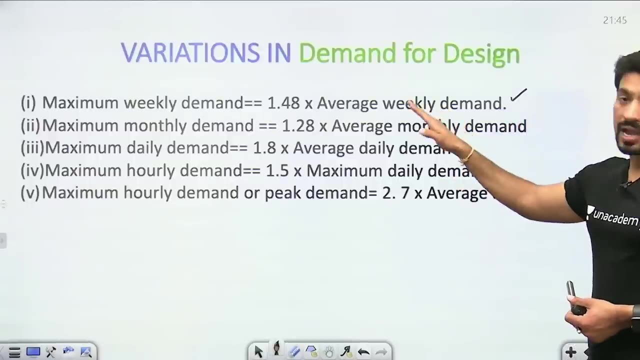 If the examiner goes into much more detail. Now he is saying that tell me maximum weekly, monthly, daily hourly, hourly demand or according to peak demand. So what do you have to do? In the case of weekly demand, you will use 1.48 times of average weekly demand. 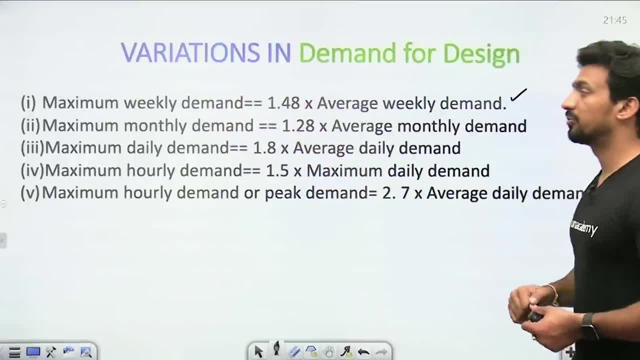 So if you want to use conversion factor on a weekly basis, then 1.48.. According to monthly, you can use 1.28.. You have already seen the daily one. You have also seen the hourly 1.5 one. 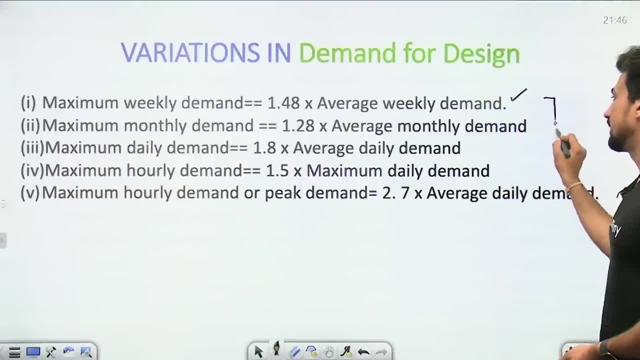 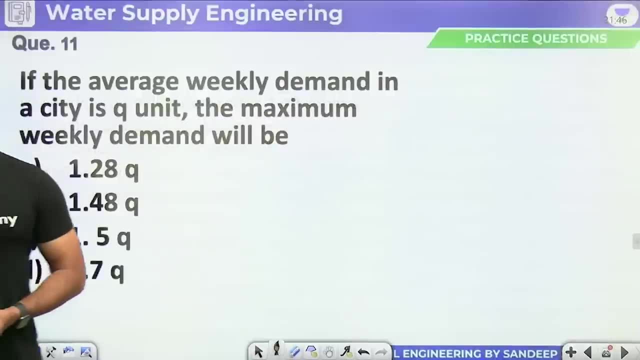 And the 2.7 one. So these two are left Weekly and these additional come. You can also see this. You can remember 1.48 or 1.28.. Let's move on to the next question. The next question says: 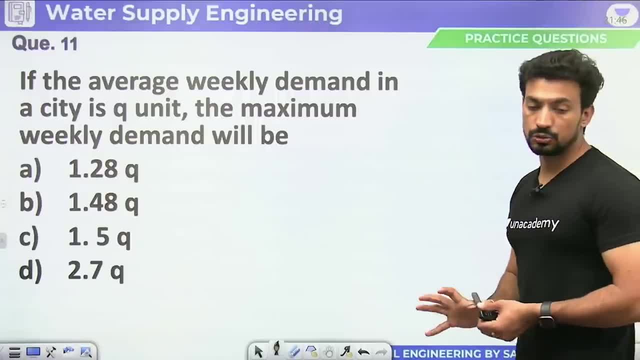 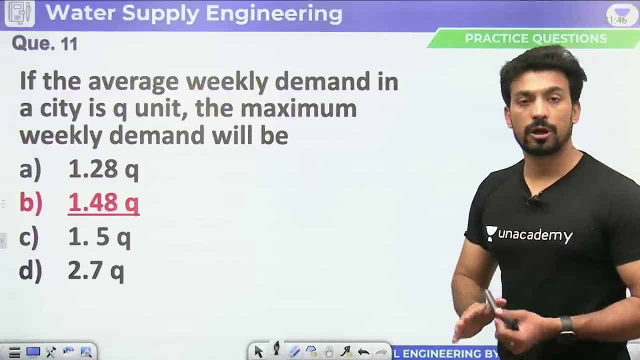 If the average weekly demand in a city is q unit, the maximum weekly demand, The average weekly demand, is given. So what will be the maximum weekly demand? It will be 1.48q. This is very simple. You have to remember this. 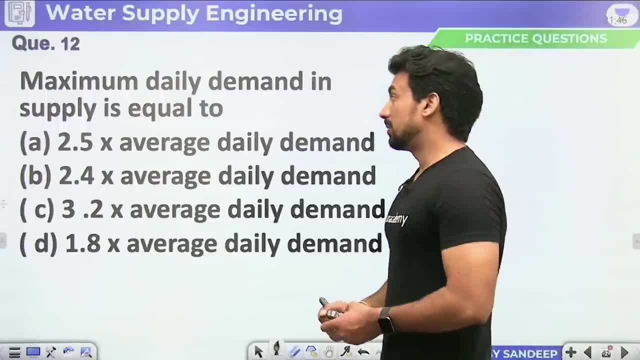 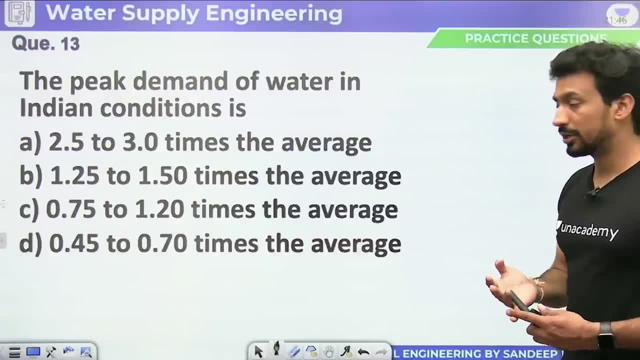 The maximum weekly demand will be 1.48q. The maximum daily demand in supply is equal to: If we talk about the maximum daily demand, then how much do you consider? You consider 1.8 times of average daily demand? The peak demand of water in Indian conditions is: 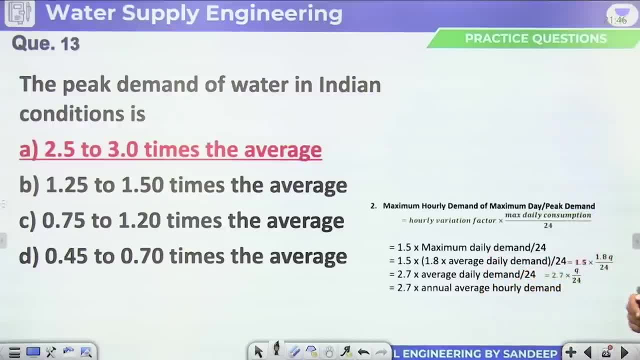 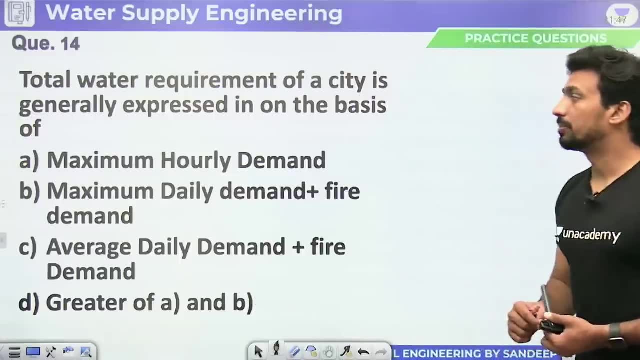 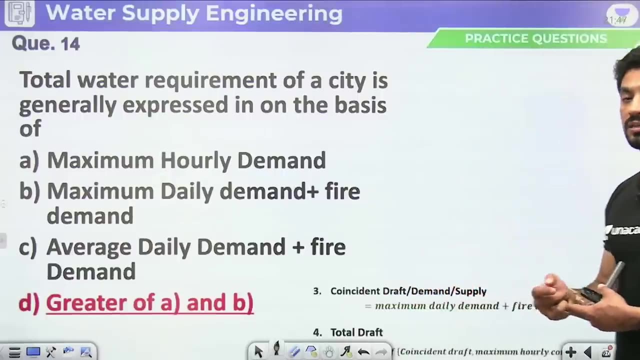 In Indian conditions between 2.5 and 3,. these peak demand factors vary. We had accepted 2.7.. Total water requirement of a city is generally expressed on the basis of The total that is expressed is considered according to the peak demand and coincident draft. 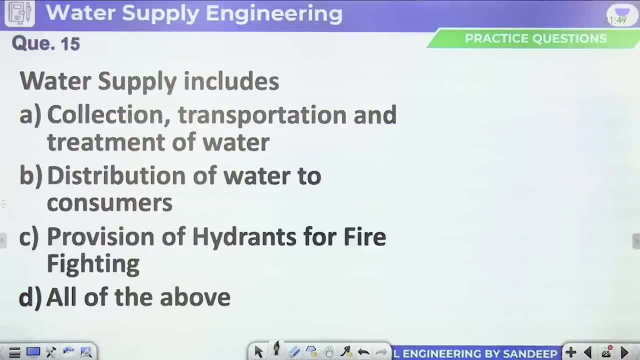 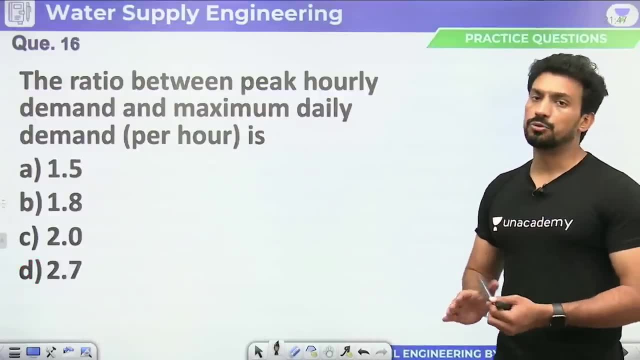 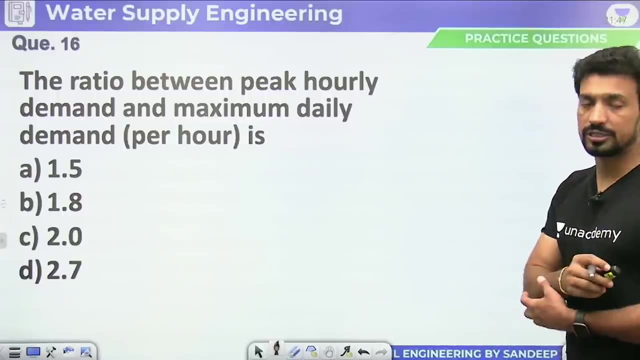 So coincident draft. and maximum hourly demand or peak demand In the water supply scheme, collection, transportation, treatment, distribution, provision of firefighting are all included. All of the above The ratio between peak hourly demand and maximum daily demand per hour according to, if we talk. 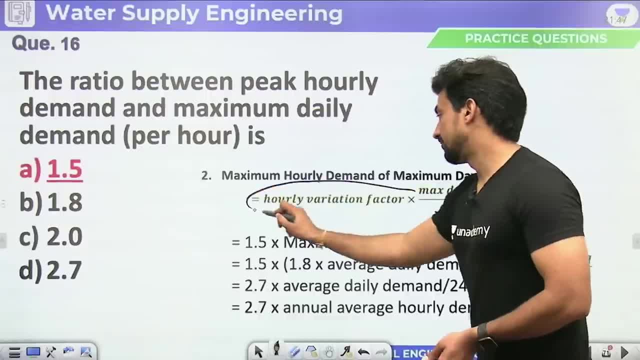 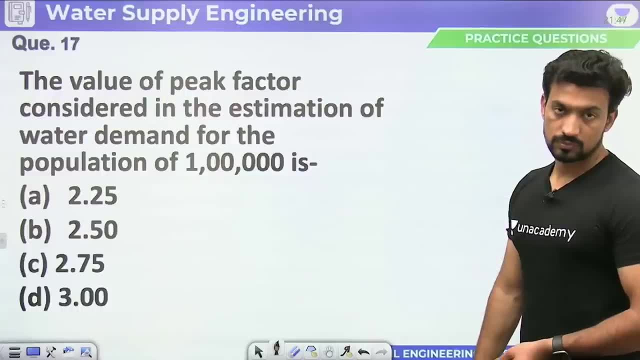 Obviously, he is asking you the hourly variation factor. And what is the value of the hourly variation factor? It comes to 1.5.. Next, The value of peak factor considered in the estimation of water demand for the population of 1 lakh. 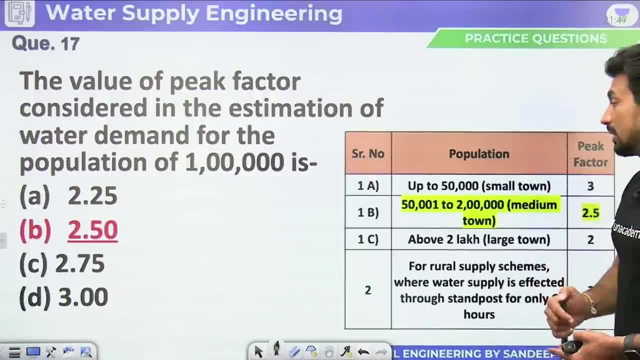 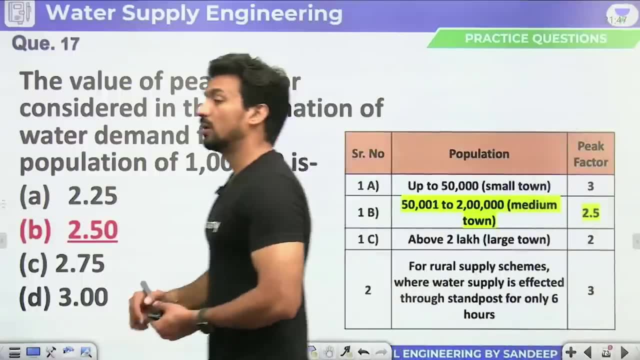 So now the small table you saw. He asked a question from that table. In that table, if you have a population from 50,000 to 2 lakh, then you have to choose 2.5 here. So these questions You will revise yourself once or twice. 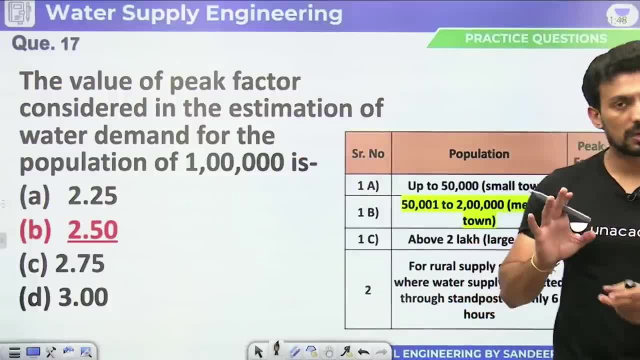 You will read a little carefully once or twice. You will see this table once or twice, So slowly it will start to set in your mind. Still, if you think that, no, no, no, I don't know what will happen in the exam. 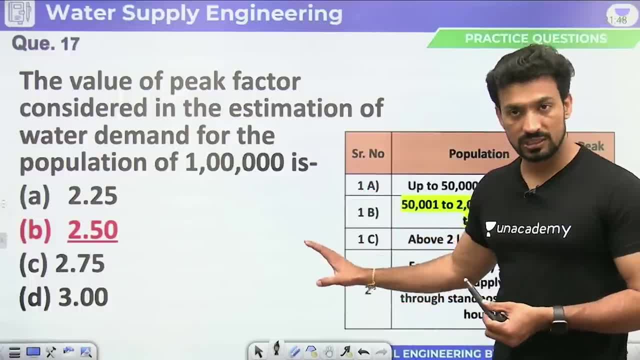 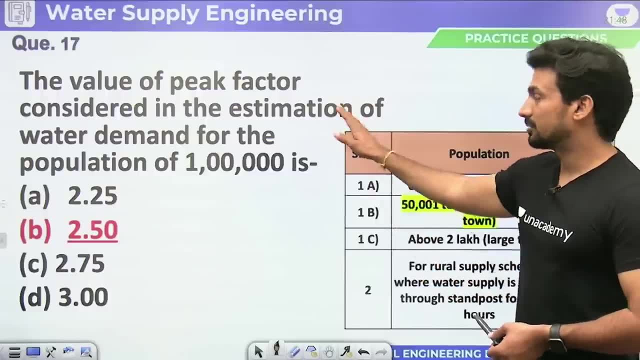 I understand now. I will not understand in the exam, So just do these questions. Whatever you get in the pdf or whatever you are seeing in the class, Understand these questions carefully, In which case you have to refer to this table. If the hourly variation factor is asked, then you have to answer 1.5.. 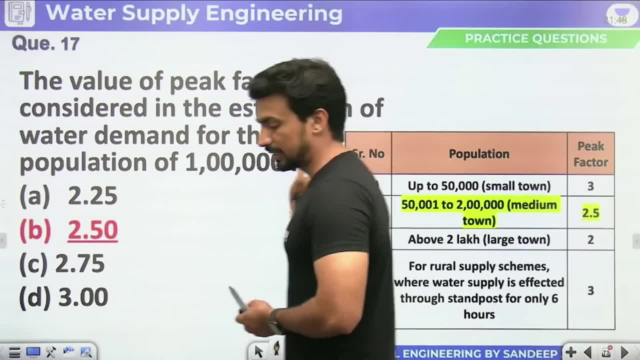 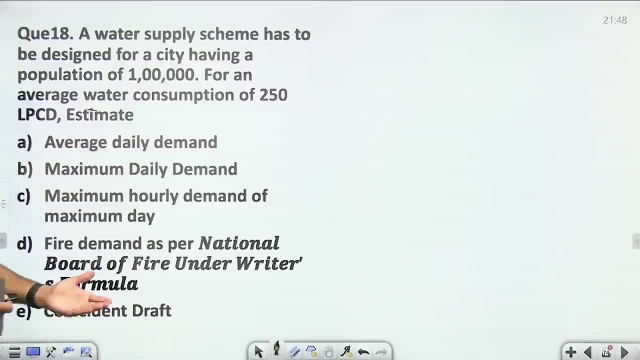 If you have to do maximum daily demand 1.8.. So all these factors See like this. Then after that we did this question in the class When we were studying in detail how to calculate one thing. We calculated them through objective questions. 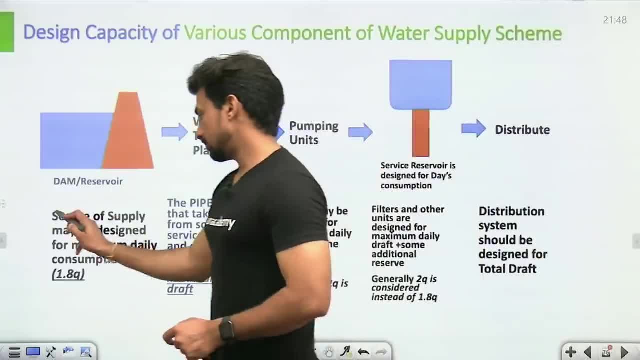 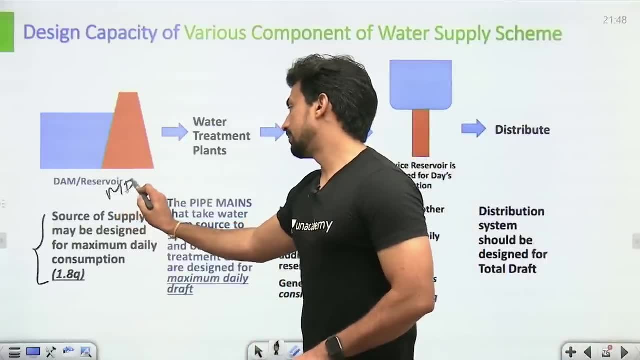 The source of your water supply. It will be 1.8 times off average or maximum daily demand. It will be designed- We will design it- for MDD. Then after that, if we talk about the pipe mains, This will also be designed for maximum daily demand. 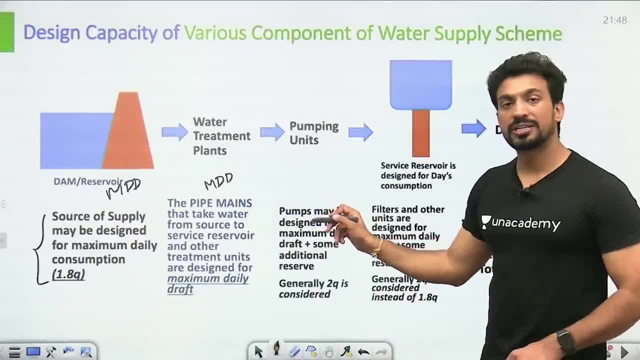 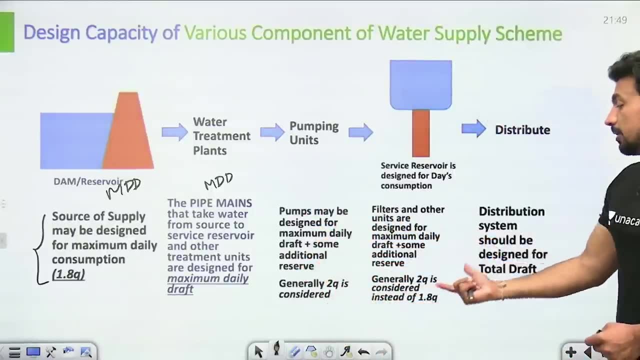 Or 1.8q. This is a little more than 1.8q. The pumping units or pumps, They are a little more than 1.8q. That is, we design it equal to 2q. Then after that, if we talk about filters and other units, 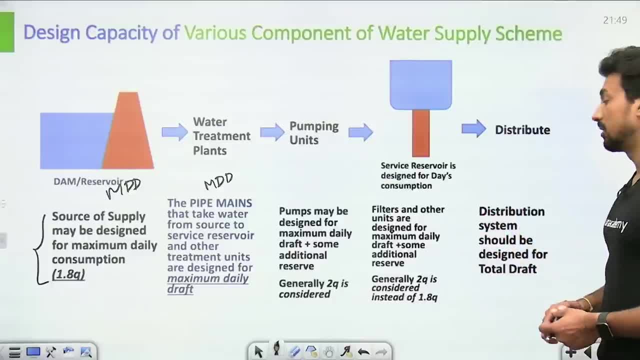 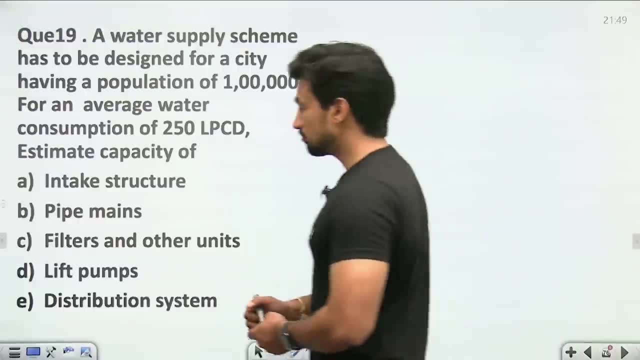 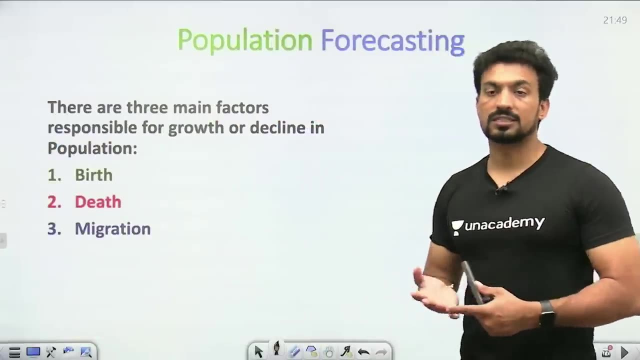 They are also designed equal to 2q Instead of 1.8.. And we design the distribution system according to the total draft or total demand. The next thing we have is that you have to do population forecasting. Why is it important to do population forecasting? 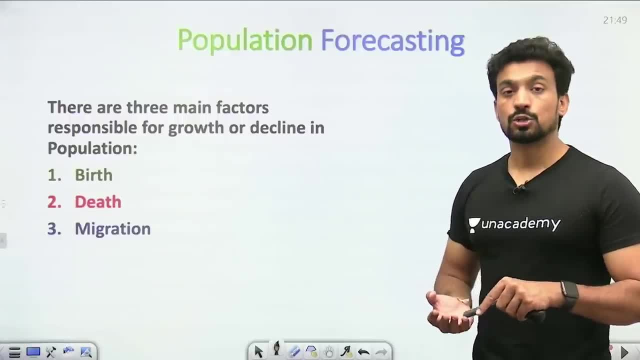 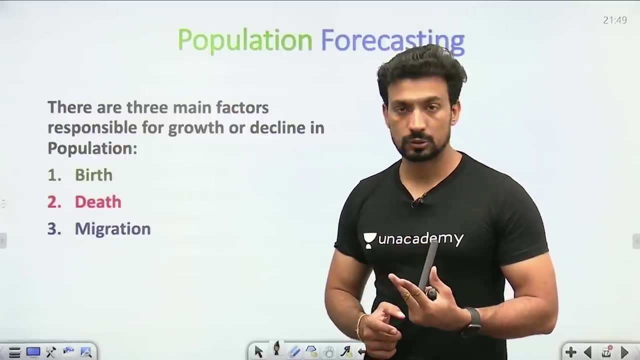 Because if you are designing a water supply scheme for any city, Then you should know what the population will be in the next 30 years, How many people are born there, How many people are dying there And how many people are coming and going there by migrating. 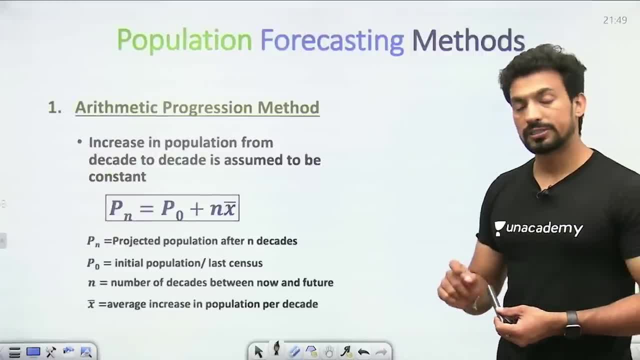 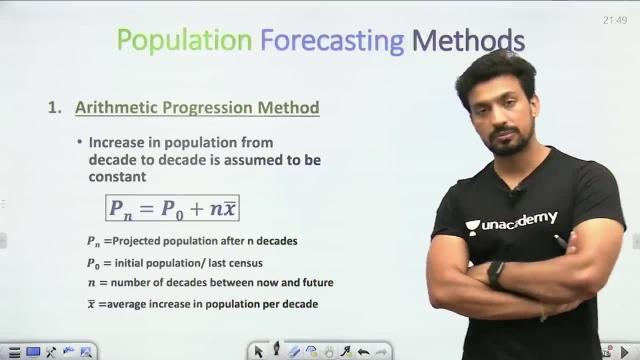 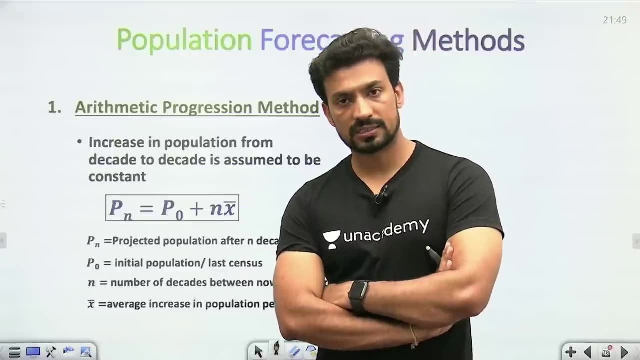 All these factors will influence the population. We have to study the three major methods of population forecasting from the point of view of JEE. The first one is the arithmetic progression method. We believe in this method That every year or every decade, We can also say yearly. 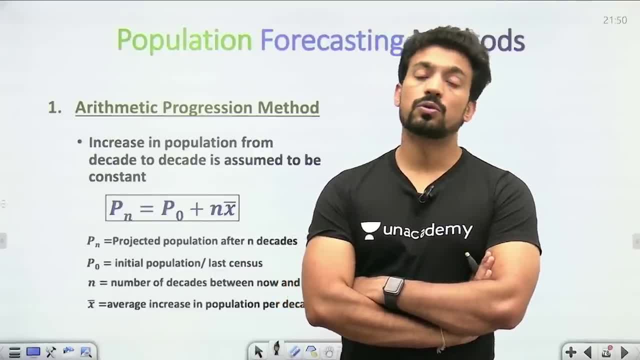 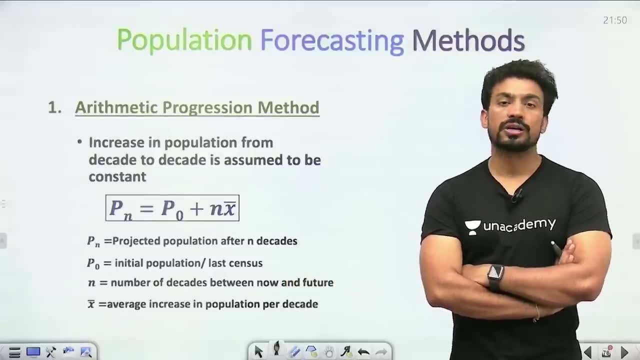 We can also say in decades. The data of the census comes in decades. It comes in decades As we say: we have 121 crore, we have 131 crore and so on. So the census that comes to India is also told to you in 10 years. 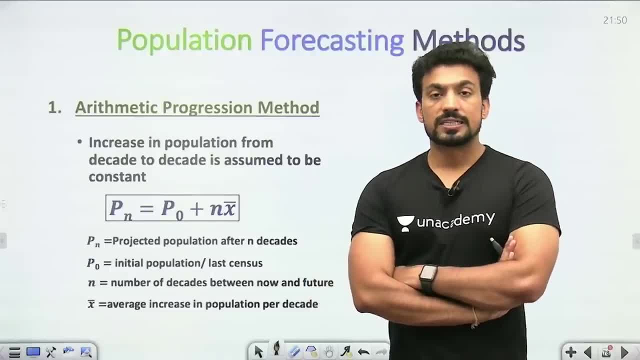 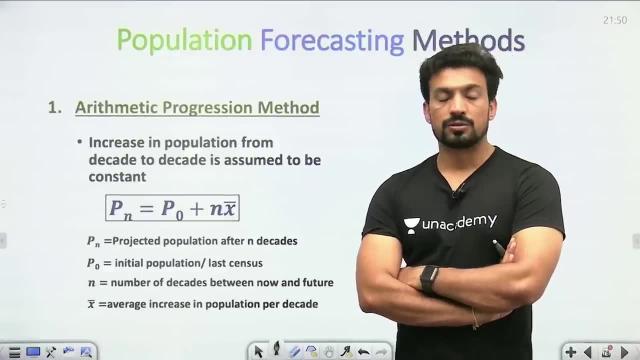 What is the population now? So it is believed that in the arithmetic progression method, The increase that comes every 10 years is the same, The same. that came from 2001 to 2011 is the same. The same that came from 2011 to 2021 is the same. 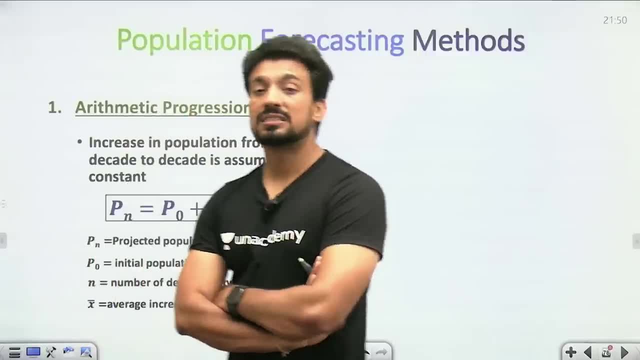 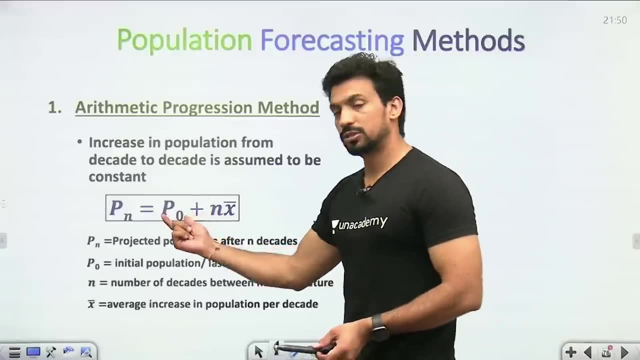 The same. that came from 21 to 31 is the same. So such an increase is considered to be the same, Or you can calculate the average and tell it according to it. So the last known population you have Plus how many years or how many decades you have to tell. 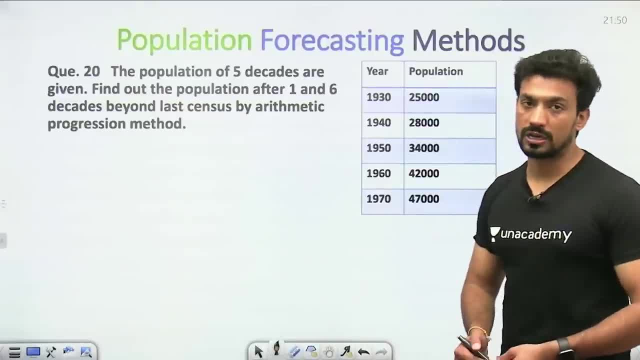 And in every decade, at an average, how much increase has come. According to it, you tell. As you don't have to do this question now, Just have to show you From 1930 to 40,, from 40 to 50,, from 50 to 60, from 60 to 60. 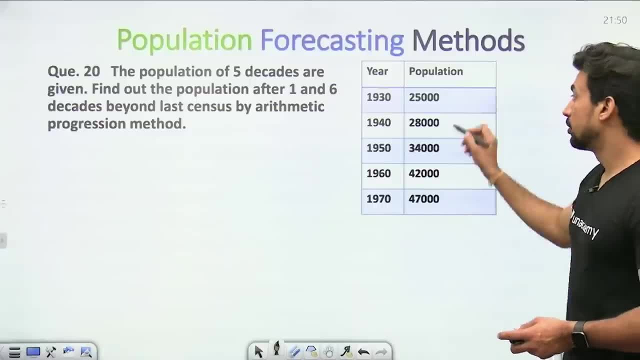 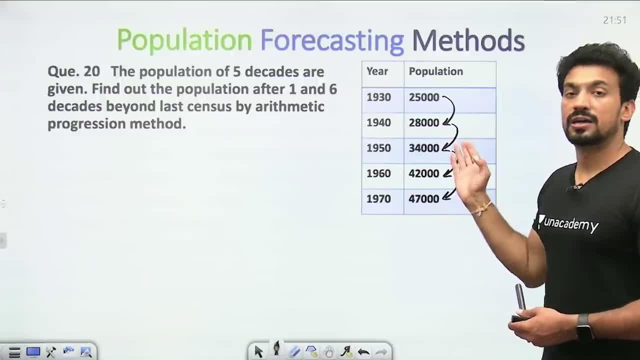 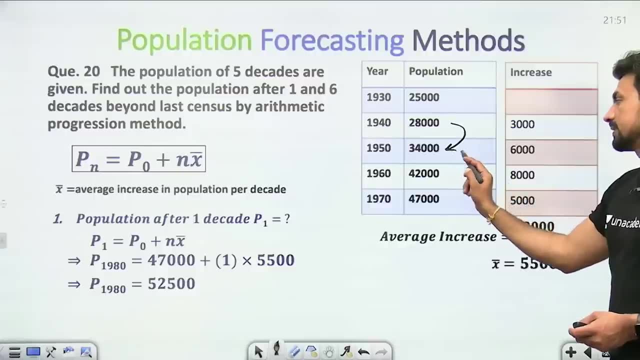 How much increase has come from here? The increases that came in the population. They will increase all of them After calculating the average, Like it came here: 3000.. Then after that, Here is the increase of 6000 from here. 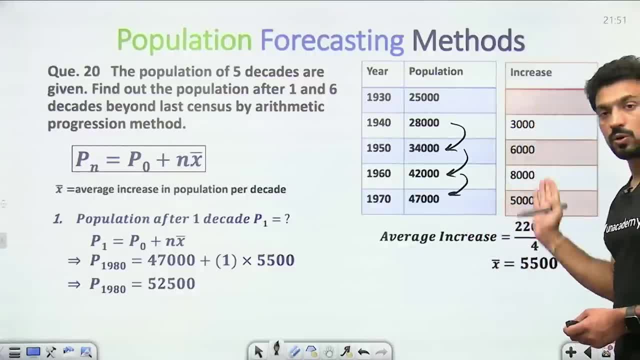 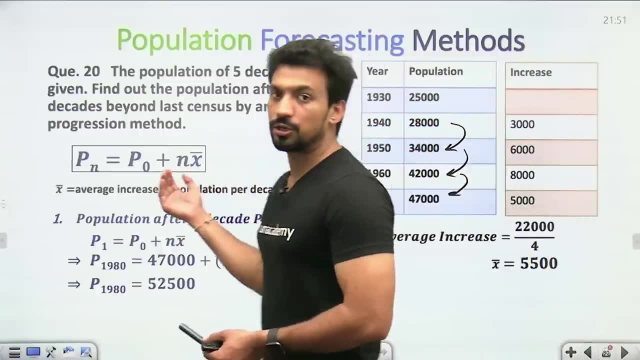 Here is the increase of 8000 from here, And here is the increase of 5000.. Added all of them and divided by 4. So the average increase came to be 5500.. So in every 10 years The population is increasing. 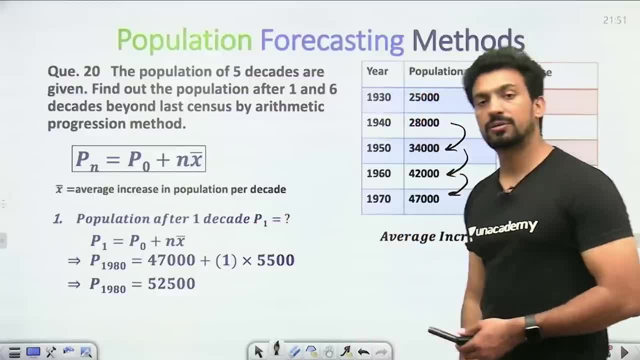 So after how many years? I asked you in the question. He asked in the question How much after 1 decade, How much after 6 decades. So you can put Last known data that we had. Last known data is 47000.. 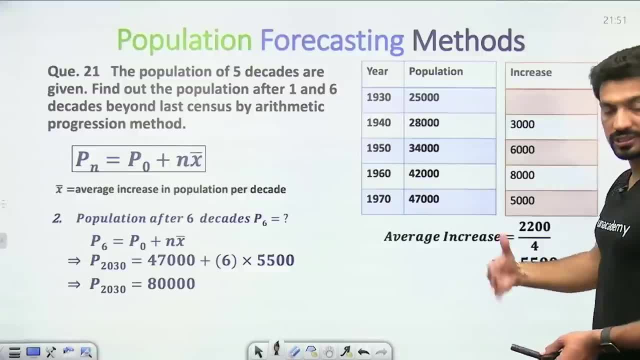 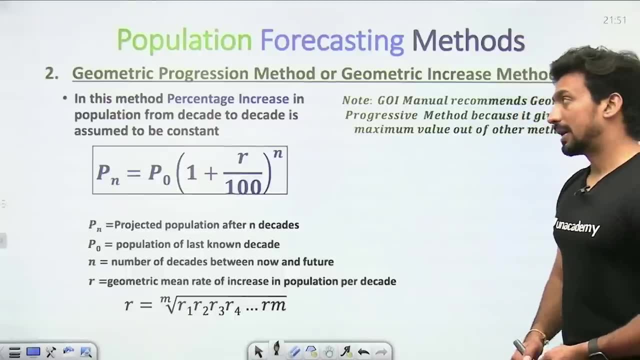 Plus: in every decade It is increasing by 5500.. So after how many decades? I asked. So last known data: Plus in every decade It increased by 5500.. How much after 6 decades, We can tell In the first method. 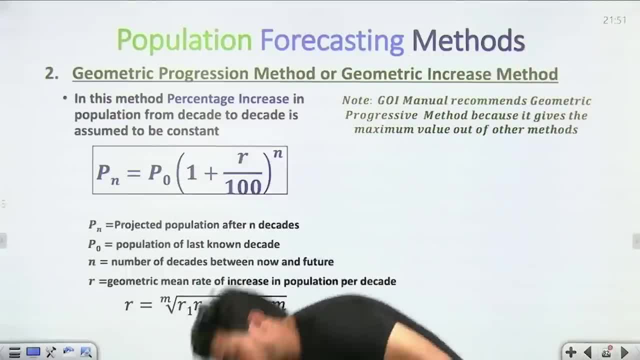 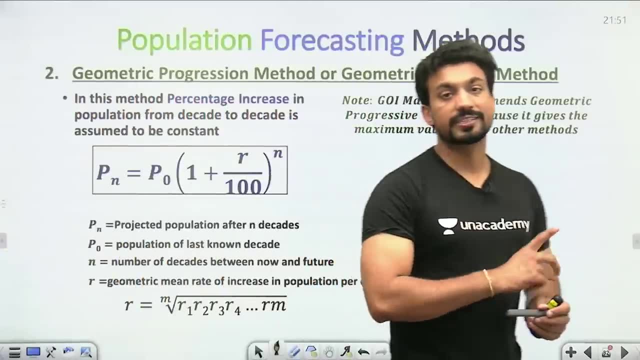 We considered it as constant In the first method. What we considered as constant, What we considered as constant- That increase in population- is constant In the second method. Percentage increase is constant, Like your pocket money today is 100 rupees. 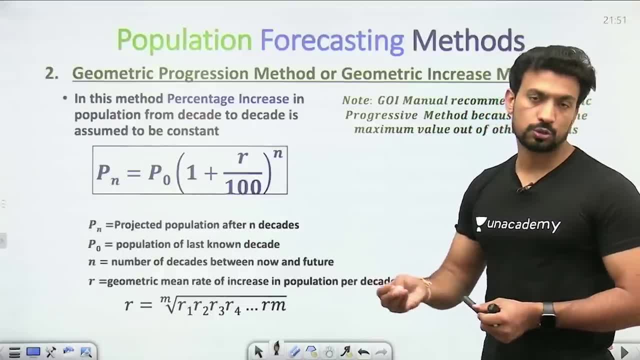 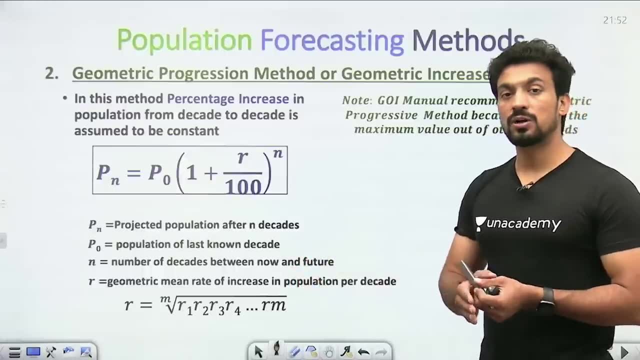 Yesterday you were given 2 rupees extra, So it became 102.. The day after tomorrow you got 2 extra, So 104. Then next day 106., 108., 110. And so on. So what happened to you? 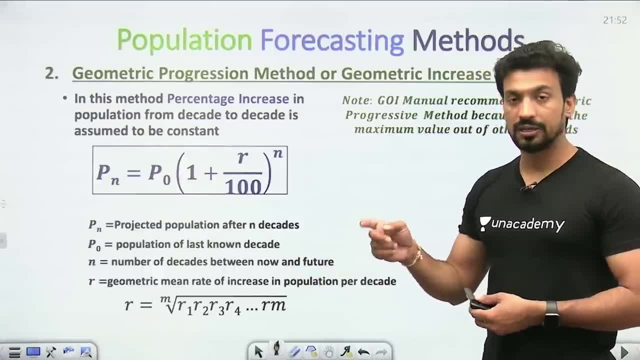 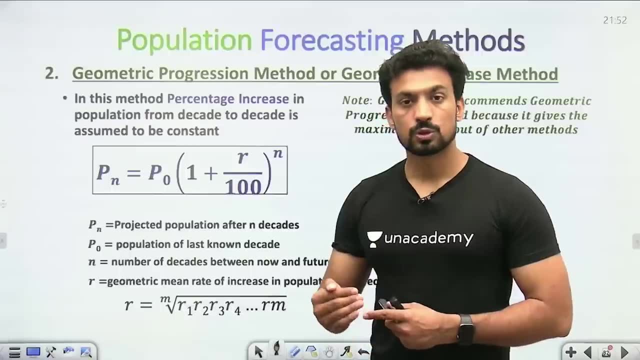 Fixed amount is increasing. So you can understand it as arithmetic increase In the second geometric progression method What we say in it. That percentage will increase. Today you got 100. So tomorrow it will increase by 5%. So tomorrow you will get 105 rupees. 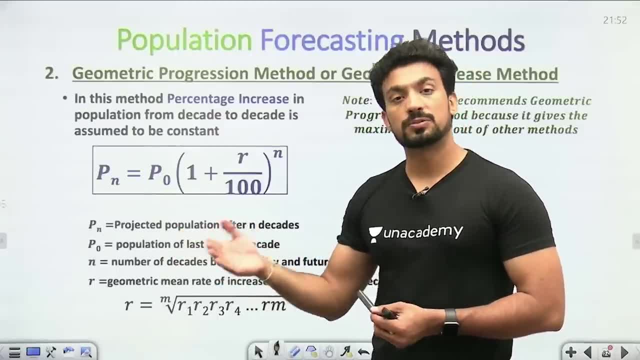 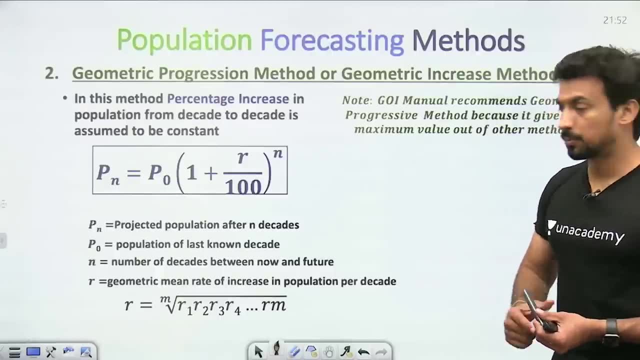 The day after tomorrow it will increase by 5%. So you have to increase by 5% of 105.. So percentage increase is considered as constant When we increase the percentage of something Like I told you. If you get 100 rupees today, 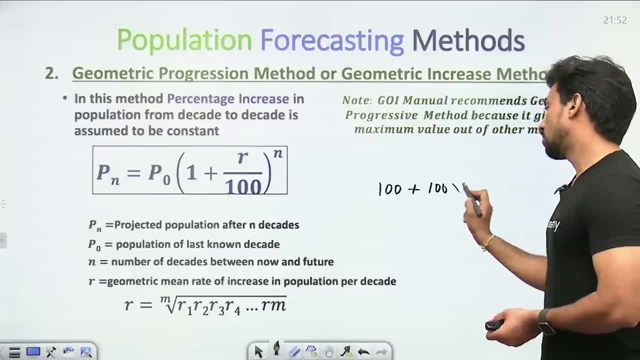 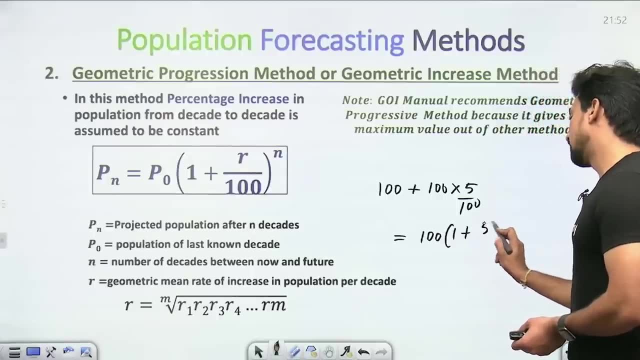 So how much will you get tomorrow? So tomorrow you will get 100 plus You will add 5% of 100.. Or what can I write this? I can write this: 100 into 1 plus 5 by 100.. 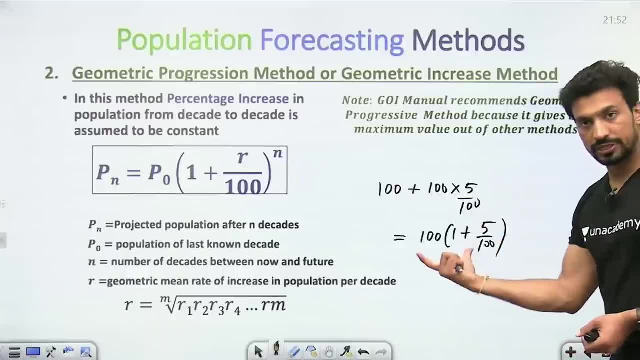 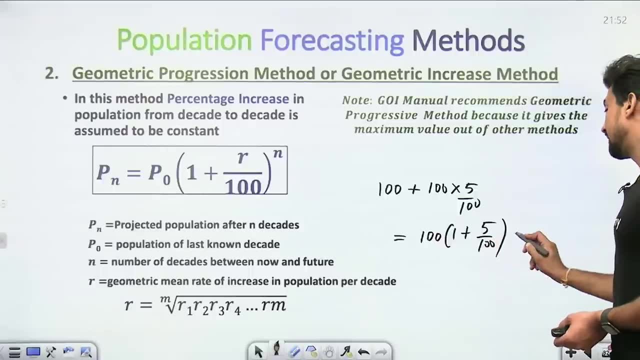 Then next day, This quantity Plus its 5%. So what we can do for that: Multiply this quantity From 1.05.. Or we can say: Multiply this From 1 plus 5 by 100.. Then next day: 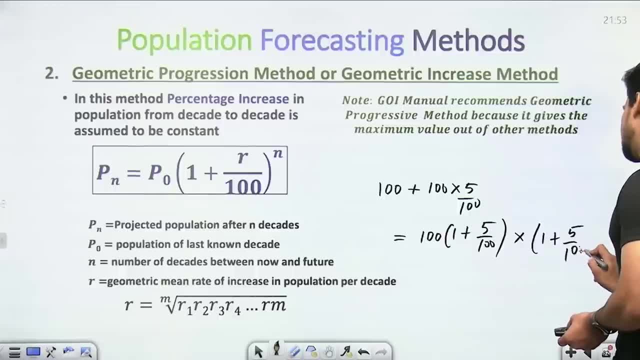 Its 5% also It has to increase by 5% more. So we will increase it again and again. So it means Here it will become its power In n. So 1 plus r by 100.. Raised to the power n. 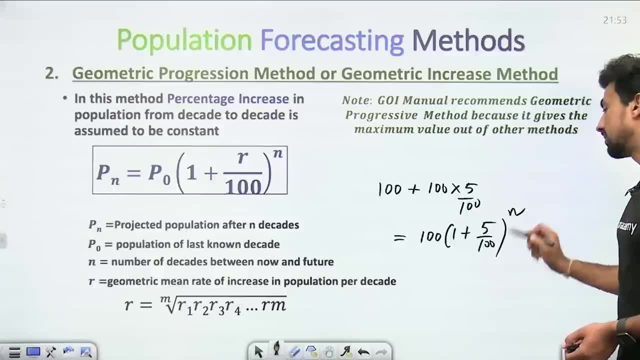 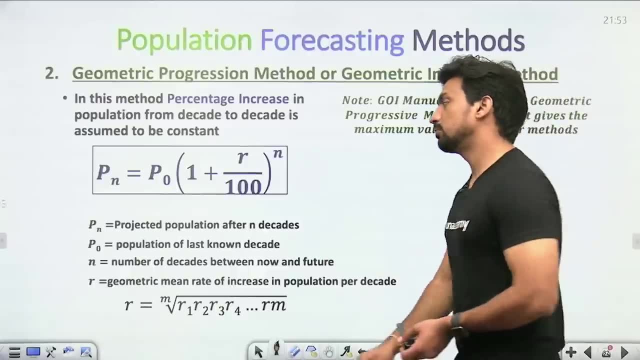 We use this formula And in it We will write r by 100.. 5 by 100. Then next day, This quantity Plus its 5%. We use this formula And in it The value of r, This r, which is: 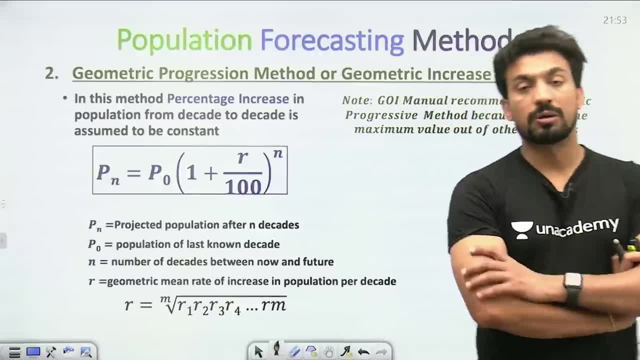 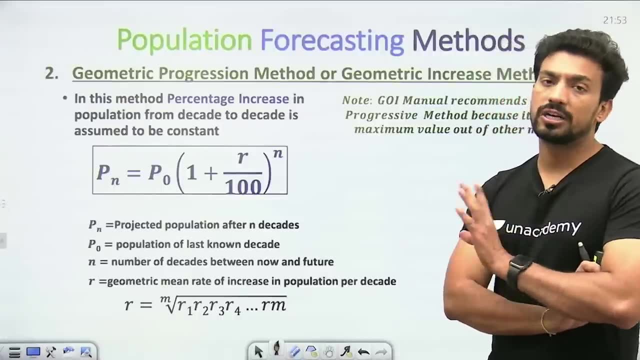 Rate of increase Or percentage Which is increased, We consider it constant. So Whatever data is given to us, We calculate their r Or percentage, Then its geometric mean Calculated. It is put How The population of a town. 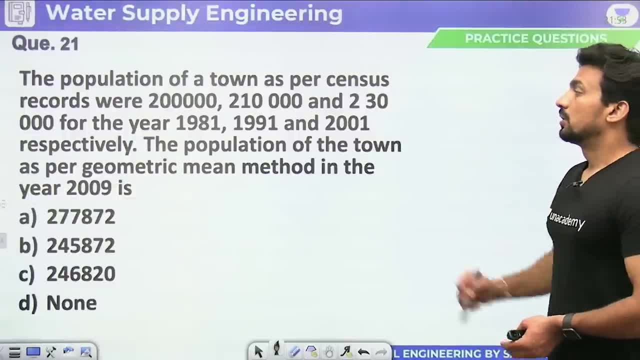 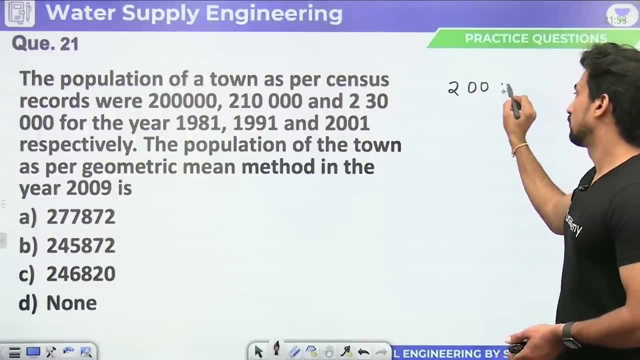 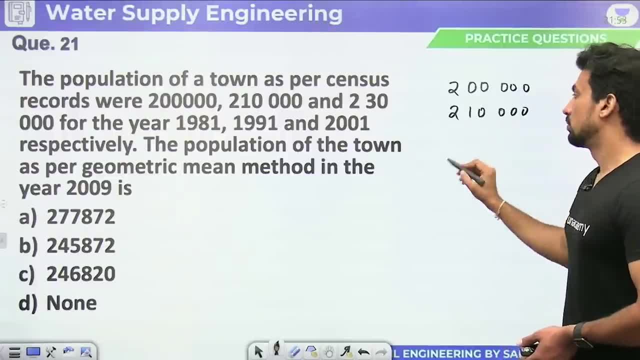 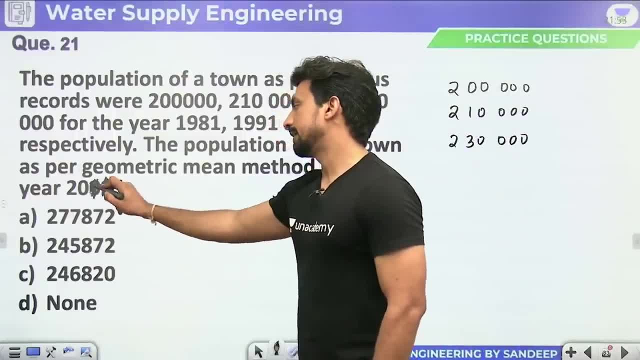 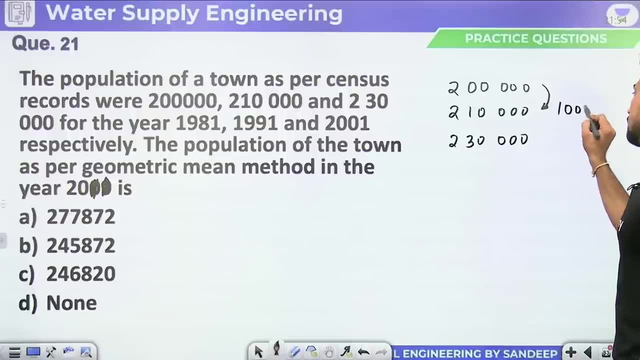 As per the geometric method In the year. Consider it as 11.. Means, After a decade, What you have to know. Then the increase. Let us know the first: How much was the increase? Here is the increase Of 10000.. 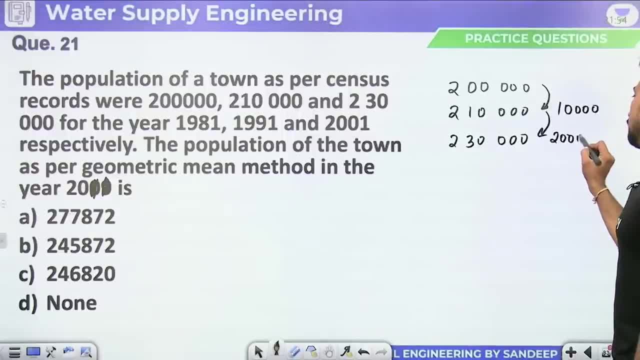 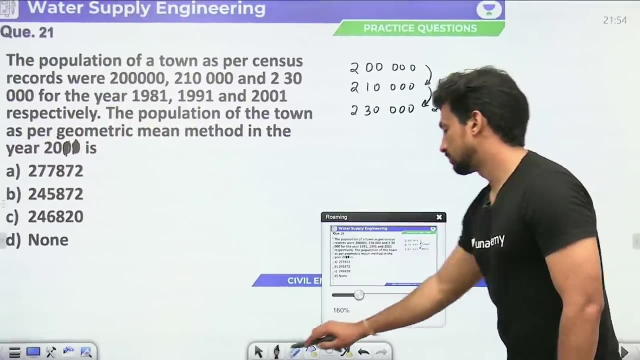 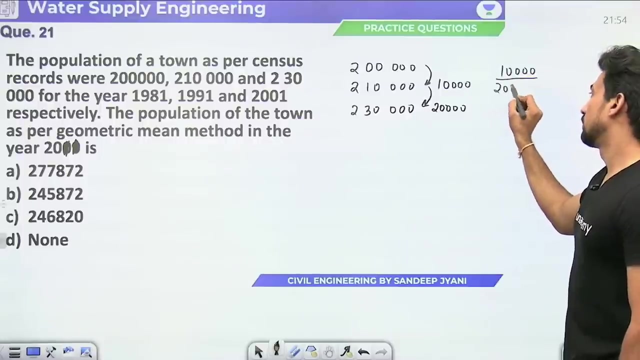 Then After that, Here is the increase: 20,000.. Now, If we talk about the percentage From here, How much is the percentage increase How much? If we talk about the percentage, then look at the percentage: 10,000 with respect to 200,000. 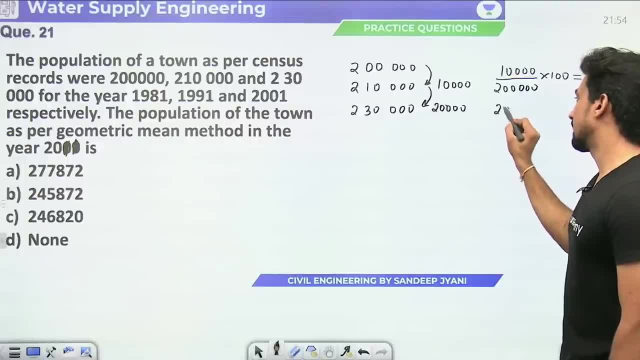 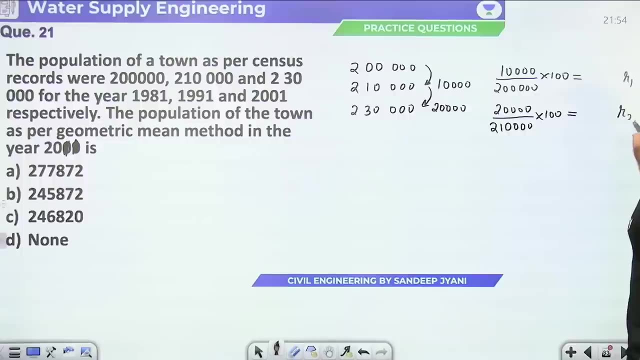 into 100, you have to tell here the increase of 20,000 came with respect to whose to 10,000, or 210,000 into 100, so you will get the values of R1, R2 from here and then you will calculate. 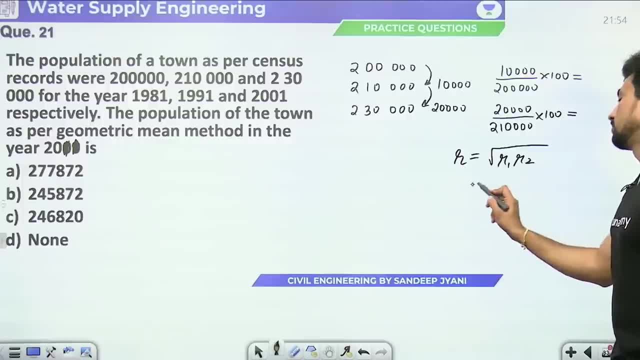 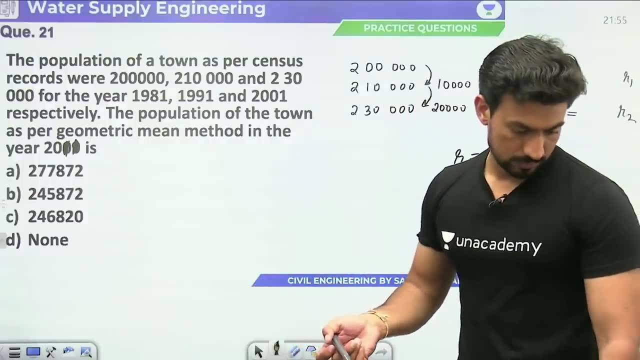 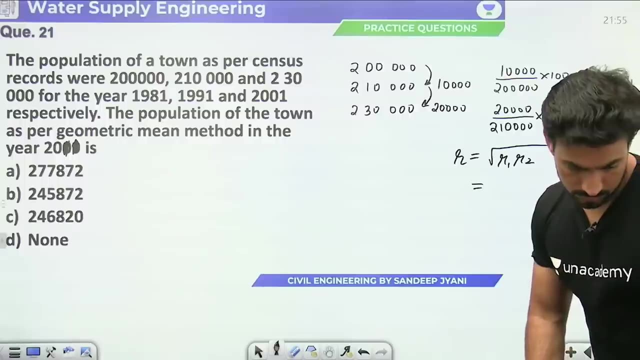 the R of geometric mean root of R1, R2,. if it was 3, then we would have taken cube root. if it was 4, then we would have taken power 1 by 4.. So I am going to take it. 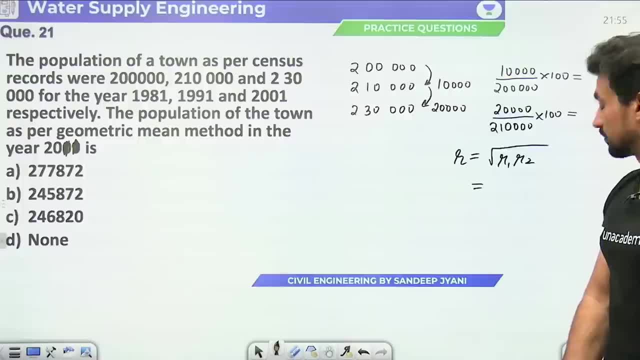 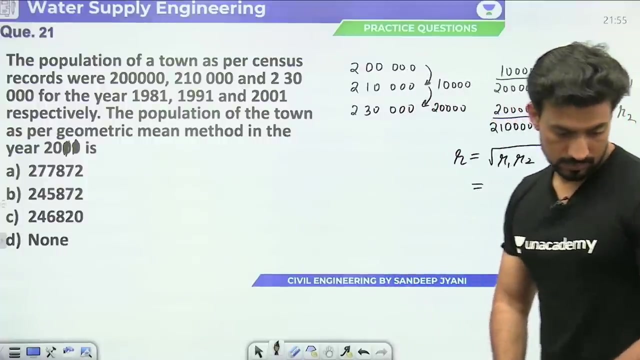 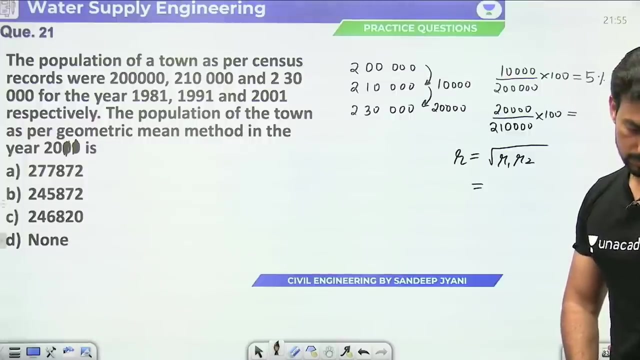 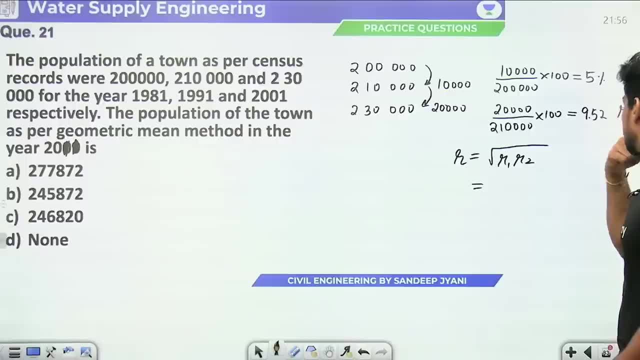 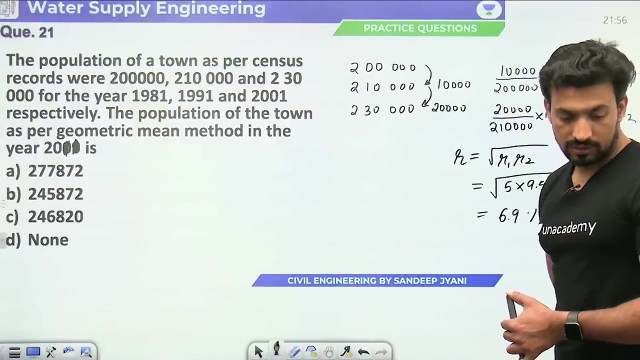 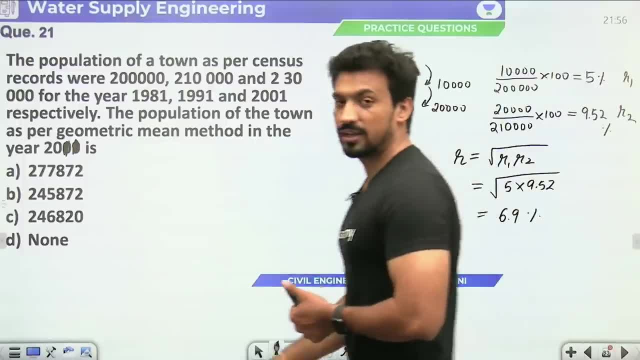 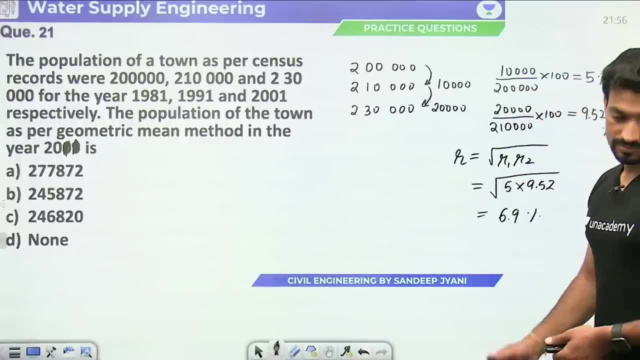 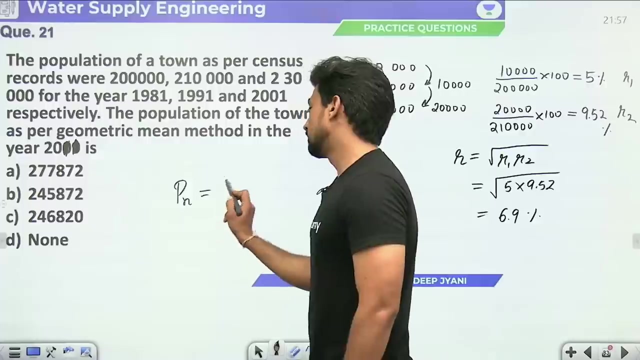 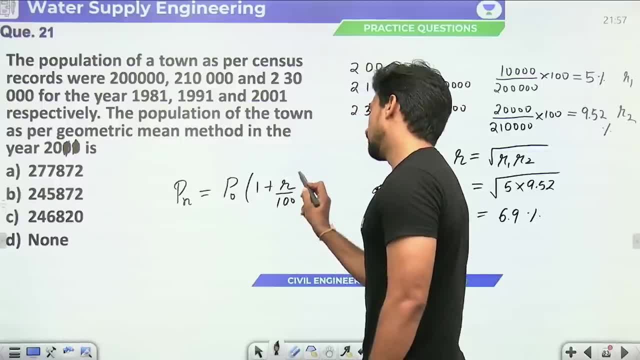 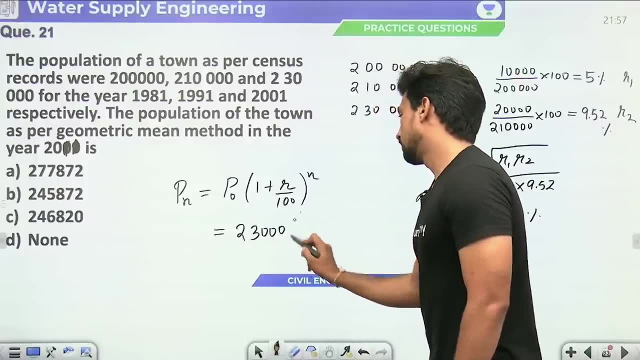 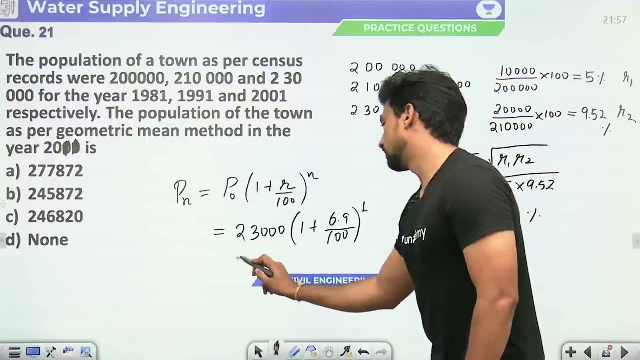 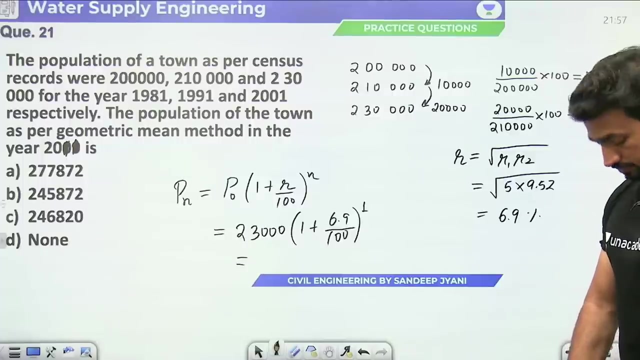 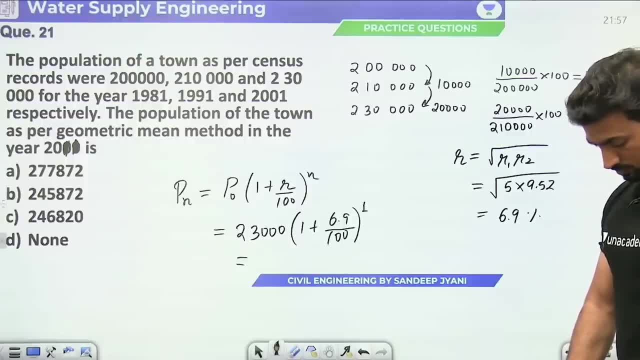 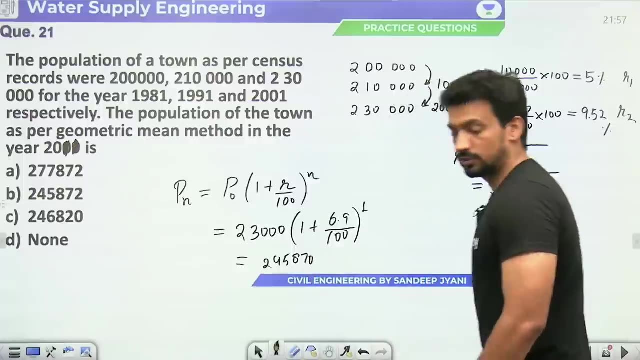 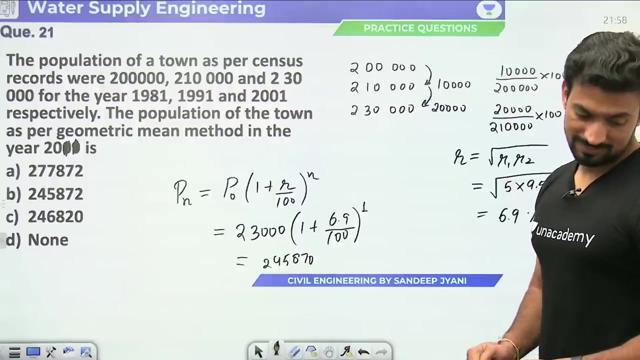 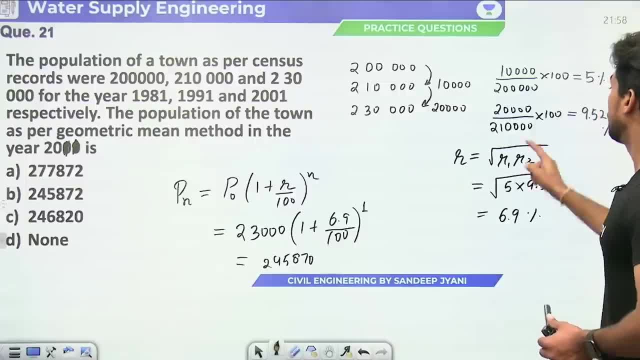 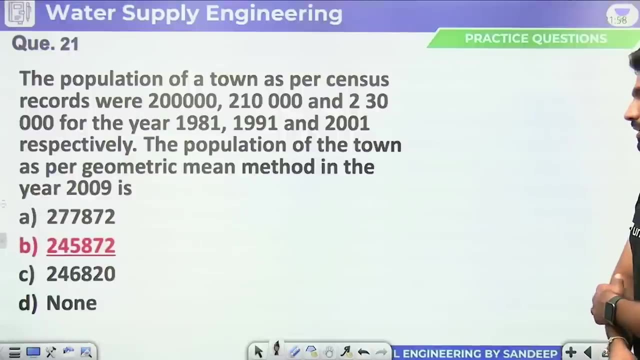 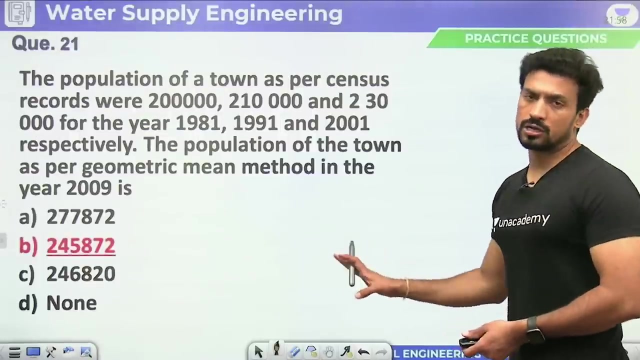 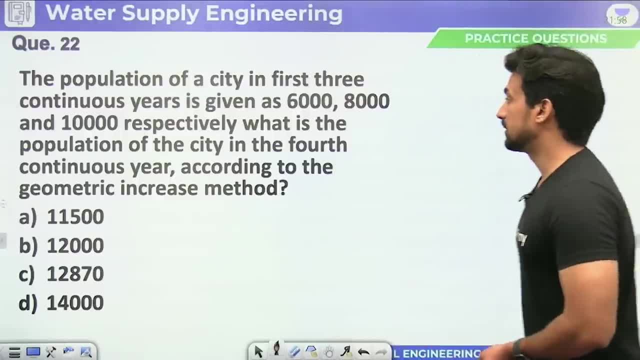 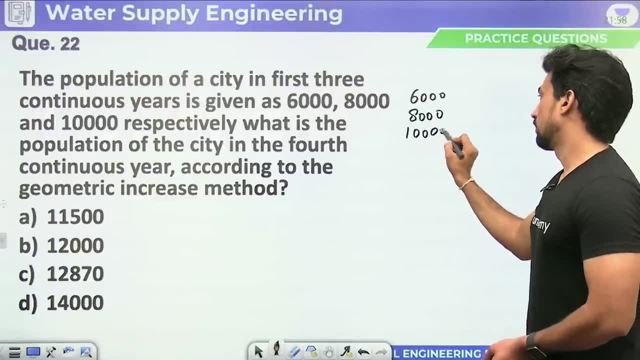 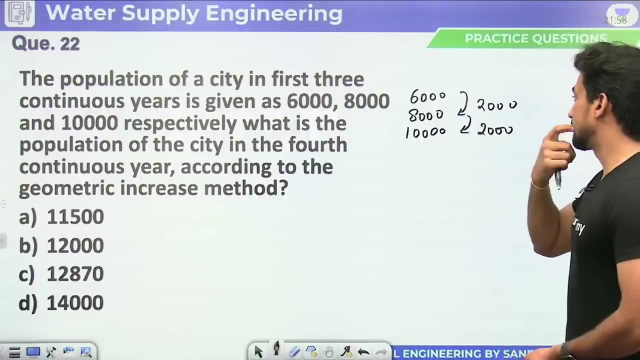 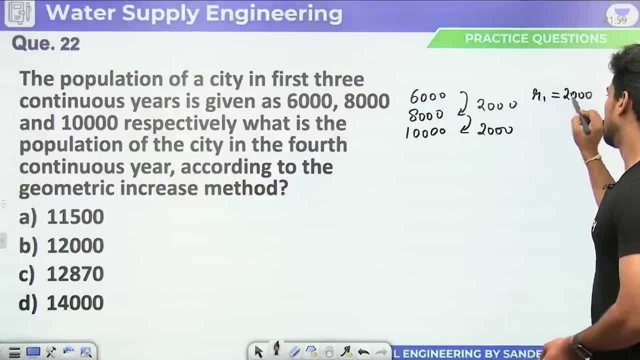 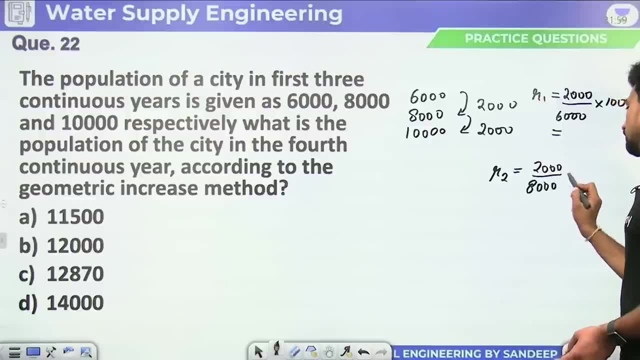 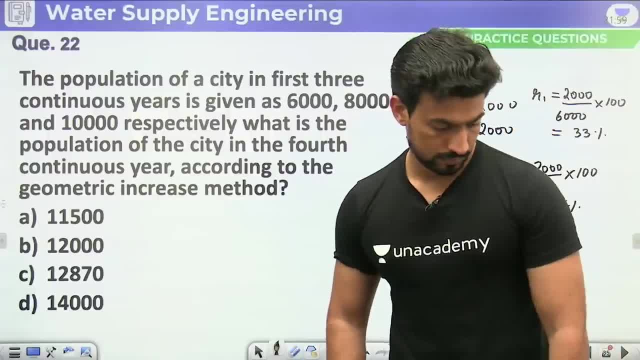 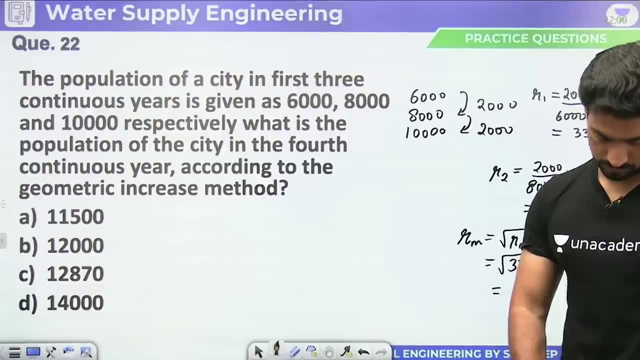 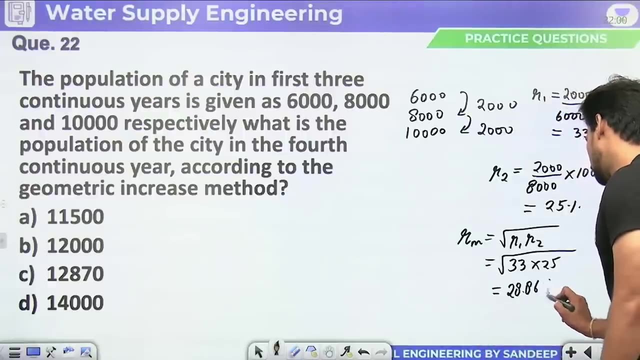 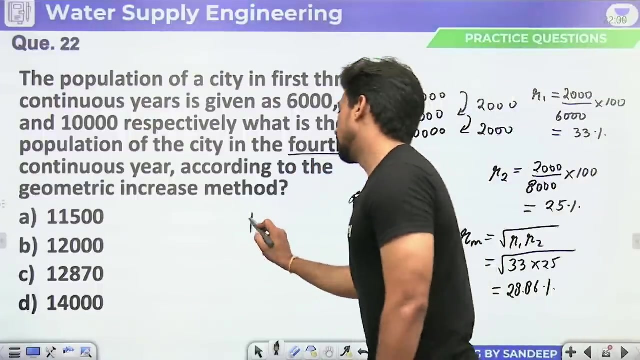 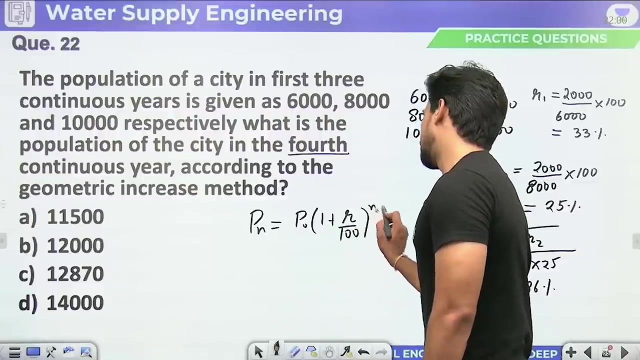 Confirmed, Confirmed, Confirmed: 28.86%. What is the population of the city in fourth continuous year? So we have asked you in one year only. Last known data is 1 plus r by 100, raised to the power n. 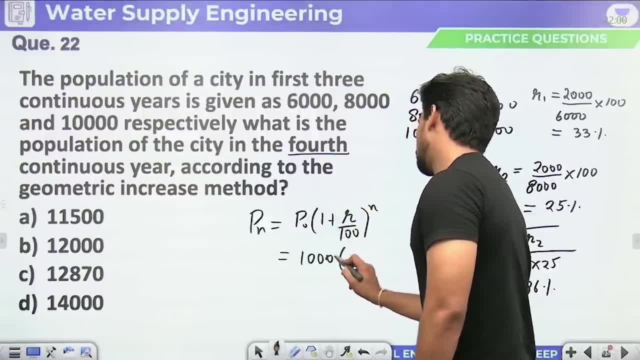 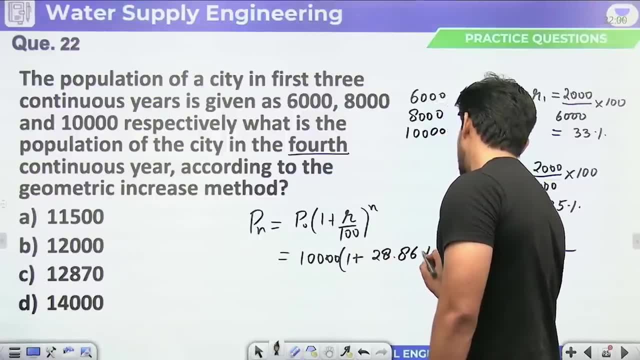 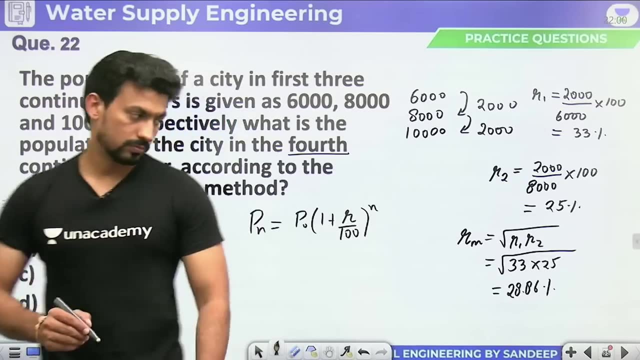 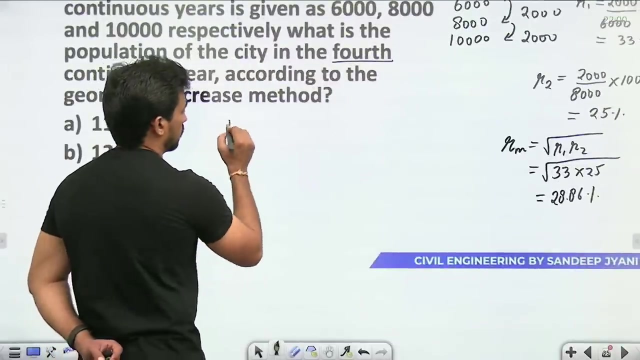 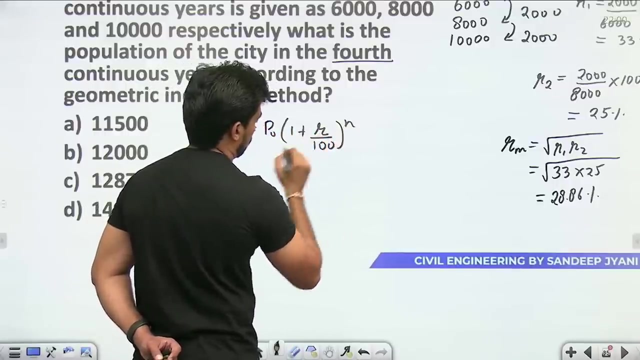 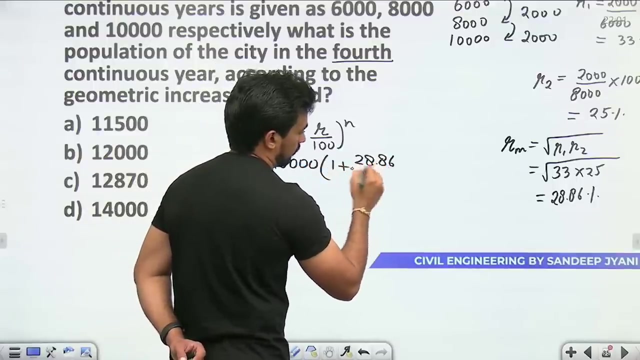 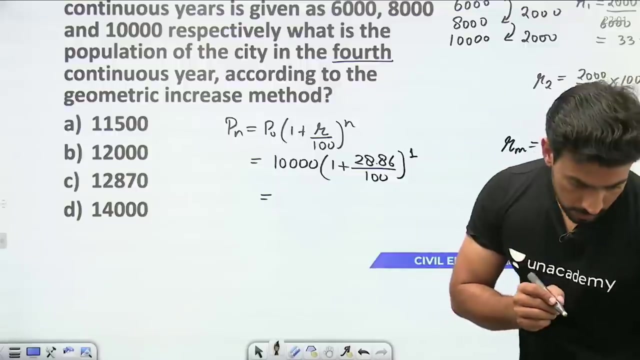 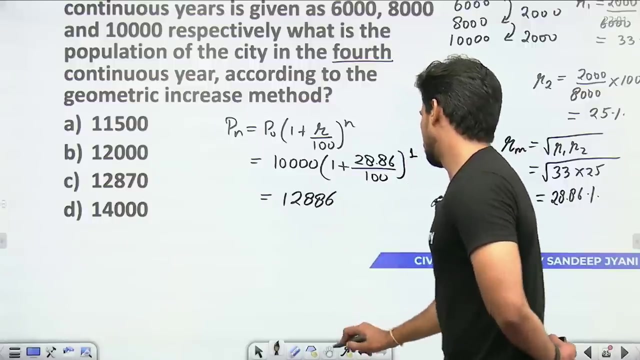 Last known data we have is 10000 into 1 plus r, value: 28.86%. So what is the population of the city in fourth continuous year: 12.886%. What is the population of the city in fourth continuous year? 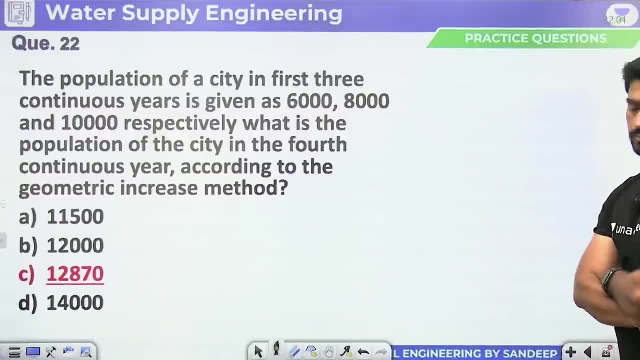 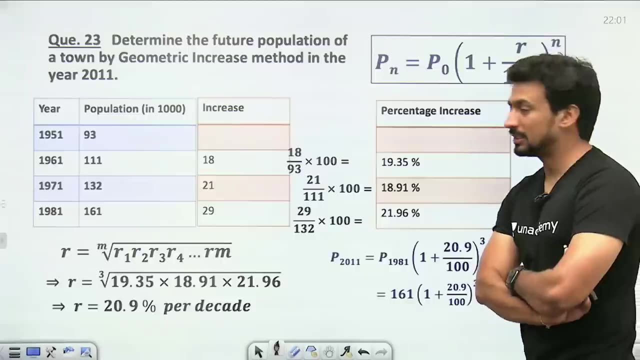 12.886%. Next, let's move on. So you have understood the geometric increase method. There was no need to explain in more detail. There was only this much maximum detail. We have to find the increase, Then we have to see the percentage of increase. 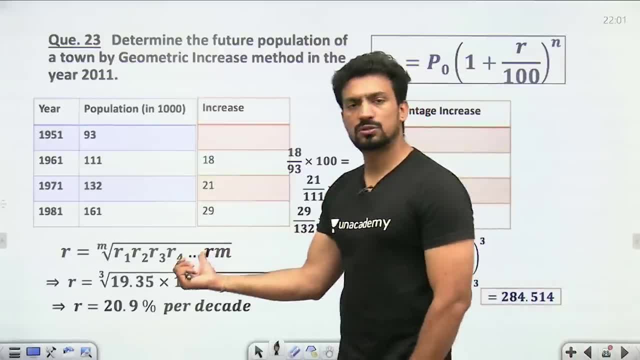 According to which how much increase happened. Whatever increase came then- r1, r2,, r3, r4 and so on- We wrote these values up to rm. Then we have to calculate their values here, Because there were only three values. then, in the case of three values, we will calculate. 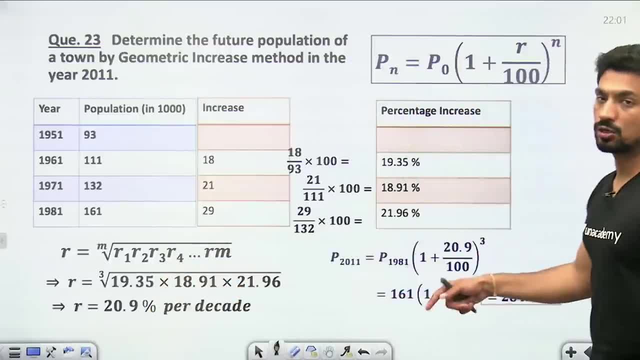 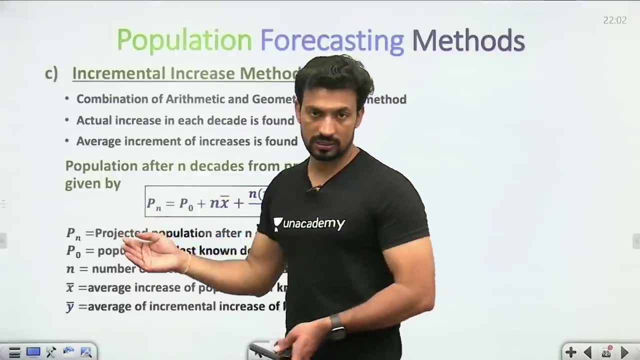 the cube root. So the value of r came. the value of r will be constant. I put it in this formula And you can find out. after all the decades, Incremental increase method comes a little more next level. It provides you the value between arithmetic and geometric. 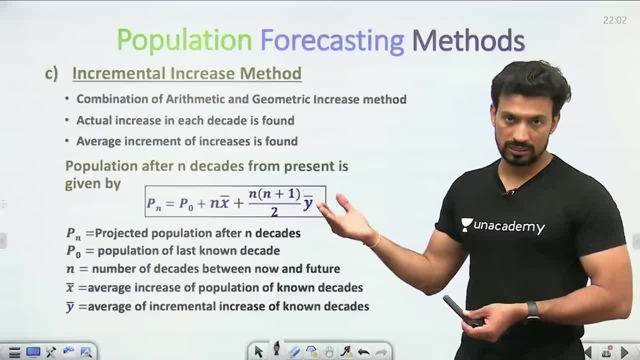 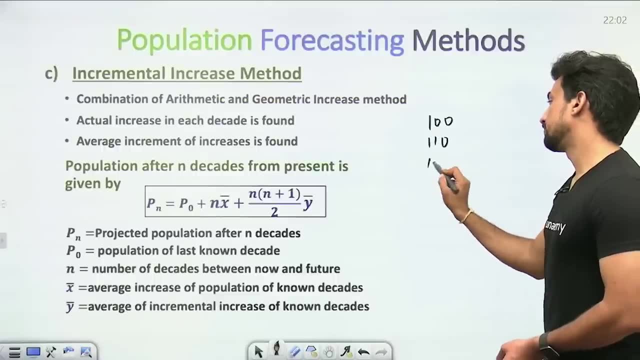 What you have to do in this case is to calculate the increase in the increase. Like today, your pocket money is 100 rupees, Yesterday it was 110 rupees, The day after it was 130 rupees, Then the next day it was 170 rupees. 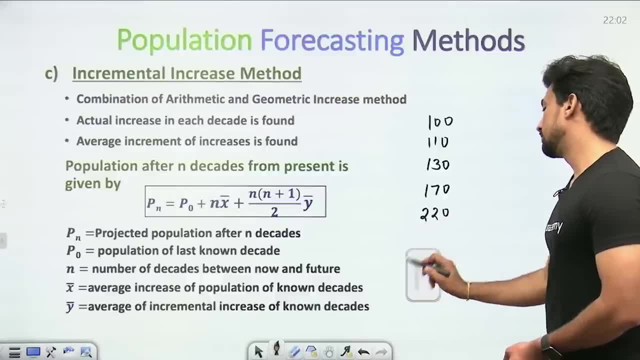 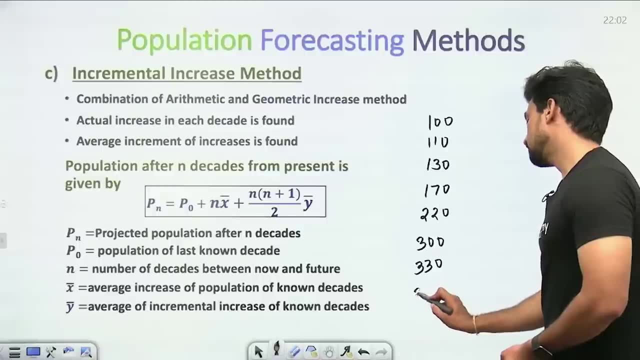 The next day it was 220 rupees, The next day it was 300 rupees, And the next day it was 330 rupees And the next day it was 340 rupees. So you saw how much increase came. 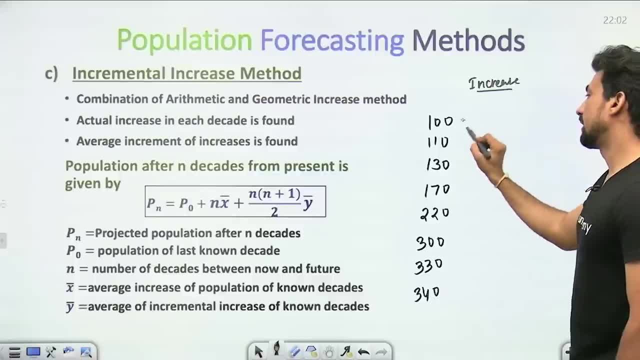 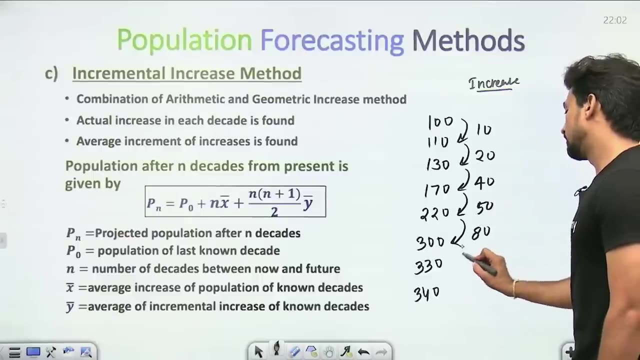 What did you see? How much increase came. So here came the increase of 10.. Here came the increase of 20.. Increase of 40.. Increase of 50.. Here came the increase of 80.. Here came the increase of 30.. 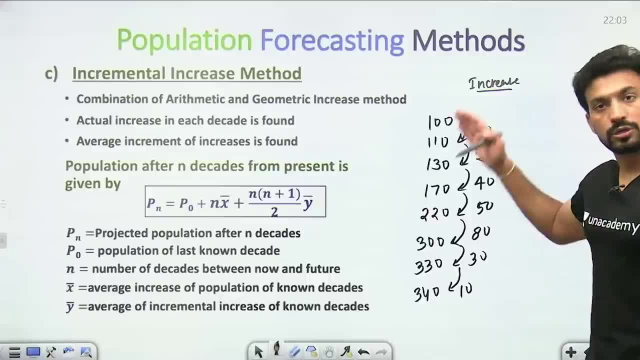 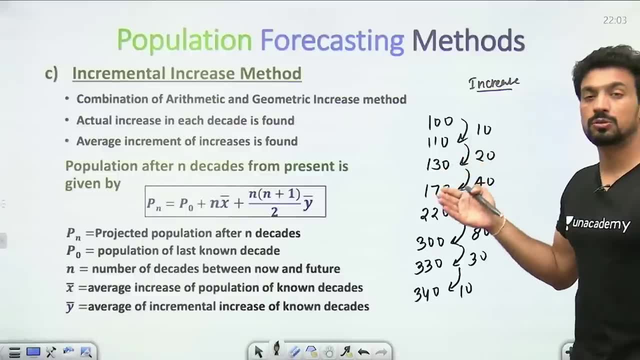 Here came the increase of 10. So the increase has increased. The amount has increased. Now, what was the increase in this increase? 10 to 10. Means on the first day you said that tomorrow I will get 10 rupees extra. 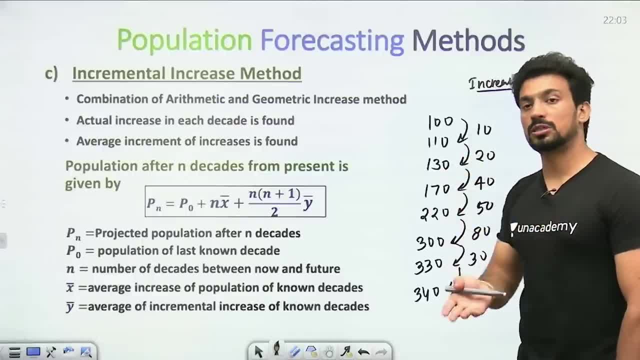 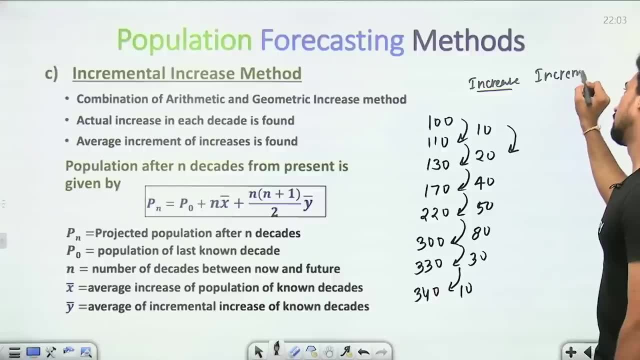 Then the next day you said that the 10 extra you got yesterday, you got 10 more extra than that. Increase to increase. So let's find out the incremental increase. What comes in the next step? In the next step, you find out the incremental increase. 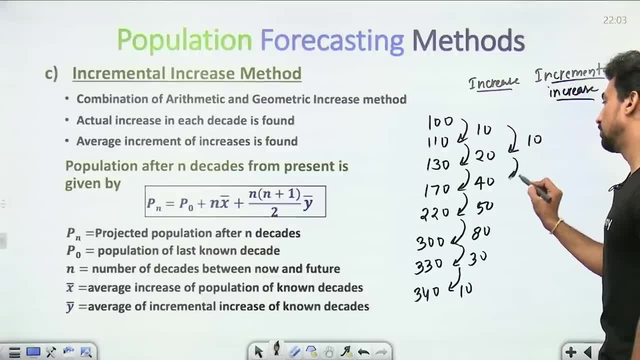 And that incremental increase 10 to 20.. How much increase? 10.. 20 to 40. What was the increase in the increase? It was 20.. Then what was the increase in the increase? It was 10.. 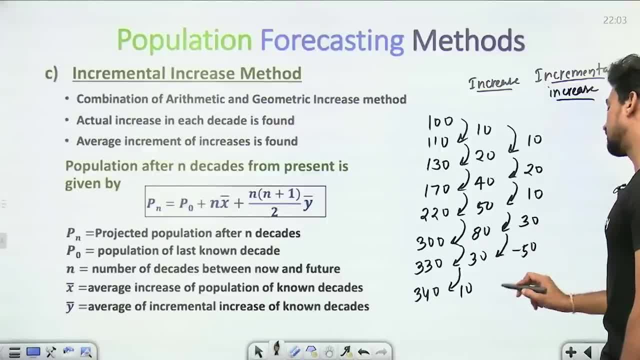 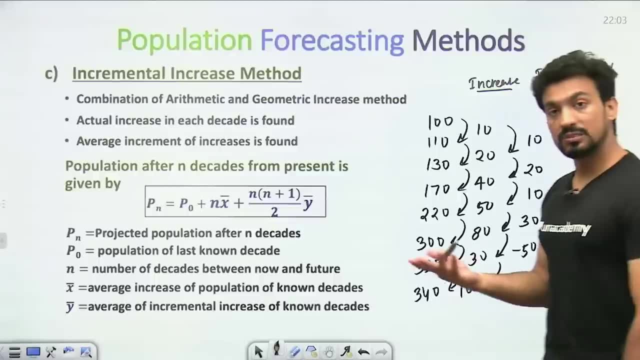 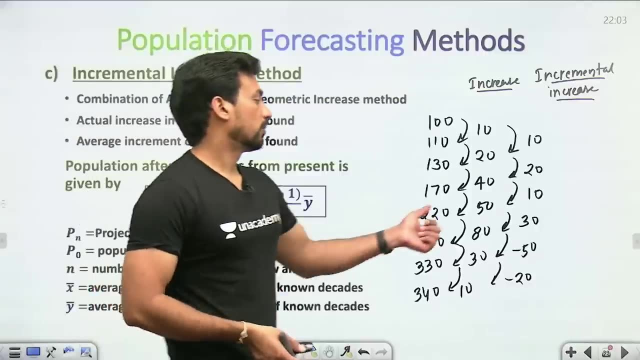 It was 30. But what happened here? Minus 50. Then what happened in the next? Minus 20.. There was a decrease in the increase. But what happened in the next? You thought that the money you got yesterday, you got 50, you got more than 80 today. 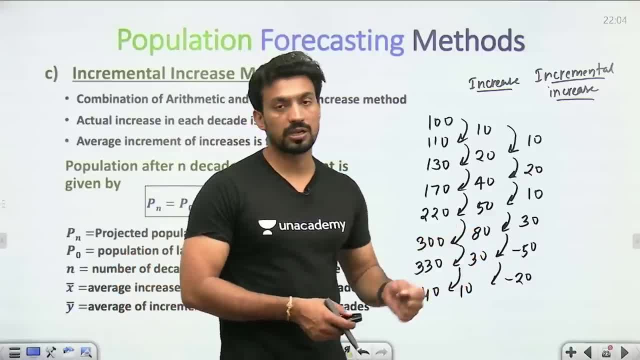 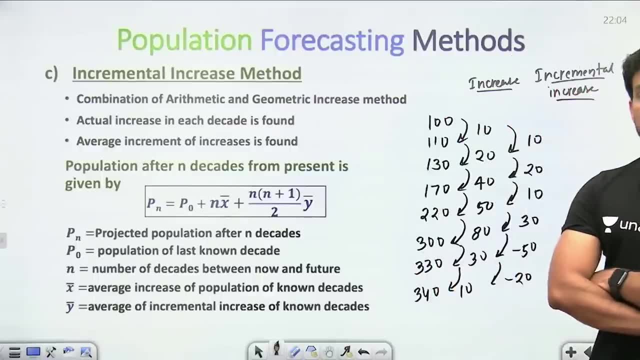 Next day you said that you got more than 30. So from the last day, you got less than 50. The increase that has happened: you got 50 less. So incremental increases can be positive as well as negative. What is the incremental increase? 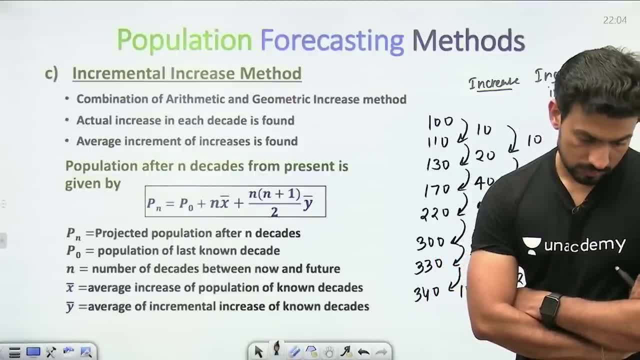 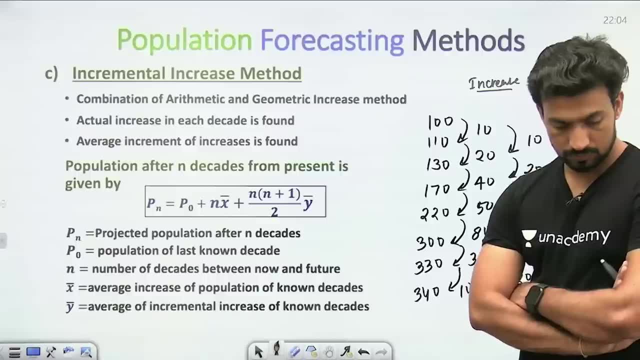 If it is positive, then it is negative. What is the incremental increase? The root of the value of r is the same as the root of the value of r. You have to find the increase in the increase. So let's find the increase in the increase. 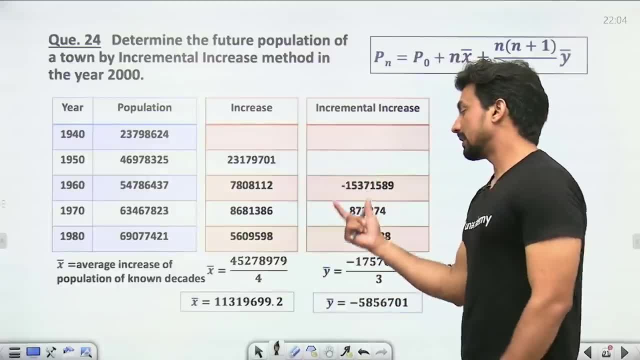 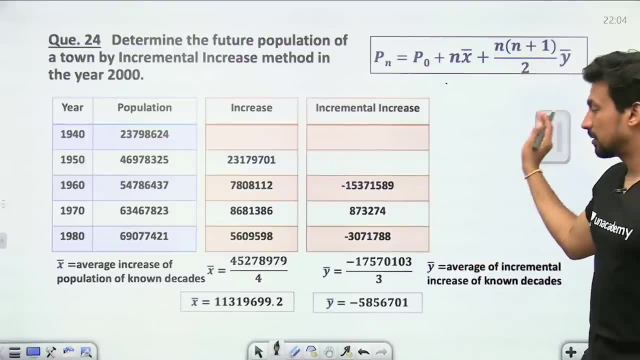 Then the average of the increase is x bar. The average of the incremental increase is y bar. The formula is p0 plus nx bar plus nn1 by 2.. nn plus 1 by 2 multiplied by y bar. So you can calculate this. 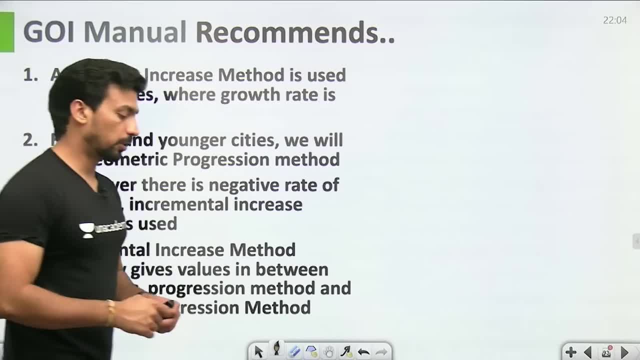 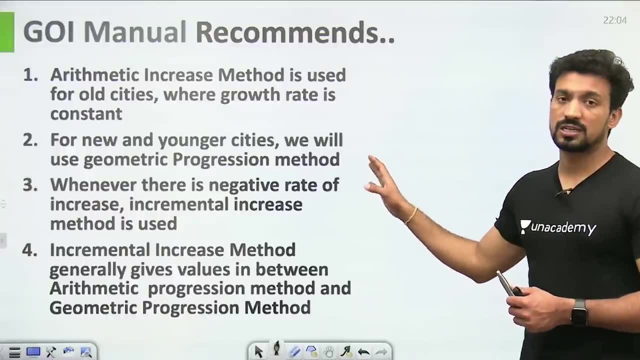 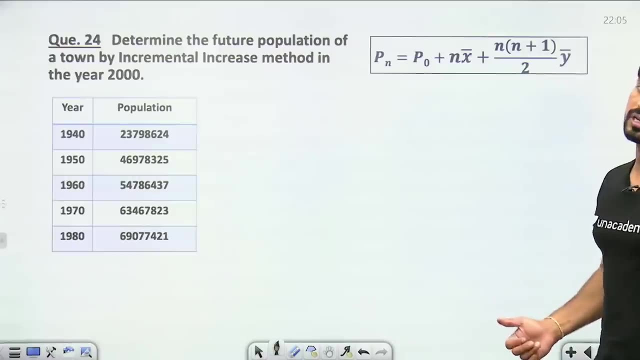 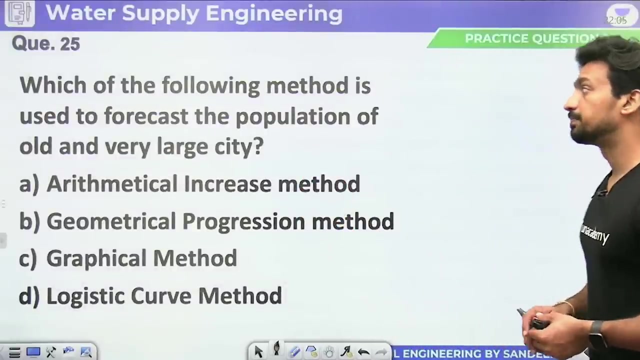 The government of India manual recommends you to use arithmetical mean method for old cities. Geometric progression is used for new or younger cities. Wherever the negative rate of increase is incremental, increase method will be used. This gives you the value between arithmetic and geometric progression method. 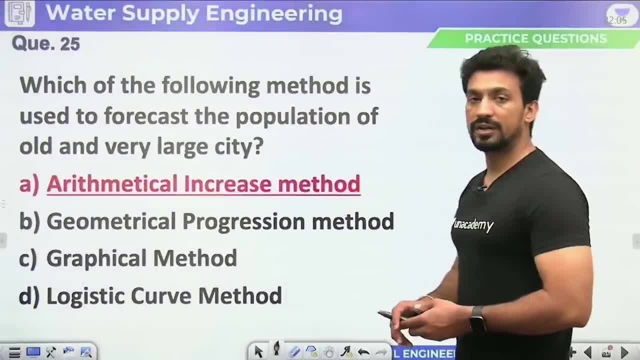 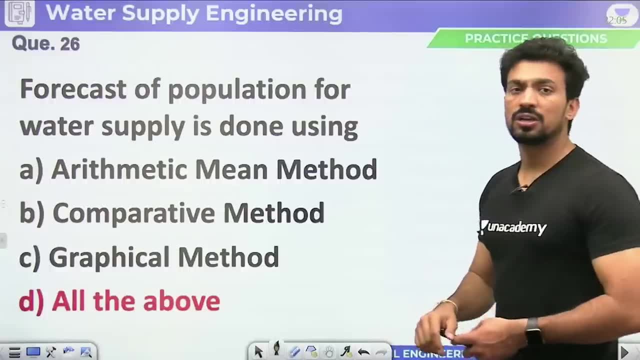 Which one of the following method is used to forecast the population of old and very large city. So Arithmetical increase method can be used. Forecast of population for water supply is done using, So arithmetic mean method, comparative. we have other methods. 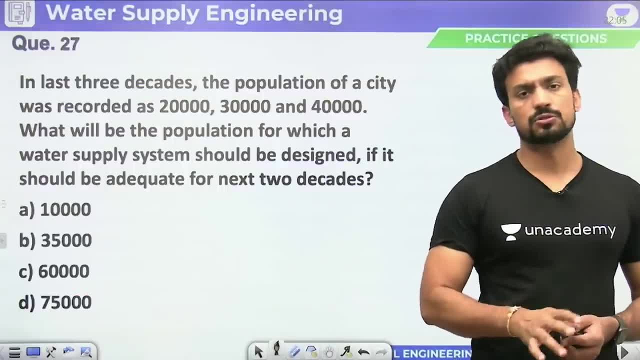 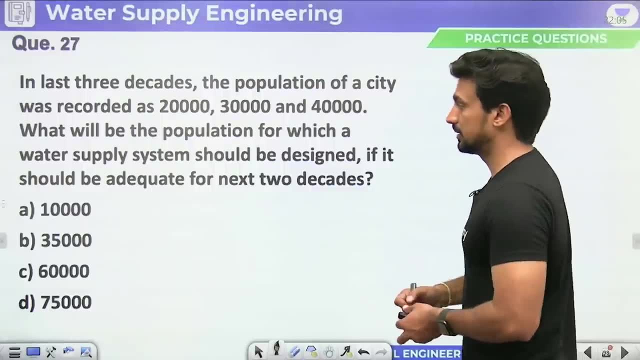 Graphical method, logistic curve method. we can use all these methods. Next comes: in the last three decades, the population was 20,000, 30,000,, 40,000.. What will be the population for which a water supply scheme should be designed? 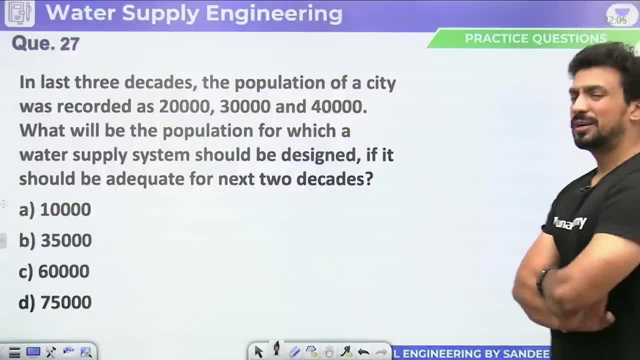 If it is to be educated for the next two decades. Next, we can calculate with arithmetic increase method: Average increase: see 10,000, 10,000, 10,000.. So what will be the population after two decades? 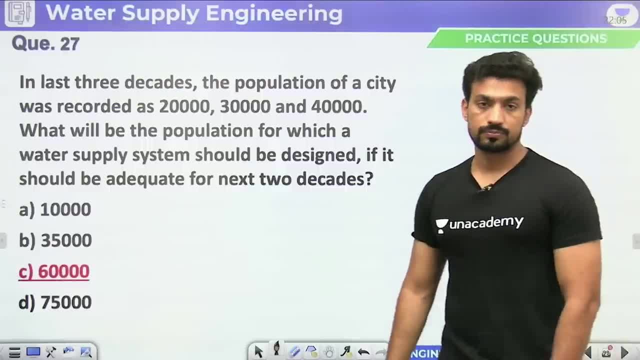 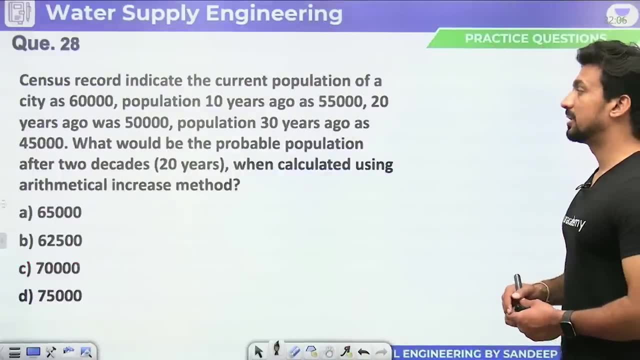 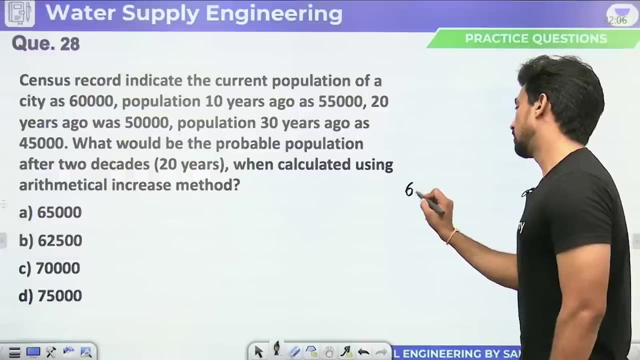 We will add and tell that it will be 60,000.. Next we have to tell you again with arithmetical increase method. Census records indicate the current population of a city as 60,000.. Current population: 60,000.. 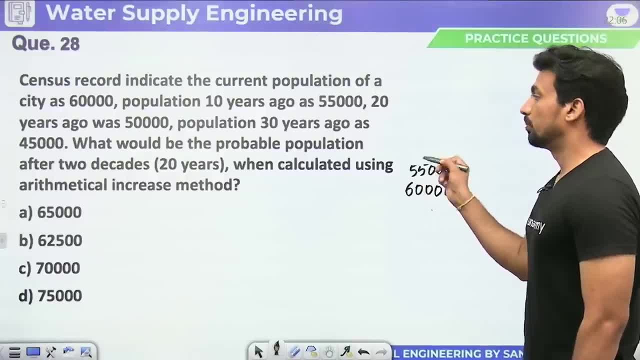 10 years ago 55,000.. 20 years ago, 50,000.. And 30 years ago 45,000.. Clearly it is visible that an increment of 5,000 has come. I have asked you after two decades, how much will it be after 20 years? 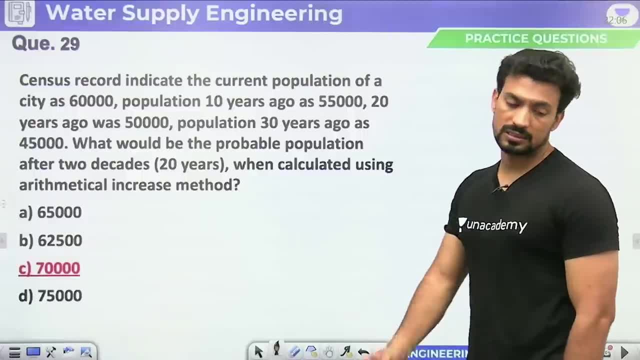 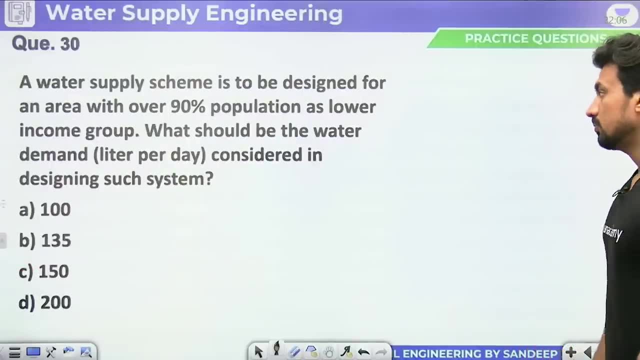 So 60,000, 65,000, 70,000.. The answer will come option C. Next, A water supply scheme is to be designed for an area with over 20,000.. 90% population as lower income group. 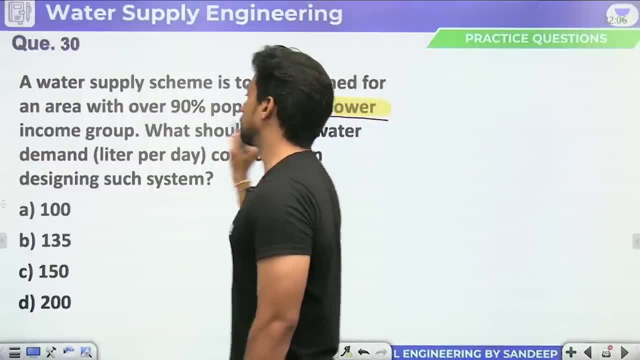 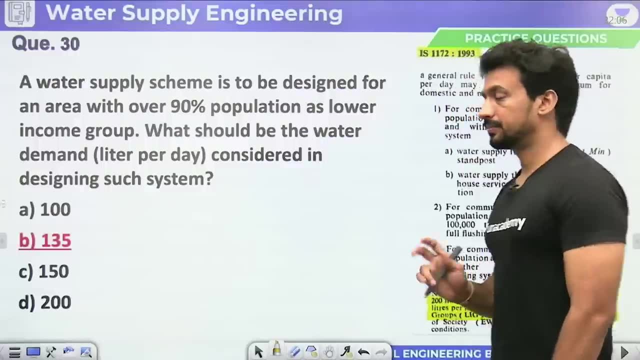 If we talk about LIG groups, then in the case of LIG groups, in the case of lower income groups, which is considered per capita demand, that 135 liters per capita per day is considered For communities with population up to 20,000,. 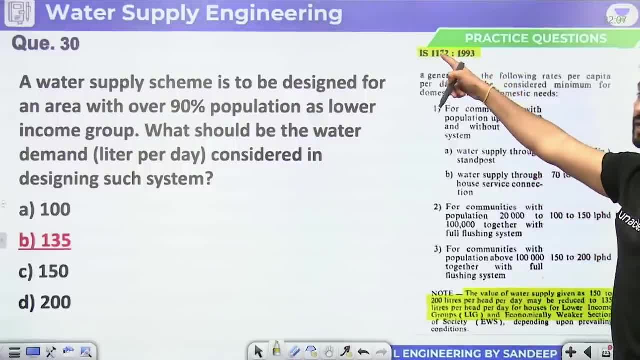 without flushing system, and according to whom is this being talked about? According to Indian Standard, 1172, 1993.. Although in 2012,, we are reaffirmed. now this reaffirming is going on of 2017.. 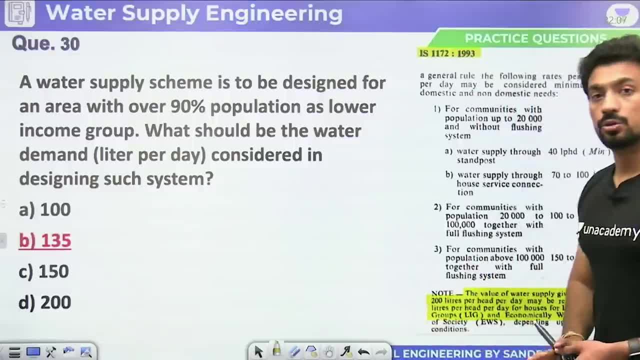 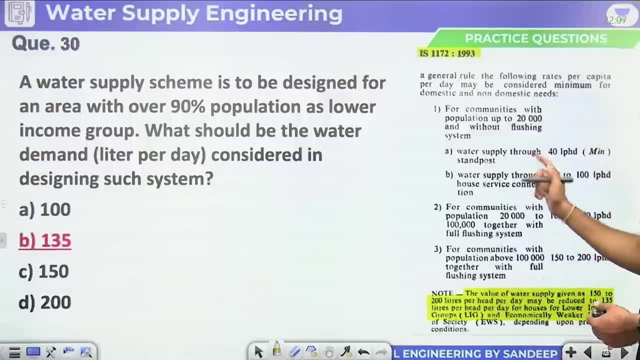 Again, it has been confirmed, things have been updated. So 2017, 1172, 1993, reaffirmed 2017.. Water supply through stand post. It has to go to a particular point and fill water and bring it. 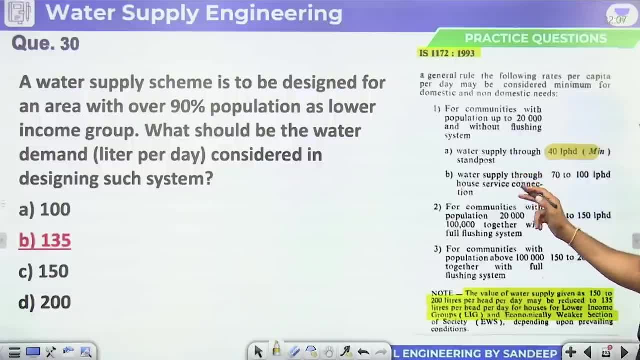 So 40 liters per head per day. Water supply through house service connections, So 7,200 liters per capita per day. For communities with population from 20,000 to 1,00,000, it is 100-150 liters per head. 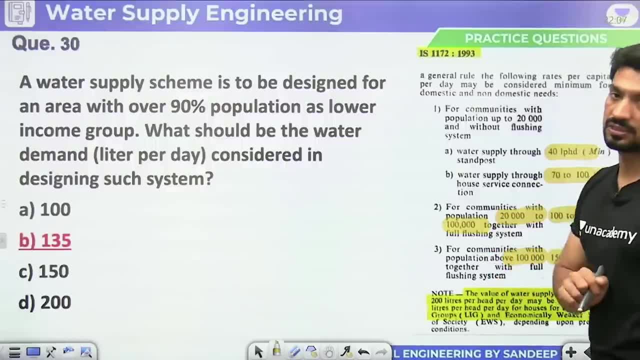 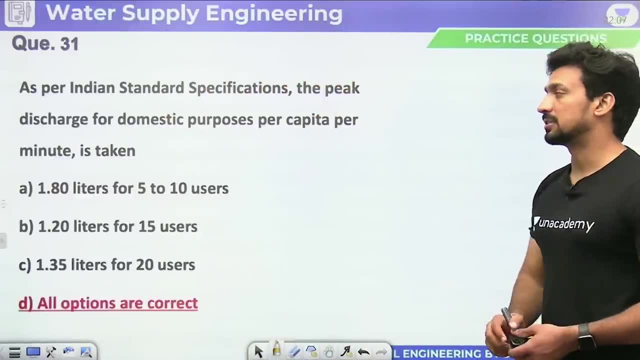 And above that, if the population is above 1,00,000, then 150-200 liters per capita per day will be considered As per Indian Standard specification. the peak discharge for domestic purposes, the peak discharge which is considered, is 1.8 liters for 10 users from Bhan. 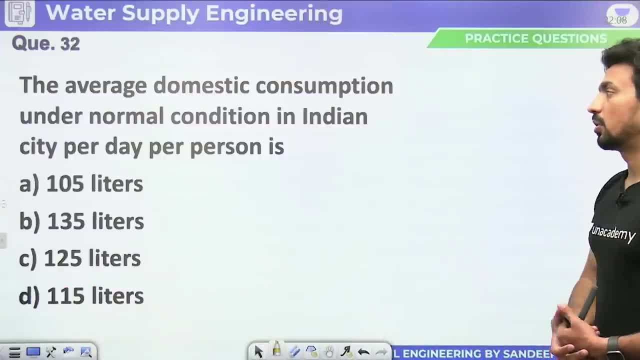 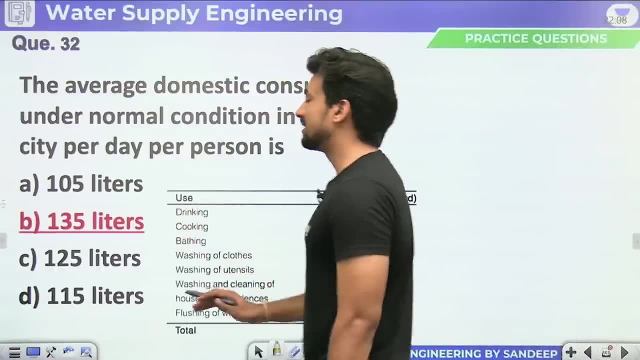 1.2 for 15,, 1.35 for 20,. all of the above options The average domestic consumption under normal condition. if we talk about normal conditions, then normal Indian conditions or LIG groups are being talked about here. 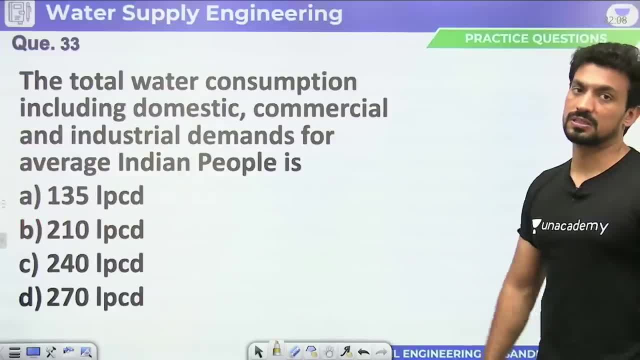 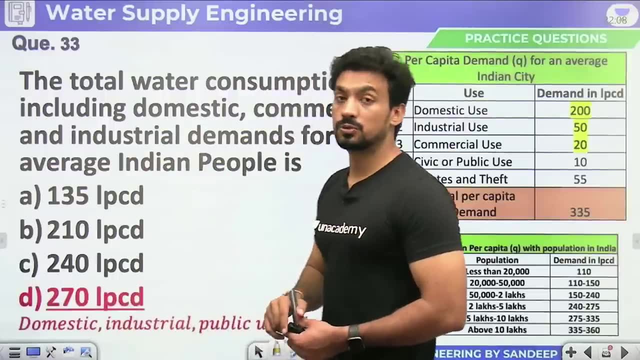 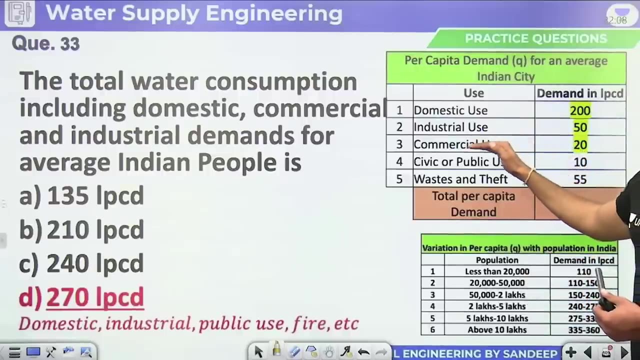 135 liters per capita per day. as per the given options, we can select Total water consumption, including domestic, commercial, industrial demand. Total water consumption, if you ask, then 270 liters per capita per day. you can consider out of which domestic, industrial and commercial. 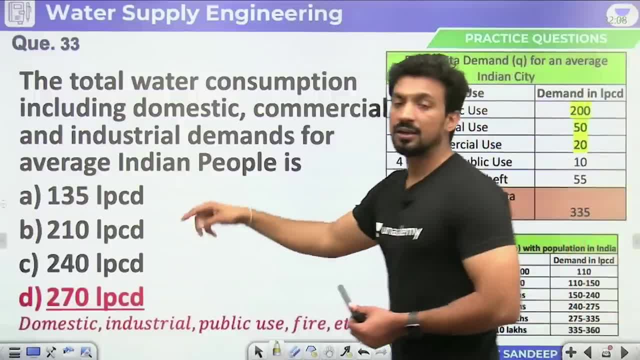 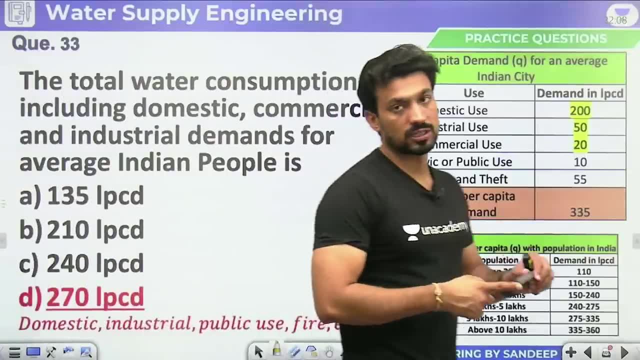 These three questions. If these three are asked, then we will tell 270.. If the overall is asked, then we can go up to 335.. Our answer is according to these, Because you were asked about domestic, industrial and commercial- The demands given here. 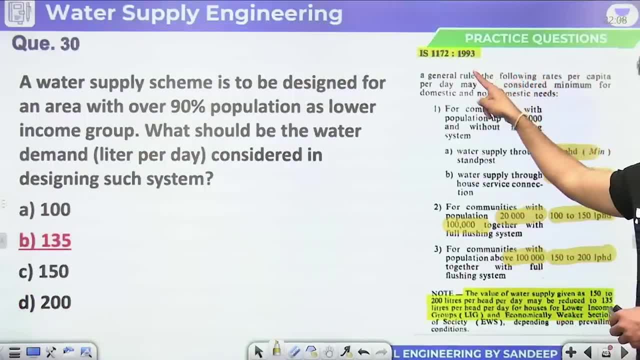 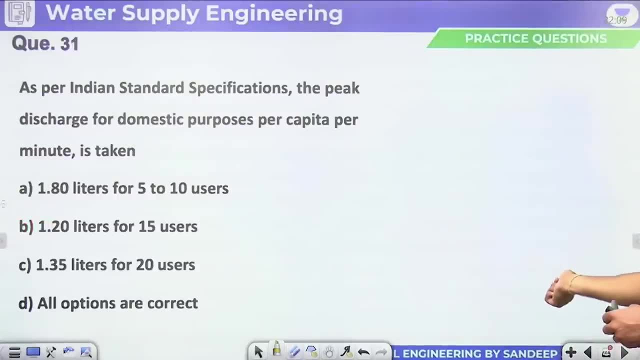 These demands have been given. A general rule has been given by the IS code 1172, depending upon the population. according to that, how much water will be given For domestic supply? we considered 200 liters per capita per day, 200 for domestic use. 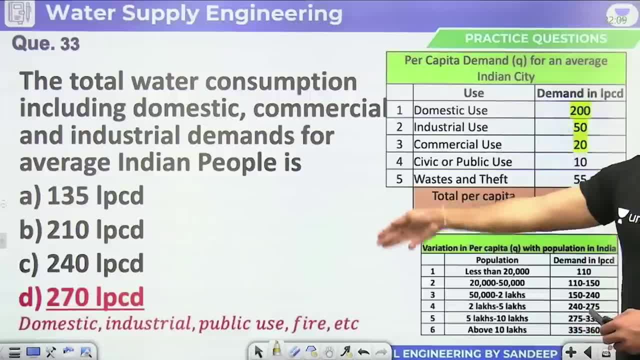 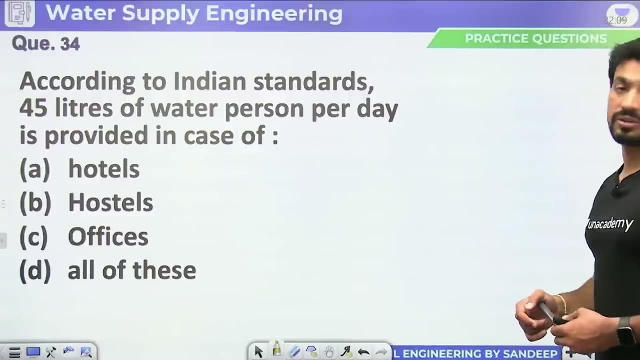 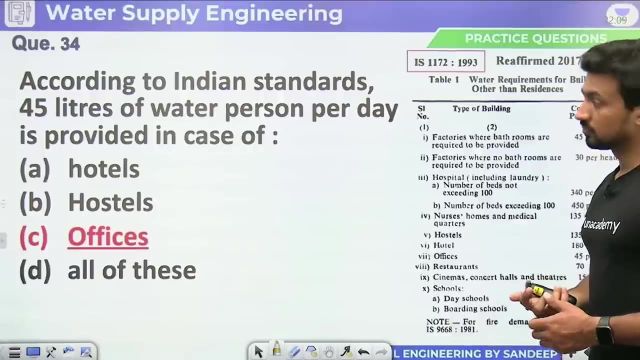 50 for industrial, 20 for commercial. Added all three, Our answer is 270.. Next, According to Indian standards, 45 liters of per person per day is provided in case of. We will provide in the case of offices. We will provide in the case of offices. 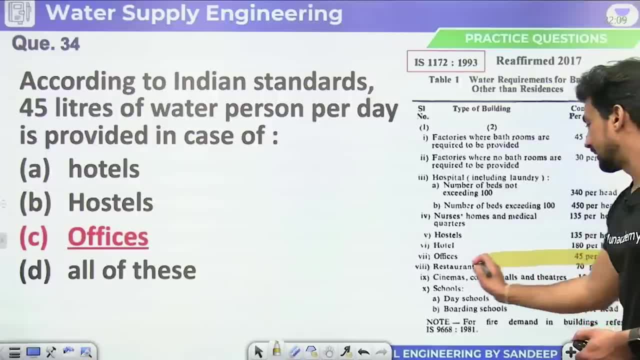 Ok, So now you can see that we have got our answer of 45 liters per head. This is 45 liters per head. I had told you in the starting that the hotel man said that the government of India Manual according to this the value of the hotel. 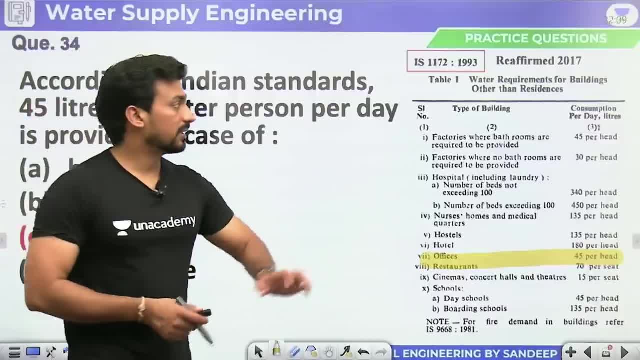 wait for a few minutes, we will give you the answer. Look at this Now. you see this. The values are called IS-1172.. All these values And, in the beginning, the code that we had read In the starting. 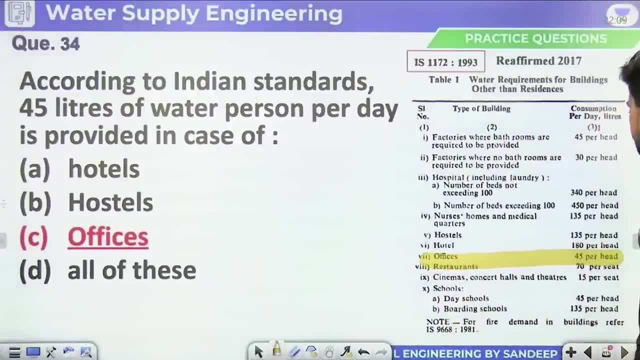 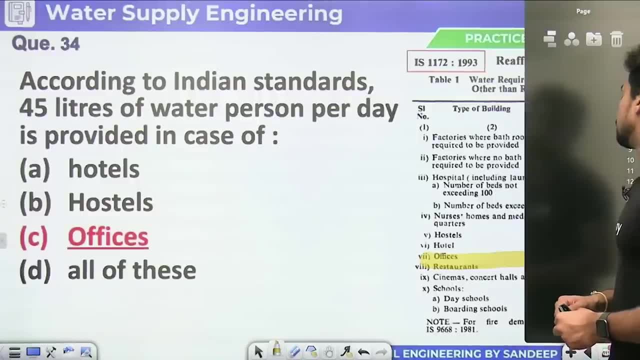 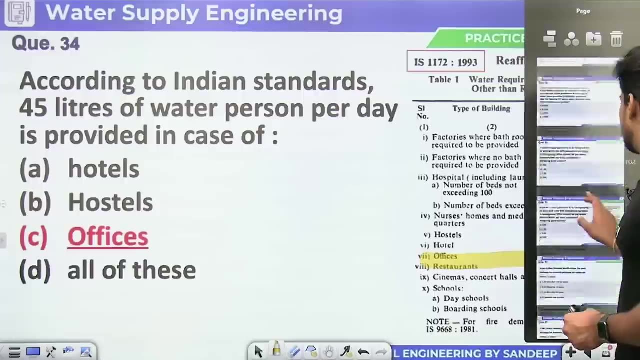 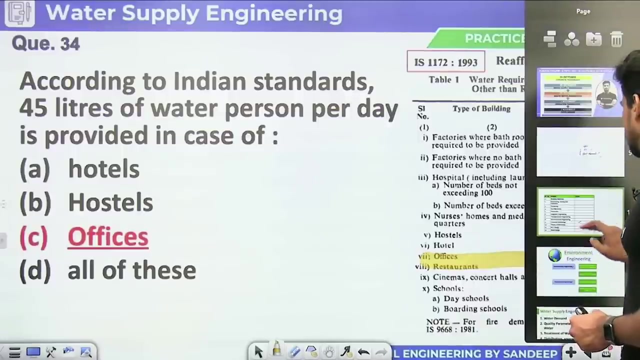 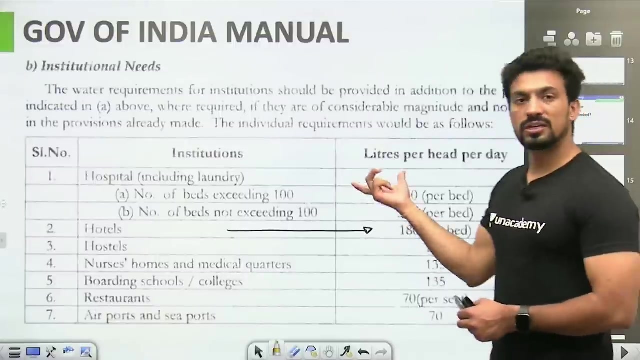 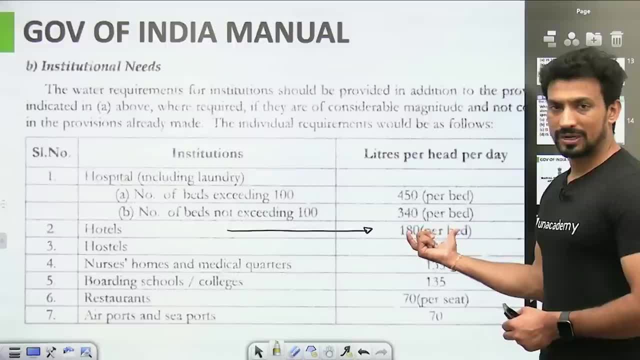 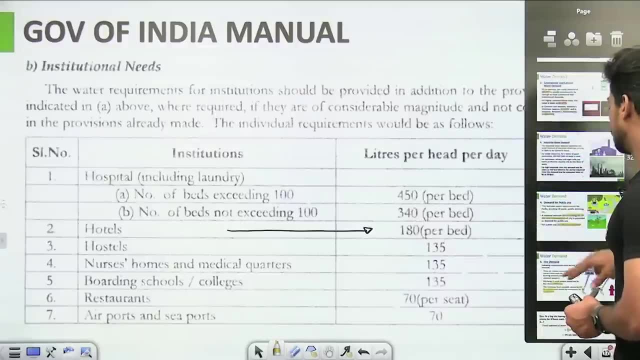 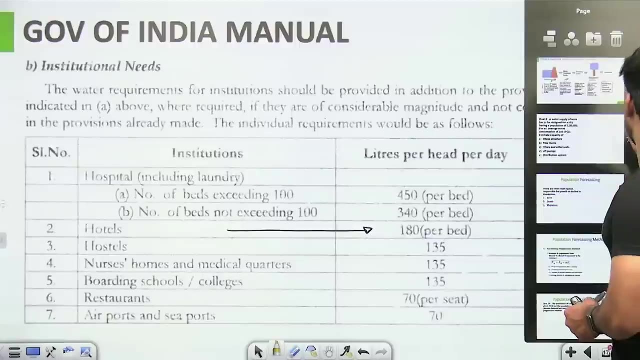 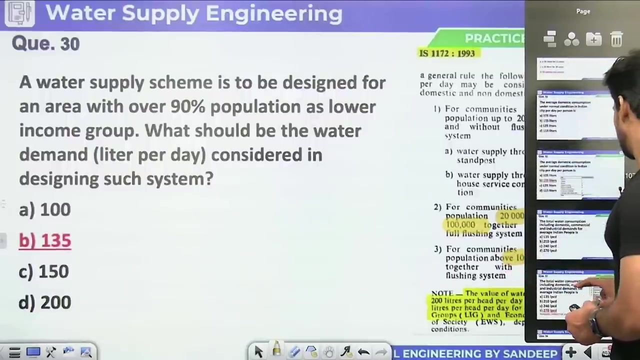 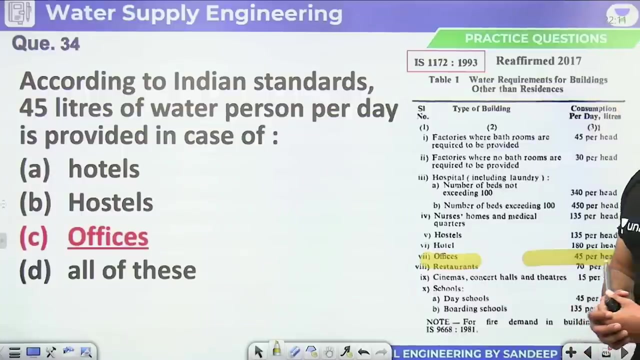 things in this way: 180 per bed. so almost the values come out there. only You will get to see a lot of changes somewhere in this. So for offices I asked you 45 per head. Now these things will not come suddenly. Just keep watching through questions. 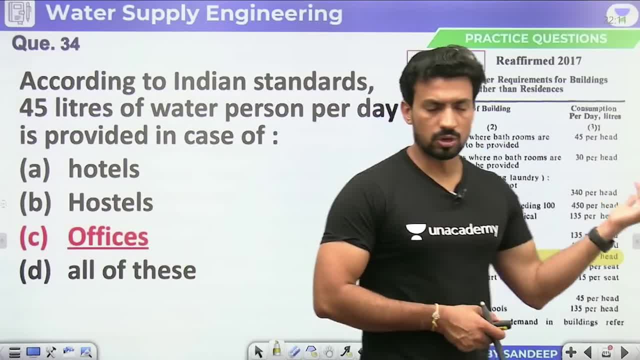 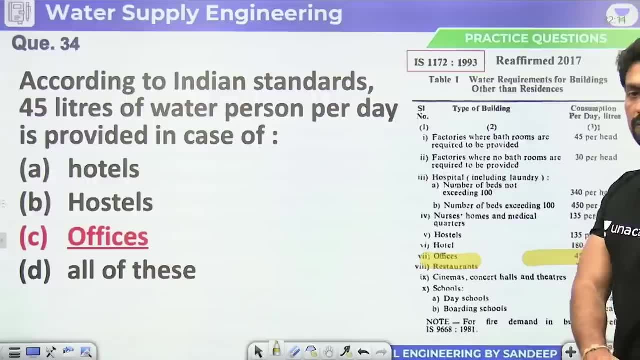 Once you see a question, you see a question again. if you see someone else for the third time, then in such a case you will start remembering easily: Was it 180? for hotels, There is a difference between a hotel and a restaurant. 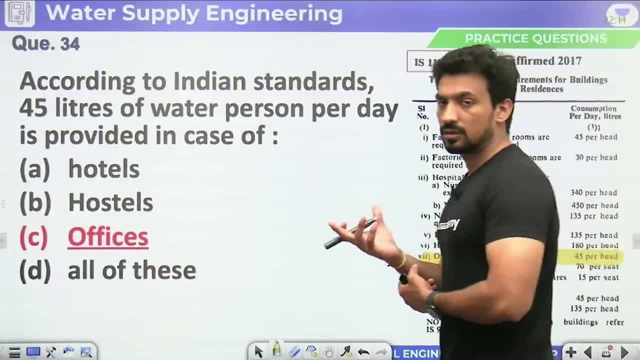 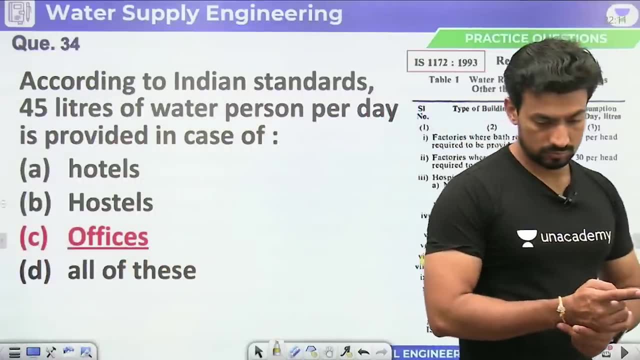 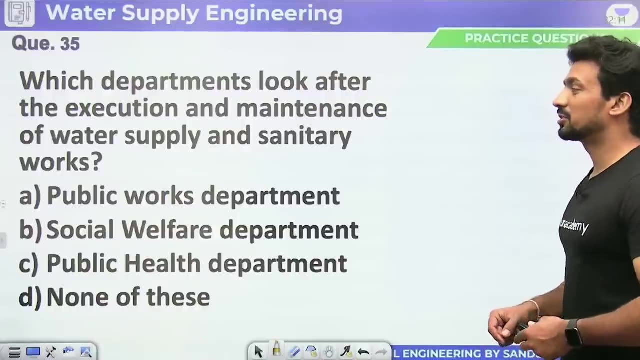 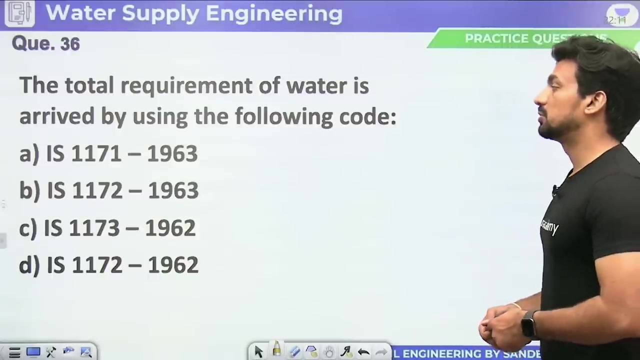 The hotel is where you stay. The restaurant is where you particularly go to eat. Let's move on. Which departments look after the execution and maintenance of water supply and sanitary works? Public health department or PHED department? The total requirement of water is arrived using the following code: 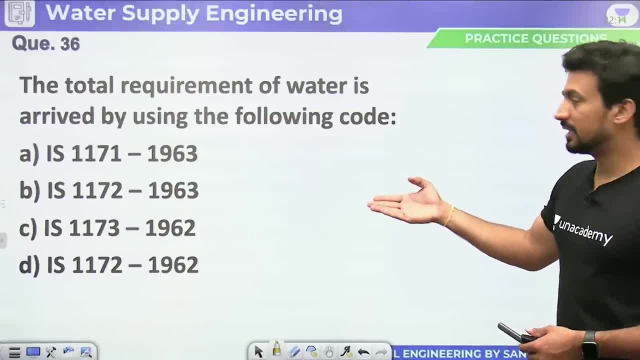 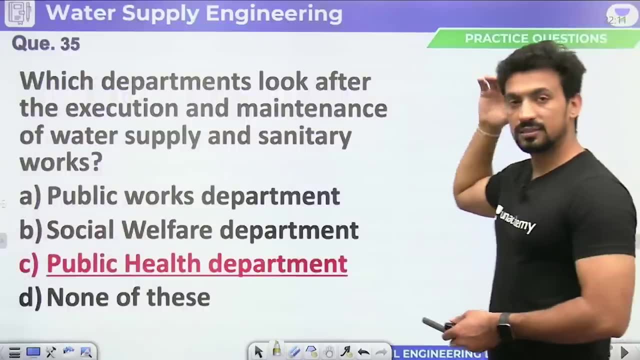 So which code do we use? This question is very old. That's why it has 1172-1963 in it, Whereas we are just seeing 1172-1993 has come. Okay, 1993 had come in 3.. 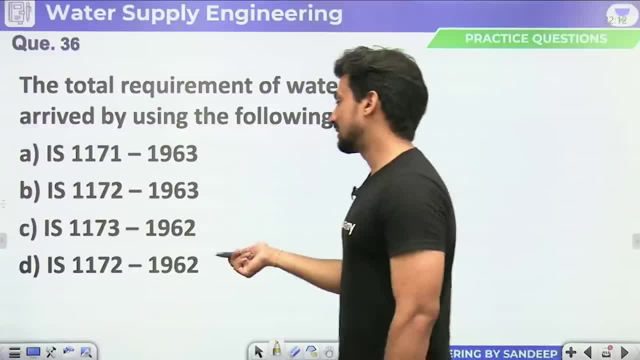 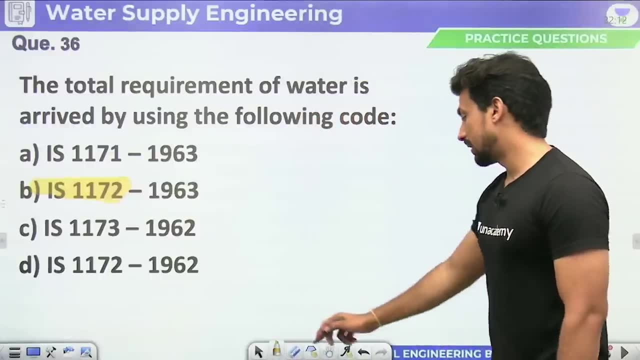 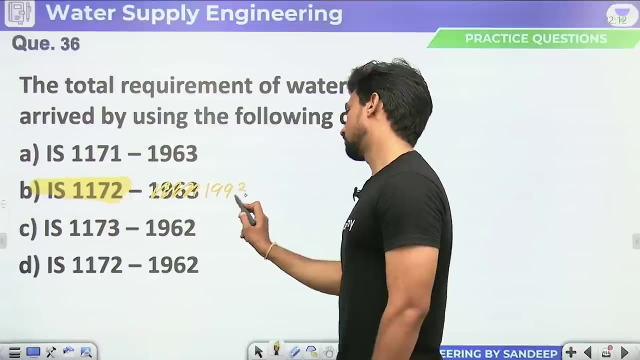 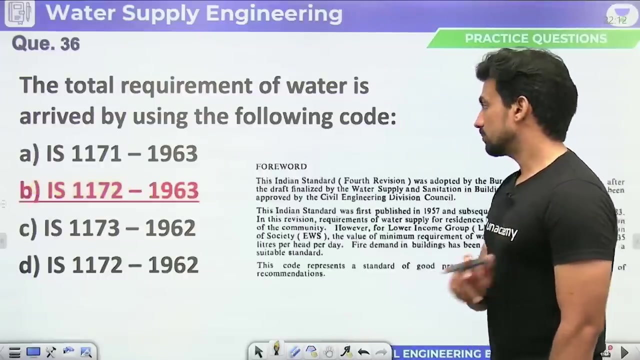 Reaffirmed 2017.. So the question was given like this. Just remember this: You have to choose 1172 and 1993.. The equation is old. The book is running in the same way. Next, The total requirement of water is 1172-1993.. 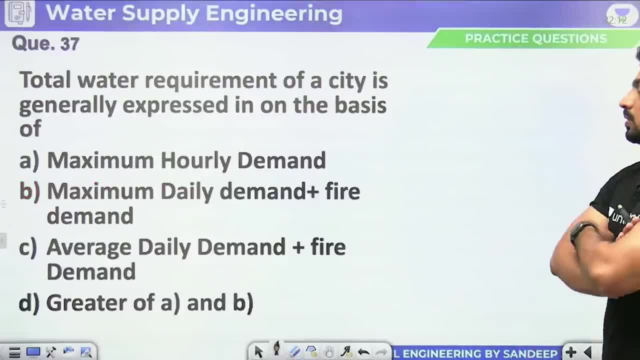 That's why it has 1172-1993.. That's why it has 1172-1993.. That's why it is 1172.. The total water requirement of a city is generally expressed on the basis of total water requirement. The question has come first. What is included in the water supply Ratio between peak hourly demand and maximum daily demand? So 1.5 hourly variation factor. Peak demand of water varies from 2.5 to 3.. If the annual average daily water consumption of a city is 48000 cubic meter, 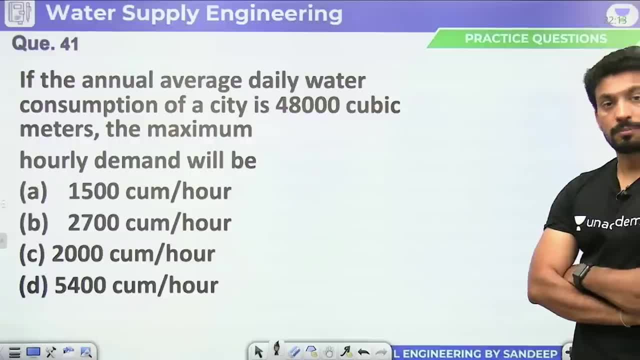 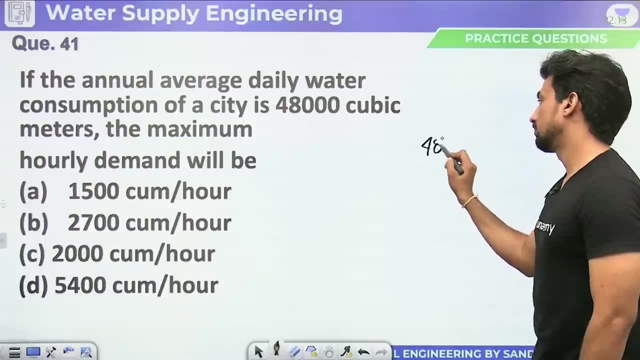 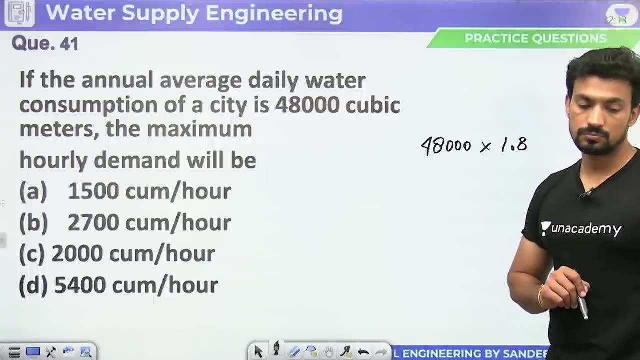 The maximum hourly demand will be. If you have asked the maximum hourly demand, What do you have to tell? Average daily demand is 48000. If I multiply it by 1.8.. So what will be yours? 1.8 to maximum day. 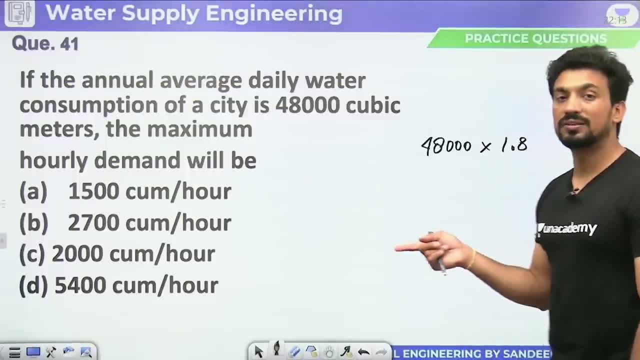 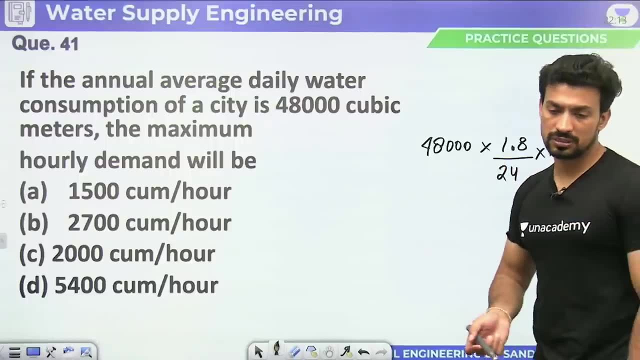 Then if you have to go above the peak demand, So from 1.5.. But according to the hour he said, So 24.. Or 2.7.. Or multiply it by 2.7 and divide it by 24.. 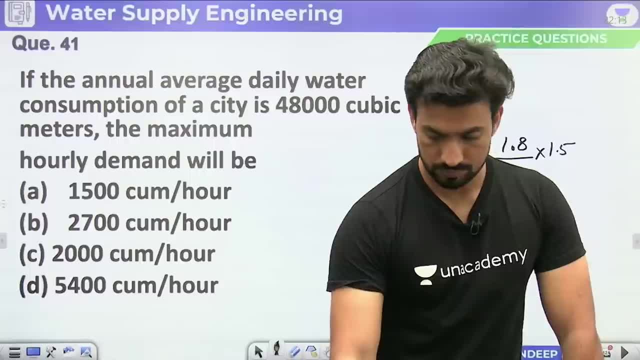 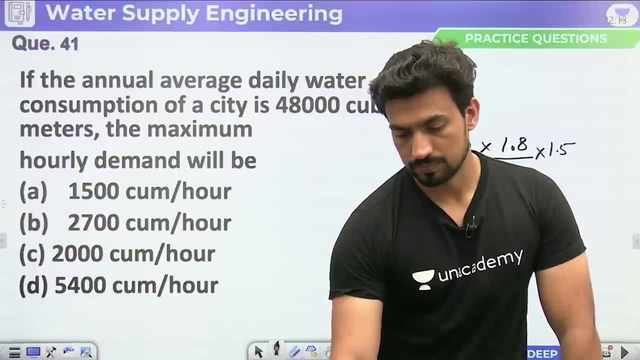 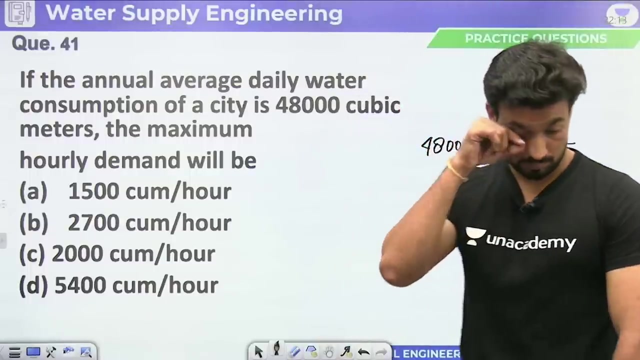 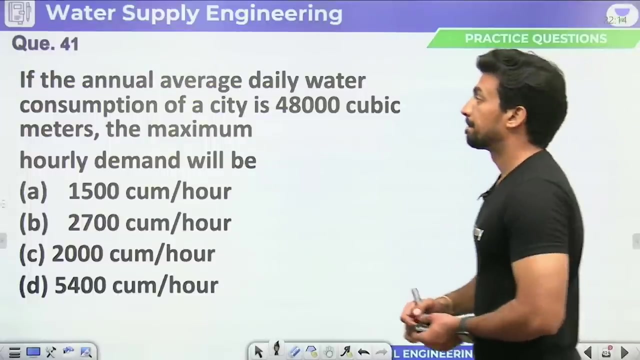 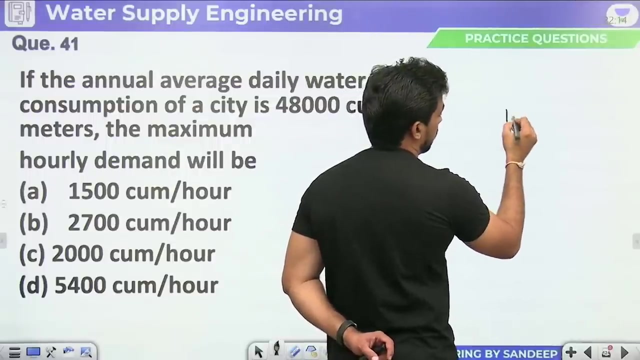 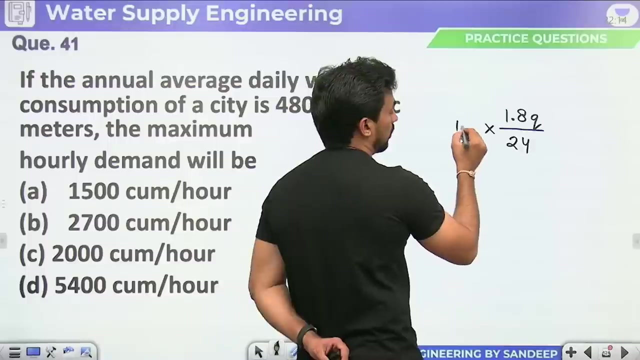 As you feel suitable. How much will be the answer? See, You were given this That 1.8q has come Maximum daily demand, Divided it by 24.. So how much will be coming on that maximum day in an hour? 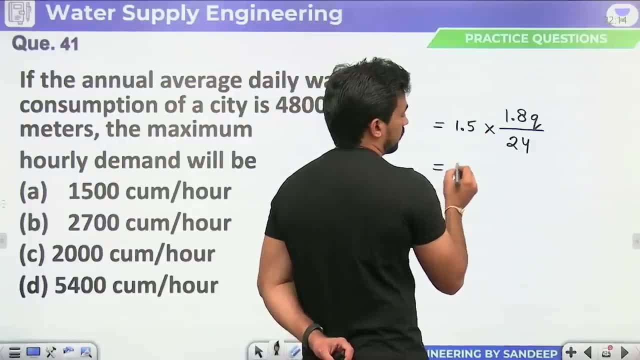 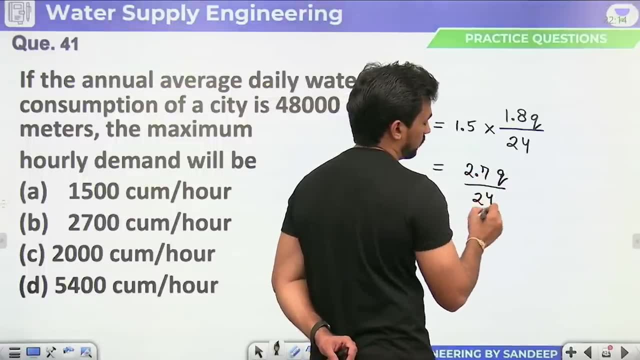 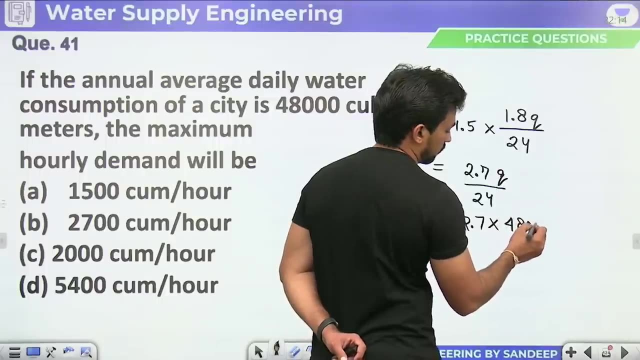 And multiplied it by 1.5. So peak demand 1.5 into 1.8q became 2.7q. 2.7q by 24. 2.7q value is 48000. By 24.. 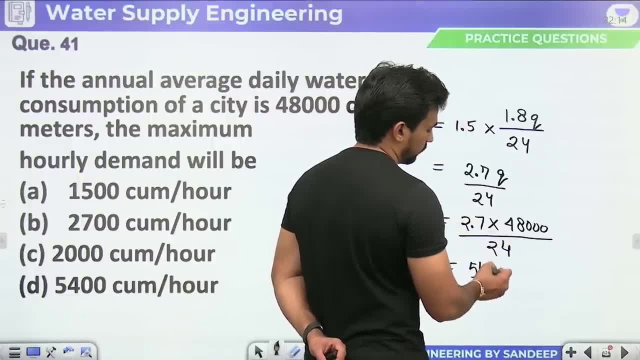 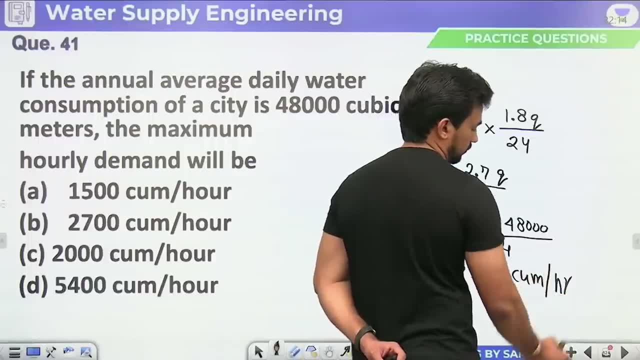 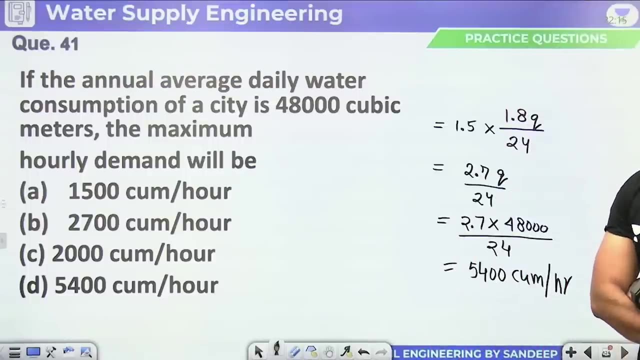 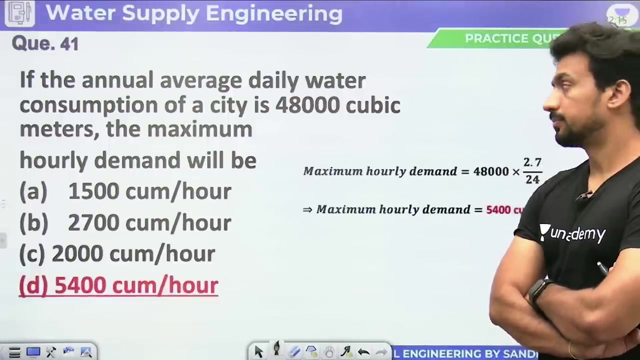 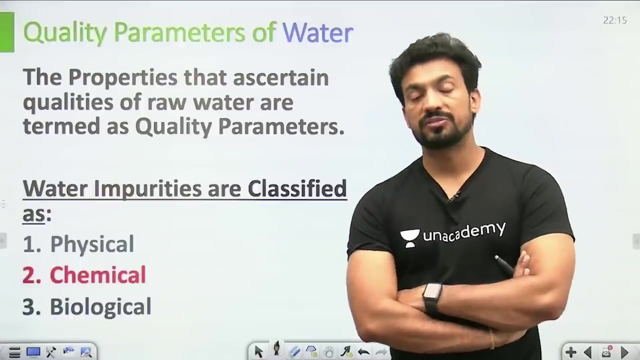 So you will get 5400.. In liters or cubic meters, 5400.. Next, Quality parameters of water come up. In the quality parameters of water We have kept three types of parameters: Physical, Chemical, Biological. According to them we have decided their impurities and their parameters. 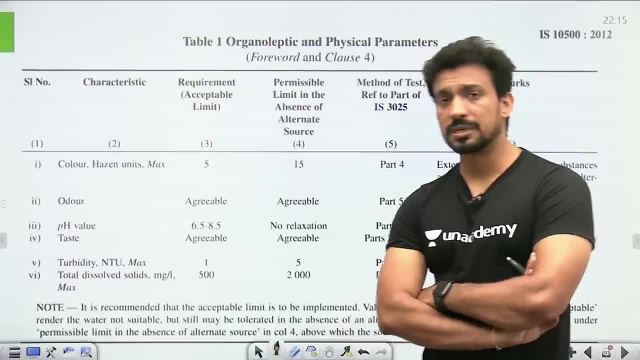 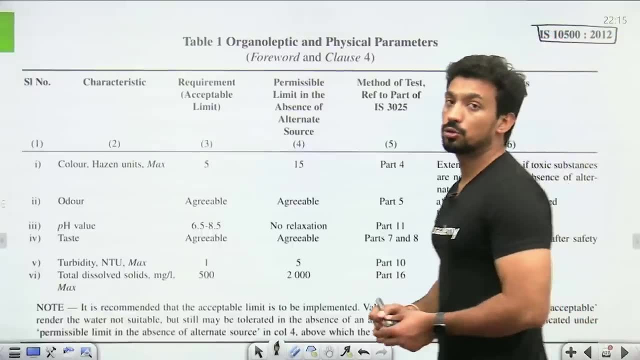 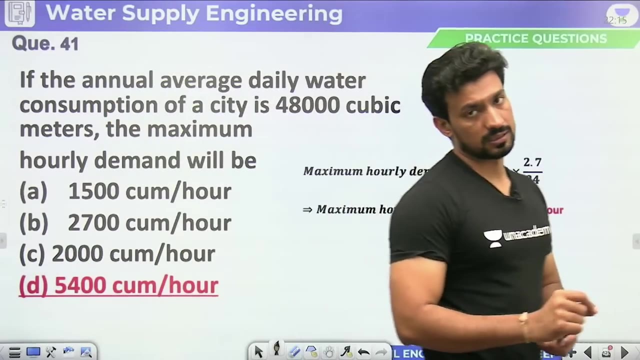 Who told us the parameters? The Indian Standard Code told us. Now, IS code is used, 10500.. 105.. 105, 00 is used whenever it comes to the specifications of drinking water. then, which was the last code that we saw in the last code? 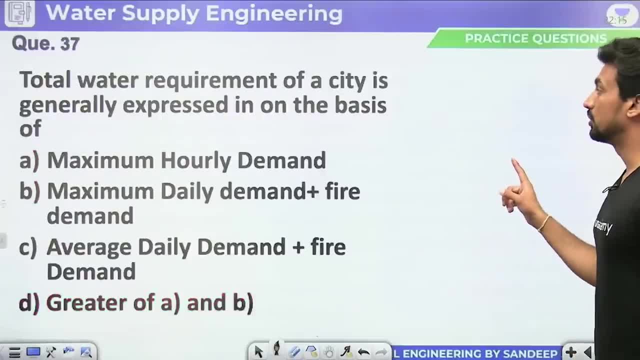 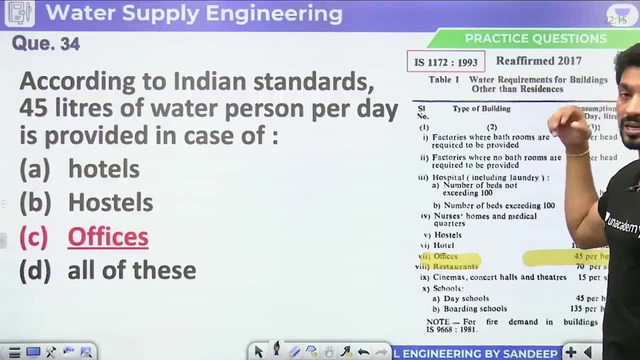 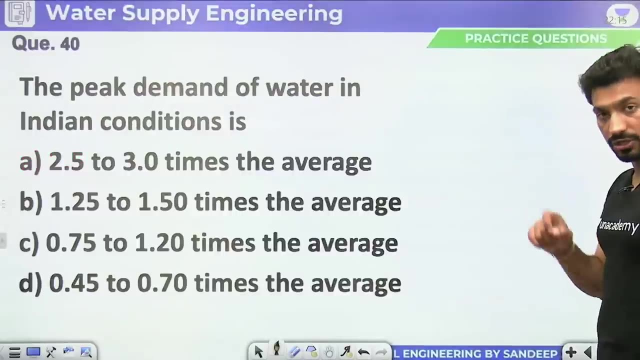 that last code was of our water distribution. the code which we were seeing a while ago, 1172,. this was related to the distribution of water or related to the requirements of water. If we talk about water specifications, quality parameters or the quality of drinking water, then for that we have the code that comes 105: 00,. do not get confused in these. 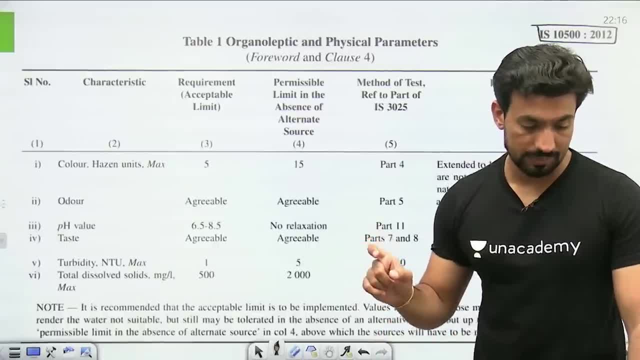 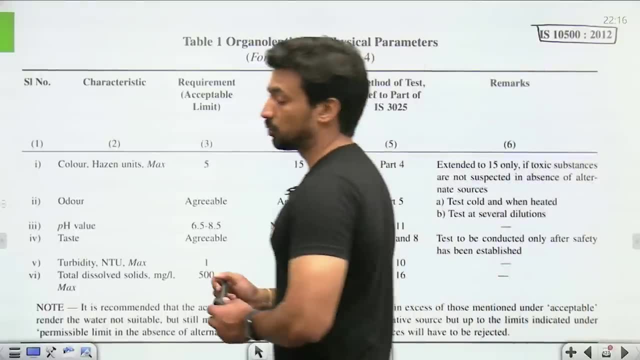 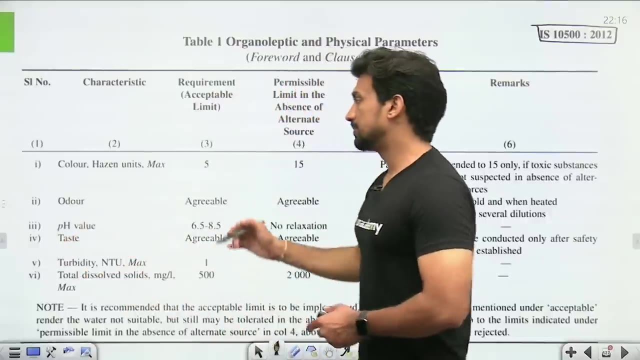 If we talk about water specifications or quality, then it tells you 105 00.. Specification: this code will tell you 105 00.. Now, what are the things you have to remember from these? now we will come topic wise also. The color is true color unit. 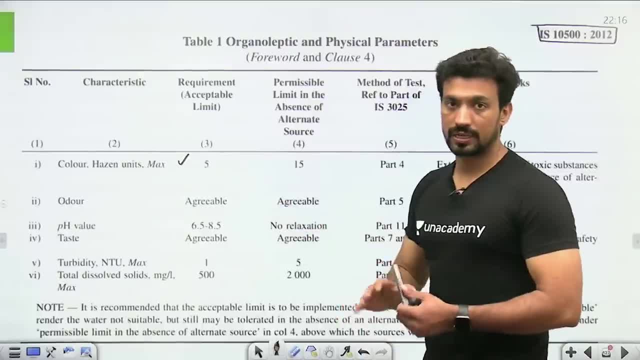 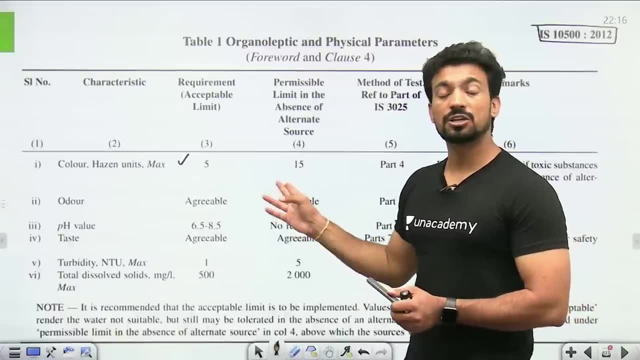 This is told in Hazen. it has a required limit of 5, which we call acceptable limit. Acceptable limit means it can go up to here. Permissible limit means if it is above this, it will be rejected. Cause for rejection will be created. we will not use that water. 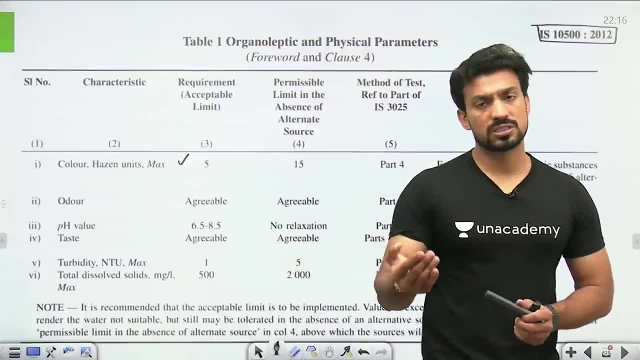 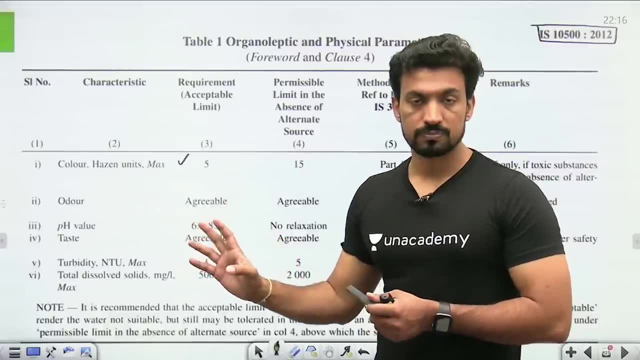 You have two water sources or more than two. after having two or more water sources, we will obviously go to that source in which there are less impurities than acceptable limits. But if there is no alternate source, Then 1 source is not there. 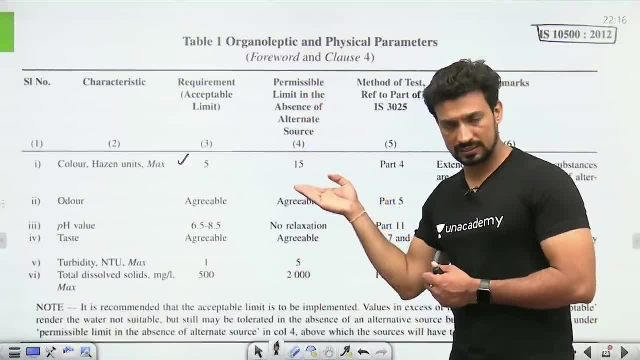 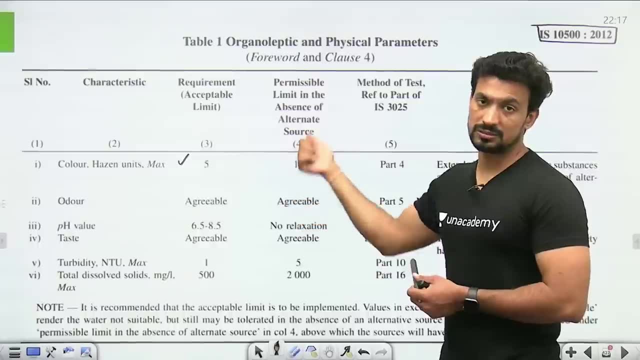 So, in the condition of having one source, we can go up to permissible limits and use it by treating it. But if there is only one source and more than this, if there are more impurities present in it than permissible limits, then it will be rejected, we will not treat it. 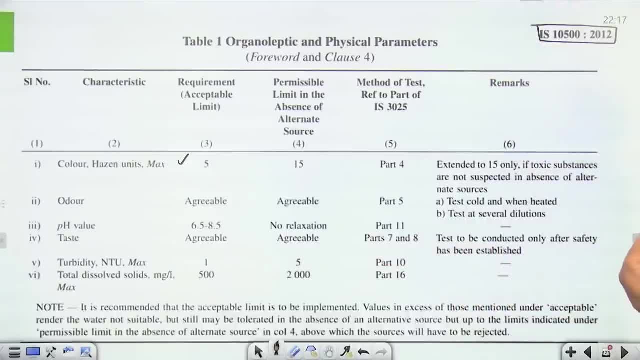 It is recommended that acceptable limit is to be implemented. Values in excess of those mentioned under acceptable render the water not suitable but still may be tolerated in absence of an alternative source, but up to the limits indicated under the permissible limits In the absence of an alternative source in column 4, above which the sources will have to be rejected. 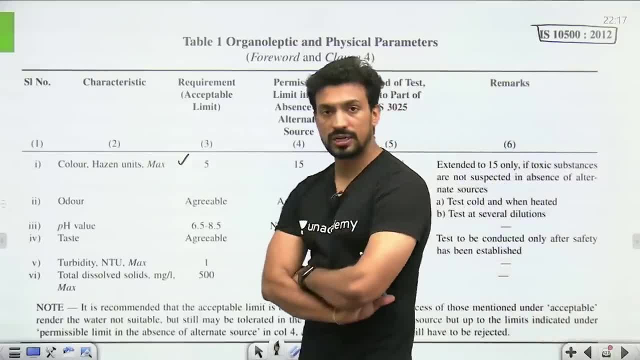 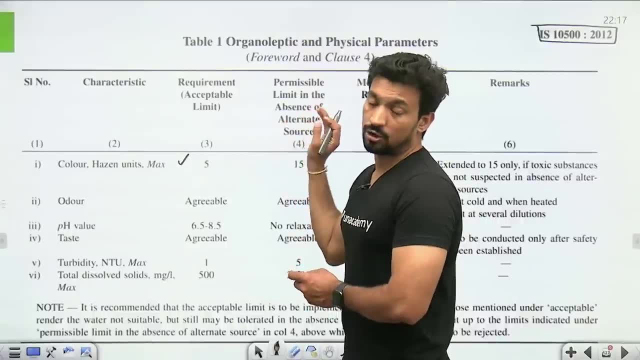 The meaning of saying which I just said a little while ago. We will try to choose a source less than acceptable limits, But if there is only one source available, then it can go up to permissible limits And after coming here you will treat this water. 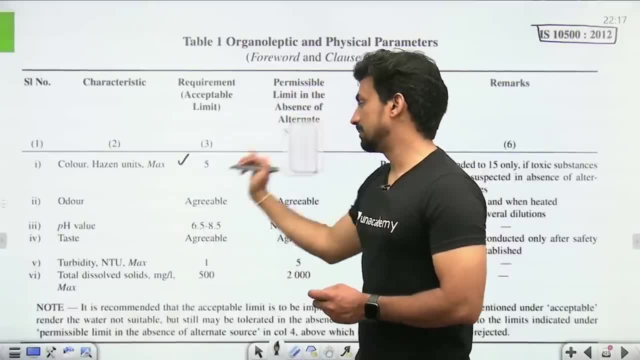 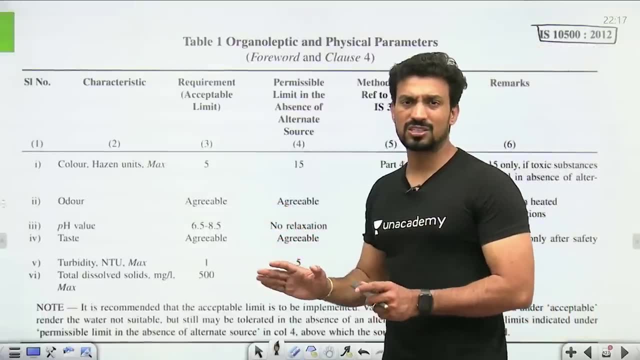 But if there are more values than these, then we will not treat it So. acceptable limit color is 5.. Cause for rejection is 15.. If we talk about the order, then the order should not be so much, it should be agreeable. 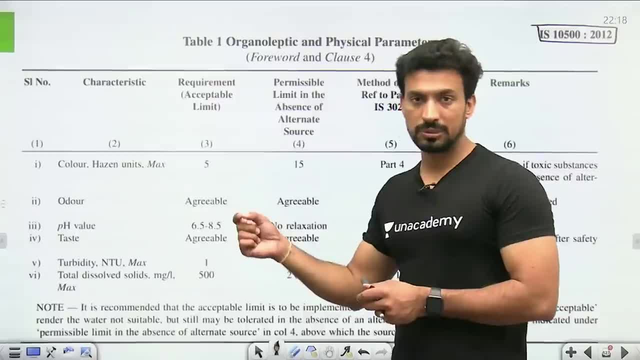 Means. it should be correct. Now let's see the order from the osmoscope. It also has degrees. we will talk about them too. If we talk about pH, then the pH value should be 6.5 to 8.5.. 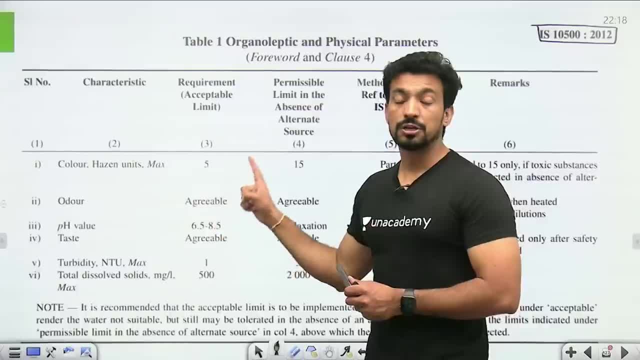 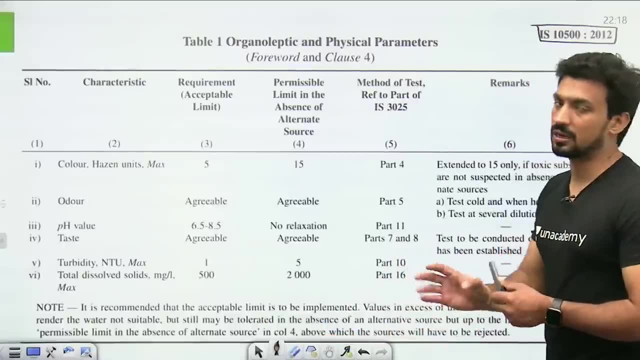 According to whom we are talking. we are talking according to the Indian Standard Code. Our Government of India manual says 7 to 8.5.. But we have to remember this, You have to remember IS code maximum: 6.5 to 8.5.. 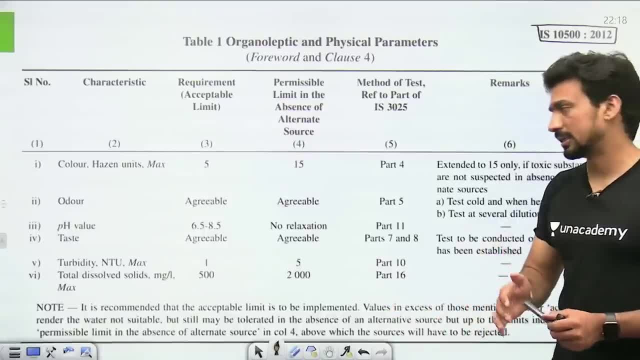 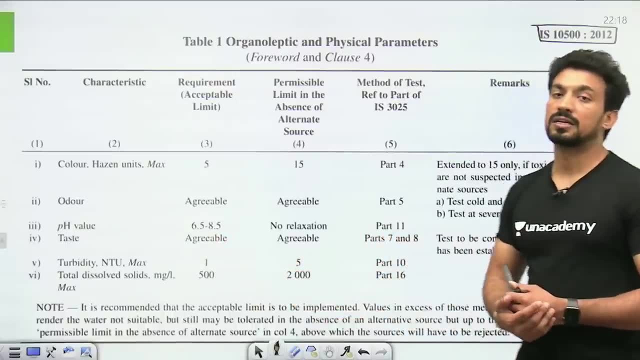 Taste should be agreeable. It should not be so that it is objectionable. Very bad taste is coming. Turbidity nephelometer is measured in the unit of turbidity. 1. Cause for rejection comes to you, Its 5.. 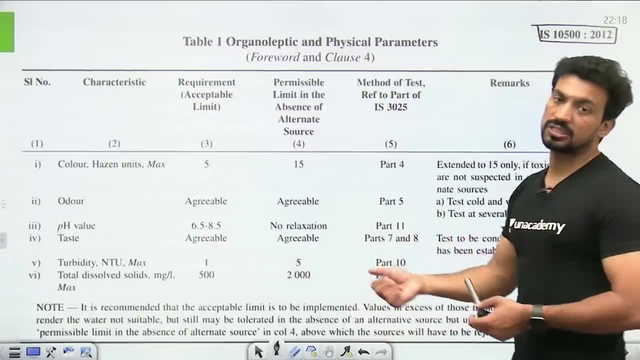 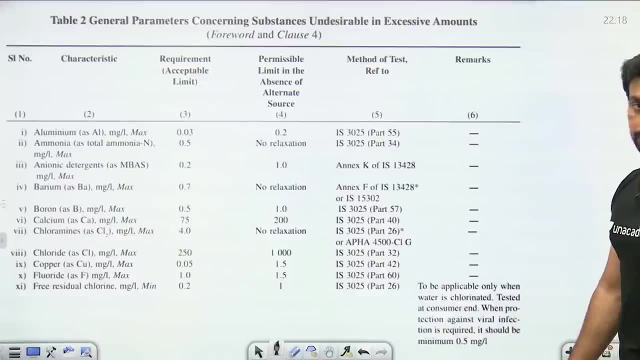 Then if we talk about total dissolved solids, TDS, then 500.. Cause for rejection comes to 2000.. You should remember all these points. as it is, It is very important from the objective point of view. After that we have to see them. 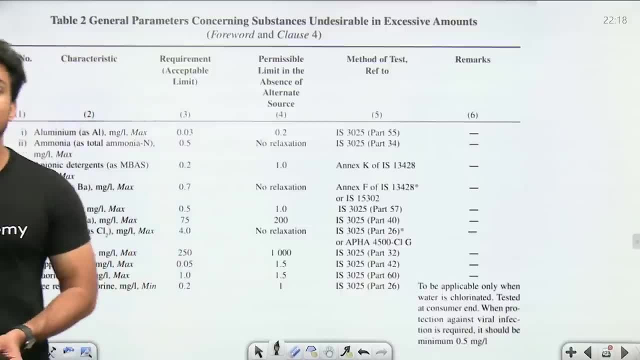 If we talk about questions, then in the questions, which terms or points have been asked to you so far? If we talk about these, then it asks you about ammonia. Its acceptable limit is 0.5.. And there is no relaxation in it. 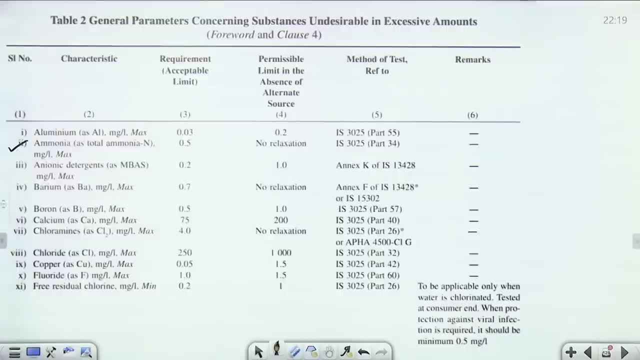 Because it is recent pollution. Then, talking about chloride, it is asked to you: Chloride content: 250 mg per liter. Cause for rejection comes to 1000.. Chloride content: 1, 1.5.. This is very favorite of examiners. 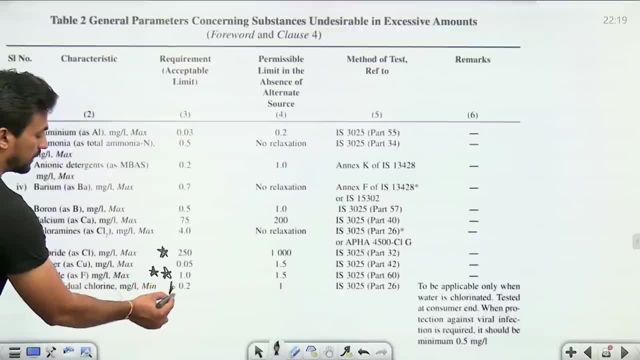 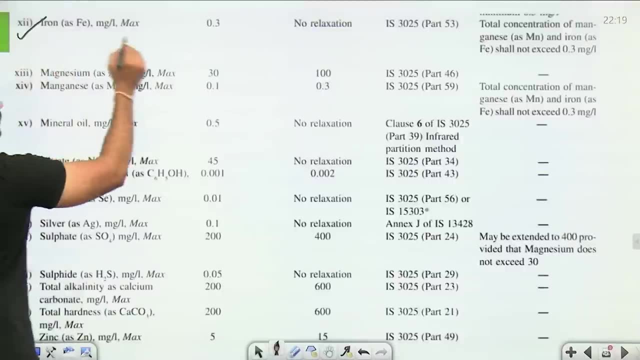 It is asked many times: Residual chlorine: 0.2 mg per liter. This is asked to you. This is important. Then, talking about magnesium, manganese, iron, Iron is asked 0.3 mg per liter. This is asked to you. 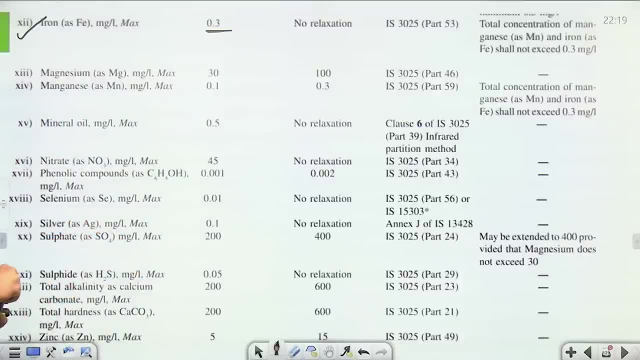 Cause for rejection has no relaxation. It should not be more than 0.3.. Then, talking about nitrate: Nitrate is asked to you. We will read them individually. This is asked to you. Phenolic compound: This has been asked so far. 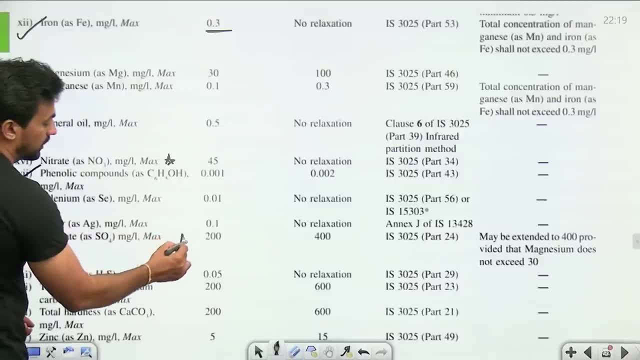 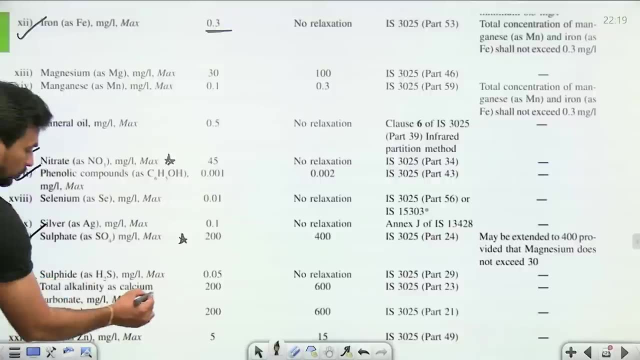 Then sulfate has been asked: 200 mg per liter, 400 mg per liter And total alkalinity- This is also important. Total alkalinity: 200 mg per liter. Cause for rejection: 600.. And total hardness: This is also important. 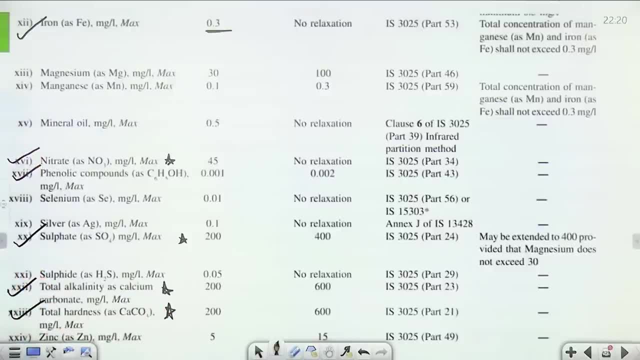 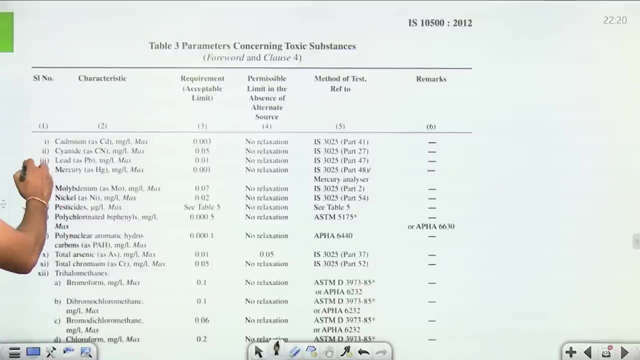 This is also asked. Same values: 200, 600.. Zinc, Then if we talk about toxic substances, Lead has been asked. Cyanide has not been asked yet, But lead can be asked. Lead is 0.01.. This has been asked. 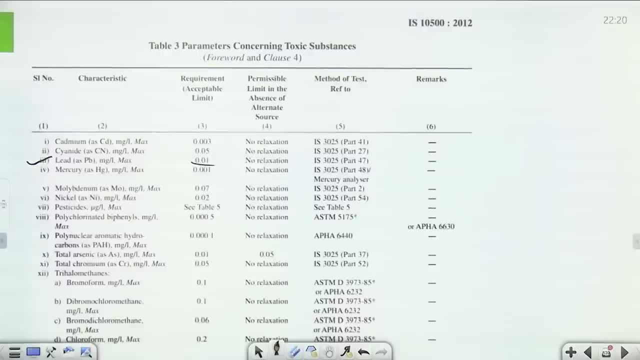 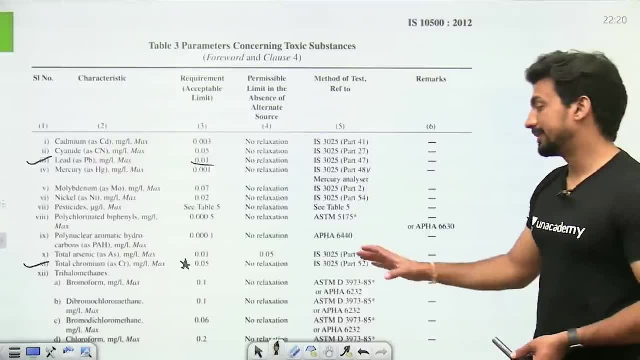 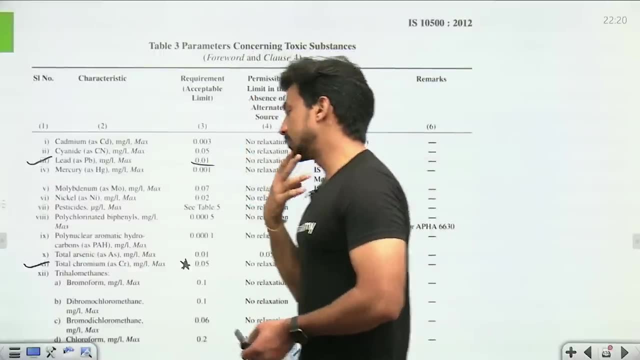 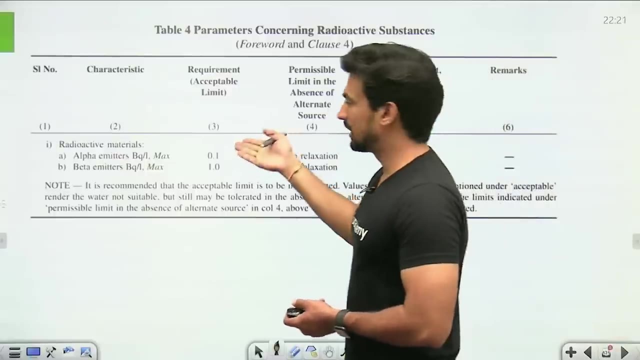 What values have been asked? What values have been asked? These values have been asked so far, so see them through questions. if you look at the table once or twice, then you will start remembering this Radioactive material has not been asked yet. you will see that the government of India manual has almost all the values mentioned here. 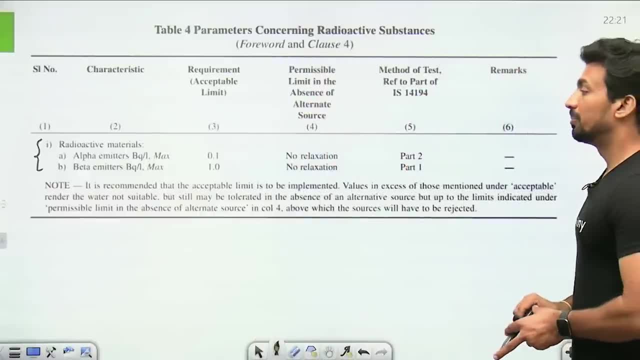 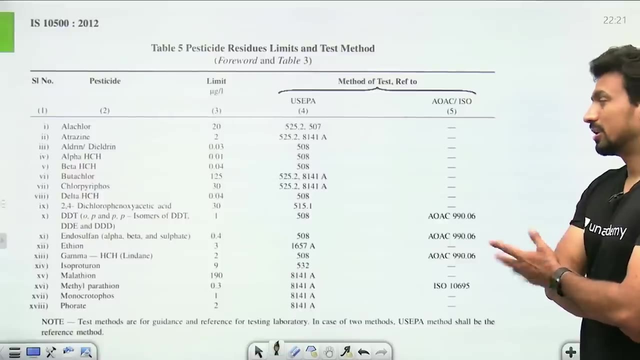 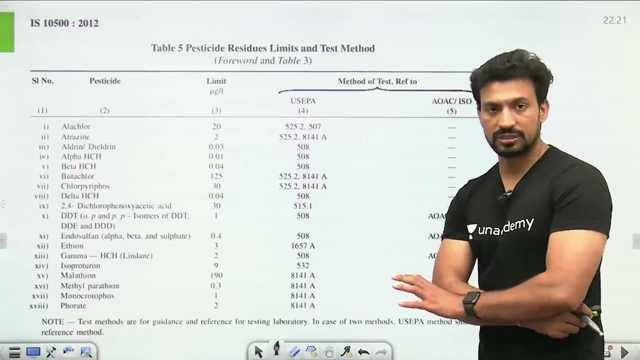 If we talk about radioactive materials, then alpha emitter, beta emitter, 0.1 and 1, there is no relaxation in them. Then comes the pesticide residue limits and test method. so such questions related to them have not come yet. You can keep the data with you for reference. if you see any question, then you can refer to them and check that. yes, it is correct in that question. 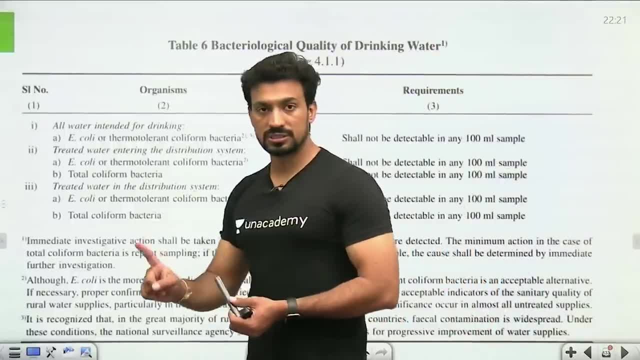 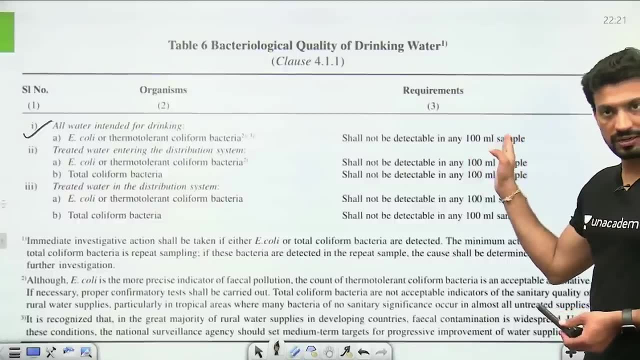 If we talk about bacteriological or biological quality, then a question related to them has been asked For drinking water, E coli should not be detectable for 100 ml sample. If such a question has been asked to you in the objective, then you have to read this portion. 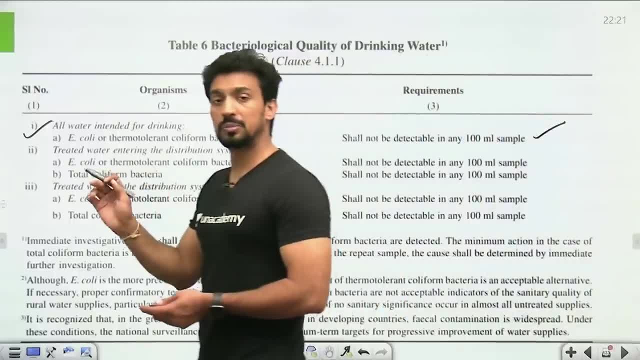 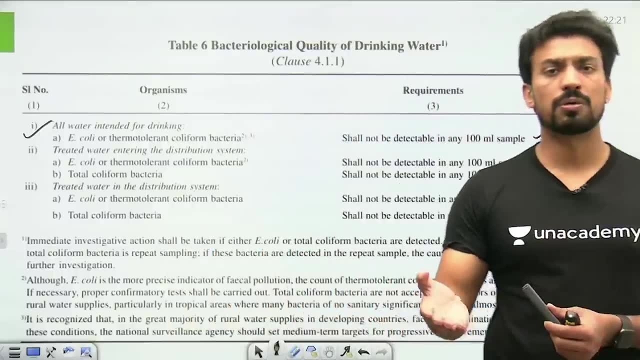 Now I have shown you these limited things in the code. among them, only limited things have been told that you have to remember this. Will you sit to read the whole code yourself, or the whole specification of the government of India manual is about 800 pages. 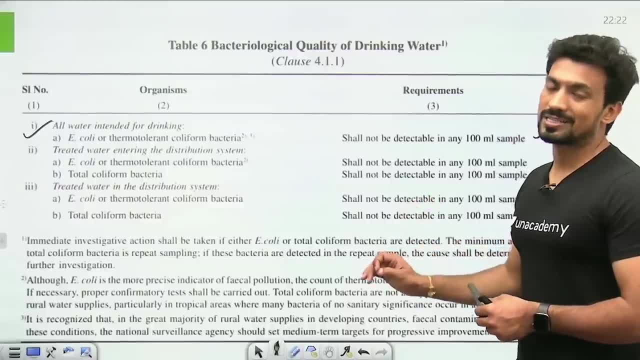 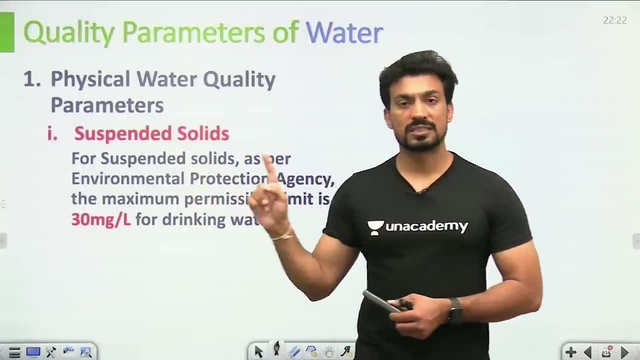 So it will be very difficult for us to read the whole thing. what is important? what comes in the exam? you have it all here. Now let's come to the first parameter above the physical quality parameters, in which the first comes: suspended solid. more than 30 mg per liter suspended solid. 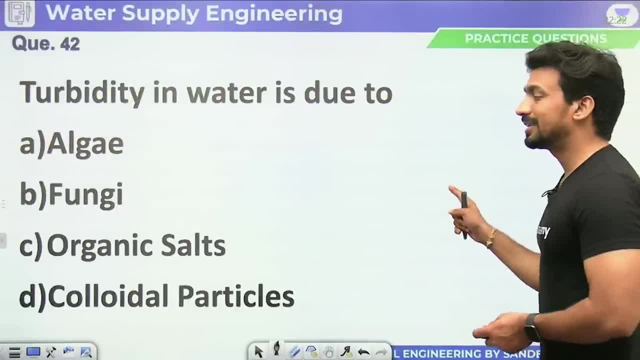 Let's see the first parameter above the physical quality parameters, in which the first comes: suspended solid: more than 30 mg per liter suspended solid. Why is the first? the first one: it is because of colloidal particles. The unit of turbidity is the 9 km turbidity unit. 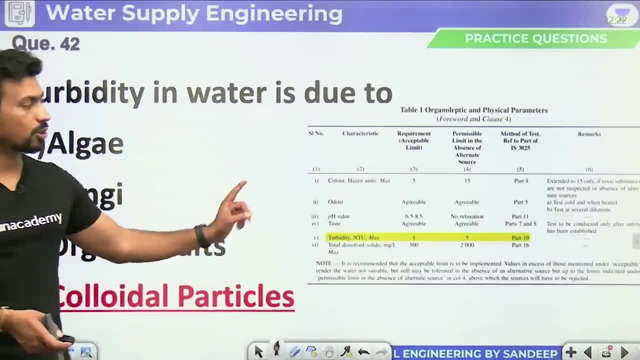 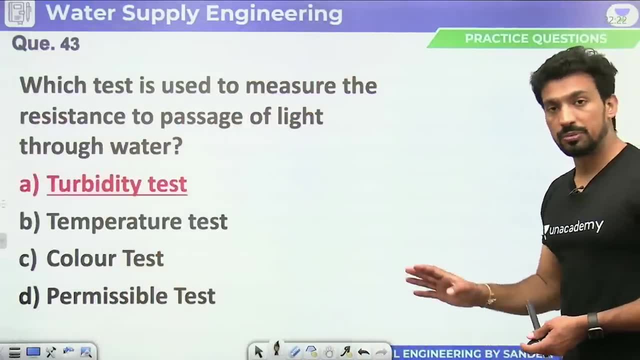 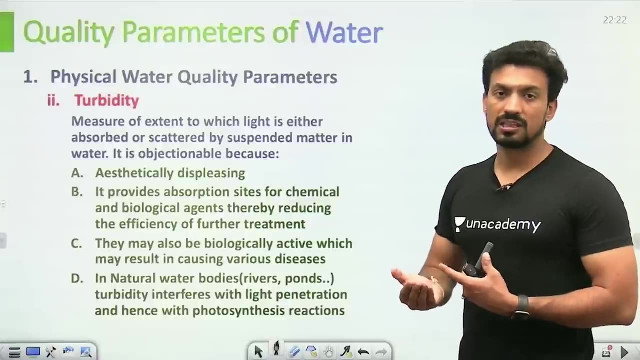 The acceptable limit is 1,. the cause for rejection is 5.. Which test is used to measure the resistance of the passage of light through water? Then we do the turbidity test. for that Why we are not liking the terms of turbidity. 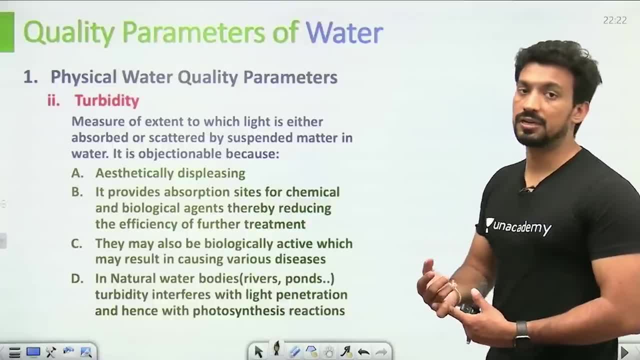 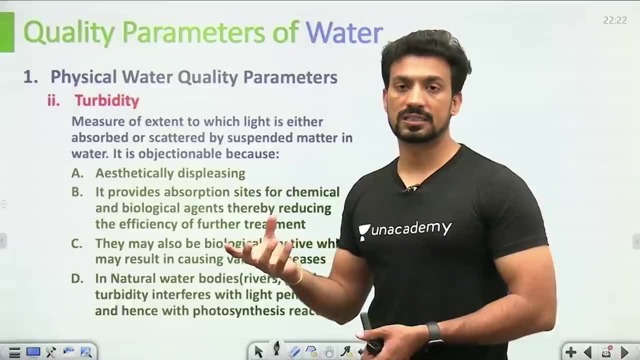 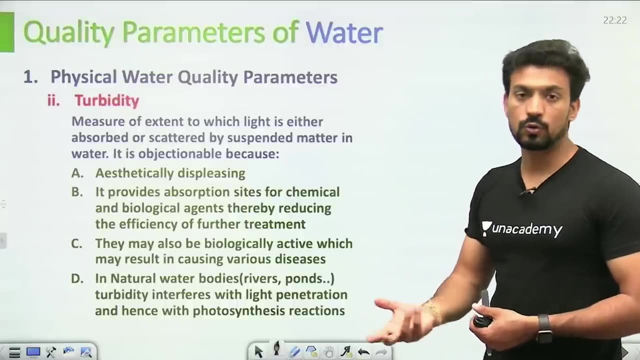 First, it is not good to see, it is aesthetically displeasing. Second, it provides absorption sites that bacteria can come and settle on those particles and grow, which will spread diseases. It is possible that those turbidity small units, which are particles, they themselves are biologically active. they themselves create diseases. 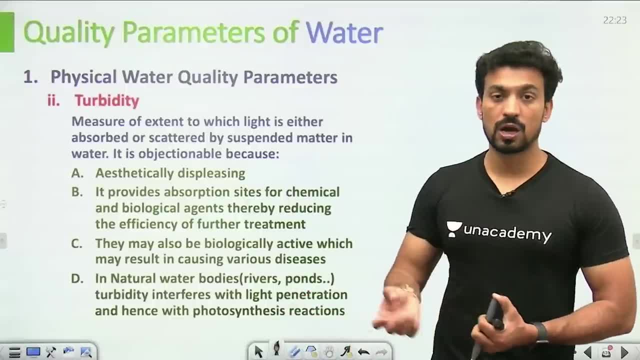 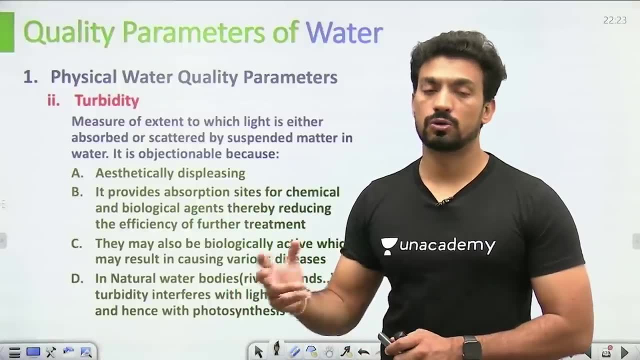 Or if natural water bodies have turbid water in them, then sunlight will not be able to reach the aquatic plants and there will be no photosynthesis in them. If there is no photosynthesis, then dissolved oxygen will be reduced in the water. It will impact the aquatic life. 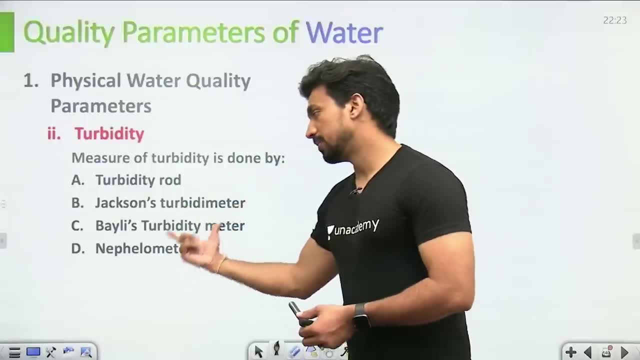 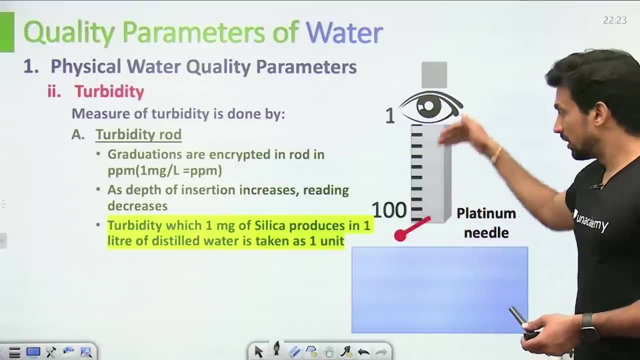 Next we can measure turbidity with a turbidity rod, Jackson turbidity meter, Bailey's or Nephilimeter. What happens in the case of a turbidity rod? A platinum needle is placed at the bottom. The more it goes in depth and we keep seeing this needle. clearly that means the less turbidity it is, the more your reading will increase. 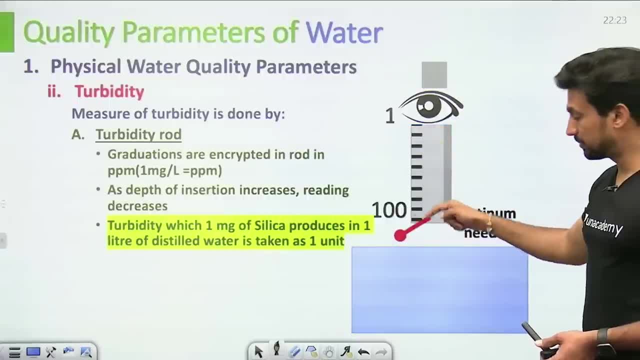 Like, the level of water will keep increasing. So the more it goes in depth, the less reading we will get. If this needle is put in the water and a little needle goes down, it will stop looking. So this means that we will get more reading here. 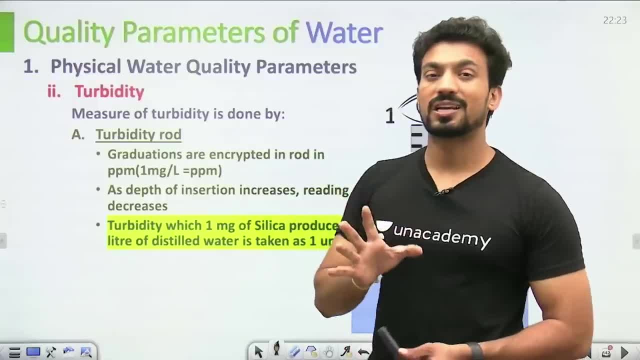 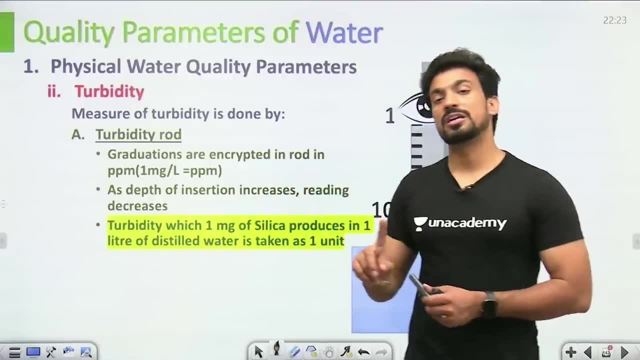 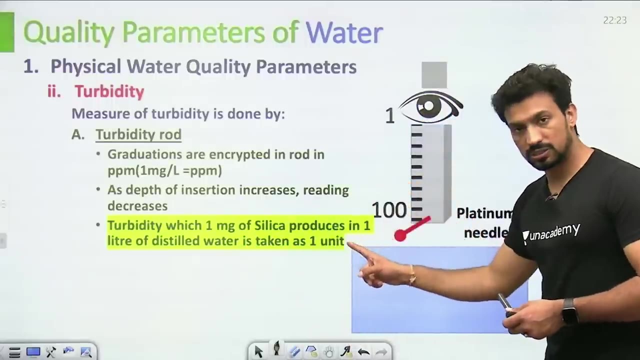 Turbidity is very high. In which reference is the turbidity measured? If 1 mg of silica is added to distilled water, then the amount of turbidity it produces will be called 1 unit. So this is also asked from you, that on what scale is the turbidity measured? 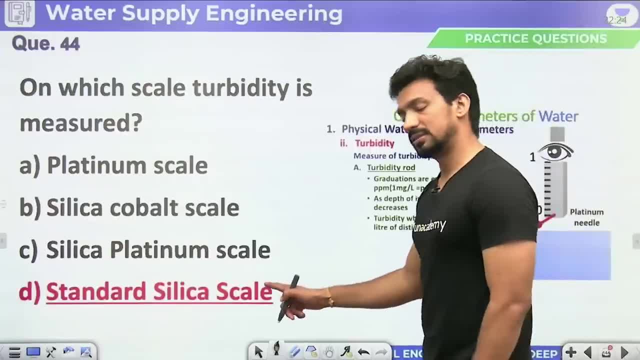 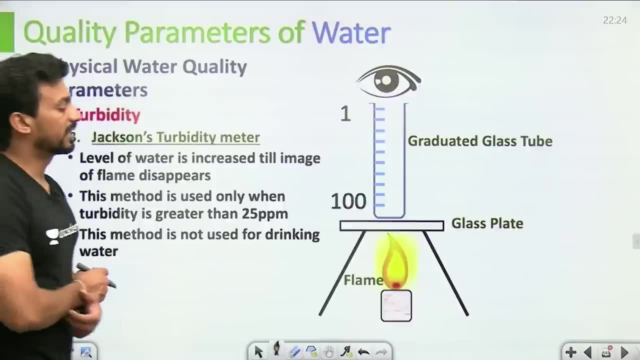 So turbidity is measured on silica scale. On the standard silica scale we measure turbidity. Next comes the Jackson Turbidity Meter. In this case a flame is placed at the bottom of the glass plate. You have placed a graduated glass tube here. 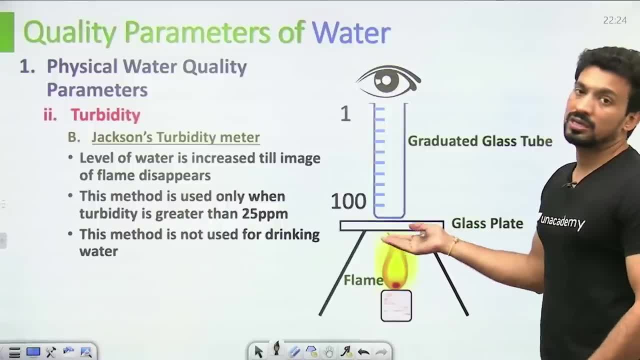 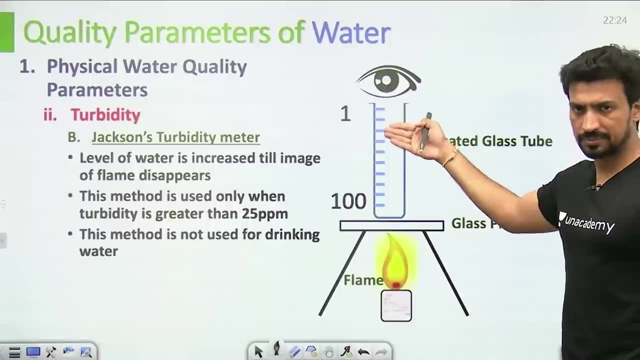 Then as much water is filled. if the flame stops when a little water is filled, it means that the water is very turbid. If we have filled a lot of water, then after that it stopped looking. it means that the water is less turbid. 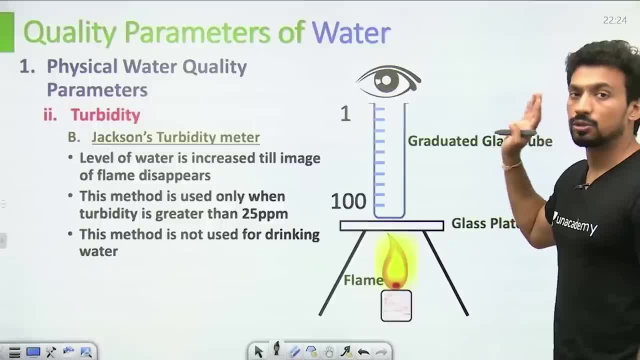 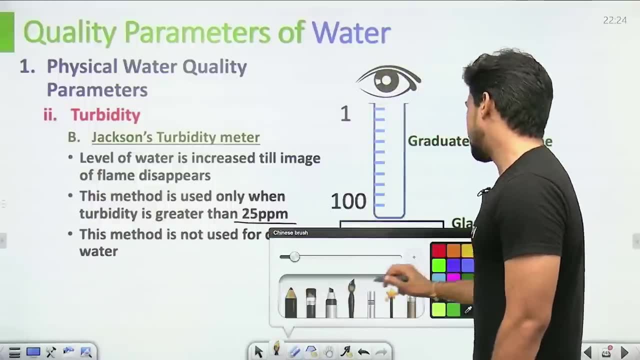 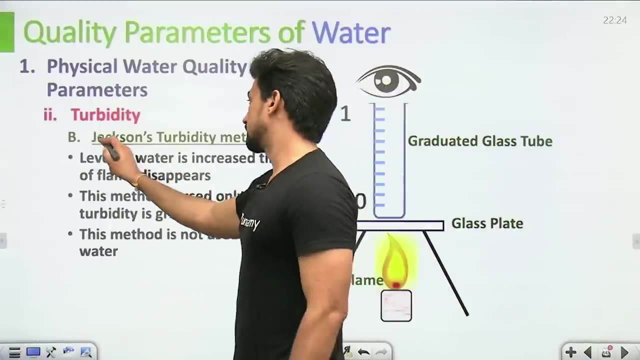 We will observe the readings on this corresponding to this. So the Jackson Turbidity Meter is used when the turbidity is more than 25 ppm In the objective. this question was asked that if the turbidity is more than 25 ppm, then which turbidity meter can be used. 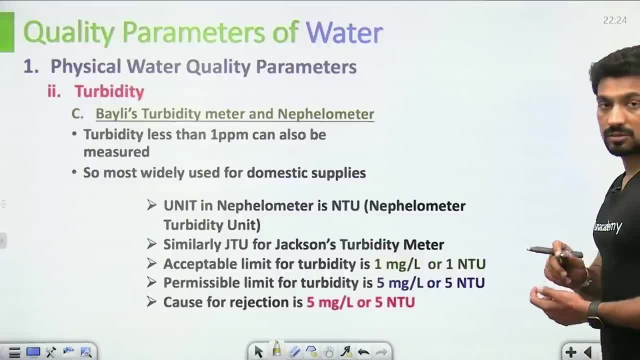 Jackson Turbidity Meter. You use Bailey's Turbidity Meter. If the turbidity is less than 1 ppm or for domestic supplies, we will use it. The unit is NTU. This is the Nephilimeter Turbidity Unit. 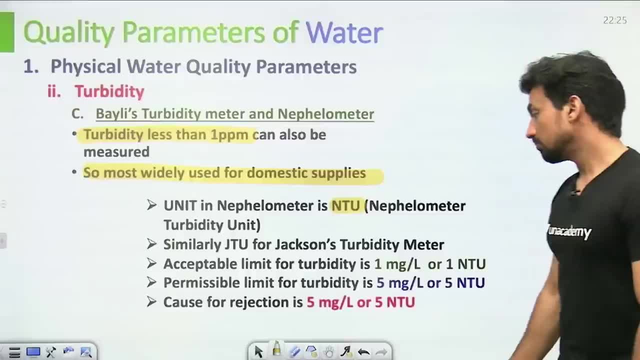 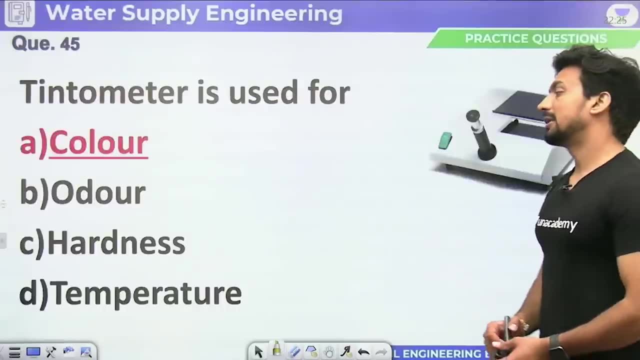 It is NTU. We can also count JTU in Jackson: 1 mg per liter Acceptable limit. You have to keep this in mind. Tintometer is used to tell the color. Tintometer is used Why is the color objectionable? 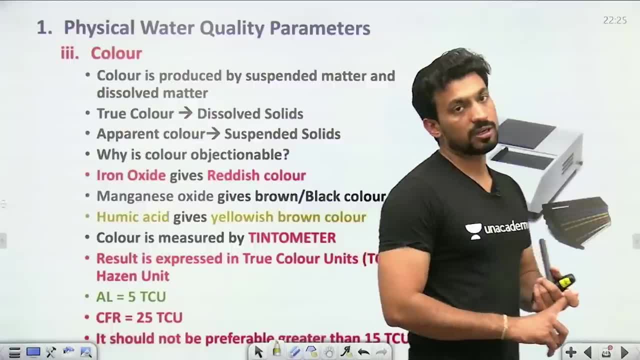 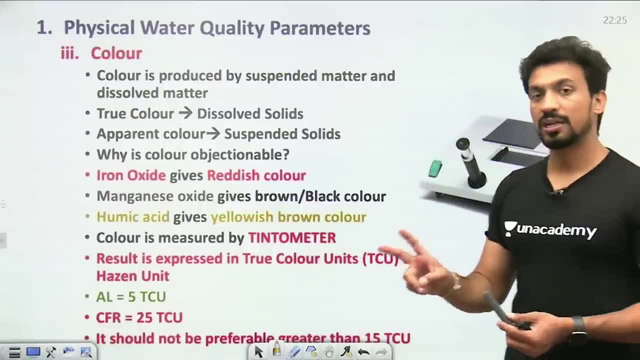 Because of the color. If the color is in some water then it can react with some further compound and can be carcinogenic. It can be cancer causing. There are two types of color. One is due to dissolved solids and one is due to suspended solids. 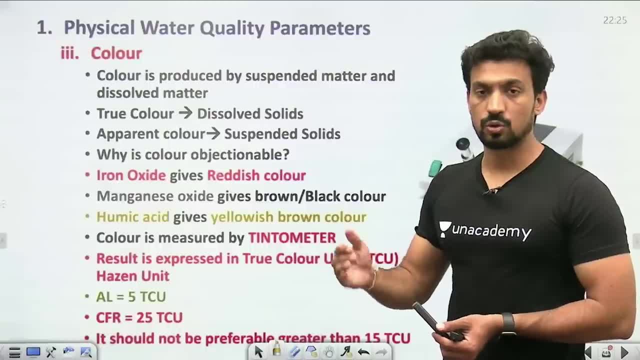 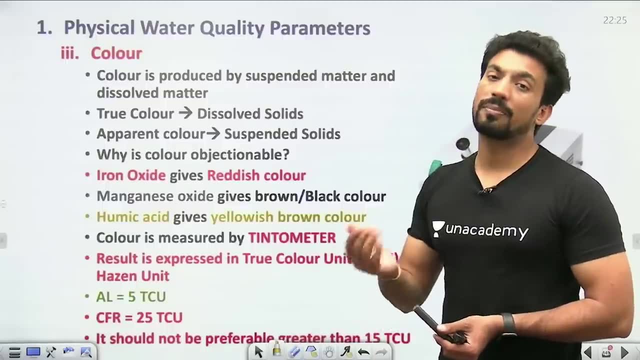 If you dissolve the soil in water, then the particles will settle after a while. So the color that was visible in the beginning will not be visible later. Why? Because it was an apparent color. It was due to suspended solids that later settled. 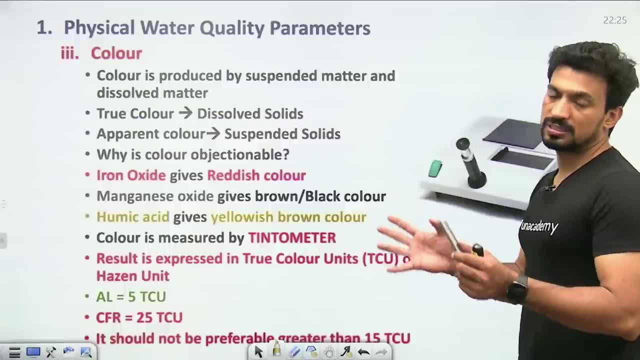 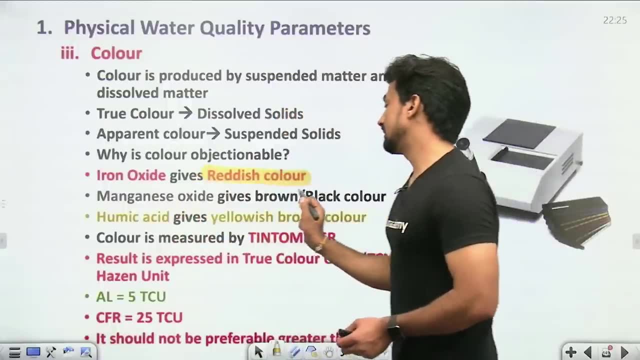 True color is like you mixed ink in water, So now that color will remain present in it. Why? Because that ink is dissolved in it. Due to iron oxide, reddish color comes. You can ask in the objective. Due to manganese, brown or black color comes. 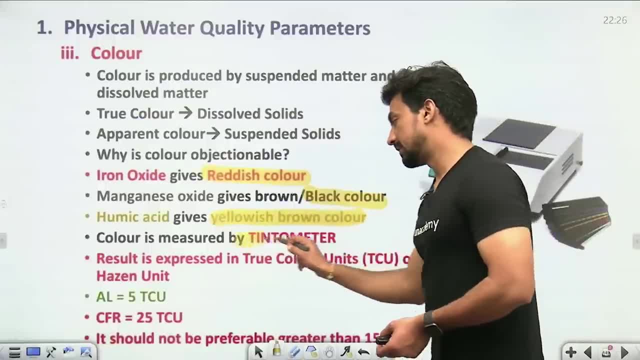 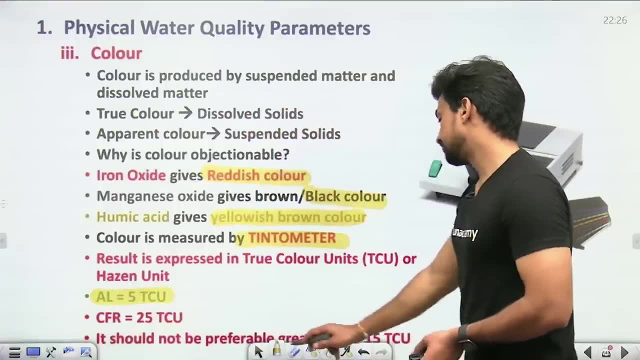 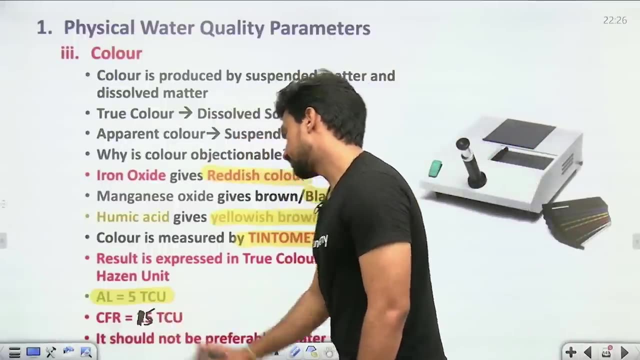 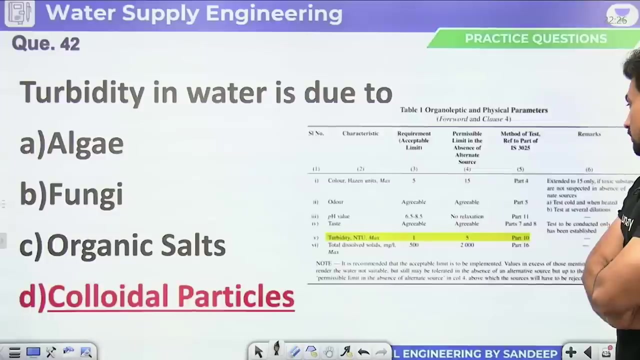 Due to humic acid, yellowish comes. Tintometer knows it correctly. It will be told in Hazen units. Acceptable limit is 5.. Cause for rejection is 15.. Cause for rejection: if we talk according to Indian standards then it is 15.. 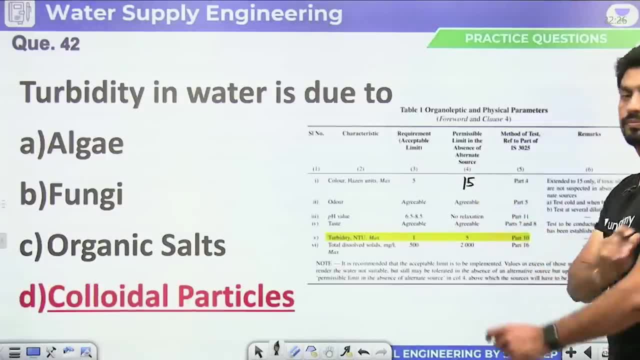 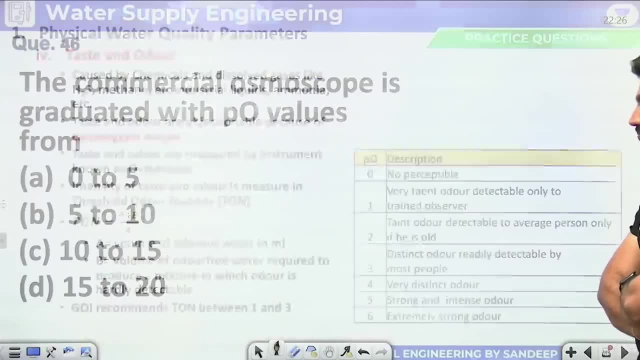 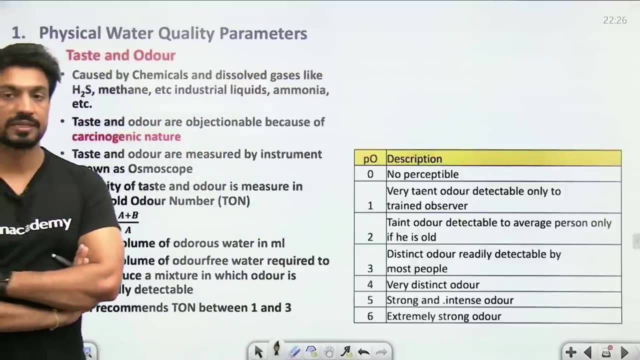 Cause for rejection is 15.. Next let's move ahead. Then, after that, let's come to the taste and order. Taste and order. How is the water in taste? Is there any smell coming from it? Let's find out from the osmoscope. 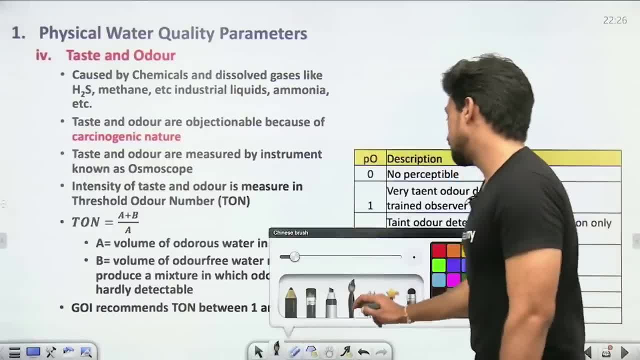 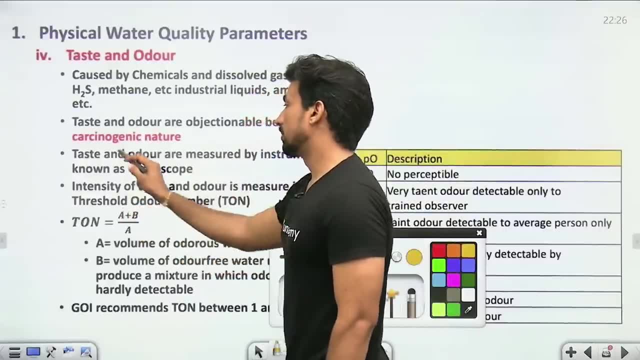 The first important thing: How do we detect taste and order? We detect it from the osmoscope. Now what do we do? We will keep mixing clean water in dirty water. We will keep mixing clean water in dirty water. So A is the volume of odorous water. 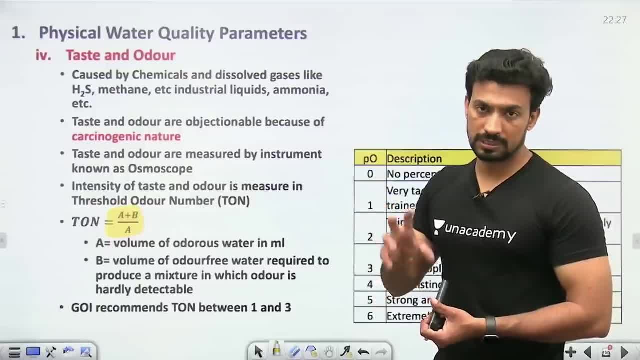 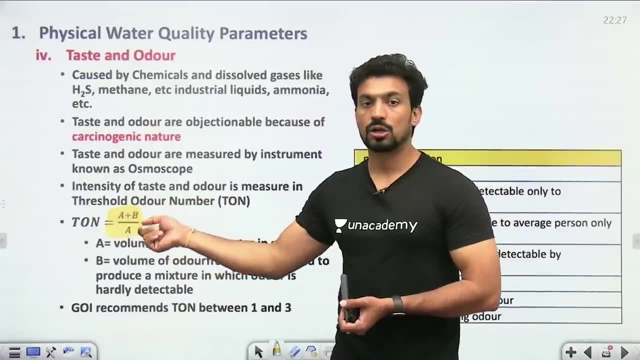 It is the water with smell, B is the clean water. We mixed B until the order or smell was stopped. So A plus B upon A, So A plus B upon A. We have told the threshold order number here And we have calculated the value of the threshold order number. 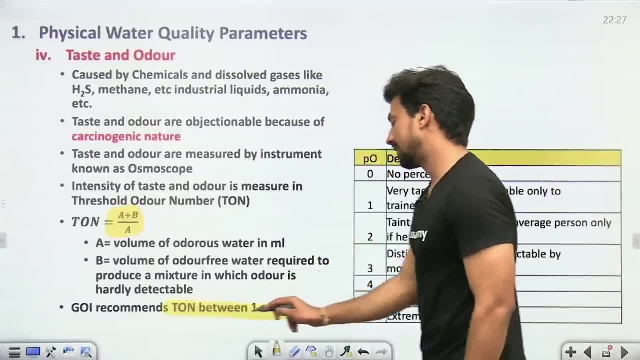 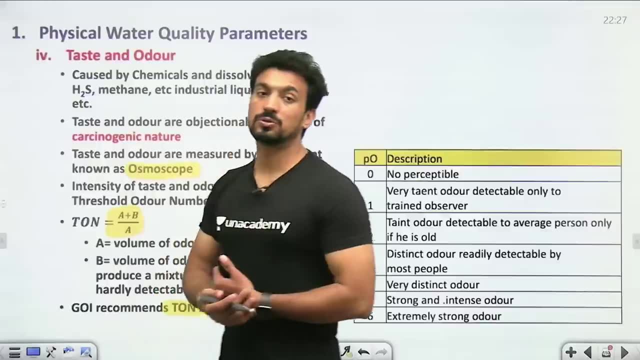 Government of India recommends that the value of the threshold order number is between 1 to 3.. Then let's come to the osmoscope. Osmoscope is a device that you can use. It can also be used in the case of osmotic pressure. 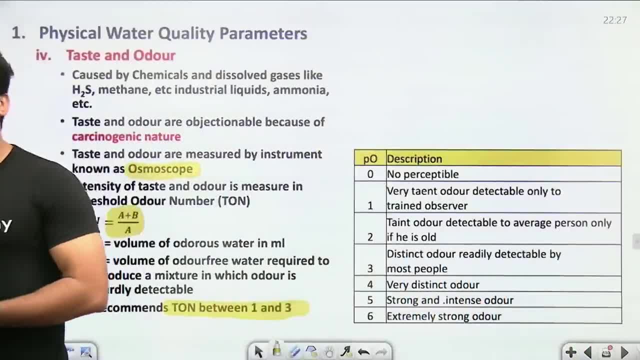 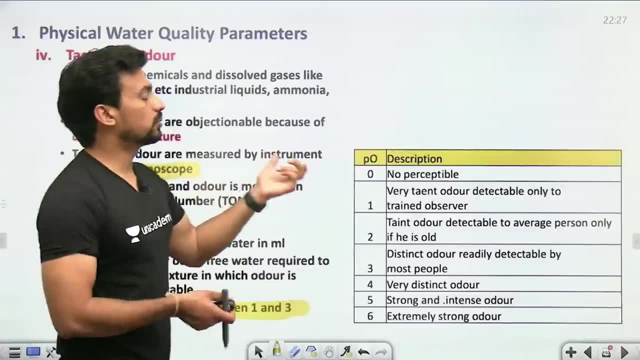 So it also tells, And one that we use from the point of view of environment engineering. It is used for taste and order, So we will tell the zero value when we are not able to check, We don't know, Smell is not being detected. 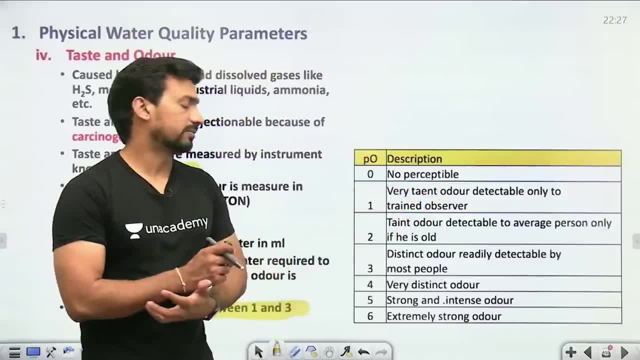 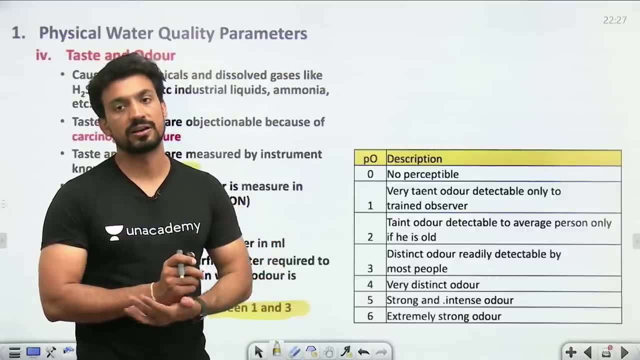 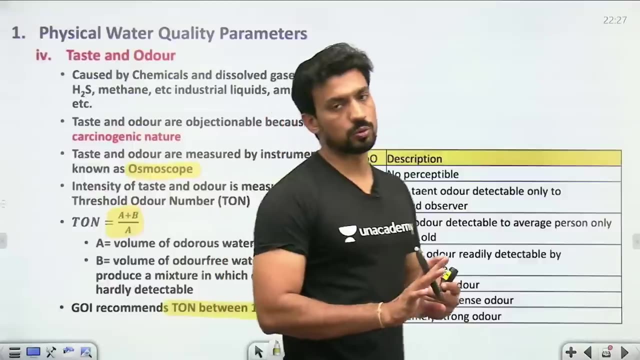 Very taint. Very taint, T-a-i-n-t means to detect the bad smell, Or taint is a word related to bad smell or taste. So very taint order is detectable only to trained observer, The one who has complete knowledge. 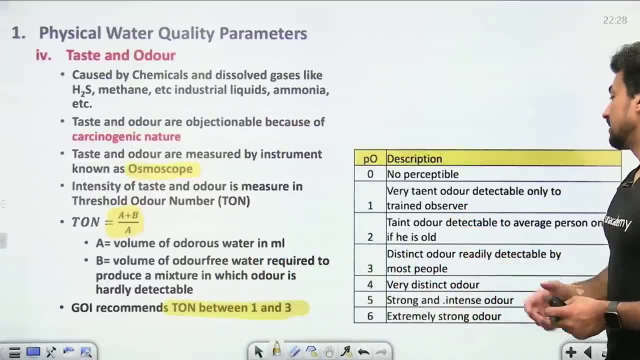 Only he will be able to detect Taint color detectable to average person Only if he is old. Or you can say that if they are smelling very carefully then they will be able to do it. Distinct order, readily detectable by most people. 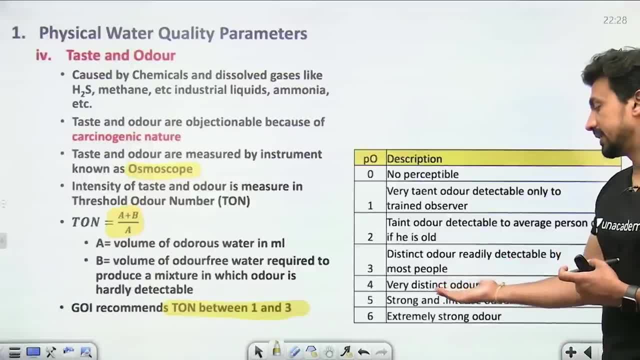 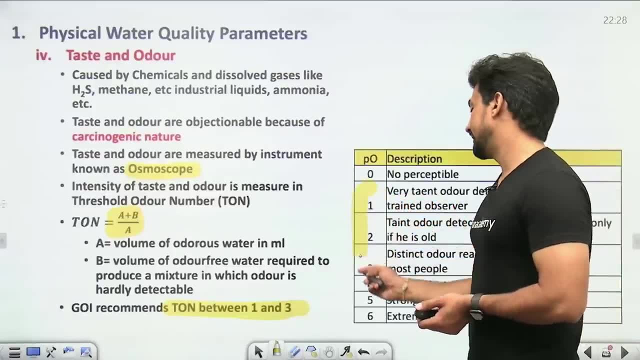 Very distinct order, Then it will come. after that It is being detected easily. Strong and intense order. Very strong smell is coming, Then extremely strong. So generally the values that come to you. The scale is mentioned from 1 to 5.. 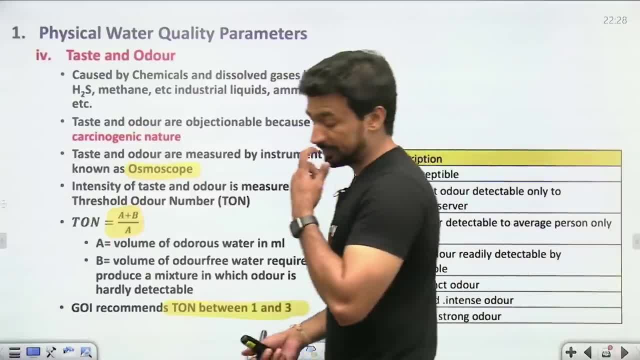 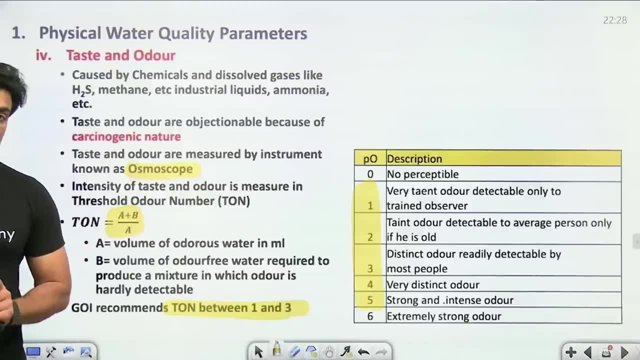 Which are your commercially available osmoscope. These values are from 1 to 5. And the government of India manual which recommends It, recommends that the values should be between 1 to 3. It should be between 1 to 3.. 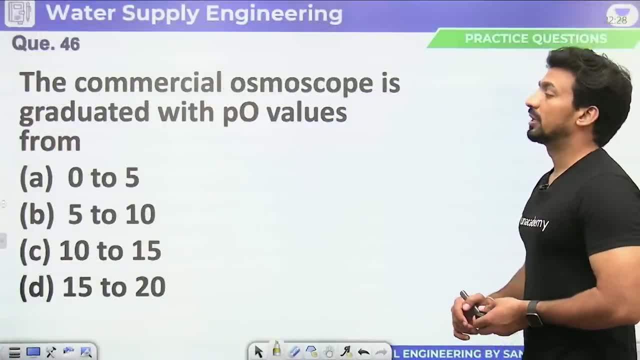 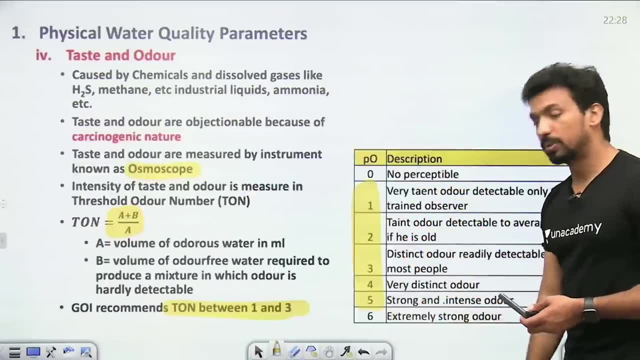 The commercial osmoscope is graduated with BO values from, So it is from 0 to 5.. By the way, we can tell them from 0 to 6. We can explain, But these values are from 0 to 5 on osmoscope. 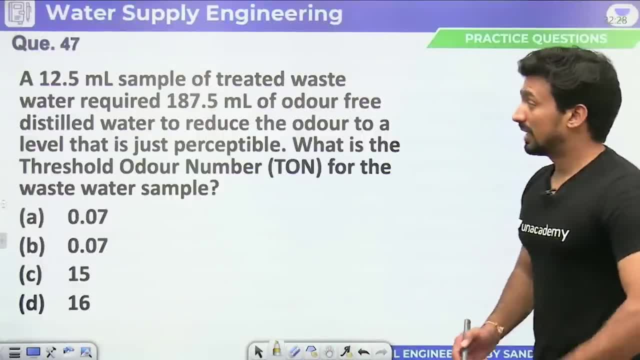 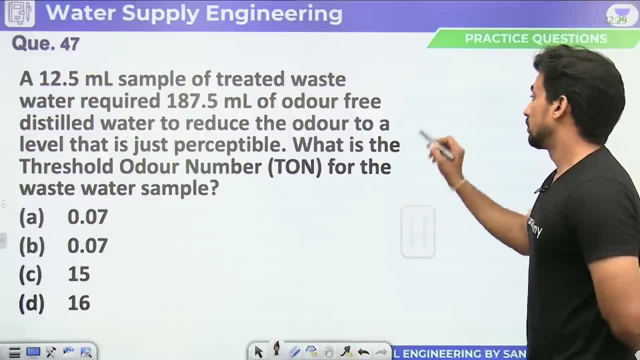 Then after that one question: 12.5 ml of treated water Treated with water, Treated with water, Treated with water, Treated waste water requires. Then you have A only value, 12.5 ml, And put clean water in it. 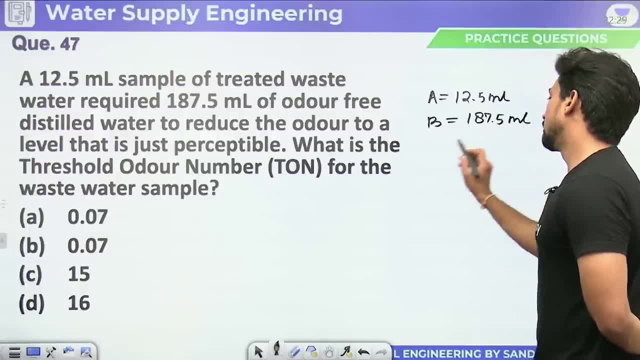 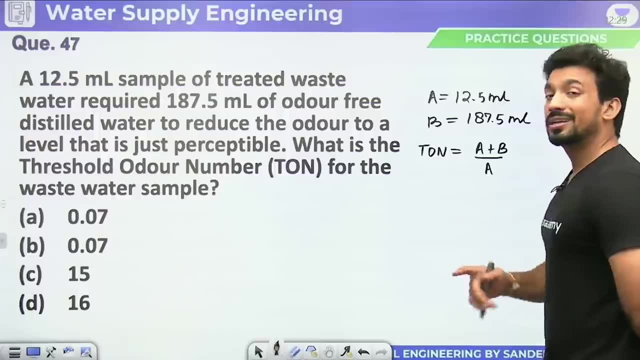 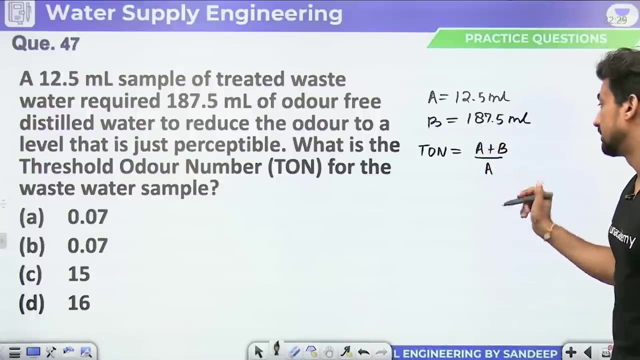 How much clean water. it explained 187.5 ml. How much is threshold order number A plus B upon A In question? it can also tell you That the volume of diluted samples is this much. That means it gave us the value of A plus B. 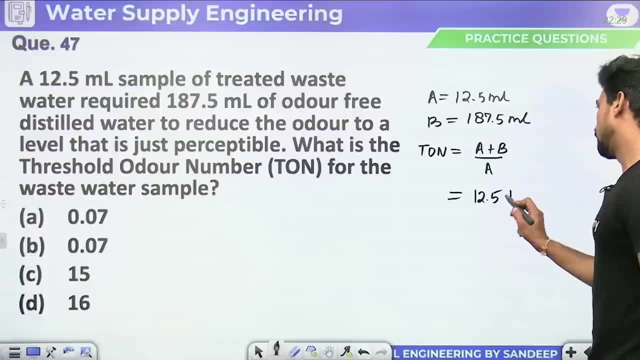 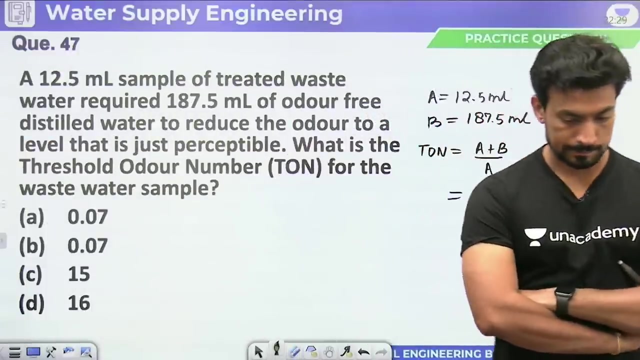 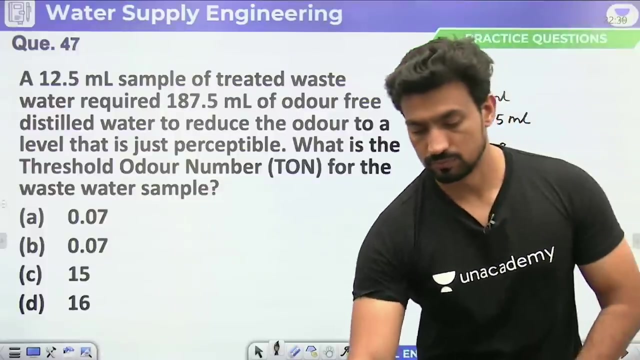 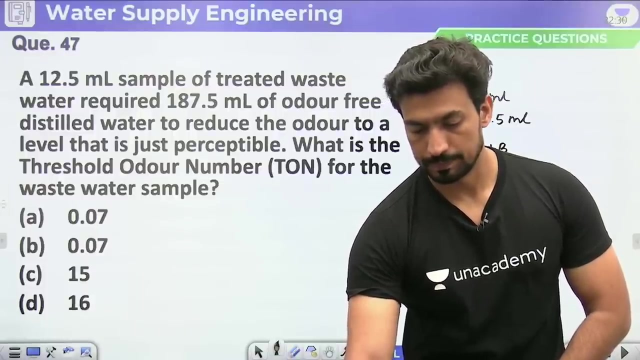 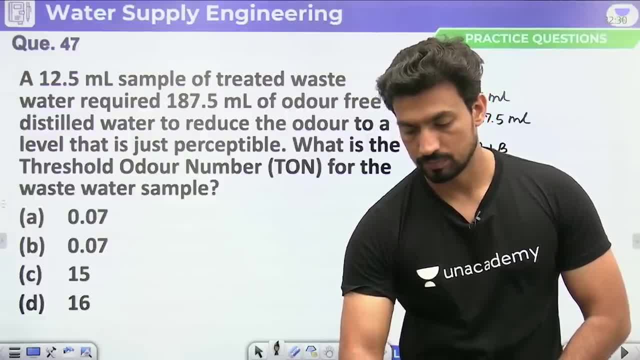 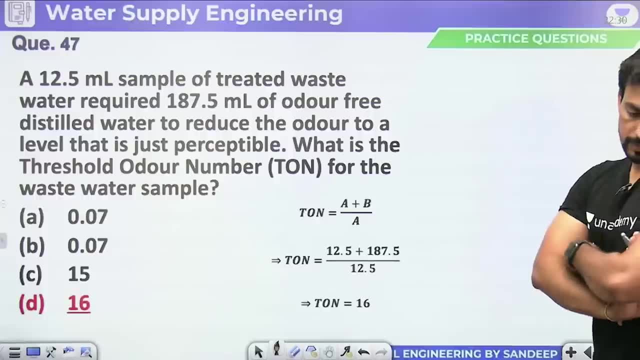 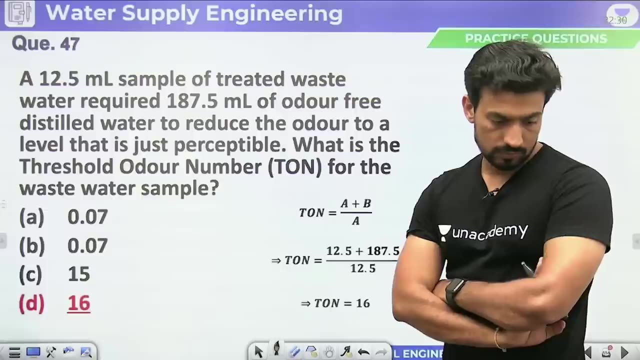 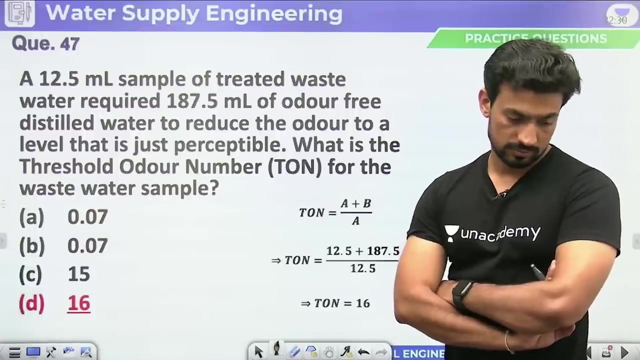 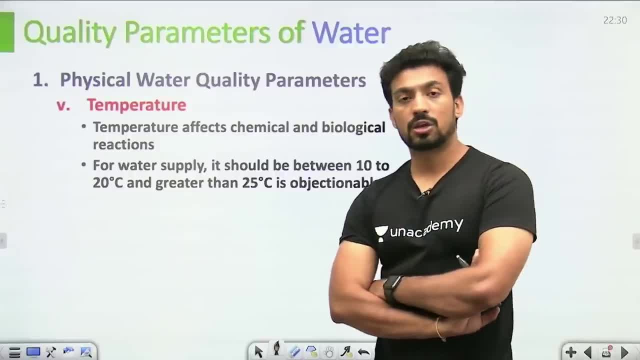 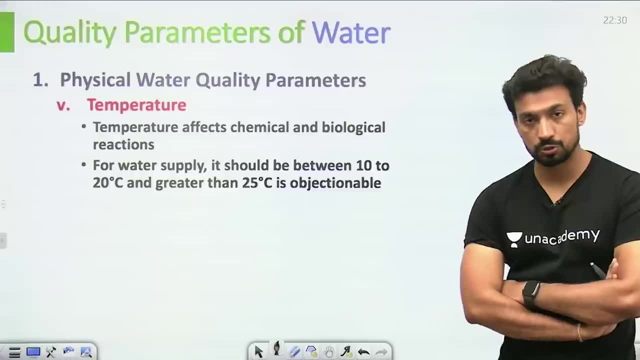 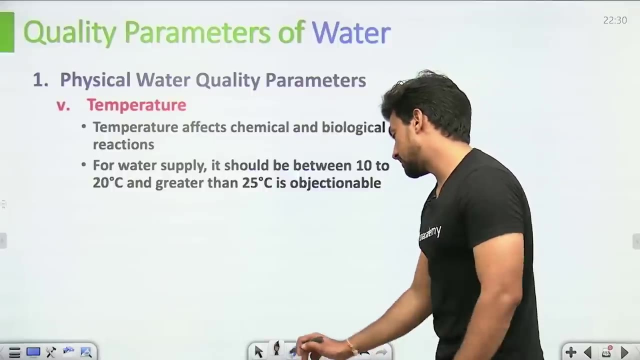 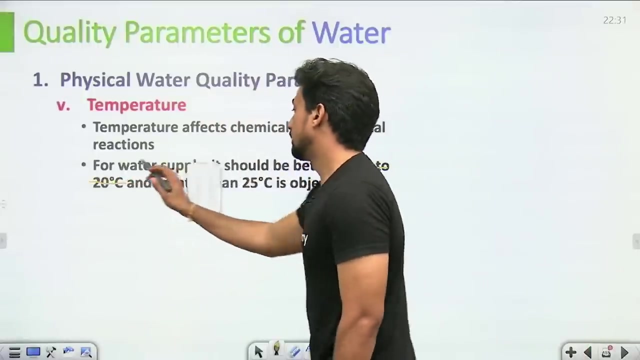 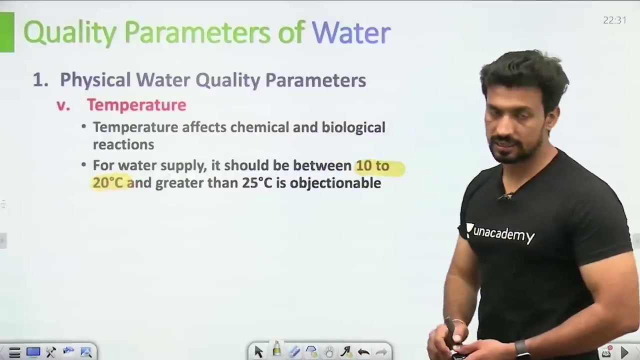 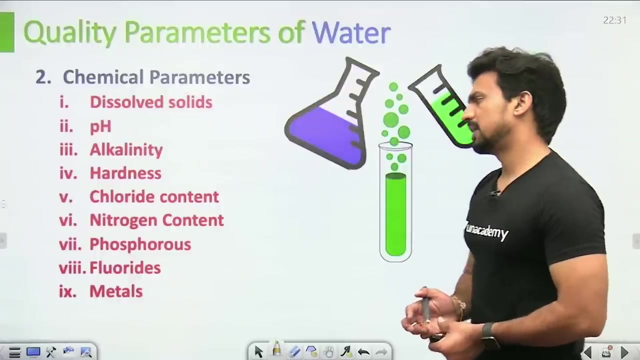 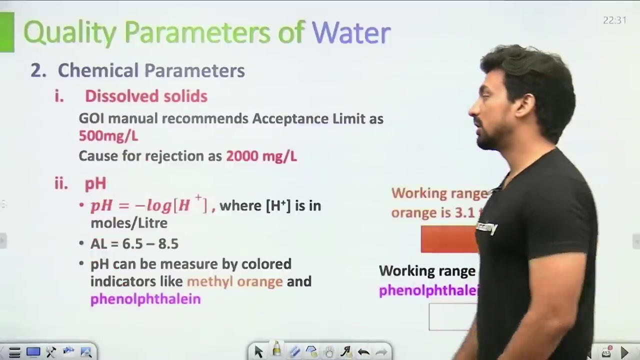 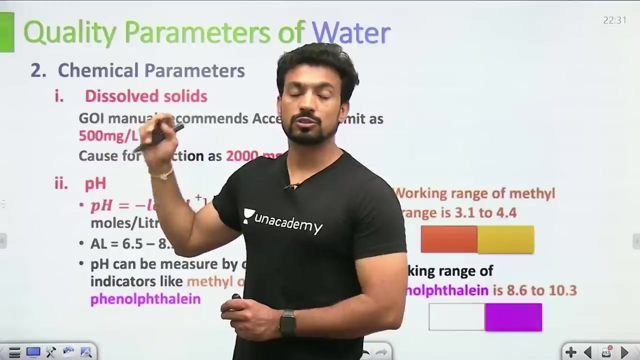 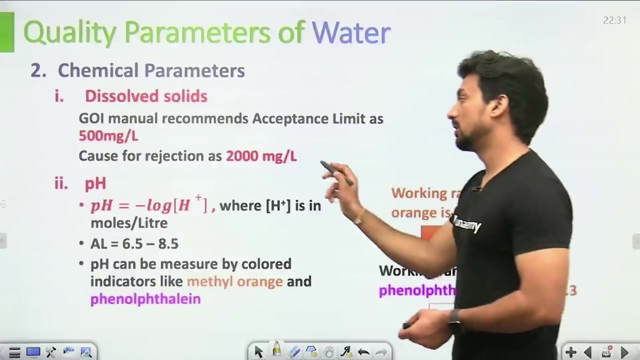 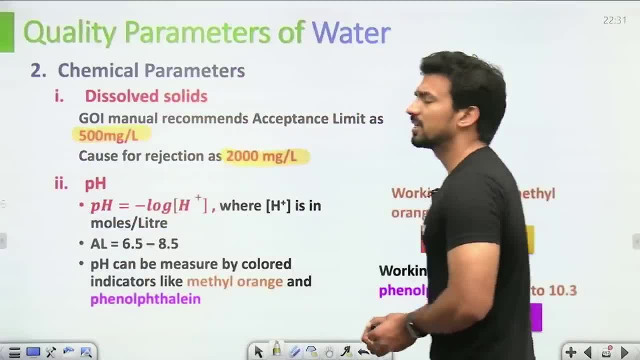 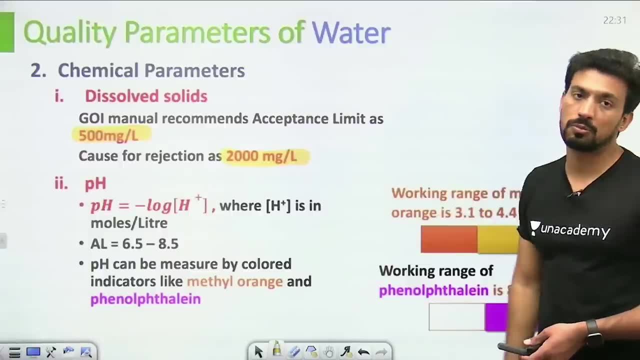 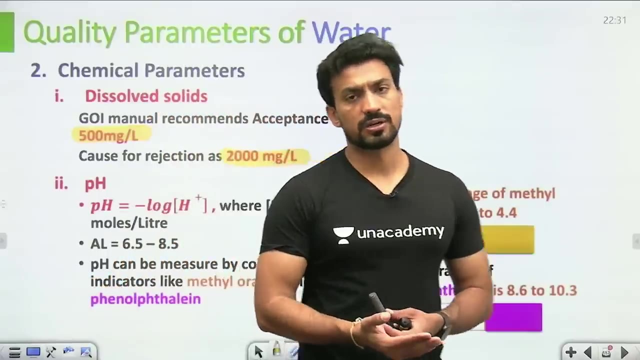 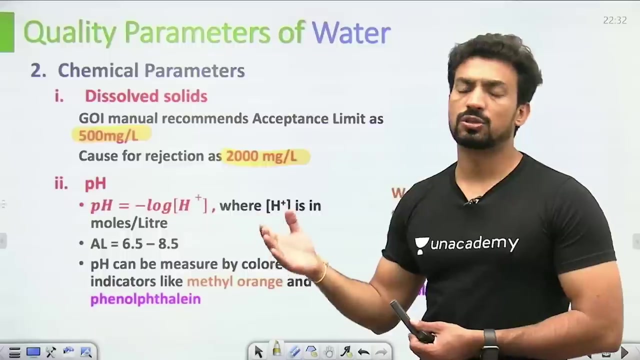 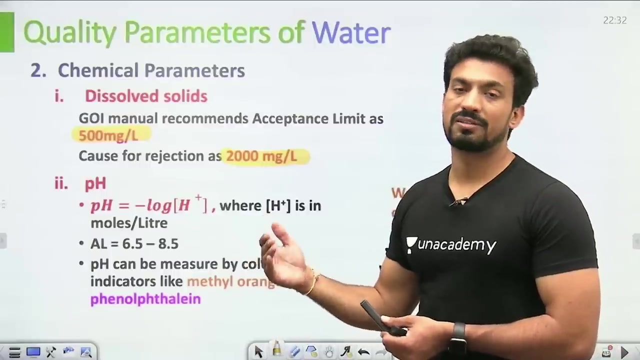 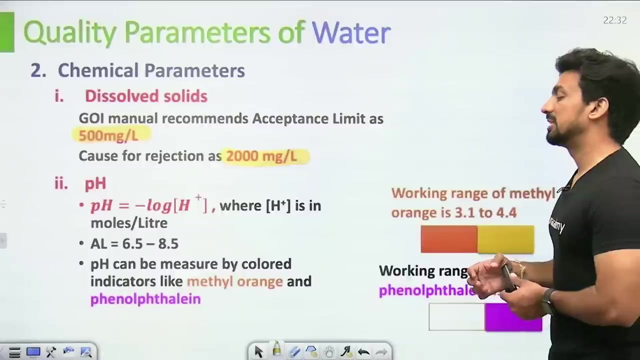 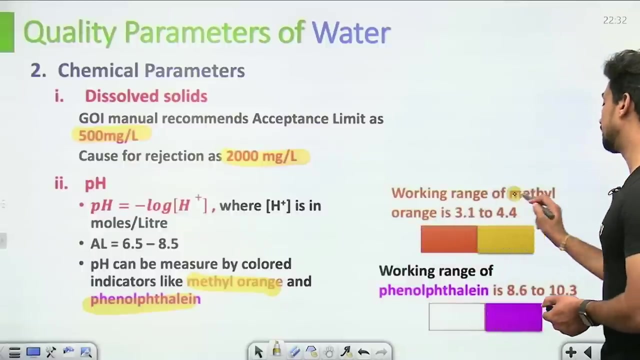 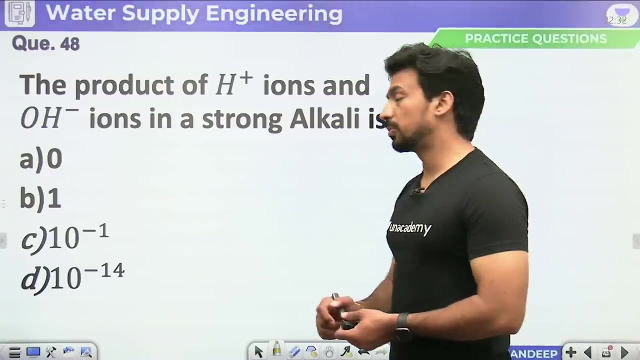 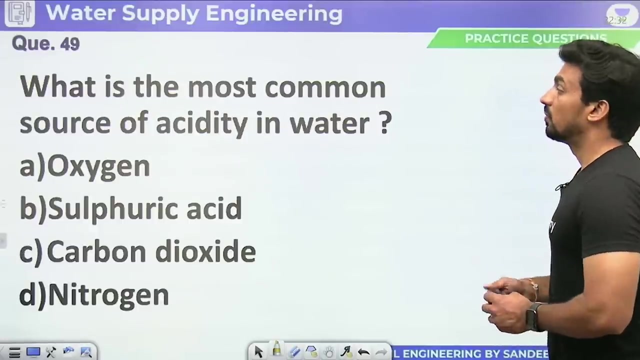 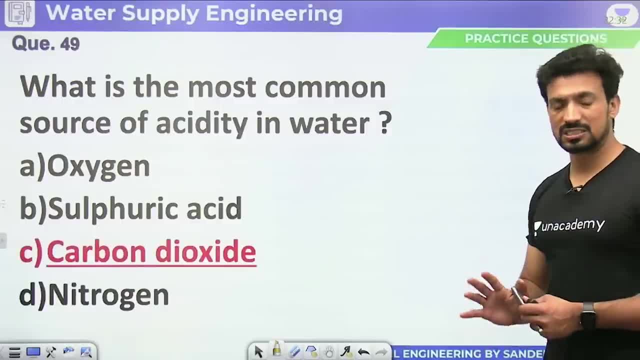 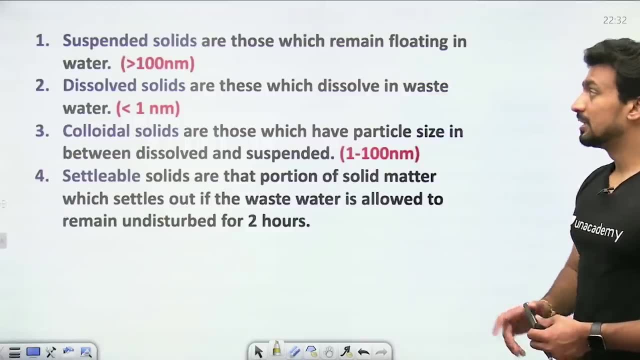 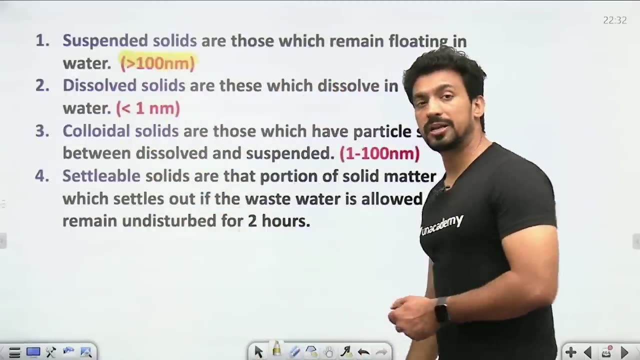 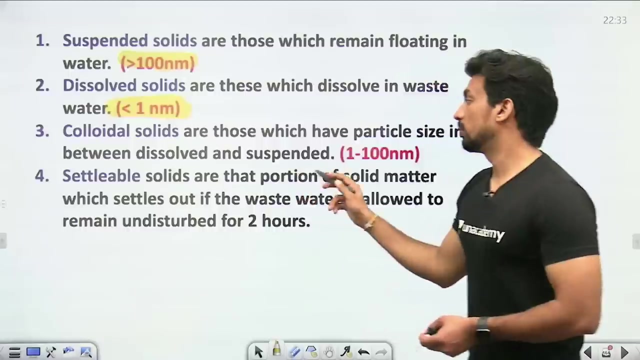 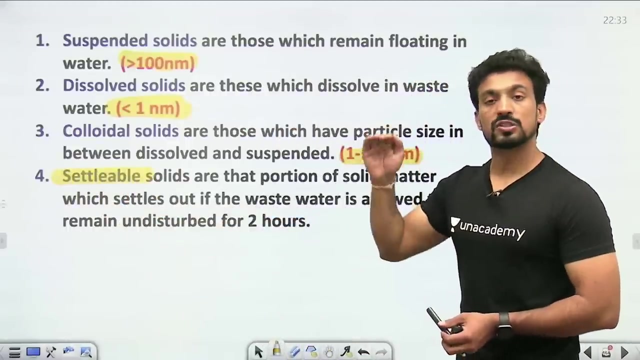 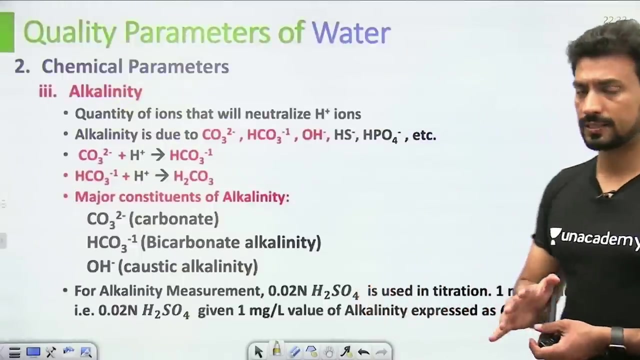 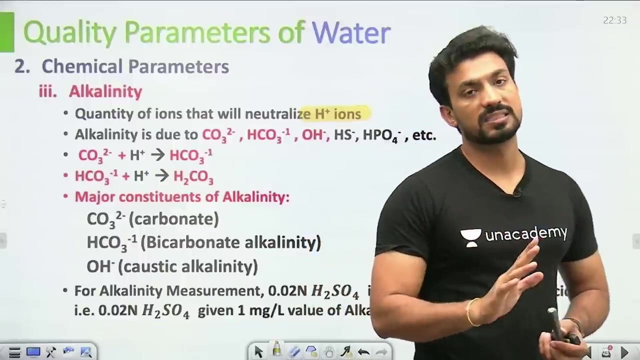 So 12.5 plus 187.5 divided by 12.5, the answer will come to be 16.. If we don't disturb them for 2 hours, then they will settle in water. Alkalinity is caused by ions that neutralize H-positive ions, like carbonate bicarbonate. 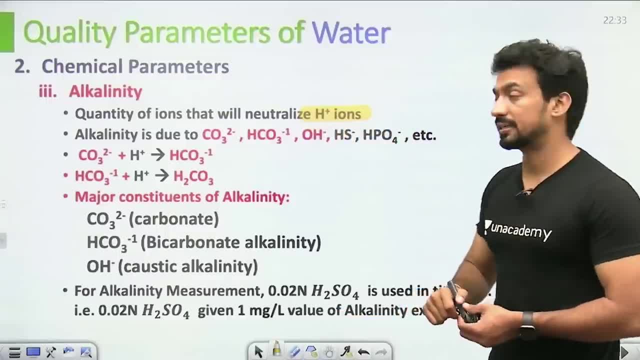 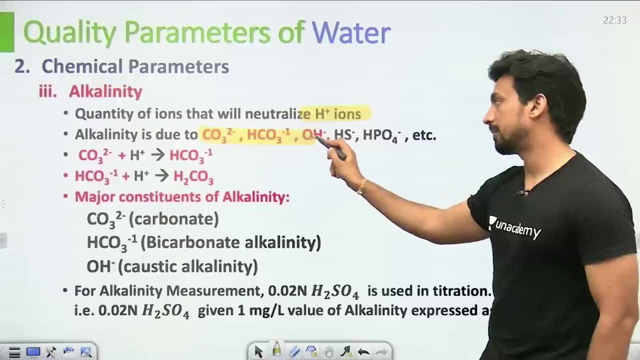 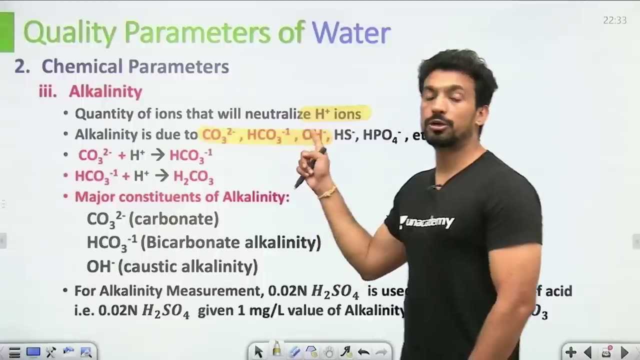 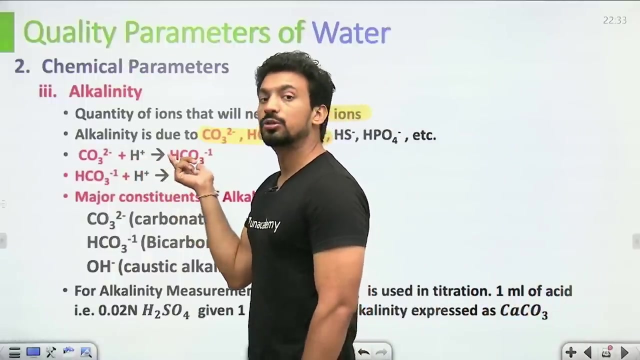 These are the ions that neutralize H-positive ions. They are called alkalis. Alkalinity is caused by carbonate, bicarbonate and OH-. If carbonate becomes H-positive with CO2-, then it becomes bicarbonate. If bicarbonate becomes H-positive, then it becomes H2CO3.. 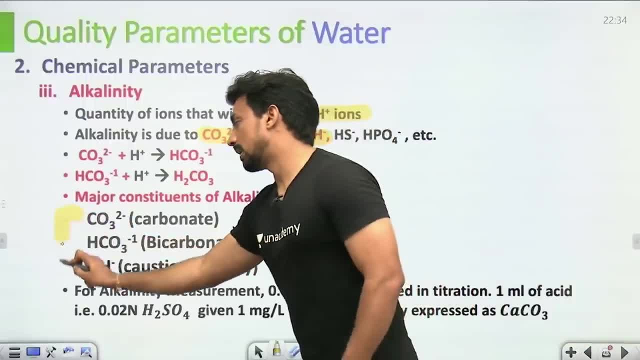 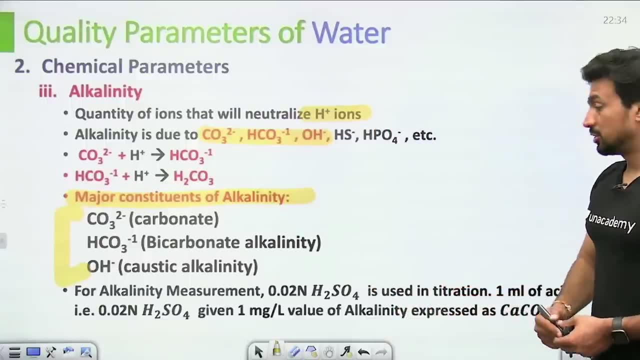 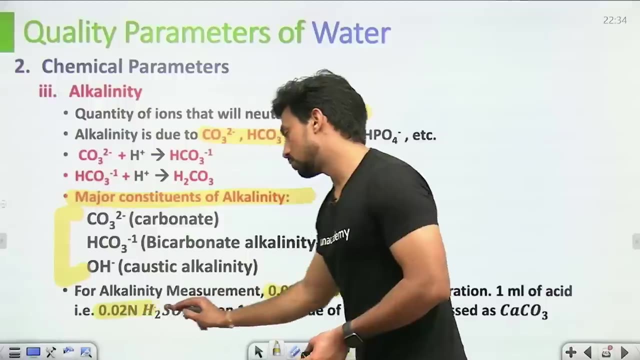 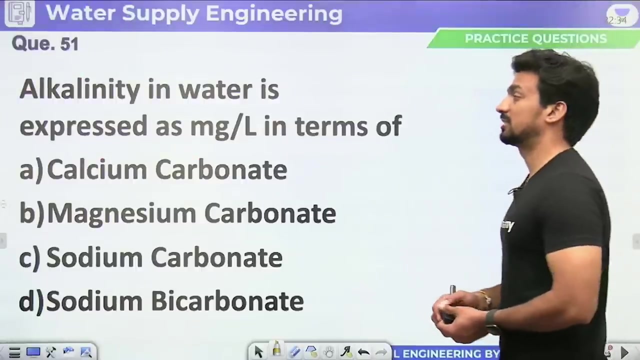 Major constituents of alkalinity are these three. You should know these three, If you don't remember anything else from this topic. For alkalinity measurement, H2SO4 of 0.02 normality is used in titration. 1 ml of acid which is H2SO4 of 0.02 normality gives 1 mg per liter of alkalinity which is expressed in the form of calcium carbonate. 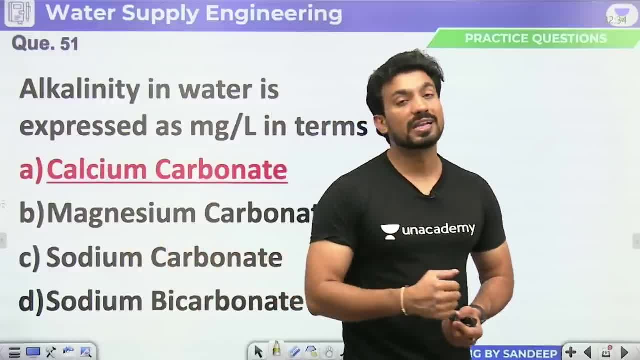 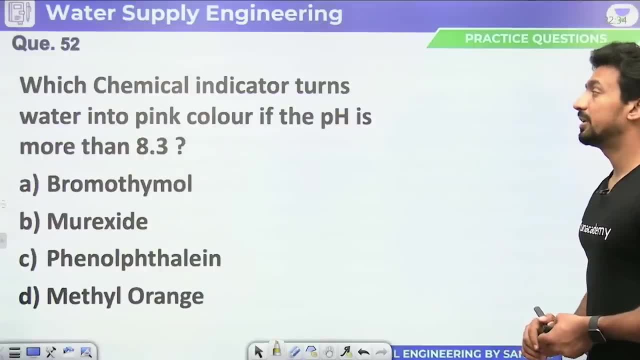 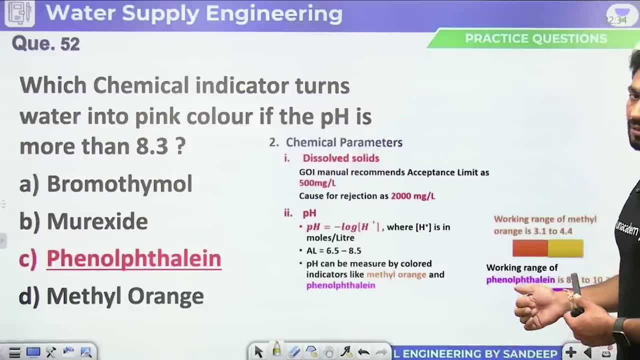 So alkalinity in water is expressed in terms of calcium carbonate. You have to remember this. Alkalinity in water is expressed in terms of calcium carbonate, Which calcium indicator, which chemical indicator turns into pink color. If you are told in alkaline range, then phenolphthalein will be given to you. 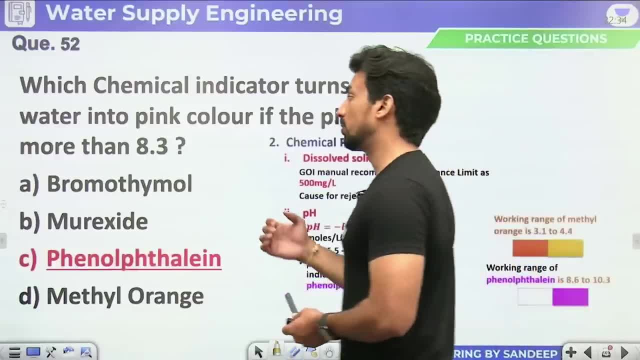 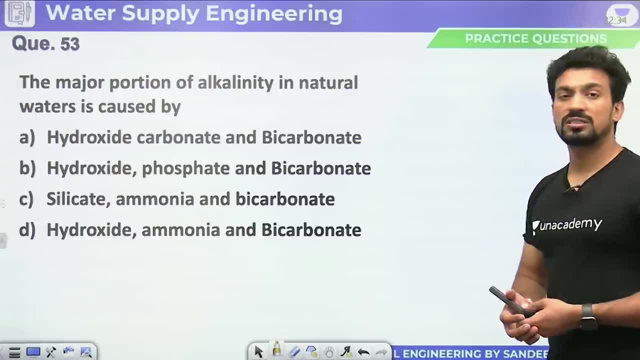 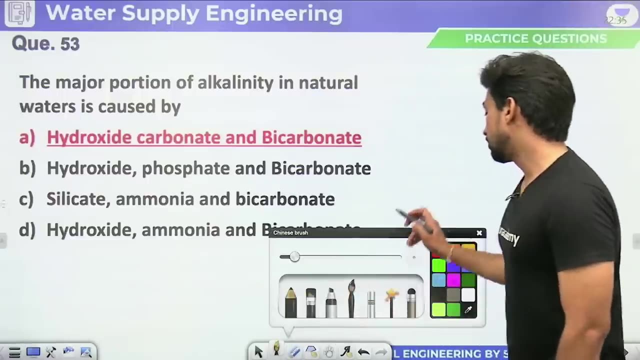 It changes from white to pink color and its working range will be more than 8.3 or it works in basic range. The major portion of alkalinity in natural water is caused by carbonate, bicarbonate and hydroxide. If we talk about carbonate, then you will denote carbonate. 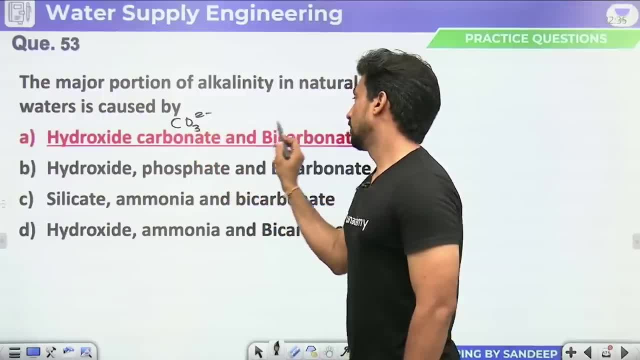 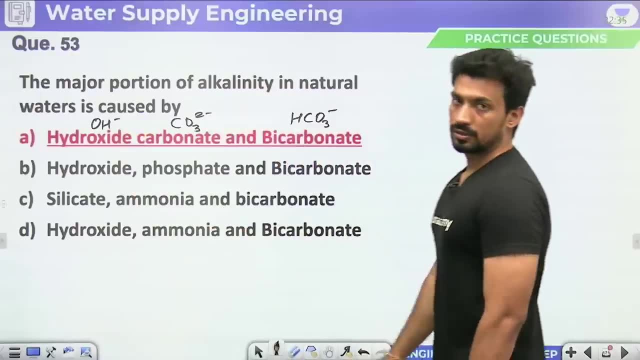 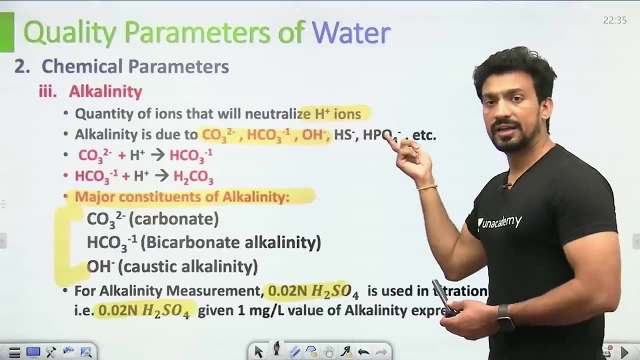 We will denote carbonate as CO3 2- bicarbonate as HCO3- and hydroxide as OH-. These are the three major ones. Apart from this, there are more. We also have minor ones. We have hydrogen sulfide, HPO4.. 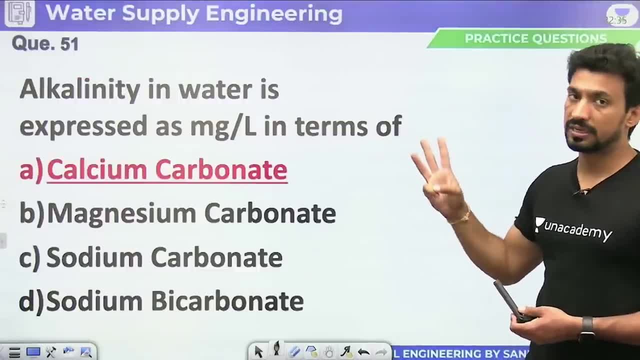 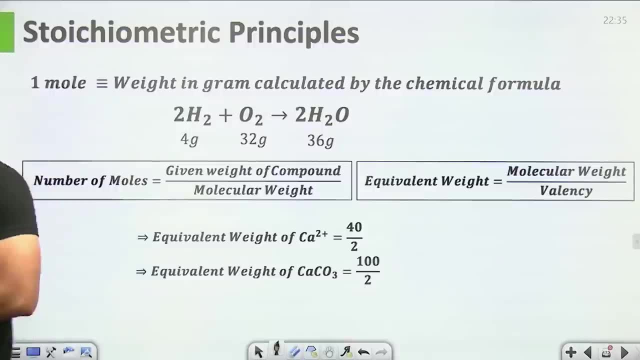 But the major ones we have are carbonate, bicarbonate, OH- These are the three major ones. Let's move on to the next question. This stoichiometry concept, I hope you will remember If you have done the classes. Even if you don't remember, then it's simple. 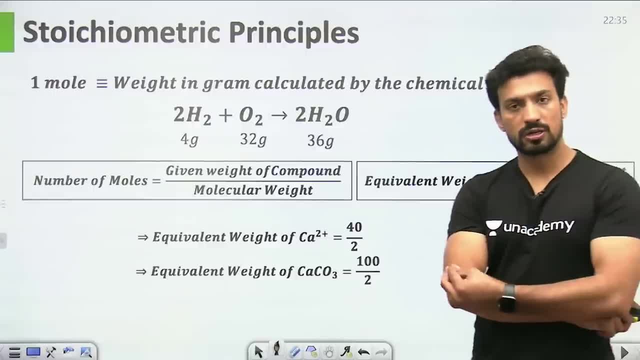 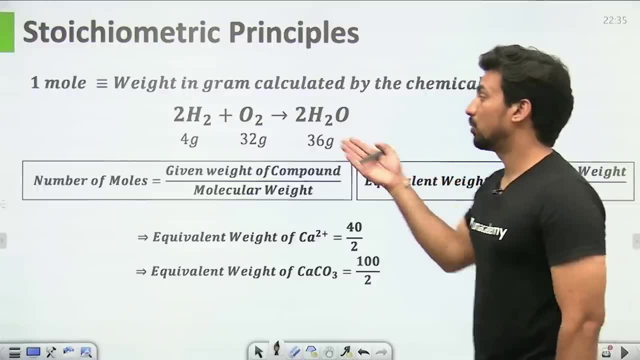 Mole is the given weight upon molecular weight of any quantity. What is the equivalent weight, Molecular weight upon valency, If I say mole of O2.. If we take 32 grams of O2, then you will say that it is 1 mole of O2.. 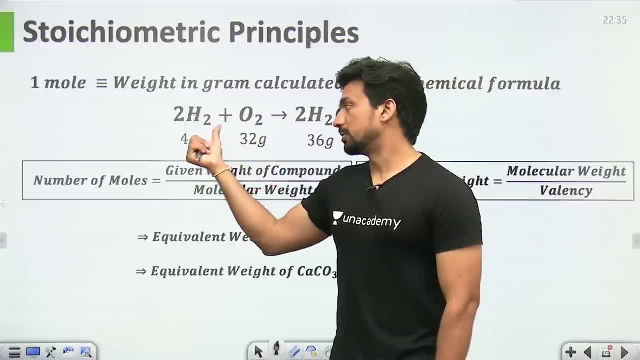 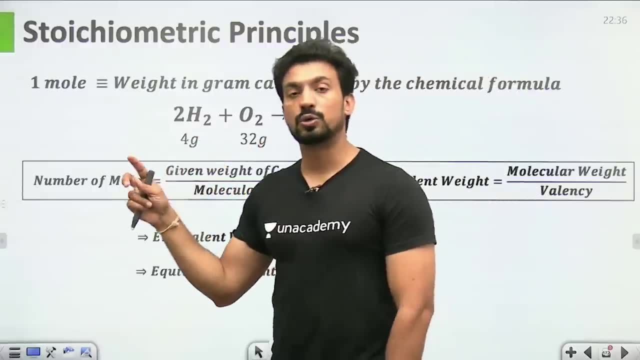 If you are told that it is the mole of H2.. If you are saying H2, then you will take 2 grams of any substance. If you take 2 grams of hydrogen gas, then you will say that it is 1 mole of H2.. 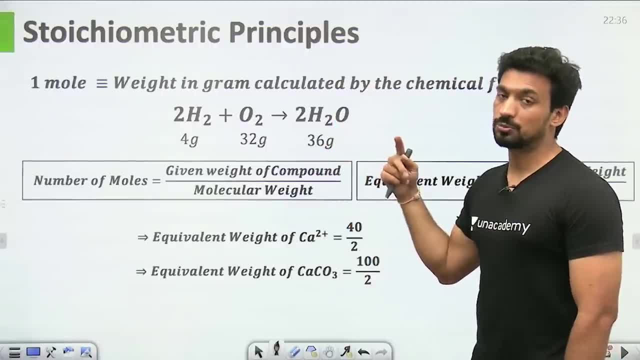 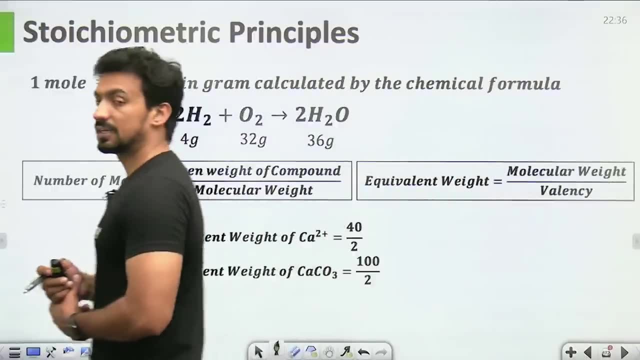 If you have H2O, If you have 18 grams of water, then you will say that it is 1 mole of H2.. If we have to calculate the equivalent weight, Then we divide molecular weight by valency, Then we get the equivalent weight. 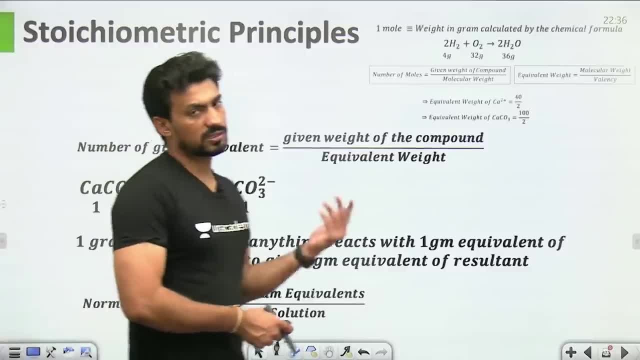 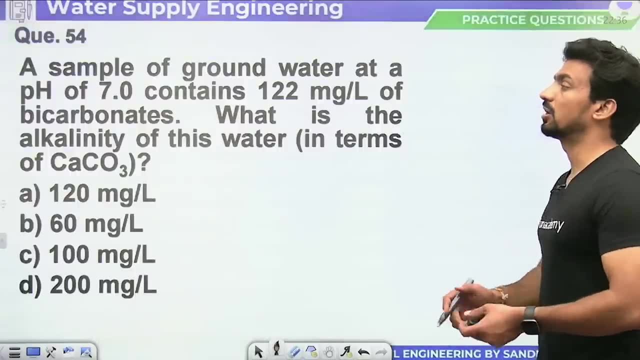 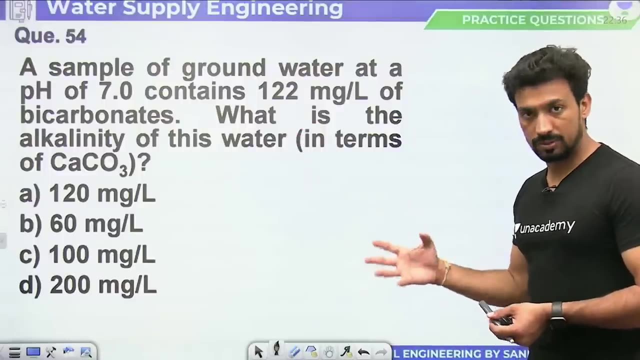 1 gram equivalent of anything reacts with 1 gram equivalent of any other thing to produce 1 gram equivalent of product. We use this concept to calculate equivalents And to convert In which terms which can be converted Like If we have to tell all things in terms of calcium carbonate. 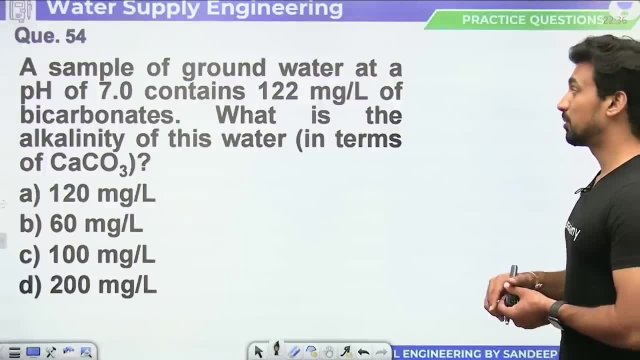 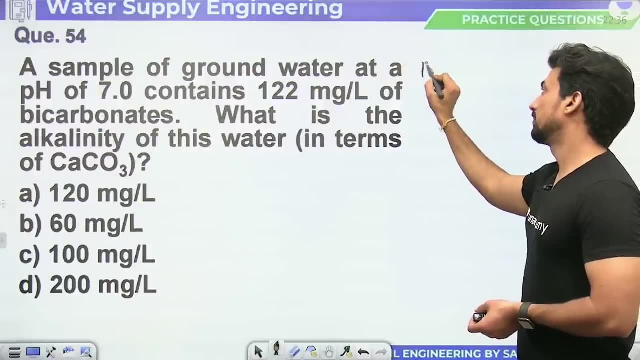 To calculate alkalinity, A sample of groundwater at a pH of 7. pH of 7 means that you have POH is also 7. Because pH plus POH is 7. So if you have pH 7, then POH is 7.. 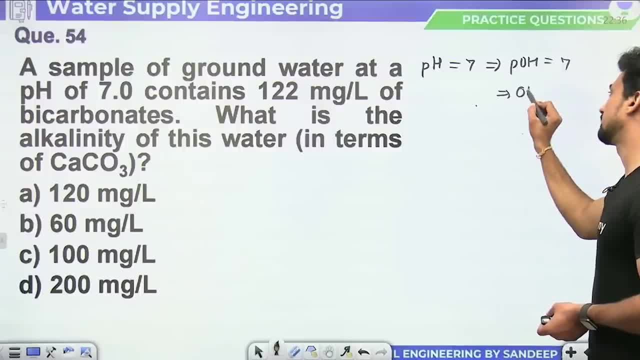 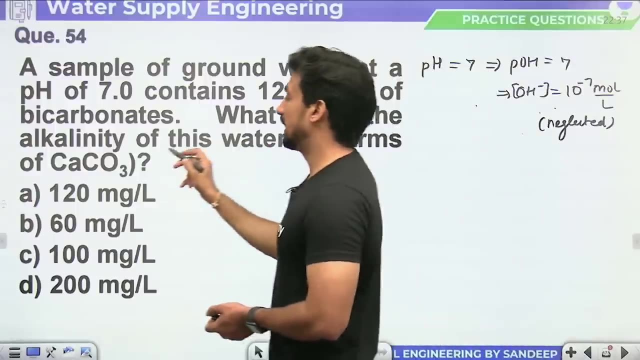 POH 7 means that here the concentration of OH minus is how much 10 raised to the power, minus 7 moles per liter. This is very less, So we will neglect this. Because of whom is alkalinity? What is the alkalinity? 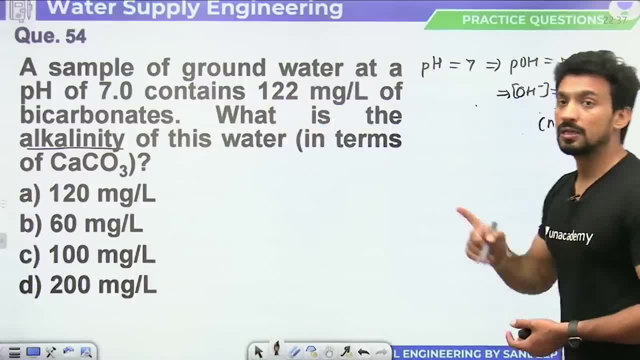 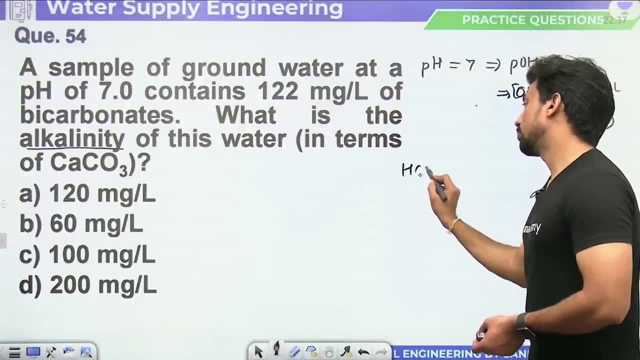 Alkalinity is carbonate, bicarbonate and OH minus. I neglected the OH minus one In the question. you are given 122 milligrams per liter. bicarbonate is present. Bicarbonate means HCO3 minus. HCO3 minus is given to you. 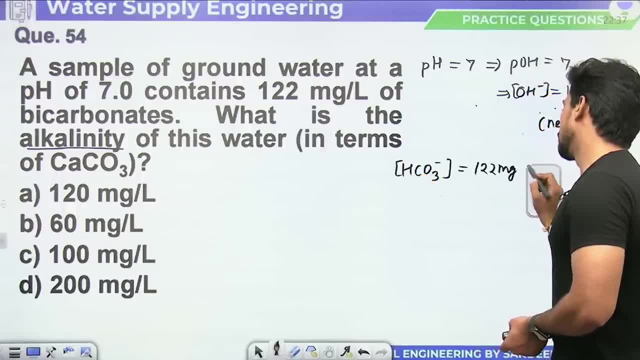 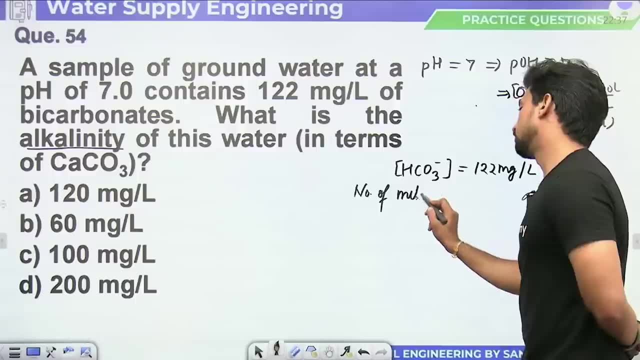 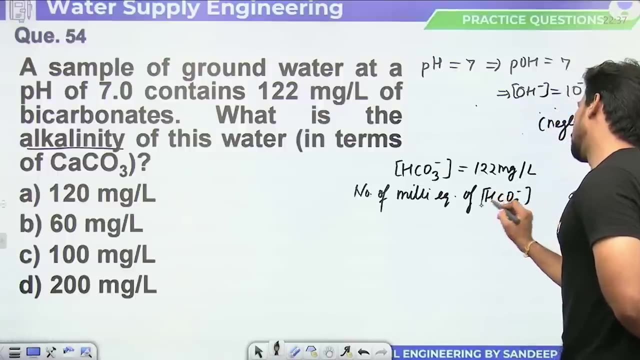 122 milligrams per liter. So calculate the number of gram equivalent Or we will say the number of milli equivalent. There is a milligram here, Number of milli equivalent of HCO3 minus. How do we calculate the number of milli equivalent? 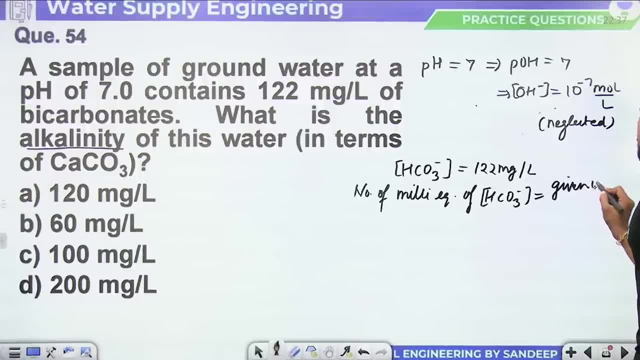 We will calculate the number of milli equivalent. How much is the given weight Upon How much is the equivalent weight? Given weight is 122.. How much is the equivalent weight? HCO3 minus is 61.. Molecular weight is 61.. 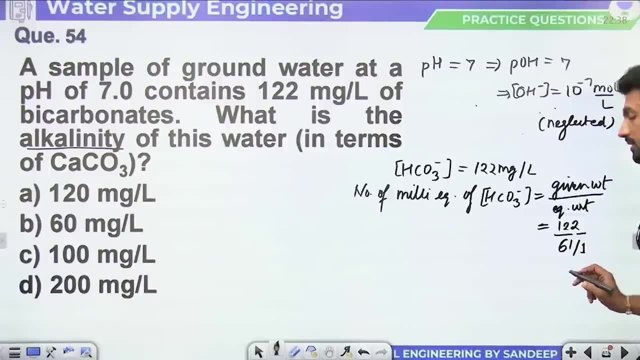 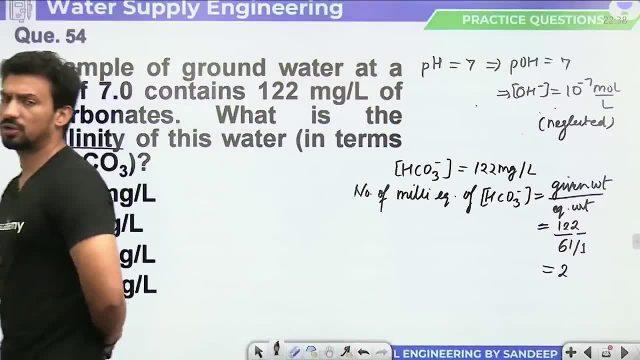 Valency is 1.. Equivalent weight is molecular weight by valency. So from here you have 2 milli equivalent And this 1 gram equivalent of anything reacts with 1 gram equivalent of any another thing To produce 1 gram equivalent of resultant. 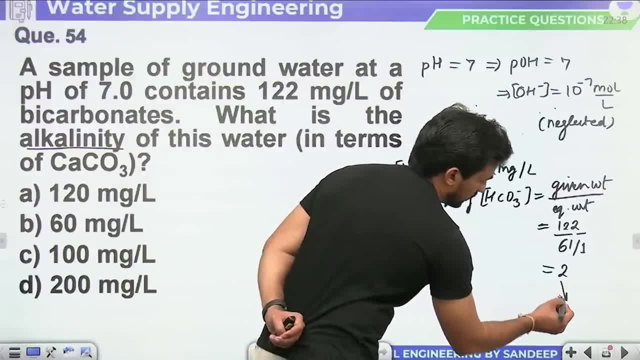 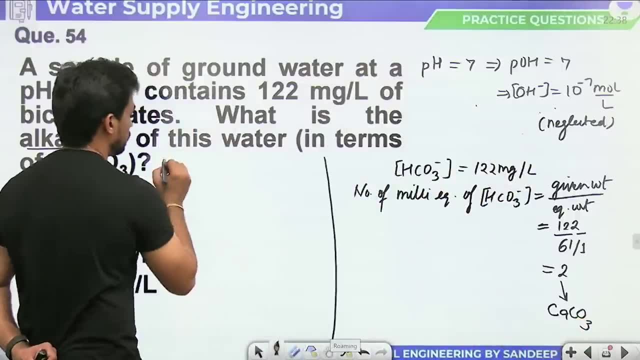 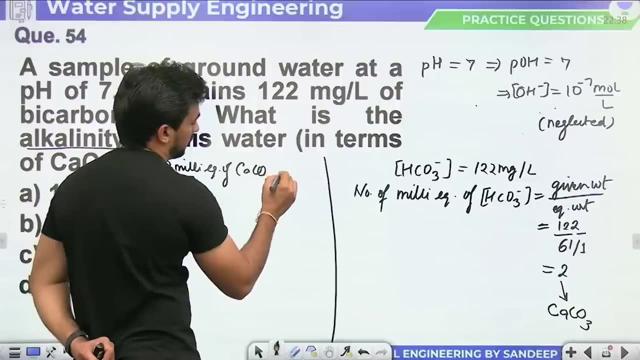 So from that we will say that this 2 gram equivalent Or 2 milli equivalent Will also be 2 of calcium carbonate. So if you will tell That 2. Milli equivalent of Calcium carbonate Will be equal to. 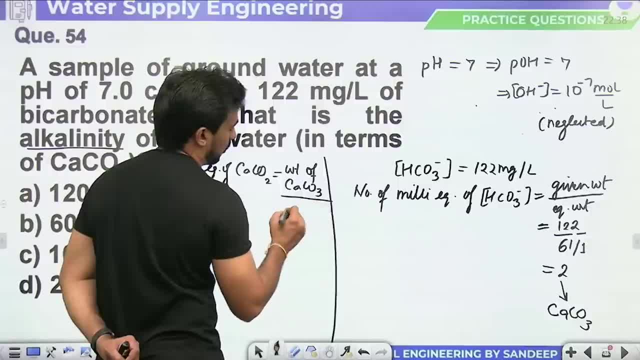 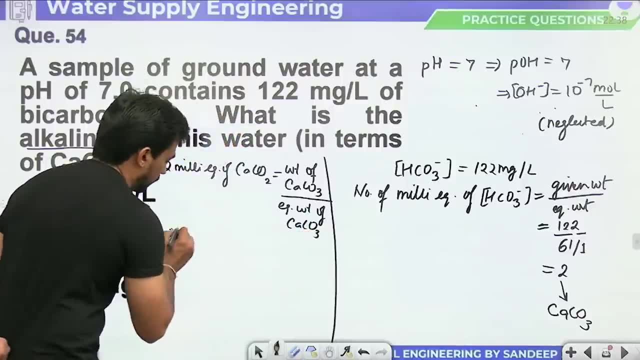 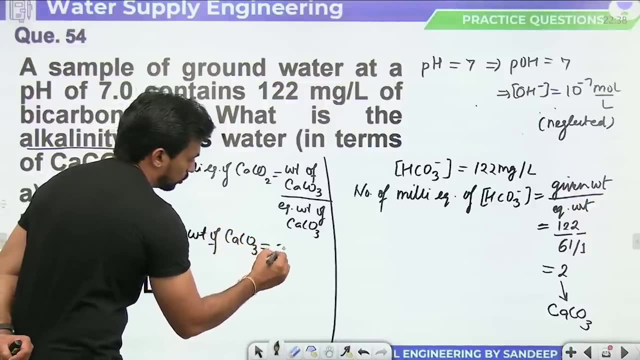 Weight of calcium carbonate Upon Equivalent weight of Calcium carbonate. We have to know the weight of calcium carbonate, Or in terms of calcium carbonate, alkalinity, So 2, into Given weight upon Equivalent weight. Equivalent weight of Sorry. Given weight upon valency, Equivalent weight of calcium carbonate will come 100 by 2.. Bring this 100 by 2. here We have the weight of calcium carbonate. So 100 milli gram Per liter Equivalent Will be equal to. 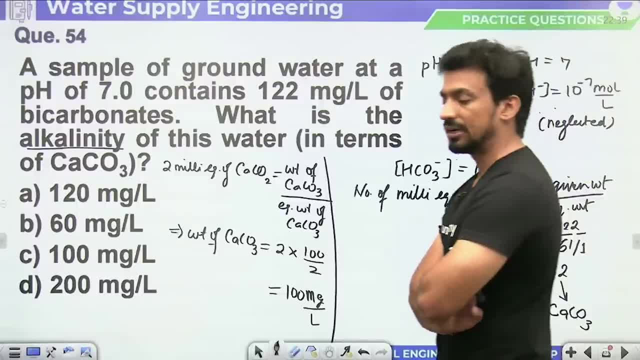 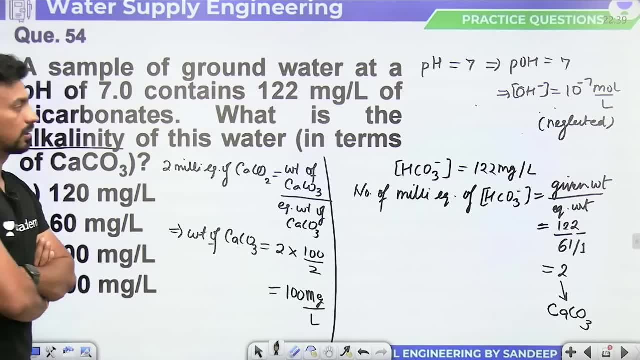 Weight of calcium carbonate Over here. So we will add, We will add 1.. So, 1. About this. So This Ray, We will calculate weight of calcium carbonate, of Calcium carbonate, Calcium carbonate Over here. 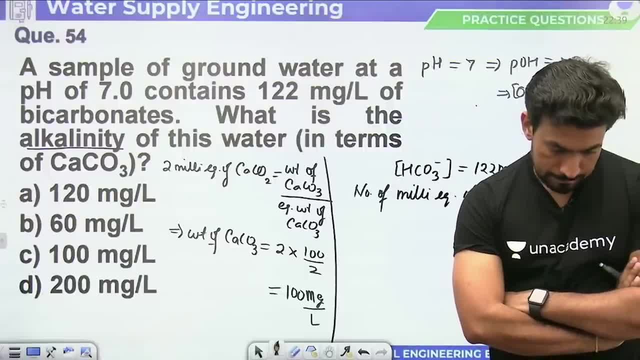 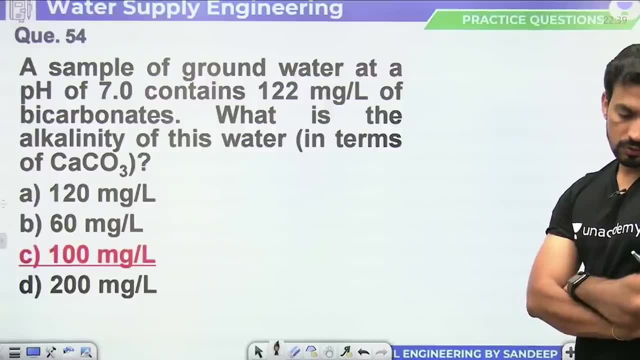 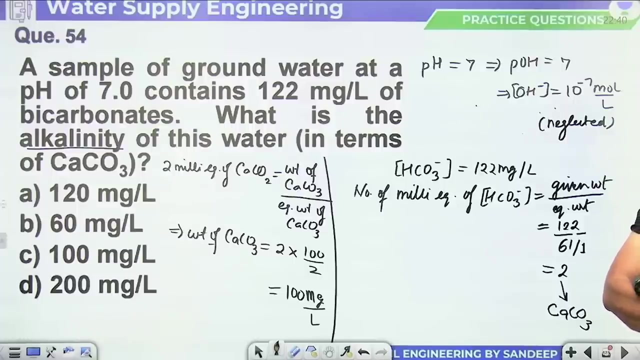 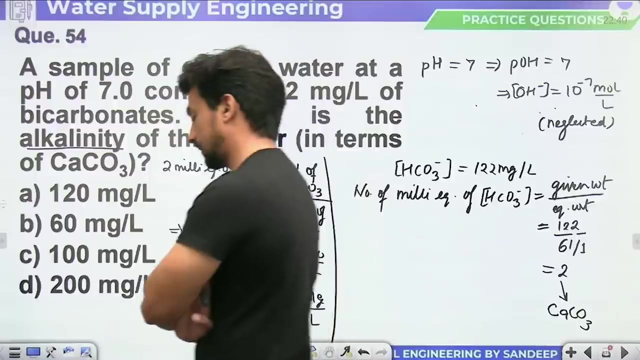 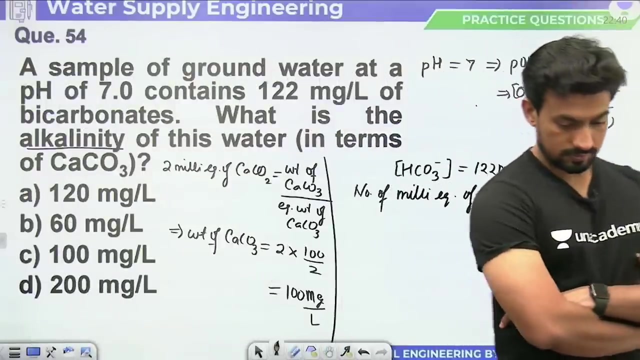 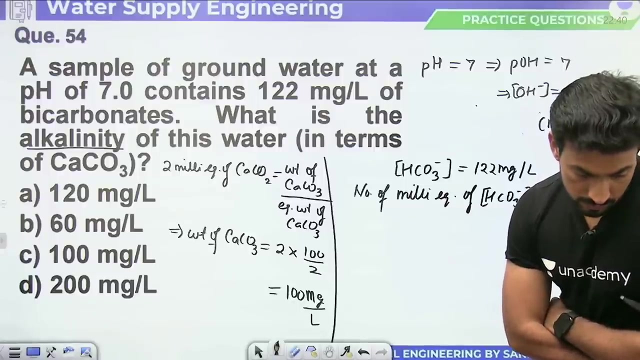 We will write That. We will write That Weight Next. The question is very big, Bigger than your dreams. These are small obstacles. Why are you looking at them Side? please Take this friend, Sir: how to make a shortcut. 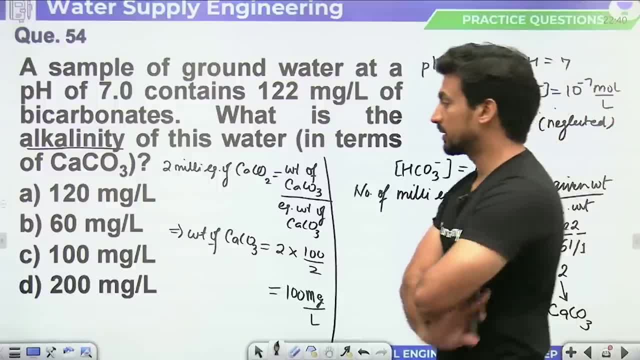 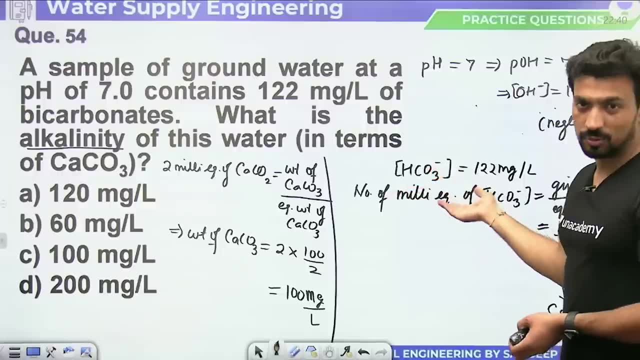 Do you want to close your eyes? Do you want to hold hands? Do you want to say Jai Maat? You will get the answer. Look, I have written the formula. Shortcut means that you do not write this formula. It is given directly. 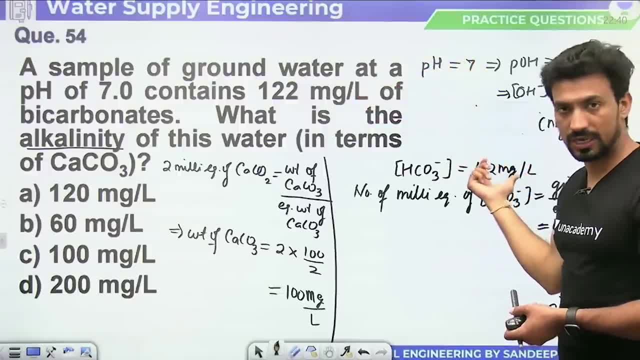 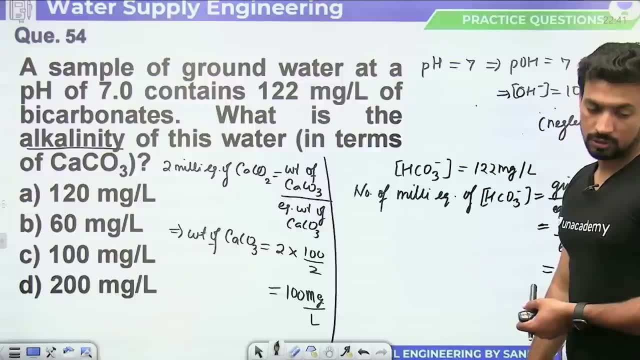 You have written directly. You have seen 122.. According to 122, number of gram equivalent: 2 came. Write it as 2 equals 2.. So you can save time in this. I have to write all this Because I have to explain it to everyone. 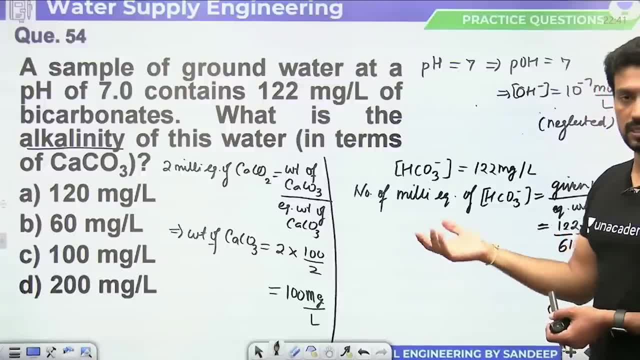 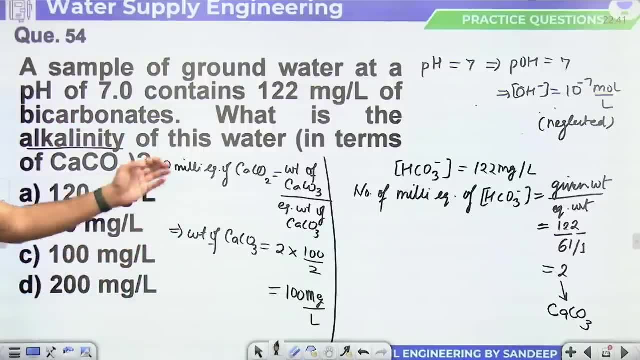 May be there is a friend who does not understand it If I write it directly So that no one is confused. That's why I have to write it all. If you get this topic, then you write it quickly. You have a lot of time to write it. 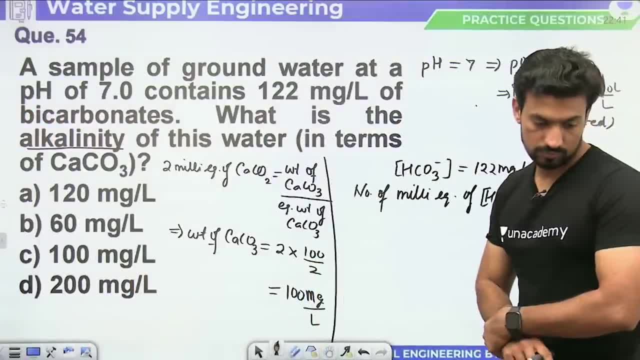 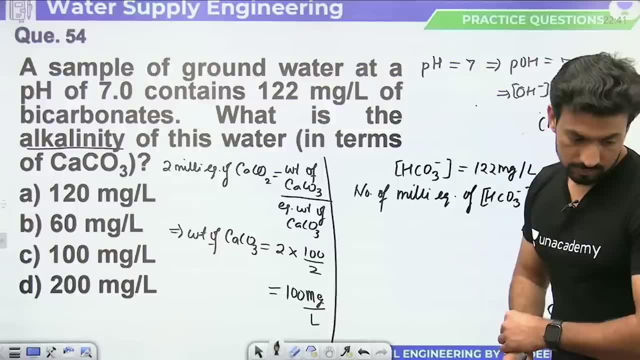 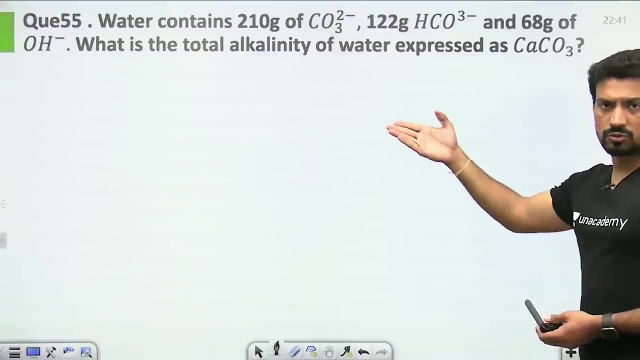 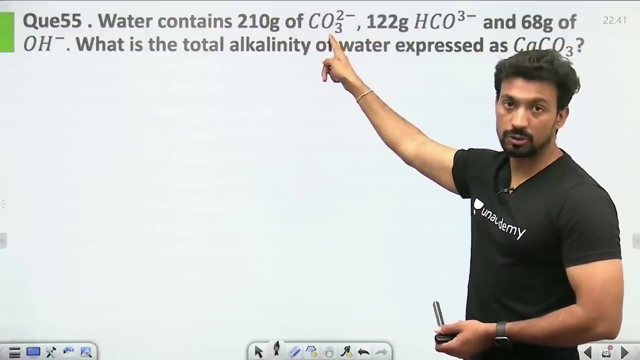 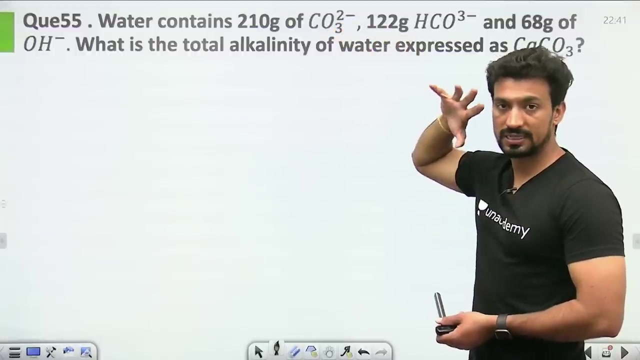 You have to do this in the objective. Let's move ahead next. in the same way, one more question was done in the class that if you have 210 grams of carbonate, then how will you convert it to 10 divided by the weight of carbonate, 60, how much is its valency? 3, so 2, so 60 divided by 2, so you will get the weight of carbonate. 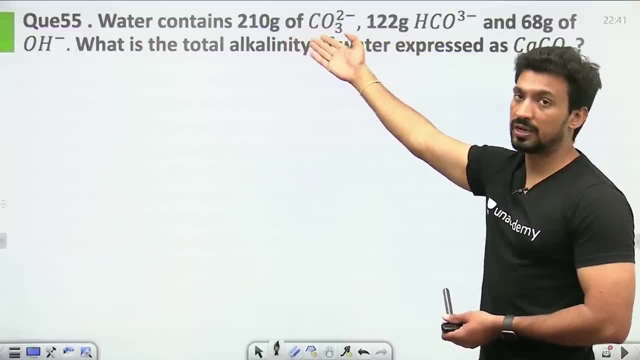 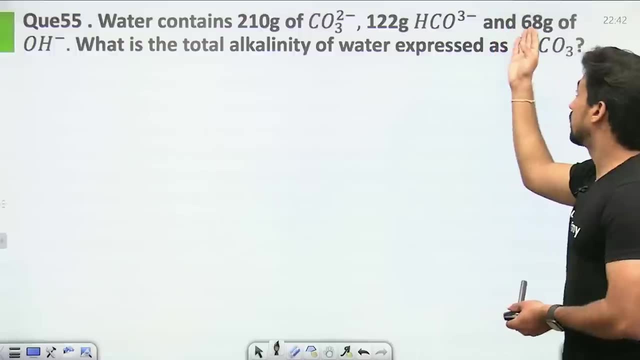 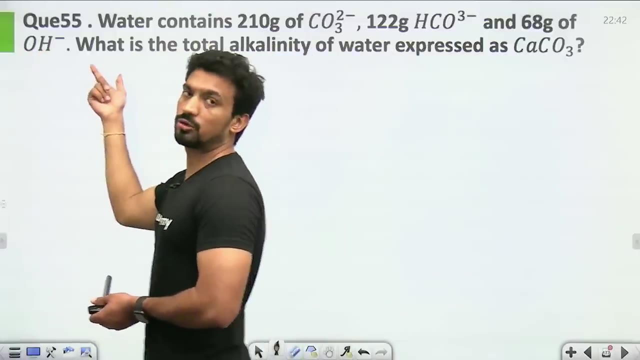 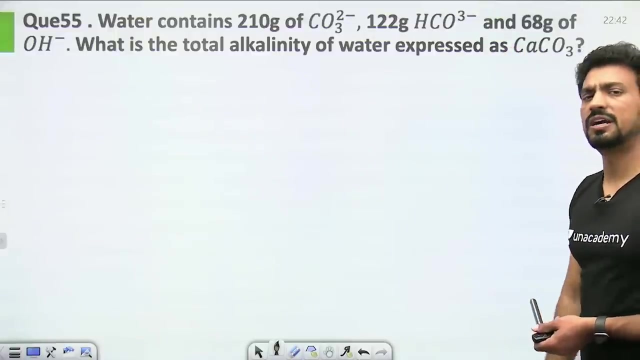 equal weight. given weight, so number of gram equivalent will come 122 gram hco3- you can write 122 divided by 60 to 1 divided by 1, this you can write 68 gram of OH- so in 68 gram of OH- you will divide that molecular weight of OH by 1, so you will get equivalent weight, 68 divided by OH. so you have to do 68 divided by 17 divided by 1,. 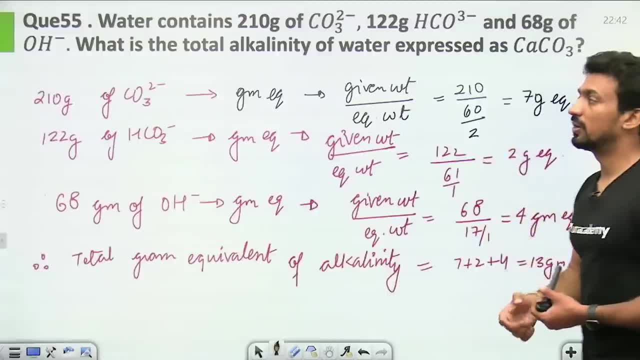 so 210 divided by 60, divided by 1, We are converting it to gram equivalent. we can write 210 gram carbonate in gram equivalent, given weight upon equivalent weight, which will be 210 by 60 by 2.. Equivalent weight is given mass upon sorry, molecular mass upon valency. 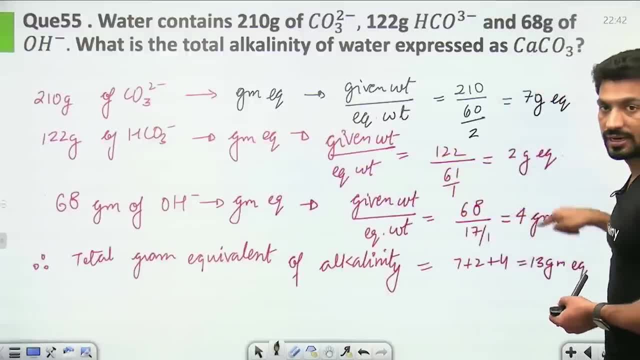 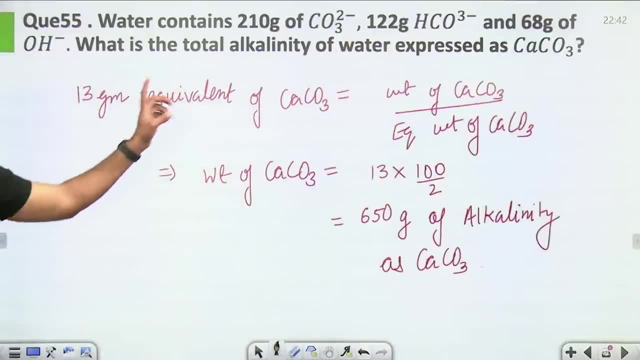 In the same way we wrote 122, one like this. we added all the weight. 13 gram equivalent came. 13 gram equivalent will be equal to calcium carbonate. so if 13 gram equivalent is of calcium carbonate, then how much weight of calcium carbonate will be? this can be. 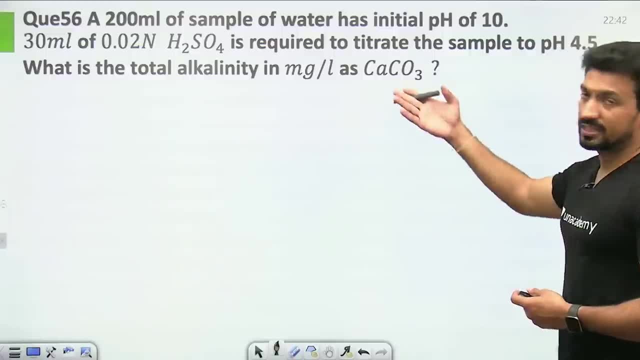 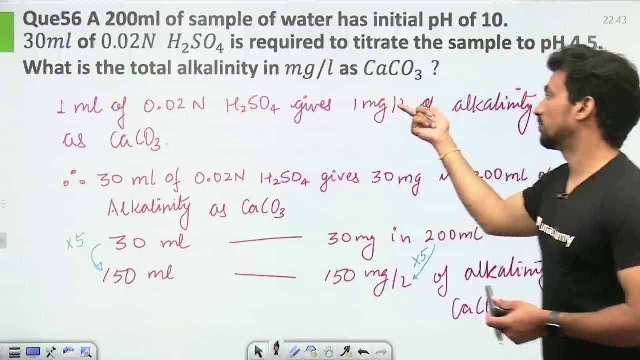 calculated. Next. then, in the same way, we had another question in which we used that 1 ml is 0.02 normality H2SO4, so it provides 1 mg per liter alkalinity- 30 ml if you have 0.02 normality. 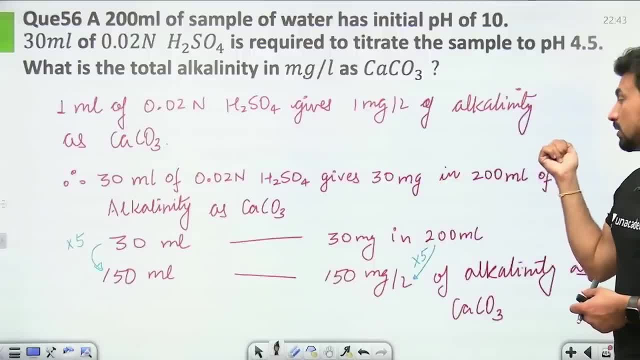 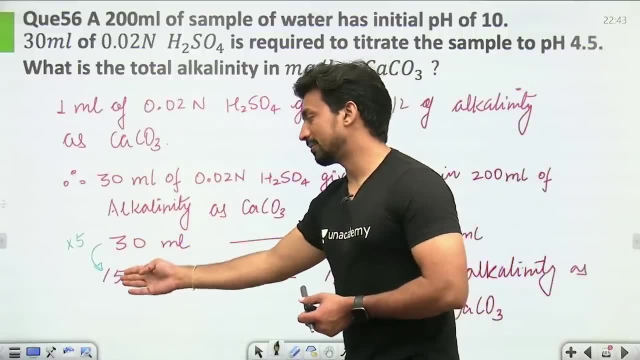 H2SO4,, then it will provide 30 mg per liter. if you use 1 liter in 200 ml, then it will provide 1 liter in 200 ml. So if you will tell the corresponding of 500 ml, then you are asking 150 ml instead of. 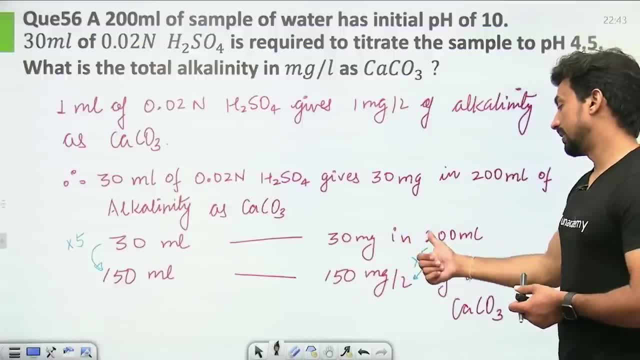 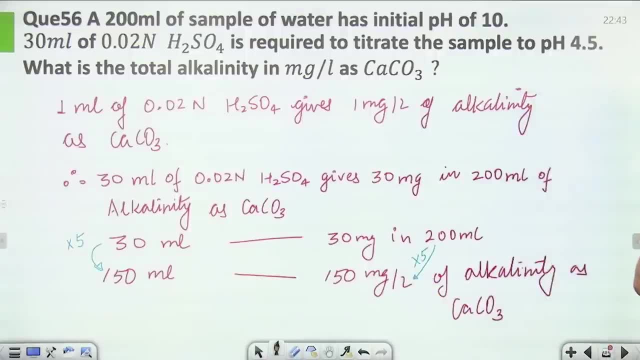 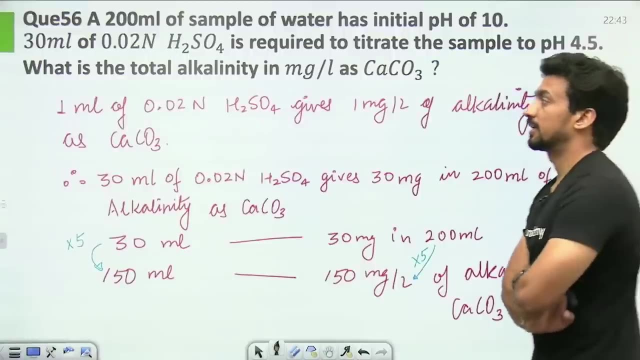 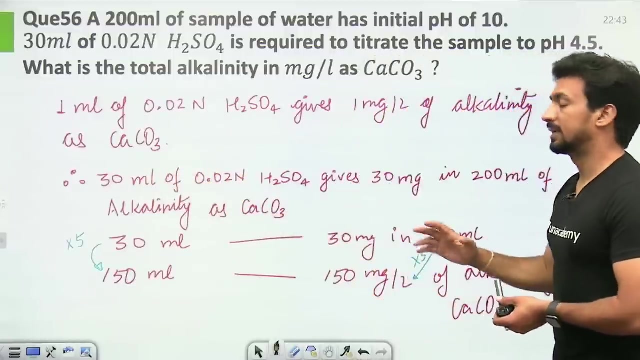 30 ml, then 30. you have to divide it by 5. on this side it will be 1 liter instead of 200 ml. In the question you were given that this much acid was utilized in 200 ml sample, then in 300 ml. if the acid of 0.02 normality was utilized then sorry, in this case the 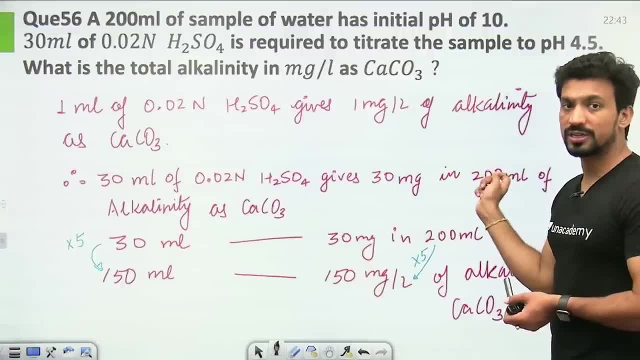 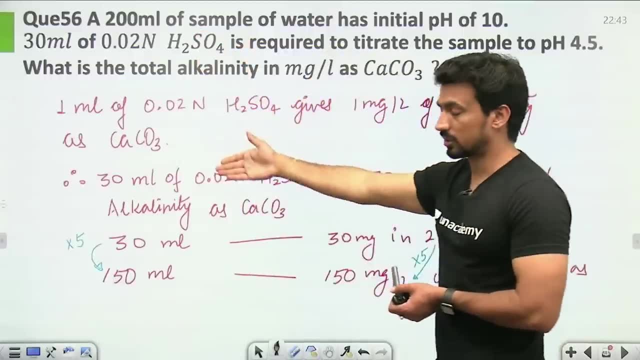 acid of 0.02. normality was 200 ml. then 200 ml of alkalinity was present in the form of calcium carbonate, 200 ml of water was present, 30 ml of acid was used, so 30 mg was provided. 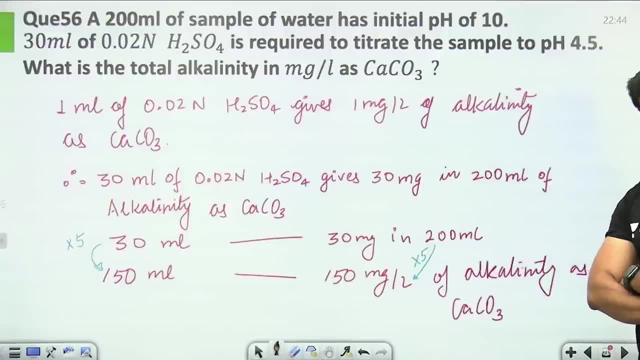 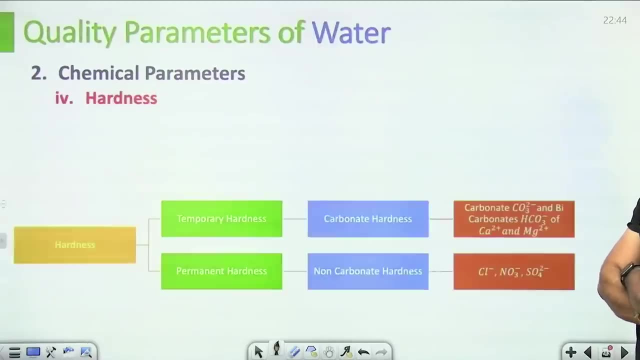 to you by alkalinity. if he provided 30 in 200 ml, then how much will be in 1 liter? we will divide it by 5.. Okay, Okay, Okay, Okay, Okay, Okay. Next let's go ahead. then comes the hardness. 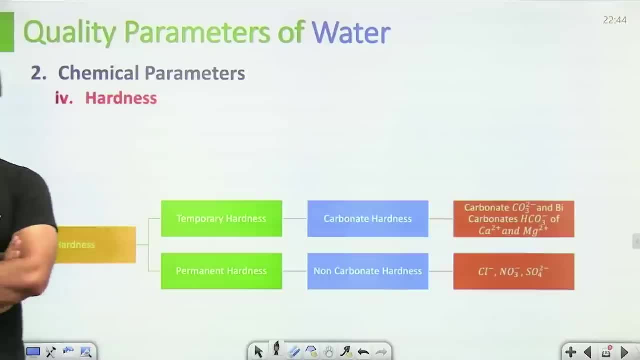 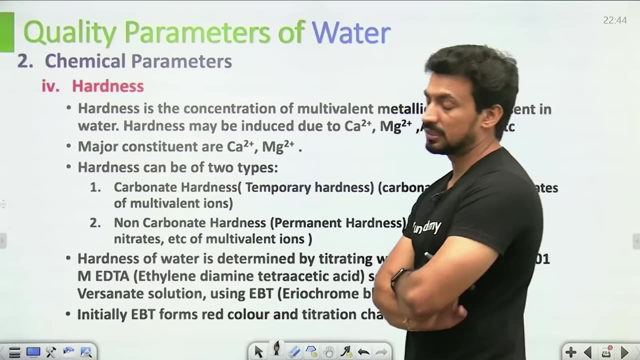 The hardness is of two types: temporary, which will be with carbonate and bicarbonate, and permanent, if that is because of chloride nitrate sulfate. Temporary hardness can be removed from boiling or simple processes. permanent hardness can not be removed. The hardness is known through titration: 0.01 normality of EDTA ethylene diamine tetra. 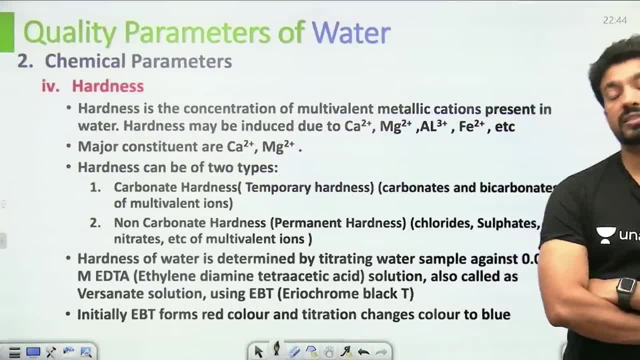 acetic acid is used in the presence of indudated acid. in the presence of cavities, The temperature is made to be 0.9 degree centigrade. that is, if the temperature is zero, then the hardness is equal to 0.2.. 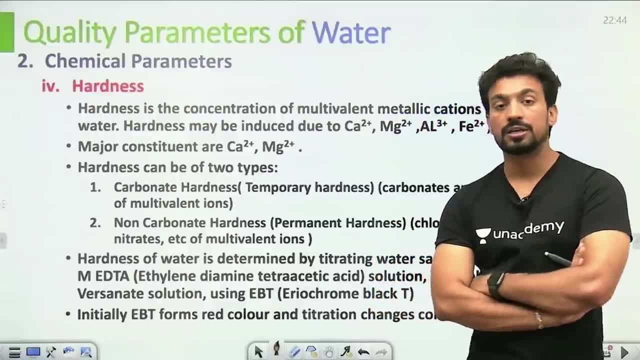 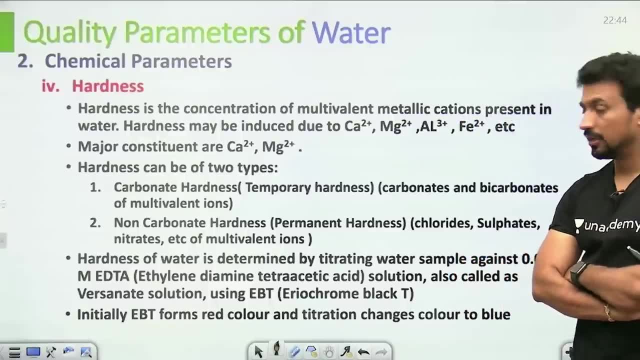 So, for example, if there is boiling, then the temperature is zero. In the presence of indicator ariochrome black tea, which initially forms a complex of red color and later, due to titration, it is converted into the form of blue, 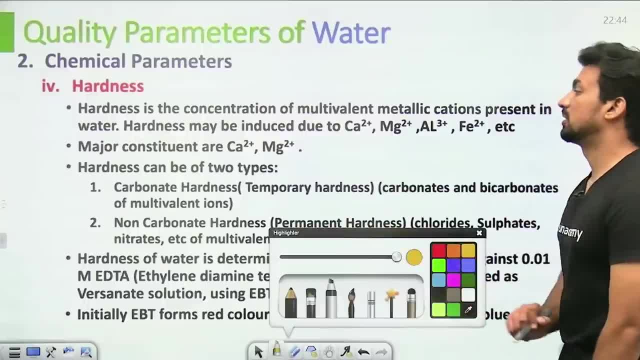 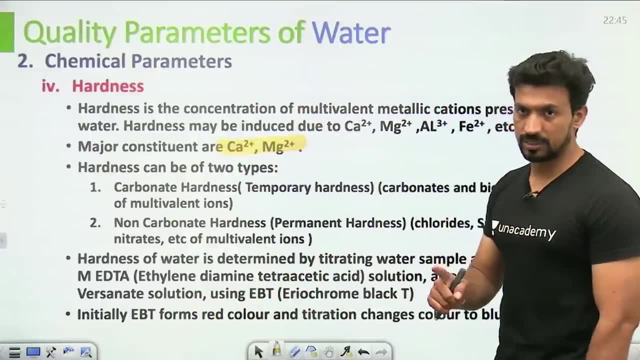 In the objective. all these questions will be asked to you. What questions will be asked? What is the major constituent of hardness? What are its cations? There is calcium and magnesium. Apart from this, aluminum can also be there. iron can also be there. 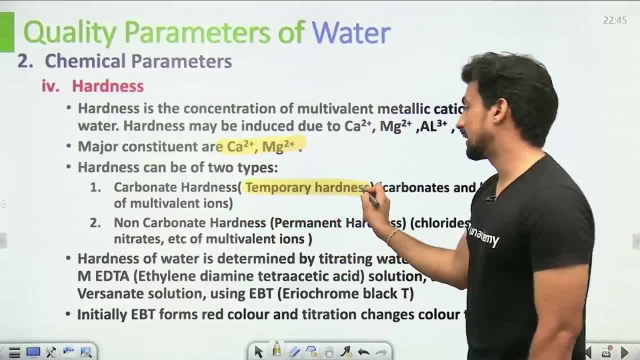 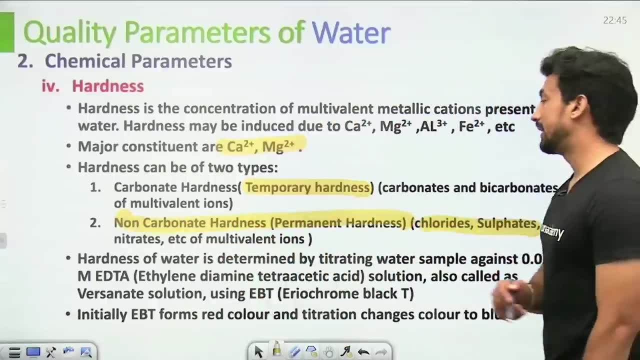 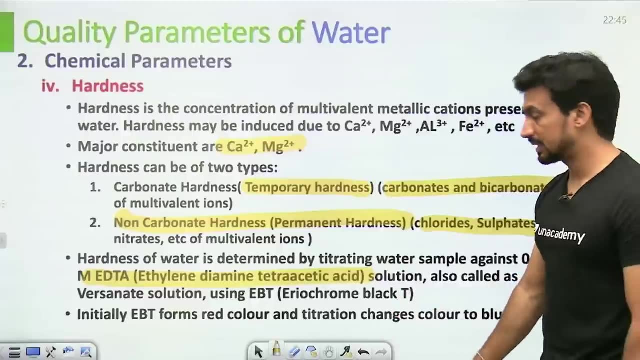 Calcium and magnesium Carbonate hardness is also called temporary hardness due to carbonate and bicarbonate. Noncarbonate hardness is called permanent hardness due to chloride, sulfate and nitrates. You should know this EDTA is used for ethylene diamine. tetraacetic acid hardness. 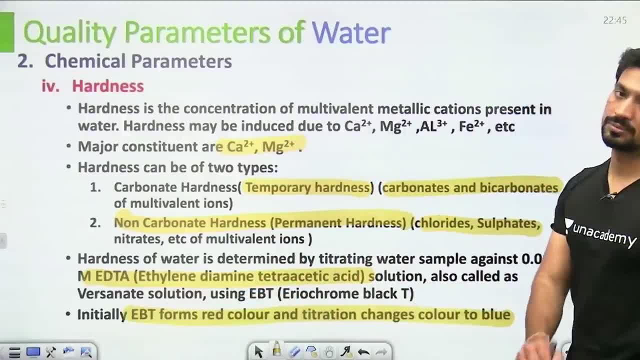 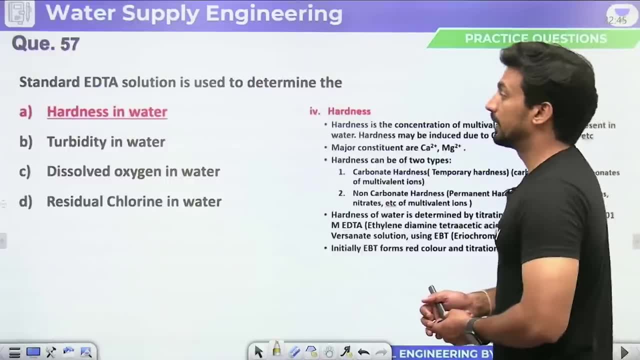 And the color formed by ariochrome black tea is also asked to you. in the objective Standard, EDTA solution is used to determine the hardness in water. Next, let's go ahead. The presence of carbonate, The presence of calcium and magnesium chloride in water causes 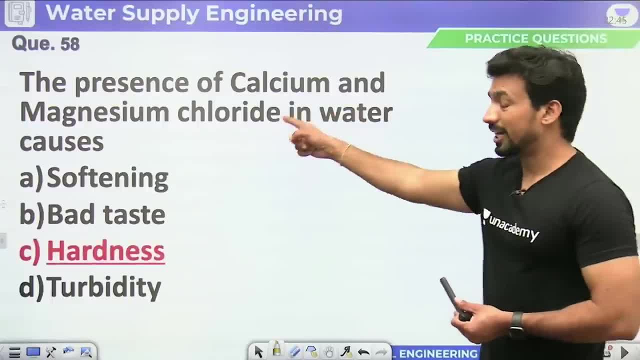 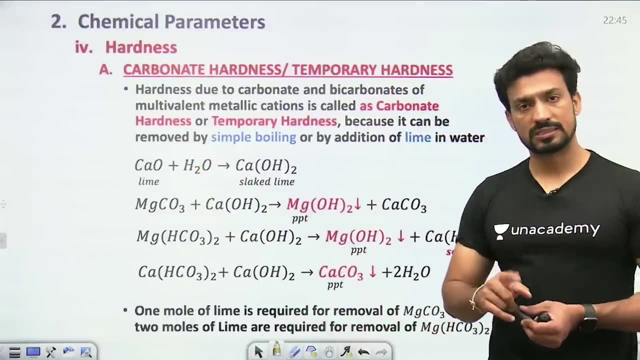 If calcium and magnesium are present, then there will be hardness. If chloride is present, then there will be permanent hardness. If I ask you that question in more detail Now, if there is temporary hardness, then it can be removed from boiling Or add lime. If you add lime in water, then it is added in the form of calcium oxide. 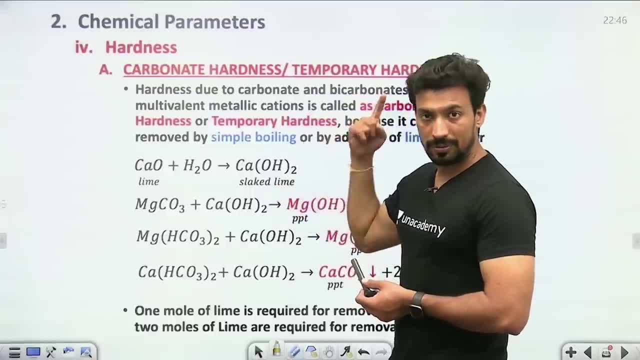 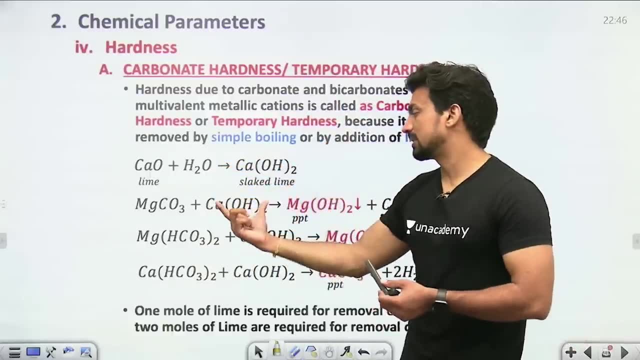 Calcium hydroxide is formed. This is calcium hydroxide. Now impurity is present in water. If the impurity or hardness in water is magnesium carbonate, Then magnesium carbonate will react with lime and make the precipitate of magnesium hydroxide. 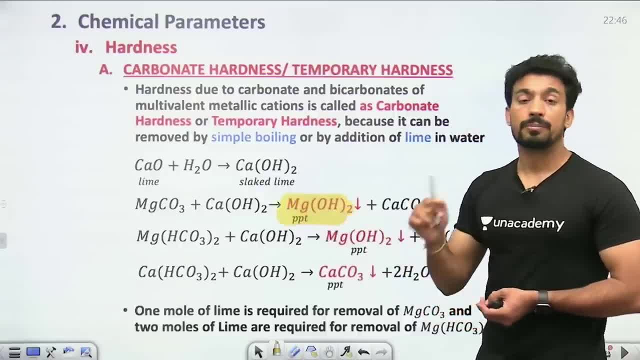 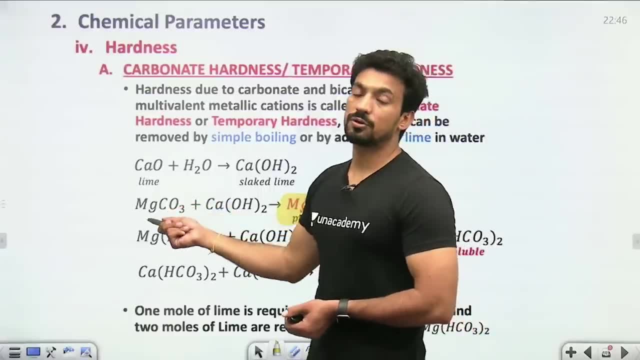 You have to remember that magnesium hydroxide makes the precipitate, Magnesium makes the precipitate of hydroxide, Calcium makes the precipitate of carbonate. If the hardness was present in the form of magnesium carbonate, Then he used only one mole of lime. 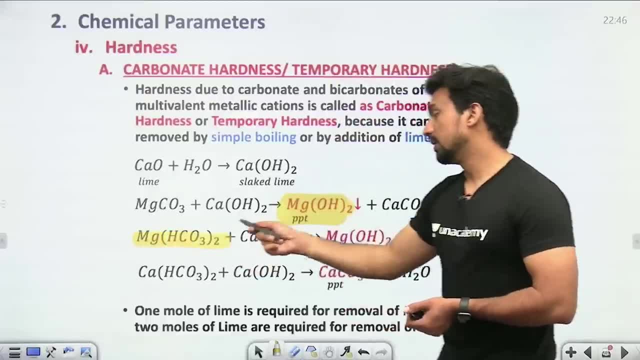 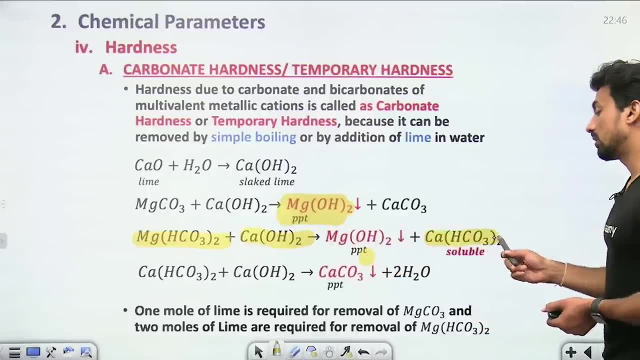 But if the hardness was produced in the form of magnesium bicarbonate, Then he would have used one mole of lime, Which makes the precipitate of MgOH whole twice. At the same time, another compound would form calcium bicarbonate, Which is soluble in water. 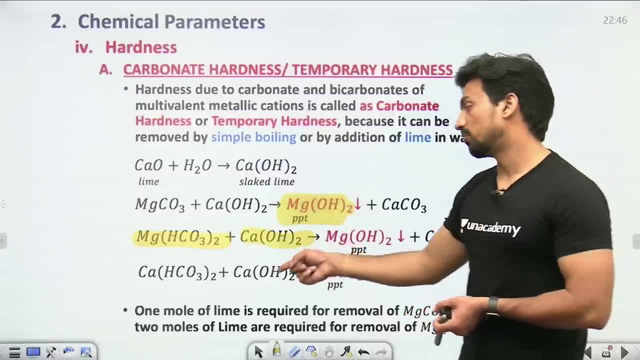 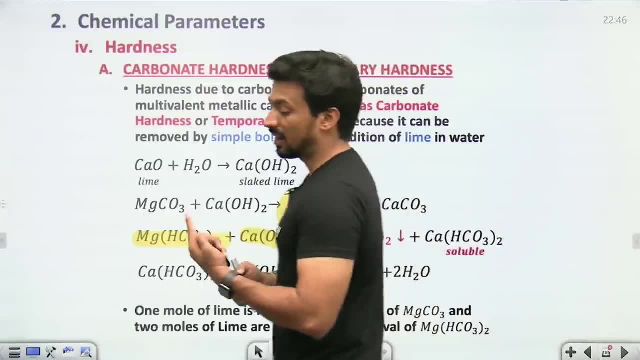 But to remove this you would need another mole of lime, After which it will form calcium carbonate. So remember the statement from the point of view of the objective. If the hardness is present in the form of magnesium carbonate, Then it will utilize one mole of lime. 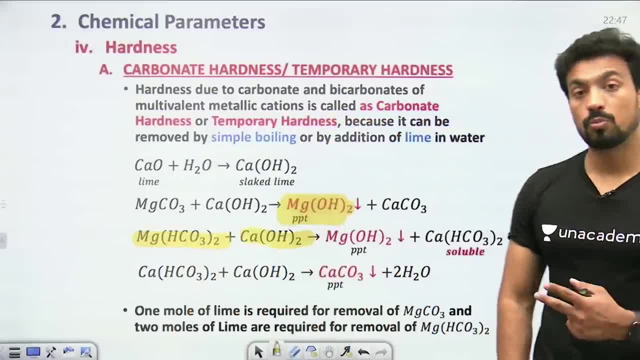 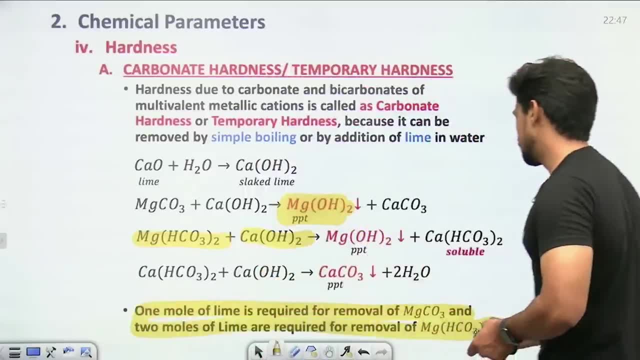 If it is present in the form of magnesium bicarbonate, Then it will use two moles of lime. This is in the objective, But if the hardness is present in the form of lime, Then it will use one mole of lime. Next, let's go ahead. 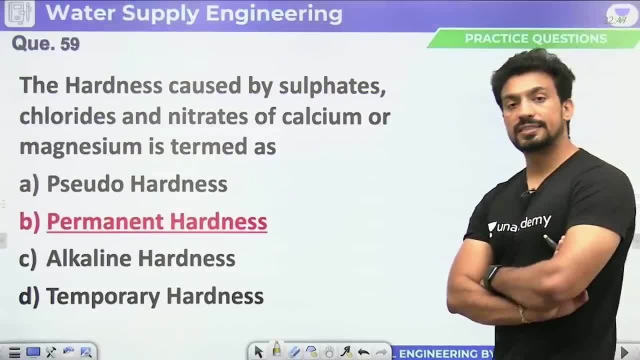 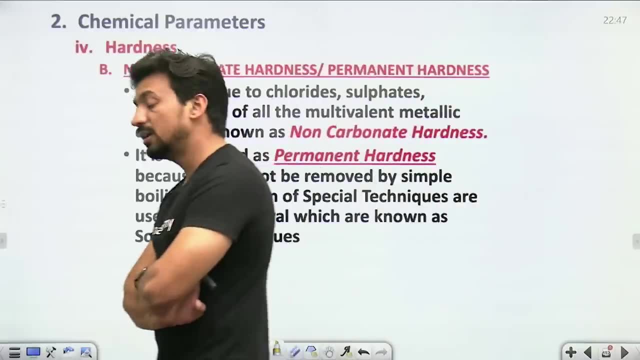 The hardness caused by sulfate chloride nitrate. This is called permanent hardness. Non-carbonate hardness or permanent hardness can't be removed from simple processes. Iron exchange method, zeolite methods or special water softening techniques can be removed from them. 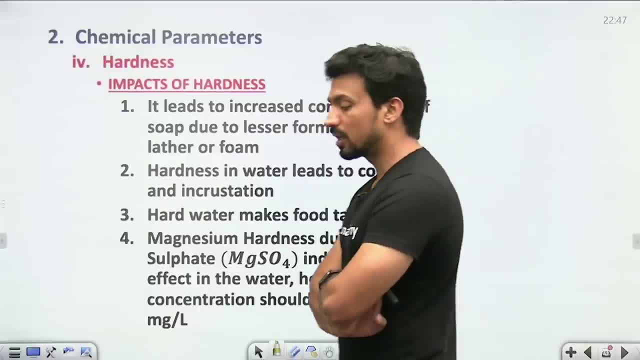 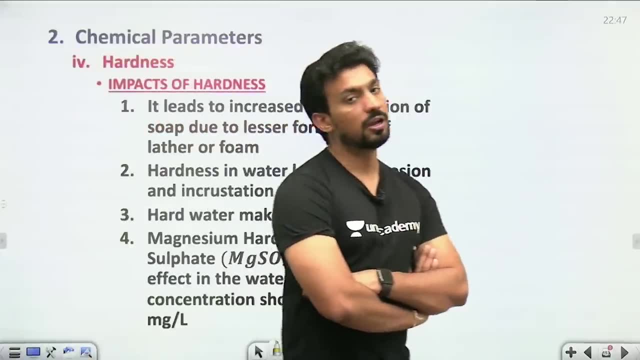 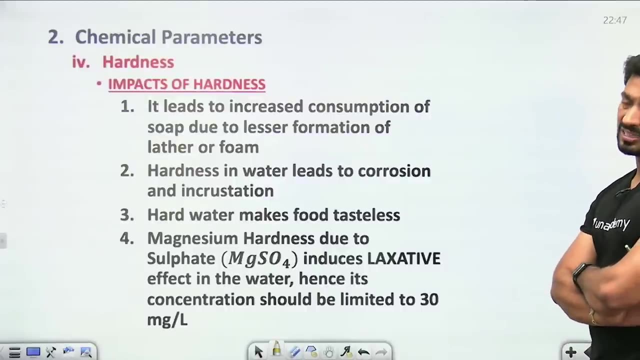 Because of hardness, food becomes tasteless. If you consume hard water then your stomach can get spoiled. Bowlery movements or laxative effect will come in it. Hard water makes food tasteless. Hardness in water leads to corrosion. Corrosion can also happen, Pipe material can be damaged and it can also be accumulated. 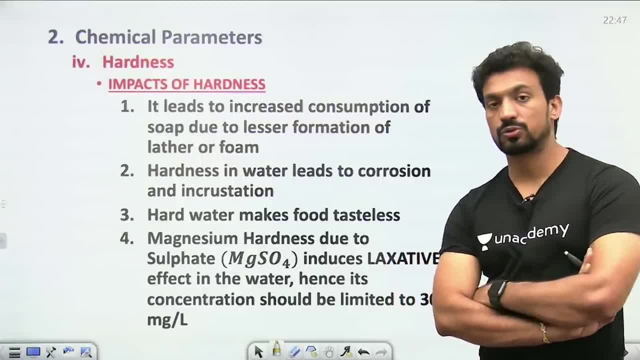 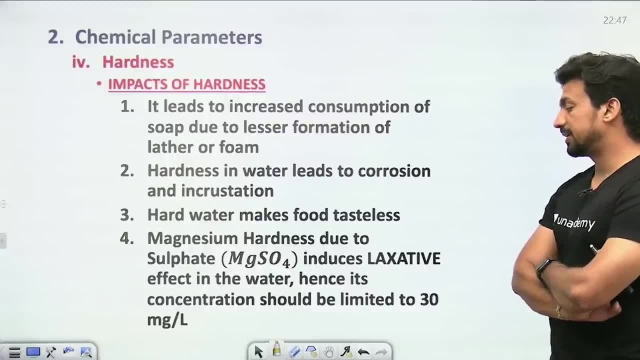 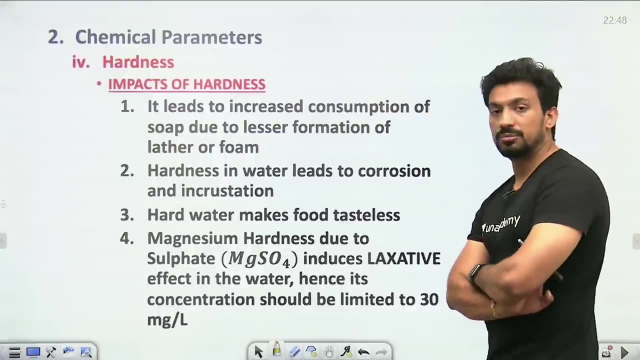 Incrustation can also happen. Material will begin to accumulate, which will reduce the net cross section area of the pipe. Magnesium hardness due to magnesium sulfate indicates or induces laxative effect in the water. Hence its concentration should be limited to 30 mg per liter. 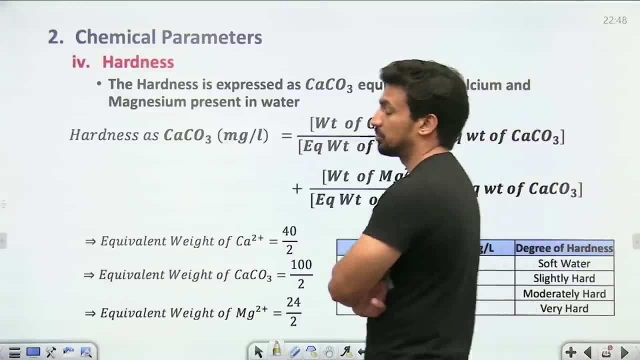 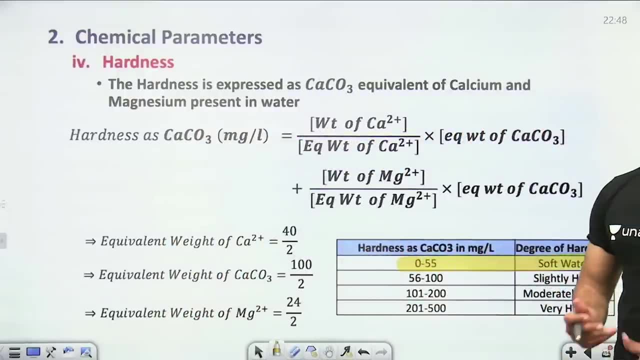 Hardness is also expressed in terms of calcium carbonate. What are the questions in the objective so far? If hardness in the form of calcium carbonate in mg per liter is between 0 to 55, then it is called soft water. If it is between 56 to 100, then it is slightly hard. If it is between 100 and 1 to 200, then it is called moderately. 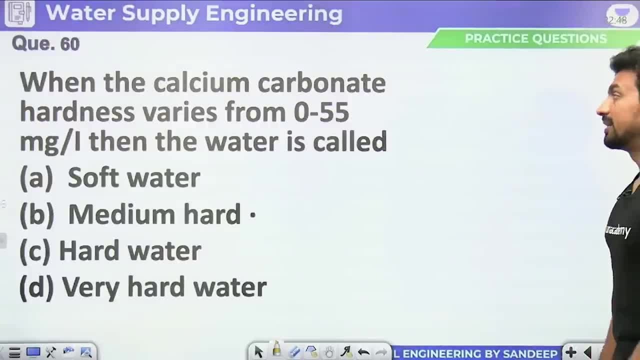 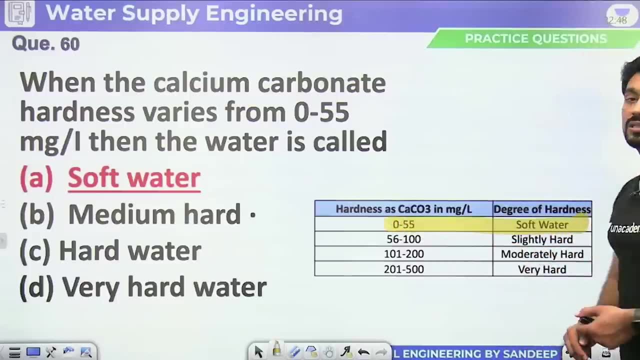 If it is between 500, then it is called very hard water. When the calcium carbonate is in the form of calcium carbonate, then it is called soft water. Calcium carbonate hardness varies from 0 to 55. So in the case of 0 to 55, we will call it soft water. 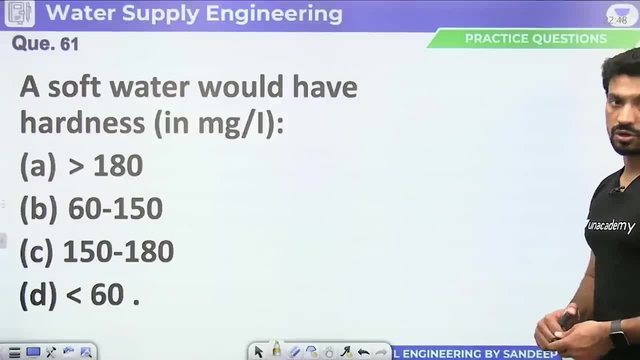 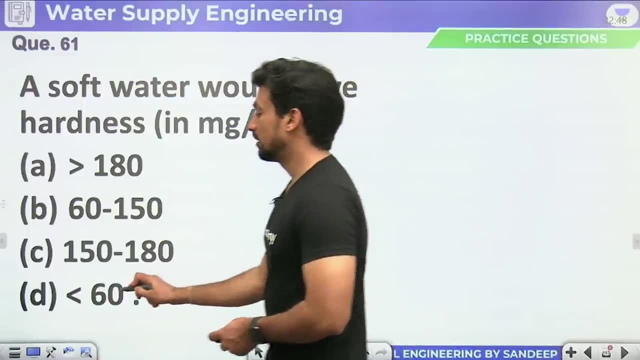 A soft water would have hardness. The hardness of soft water should be between 0 to 55 or less than 55.. We have not been given the 55 option in the options. We have given the 60 option, so we will choose it. 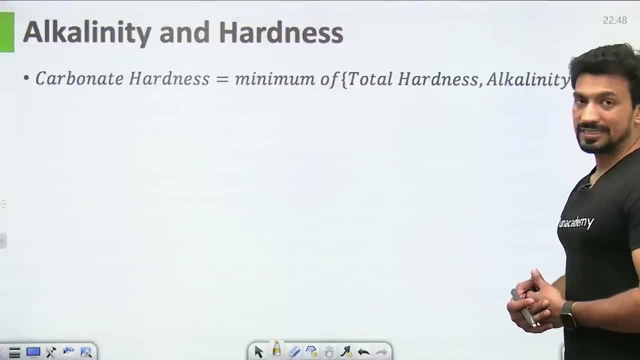 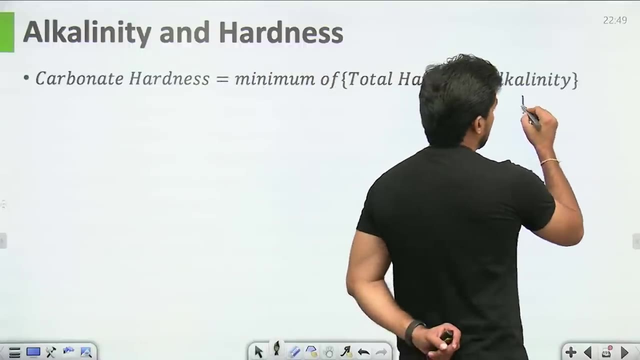 Less than 60. If you want to know the carbonate hardness, then how can we tell the carbonate hardness? That would be the minimum of total hardness, or alkalinity. Now, if you understand a little less in this, then you pay attention. What is alkalinity? 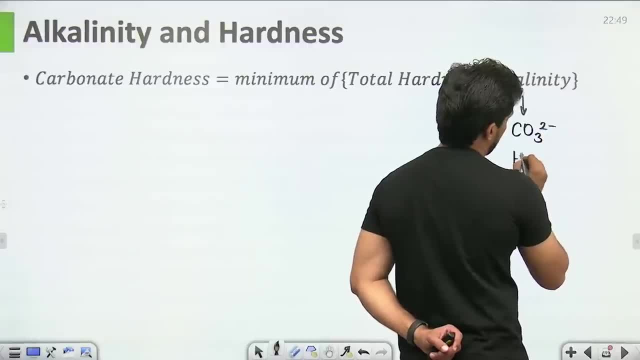 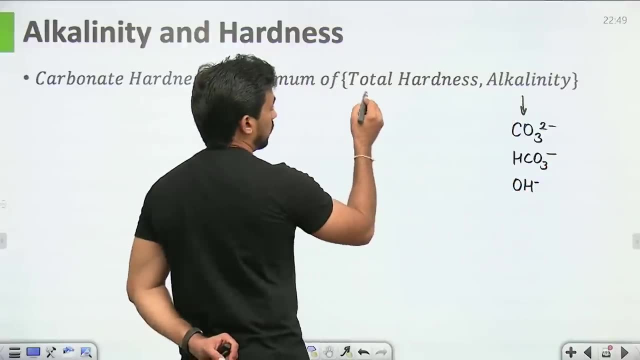 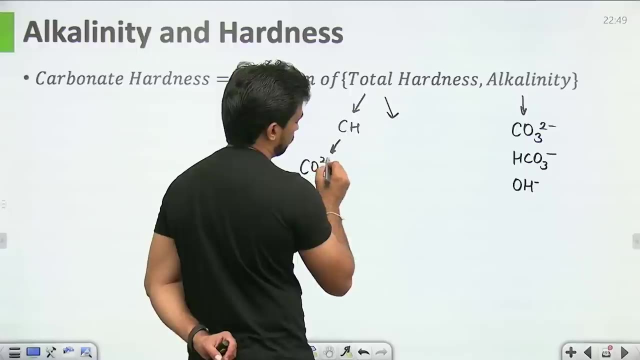 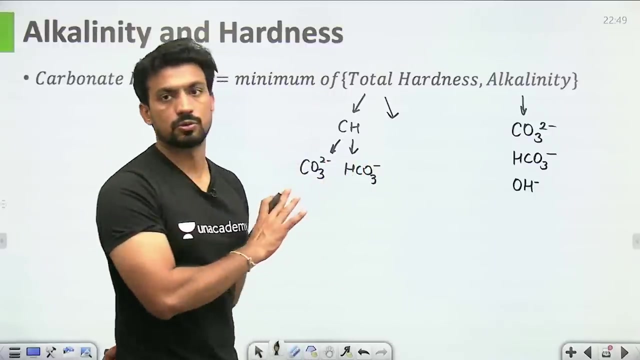 Alkalinity is due to carbonate, bicarbonate and OH-. If we talk about hardness, then we have two types of hardness. One is carbonate hardness, which would be due to carbonates And bicarbonates. Obviously, these will only be found with magnesium or calcium. 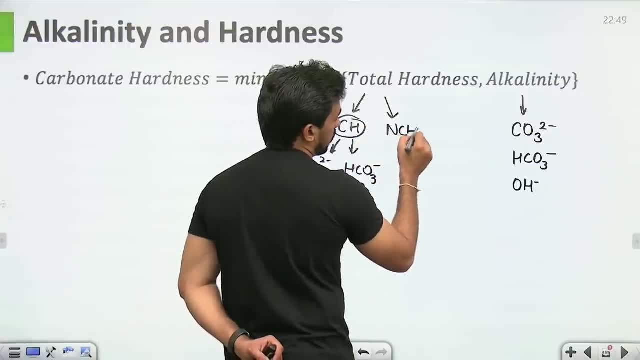 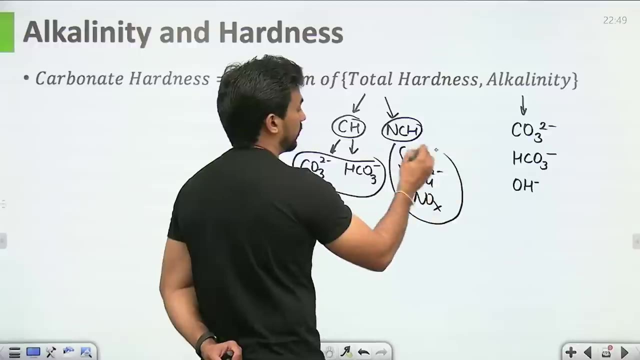 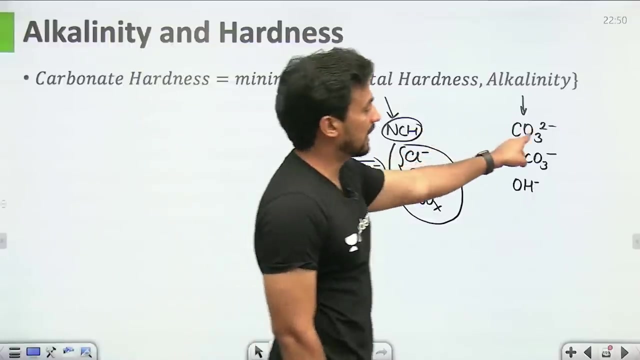 After carbonate hardness, the noncarbonate hardness is due to chloride, sulfates or nitrates. So this hardness is called permanent. This one is temporary. So now if we have to tell the carbonate hardness, Carbonate hardness is due to carbonate bicarbonate and alkalinity. 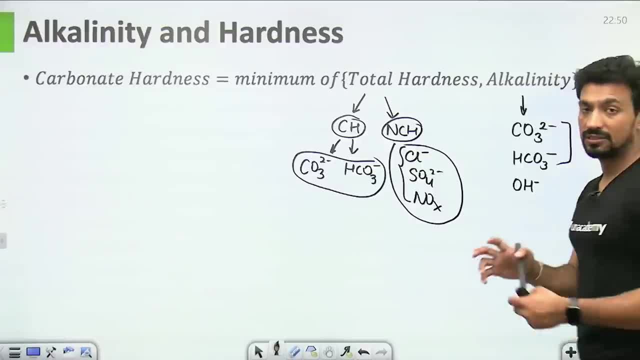 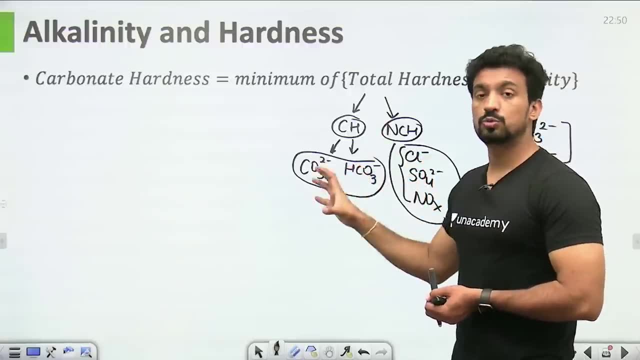 So these two are common. Now, in some water, carbonate is also present, bicarbonate is also present, chloride is also present, sulfate is also present. All these are present. So if you want to tell in that, what is the carbonate hardness? 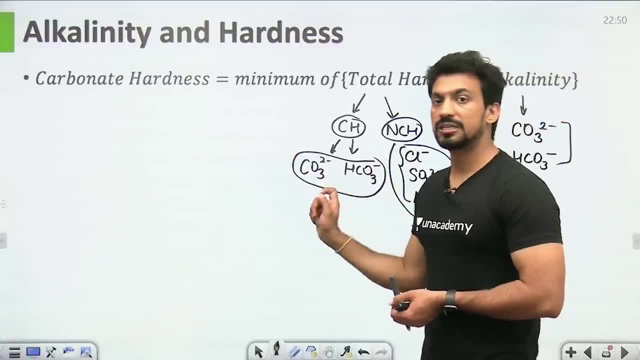 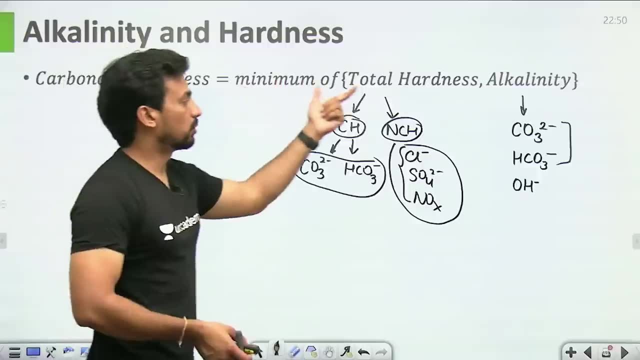 What is the noncarbonate hardness? If you want to determine this, then what will you say? You will take the minimum, That carbonate hardness will be minimum of total hardness And alkalinity will be minimum of total hardness. Why did you choose minimum? 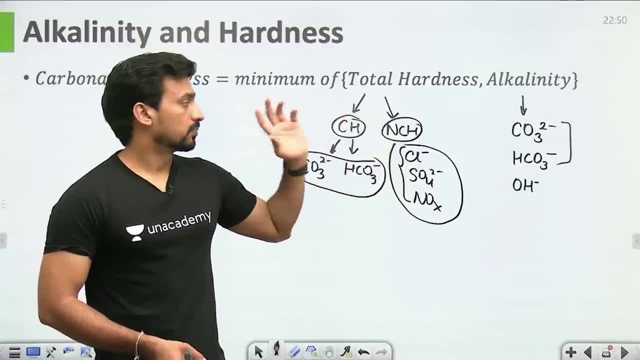 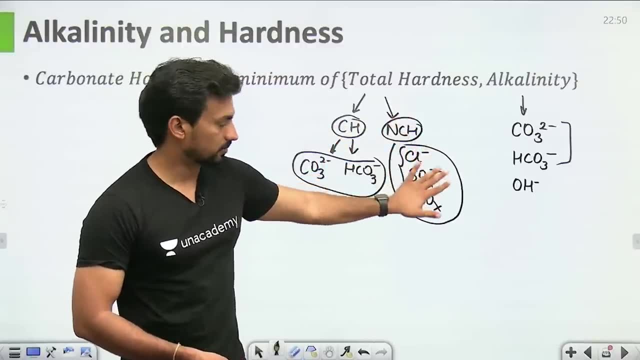 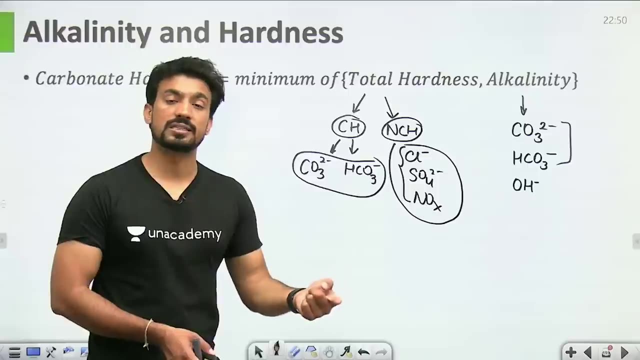 Because if it happens that in some water carbonate is present, bicarbonate is present And there is no permanent hardness in it, These terms are not there. If these terms are not there, then still its total hardness value is less and alkalinity is more. 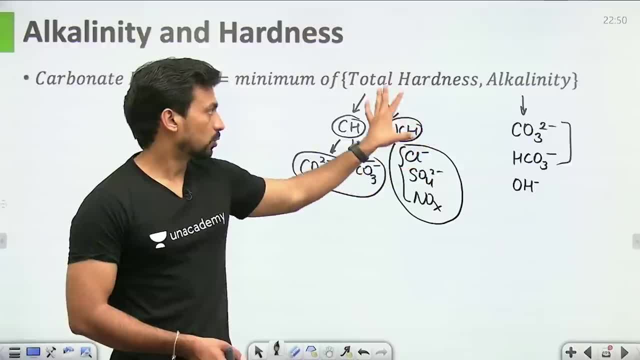 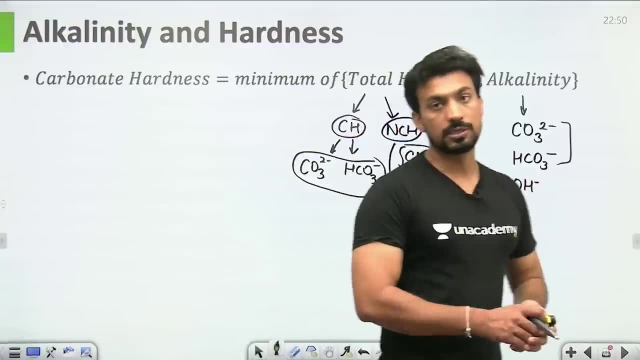 So this means that if this does not happen, alkalinity is more than total hardness. That means there is carbonate in it, bicarbonate is present and OH- is present. That is why, in total hardness, these two terms were also present. These two terms were also present in alkalinity. 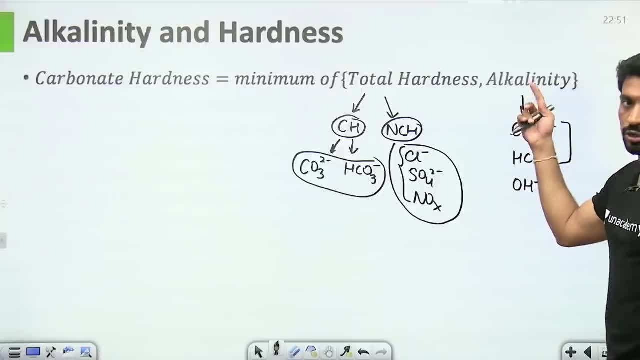 So OH- was more, due to which alkalinity was more. So we said that how to recognize carbonate hardness? So we said, take the minimum of these two, Total and alkalinity, So that we can tell that, yes, what is the hardness? due to carbonates. 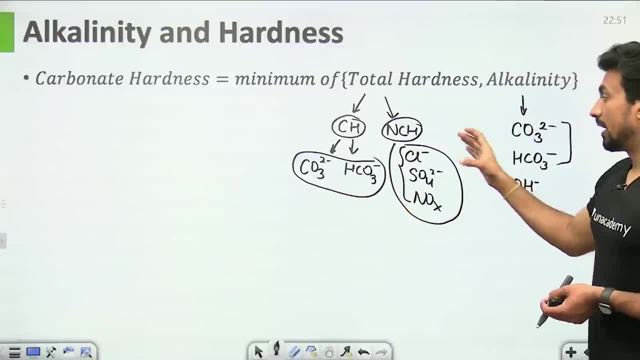 Noncarbonate will obviously become zero. in that case, If these are also existing, these are also existing. So in that case we will say that what will be the minimum of total hardness, or alkalinity? It will become alkalinity. So we will put carbonate hardness equal to alkalinity. 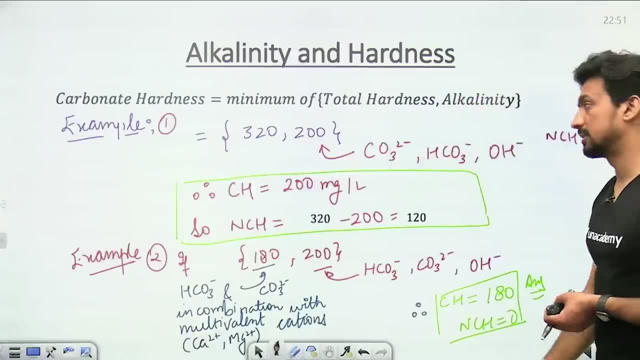 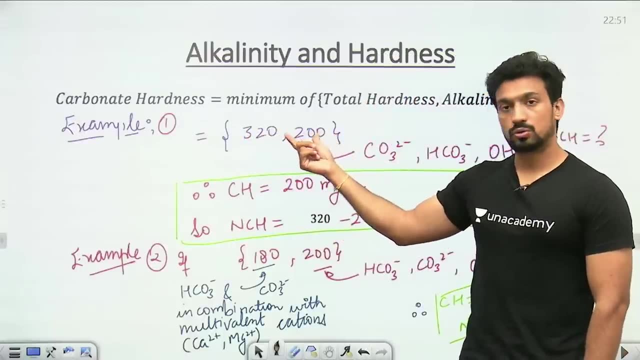 And then we will subtract it from the total. then noncarbonate will come As an example, if total hardness is given to you as 320 and alkalinity 200. So why would 200 come? Due to carbonate, bicarbonate and OH- 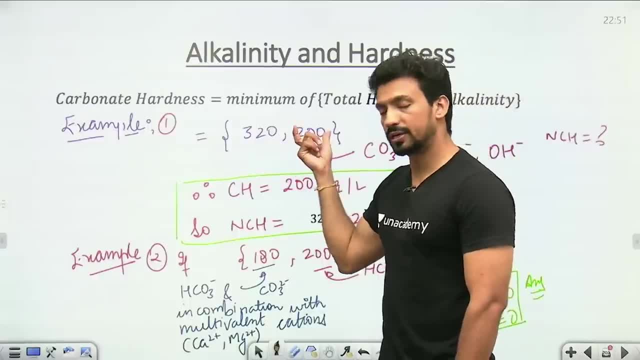 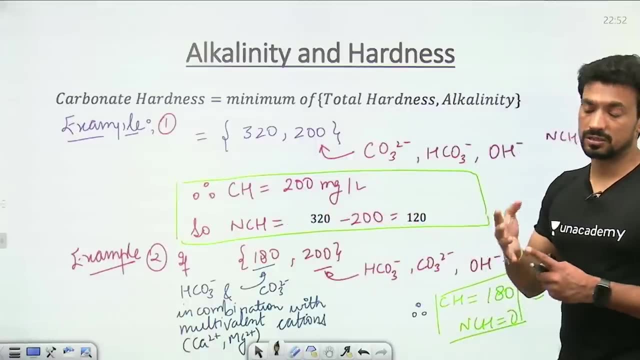 So you said that carbonate hardness will come 200. Minimum of these two. So what will be the remaining 120? Noncarbonate hardness. Because of what? Because of carbonates, sorry. because of chloride, because of sulfate, because of nitrates. 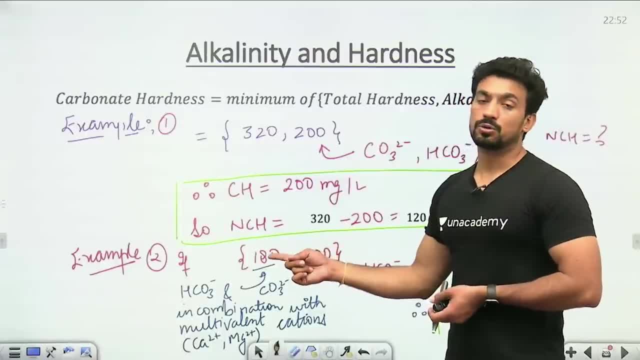 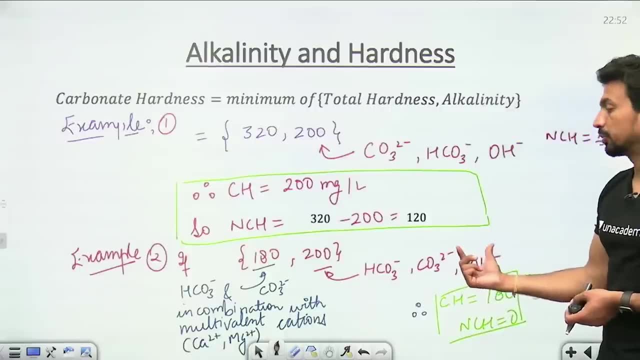 If 180 and 200 were given, it means that total hardness is 180.. How did alkalinity 200 come? Alkalinity came because OH- was also there, So these two came to you. The minimum of these two is carbonate hardness. 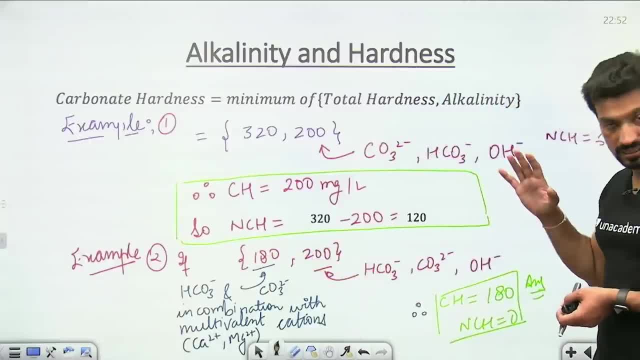 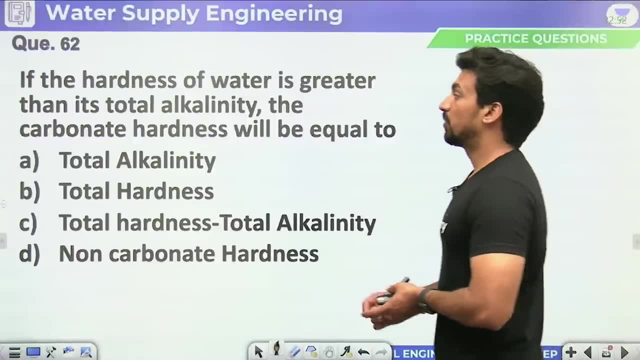 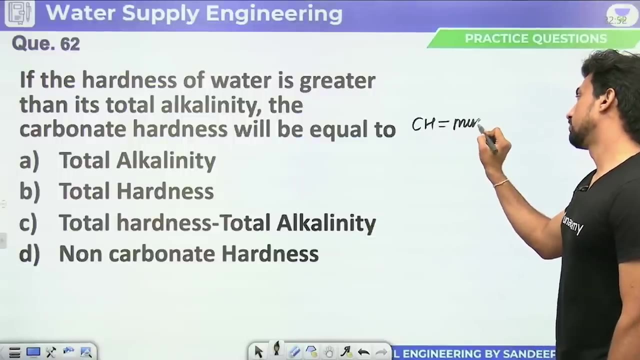 Carbonate hardness is 180.. If the total hardness is 0. We will subtract carbonate, So noncarbonate will become 0.. If the hardness of water is greater than its total alkalinity, We say that carbonate hardness is minimum of total hardness and alkalinity. 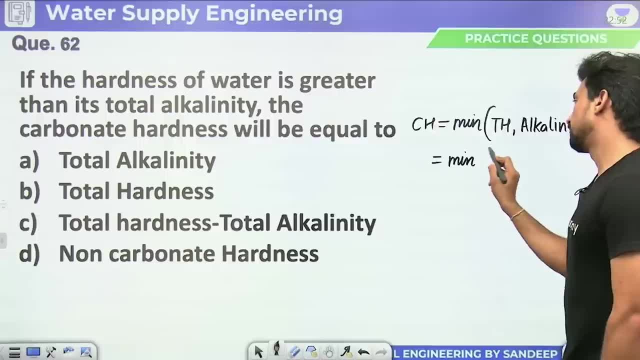 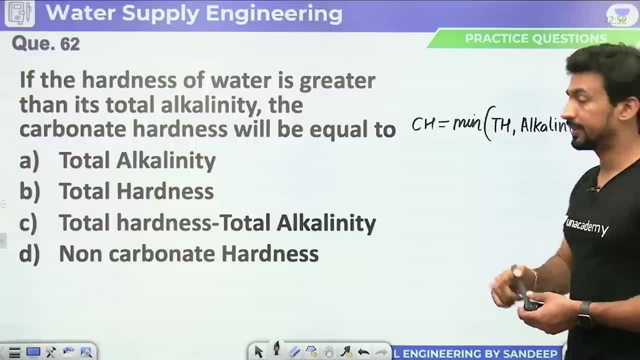 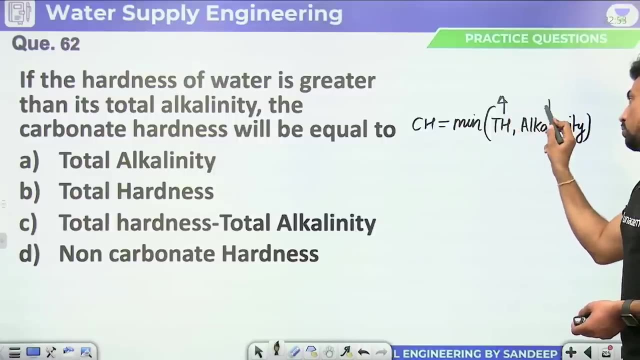 So it is minimum of total hardness. If it gave you the statement in the objective, If the hardness of water is greater than its total alkalinity, If hardness of water is greater than its alkalinity. So if this value is high, If this value is small, 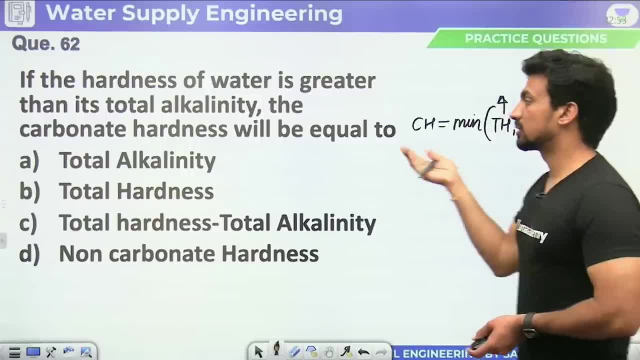 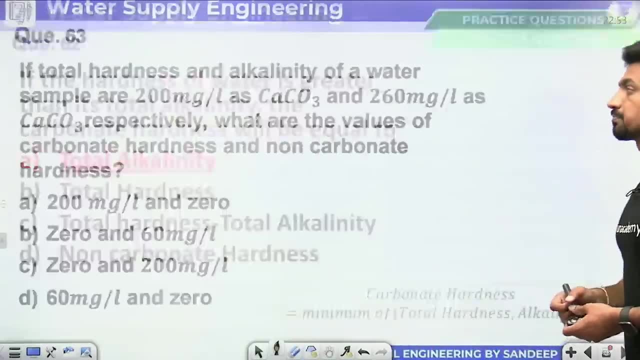 So the minimum alkalinity will come from these two. So what will be our answer? Carbonate hardness will be equal to total alkalinity. The answer will come option A Next, If the total hardness and alkalinity of water sample are 200 and 260. 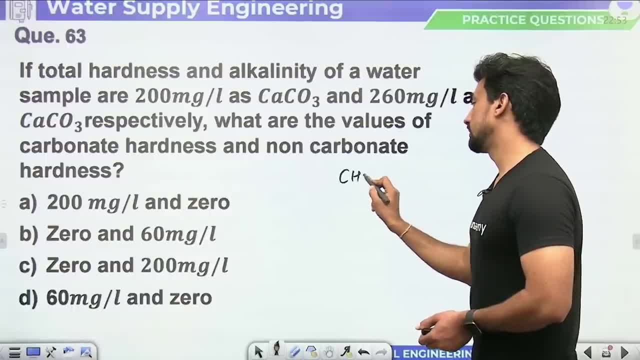 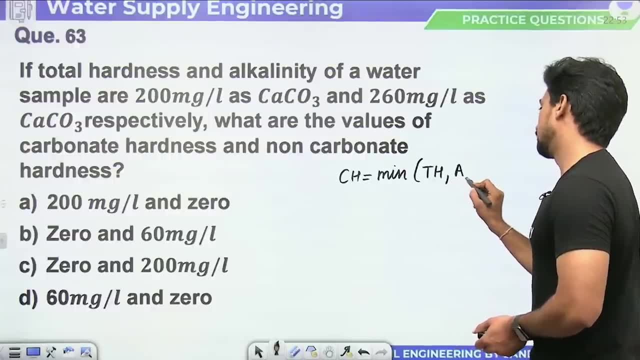 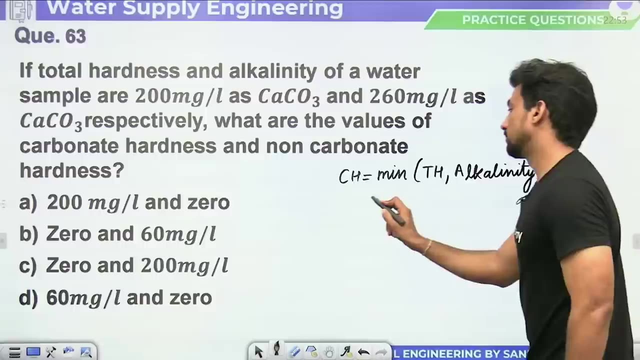 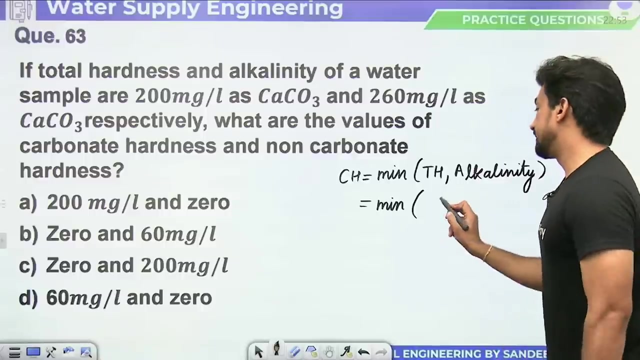 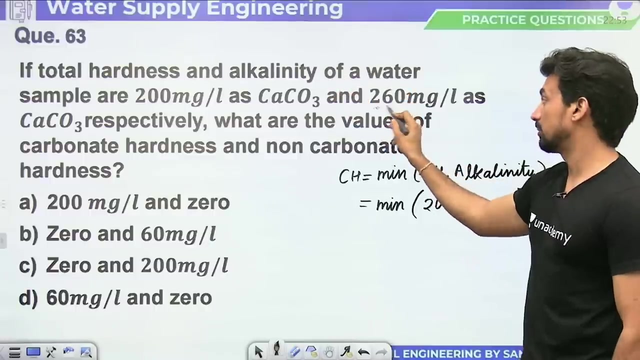 So you have to use the same formula again, that carbonate hardness is equal to minimum of total hardness and alkalinity. so it will be minimum of. if the total hardness and alkalinity is written first, then total hardness is written, then alkalinity is written after that, then 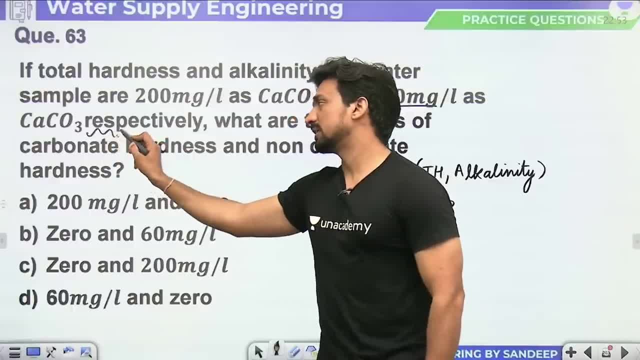 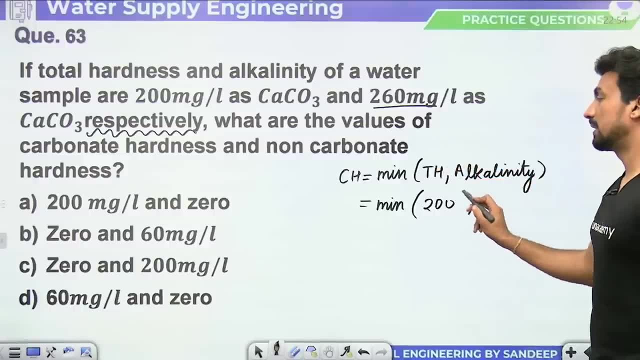 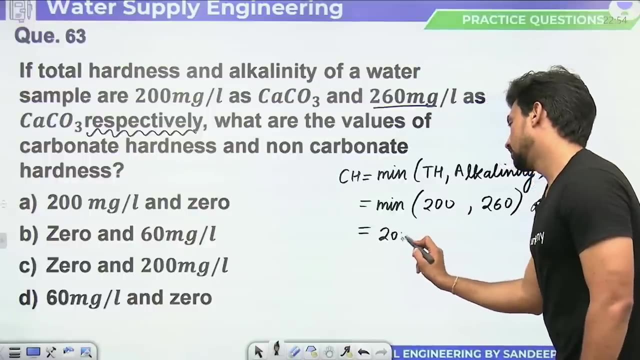 it means alkalinity is told that whenever the word is visible respectively, then read the question carefully or choose the answers carefully. then first the total hardness is written, then 200, alkalinity is written later and respectively word is written, then 260 means that carbonate hardness has come to you 200 milligrams per liter. we know that. 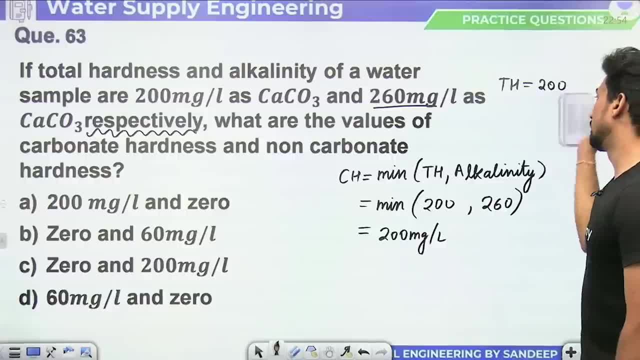 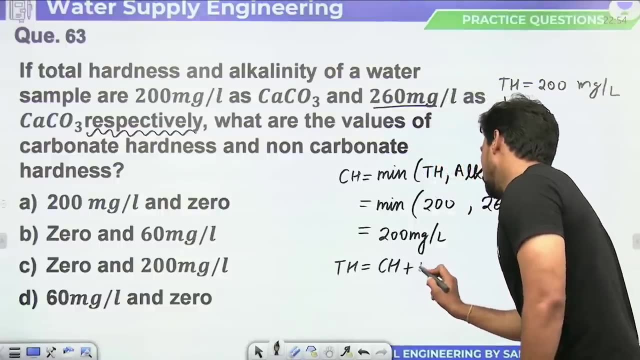 total hardness is also 200. This means that the total is due to carbonate plus non-carbonate. so you will say that total hardness is equal to carbonate and non-carbonate, of which this is also 200, this is also 200,. 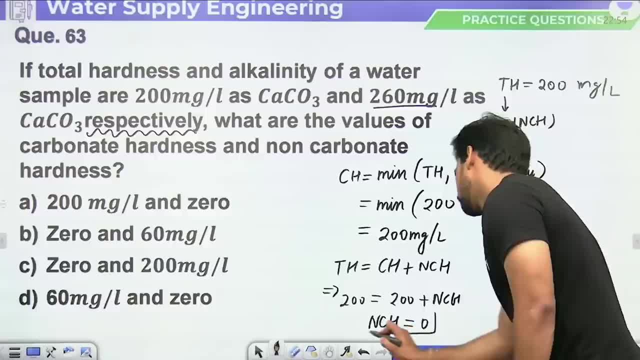 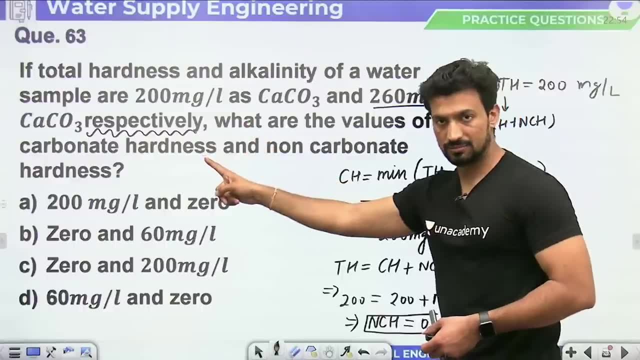 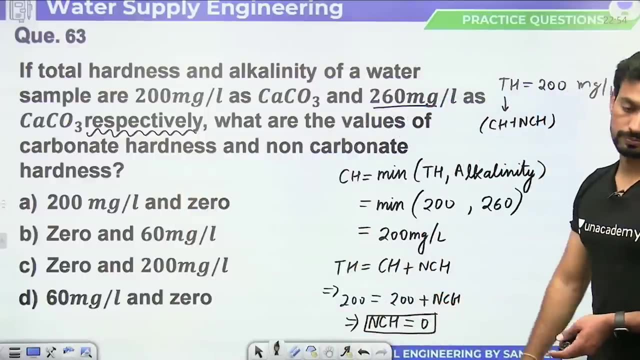 then how much is non-carbonate hardness? Now read the statement of the question carefully. He asked us: what are the values? of carbonate hardness first said non-carbonate hardness said later, then what is written first. then our 200 came, then 0. now this question: how? 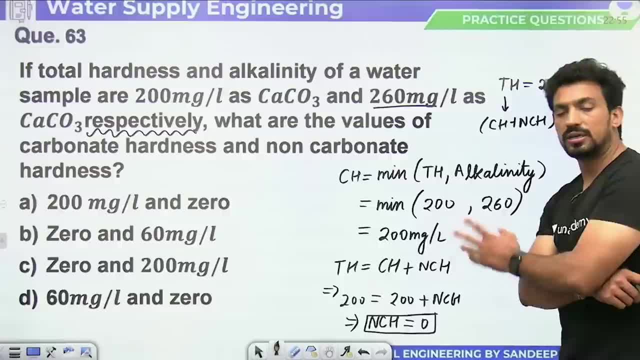 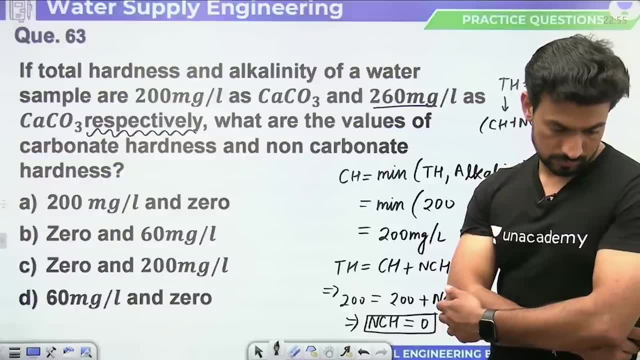 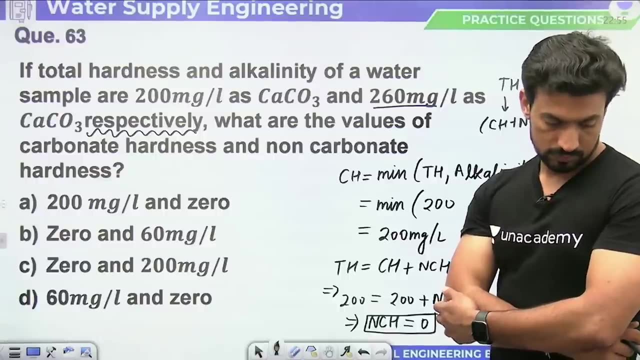 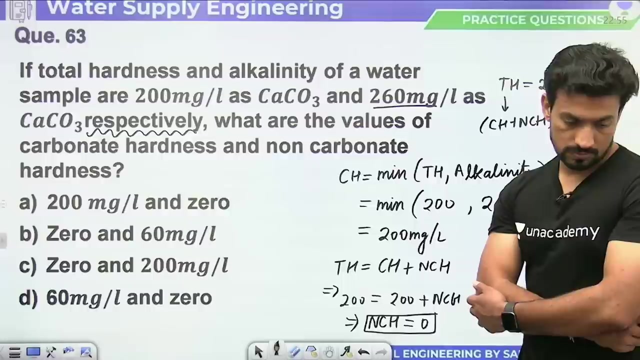 will the sir do it quickly, so quickly. I will do it like this. I wrote the whole formula, wrote values. you could have told directly. you could have done this orally by looking at the question. Sir. question Friends. I don't know what happened. so what can I say about support right now? 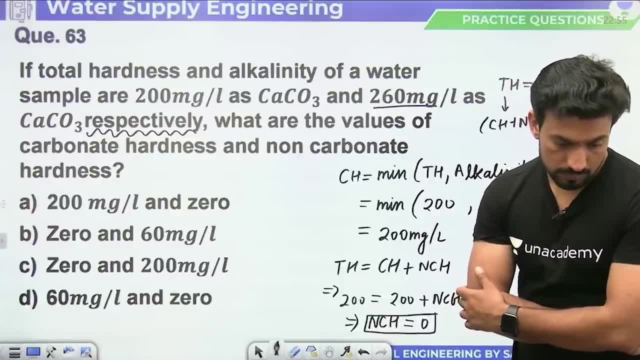 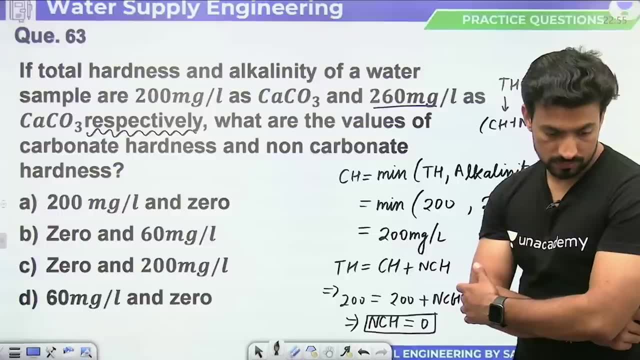 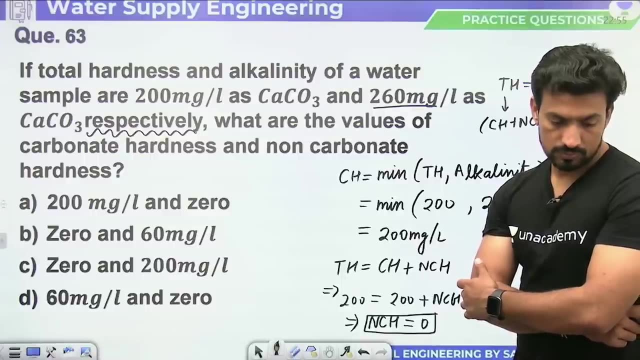 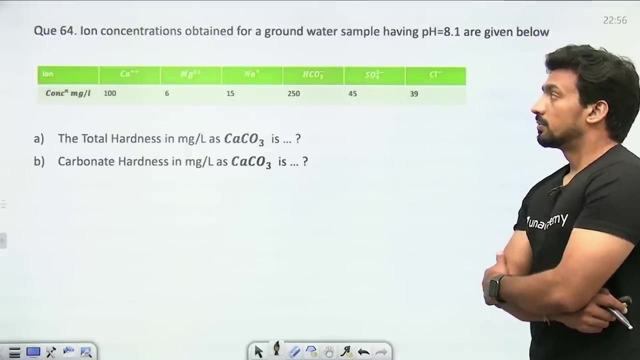 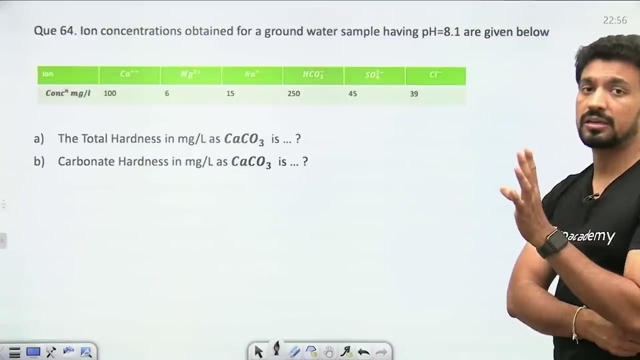 Complete it, sir, absolutely sir. why won't you do it if you have told me to? Did you understand? Next, We have given you iron concentrations. we have to tell you the total hardness in the form of calcium carbonate. so keep that thing in your mind. the basic one. 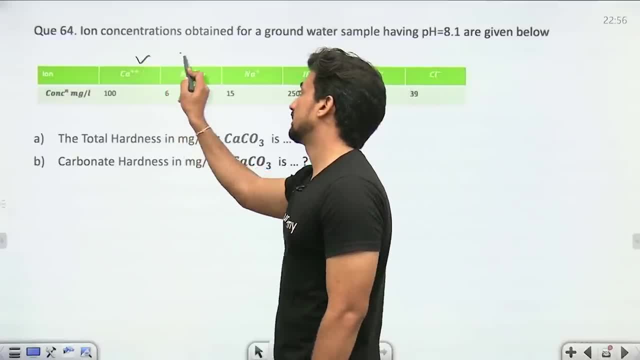 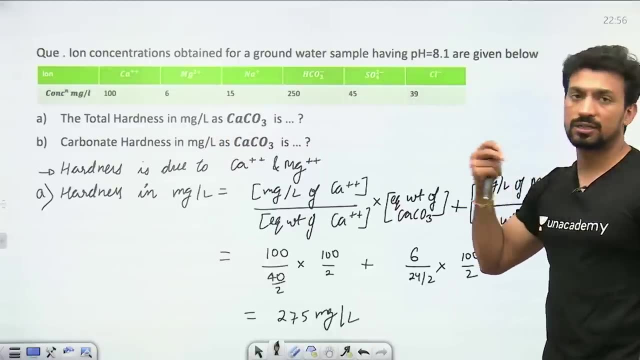 What components will be responsible for total hardness. Calcium and magnesium are the most according to these two. we will tell you here. We have to consider this. if you want to tell you the carbonate hardness, then the total will come. the alkalinity will come according to that. we will tell you both carbonate and non-carbonate. 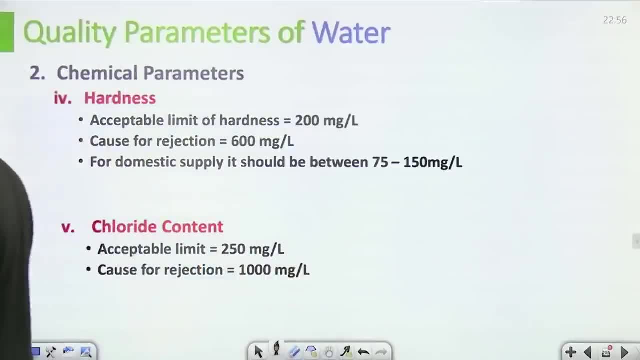 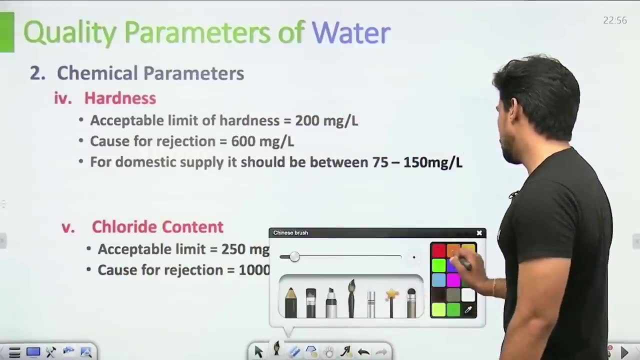 So we don't need to give much time here because we have already done these questions. If we talk about hardness, then what will be the questions directly from the objective? The table you saw of IS code. see from that also. if you want, then you can see from here. 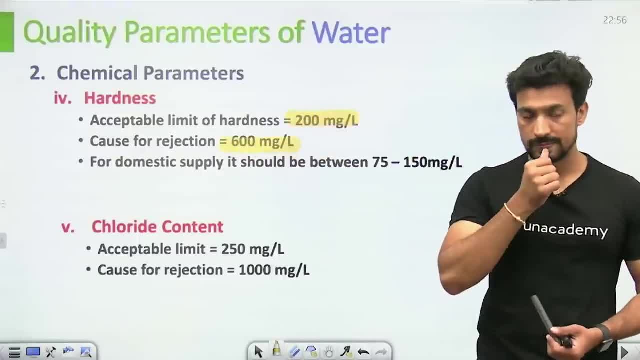 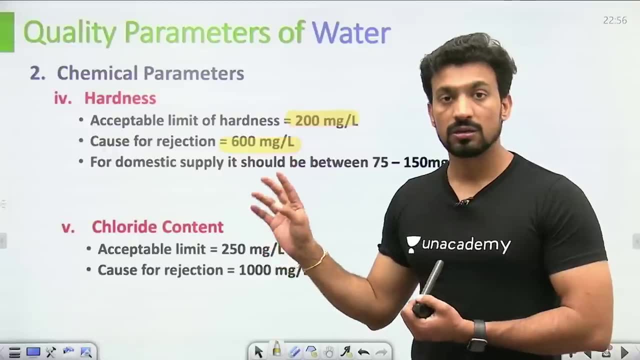 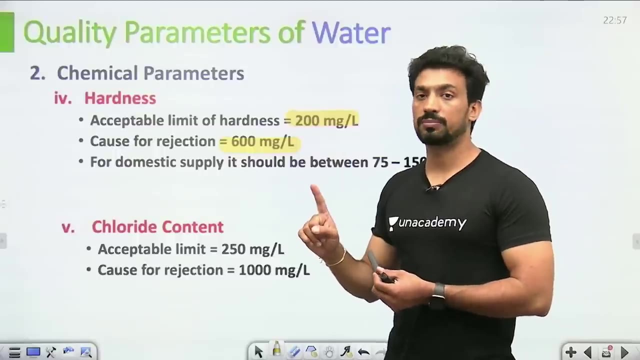 200 mg per litre acceptable limit. If there is no alternate source of water available, then in that case we will tolerate up to 600.. But if it is more than 600, then we will not even treat it. If the alternate source is not available, there is only one source of water in your city or village, then you can go up to here. 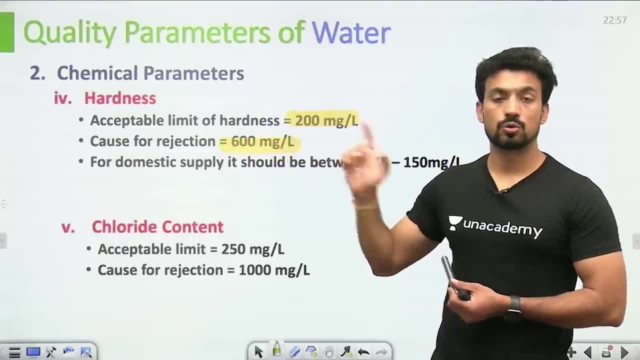 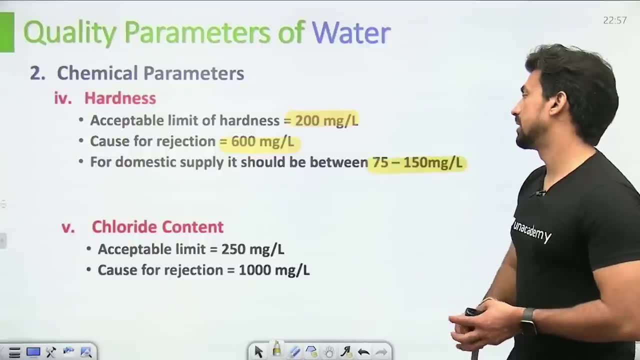 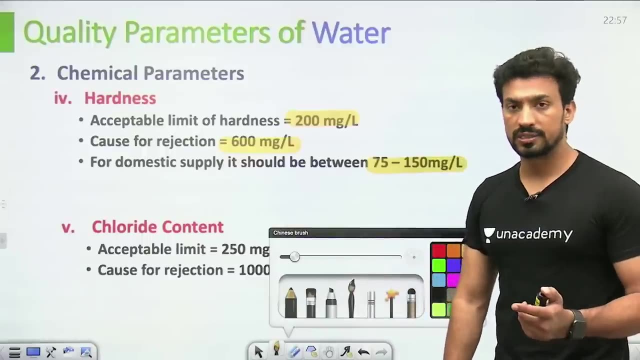 Then we will treat the water. but if it is more than this, then we will not use that water. if it has more hardness than this, For domestic water supply it should be between 75 to 150 mg per litre. If we talk about chloride content, then chloride content. now again the question comes: how much? according to WHO? 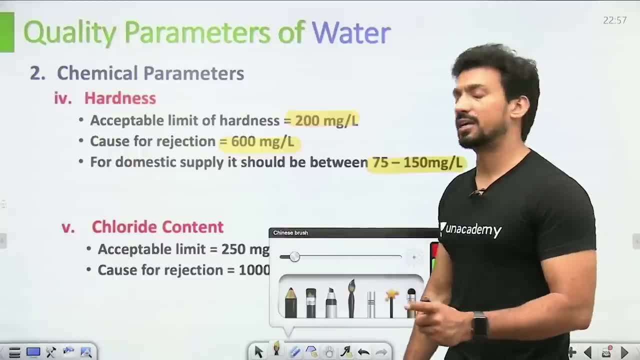 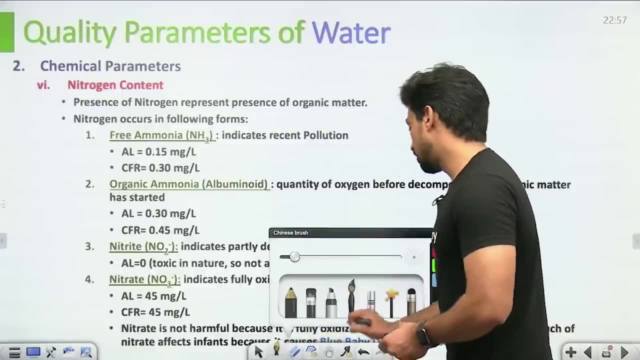 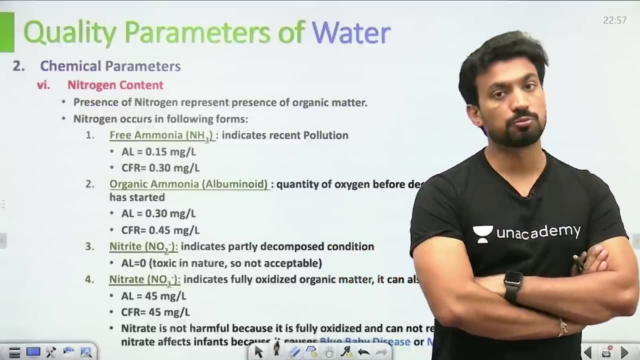 According to WHO it is 200.. But what we have to remember? we have to remember the Indian standard: 250 mg per litre. cause for rejection: 1000 mg per litre. Then, after that, comes the nitrogen content. Nitrogen content tells you that if a waste water is added in clean water and it is polluted, then first of all ammonia will be present in it. free ammonia will be present in the form of NH3.. 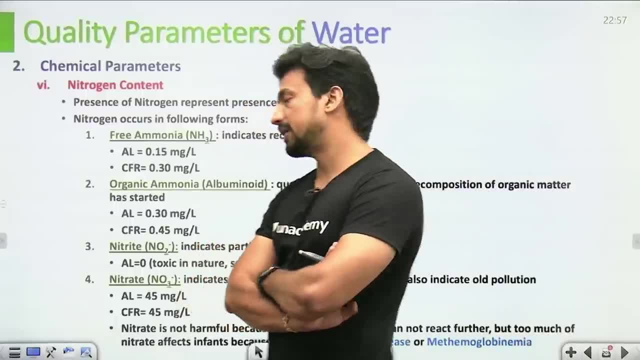 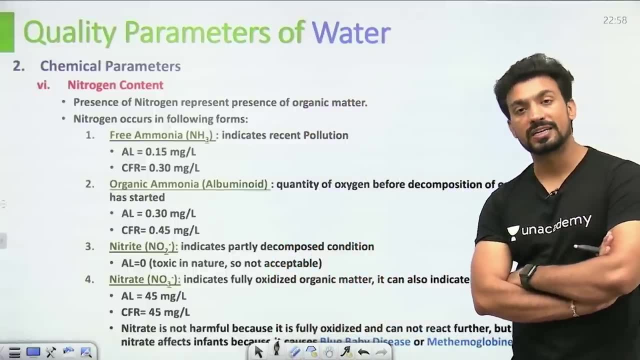 And its limit is 0.15 mg per litre. cause for rejection is 0.3 mg per litre. If free ammonia is present in some water, then it indicates that recent pollution- some waste water has just been added in fresh water, due to which it is polluted. 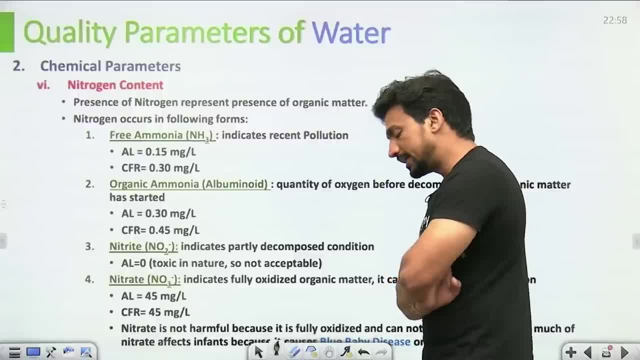 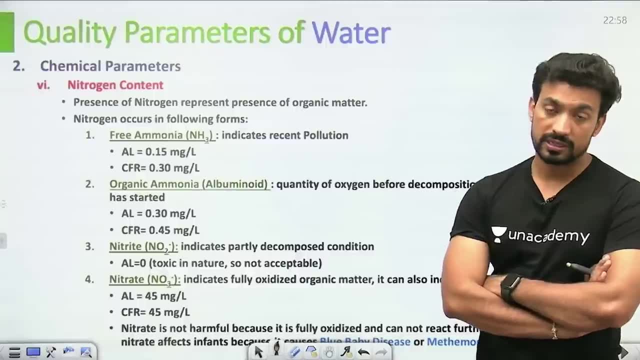 So it tells organic waste. Then its decomposition will start. Now the obvious thing is that dirty water has been found in clean water. so the oxygen in the clean water will start decomposing that dirty water. So organic ammonia will form, albuminoid will form. 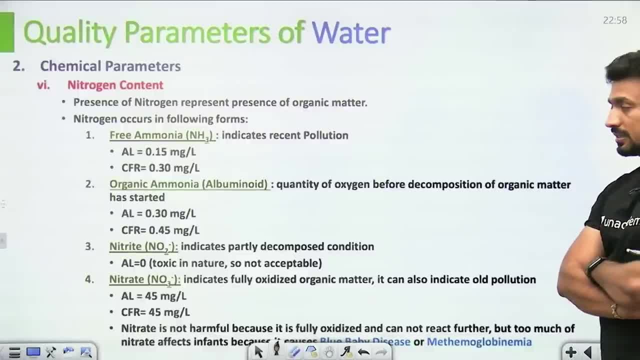 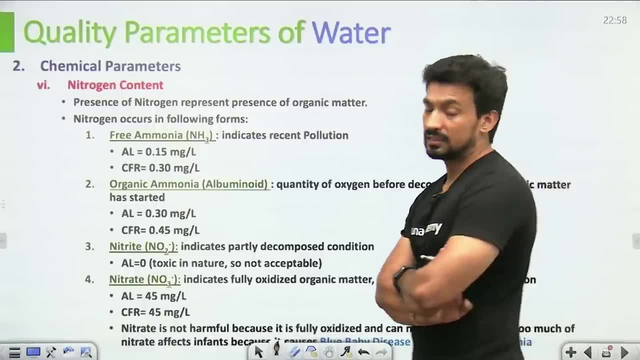 So quantity of oxygen: before decomposition of organic matter has started, Its acceptable limit is 0.3 mg per litre. cause for rejection is 0.5 mg per litre. Then after that comes partly decomposed matter, which is called nitrite. 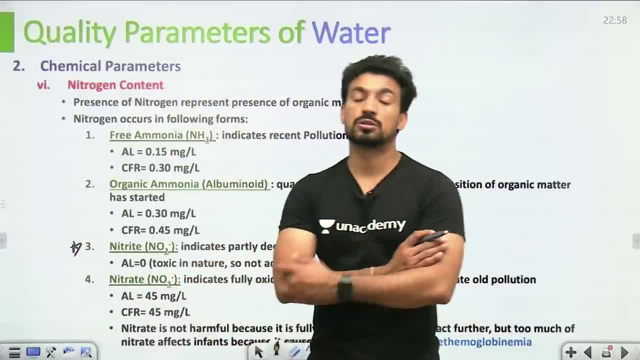 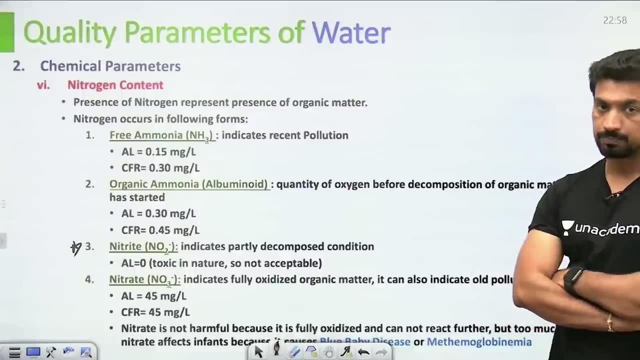 Nitrite is its acceptable limit. Its acceptable limit is 0.. It is toxic. Partly decomposed matter, Half incomplete decomposed matter. It is toxic. It is not acceptable. Then after that comes nitrate- Nitrate NO3-. 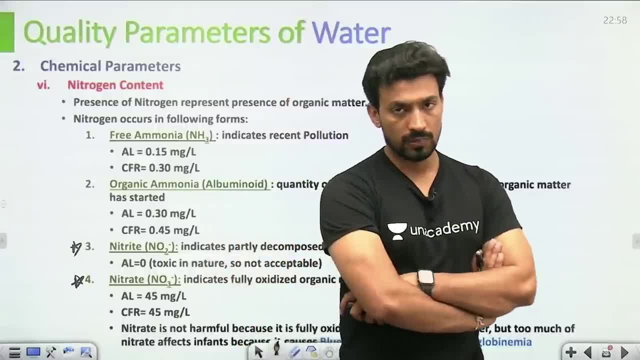 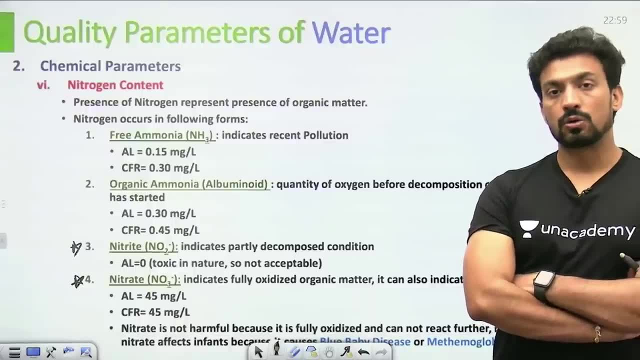 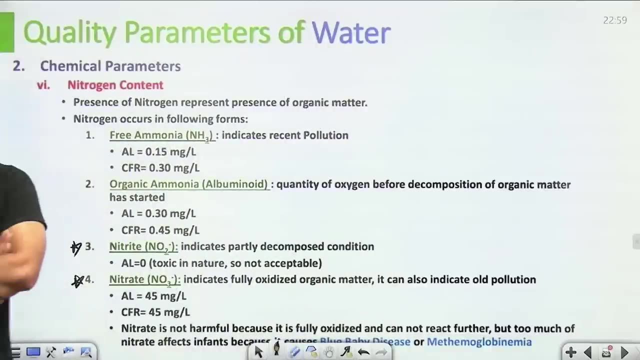 Its acceptable limit and cause for rejection is 45.. Children, infants, newborn babies do not have so much acidic medium present in their stomach, due to which they cannot properly handle nitrate. It affects them, harms them, due to which they look lethargic. 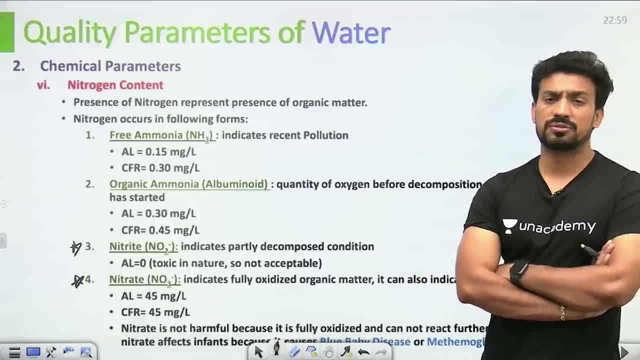 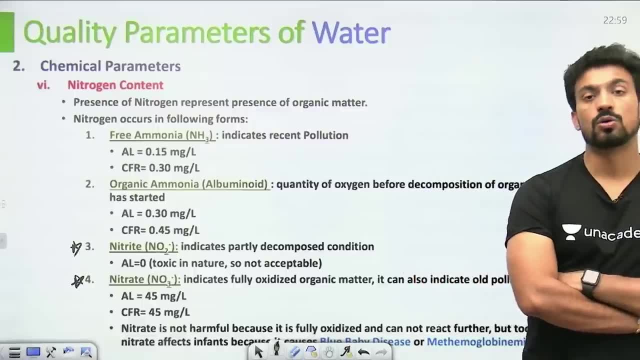 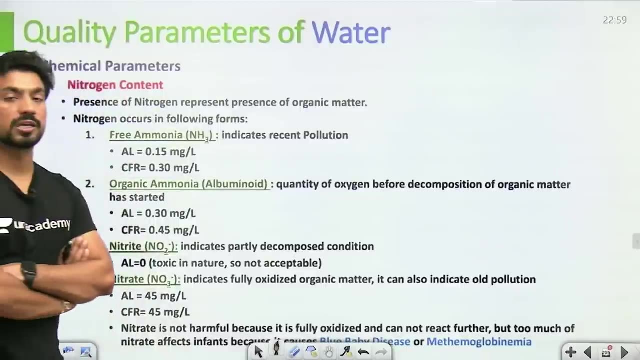 Their skin color becomes pale. A little bluish tint starts coming. That is why it is called Methemoglobinemia. This disease is called Methemoglobinemia And it is known as Blue Baby Disease. If you look at the baby it will look like he is so much worried, like he is born with BTEC. 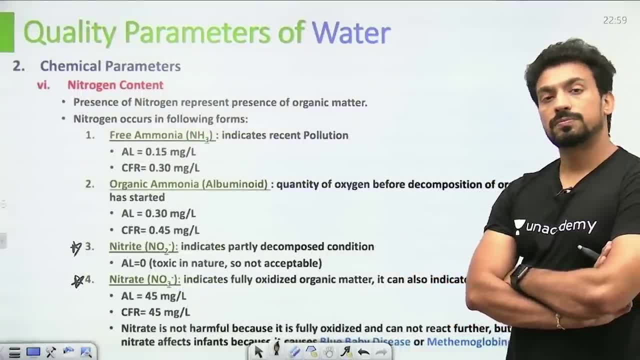 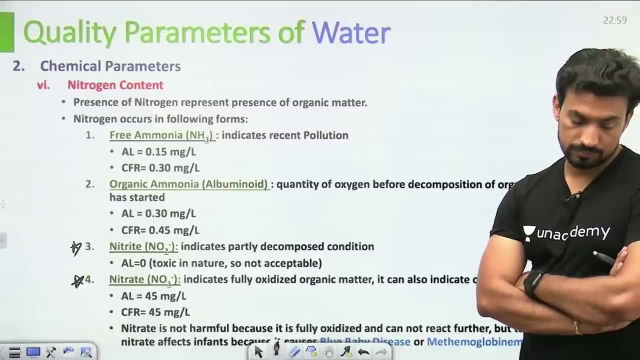 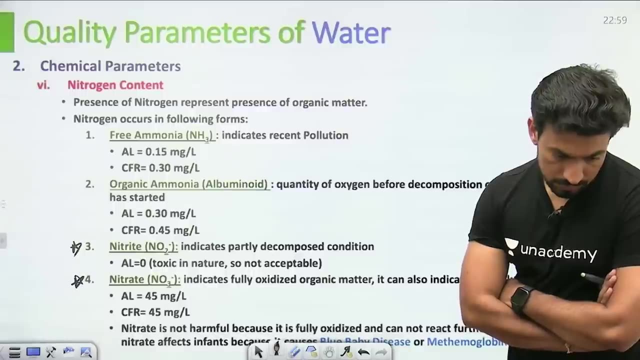 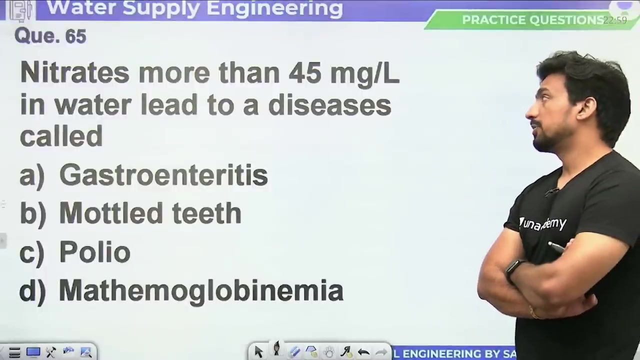 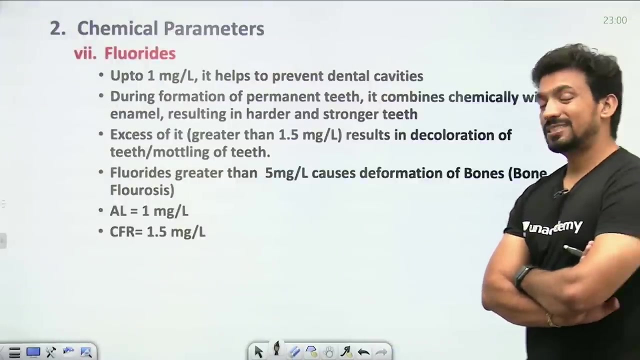 So it looks lethargic, tired and the skin tone becomes blueish. Methemoglobinemia Nitrates- more than 45 mg per litre in water lead to a disease called as Methemoglobinemia. If we talk about fluorides, you must have seen in the advertisement that this toothpaste also contains fluoride other than salt. 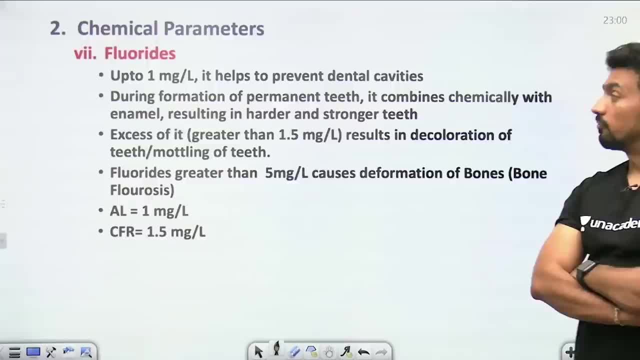 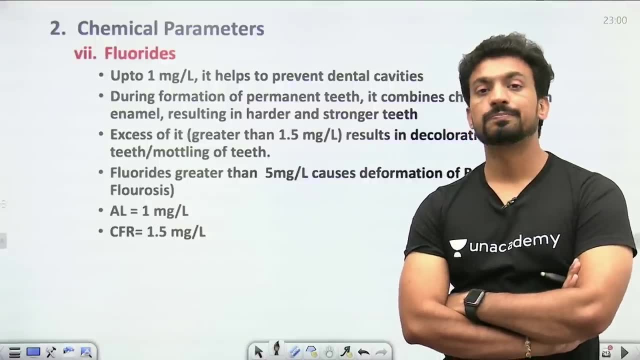 Okay, Why salt? I don't know what they are trying to say. in salt, What does fluoride do? 1 mg per litre of concentration? Now, if you look at the concentration in toothpaste, sometimes, if it is free, the phone is switched off, it is not being charged for some reason. 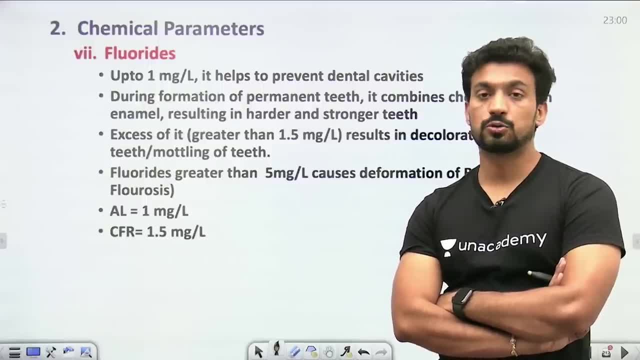 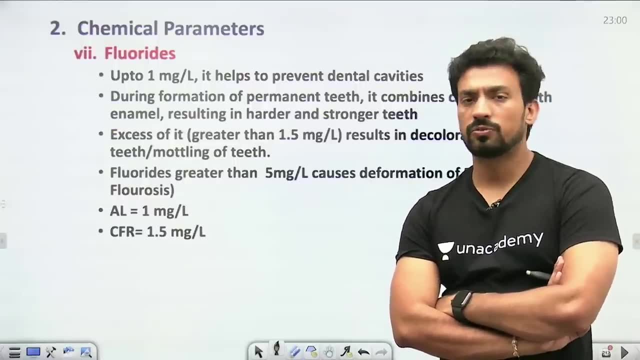 They are getting bored. One day the phone was not taken to the washroom, the toothpaste was seen, so you can see the ingredients of toothpaste. If you look at its composition, you will see fluoride in it, But the composition of fluoride will be seen. 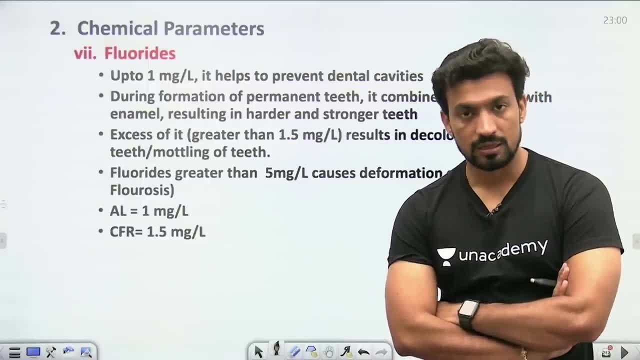 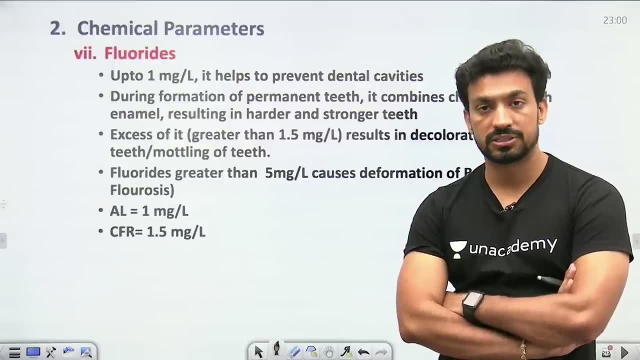 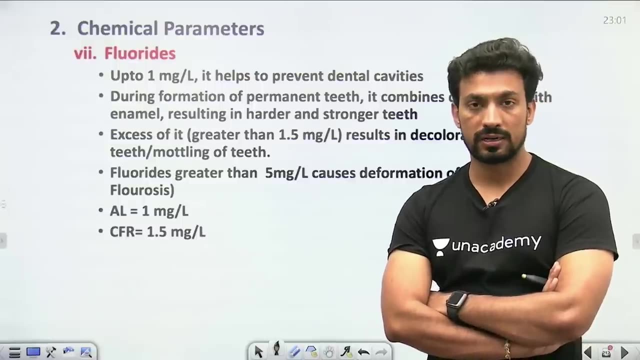 It will be seen more because fluoride helps to make the teeth strong. But the fluoride concentration of toothpaste is only for cleaning your tooth or for its physical contact. It is not to be consumed in the body. You don't eat toothpaste Until and unless your taste is completely different. 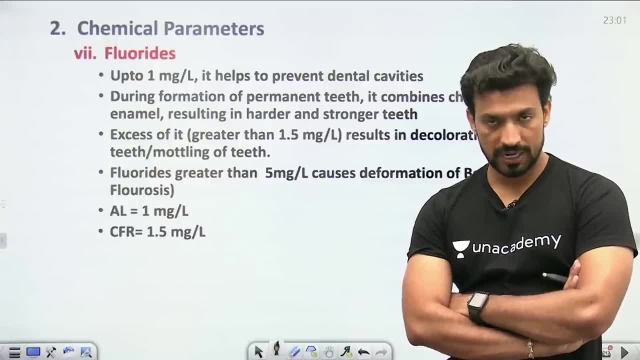 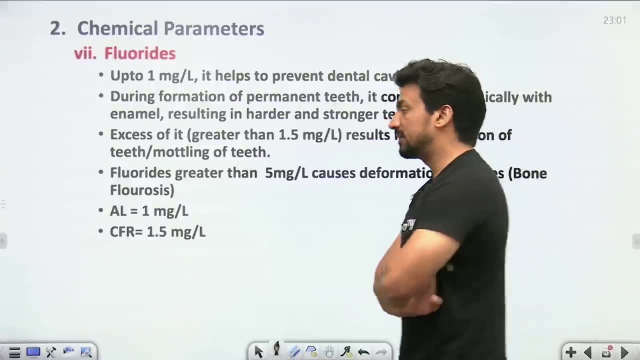 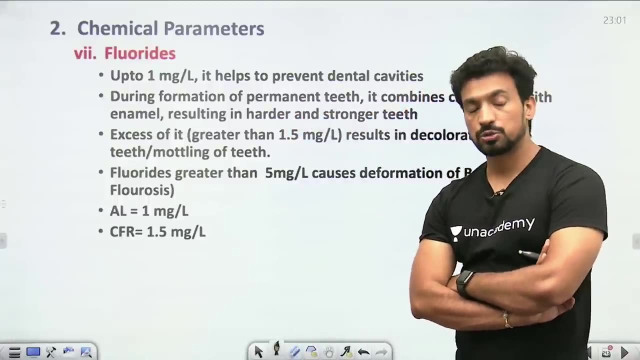 So the toothpaste also contains fluoride. We are studying the properties of drinking water here. So if fluoride is up to 1 mg per litre then it will help to prevent cavities or dental caries. If it starts to be more than that it will go up to 1.5 mg per litre. 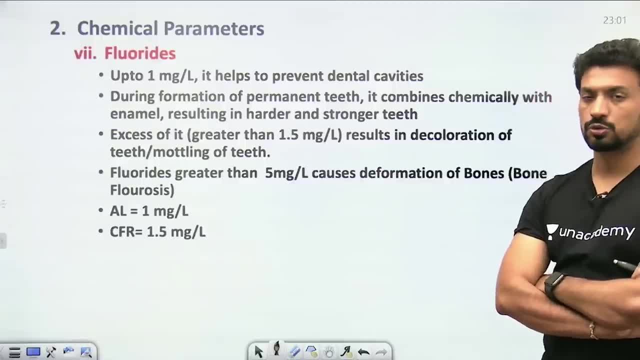 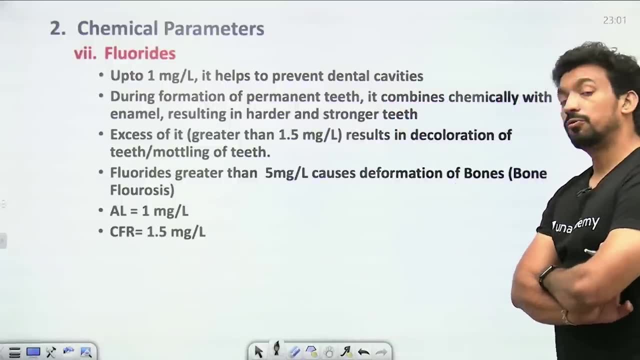 In that case the color of the teeth will start to be decoloration, They will start to be yellowish. The yellow tint will start to come in it. Now, if it is more than 5 mg per litre, then in that case the bones or joints become stiff. 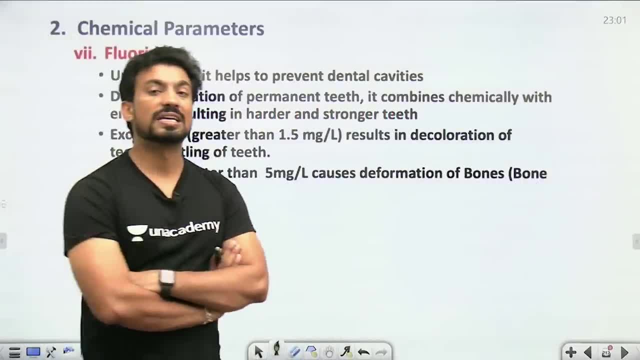 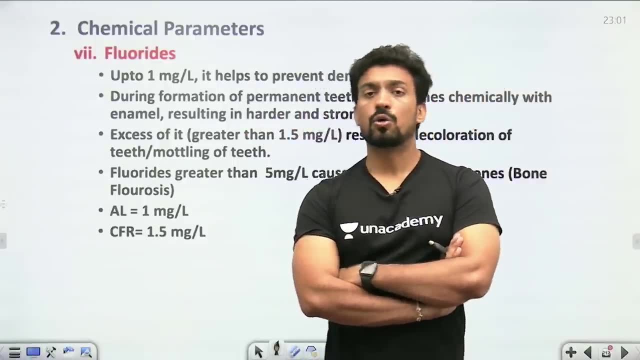 The shape of the bones will start to deteriorate. There will be deformation of the bones. It is not that it starts to happen in a day that you drank fluoride water and it happened. No, It happens over the time. It happens after consuming a lot of time. 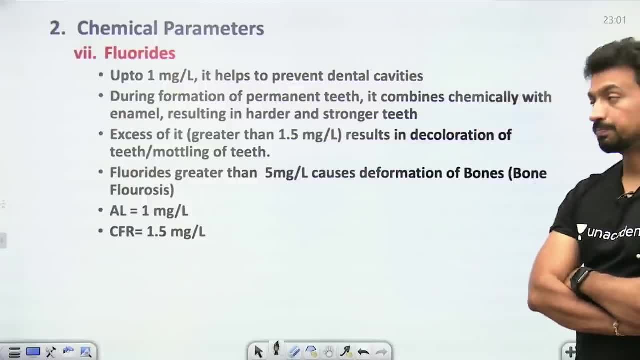 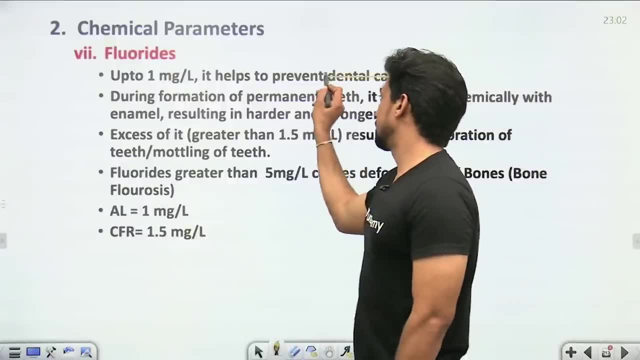 But after that it becomes very difficult to treat it. So 1 mg per litre helps to fight dental cavities. It does not allow dental cavities to happen. It does not allow dental caries to happen If it is more than 1.5 mg per litre. 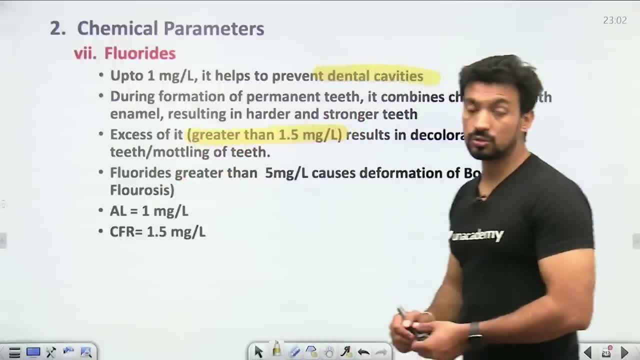 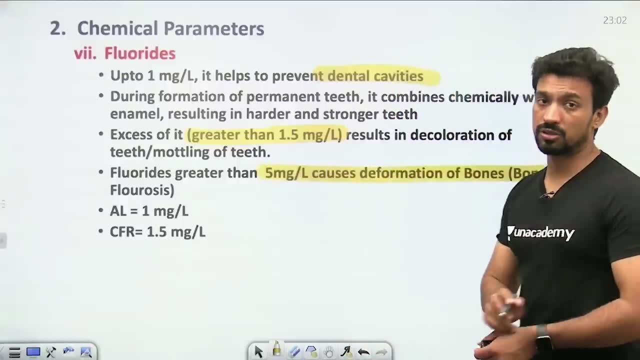 In that case it causes decoloration of teeth. If it is more than 5 mg per litre, then there will be deformation of the bones. Acceptable limit is 1.. Cause for rejection is 1.5.. Next let's move ahead. 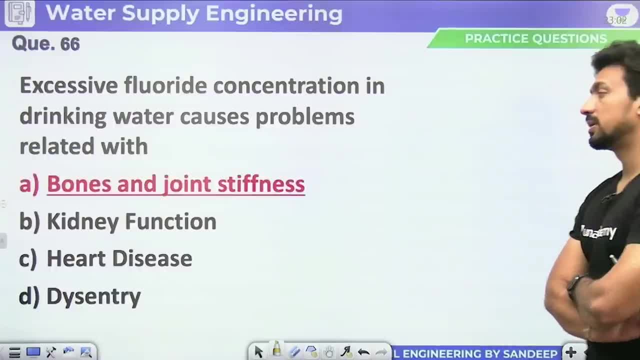 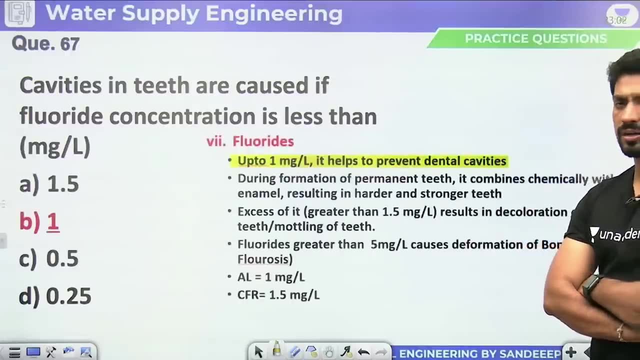 Excessive fluoride concentration in drinking water causes problems related to bones and joint stiffness. Cavities in teeth are caused. if fluoride concentration is less than 1 mg per litre Or if it is less than 0.5 mg per litre, then it will happen. 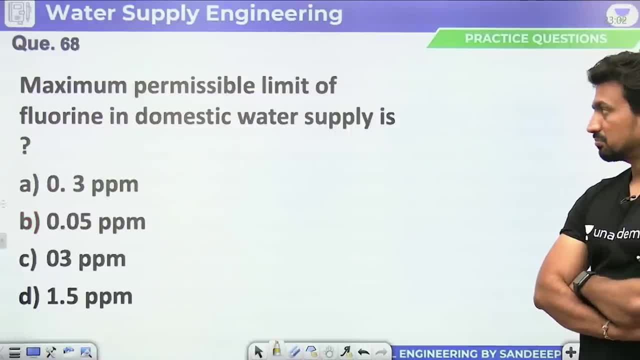 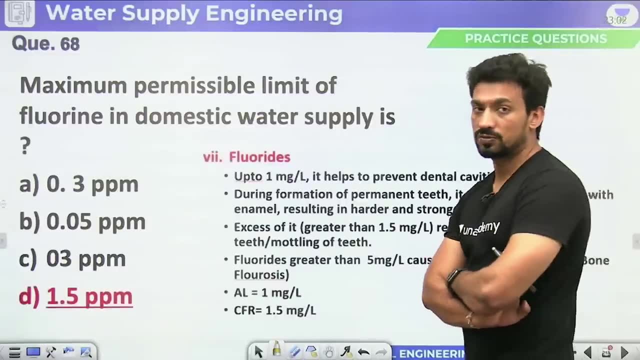 1 mg per litre is an acceptable limit. Maximum permissible limit of fluorine in domestic water supply is 1.5 ppm, Or it is called cause for rejection. If we talk about iron and manganese, then iron is 0.1 or 1 mg per litre. 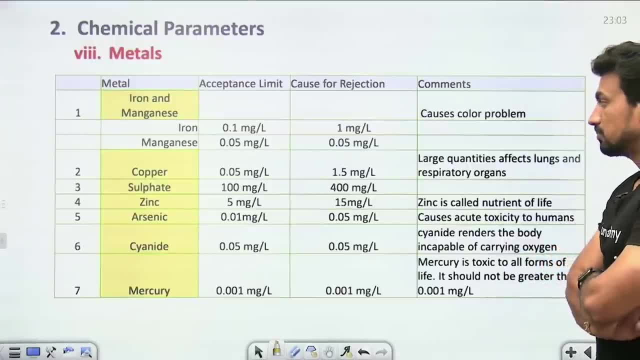 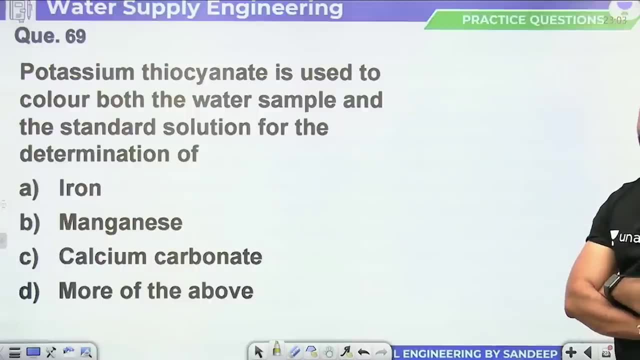 It has an acceptable limit. Manganese is 0.05.. If you have copper, then 0.05.. Sulfate is 100.. Zinc is 5.. Arsenic is 0.01.. The table that I showed you in the beginning. 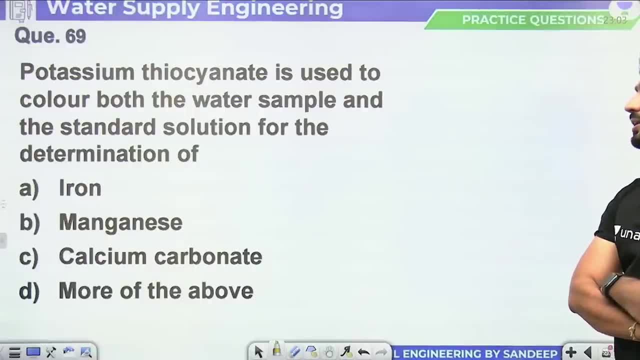 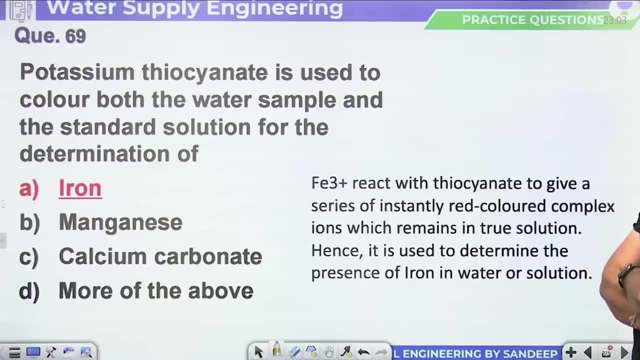 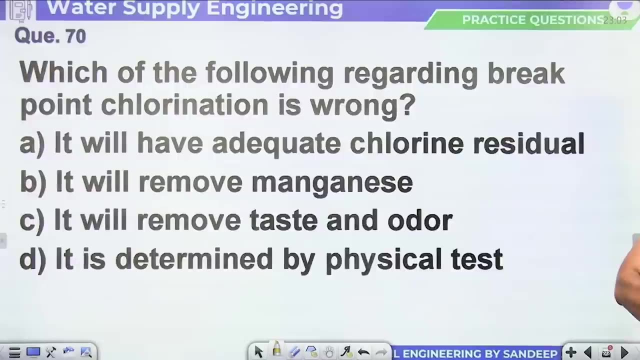 These values are related to that. Let's use potassium thiocyanate in the water sample. What to find out? To find out the iron. you use potassium thiocyanate, Which makes a red coloured complex Which is present in the solution and determines the iron. 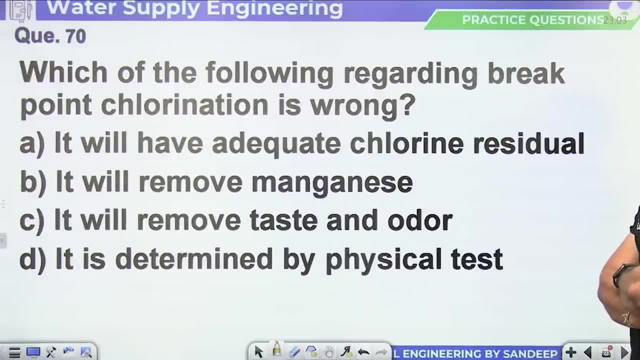 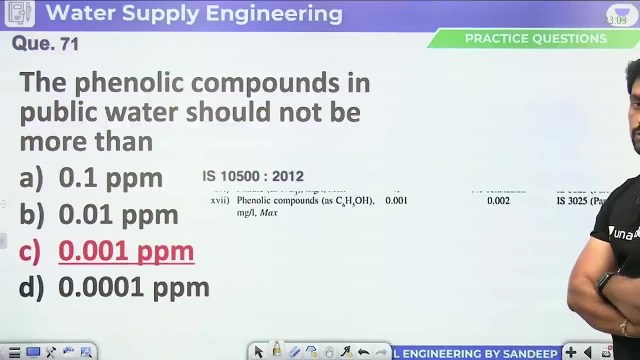 Which of the following, regarding breakpoint chlorination, is wrong? Which of these is wrong about breakpoint chlorination? We will get to that in the lab test and this question will be added first. Phenolic compounds in public water should not be more than Phenolic compounds should not be more than 0.001 ppm. 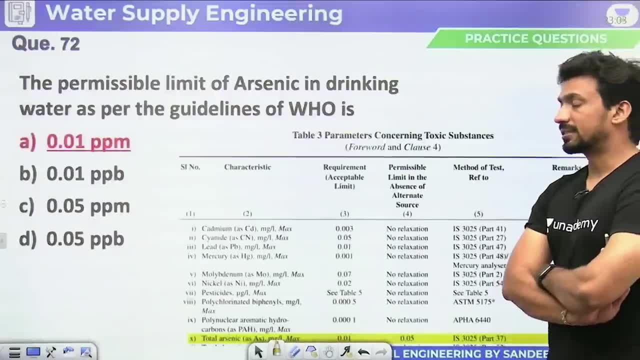 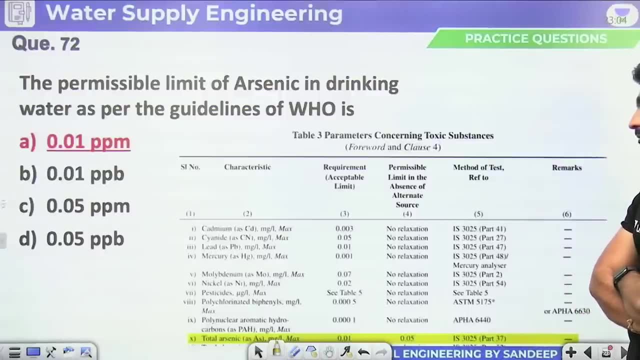 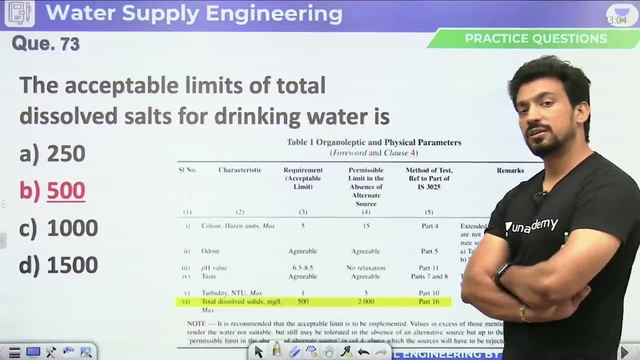 The permissible limit of arsenic is 0.01 ppm. If the objective asks you, then the limit of arsenic is 0.01.. Acceptable limit of total dissolved salts: 500. Cause for rejection: 2000 As per Indian standard: 10500. 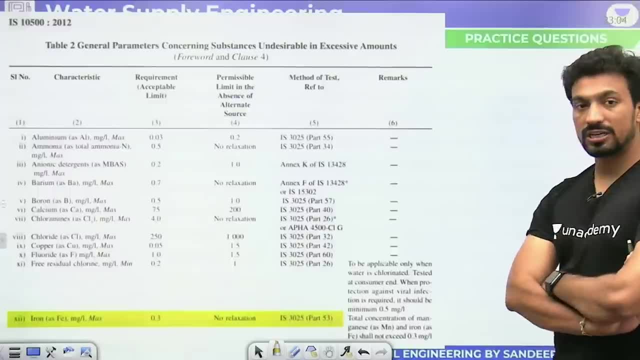 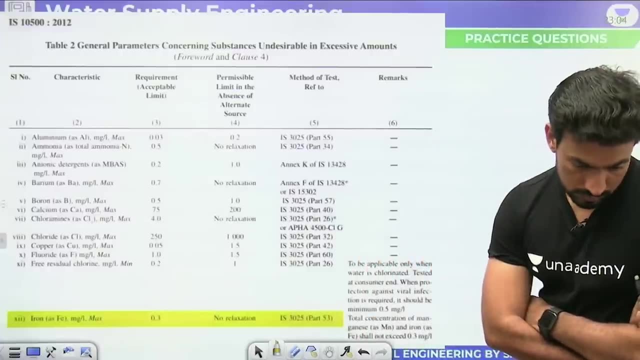 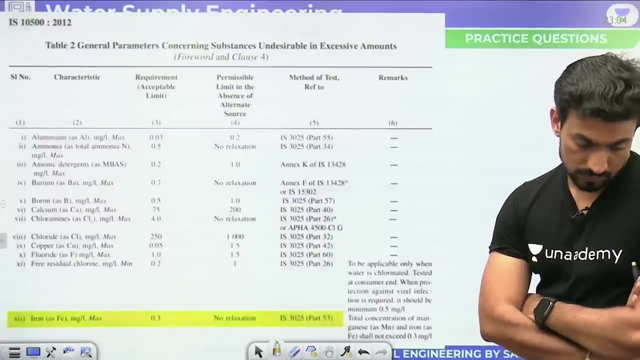 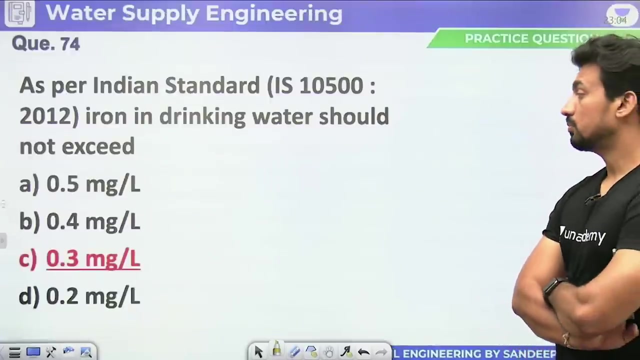 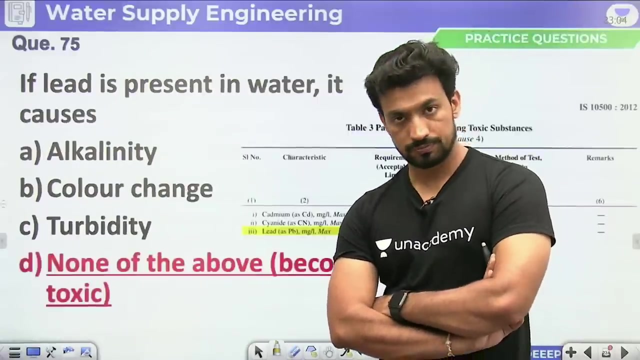 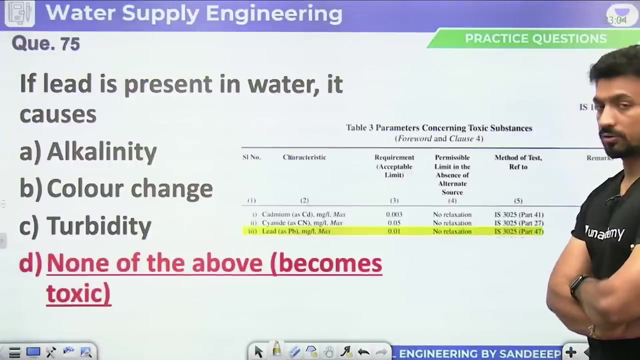 Iron in drinking water. So if we talk according to Indian standard, then you get 0.3. Next, If lead is present in water, Lead is toxic. We will not want it to happen. Lead is toxic. Lead's acceptable limit is 0.01 And there will be no relaxation from that. 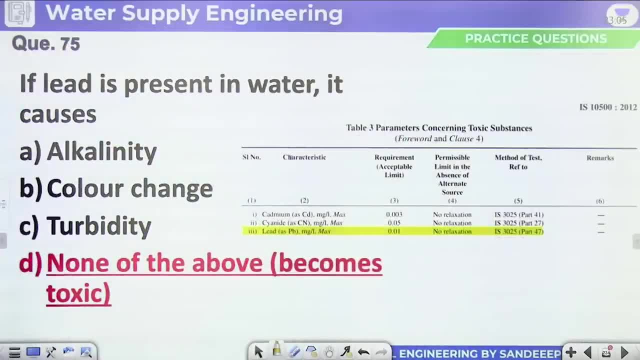 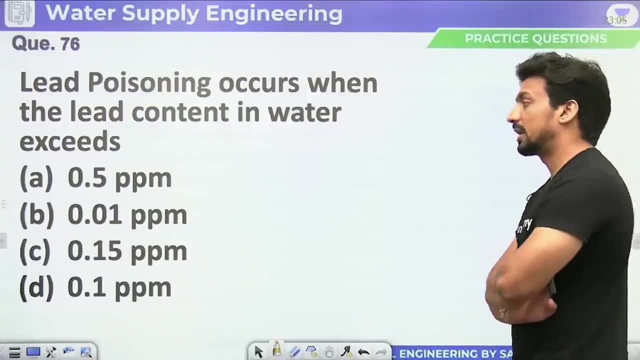 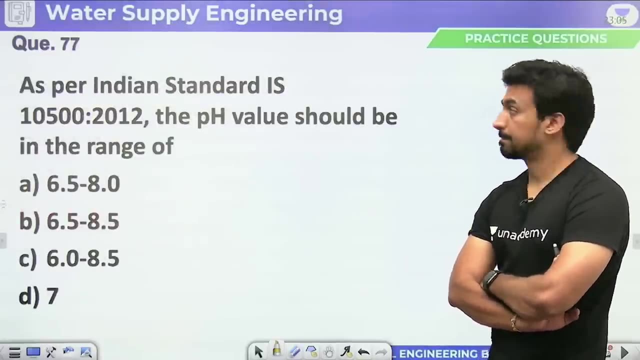 Or cause for rejection will also be considered. 0.01. We will not provide it above that. So if there is a question in objective that when will lead poisoning start, Lead poisoning starts. Lead poisoning starts If it is more than 0.01 ppm. So this question is also asked in objective. As per Indian standard 10500, The pH value should be in the range of pH should be from 6.5 to 8.5 For drinking water, And all this data is going according to 10500, Why I am providing you all these tables. 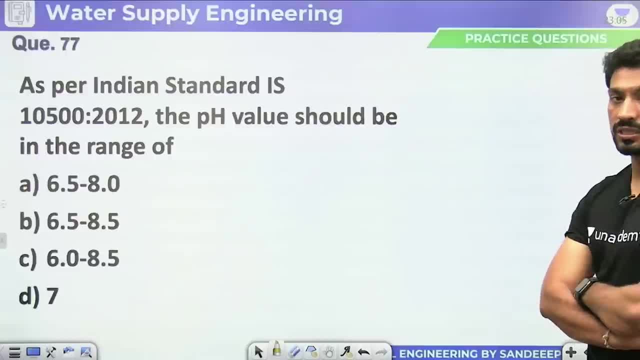 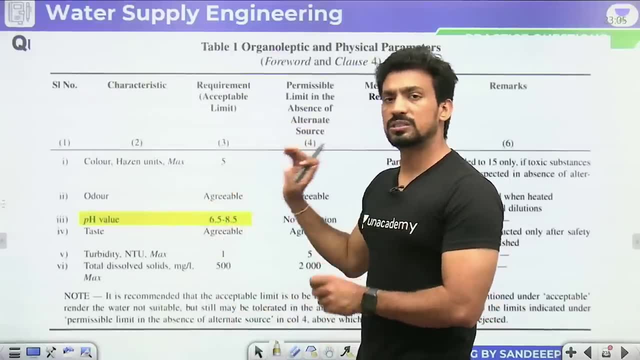 Just to see the effect. If we see any question Now, it is going according to This table. Now we are getting more confusion in this question That it will be 6 or 6.5 or 8.5. If you see this table, Then obviously understand. 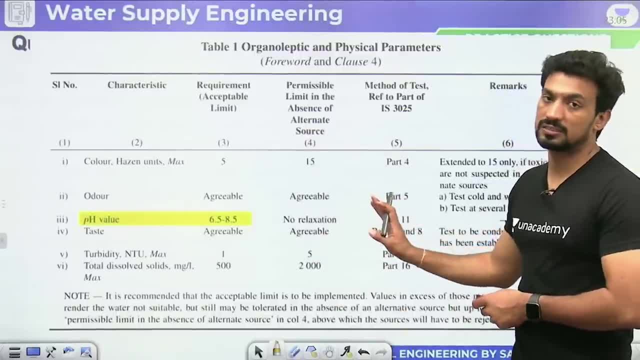 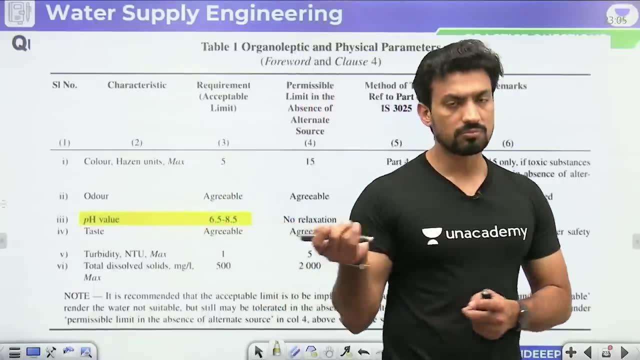 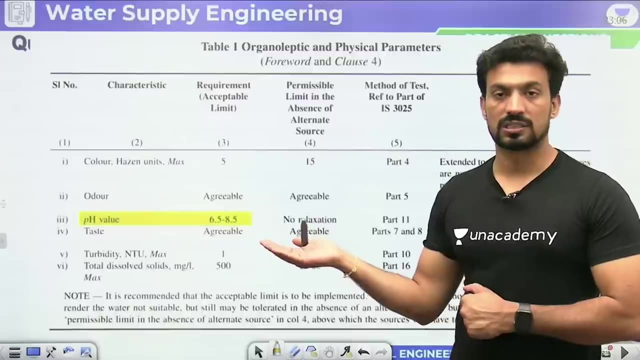 That this code is given as it is And we have chosen the correct answer In environment engineering. this is very important. This is as it is. Provide screenshots to you Because The values of WHO, Then after that Your government of India, manual values, comes And our values of this code comes. 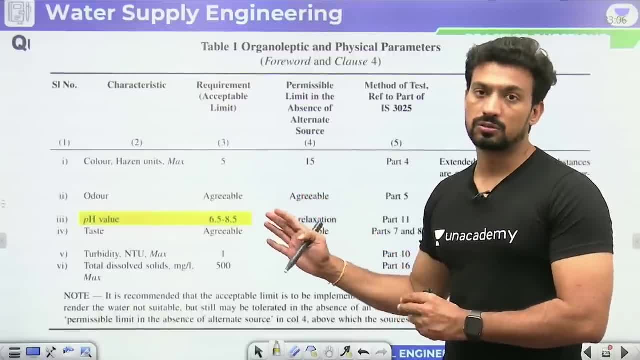 So, at all times, we are adhering to Indian standards only. So that's why we are adhering to Indian standards only. So that's why we are adhering to Indian standards only. That's why you are given these screenshots of this code. I am providing you side by side. 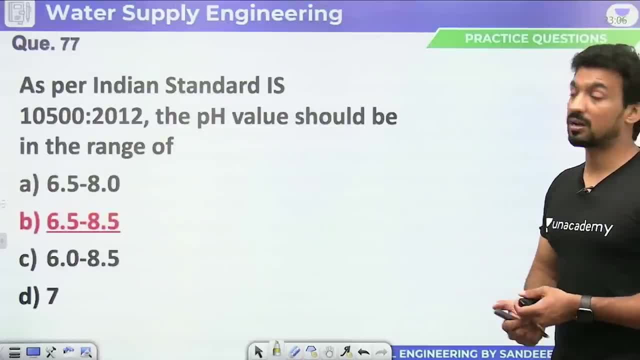 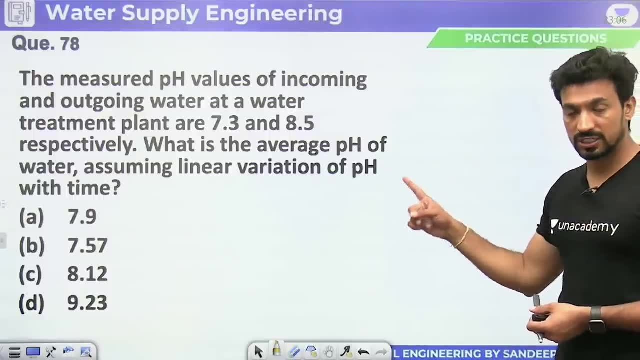 So that you don't have to study the code yourself: How much to read, What to read, Where to read. There should be no confusion of all of them, The measured pH values of incoming and outgoing water. Now a question related to pH. It was asked in SSE. It was also asked in EAC. 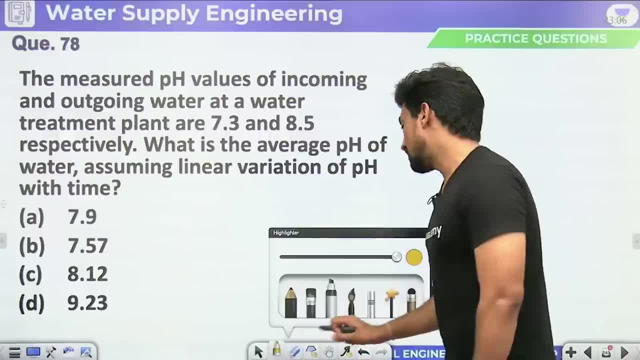 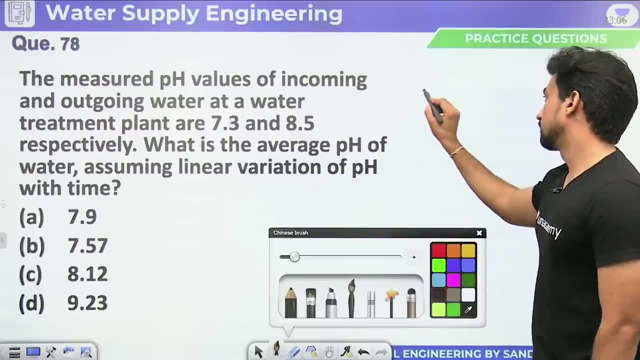 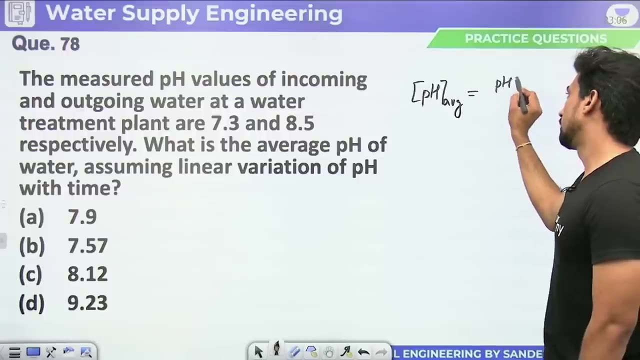 It was also asked in GATE. It is a very simple question. The pH value is to be calculated by the average. You have added two types of water So you have to tell the pH average. Tell the answer quickly. So if you want to calculate the average, then you take the pH of the first water and take the pH of the second water and divide it by 2.. 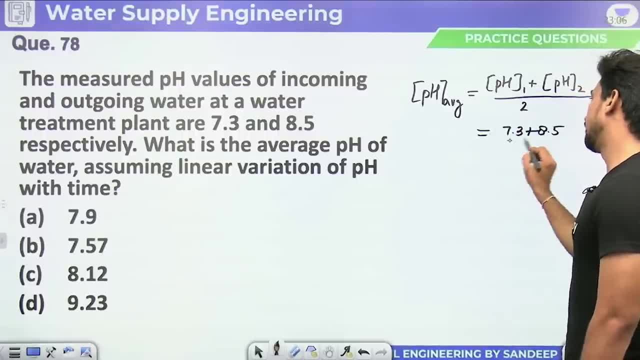 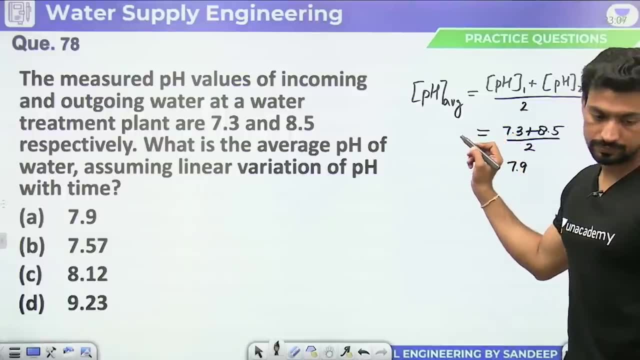 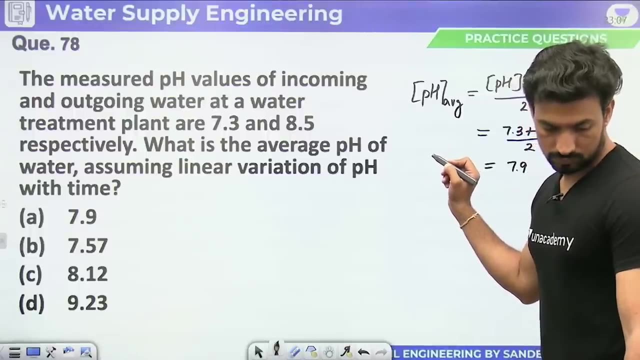 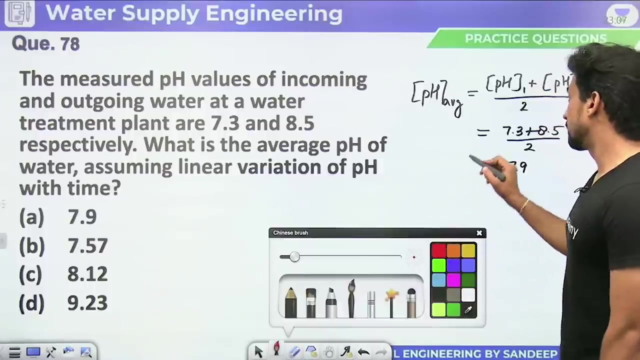 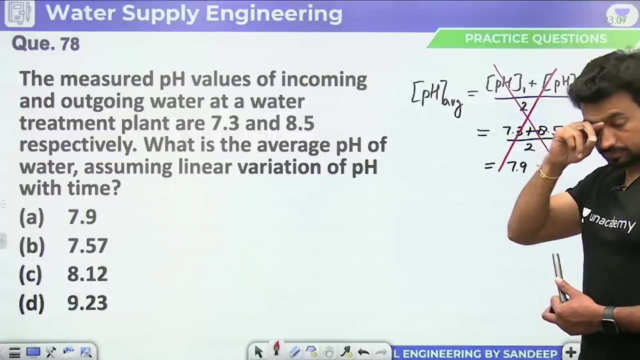 So we will divide it by 7.3 plus 8.5.. So you will get the answer 7.9.. This will come Option A, Those friends who have told Option A. tomorrow morning they will wake up, work, go to the market, bring a red pen from the stationery shop and then ask themselves: what did I do? 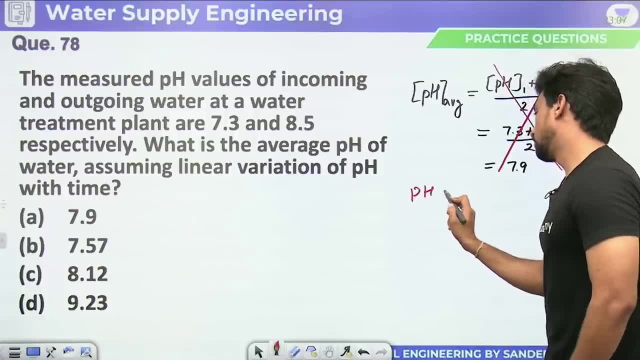 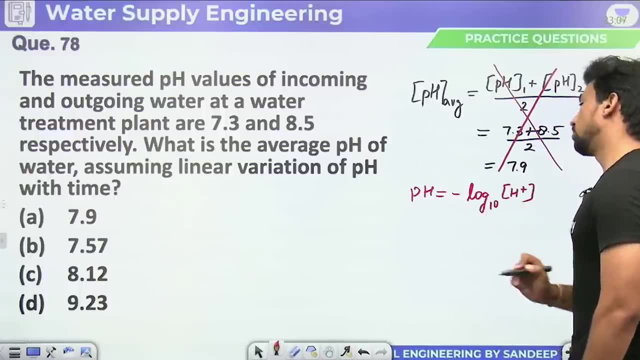 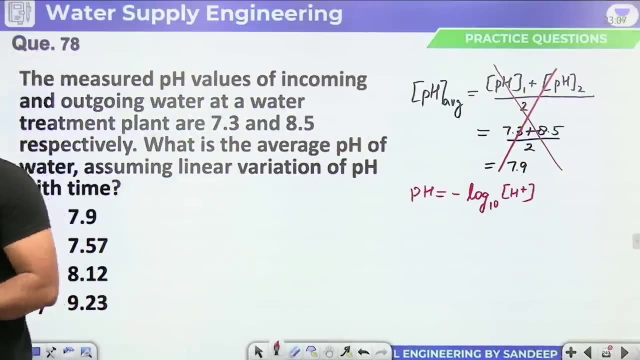 We had the basic formula of pH. that pH is equal to minus of log base 10, H positive concentration. So you just have to see that if those two water are mixed, then after mixing how many H positive ions have become in that water? 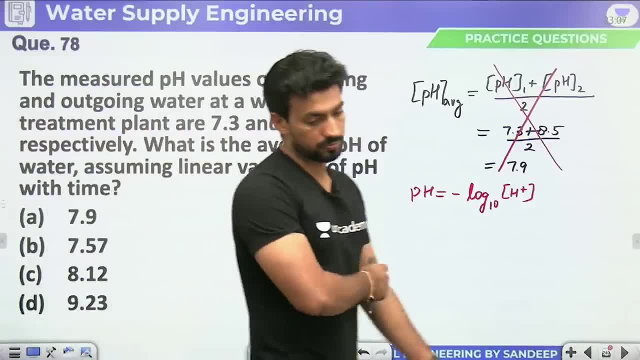 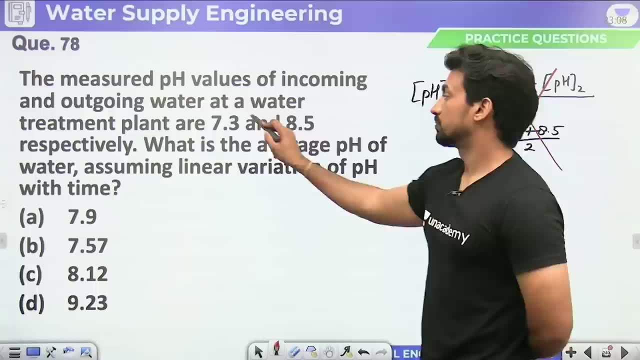 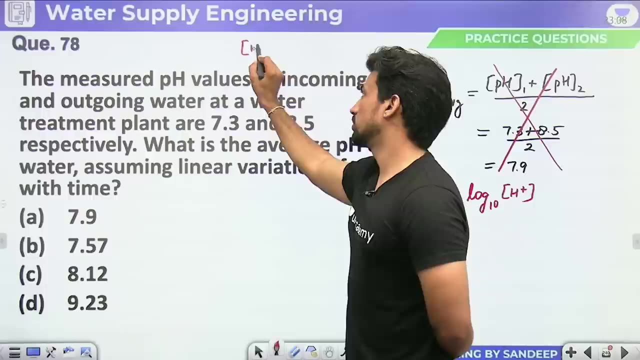 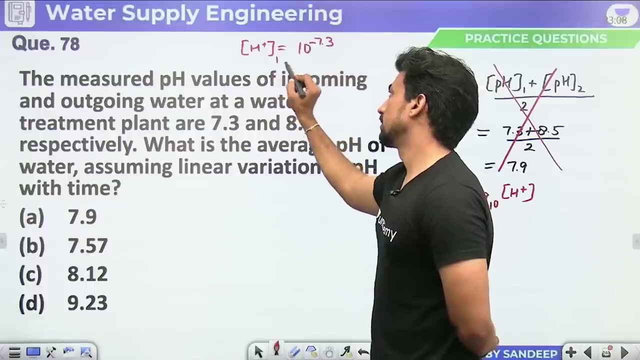 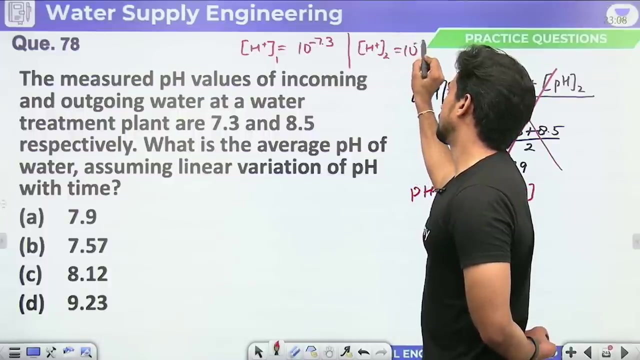 After calculating that you have to tell the pH after that Clear. So what will you do first If the value of pH You see like this: that pH is equal to minus of log base, 10, H positive concentration. So if you want to calculate H positive concentration, then 10 raised to the power minus 7.3 will be done in the first case and H positive concentration will be done in the second case, 10 raised to the power minus 8.5.. 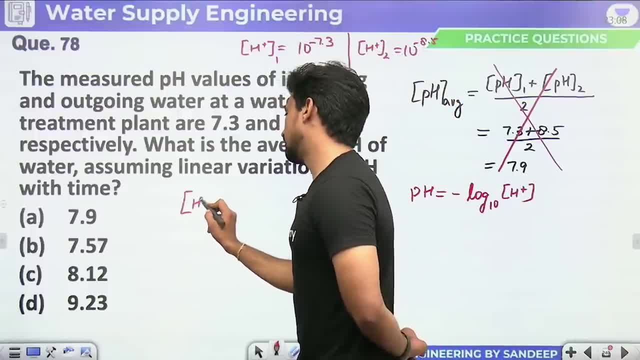 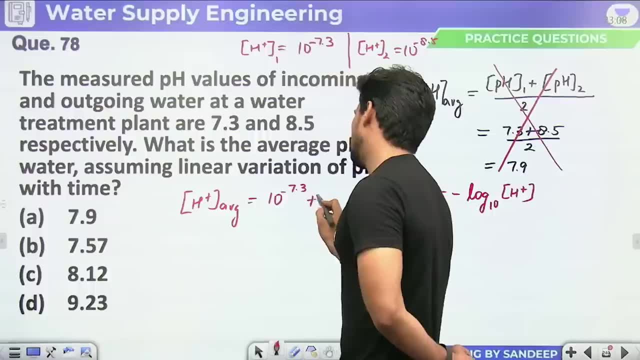 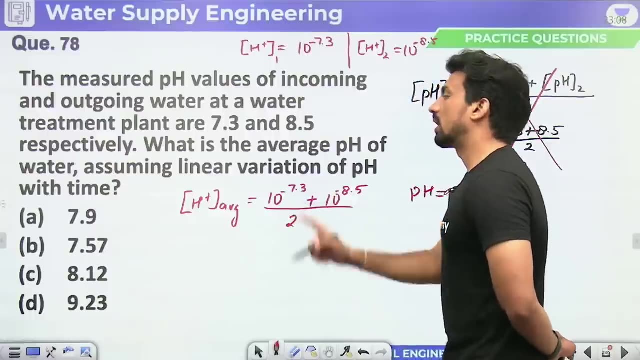 And now you will calculate the average of H positive ion, Which will be 10 raised to the power minus 7.3, plus 10 raised to the power minus 8.5, divided by 2.. And now you will calculate its log. 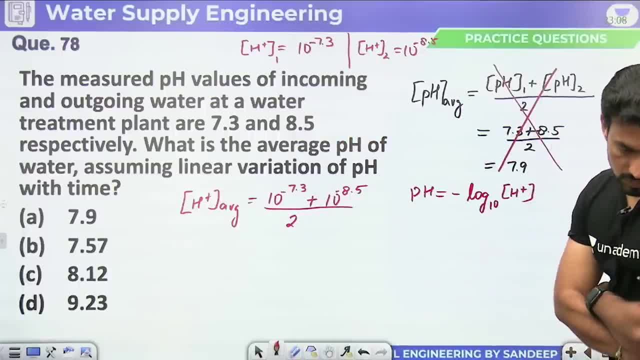 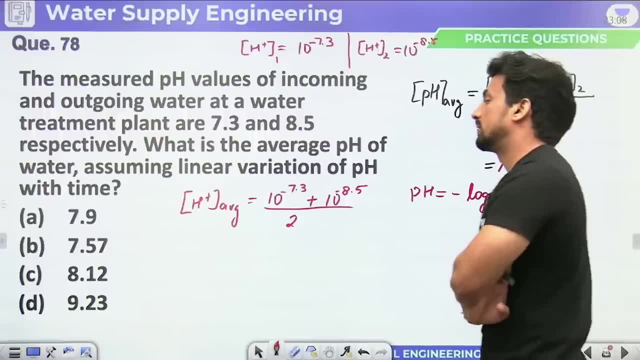 You will take. its log Calculator will not be allowed. How will this question be? This question was already in the gate. Then this question will be taken as it is. in some state It was used in the state exam, So such a question has to be done in the last. 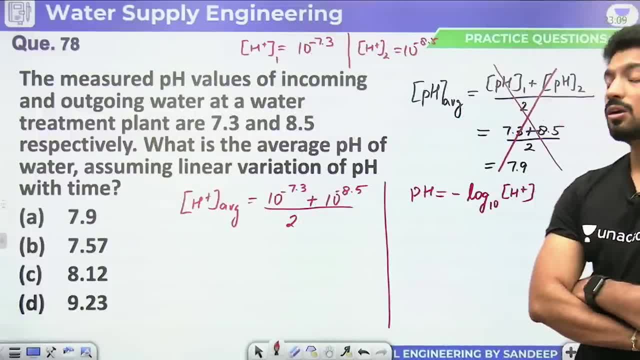 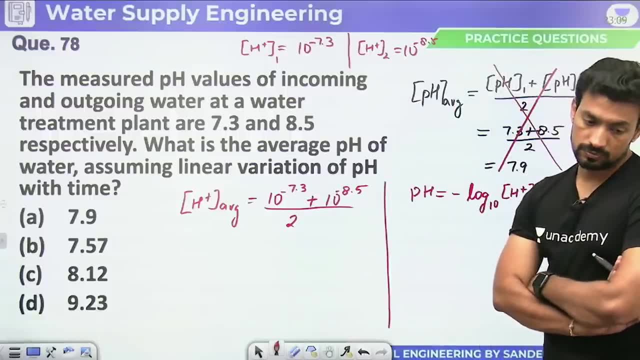 Have to do it in the last, In which it takes a little time in calculation. It is not very difficult to do. You can take the common from it, You can take the common of minus 8.5.. And still, if it is not possible, then we will see in the last. 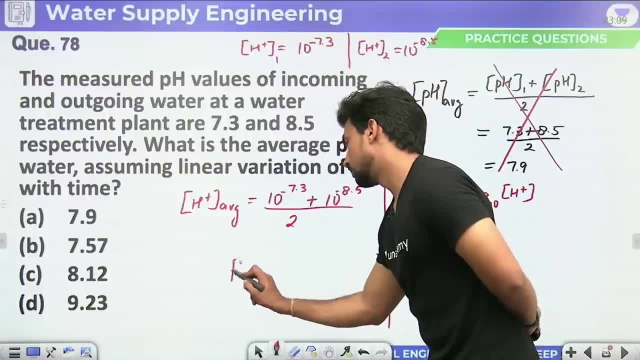 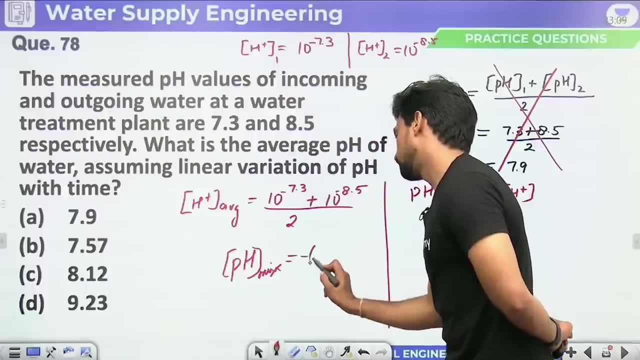 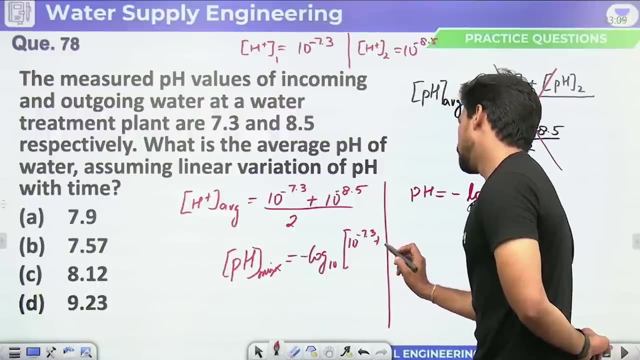 7.57 is coming. It is the value of H Of mix, Or it will give you only the value as it is, In which you will be able to do something by taking common What, What, What, What, What. 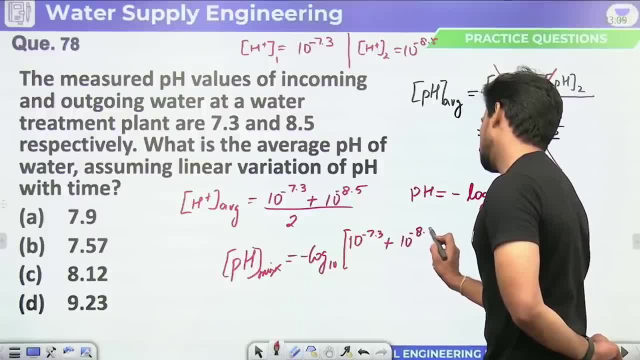 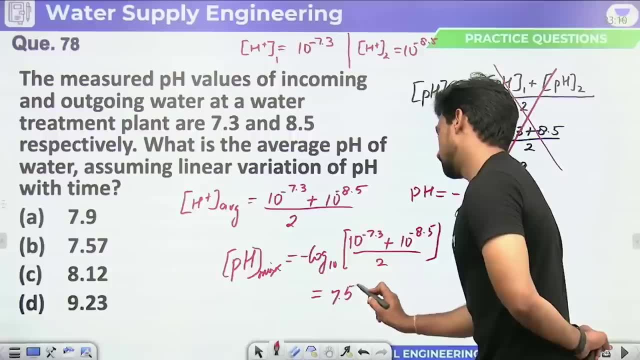 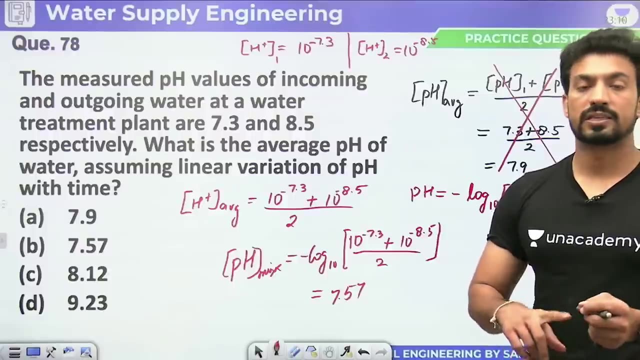 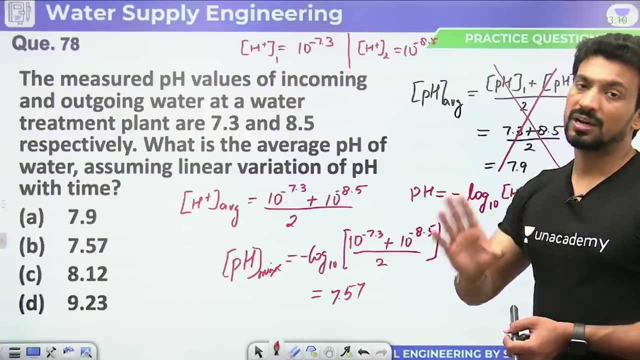 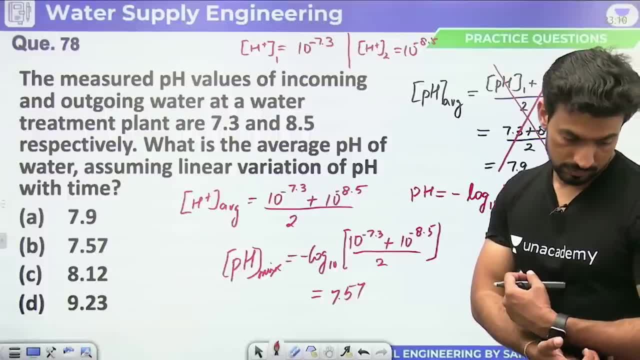 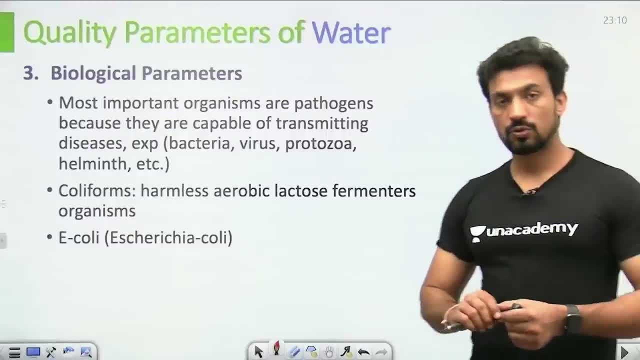 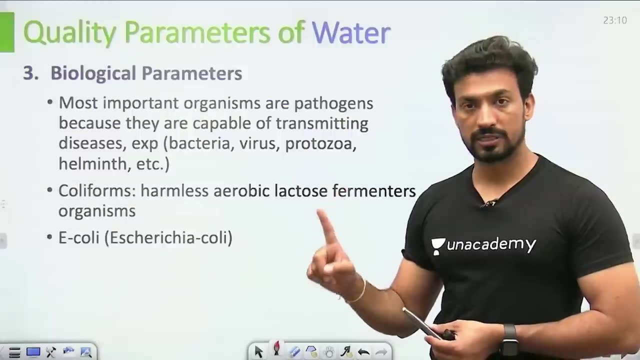 you can also do 11. ok. next let's move forward. let's come to biological parameters. in biological parameters, how do you check the quality of water? to check the quality of water in biological parameters, e-coli is used. e-coli is a harmless bacteria. if that harmless bacteria is also not, 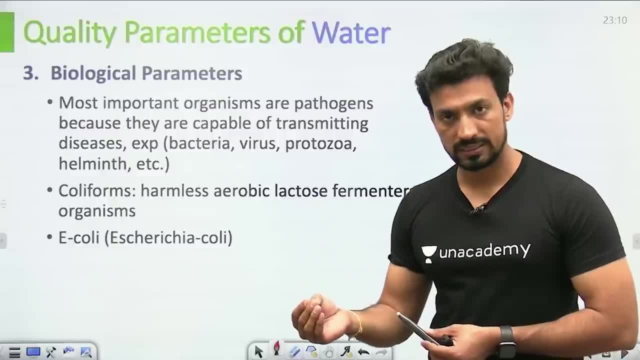 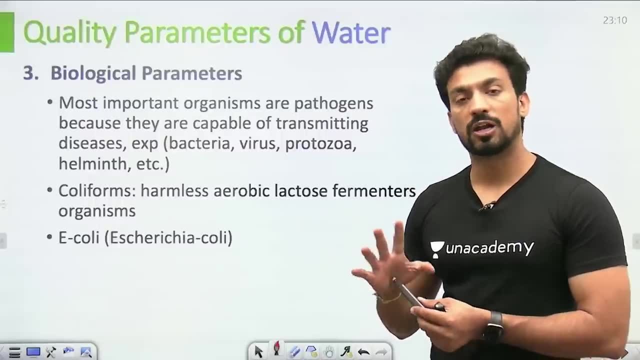 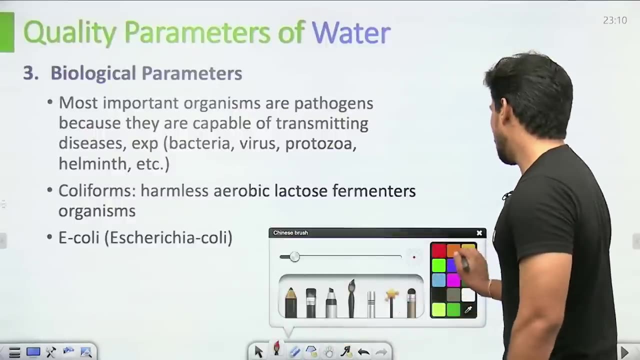 present in water. their life is the most. if harmless bacteria e-coli life is the most. and even if it is not present in water, then it means now our water is free of biological impurities. it is not present in it. e-coli is used and that should be. 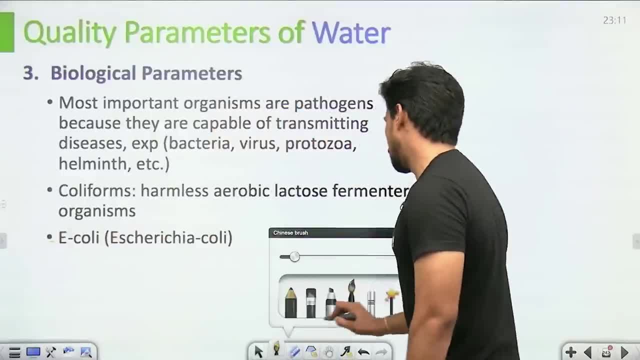 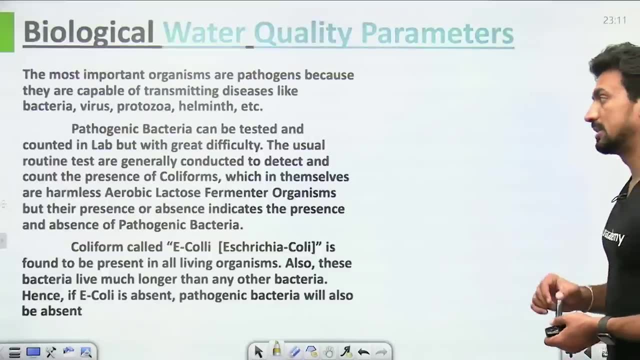 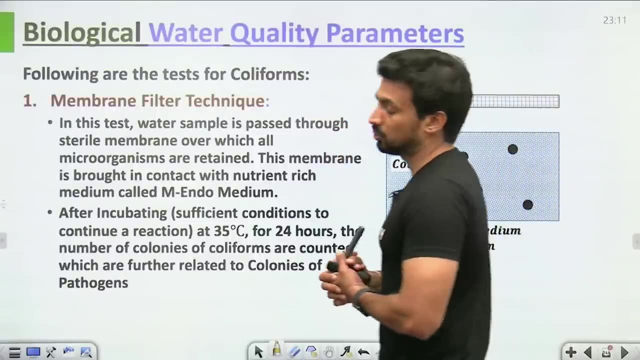 hardly detected in 100 ml of water. this is the objective question asked to you. so e-coli is used. you should remember this. e-coli is a coliform which is harmless. then, after that, membrane filter technique is used, water is brought in the contact of a nutrient-rich membrane. 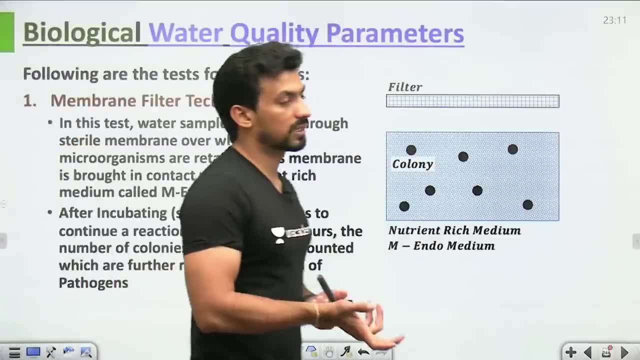 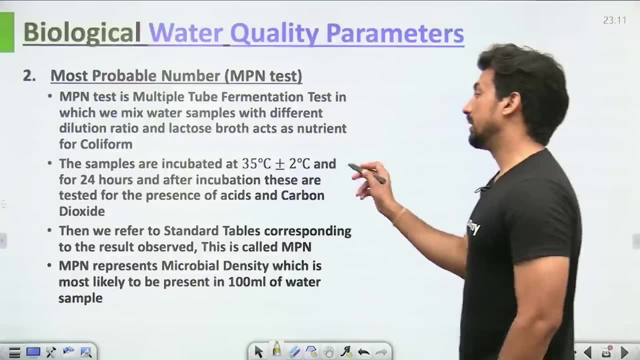 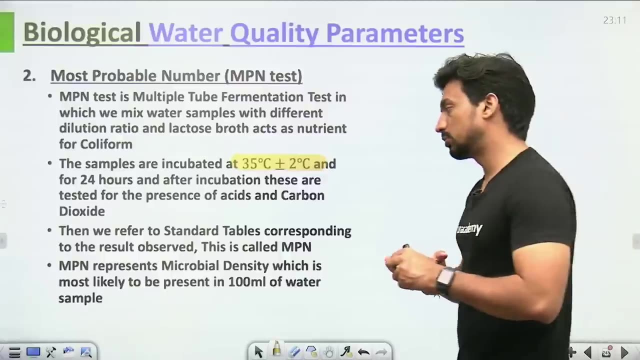 here their colonies are counted, how much growth is happening, how much microorganism is present in it. similarly, mpn charts or mpn test, through that we can do their temperature. Remember the temperature it is incubated at 35 ± 2 ºC when you represent its microbial density or calculate the MPN numbers. 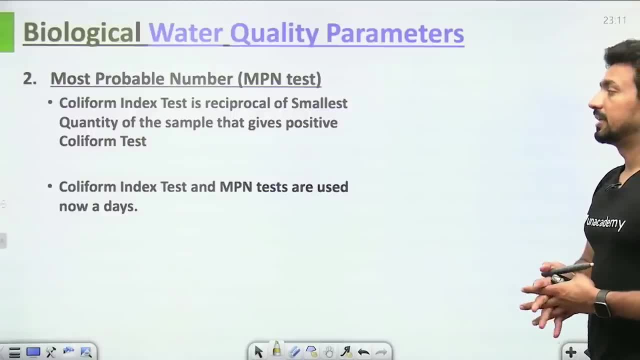 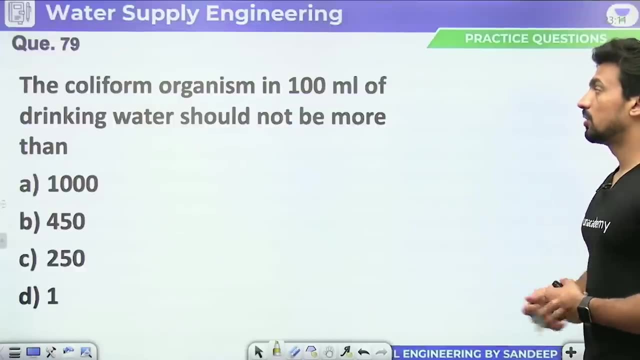 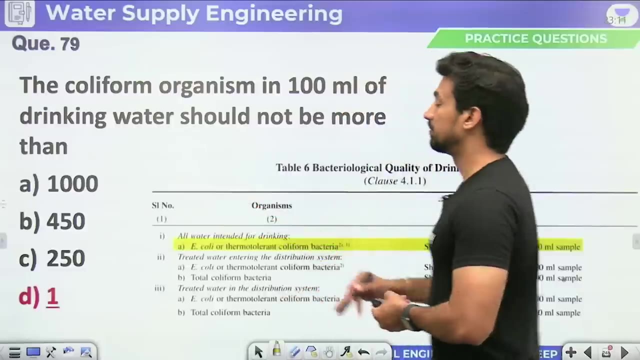 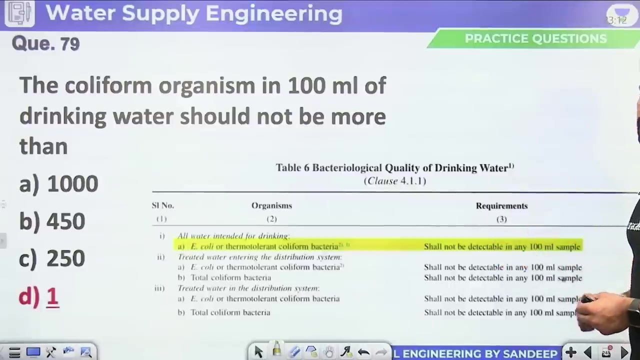 Coliform index test is reciprocal, of smallest quantity of sample that gives positive coliform test. So you will use these. Coliform organism in 100 ml of drinking water should not be more than 0, but it was not given. E coli or thermo-tolerant coliform bacteria shall not be detectable in 100 ml of sample. 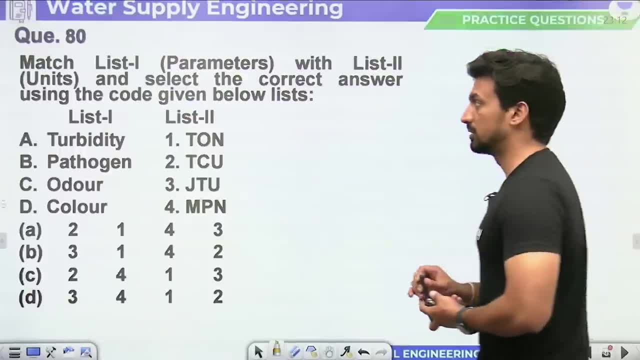 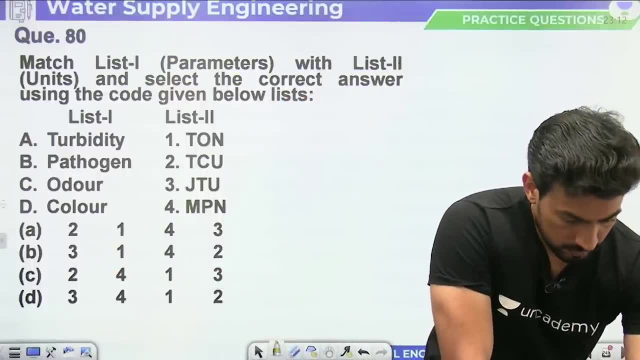 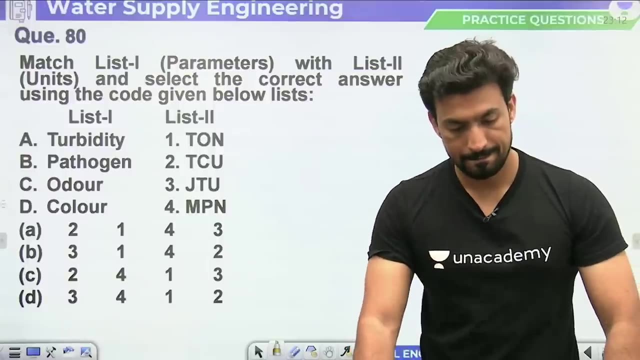 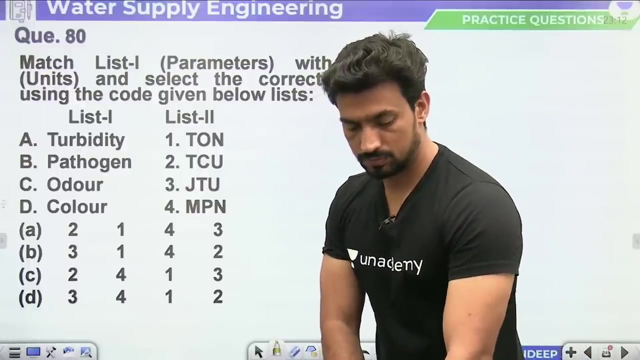 This is the requirement for drinking water from objective point of view. Next statement is for you, Match the following: Tell me quickly: When it comes to drinks, you must not drink it when it is not the right water. If it is not the right water, it is not good for you. 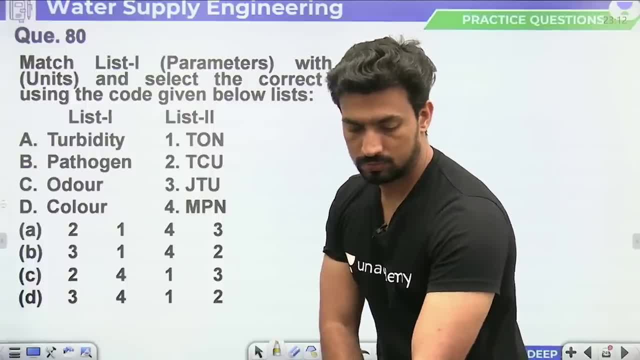 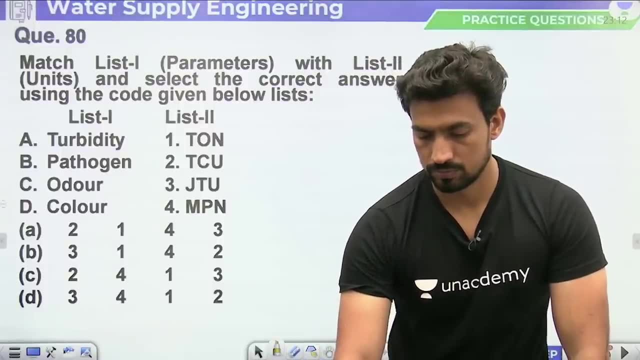 Anyhow, if you don't drink that water, you might be infected. The patient, Michael Eli MD, is the leader of the panel of glasses in the world of Dr RIS. He has been working with us on the study of the lactic acid and lactose secretions in our body. 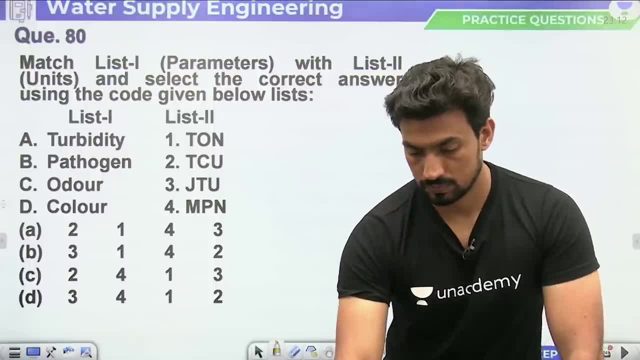 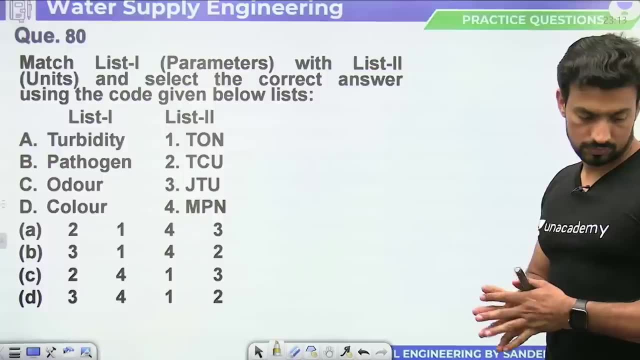 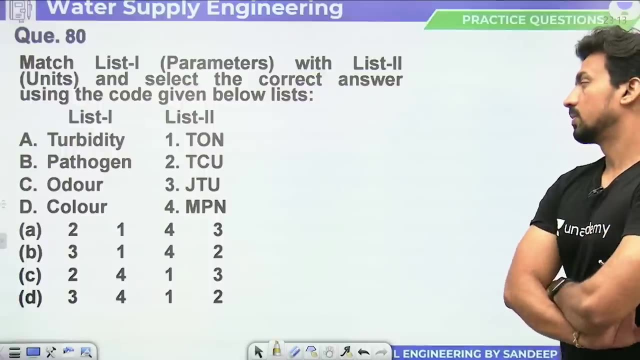 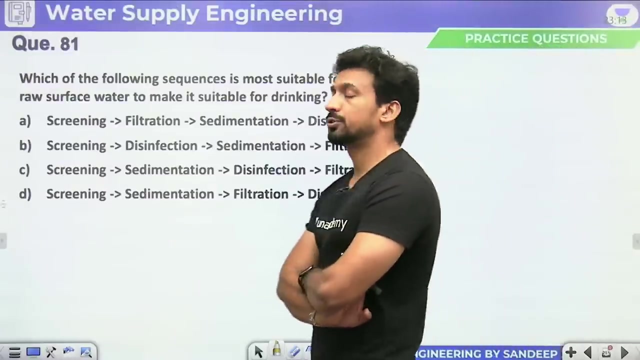 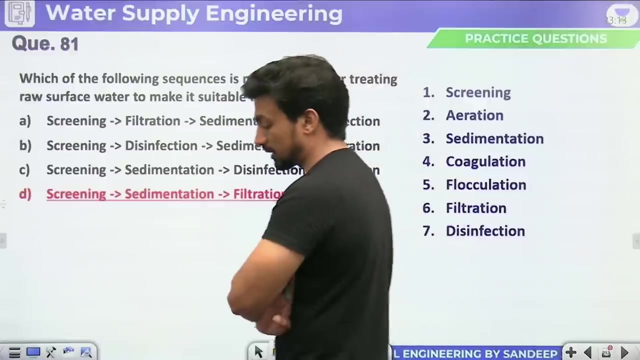 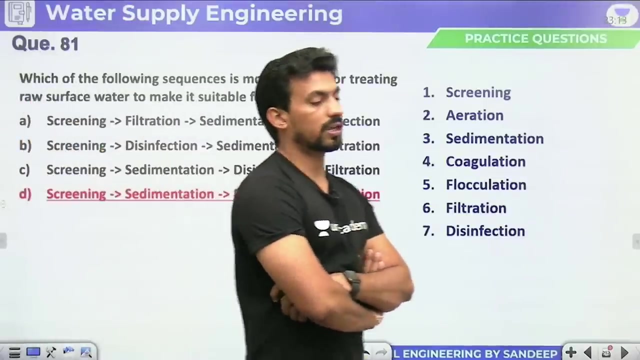 Which of the following sequence is most suitable for treating raw surface water to make it suitable for drinking? So first of all, we will do screening after screening, we will do aeration, then sedimentation, then coagulation after coagulation, we will do flocculation after flocculation, we will 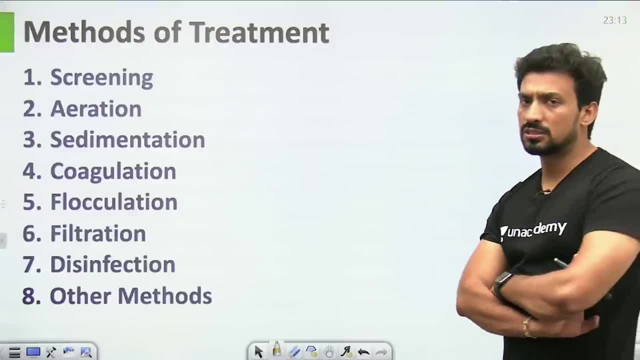 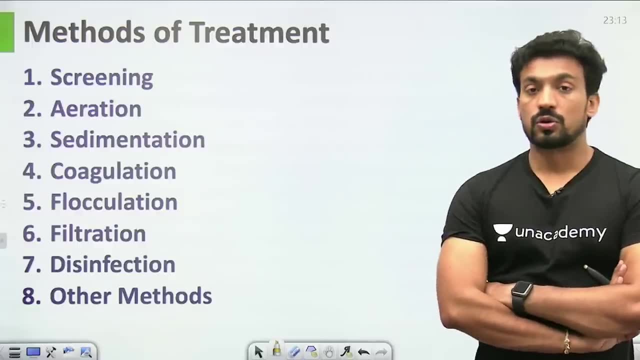 do its filtration, then we will do disinfection or any other process is needed, then we will do that. Large impurities will be removed in screening. in aeration, H2S and the gases like H2S, carbon dioxide, will be removed. 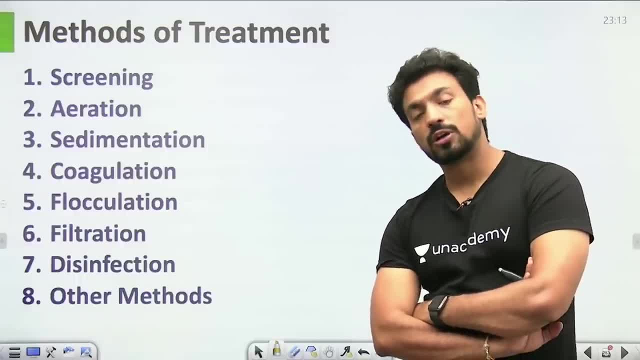 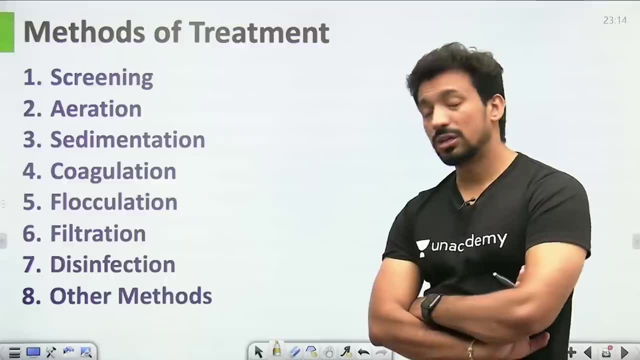 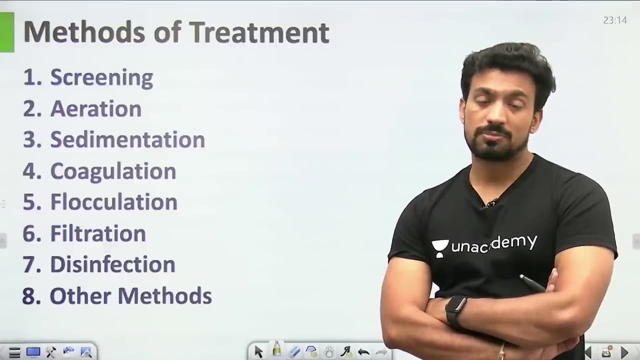 Ions like iron and manganese will be removed. large particles in sedimentation that can be settled due to gravity will be settled. coagulation will be added in coagulants like alum copperas, from which the charged particles that were not settling will be settled slow. 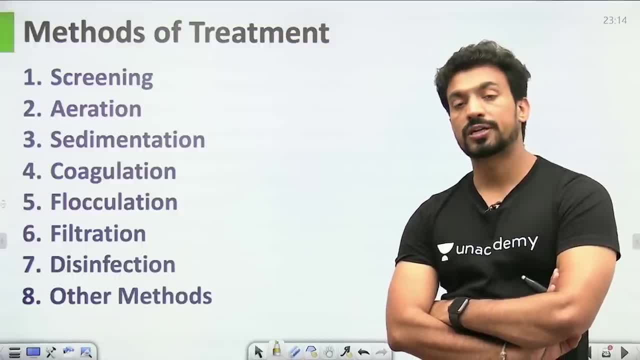 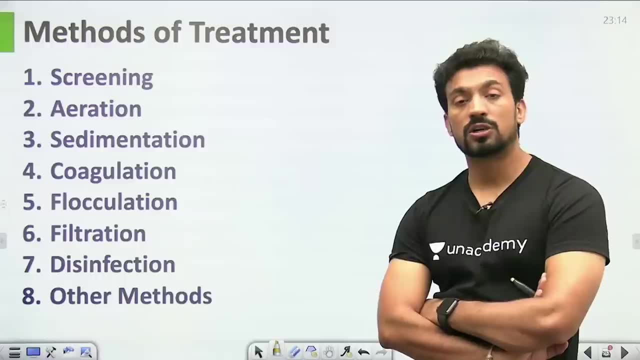 mixing will be done in flocculation so that the contact time between the particles increases and they make a group, make flocs, which will become heavy and they will settle. The particles that are present in filtration will be removed. The flocs that were not settled will be settled on the filter media. 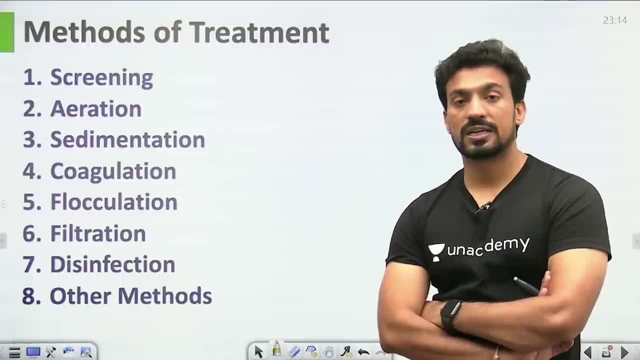 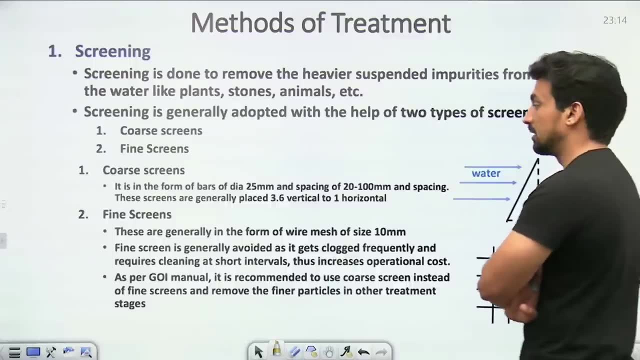 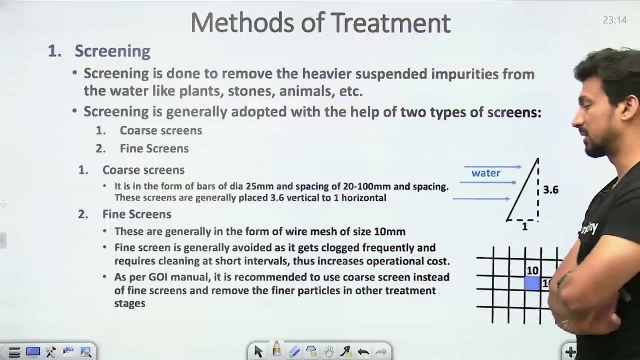 Then microorganisms or pathogens present in disinfection have to be killed in water so that the water is safe to use. What questions were asked to you in the screening objective? In the screening objective you were asked for an angle from 45 to about 60 degrees. 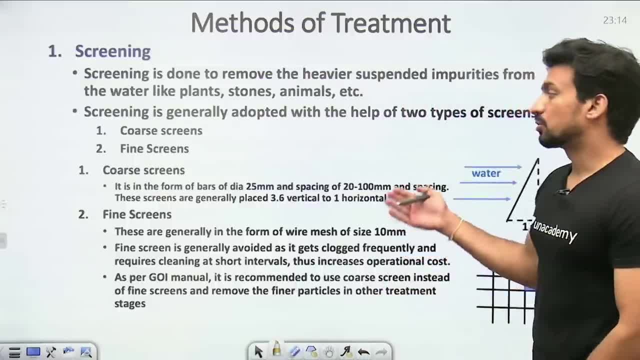 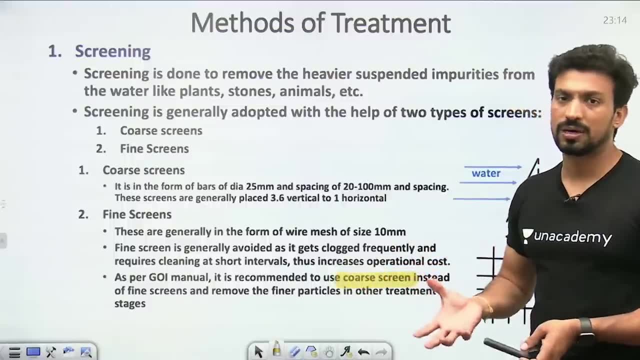 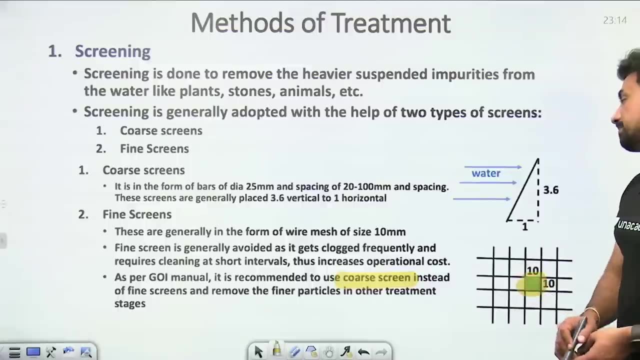 These screens will be kept. Screens are coarse and fine screens. Government of India manual recommends that you keep the angle between coarse and fine. If you use a fine screen, it will block the impurities again and again. You have kept a mesh of 10 mm and 10 mm size and kept a gap here. 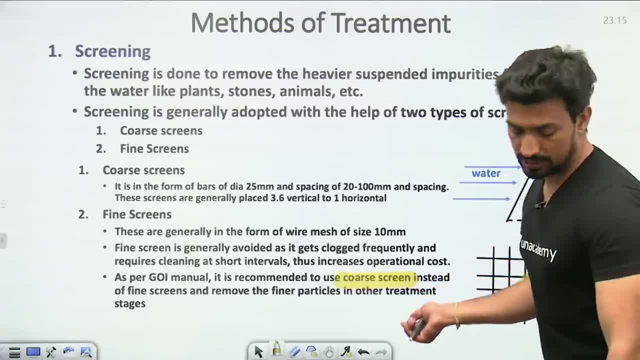 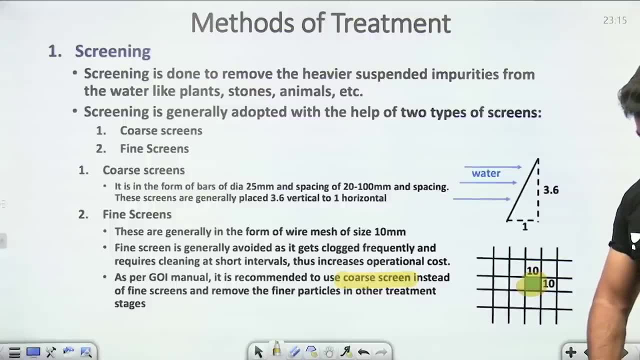 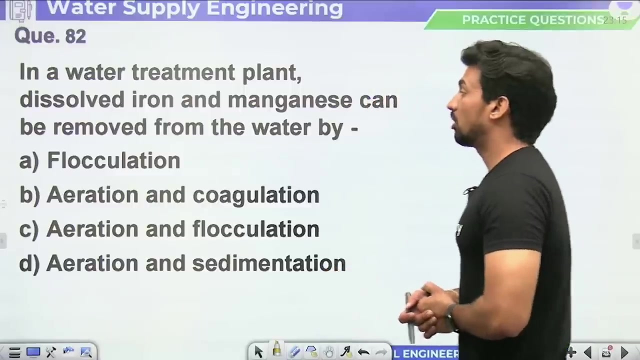 You use it in 1 to 3.6 proportion. The screen angle is 45 to 60 degrees. In a water treatment plant, dissolved iron and manganese can be removed by. They can be removed by aeration and later by sedimentation. 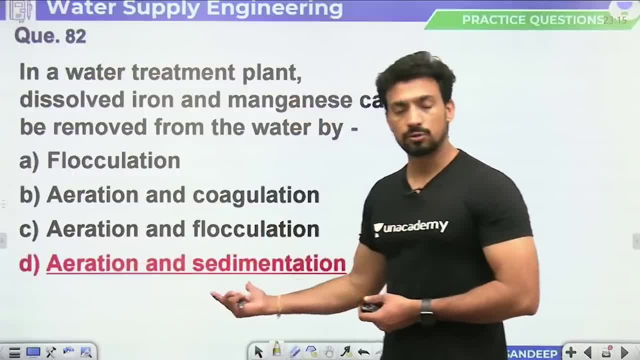 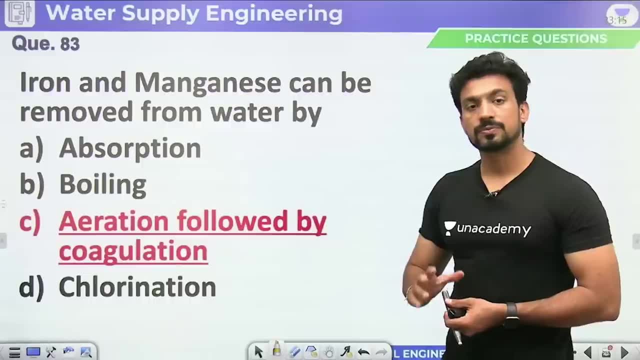 By aeration their precipitates will form and then they will be settled in the sedimentation tank. So we do aeration and sedimentation. Iron and manganese can be removed from water by. They can be removed by aeration and sedimentation. After aeration they will be settled in the sedimentation tank. 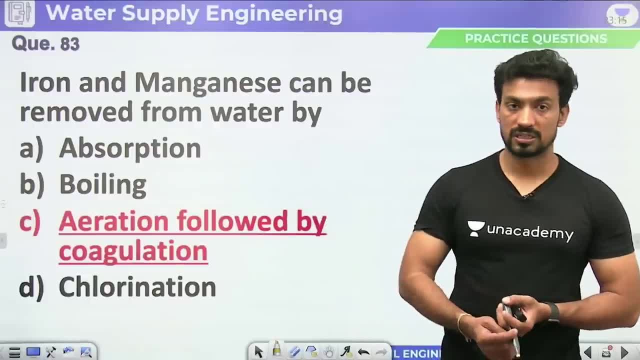 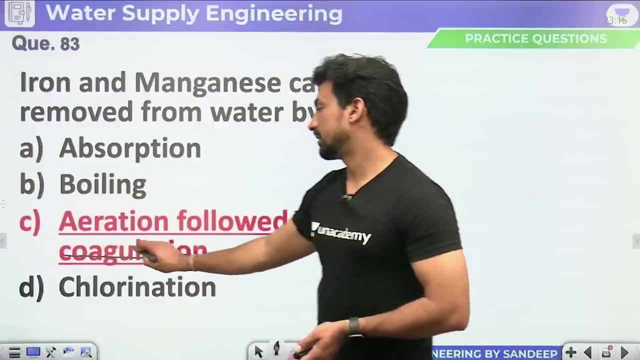 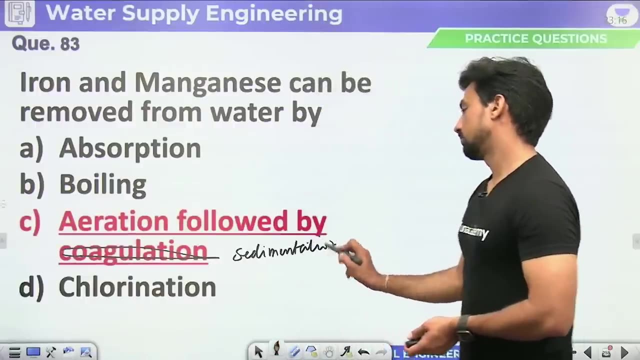 There is no option like sedimentation here. So coagulation is mentioned here. There should be a better word here: Sedimentation. There should be a better word here: Sedimentation. Next, If we talk about aeration, then for whom do we get aeration done? 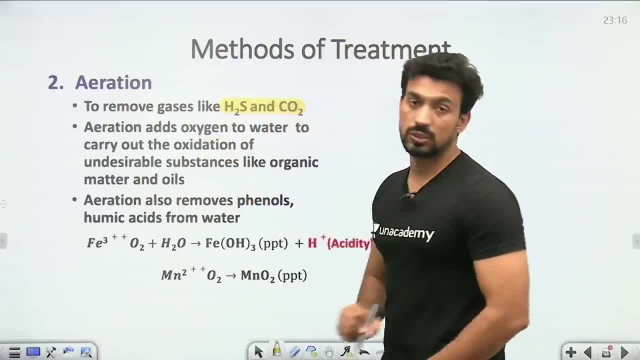 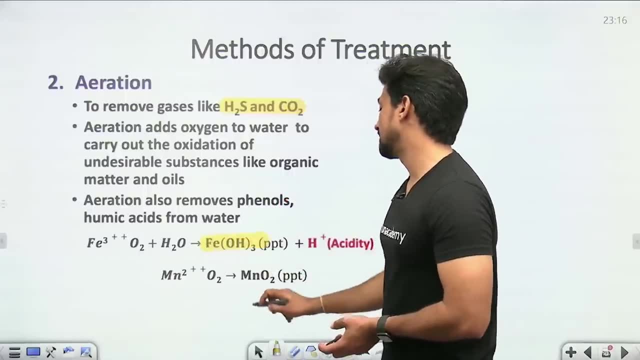 In the objective. the next question is asked to you. Let's get aeration done To remove gases like H2S and CO2.. Iron and manganese will also make a precipitate. The precipitate of iron hydroxide, The precipitate of MnO2 will be made. 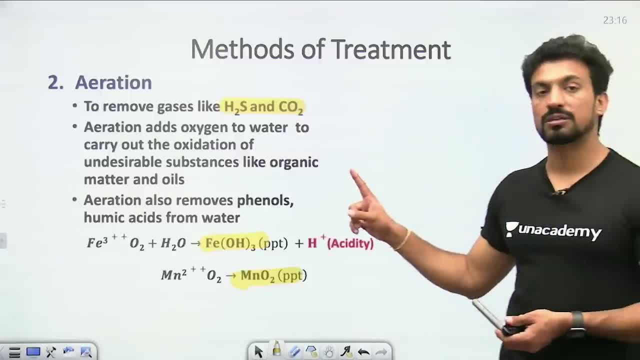 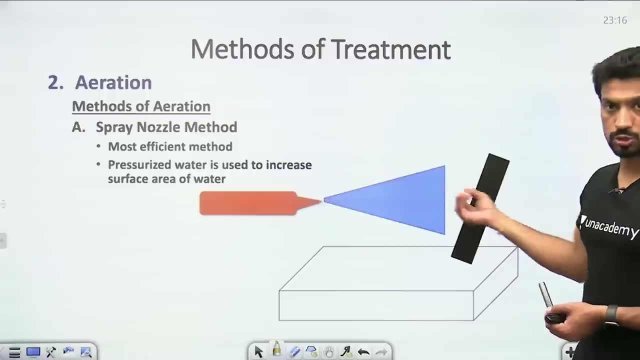 Which we can remove with the help of aeration, And later we will get it done. Sedimentation Aeration can be done by spray nozzle method. We will spray water on a screen. This is the most efficient method. Cascade can be an aerator. 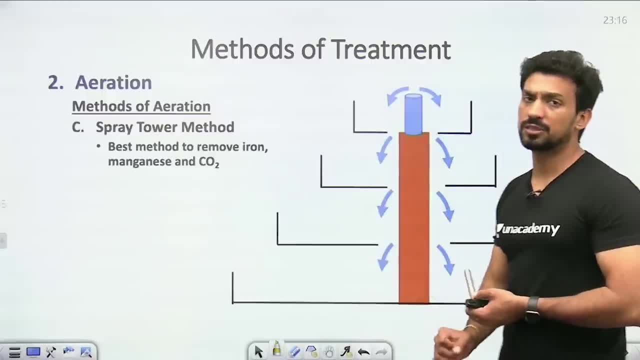 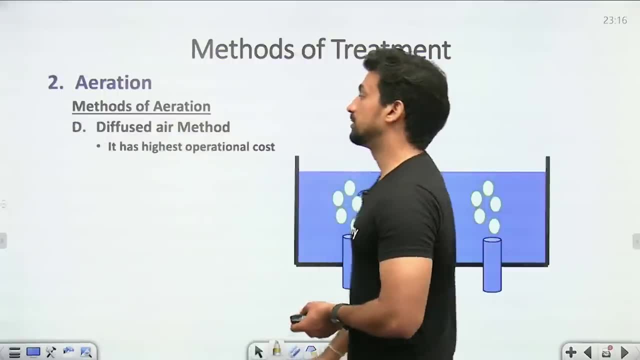 So its efficiency is about 40%. Spray tower method is the best method. It is the most efficient method But it is a little expensive. Best method to remove iron and manganese And CO2.. Diffused air method, Because here you have to diffuse electricity. 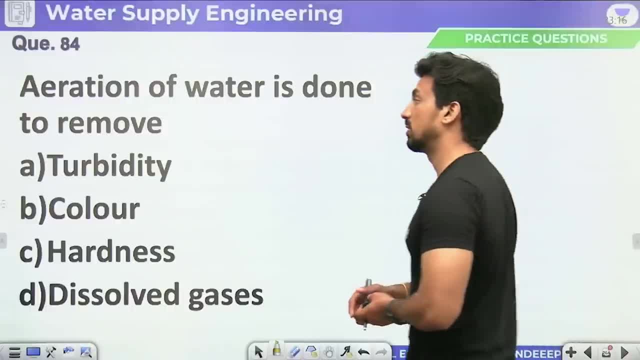 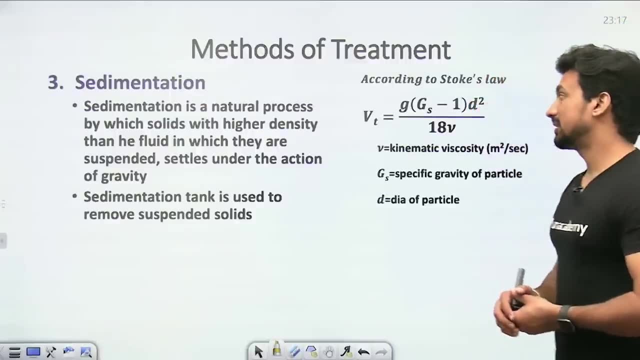 Here, bubbles will have to be diffused in the water. We are getting its aeration done, So its operational cost is high. Aeration of water is done To remove dissolved gases like H2S and carbon dioxide. What do we say in sedimentation? 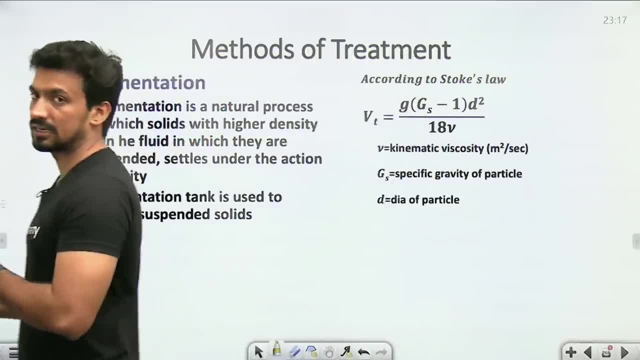 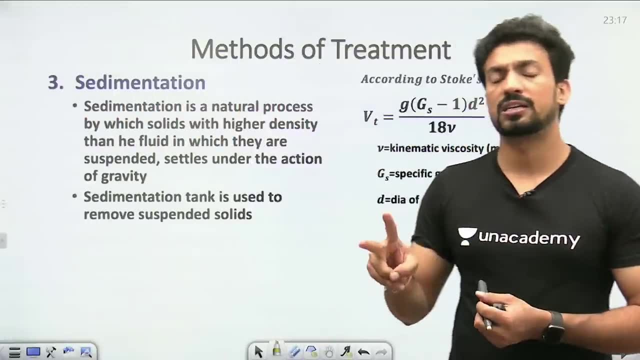 In sedimentation. we will say that Particles should settle due to gravity. Stokes law tells you that If particles are discreetly settling Settling of one particle, Settling of another particle, It is not disturbing According to Stokes law. 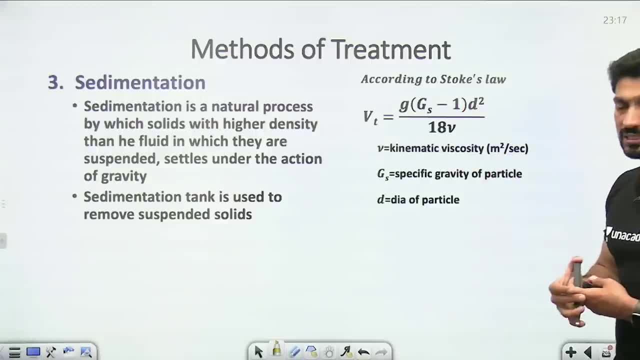 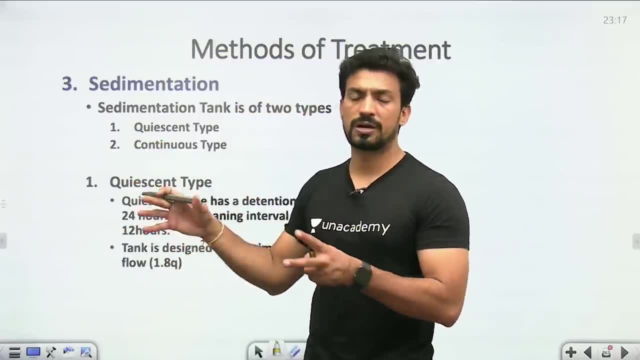 Gs-1 upon 18 mu into Gd2.. We can tell its terminal velocity Or settling velocity According to Stokes law. There can be two types of sedimentation tanks. One is of quiescent type. Water is filled in it. 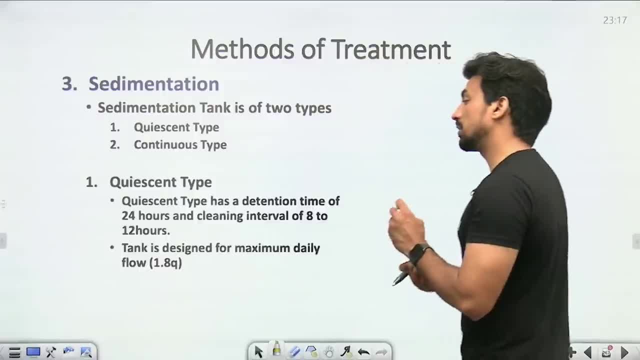 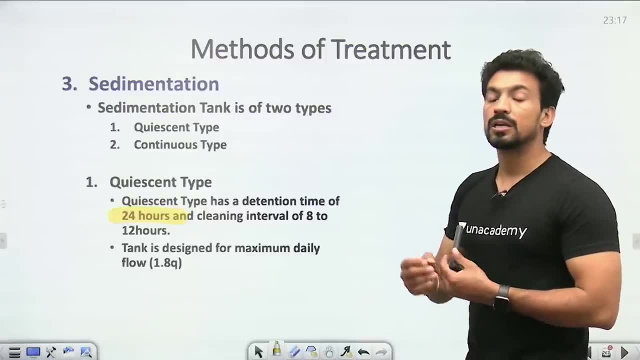 One is of moving type, Which will keep moving in the water. We will leave water in it for 24 hours, Detention time will be 24 hours And its cleaning will be done every 12 hours. This tank will be designed. 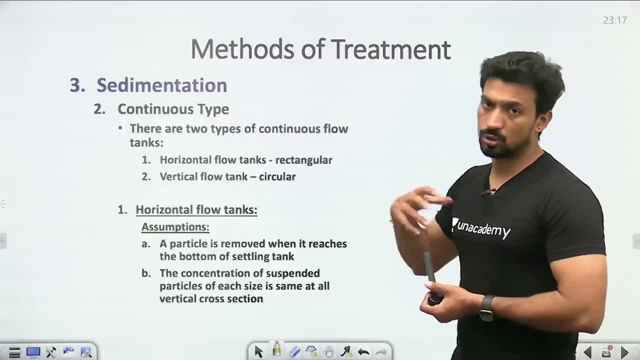 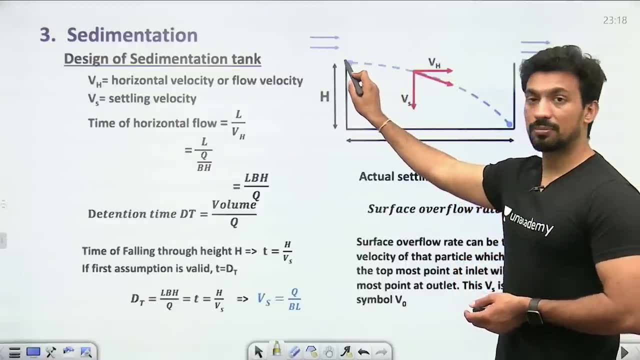 For maximum daily demand. If we talk about continuous type, Then horizontal flow tanks can also be there. Vertical flow tanks can also be there. What will be our assumption? Assumption will be that If water was flowing left to right, If water was flowing in this direction, 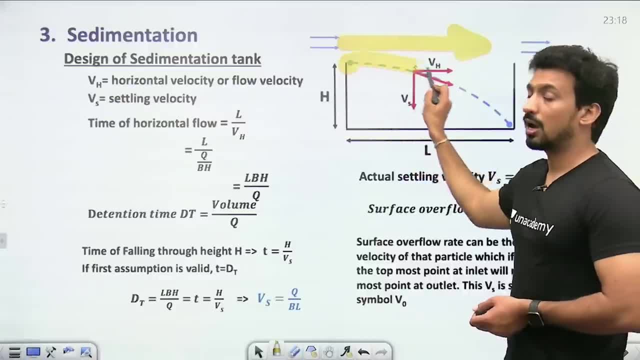 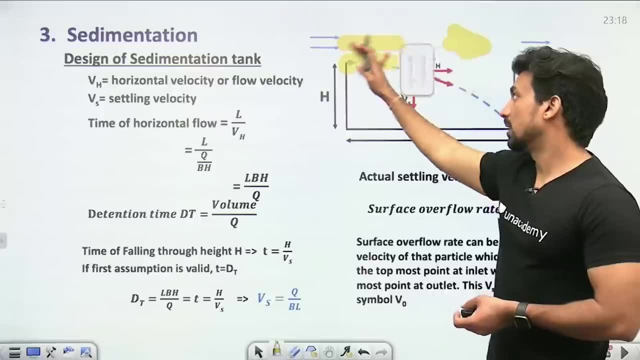 Then we will assume that A particle which was in the top of the tank Going to the outlet, Then only we will say This particle will be completely removed. All these particles will be completely removed. Now we have seen some small things in it. 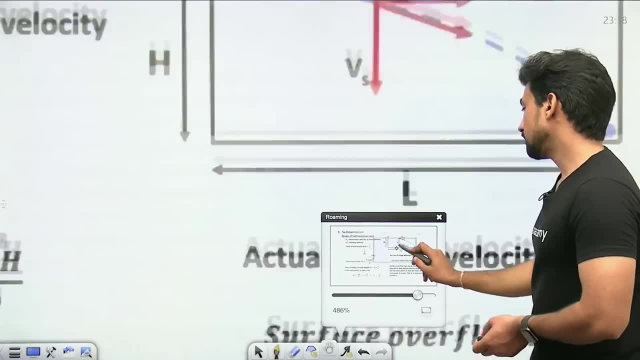 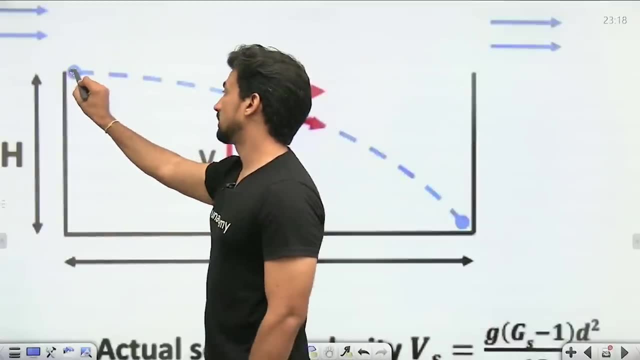 What we have seen in it. We have seen some small things in it. We have seen some small things in it. If any particle was at the top of the tank In the inlet, Then while reaching the outlet It came to the bottom of the tank. 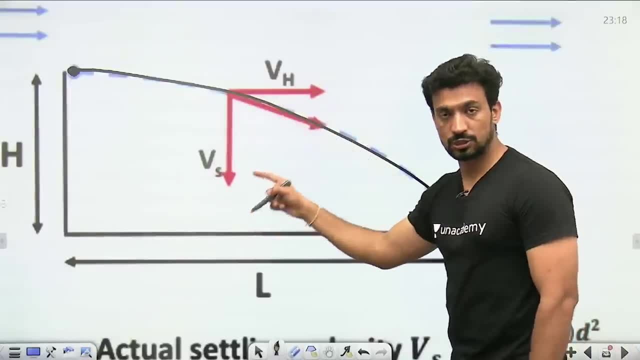 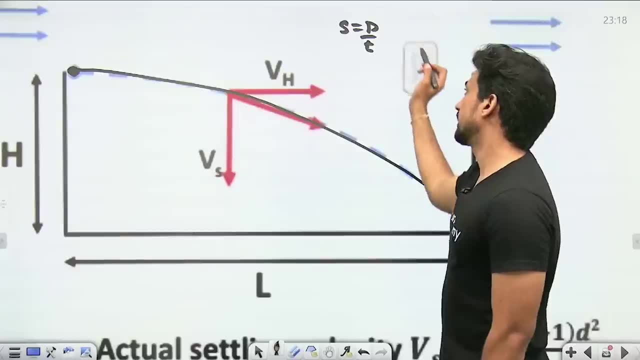 If it did so, Then it will have some horizontal velocity, Some vertical velocity. Remember those childhood days. So if I talk about time- Or I will say detention time here, So I will denote detention time with dt, It will be equal to. 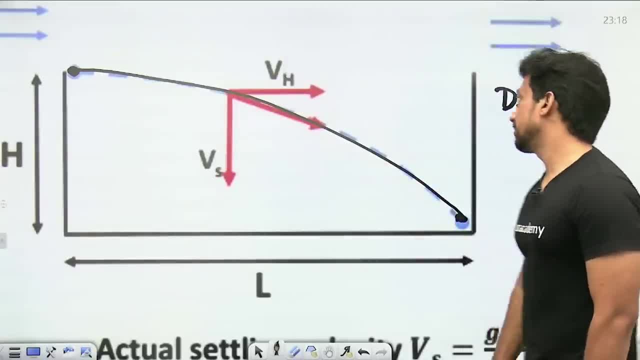 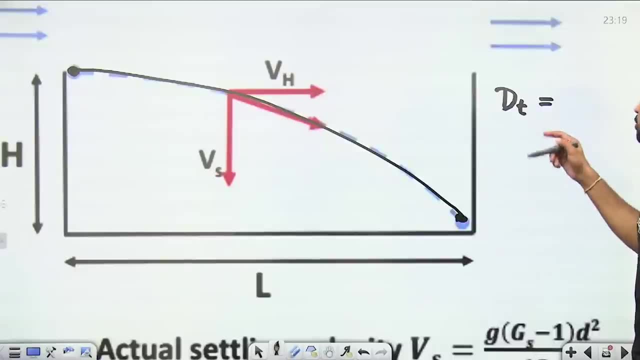 Distance upon speed, So time is equal to distance upon speed. Now, distance, If I talk about horizontal speed, Or we will call it flow velocity, So for that Time will be distance. How much distance did we travel L Upon? 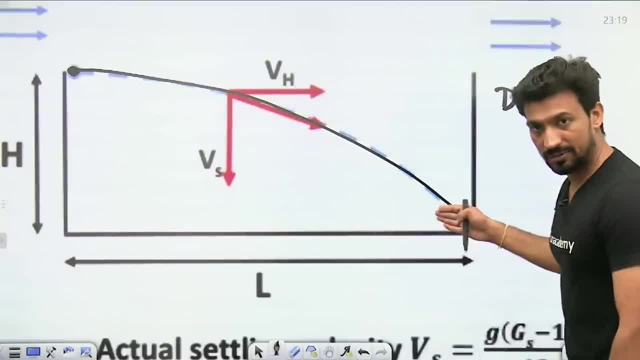 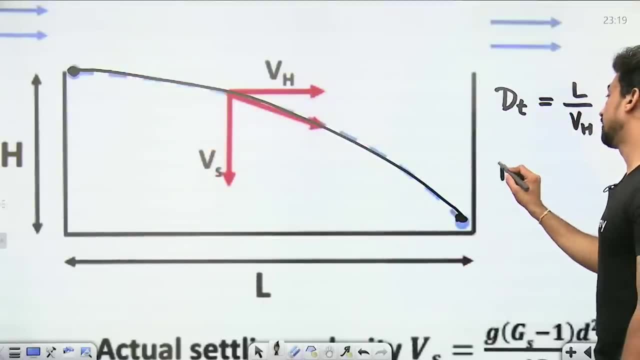 Vt. Now the time that the particle Travelled in the horizontal direction L distance. The same time the particle Travelled in the vertical distance H. So we can write the same detention time That this time it travelled distance H. 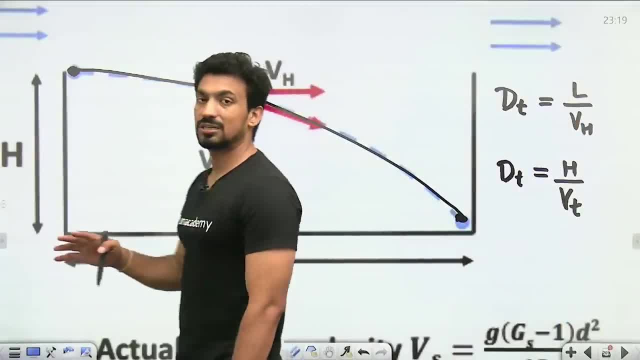 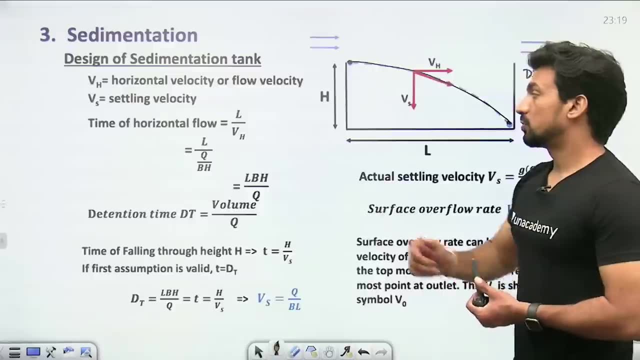 With Vt. We can equate these two. We will have a relation between them. We can also tell one more relation, Which will be between you: Time of horizontal flow, L upon Vh And Vh, The horizontal velocity that you will tell. 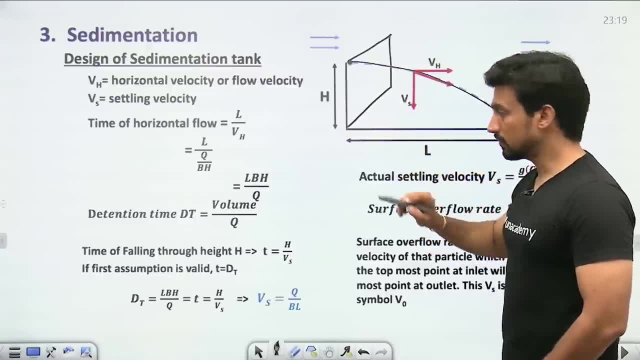 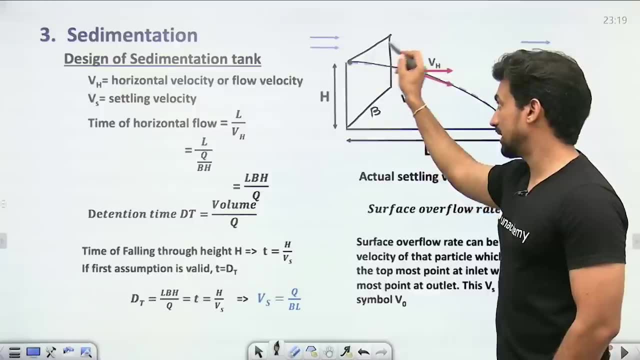 How will you tell the horizontal velocity That you saw this tank in 3D, So you have this L, This H And this width of the tank. So if we have to tell discharge, So which is the perpendicular velocity of this plane? 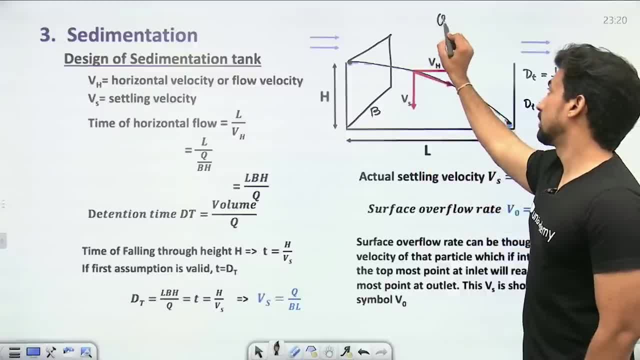 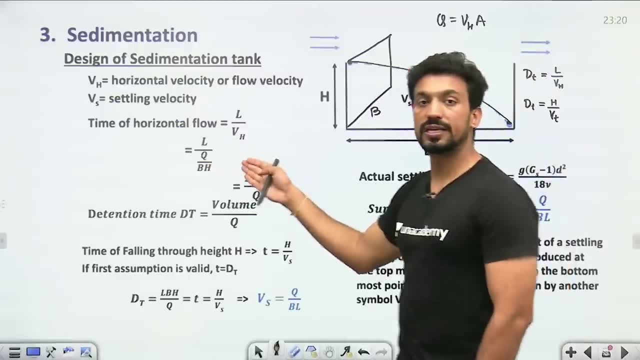 So you write Q equals to velocity into area. If you write Q is equal to velocity into area, So you can write Vh, Q by A, Which is the area of A, Which will be the area of B into H. So from here we have 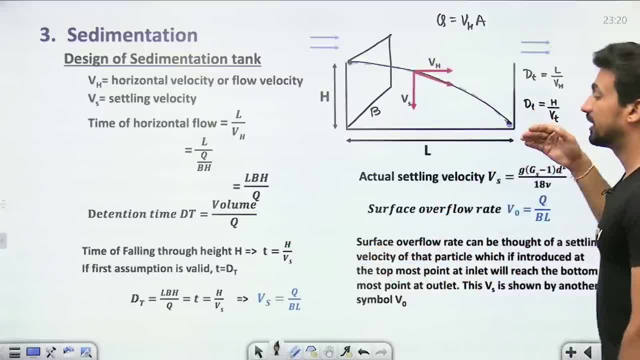 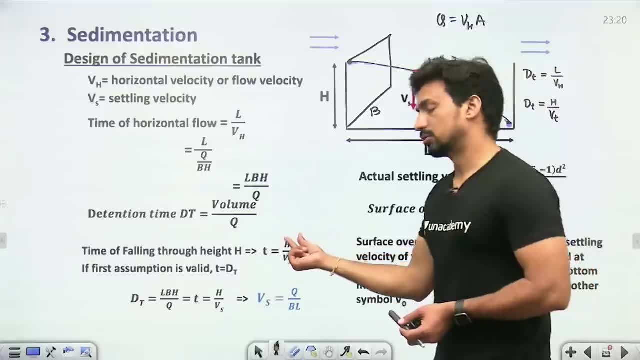 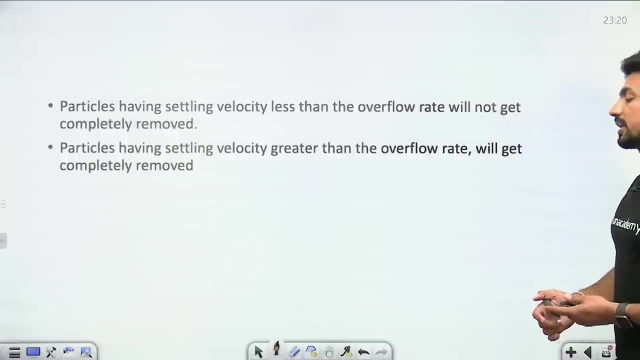 LBH upon Q, The value of time. You can calculate the same detention time In this way, In the way of H upon Vt Or with settling velocity, So the distance travelled in the vertical direction With the settling velocity Equate these two. 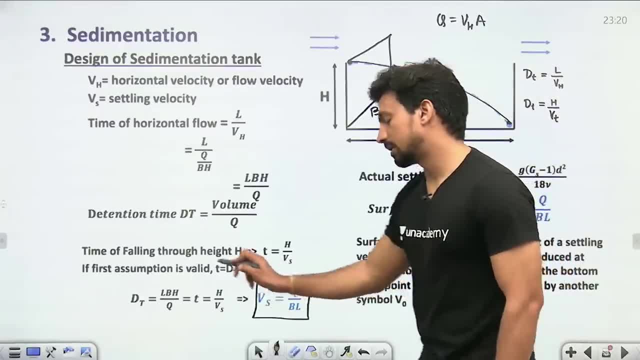 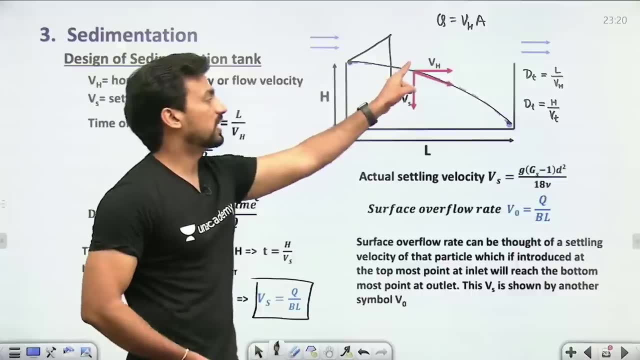 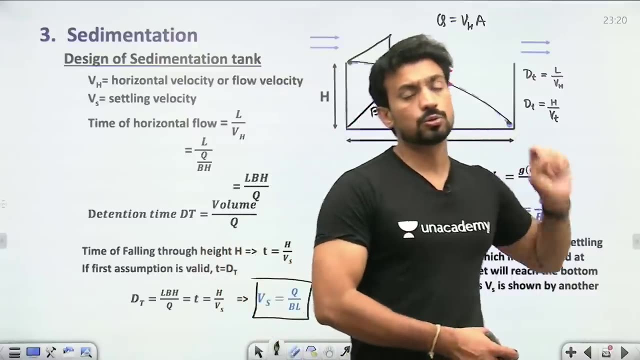 After equating these two, We have the expression That settling velocity is equal to That velocity, That velocity of the vertical direction, That settling velocity Due to which, If any particle was in the top of the tank, at the inlet, And reached the bottom of the tank, at the outlet, 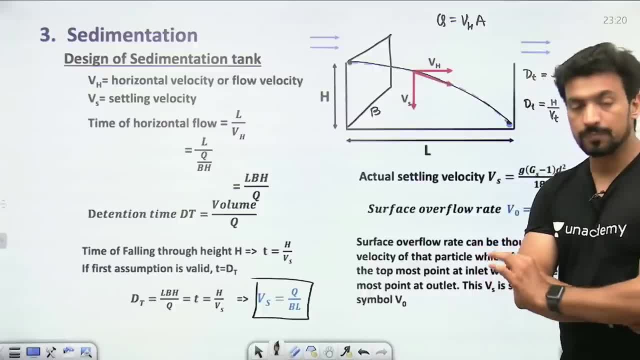 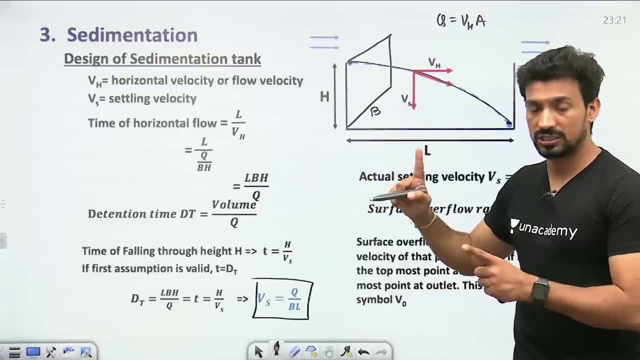 So that is called surface overflow rate And its formula is Q upon BL. If the velocity of any particle to settle Is very high, That surface overflow rate, That velocity Due to which it is settling, If it was in the top of the tank, at the inlet. 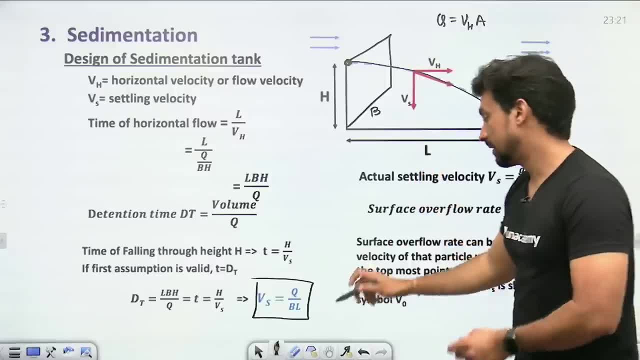 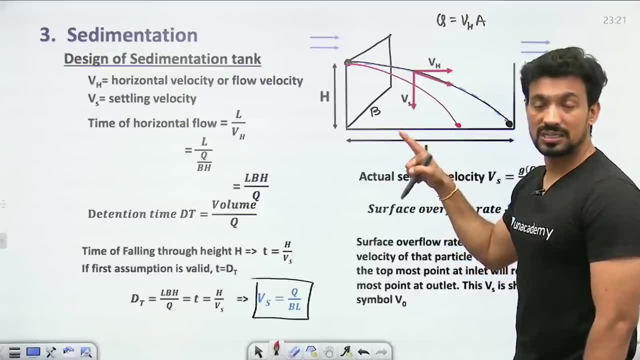 And reached the bottom of the tank at the outlet. Now, if there is any particle Whose settling velocity is high, If it is high, Then it will settle here. So if the settling velocity of any particle Is higher than the velocity of the surface overflow rate, 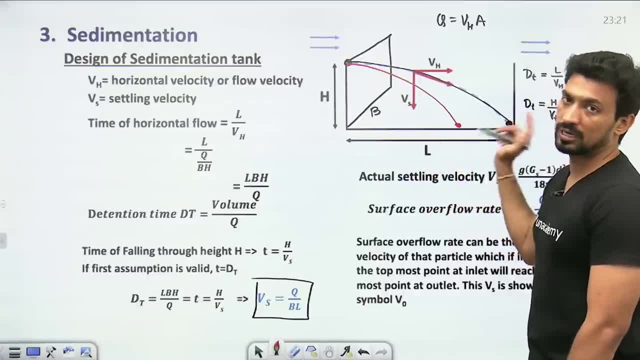 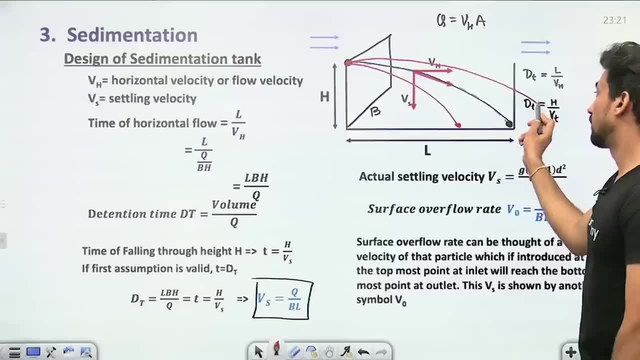 Then it means It is settling down quickly, So it will settle down earlier Means it will be removed 100%. If someone's settling velocity is low, Means it is not reaching the bottom of the tank, Then such particles Will not be removed 100%. 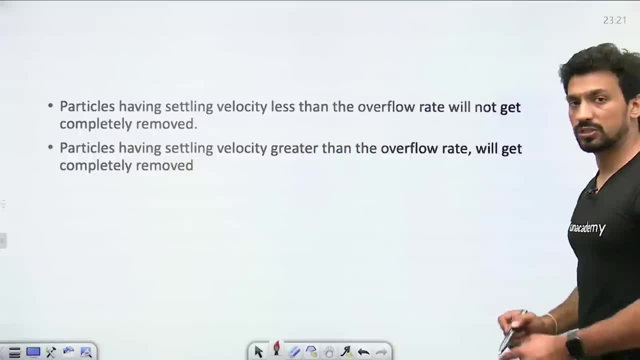 In this sedimentation tank. So this is the question asked. in: the objective, Particles having settling velocity Less than that of surface overflow rate Will not get completely removed. Those whose settling velocity Is less than V0. Will not be removed completely. 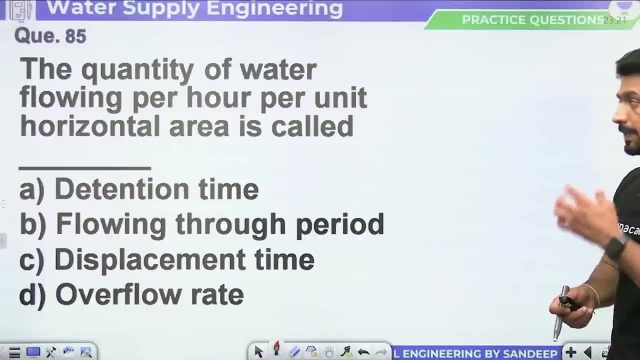 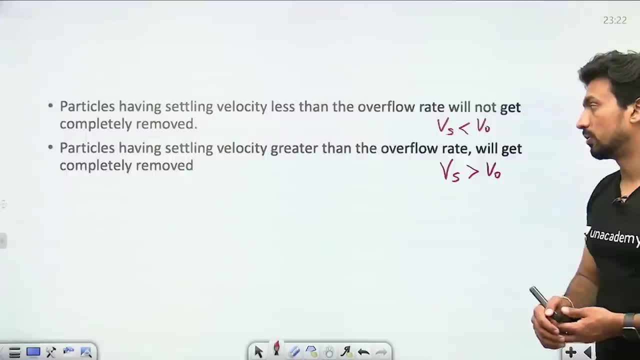 If their settling velocity is more than V0. Then they will be removed 100%. The quantity of water flowing per hour Per unit horizontal area Is called, as This is called overflow rate. See in the formula The quantity of water flowing. 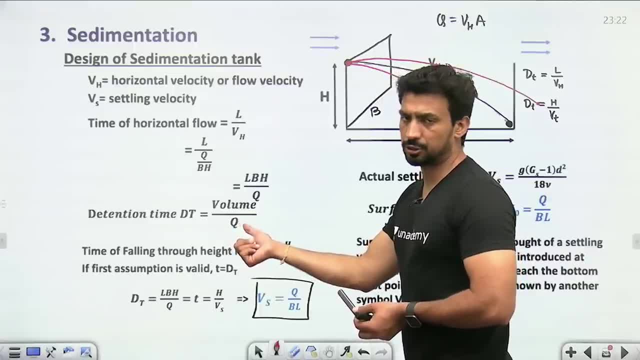 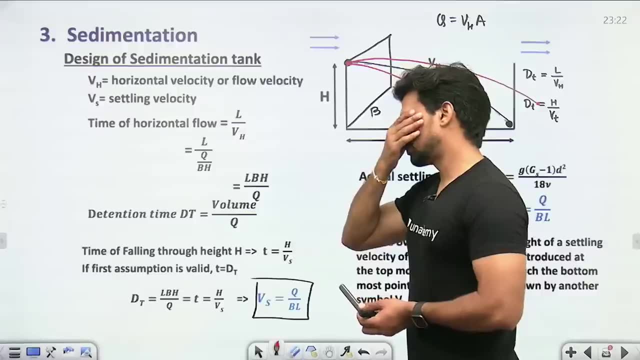 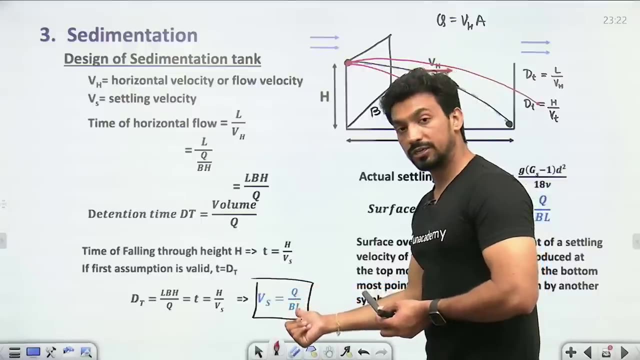 Per hour. per rate Means the discharge Is meter cube per second. So rate is below, Quantity of water is above. So what we call this, This is your detention time. Volume upon discharge. We are telling That surface overflow rate. 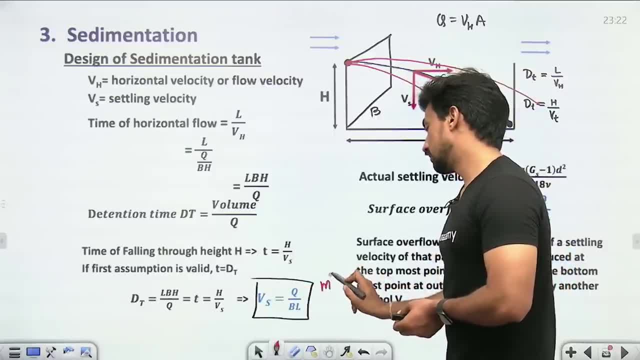 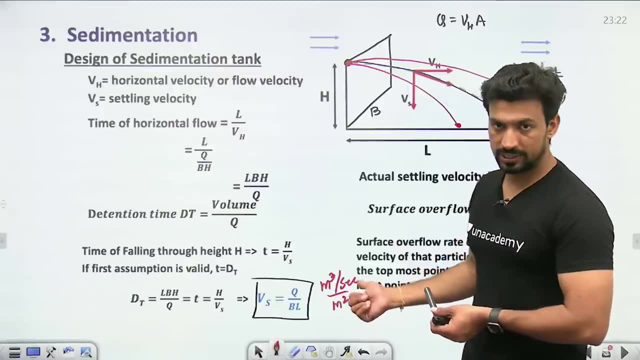 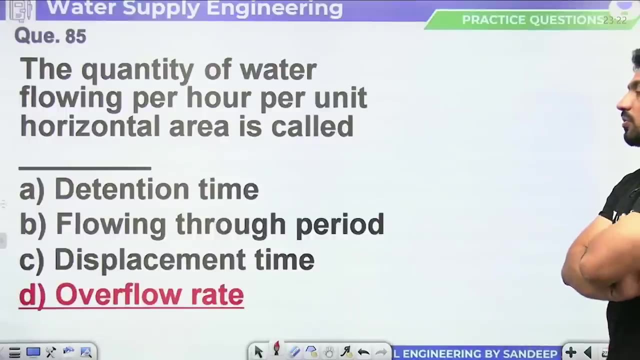 How much discharge per unit area Is flowing. So you will get Q unit Per meter square. So quantity of water Per unit time Per unit surface area, So meter cube per second Per meter square. This is called overflow rate. 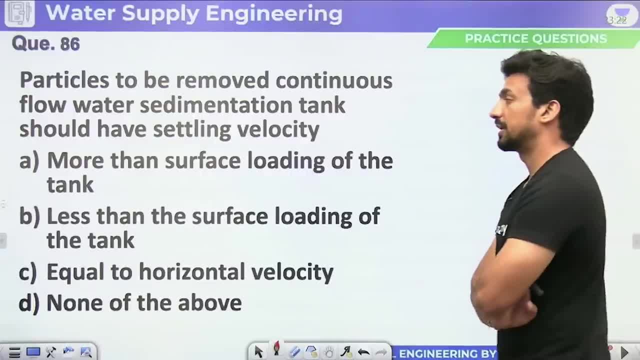 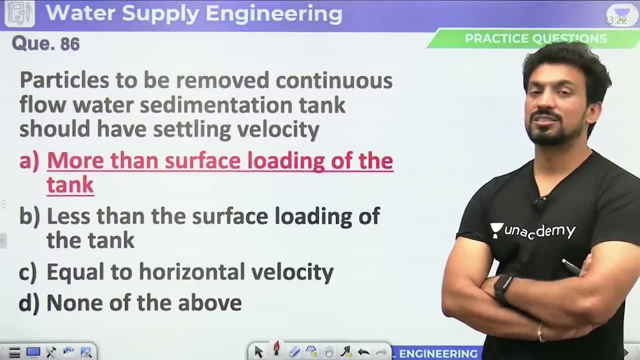 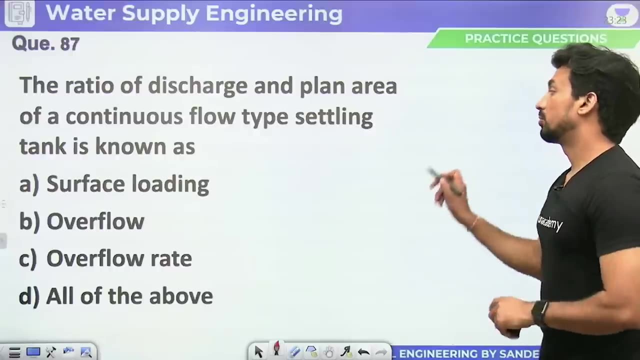 Particles to be removed. Continuous flow of water sedimentation tank Should have settling velocity More than the surface loading rate. What is surface loading rate, What is overflow rate Or what is critical settling velocity? What is critical settling velocity? Discharge and plan area. 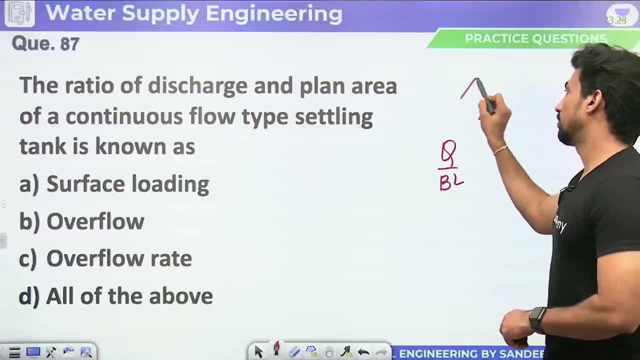 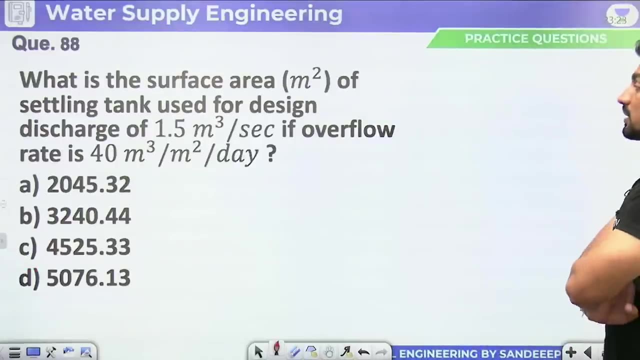 So Q upon B L, Q upon B L. Plan area means top area, This is B, This is L And this is B. So Q upon B L. This is surface loading, Overflow or overflow rate. What is the surface area of settling tank? 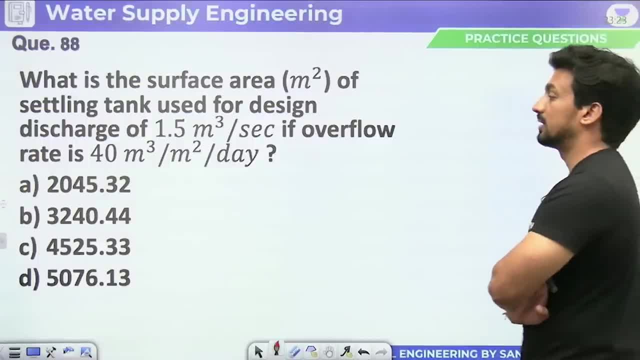 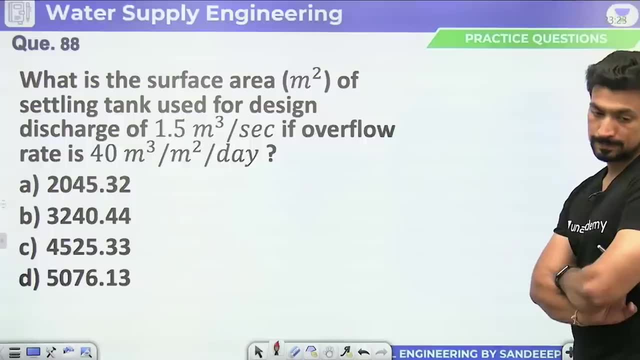 Used for design discharge Of 1.5 meter cube per second. If overflow rate is 40 meter cube Per meter square per day, We draw surface area as line Rectangle like this, This one we will draw Now. I will show you. 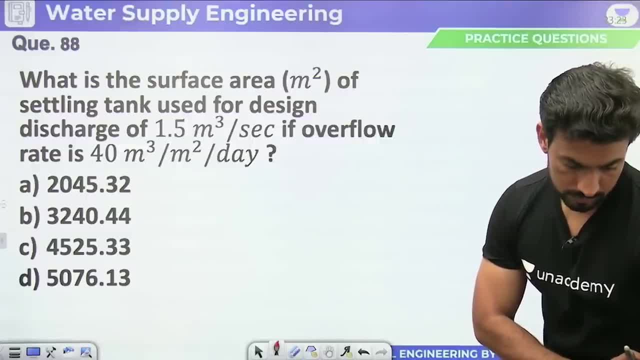 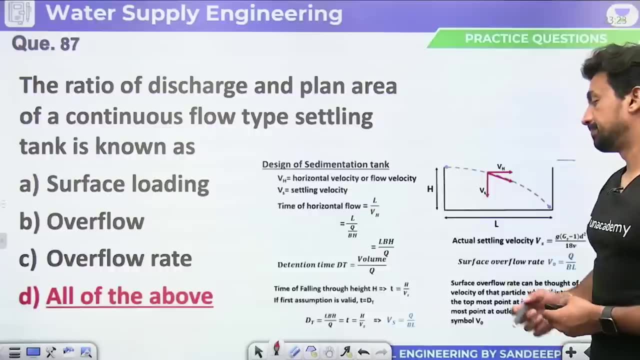 How to calculate the flow rate of the surface over flow. You can write down in the description. This is the flow rate. What is the surface area of settling tank? Value of V naught, V naught, Q upon B. L Depictive of the surface area. 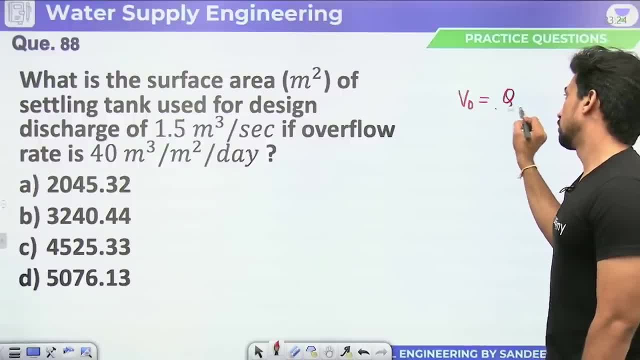 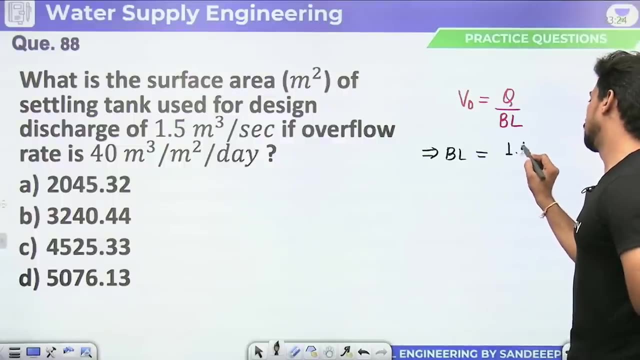 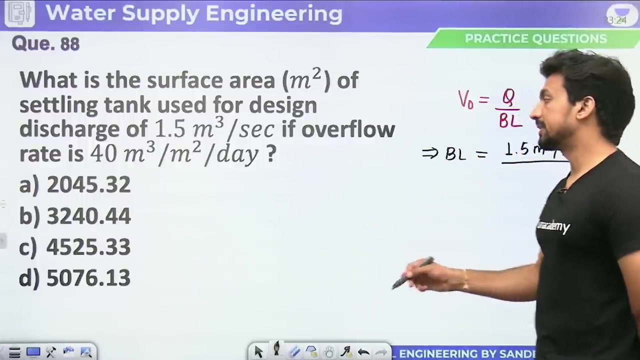 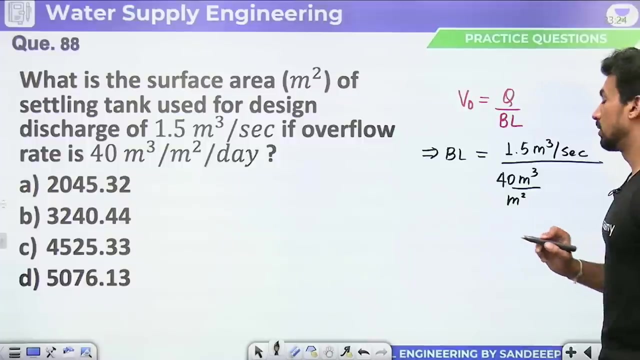 And this is the current flow rate. We will write down upon BL. What is the surface area? We have to tell the value of BL. Q0. Discharge: 1.5 m3 per second Surface overflow rate: V0.. 40 m3 per m2 per day. Now I will tell per day. 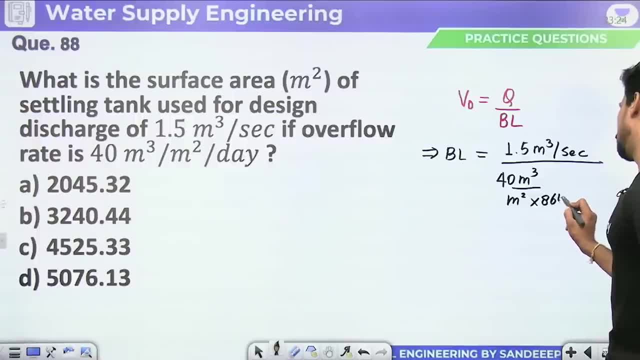 what I can write here. As our influencers have told that in a day we have 864.00 seconds, We will take 864.00 up. m3, m3. cancel second, This second cancel: 1.5 into 1.5, into 1.5, into 1.5.. 3 to 4: 0.. 3 to 4: 0 m2.. 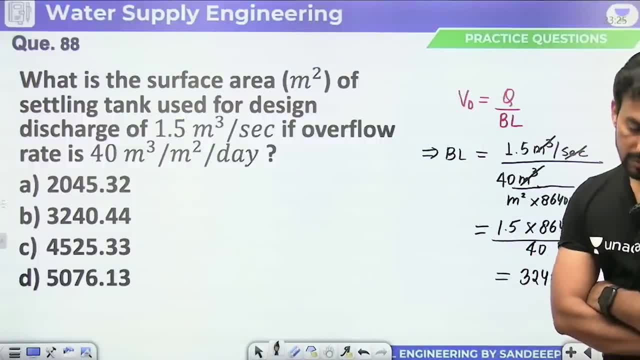 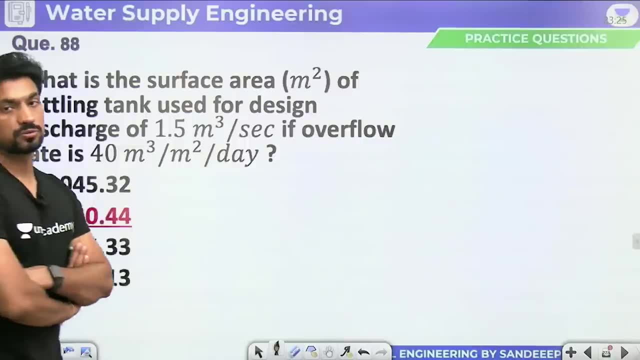 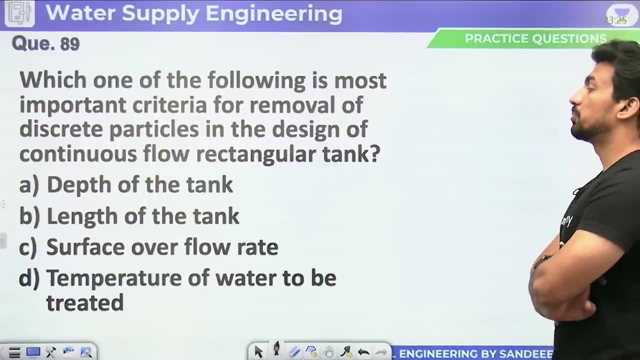 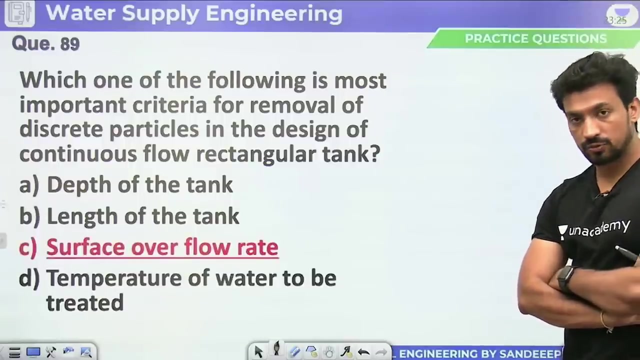 How long is the detention time? How long are you allowing it? Next, Which one of the following is most important criteria for the removal of discrete particle in the design of continuous flow rectangular tank? So the most important criteria is surface overflow rate, Or let's say that settling velocity, due to which, if any particle is stopped, 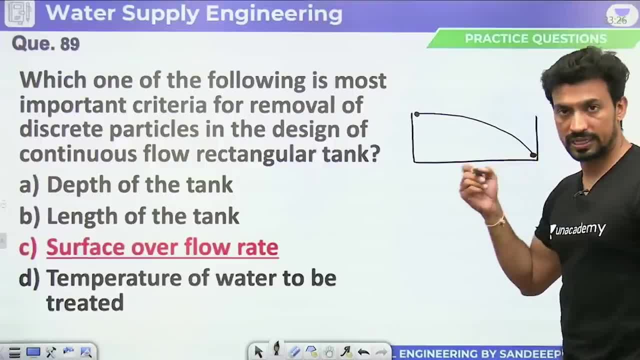 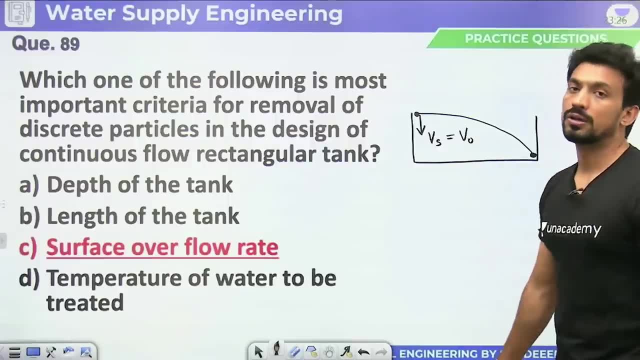 at the top of the tank, then it reaches the bottom of the tank while going to the outlet. So the settling velocity in the vertical direction of such a particle is called surface overflow rate. Some important data related to sedimentation: tank: Plain sedimentation. Plain sedimentation. 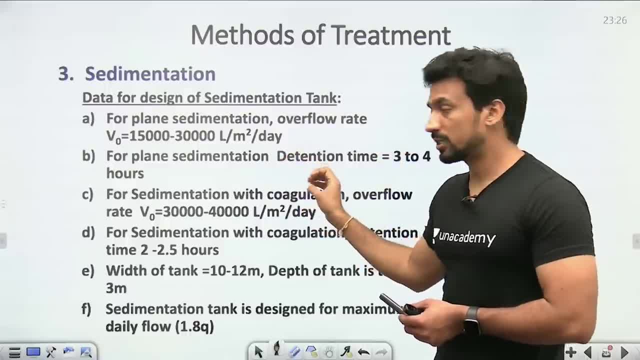 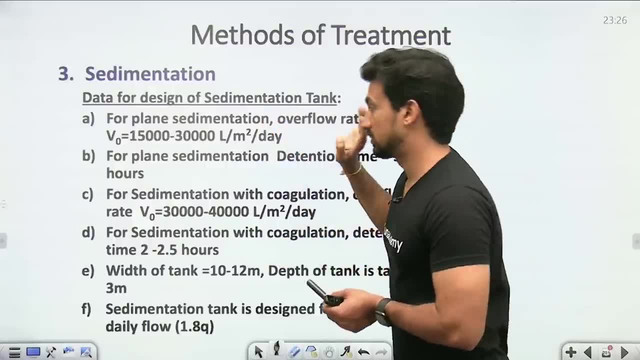 means that you have not added any coagulant or anything in it. So in that case, from 15,000 to 30,000 liters in 1 m2 area in a day. so much water can be sedimented In. 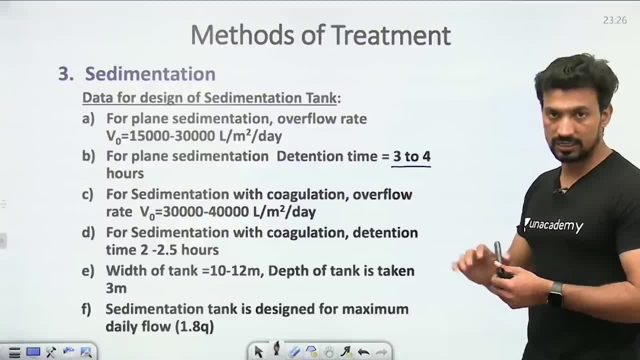 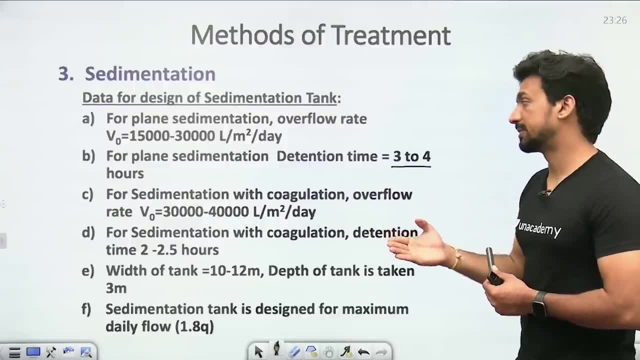 a day. it will take 3-4 hours For plain sedimentation. the detention time is 3-4 hours. For sedimentation with coagulation, if any coagulant is added then the value of V0 will increase. It will. 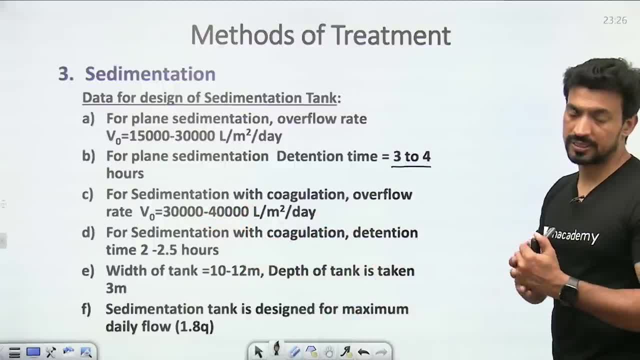 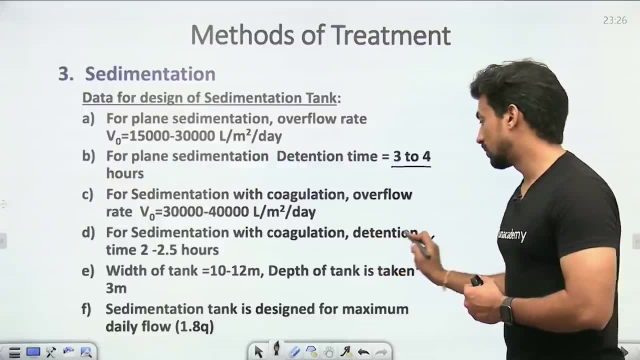 be from 30,000 to 40,000 liters per m2 per day And the time required to do sedimentation will be 2-2.5 hours. This is asked in the objective in the state exams. Let's consider the width of the tank: from 10 to 12 meters, The depth of the tank is 3 meters. Let's design the sedimentation tank: Maximum 2.5 to 3 meters. The depth of the tank is 3 meters. Let's consider the width of the tank from 10 to 12 meters, The depth of 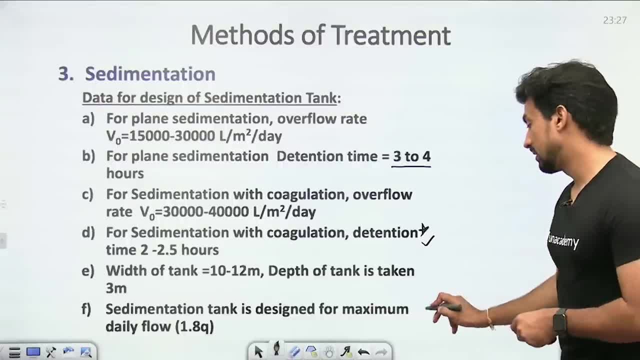 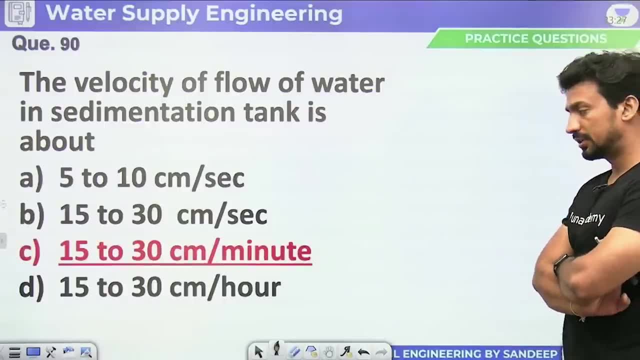 the tank is 3 meters, The length of the tank is 4 meter and that entire length of the tank is 4 meter. Let's consider the depth of the level of the sedimentation tank. Let's carefully düş 전� agriculture, or the way they design these tanks, The fact that 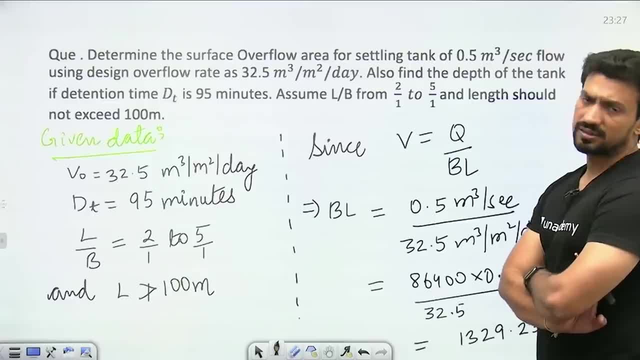 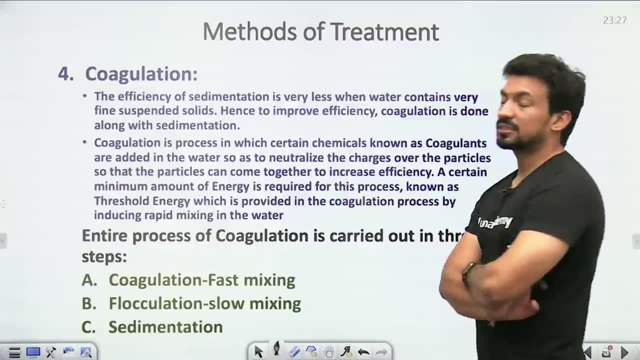 the level of industry design is 15 to 1 m2 per minute is the regular number of sites. whichback If we go further, we can see that the design of the tank is less important than the objective point of view, that we don't need to read it. 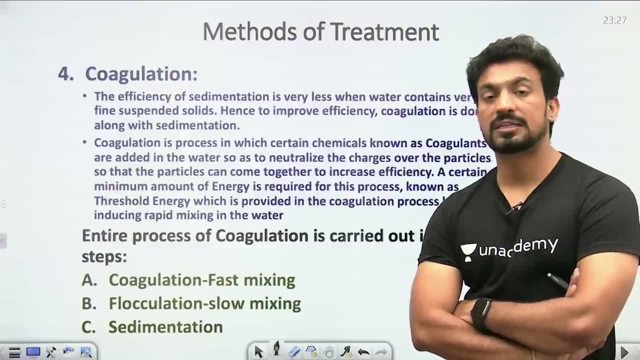 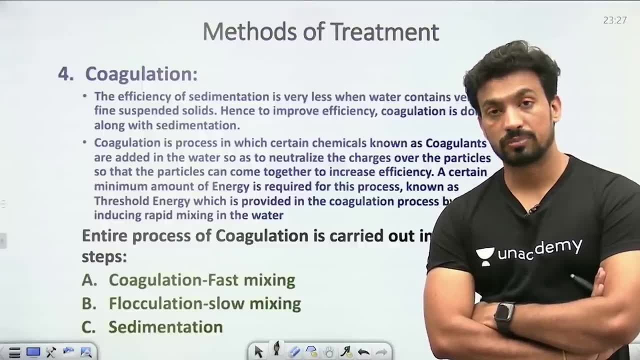 before the exam. and that's not the essence of Under-resolution. By adding coagulant, the charges of the particles will be neutralized. Now that coagulant reaches all the particles quickly, It is important that we mix it quickly. We will do fast mixing when you have to mix coagulants. 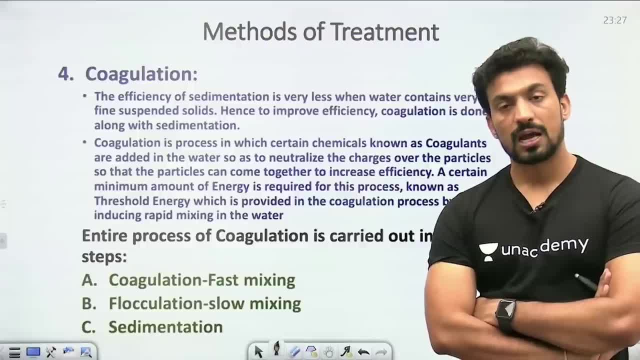 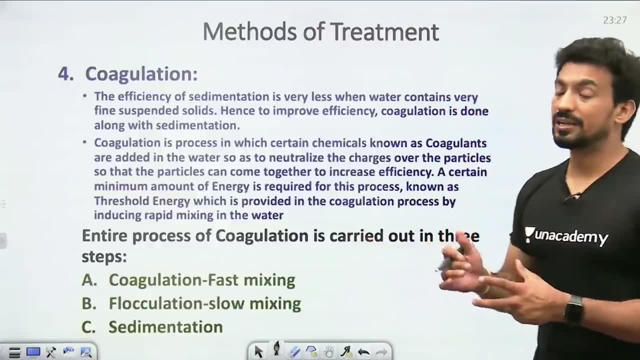 After that, when the charges have been neutralized, now we have to increase the contact time of those particles So that they come around, come in contact with each other's particles, Make a group or make flocks. So when they make a group or make flocks, 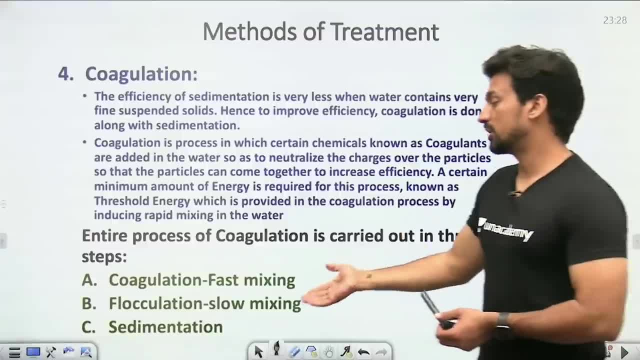 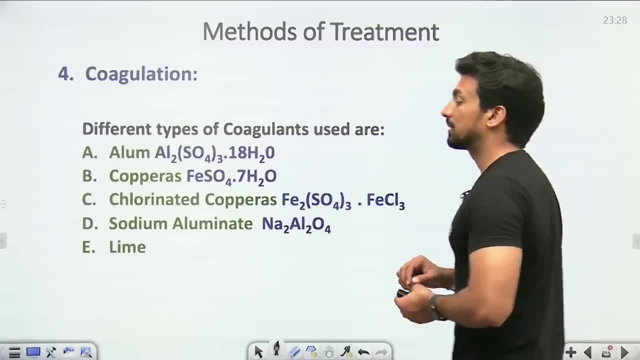 we will do slow mixing to increase the contact time. So there is slow mixing in flocculation. Then we will allow them to settle Or we will send it to filters later. So alum, copperas, chlorinated copperas, sodium, aluminate lime. 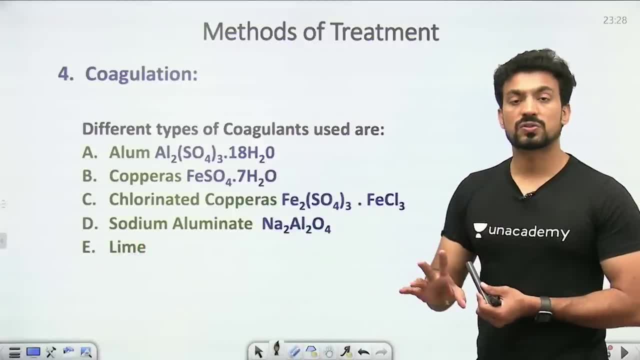 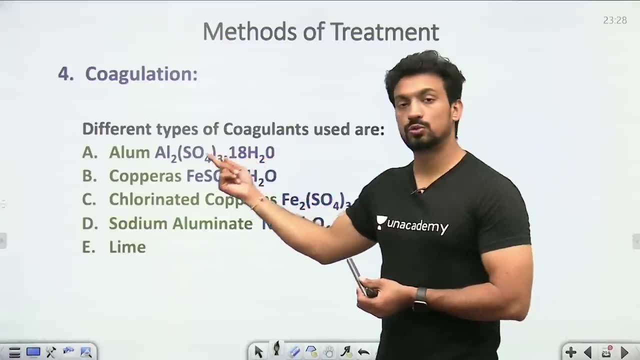 they are used as coagulants. Which out of the following is coagulant? So you should be able to identify that. any of these names will be visible. It is coagulant. Aluminium sulfate dot 18. H2O is alum. 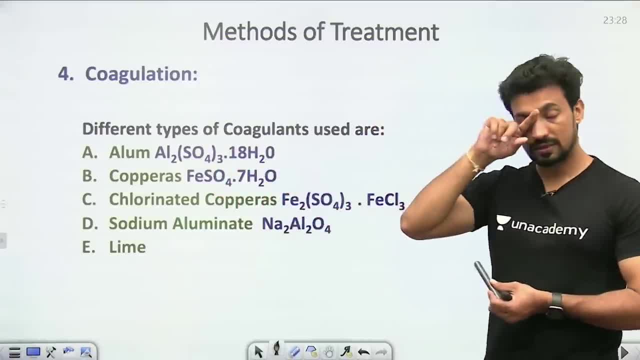 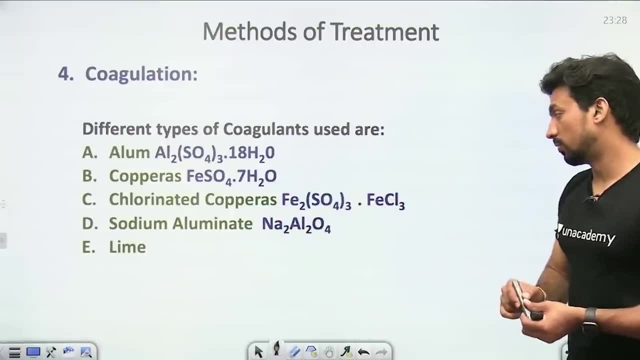 Formula can also be asked in the objective. Copperas: ferrous sulfate dot 7- H2O. is there? Chlorinated sulfate, dot 18- H2O. is there? In coagulant copperas FeCl3 will come. You have sodium aluminate, Na2Al2O4 and lime. 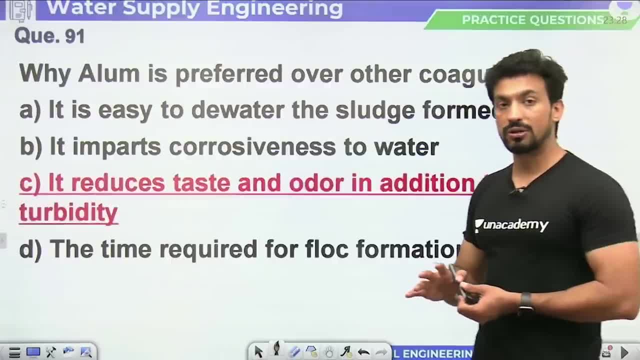 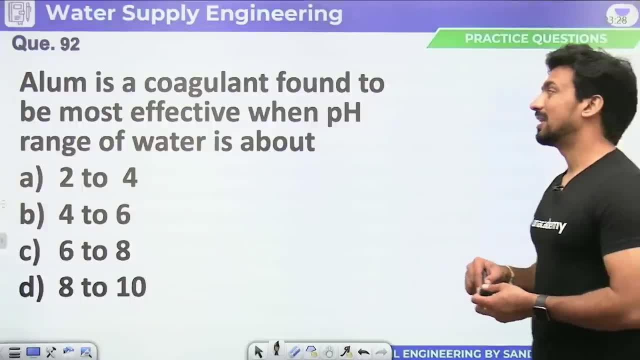 Why alum is preferred over all other coagulants? Because it removes the taste and the order, In addition to turbidity, Alum is coagulant found to be most effective. It is most effective in the alkaline range Between 6 to 8.. 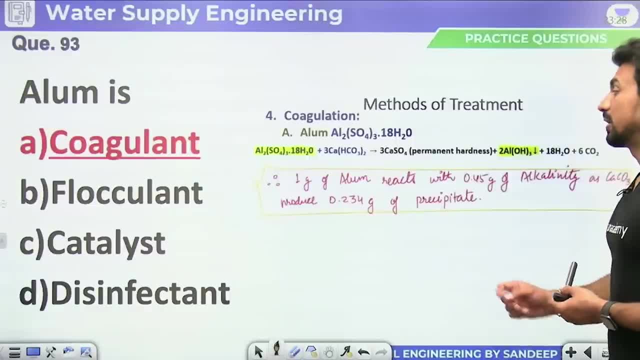 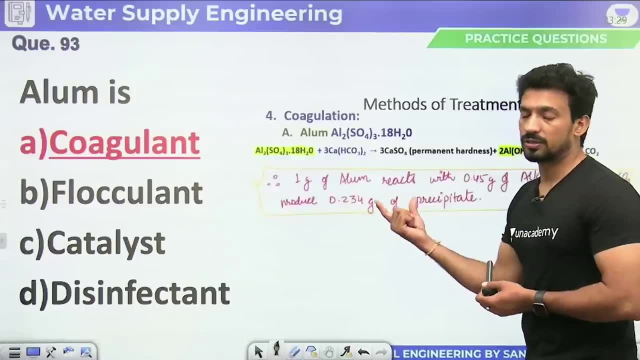 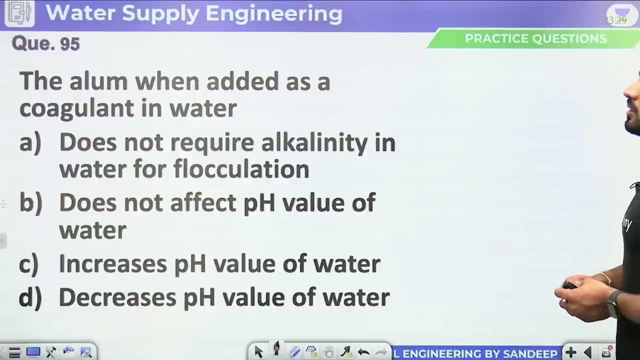 Alum is a coagulant And alum reacts. 1 gram of alum To produce 0.234 gram of precipitate. Why alum is preferred, The alum when added as coagulant in water. If alum will be added with coagulant, Aluminium sulfate dot 18 H2O. When calcium bicarbonate is present in the presence of alkalinity, Calcium sulfate produces permanent hardness And also produces 6 CO2.. Due to which further acidity also comes. Due to 6 CO2, acidity also comes. 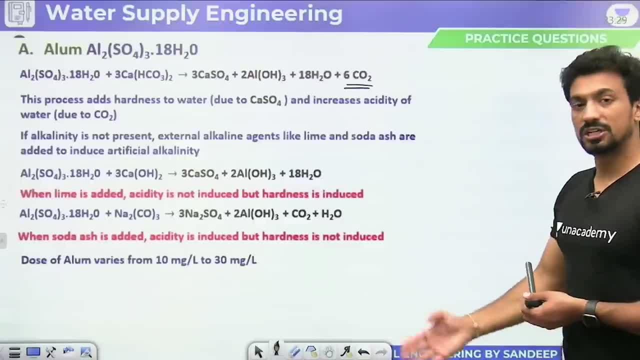 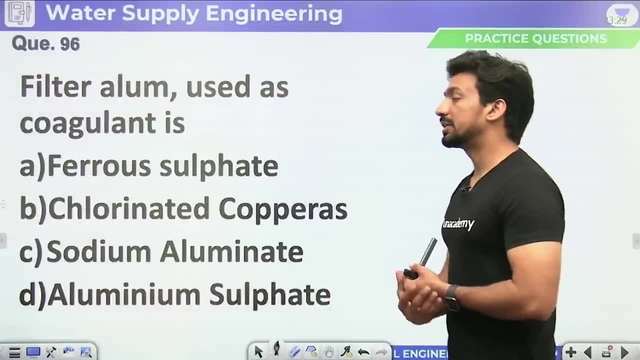 So will anything happen in it related to acidity or pH? To reduce pH means to increase acidity, So our answer will be: Decreases the pH value of water Filter. alum used as coagulant. So what happens? Aluminium, sulfate, dot 18, H2O- happens. 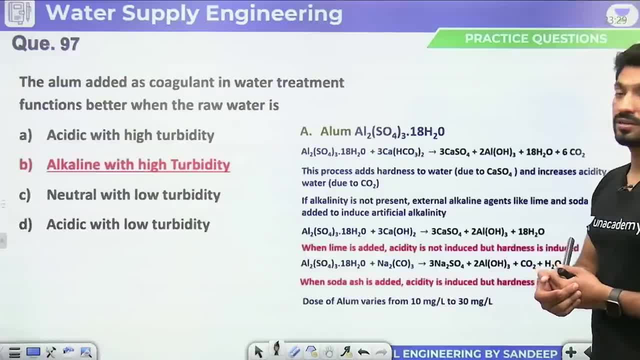 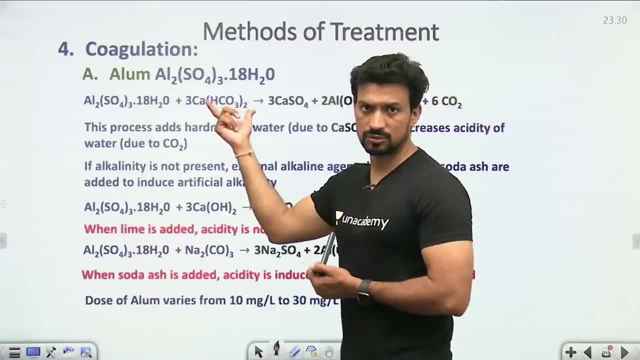 The alum added as coagulant in water treatment functions better When the raw water is alkaline, with high turbidity. Now the alum that reacted With calcium bicarbonate. It produced here Calcium sulfate, which is permanent hardness, And carbon dioxide, which introduces acidity. 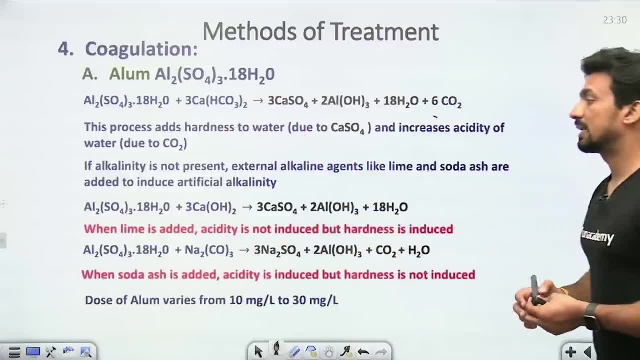 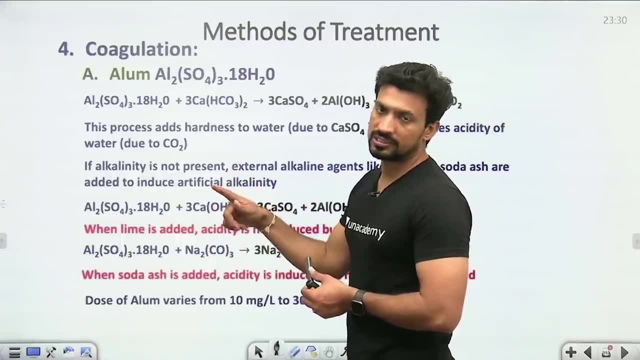 If alkalinity is not present. So you can add external alkaline agents Like lime or soda. If lime was added, Means CAO was added. It became calcium hydroxide in water, So 3 CAOH whole. twice. So from here. 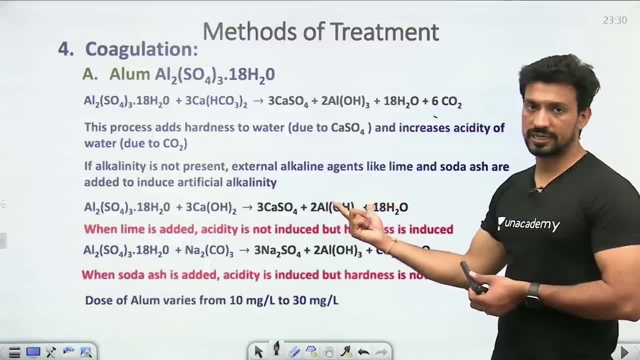 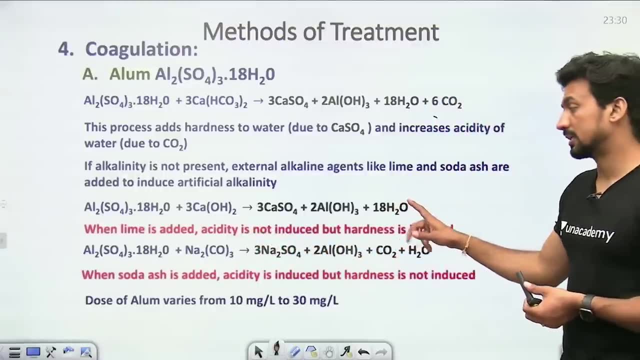 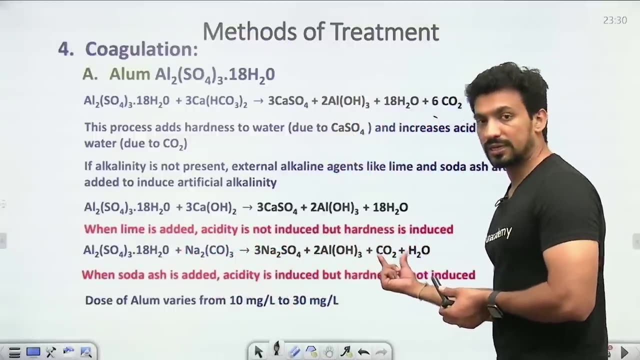 Calcium sulfate and aluminum hydroxide precipitated. So when we add lime, So acidity is not introduced, But permanent hardness is introduced here. When we add soda ash Means, you added sodium carbonate, So this forms carbon dioxide Means. when we add soda ash, 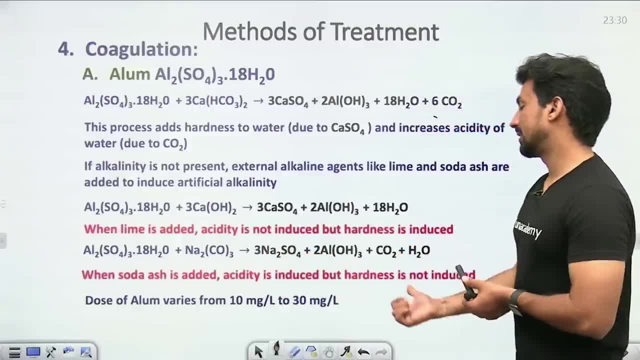 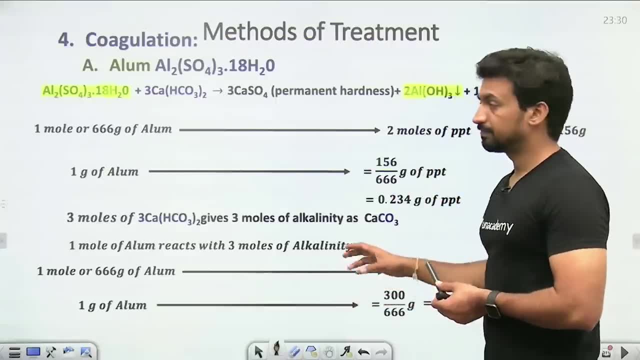 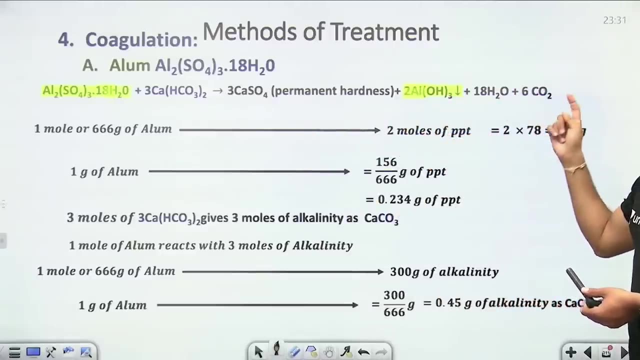 With alum. So acidity will be introduced But hardness will not be introduced In their reactions. If we see, 1 mol of alum means 666 gm of alum reacted To make 2 mol of precipitate. If we talk about 1 gm of alum, 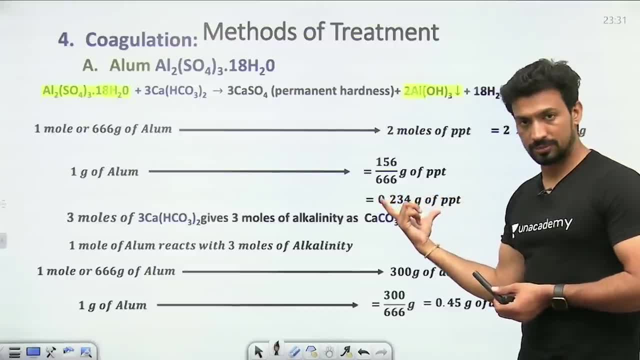 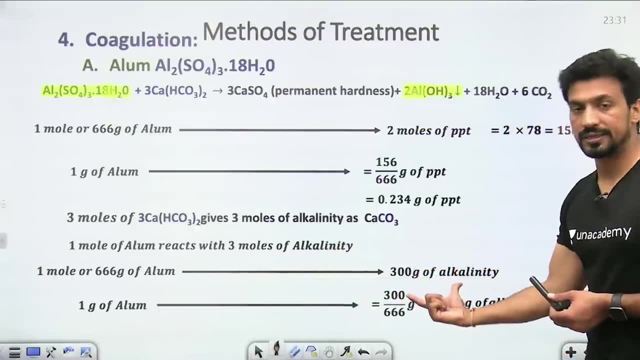 So 0.234 gm of precipitate was made In the same way, 1 mol and 666 gm of alum Is reacting with 300 gm of alkalinity, Or you can say If 1 gm of alum is there. 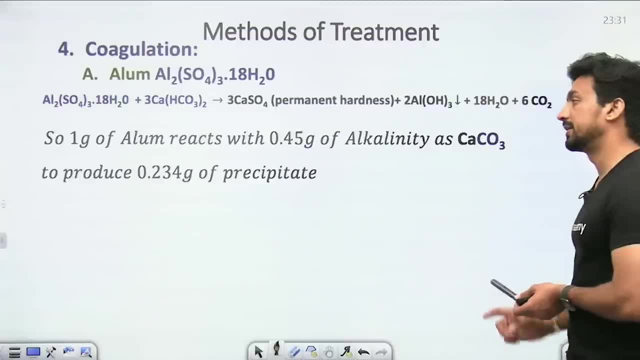 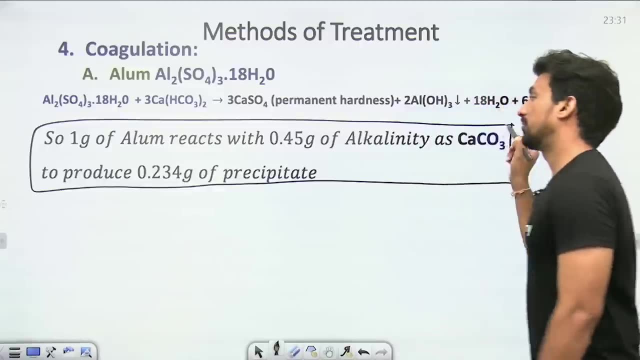 Then 0.45 gm of alkalinity. So the point is 1 gm of alum, 1 gm of alum, Reacts with 0.4 gm of alkalinity As calcium carbonate To produce 0.234 gm of precipitate. 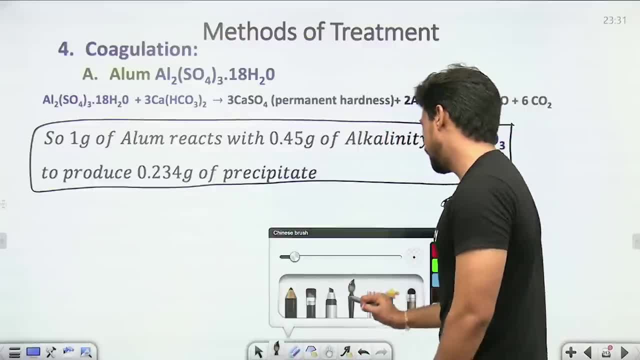 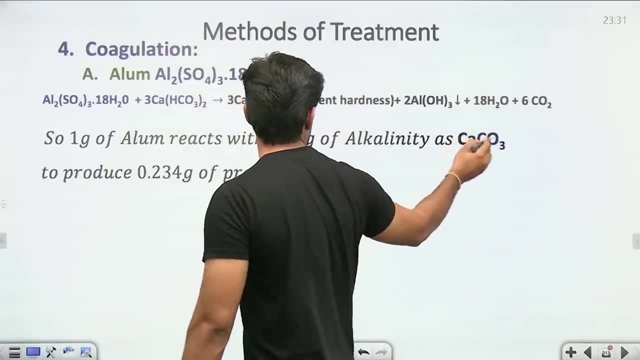 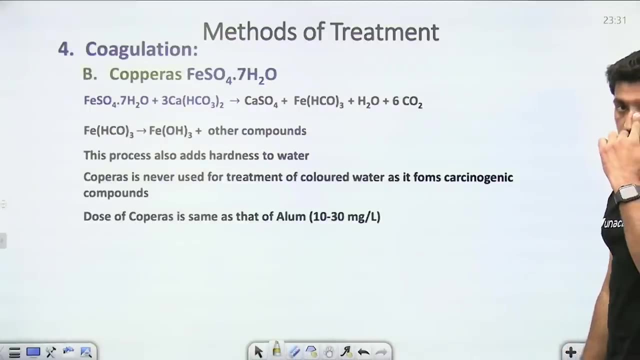 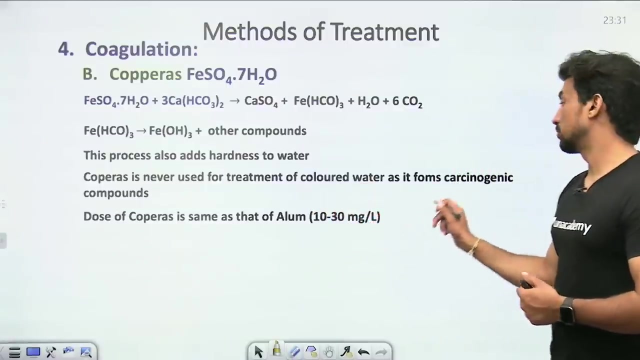 Remember this statement In the objective. If you are asked, Then you should know this statement. Next, let's move on. If we talk about copperas, So copperas Is used in water. It is never used in colored water Because it forms carcinogenic compounds. 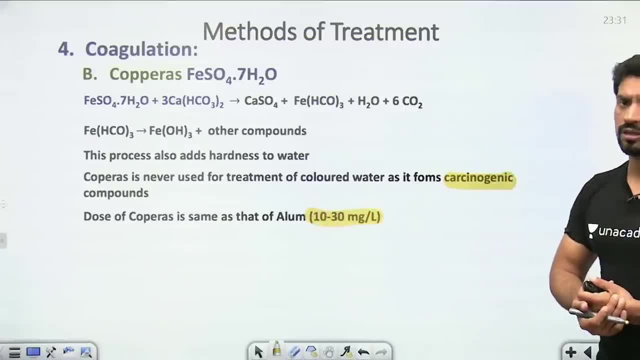 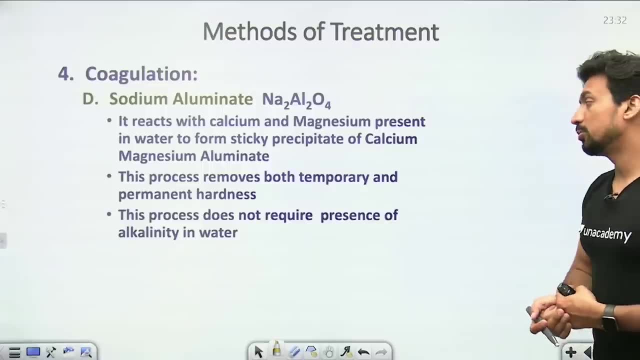 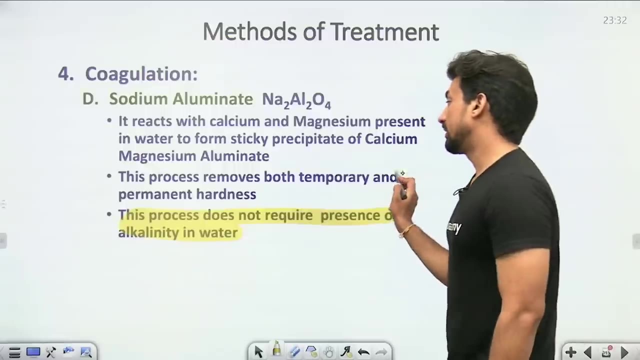 Its dose is also equal to 10-30 mg per liter Clorinated copperas In this Chlorine is also added. The special thing about sodium aluminate Is that There is no need of alkalinity presence To work. 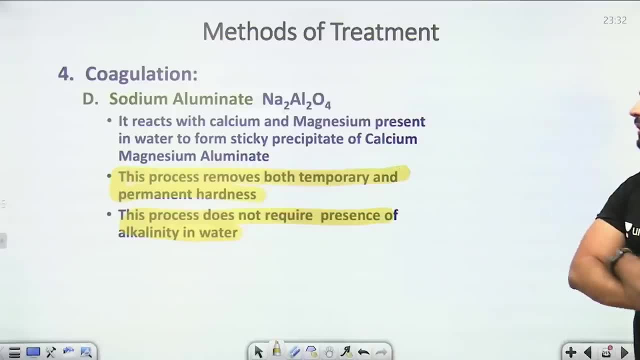 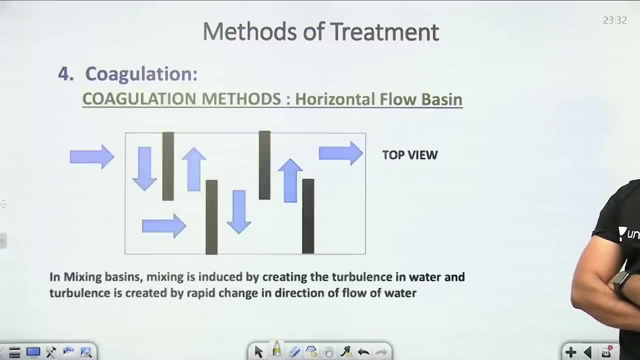 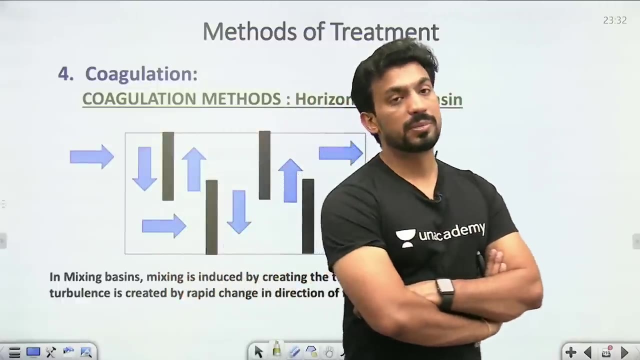 And it removes Temporary and permanent hardness. And with this, Calcium and magnesium react And make sticky precipitate And they will settle down. Next comes the mixing process, Or coagulation process. Coagulant added, So you mixed it. 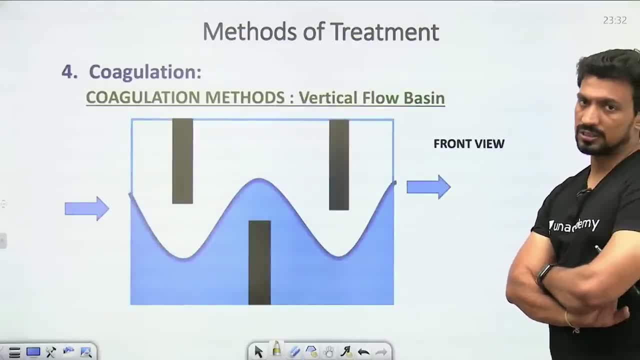 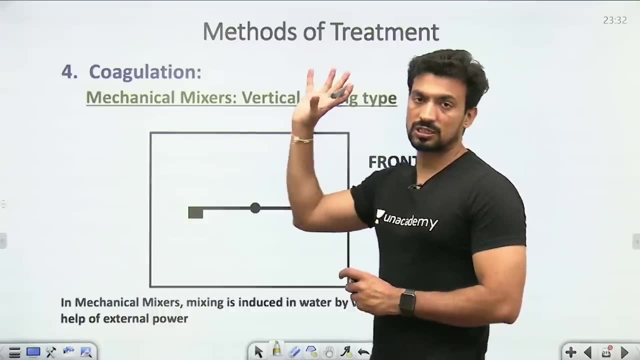 So in the case of mix, Vertical flow basins can also be, Horizontal flow basins can also be. There is not much objective question in this. There can be mechanical mixer Who will just mix. Now, one mixer can be Moving in horizontal plane. 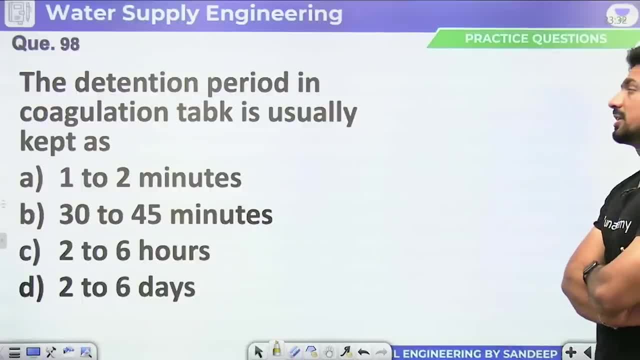 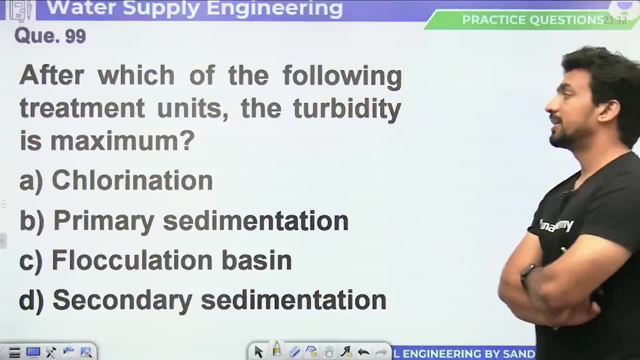 And moving in vertical plane. The detention period in coagulation tank Is usually. Detention period of coagulation tank Is 2-6 hours. After which of the following treatment units The turbidity is maximum. Turbidity will be maximum. 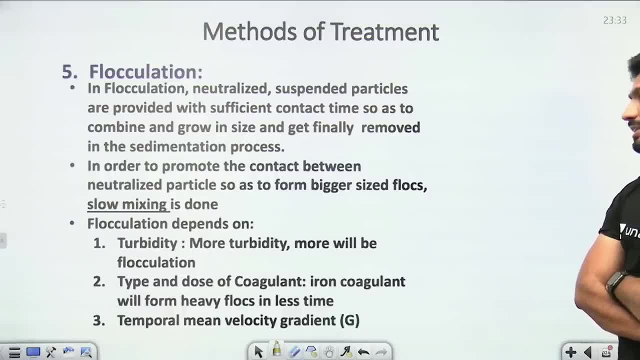 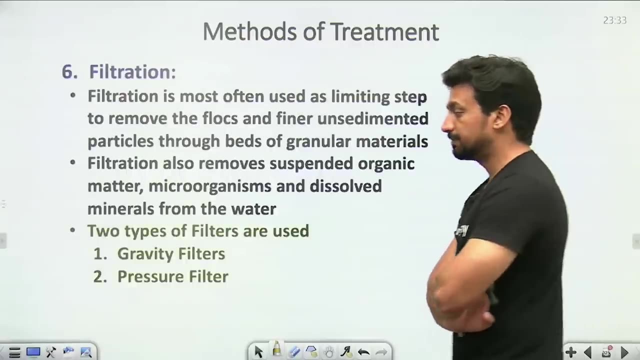 In flocculation basins. So in flocculation, Slow mixing is done To increase the contact time of particles. So on turbidity, What coagulant was added? It will depend on temporal mean velocity gradient. After that, Next process is filtration. 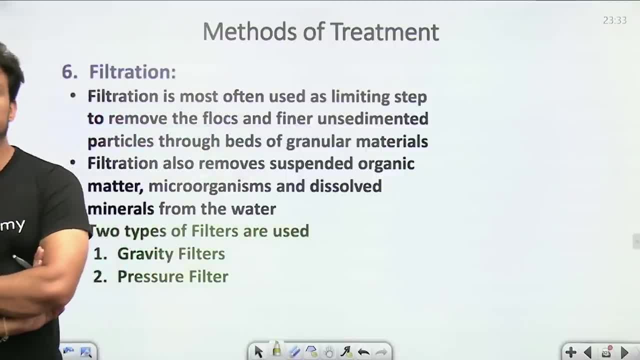 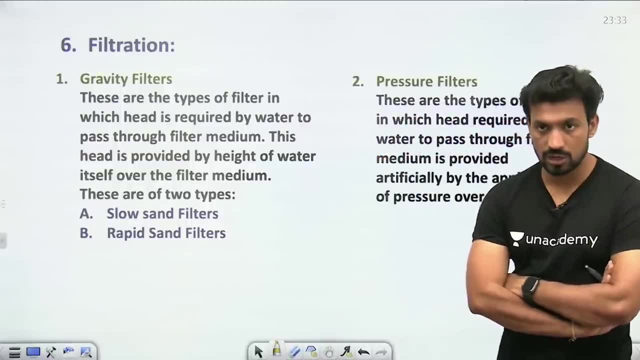 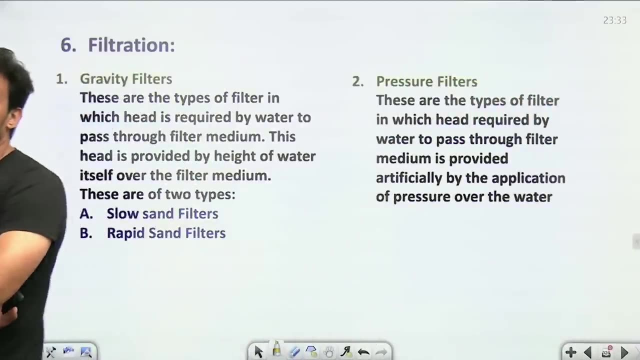 There are two types of filters in filtration: Gravity filter or pressure filter. What happens in gravity filter? The water will go according to The gravity head And filter will be out. In pressure filters We will provide external head Through pressure. 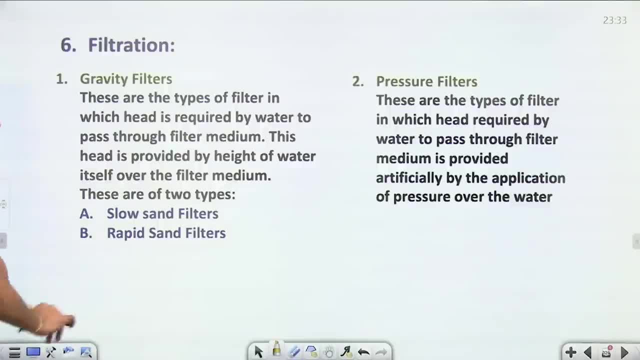 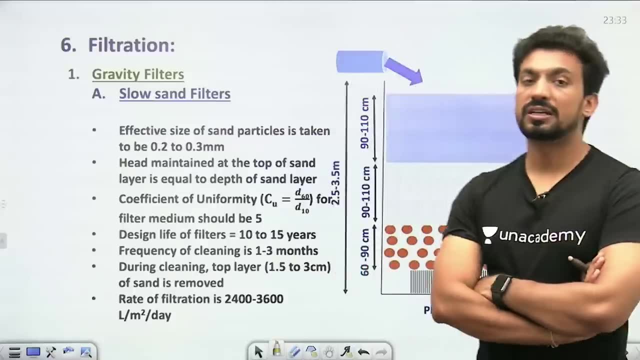 We will make. the water flow. Gravity filters are in our scope: Slow sand filter, Rapid sand filter. What objective questions are asked? We will focus on them. In slow sand filter, Effective size of sand particle Is 0.2 to 0.3 mm. 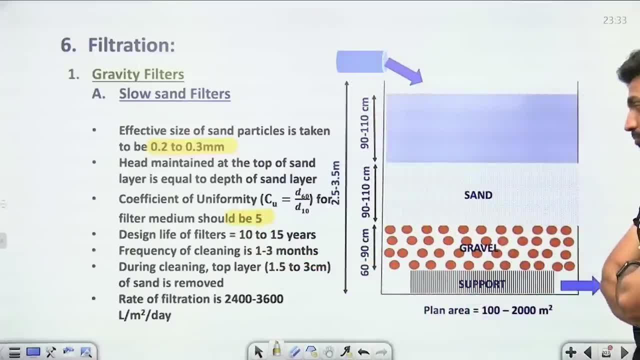 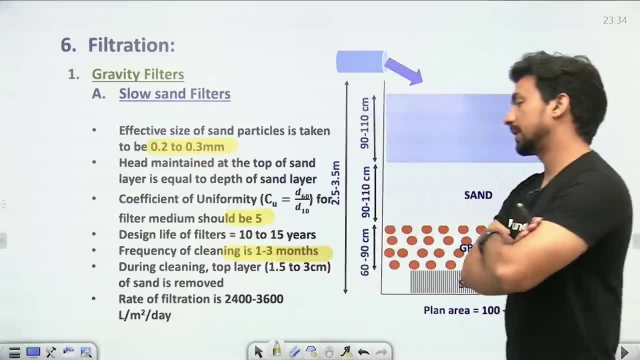 In this, Coefficient of uniformity Should be up to 5.. Design life of filter is 10 to 15 years. Frequency of cleaning is 1 to 3 months. This was asked in objective How to clean it. This was asked in objective. 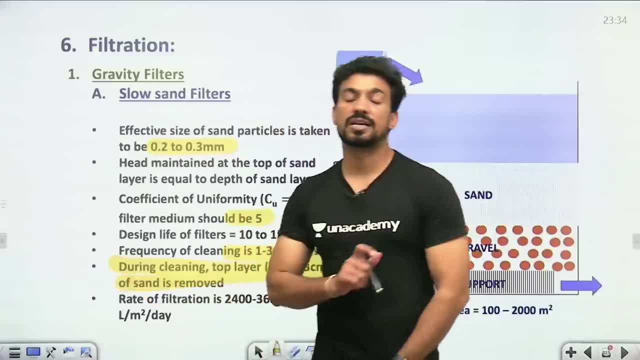 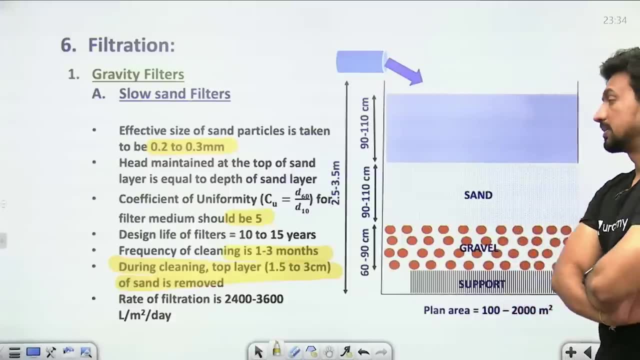 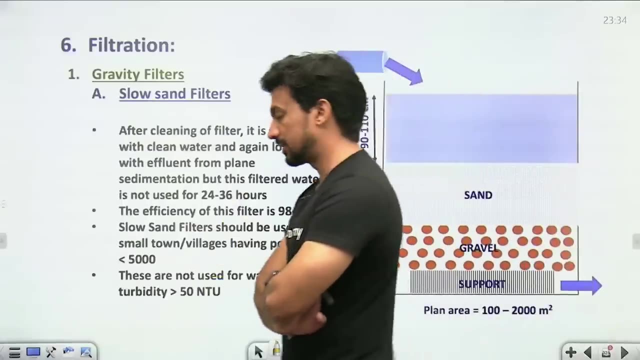 How to clean slow sand filters. For cleaning, It is removed And fresh layer will be used. This comes to you, So for cleaning You have to scrap the top layer. Rate of filtration From 2400 to 3600 liters per meter square. 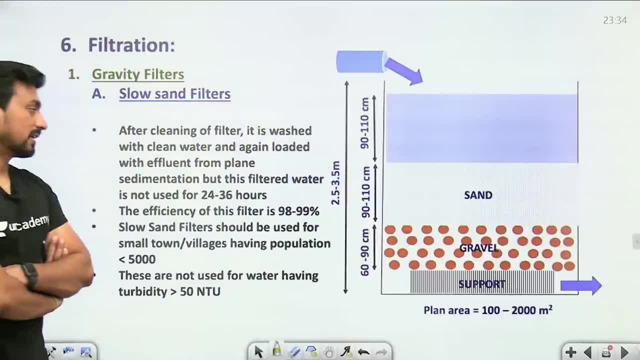 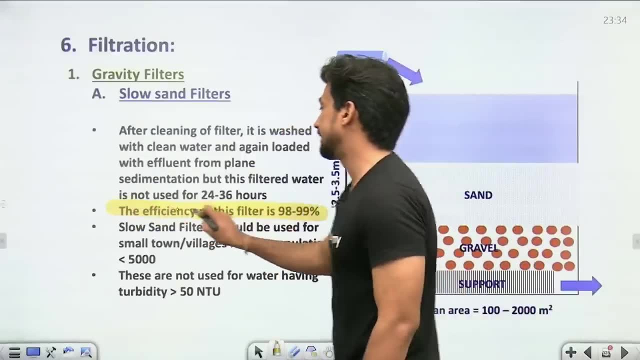 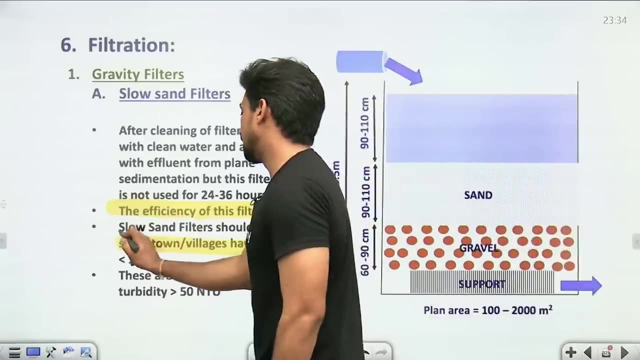 Per day, If we talk about next. So related to its efficiency. Question asked: Efficiency of the filter is 98 to 99%. Related to this Question asked in objective. Slow sand filter should be used For small town villages, So this question was asked. 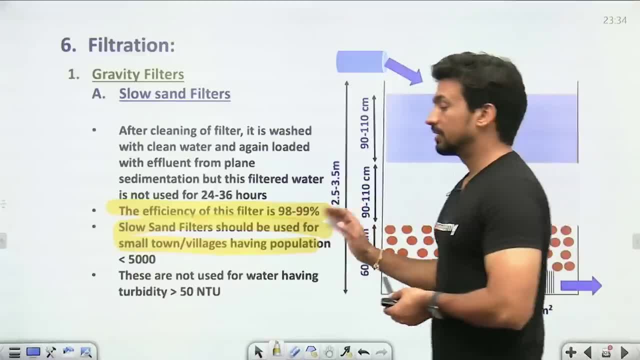 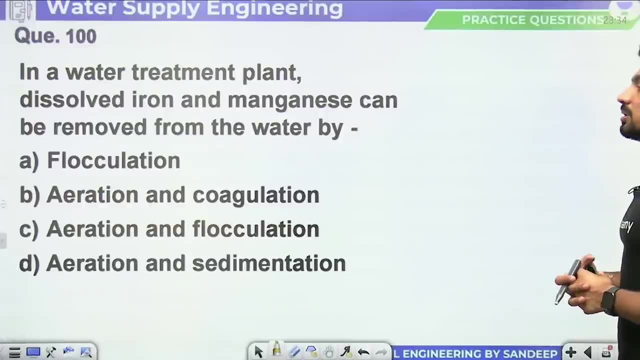 Which filter is used for small town or villages? Slow sand filter is used Where the turbidity is very high, More than 50 NTU. We will not use it there. In a water treatment plant, Dissolved iron and manganese can be removed from the water. 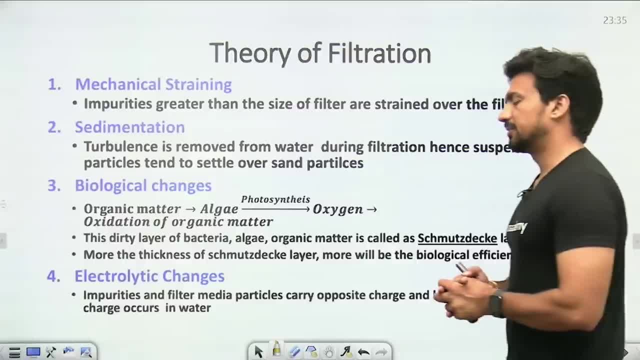 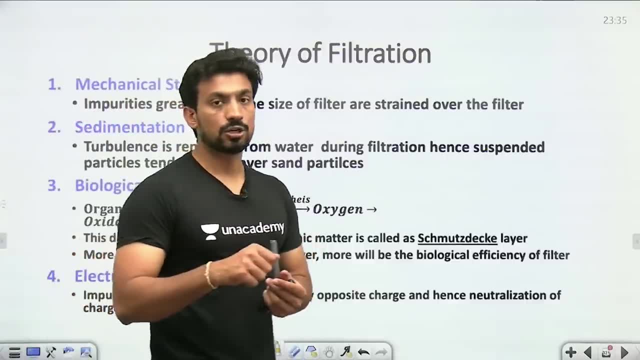 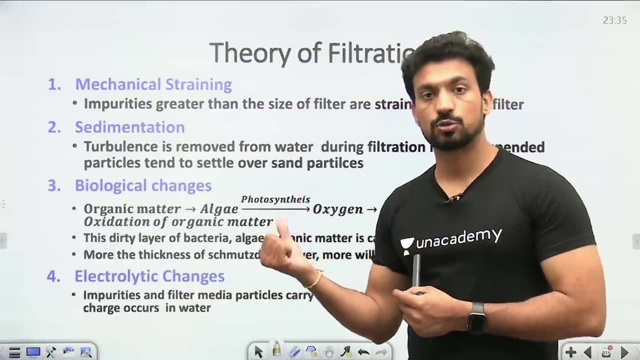 By aeration and sedimentation. Now come to the theory of filtration. Why filtration is working? Like tea, We use a strainer, So what does it do? Big size particles, Bigger than the strainer Particles, are kept up. 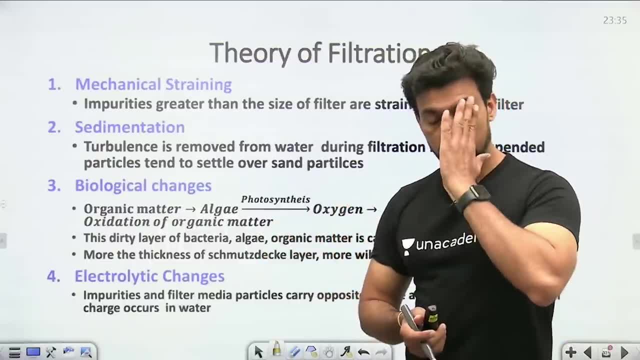 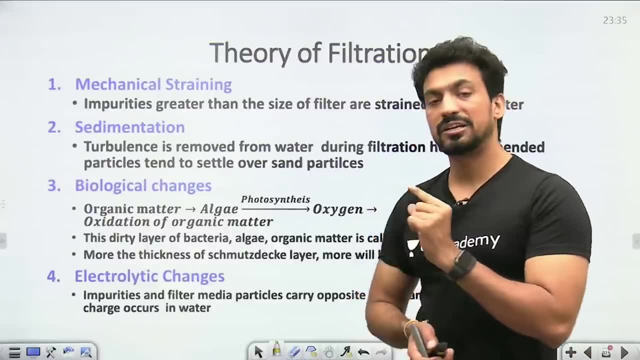 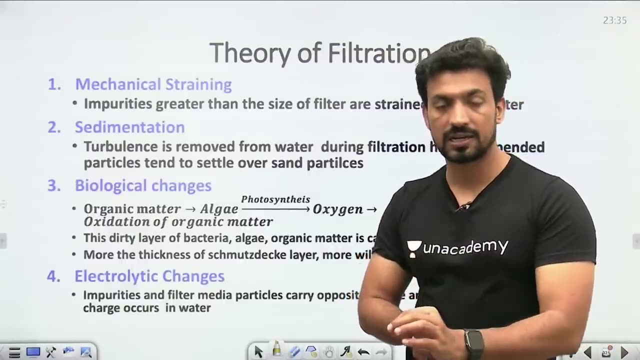 Removes them In the same way. The first purpose of filters, Or how it is doing filtration, How it is working First is mechanical straining. It kept big size particles separate. Second is sedimentation, When water Turbulence will reduce. 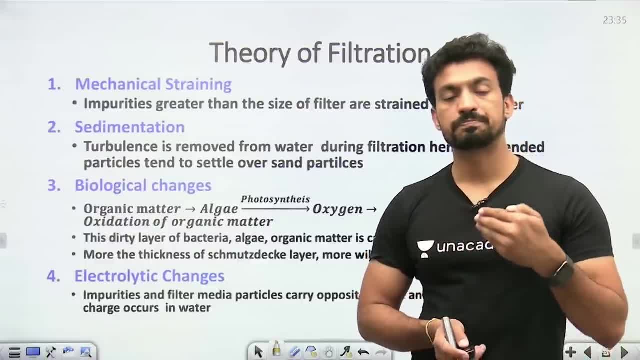 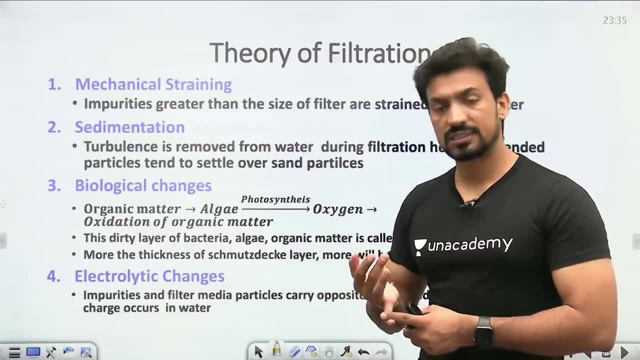 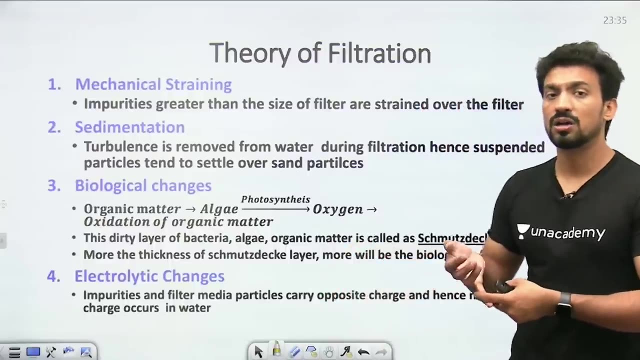 Then filtration. In filters, Multiple phenomena are happening. Second is sedimentation. Third is biological changes. Biological changes will be. If organic matter is present in filters Or algae is present, Photosynthesis will be there. Oxygen will be present. Oxygen will be there. 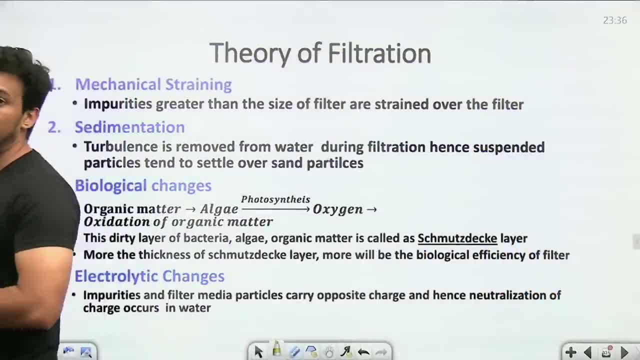 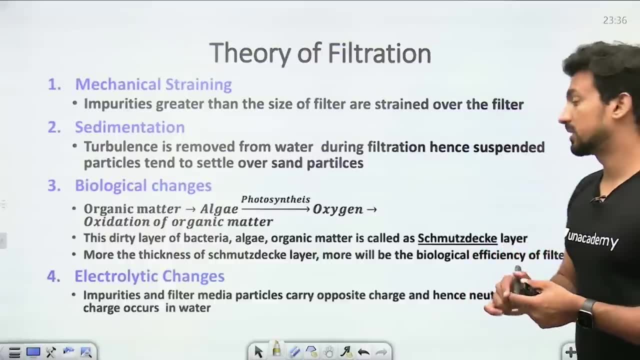 Then again, oxidation of organic matter will be there. Now, what will happen with this? That water will be purer, But at the same time, Organic waste will be mixed, Which is called smooth deck layer. What is it called Smooth deck layer? 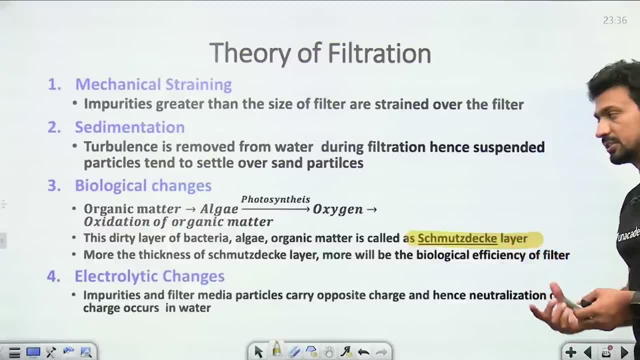 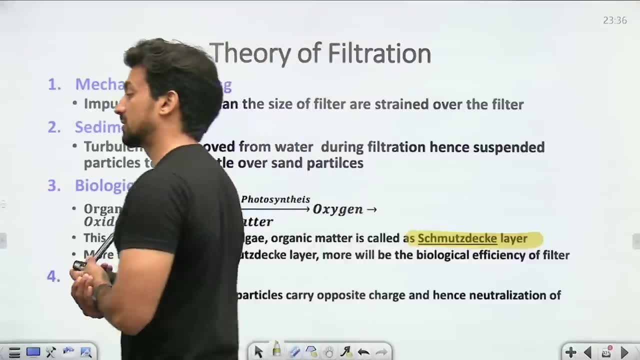 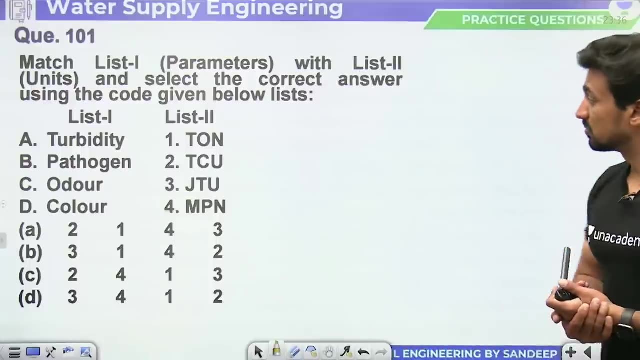 More the thickness of smooth deck layer, More will be the biological efficiency of filter. Third is Electrolytical changes: Neutralization of charges. Neutralization of charges on impurities Due to which they are removed. Next, This question Is a little different. 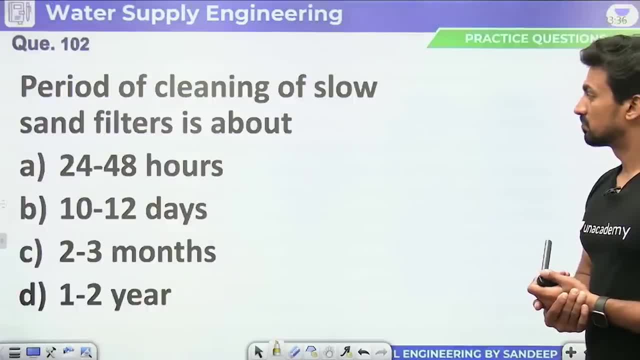 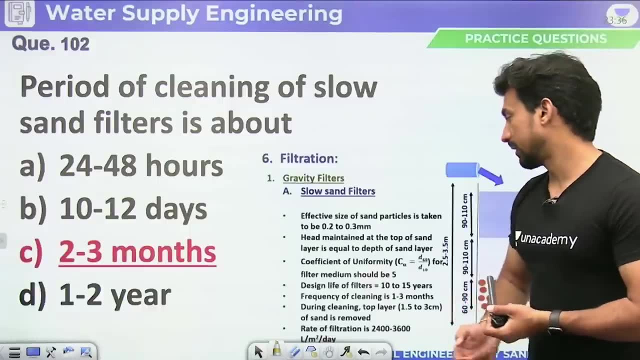 This is done. DE came. Period of cleaning of slow sand filter is about. The answer to this question will be Approximately 2 to 3 months. We wrote 1 to 3 months In option. only 2 to 3 were present. 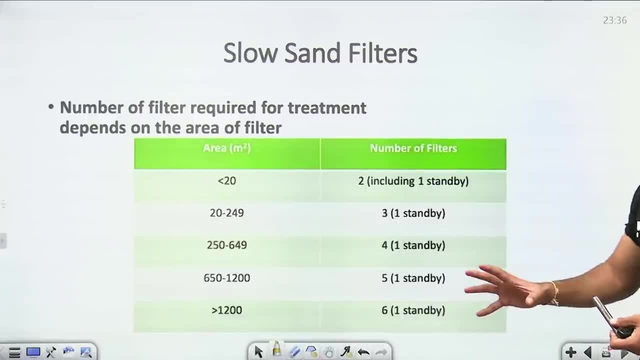 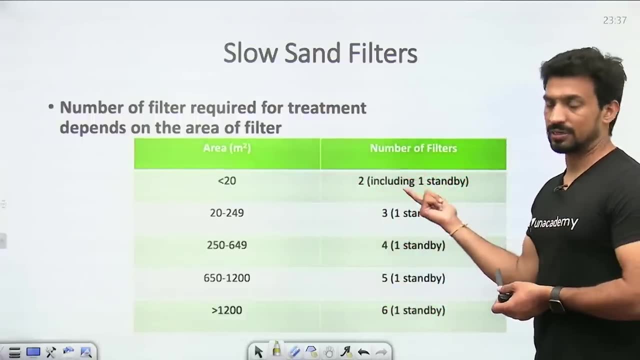 How many filters will be used. This is used in design. If area of filter required is less than 20 m2., Then you will use 2. One working and one standby, 22 to 49. So we will use 3.. 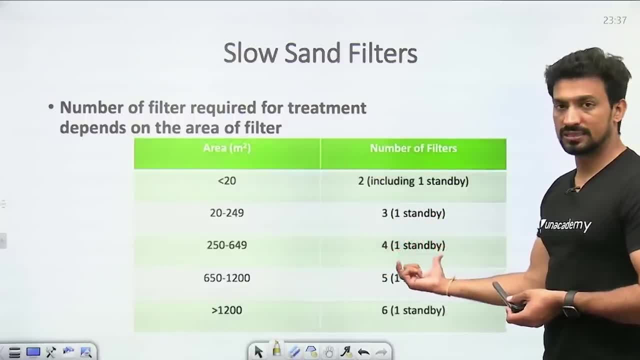 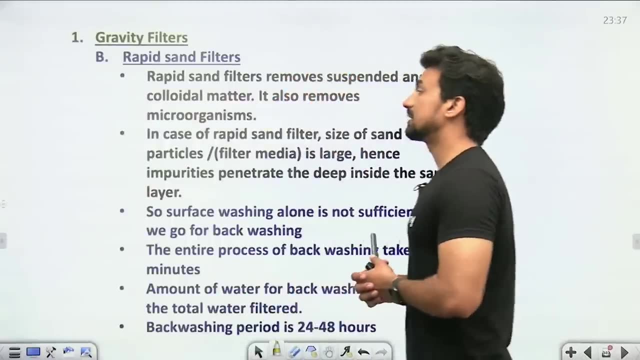 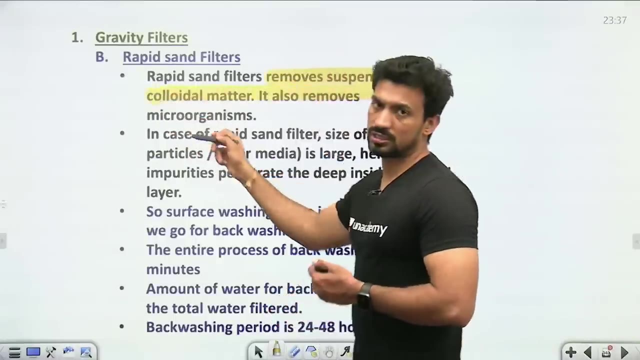 In which 1 will be standby, And so on. Next, Their design is not in our scope. Talking about rapid sand filters. In rapid sand filters You can remove suspended or colloidal matter. It also removes microorganism. It also removes slow sand filter. 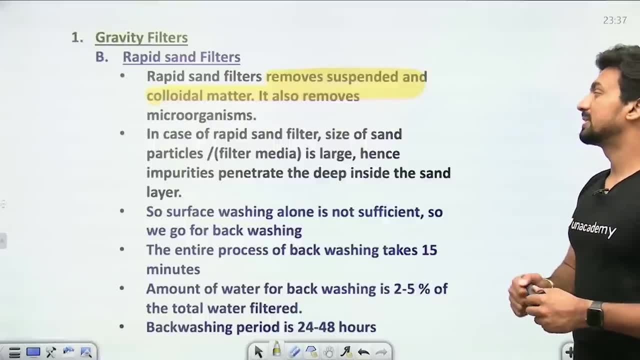 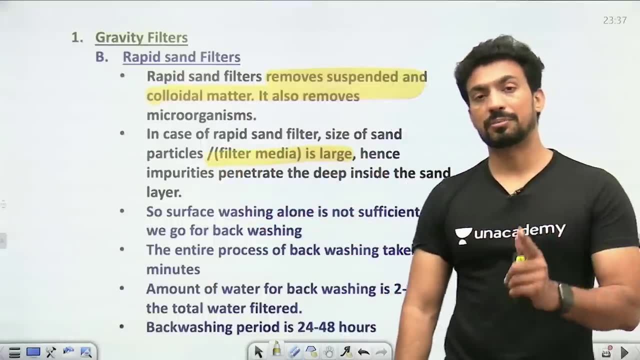 In case of rapid sand filter, Size of particles is large In comparison to you. This question can be asked In slow sand filter or rapid sand filter, In which particle size is small. In slow sand filter, Size of particle is small. 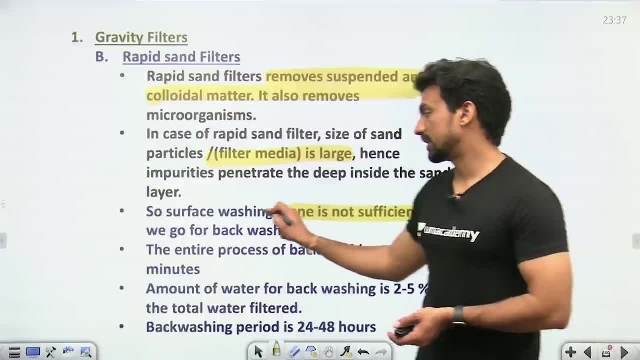 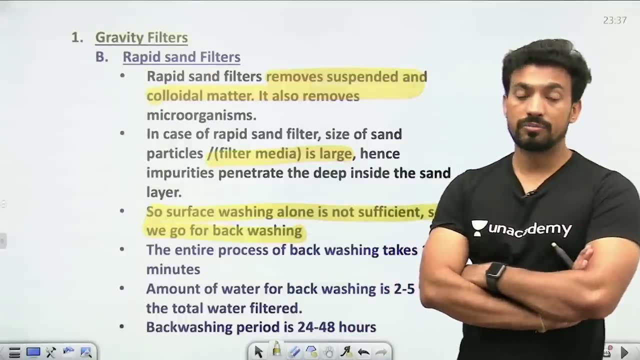 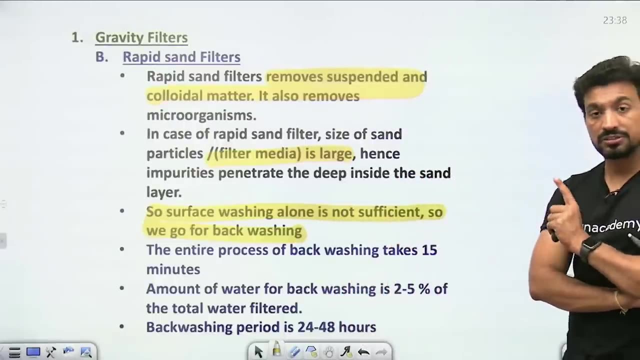 In slow sand filter, Surface washing is not sufficient. Objective question is Difference between slow sand and rapid sand filter. What is the difference of cleaning? In slow sand filter, Top layers are removed. In rapid sand filter, Backwashing is done through cleaning. Quantity of water: The filter water, 2 to 5% is considered. Backwashing period: 48 hours. Area of tank: 10 to 100 m2.. Effective size: 0.3 to 0.6.. Coefficient of uniformity. 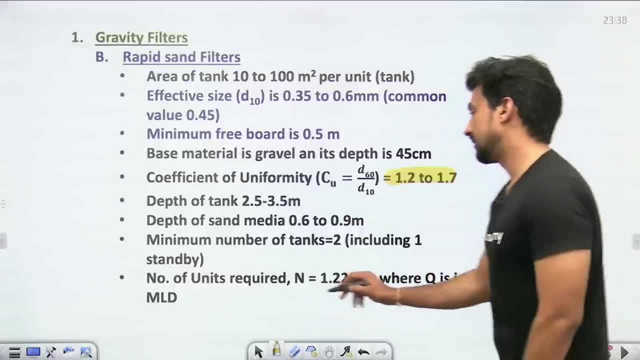 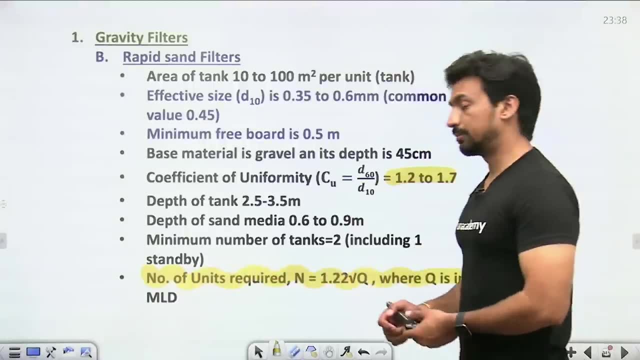 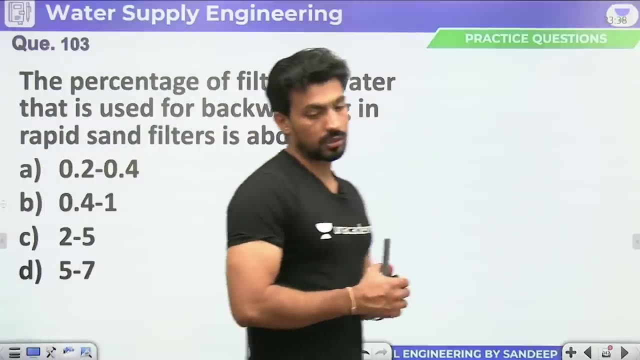 1.2 to 1.7. Objective question: Number of units. Number of units required. Related objective question: In rapid sand filter, Number of units Calculate from which formula 1.2 to root? q. Percentage of filtered water. 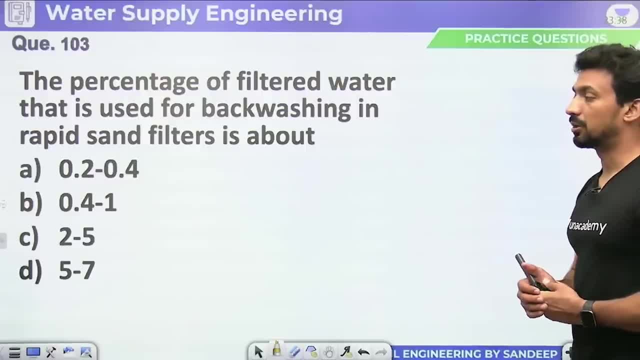 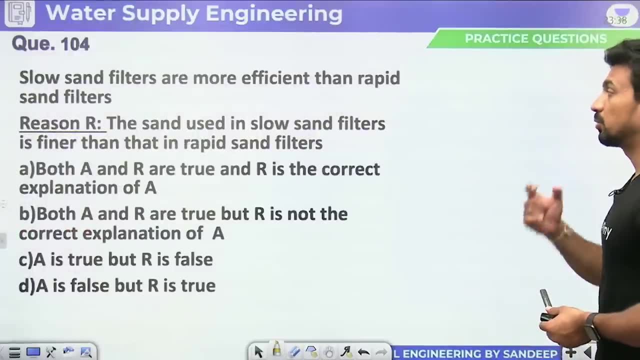 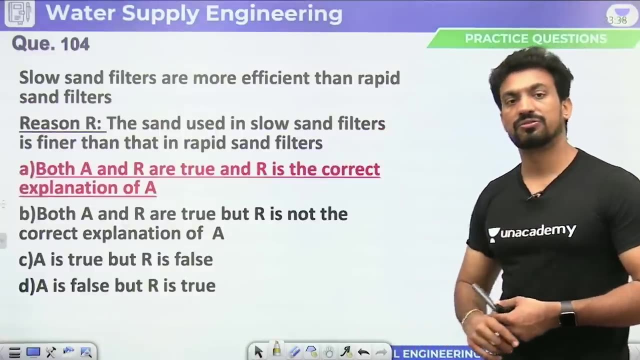 That is used for backwashing. Rapid sand filters is about 2 to 5%. You should know this. Next, Slow sand filters are more efficient than rapid sand filters Because The sand used in slow sand filter is finer Than that in rapid sand filter. 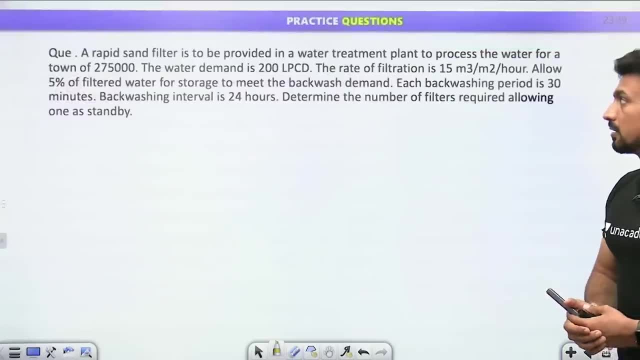 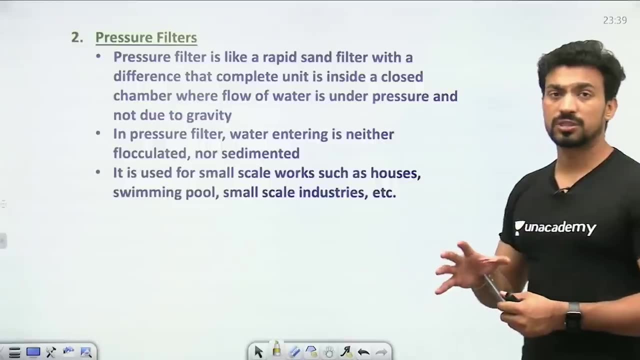 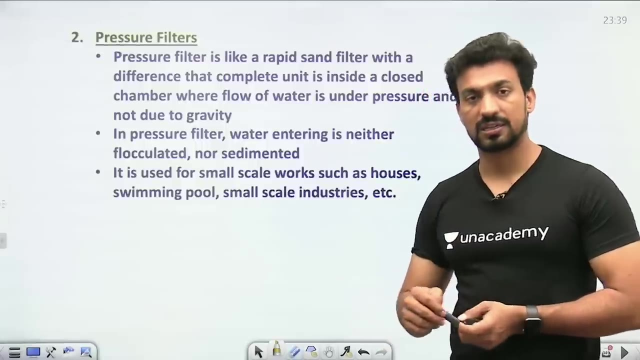 It is correct And it is explaining. Next, We will not go on their designs now. Pressure sand filters: Pressure filters: Because of gravity, Water is not flowing. We pass water through filter media. So wherever small scale treatments are required, 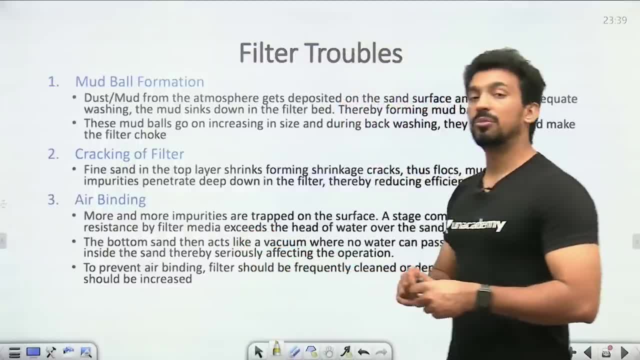 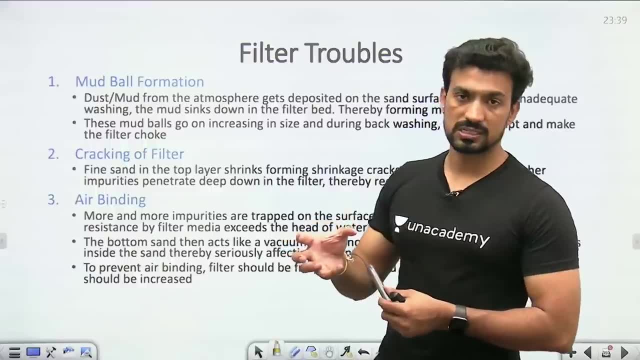 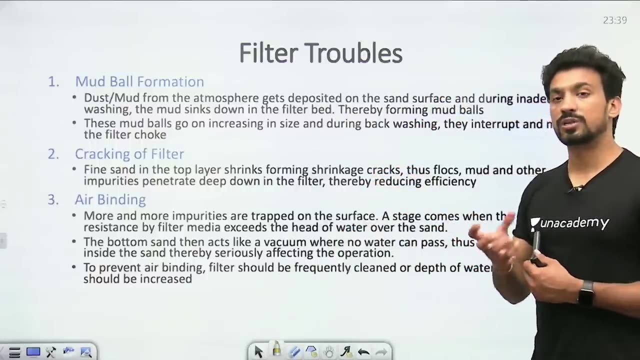 Pressure filters can be used there. In filter Mud ball formations can occur, Mud or dirt. If it goes in filters It will accumulate there. Due to that, filter can be blocked Cracking of filter If the sand in the filter 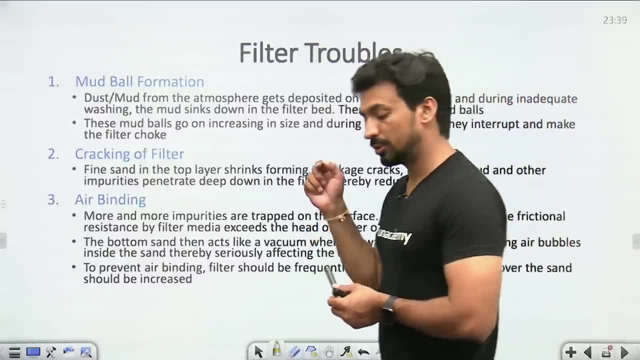 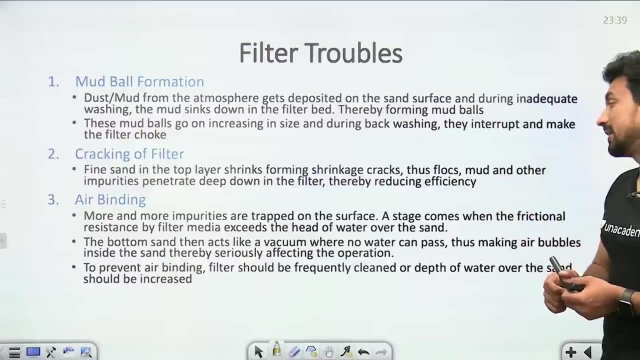 Shrinkage has occurred. Due to that, cracks can occur In which impurities will go inside Air binding Because of negative head. Question asked in objective: Due to which air binding occurs? Air binding occurs, Vacuum or negative head? Air binding occurs. 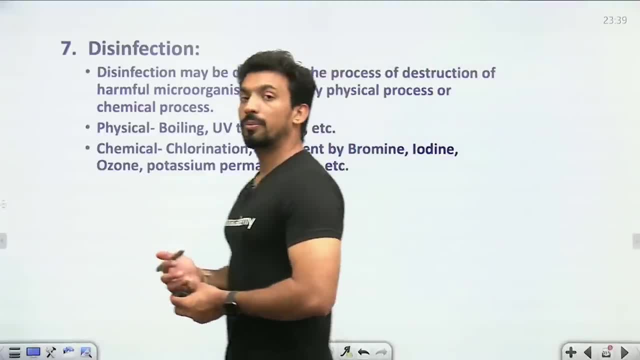 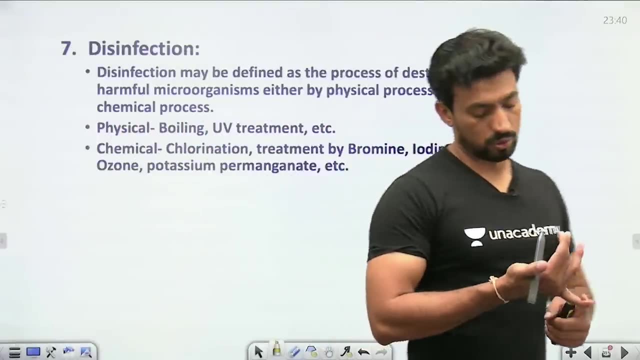 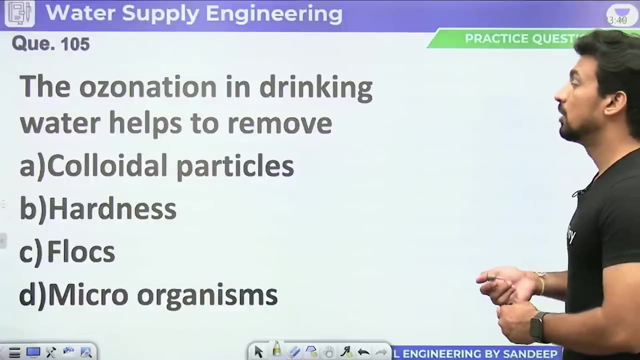 Next step: Disinfection. Disinfection means Biologically active microorganisms. Kill them. Chlorination, Bromination, Iodine, Ozone, Potassium permanganate- We can disinfect with their help. Ozonation in drinking water helps to remove microorganisms. 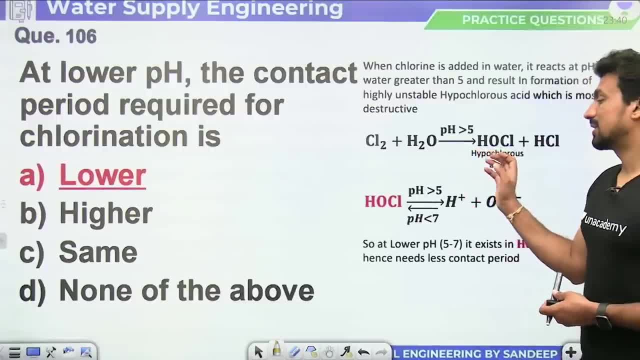 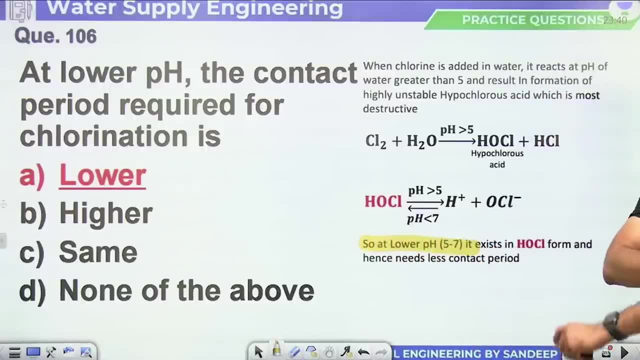 At lower pH, The contact period required for chlorination is lower. If we talk about pH, The suitable range for pH For your chlorination- Lower pH 5 to 7.. It is more destructive. It kills bacteria better When chlorine acts with water. 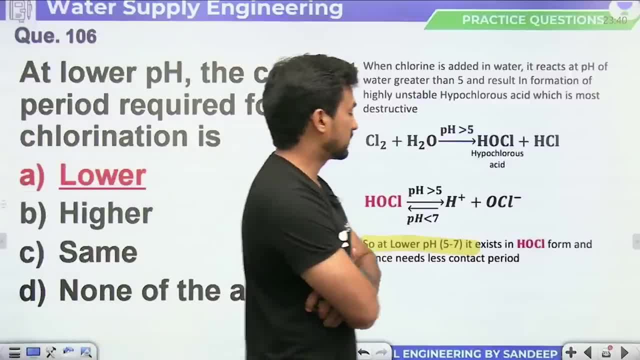 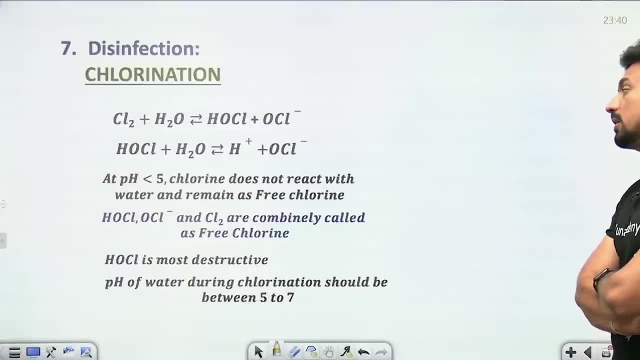 It forms HOCl plus HCl, And HOCl again Exists in H positive and OCl minus form When pH value is 5 to 7. In that case HOCl forms And it is more destructive. So objective question asks you: 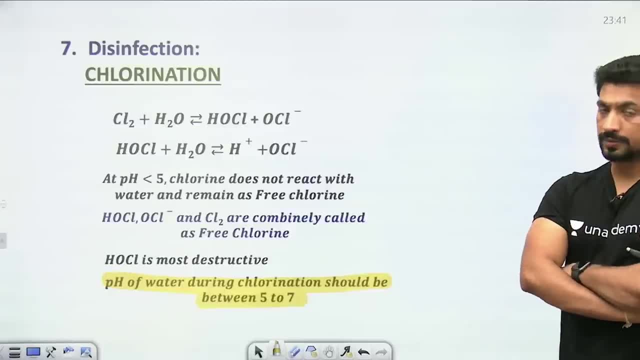 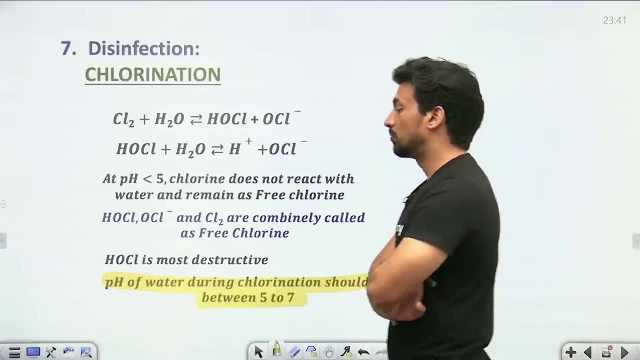 How much should be the pH of water for chlorination? It should be between 5 to 7.. At pH less than 5. It will remain in free chlorine form, HOCl, OCl minus and Cl2 form, Out of which 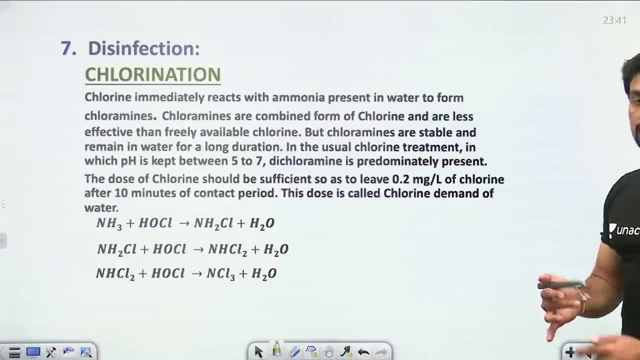 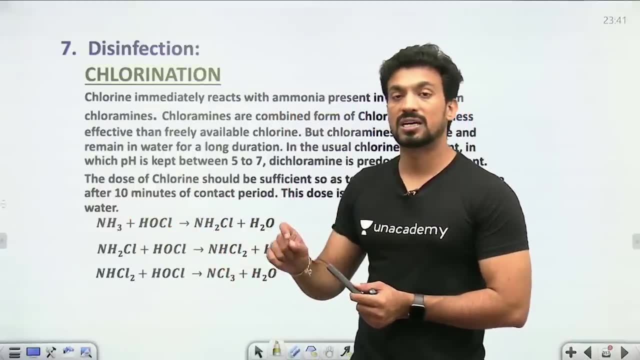 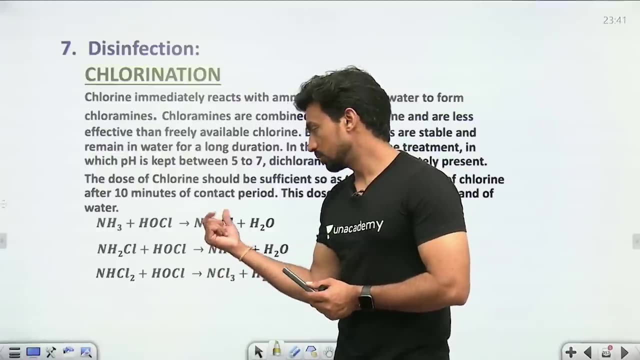 HOCl is most destructive. When HOCl forms In water, Ammonia is present, It is NH3 form. It forms chloramines with it, First Monochloramine, Then Dichloramine, Then Trichloramine. In monochloramine there was A-chlorine. 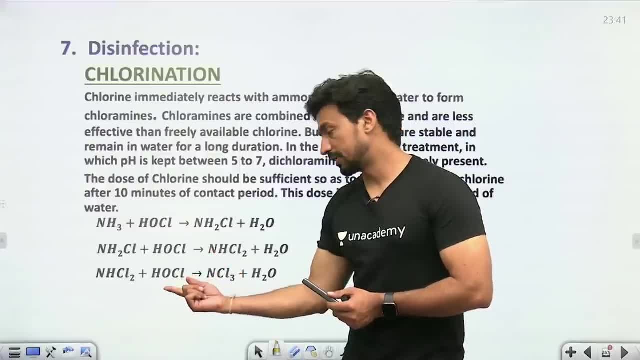 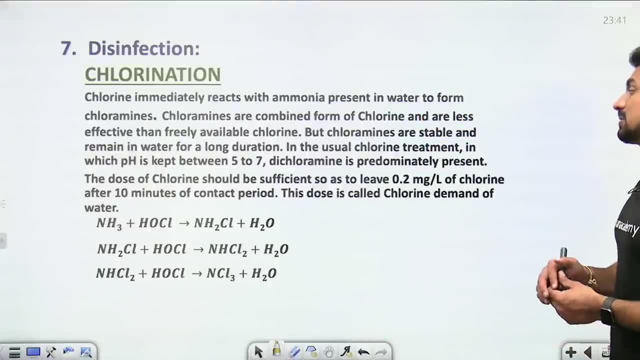 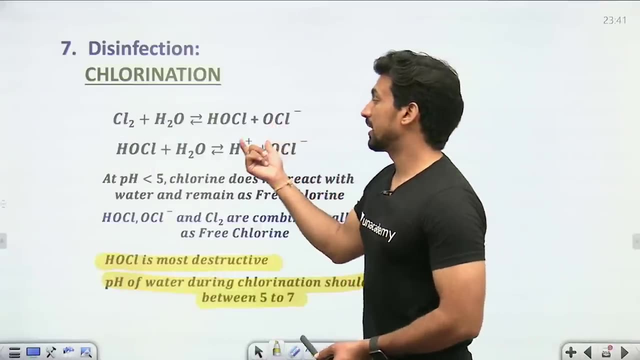 Further it reacted with HOCl. So one more chlorine came: Monochloramine, Dichloramine, Trichloramine, Out of which the most stable, Which is Dichloramine- Now what they talked about, Why this was needed. 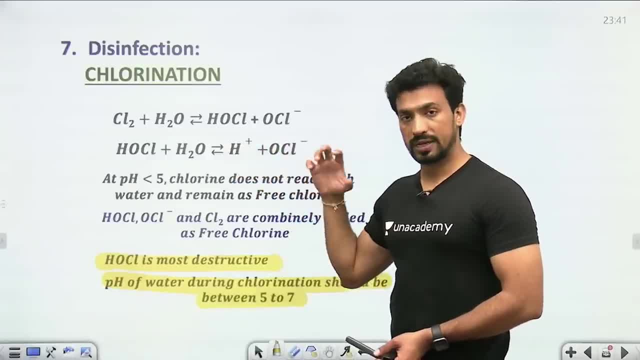 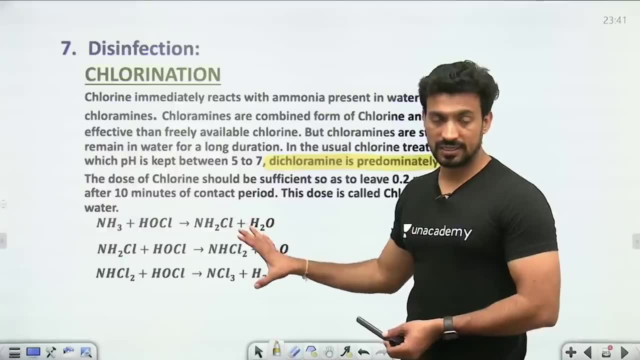 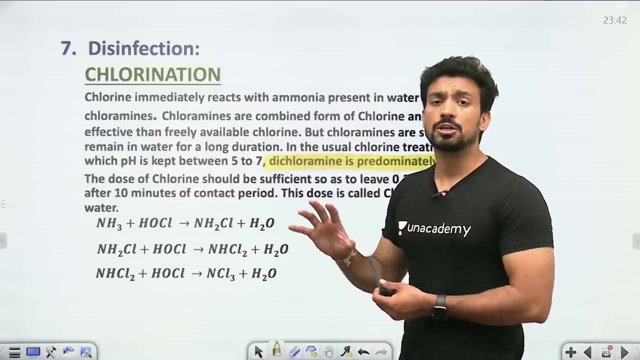 OCl minus HOCl- These are all forms of chlorine Which will work for disinfection. But those who can stay for the longest time, Even if they are not as efficient But, Excuse me, For the longest time, Those who will stay stable in water, 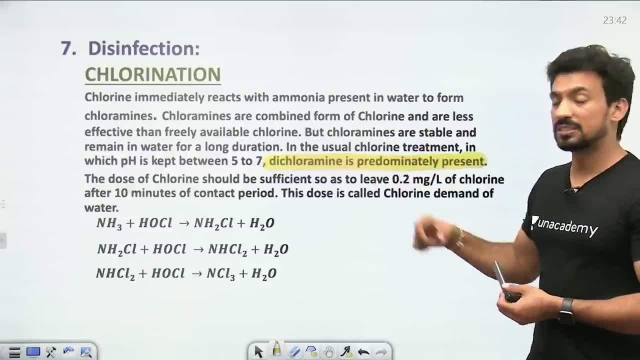 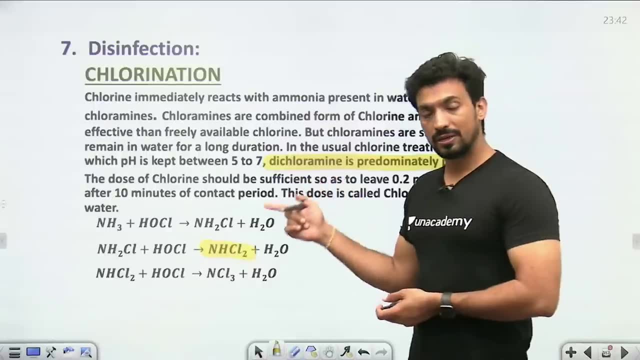 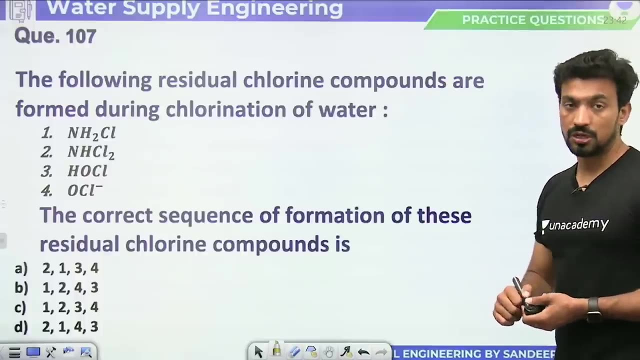 They are chloramines, So out of these, Dichloramine Will be most efficient. So not so efficient, But they are present for a long time. That's why we are using them. The following residual chlorine compounds Are formed during the chlorination of water. 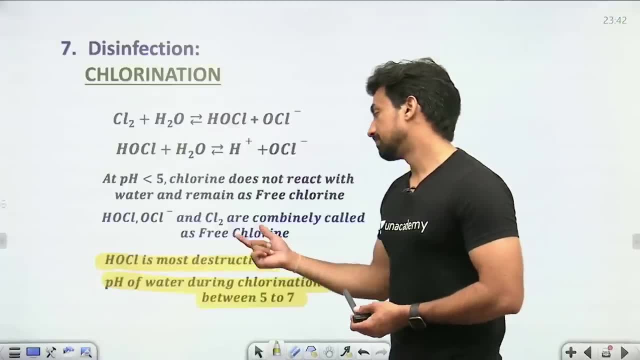 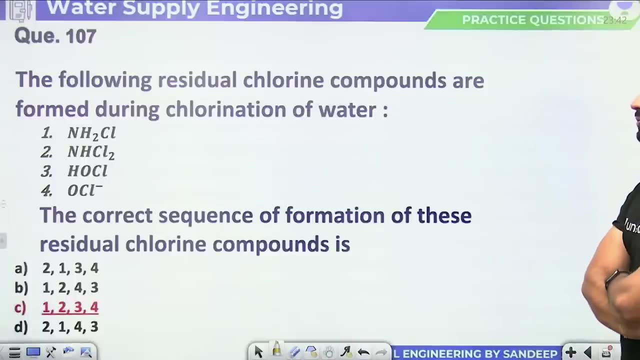 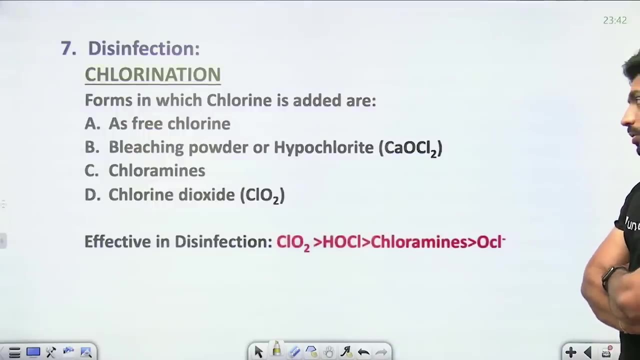 So what is their correct sequence? First our monochloramine, Then Dichloramine, Trichloramine is formed. So the correct sequence: NH2Cl, NHCl2.. OCl, Then OCl minus. How can you add chlorine? 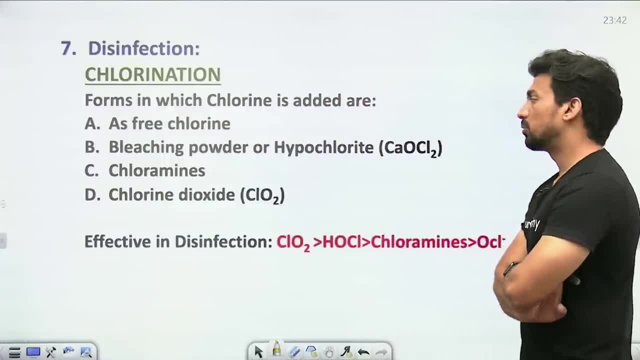 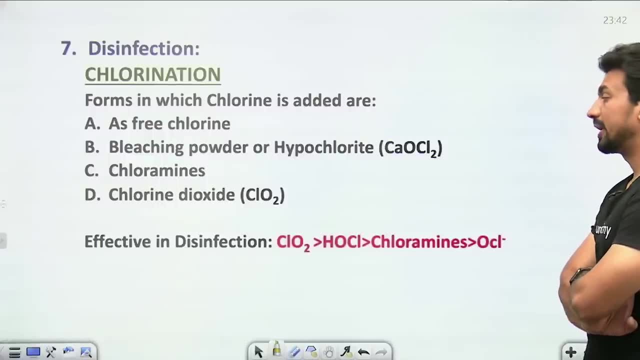 How can you do? chlorination In the form of free chlorine, Bleaching powder or hypochlorite CaOCl2 can be added. Chlorine can work in the form of chloramines Or it can work in the form of chlorine dioxide. 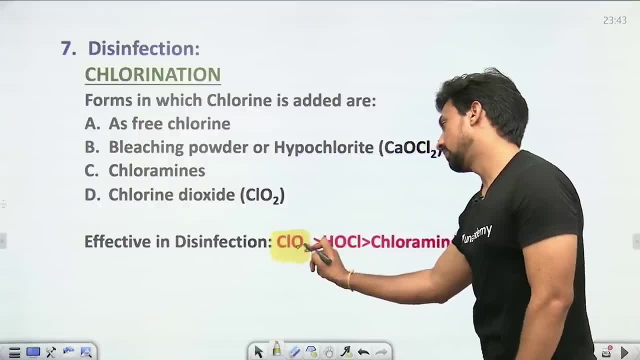 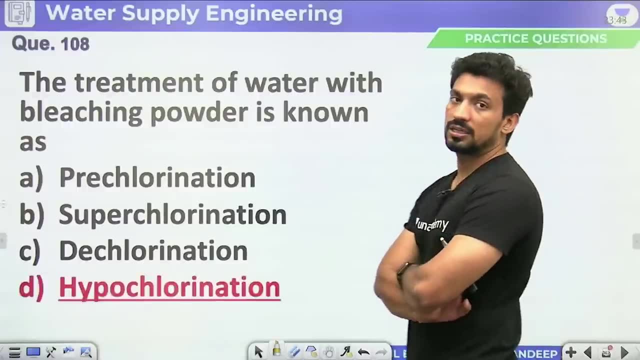 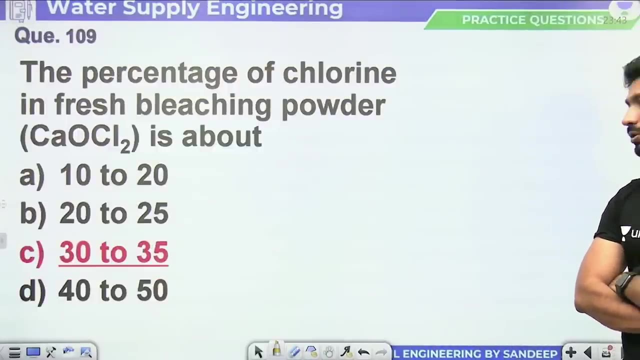 Out of which chlorine dioxide Is most destructive, Then HOCl, Then chloramines And then OCl minus. The treatment of water with bleaching powder Is known as hypochlorination Percentage of chlorine In fresh bleaching powder. 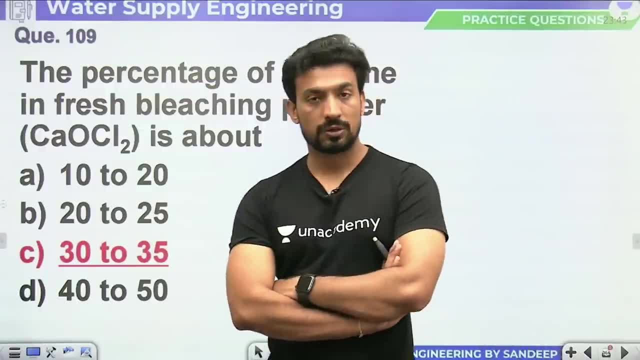 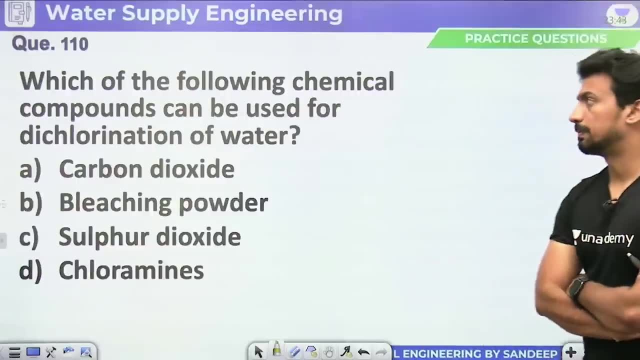 Is about 30 to 35%. If you have taken bleaching powder In that bleaching powder, How much chlorine will be there? Chlorine is about 30 to 35%. Which of the following Chemical compounds can be used For dechlorination of water? 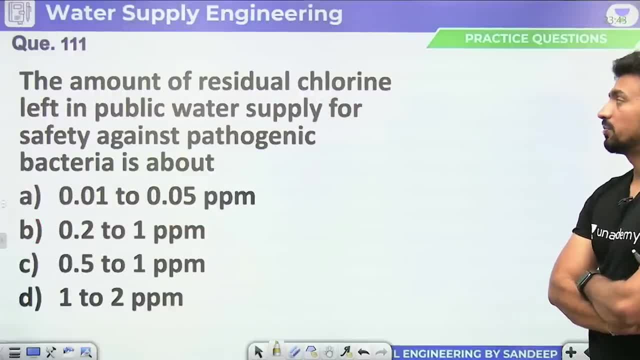 For dechlorination You can use sulfur dioxide. The amount of residual chlorine Left in public water supply. For safety against pathogenic bacteria, Residual chlorine is kept From 0.2 to 1 ppm. Further bacteria impurity. 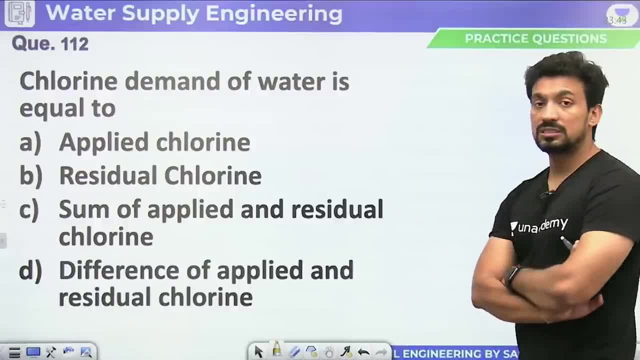 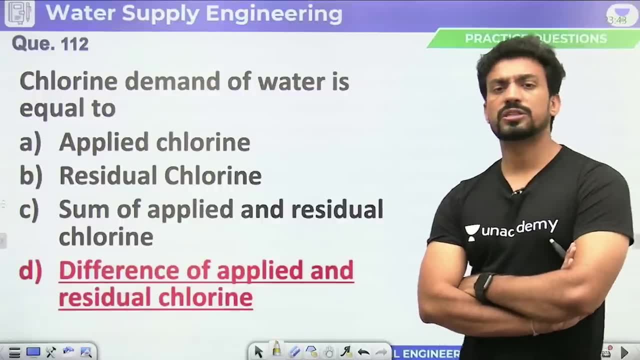 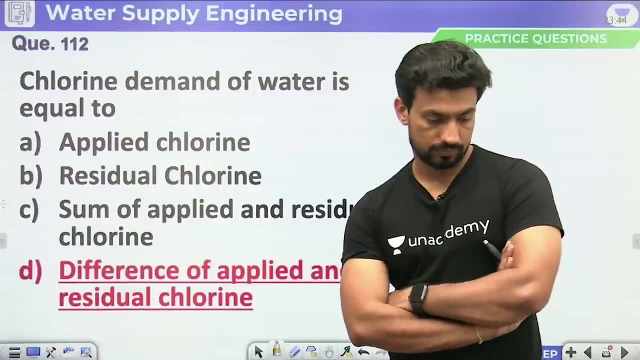 Will come in water To treat it. Chlorine demand of water is equal to Chlorine demand, First for disinfection And then to leave some residual chlorine. So difference of applied And residual chlorine Will be your chlorine demand. How much chlorine was needed? 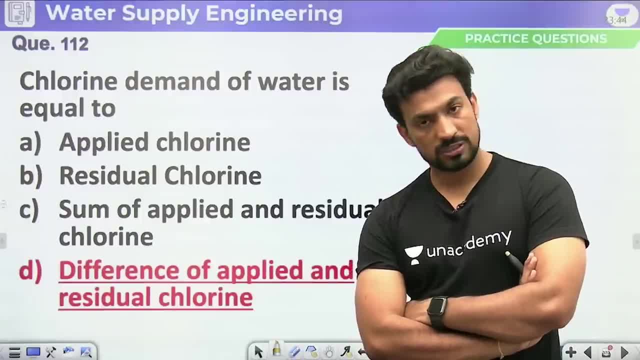 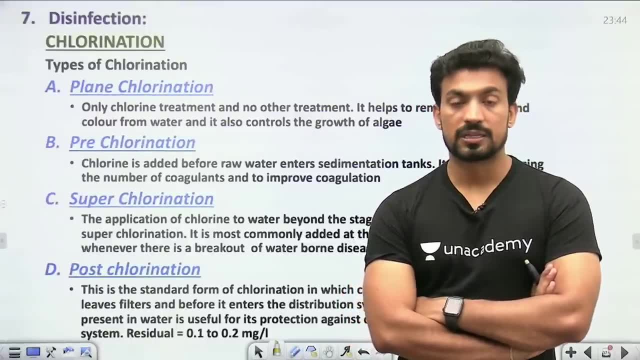 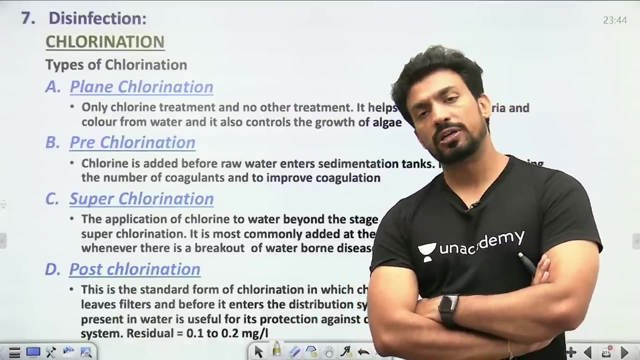 How much chlorine was utilized, How much was applied? How much was left? Chlorine demand was utilized. Now chlorination. There are some types. First is plain chlorination. Plain chlorination means You are not giving any other treatment to water. 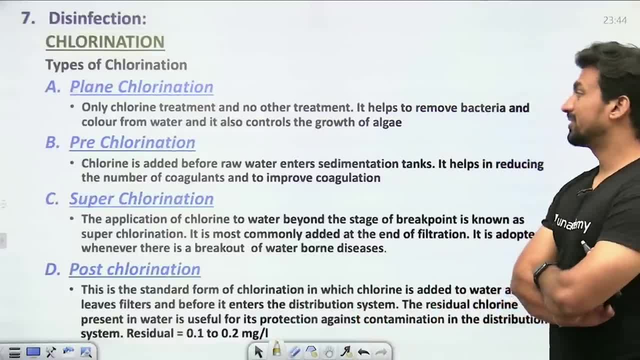 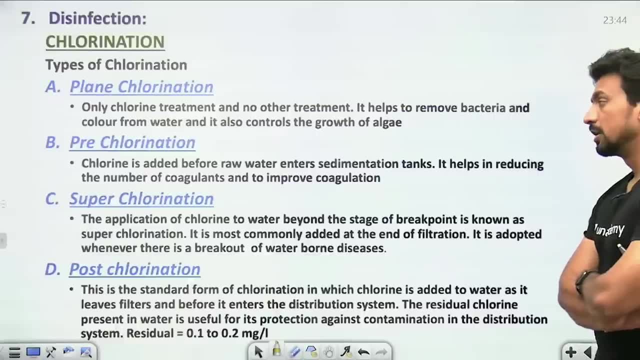 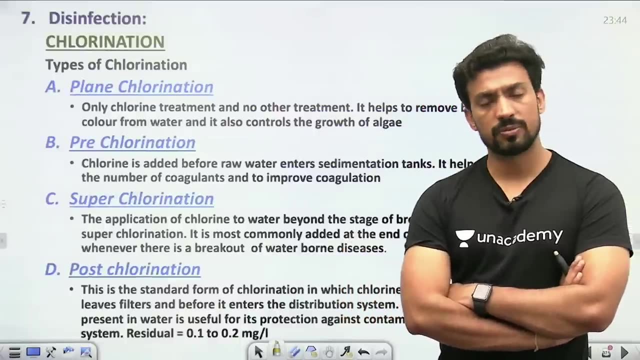 Chlorine is added To treat it. So only chlorine treatment And no other treatment. It will remove bacteria, Color will be removed And algae growth will be controlled, If we talk about pre-chlorination When water treatment was starting. 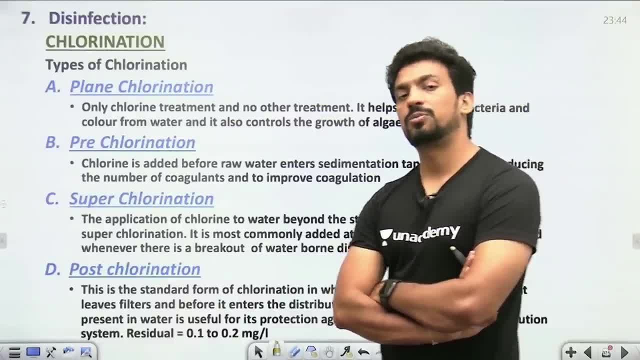 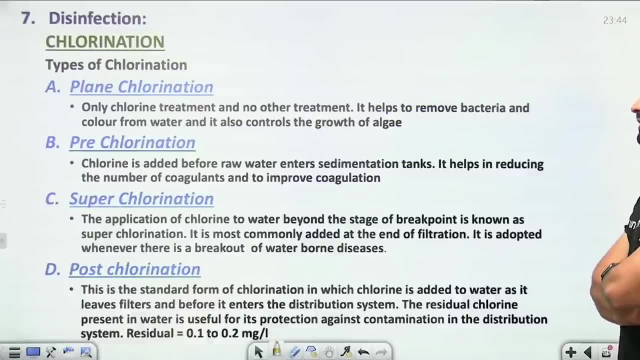 Before that, Before sedimentation, Chlorine was added to water. So as the process goes further, Your treatment efficiency Becomes better. It helps in reducing the number of coagulants And to improve coagulation. When do we do super-chlorination? 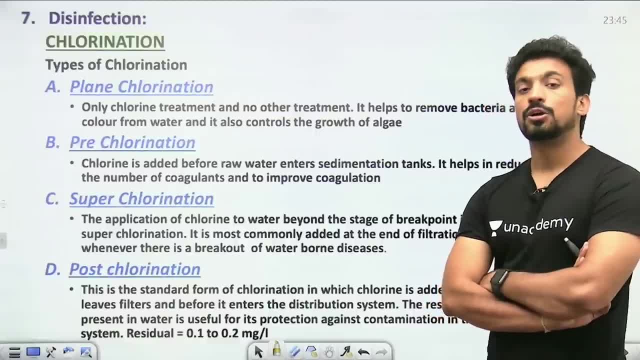 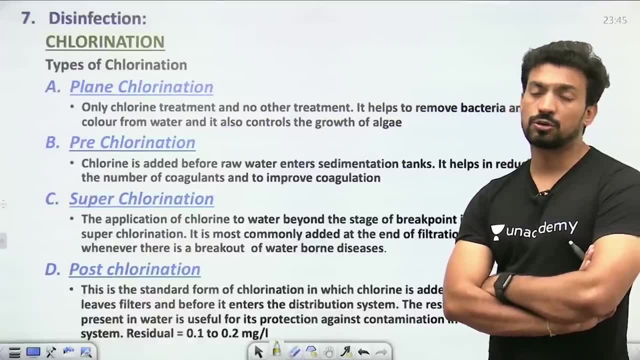 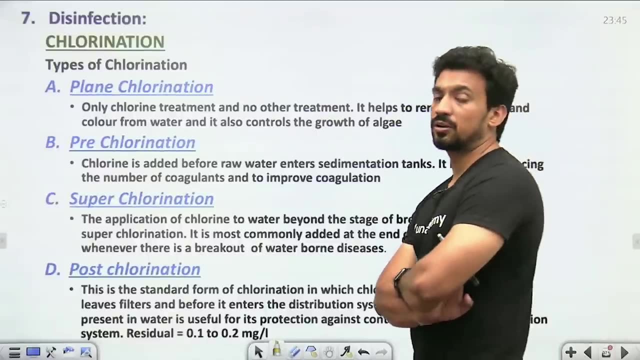 When an epidemic spreads. When an epidemic spreads, So in large amount Chlorine is added to water So that as soon as Bacteria or virus comes in contact It will kill it immediately. So super-chlorination is done, But remember: 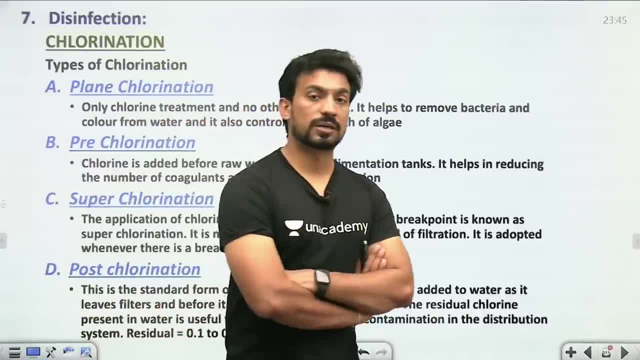 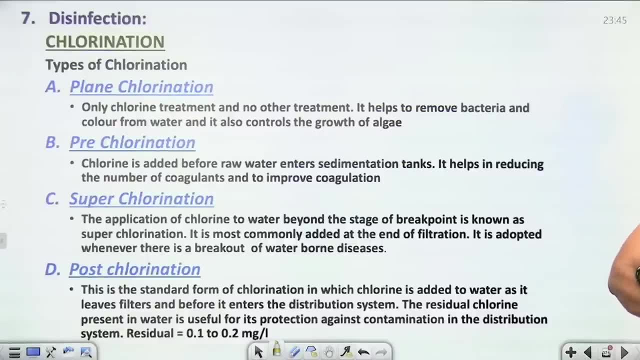 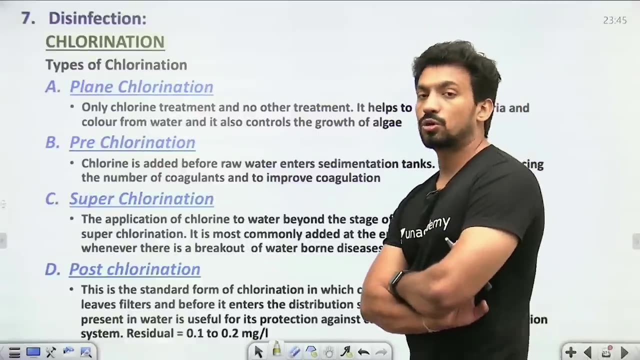 After doing super-chlorination, When water will be used, We will do de-chlorination first, Post-chlorination. What happens When it leaves filters And water will go to the distribution system, Distribute So at that time. 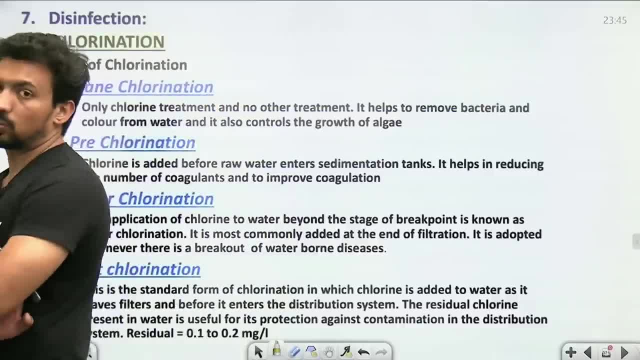 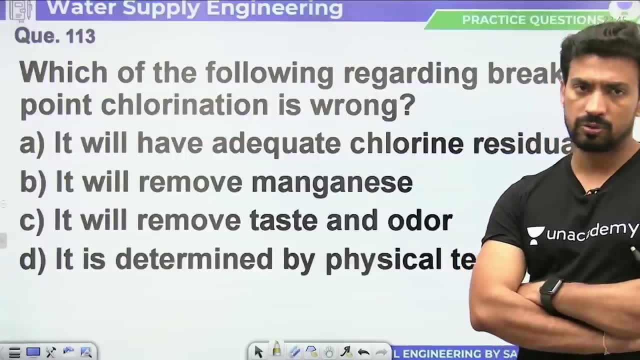 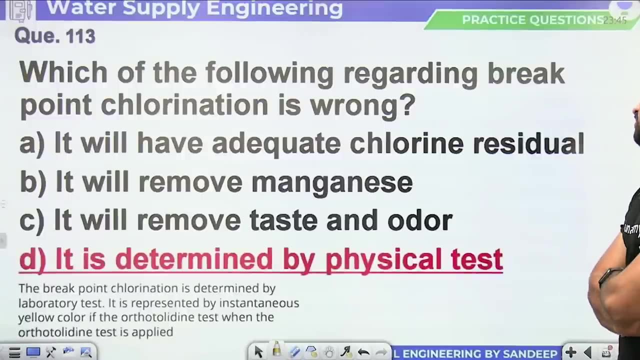 Some more chlorine was added to it For further impurities. So you provided post-chlorination For residual chlorine. So you provide 0.2 mg per liter. Which of the following? Regarding the breakpoint, Chlorination is wrong, So it is determined? 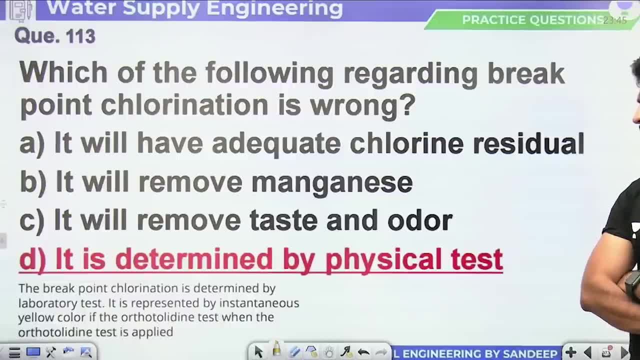 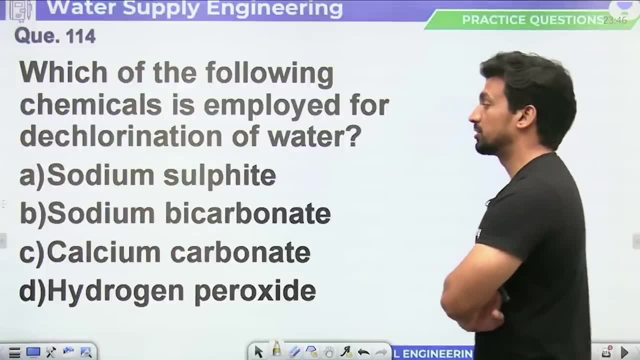 By physical test. It is wrong. We do it with laboratory test With the help of ortho toluidine test. Which of the following chemicals Are employed for de-chlorination of water? For de-chlorination of water, Sodium sulphide is used. 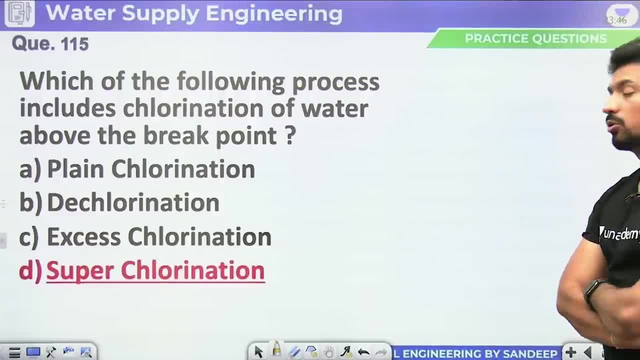 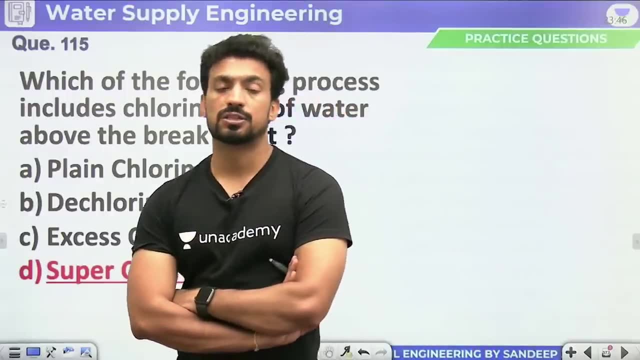 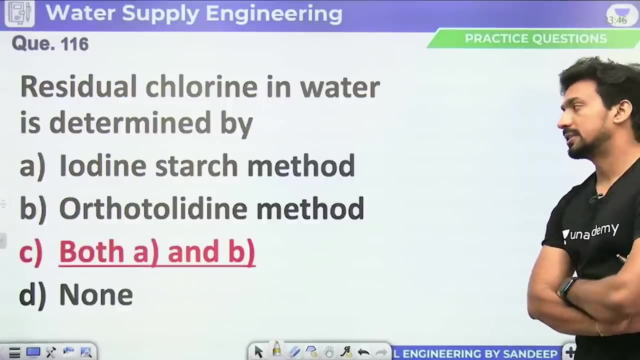 Which of the following process Includes: chlorination of water Above the breakpoint In super-chlorination, More than the breakpoint When all the pathogens have killed you? Residual chlorine From which it can be determined Iodine starch method. 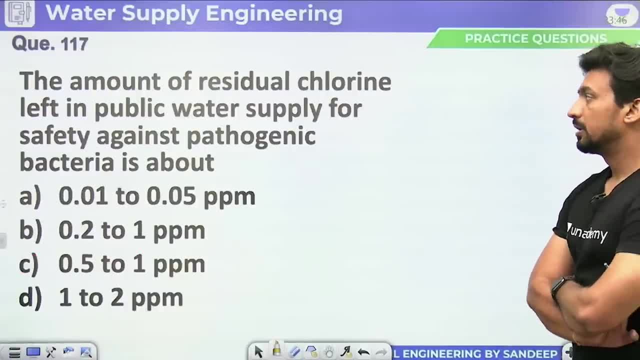 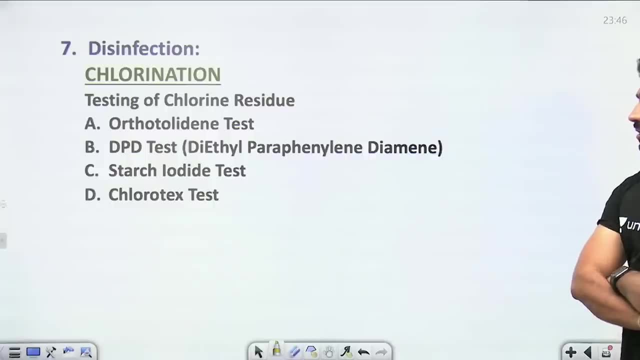 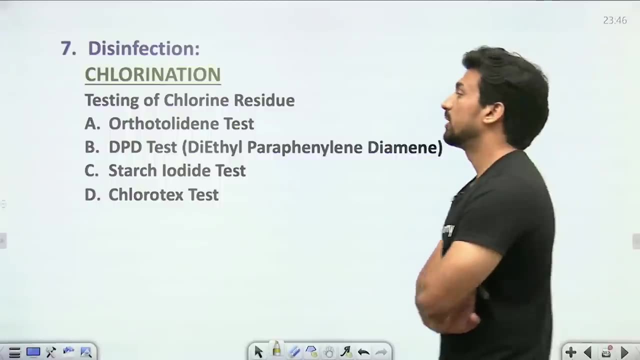 Ortho toluidine method, We can find out The amount of residual chlorine Left in public water From 0.2 to 1 ppm. Ortho toluidine test, DPD test, Starch iodide test, Chlorotex test. 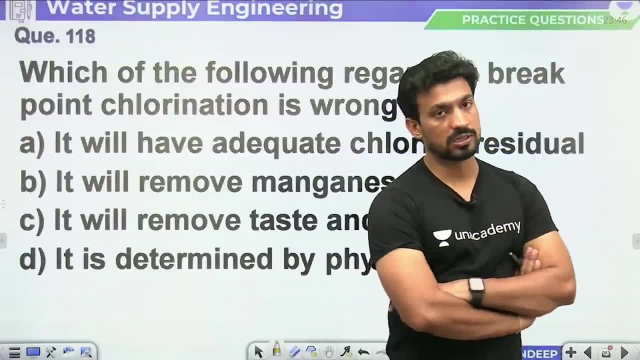 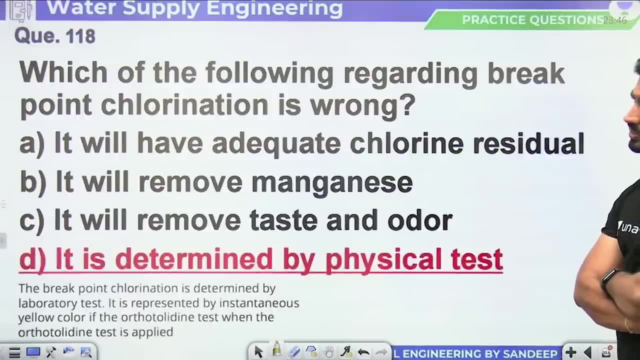 We can do all these tests To find out the residual form of chlorine. Which of the following Regarding breakpoint chlorination Is wrong? These questions came 2-3 times. There are 5-7 such questions Which are repeated. 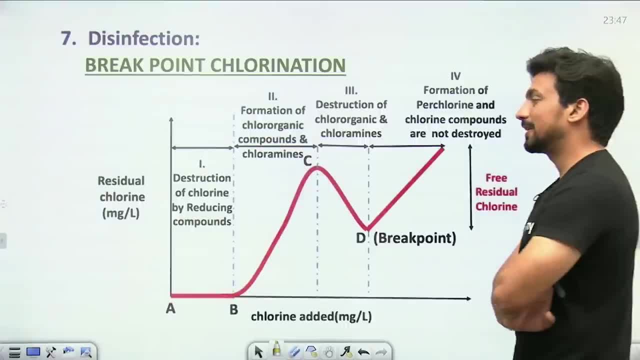 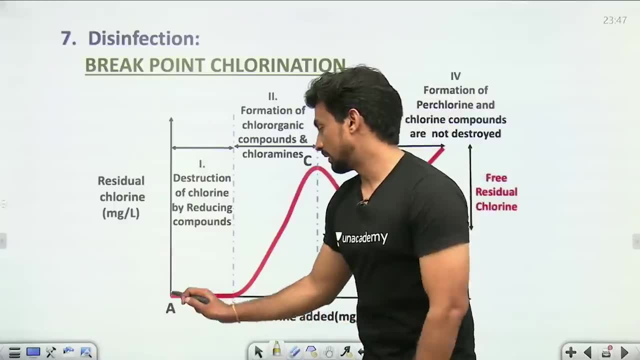 What is breakpoint chlorination? What did you do first? Yes, there was such a question. The graph of chlorination was given to you And in it This graph was given like this, In the beginning, at the level of zero, And he asked why it is horizontal here. 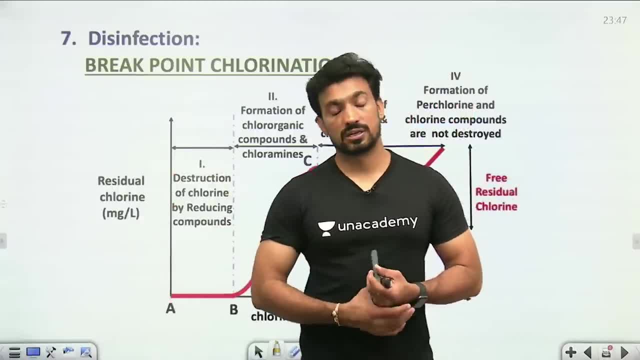 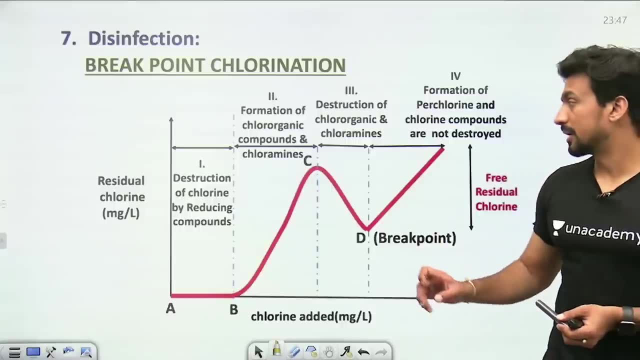 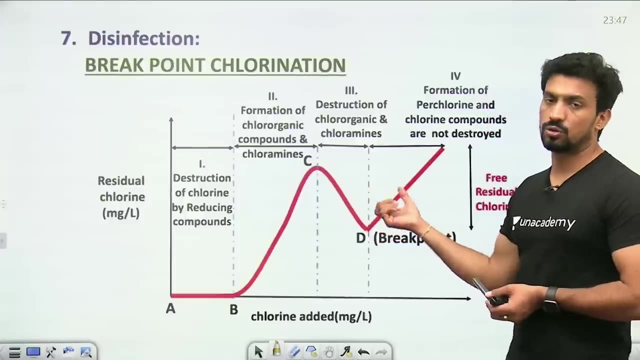 So this is zero, Because in the beginning Chlorine-reducing compounds, Chlorine reacted with them first, So you did not get residual chlorine, Then after that Chloramine or chlorine. When the compounds of chlorine started to form, Then destruction of chloramine. 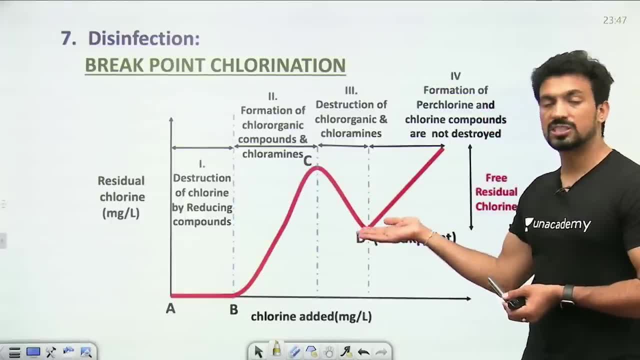 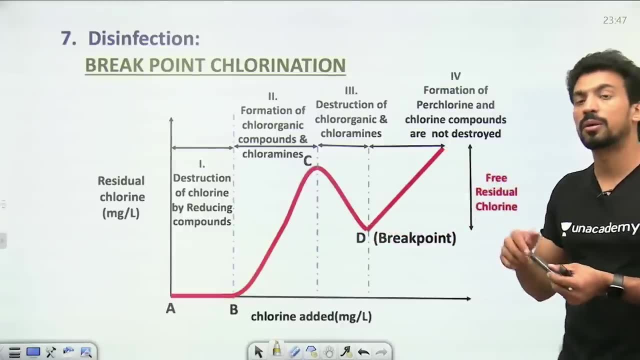 Or the compounds of chlorine. Then came the breakpoint, On which we will say: Now all the bacteria are killed, Chlorination is done, Chlorine will be added in the form of chlorine. So this is called breakpoint chlorination. A rural water supply scheme. 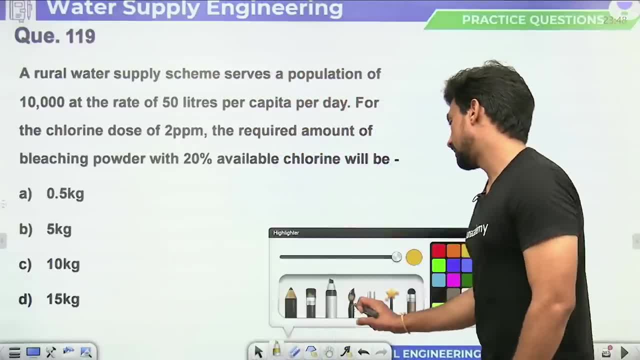 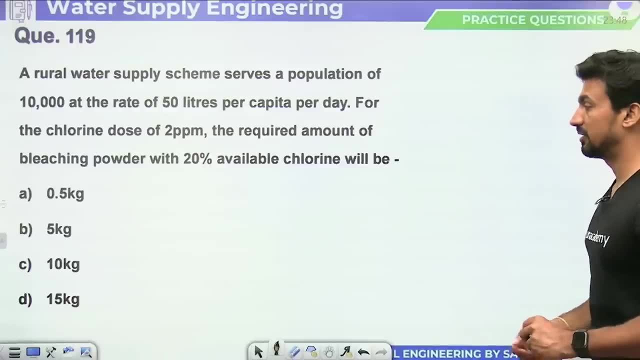 Serves a population of 10,000.. At the rate of 50 liters per capita per day, For chlorine dose of 2 ppm, The required amount of bleaching powder With 20% available chlorine will be. There are 10,000 people. 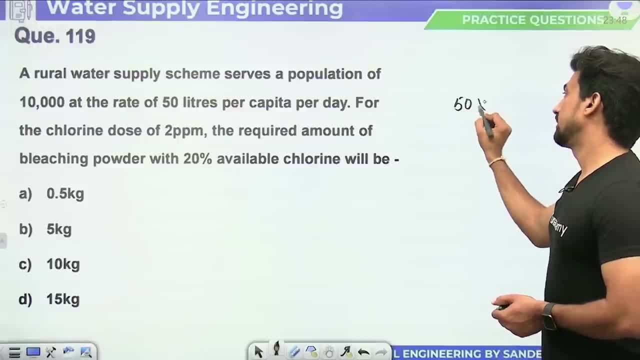 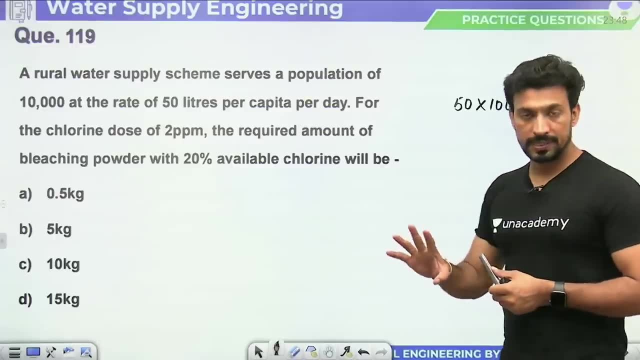 50 liters of water is required daily, So 50 liters daily is required. How many people- 10,000 people- need this much liter of chlorine, For chlorine dose of 2 ppm, 2 mg per liter is to be provided. 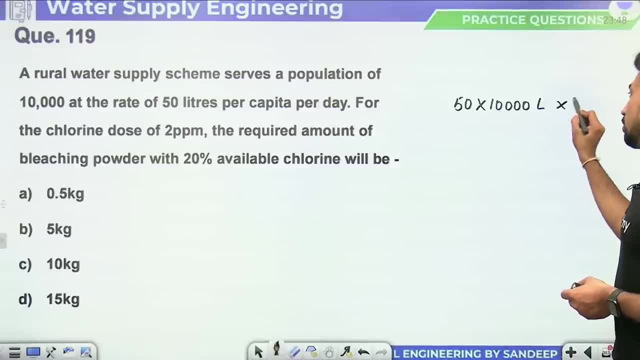 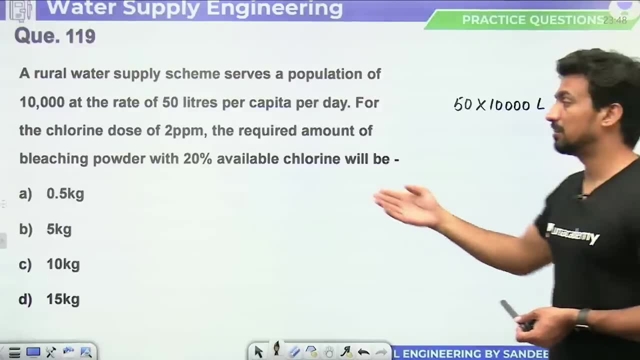 There are so many liters And if 2 mg per liter is to be provided, Then this much chlorine will be required. But the chlorine which is present, In which form is present? Bleaching powder, The amount of bleaching powder we will add. 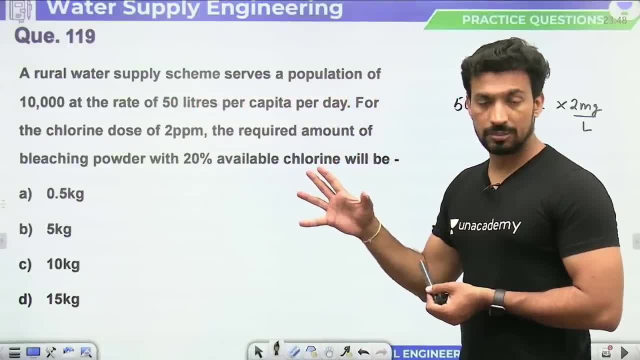 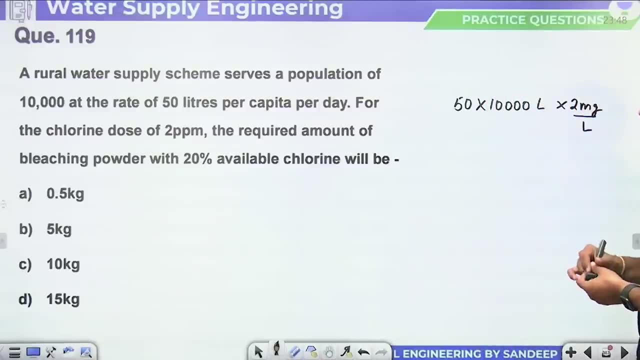 It has 20% chlorine, Means 5 times bleaching powder will have to be added. Then only The need of chlorine will be fulfilled. So in the bleaching powder There is 20% chlorine If you multiply it with 100 by 20.. 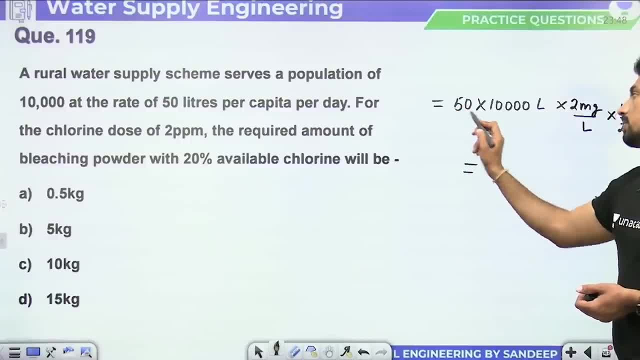 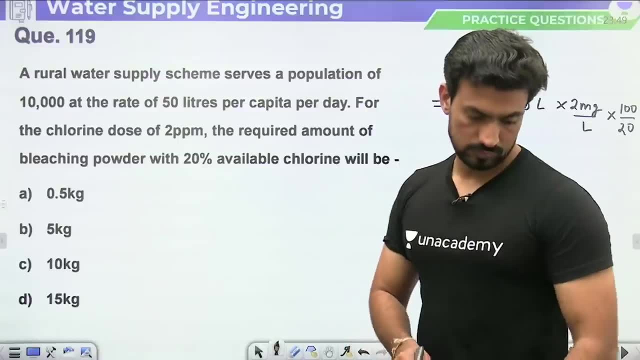 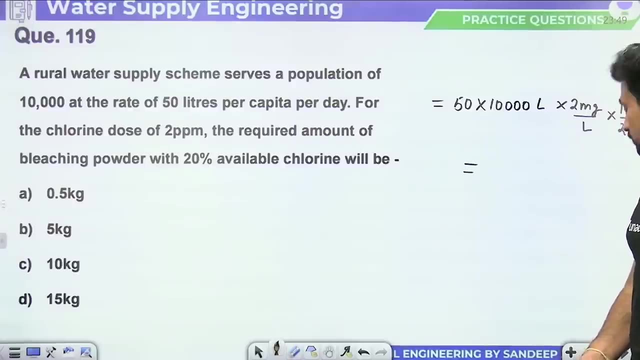 Then you will get this much chlorine. So tell me What is our value? Whatever answer, you will get 5 into 10 raised to the power 6.. This came in milligrams And this we will write: 5 kg. 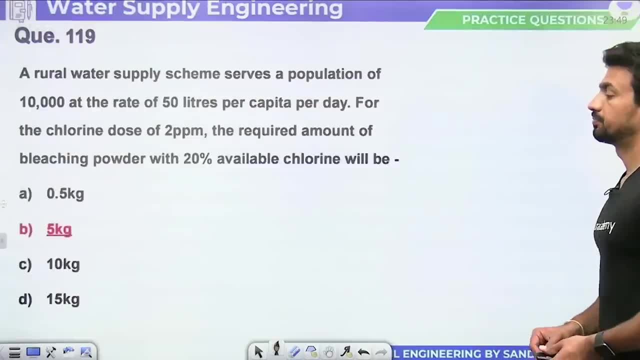 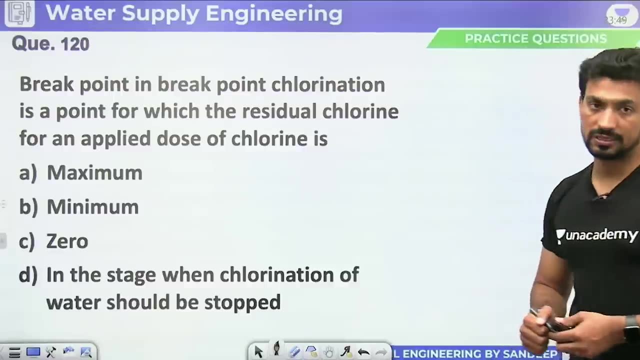 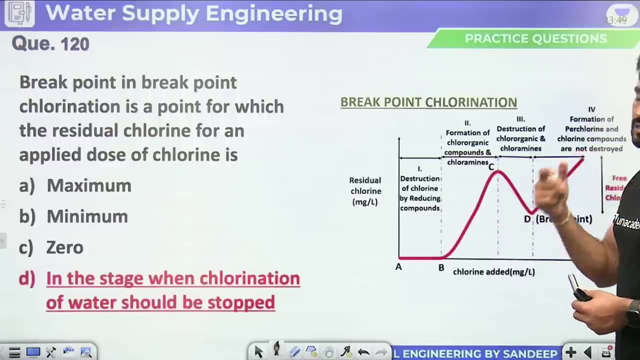 Next, Let's move ahead. Breakpoint in breakpoint. chlorination Is a point For which the residual chlorine For an applied dose of chlorine is Now in that stage. This should be stopped, Because more chlorine will be added In the form of residual chlorine. 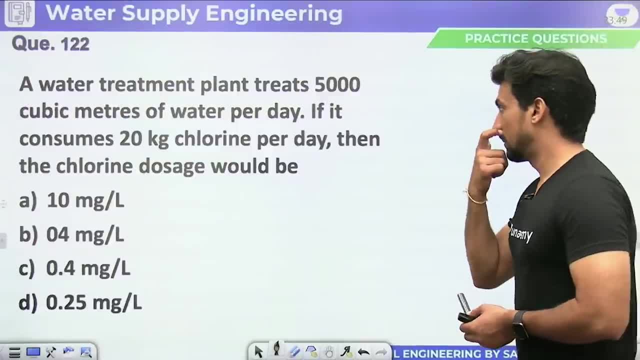 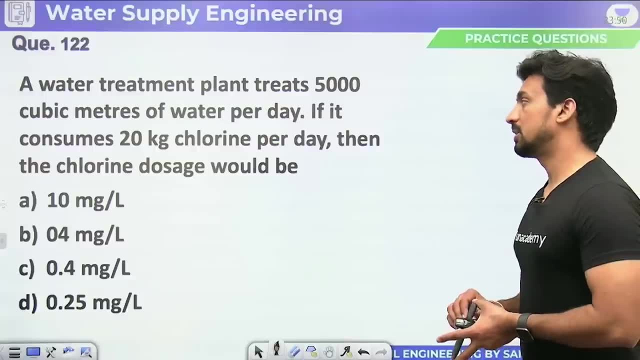 The percentage of chlorine. This is repeated again. A water treatment plant Treats 5000 cubic meters of water per day. If 20 kg of chlorine is utilized every day, Then what is the dosage of chlorine? 20 kg is used. 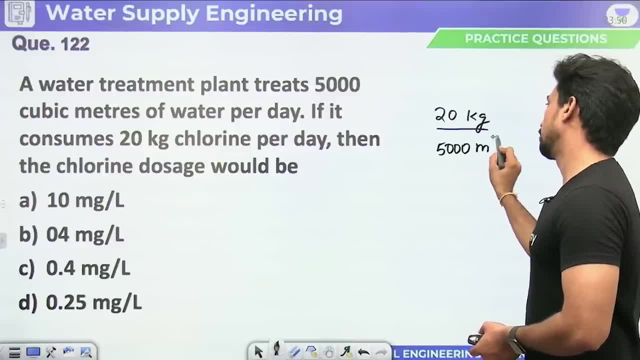 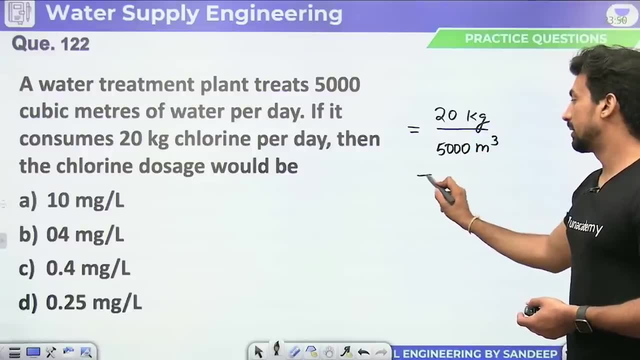 For how much water? For 5000 m3.. So this is the dosage. Then the chlorine dosage would be: You have to express in milligrams per liter: 20 into. To convert kilogram into grams, 10 raised to the power 3.. 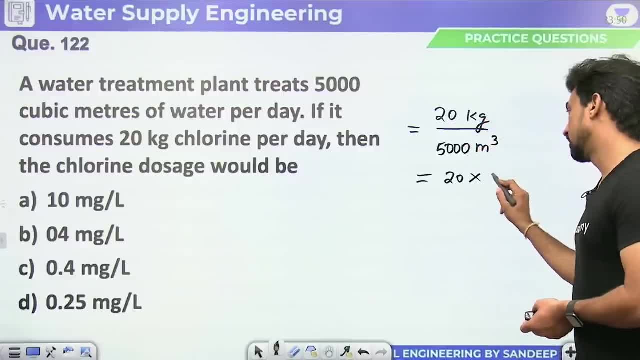 Then to convert into milligrams Again, 10 raised to the power 3.. So you can write: 10 raised to the power 6.. Milligram Upon 5000.. To convert meter cube into liters, 10 raised to the power 3.. 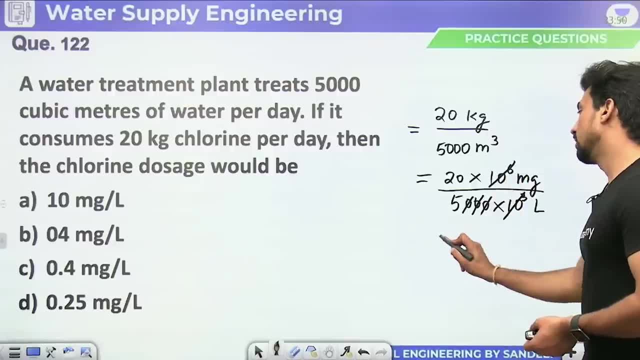 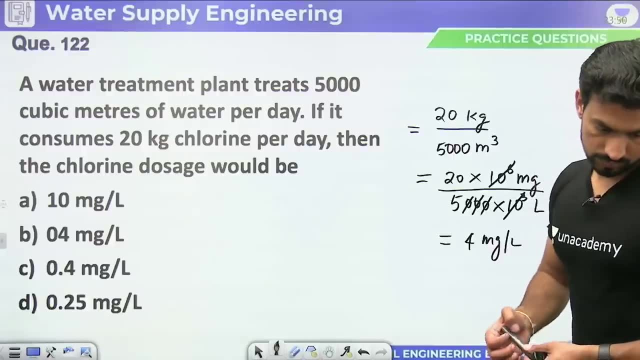 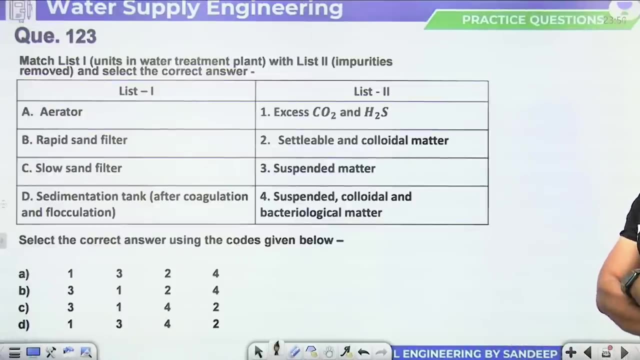 10 raised to the power 3.. And this 3 and this 6 will be cancelled out. 30 by 5 will be 4.. Next let's move on. Those friends who have not liked the session yet. You can like the session. 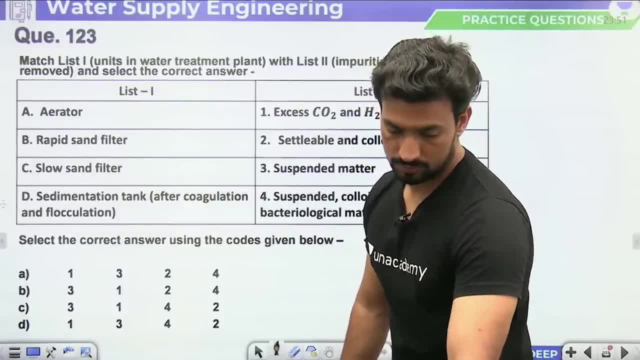 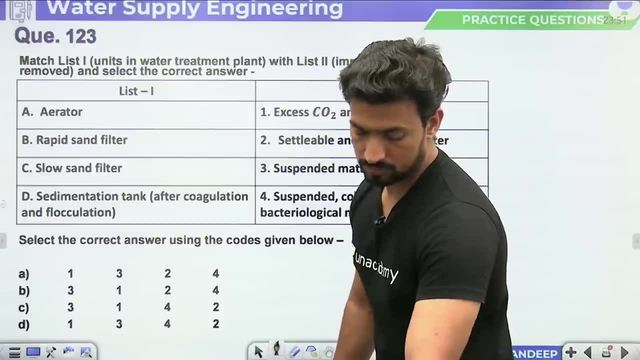 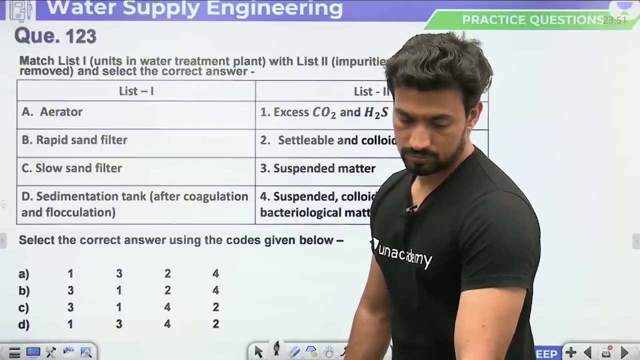 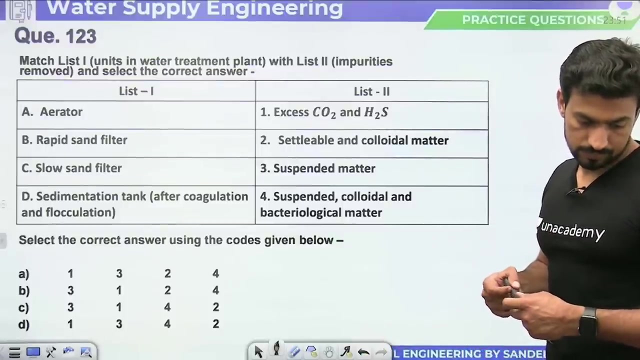 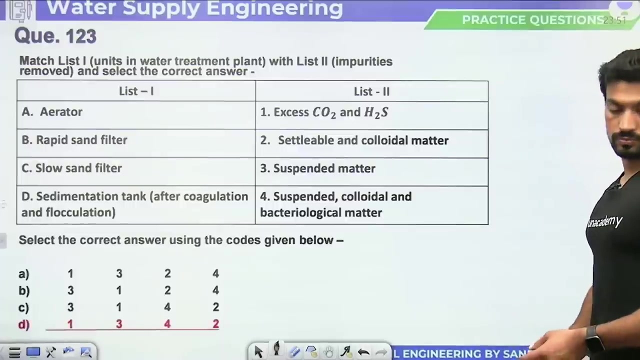 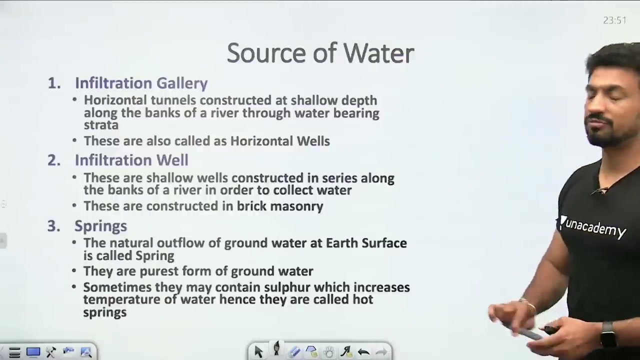 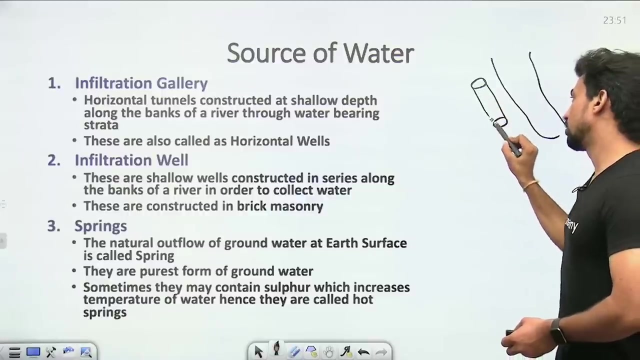 If you like these sessions, Then please like and subscribe. 30 more hours, Almost done, In sources of water supply: infiltration galleries. if any river is flowing, then parallel to this river, horizontal wells are provided so that the water coming from the sea can be extracted. 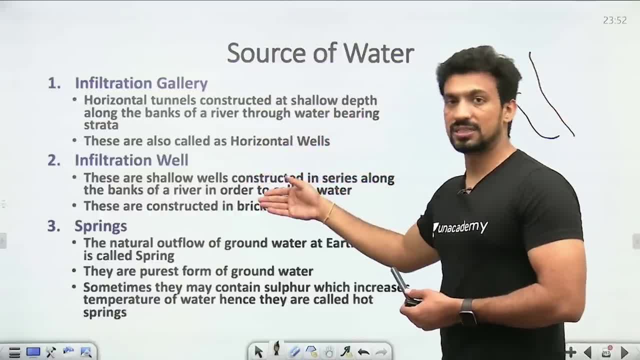 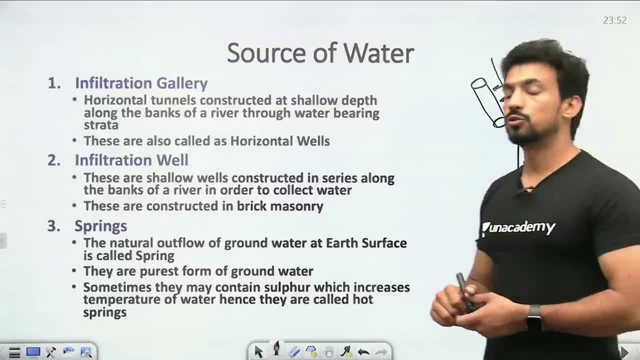 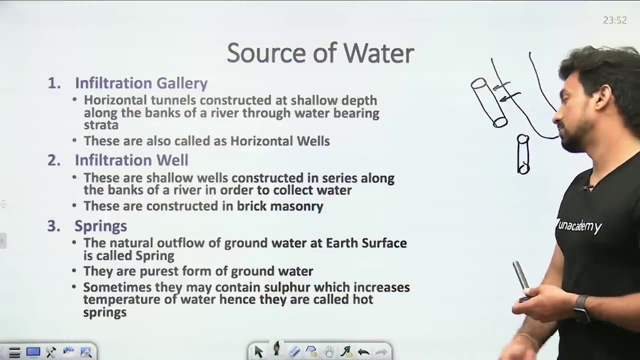 Water can be taken from infiltration galleries. Filtration wells can be made. proper wells like this is a gallery. in the same way, the wells that you have made in the vertical direction, you can use them. There can be springs. groundwater is coming out anywhere in the form of a stream. you can use them. you can use spring water. 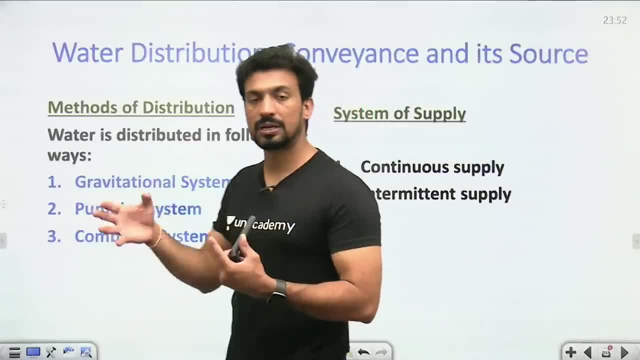 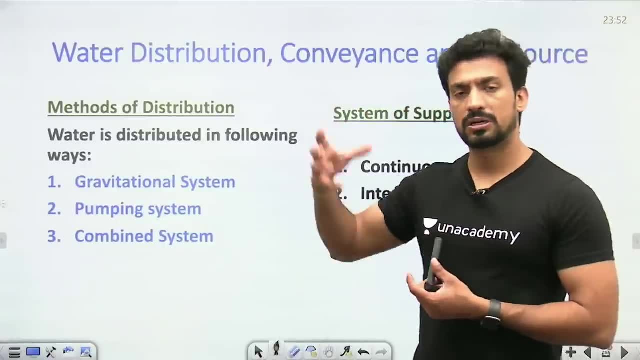 If we come to the methods of distribution, then the first one is gravitational: water is flowing and distributing by itself due to gravity. Second: pumping: you are making it flow by pumping. Third, combined, first pumped and stored at a high height. 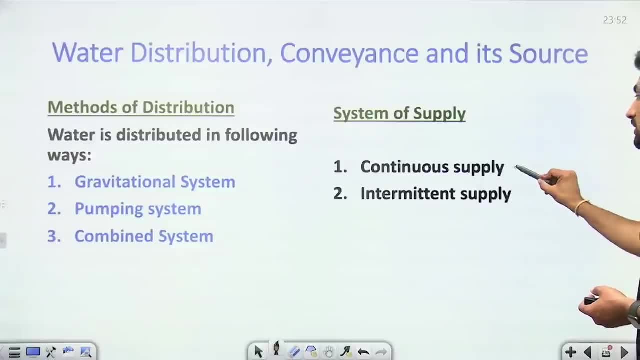 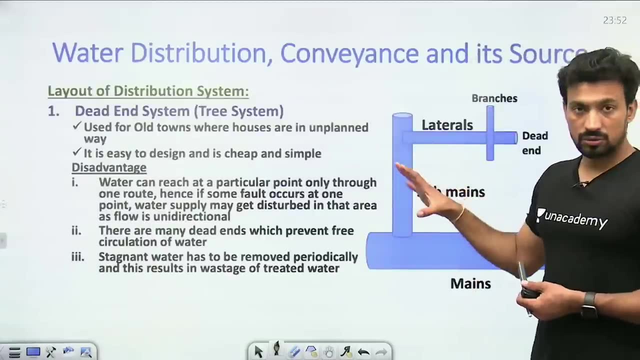 After that it is distributed. due to gravity System of supply, 24 hours of water is being given, or it is morning, evening or intermittent. sometimes it is being given So that one has come. Now. if we talk about the layout of the distribution system, then the first one comes in the dead-end system. 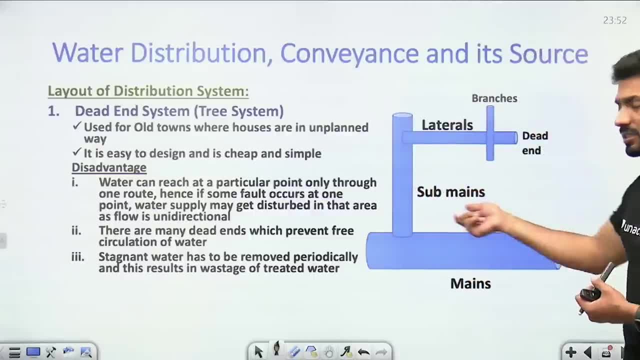 In which what happened in the old cities, with no planning? one main went, all the mains went, laterals went, branches went as needed, pipelines were taken And a dead-end will also be formed by going somewhere. So this will be used in these old towns. 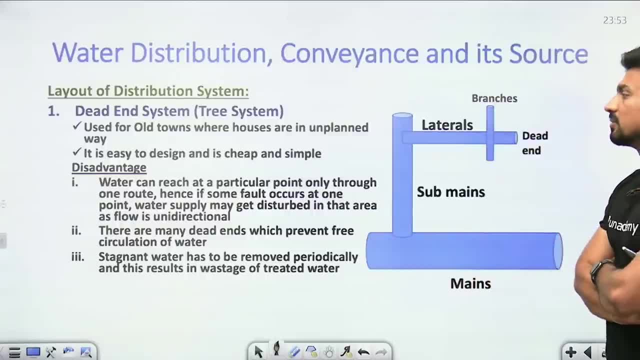 Anyone can use it. There is no need to design in it, So that's why it is simple and cheap. What is the disadvantage? If there is any problem here, then the entire water supply scheme in front of it will stop. It will be fine here, then only the water will reach the whole area. 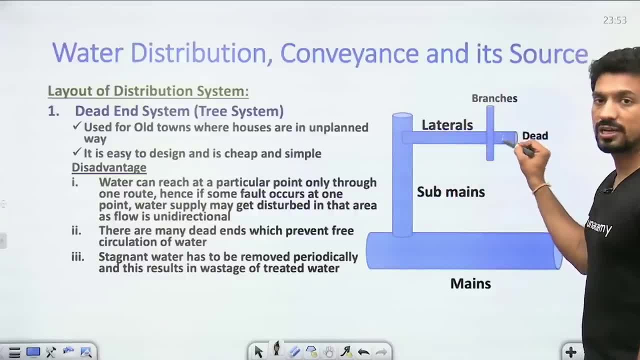 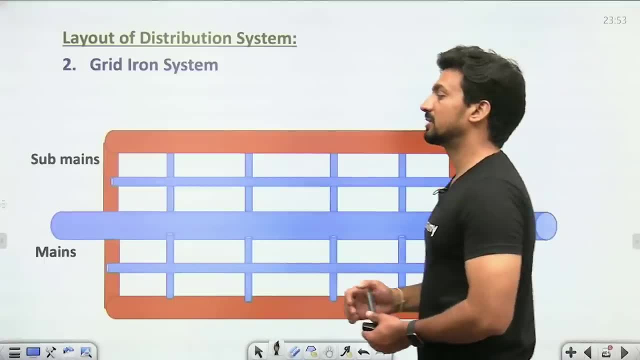 So this is its drawback. If the water here is not being used, then stagnant water will be formed. Stuck water will create a problem again. It will start getting bad. Next comes the grid iron system. Mains will go in the grid iron system. 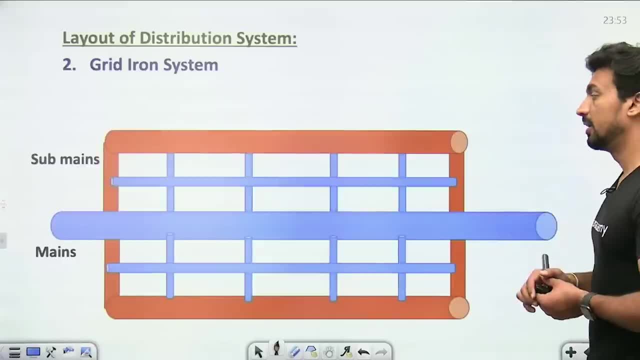 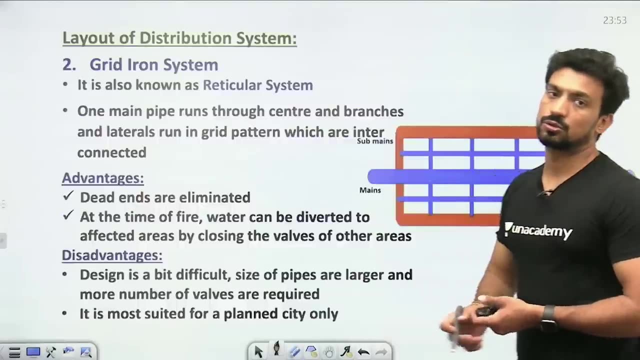 Laterals will be distributed like this. The advantage of this is that if there is a blockage somewhere, then the water can be delivered in a different way to other areas, So this is a good thing about it. We also know it by the name of reticular system. 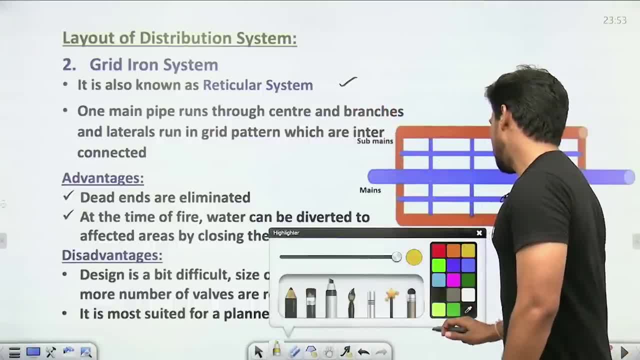 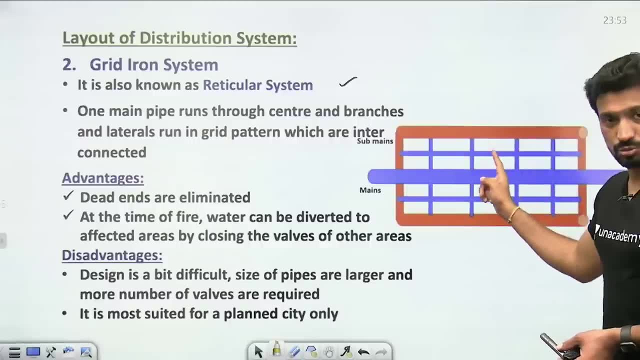 And it can be used only in well-planned cities, Because if you make a grid in it, then there should be a proper way. If the pipes are used more, then this is also its disadvantage, That the pipes will be used a lot. 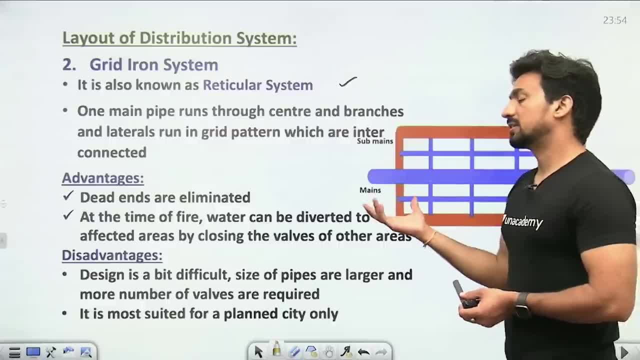 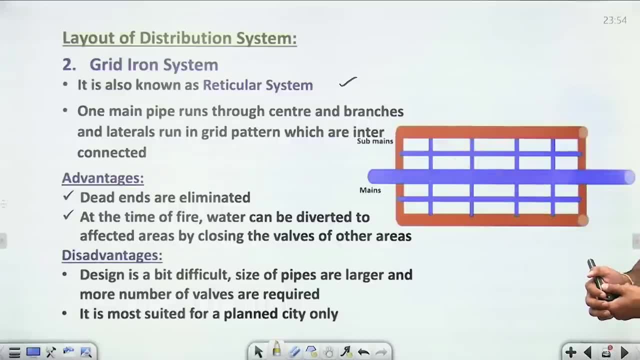 The number of walls will be used a lot. If there are fires, then in that case all the other walls can be closed and water can be given in the area where more water is needed. So this is also its advantage here. So you have to remember the name of its reticular system. 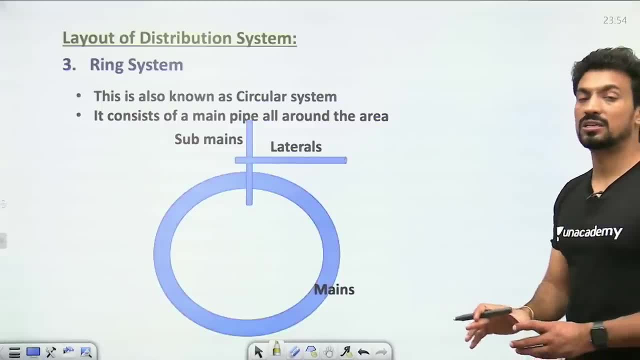 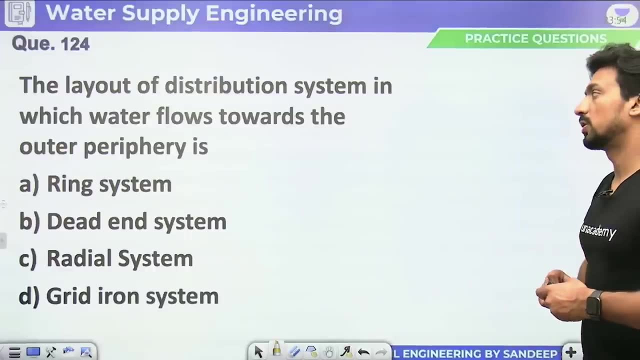 What will happen in the ring system? A circular pipe will run around the whole area And then we can distribute the water further in that area. The layout of distribution system in which water flows towards the outer ferry, So we will call it ring system. 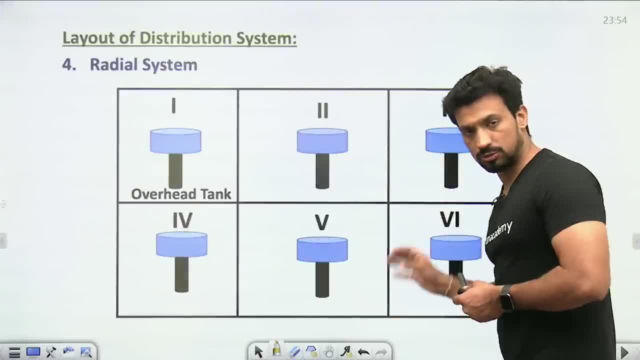 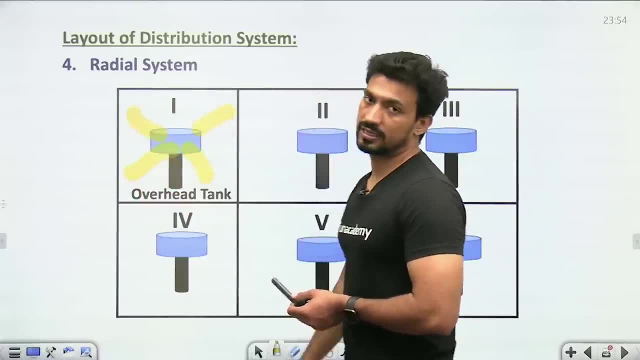 What will happen in the radial system? The whole area will be divided into different zones. There will be an overhead tank of each zone Which will spread or distribute water in this particular area. So this is called radial system. What is the advantage? 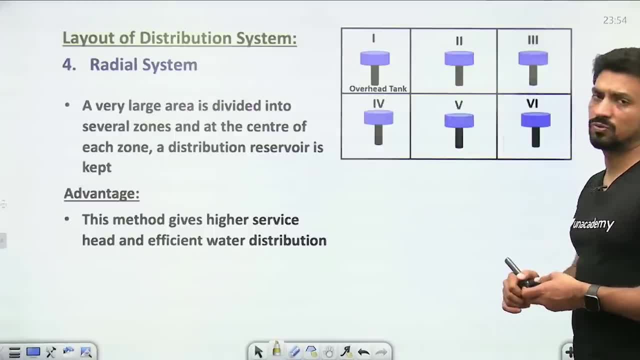 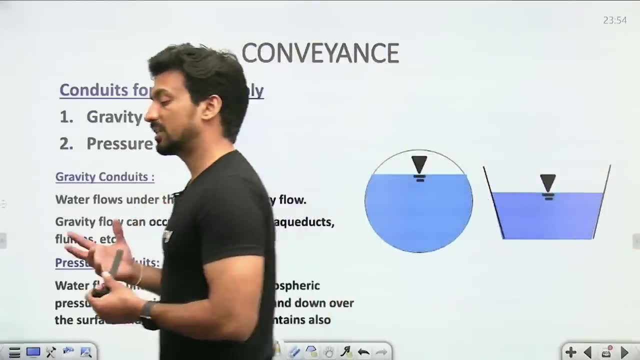 Higher service head is available With the help of your service reservoir or tanks. If you want to do convey, then you can do it through pipes In which water will go through pressure, So pressure conduits can be done. Second is like open channel flow. 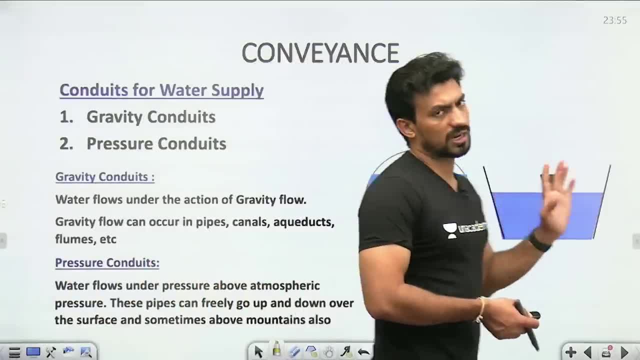 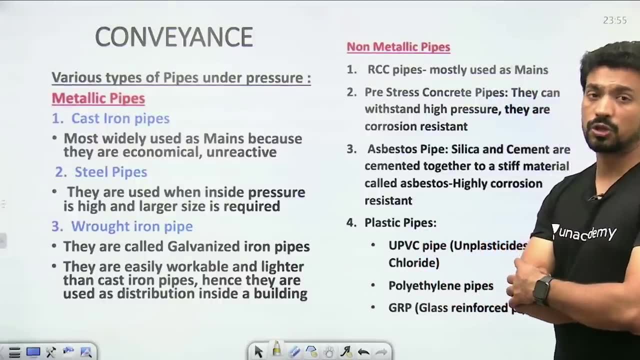 In which water is not flowing. The pressure on the surface of the water is atmospheric pressure Can be done in this form. Cast iron pipes are mostly used in the form of main pipes Because they are economical. This has been asked from you in the objective. 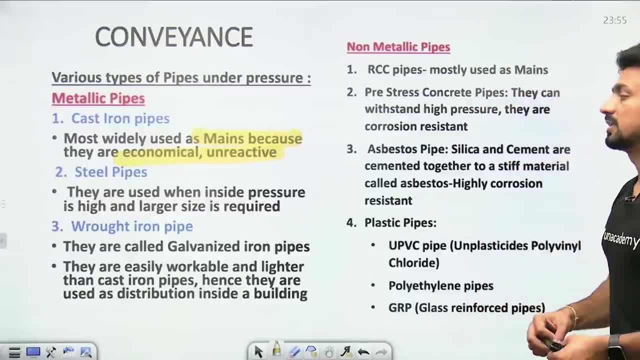 Economical and unjective. Steel pipes can be used when the pressure is too much. Rot iron pipes can be used in the form of galvanized iron pipes And they are light. If you have to do distribution in any building, then you can use them. 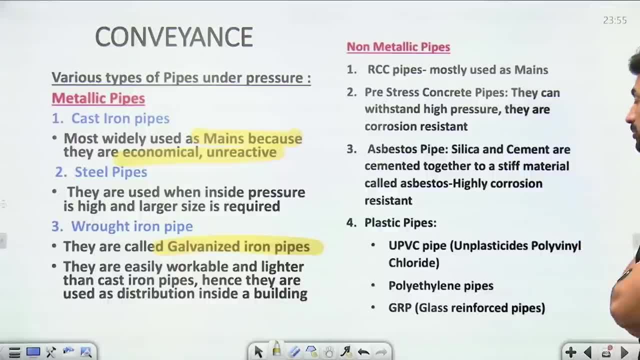 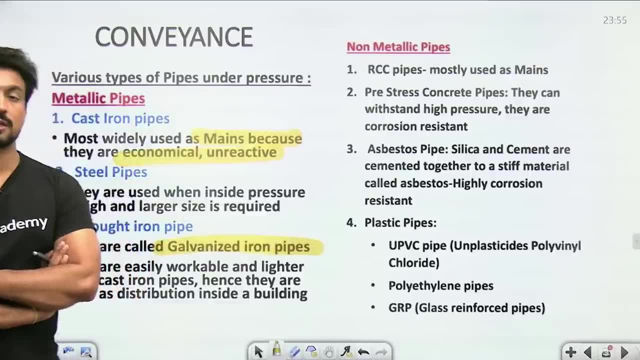 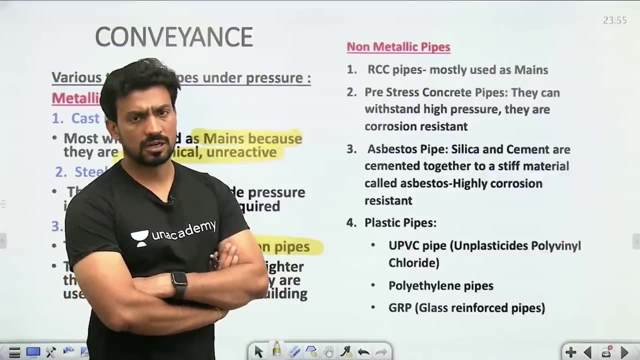 These days, PVC. PVC pipes are used Because it is non-reactive. It also resists high temperature. It is economical, It does not break. It is repairable. If there is a crack somewhere, it can be repaired. RCC pipes are used in the form of mains or where more water is needed. 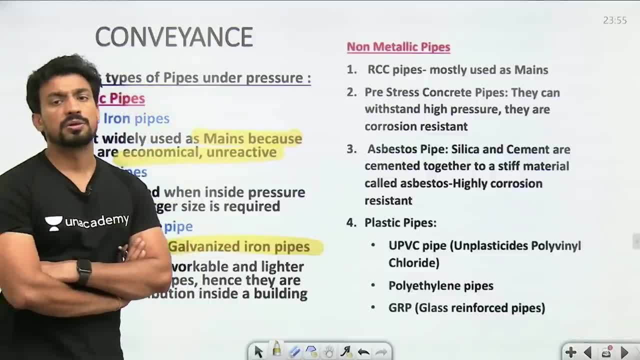 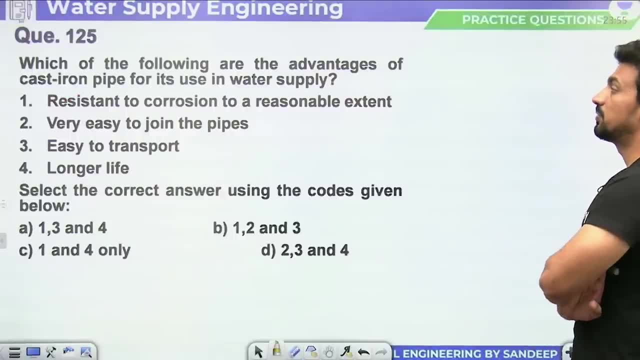 Pre-stressed concrete pipes can be used. Asbestos pipes can be used. PVC UPVC can be used. Glass reinforced pipes can also be used. Which of the following are advantages for cast iron pipe for its use in water supply? The advantages are its resistance to corrosion and longer life. 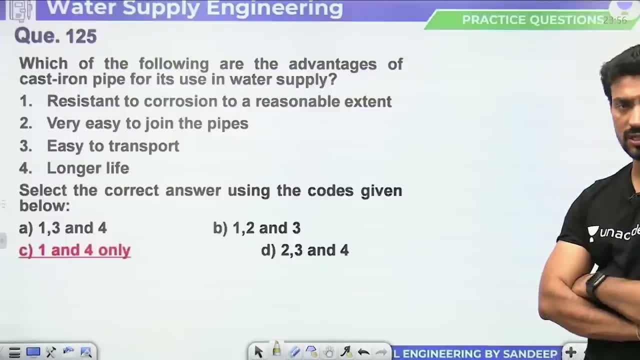 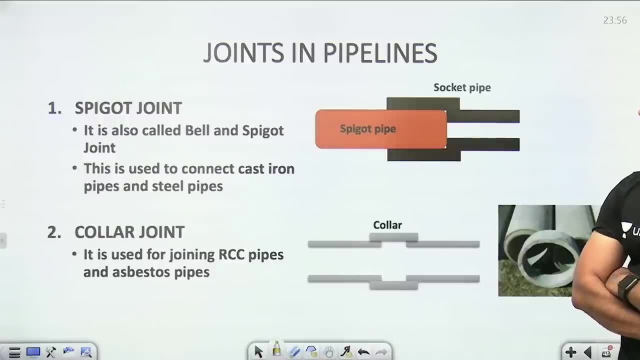 It is not so easy to join pipes And they are heavy So it is not easy to transport. Bell and spigot joint is called spigot joint. It is used to join cast iron and steel pipes. Collar joint is used to join the RCC pipes. 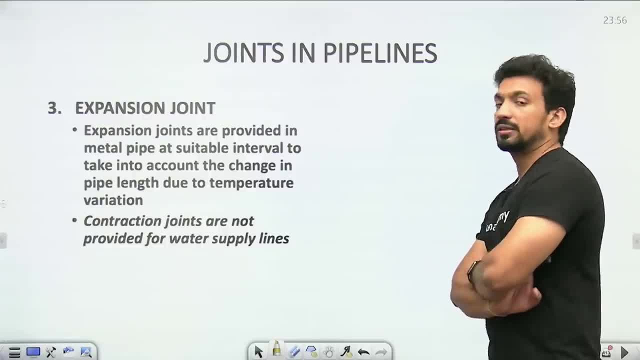 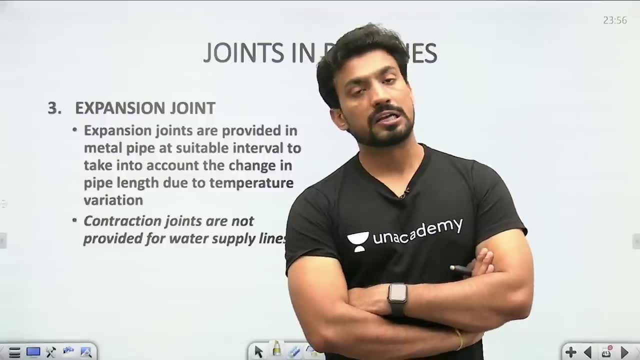 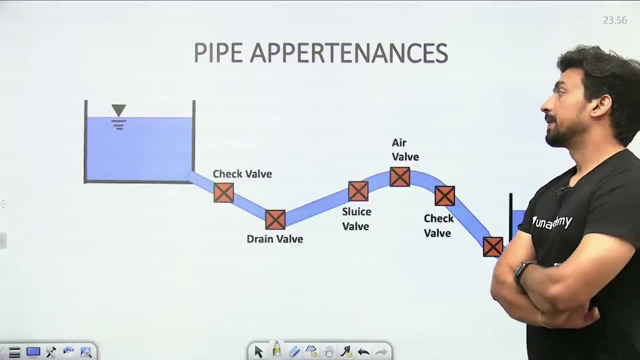 Expansion joint, Which are your metallic pipes In which you worry about expansion and contraction, Expand and contract due to temperature. But we only provide joints for expansion. Joint is not provided for contraction In water supply lines. Different types of walls are used in the pipe. 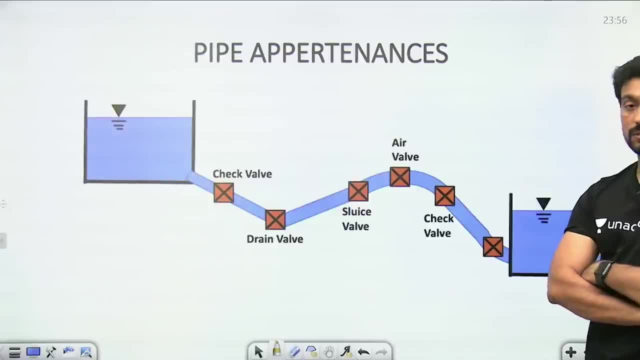 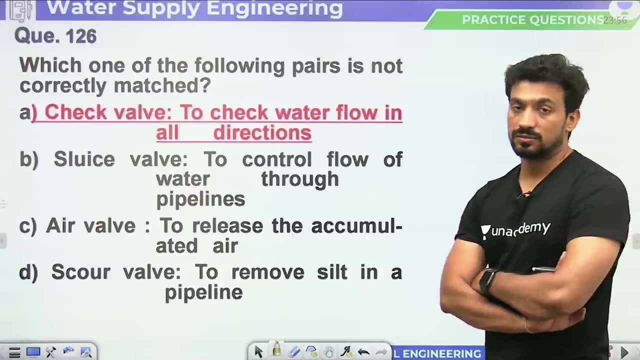 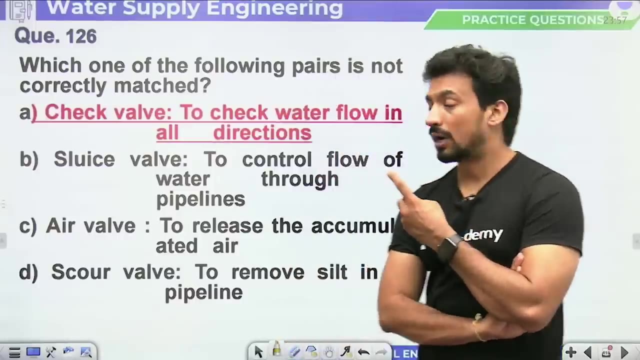 Check walls, drain walls, sluice walls, air walls. These walls are used in such pipes, If we talk about them. So check wall For that check wall or reflux wall. It allows the flow of water in one direction. So I have asked you in the question. 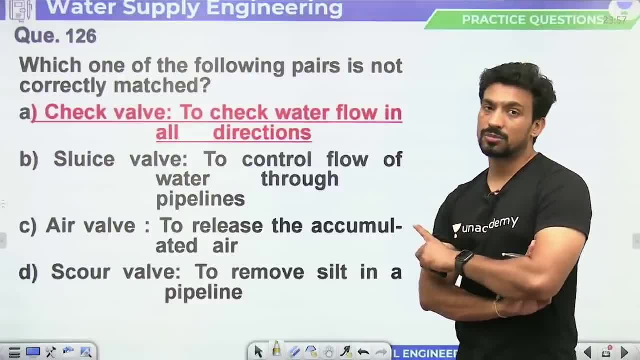 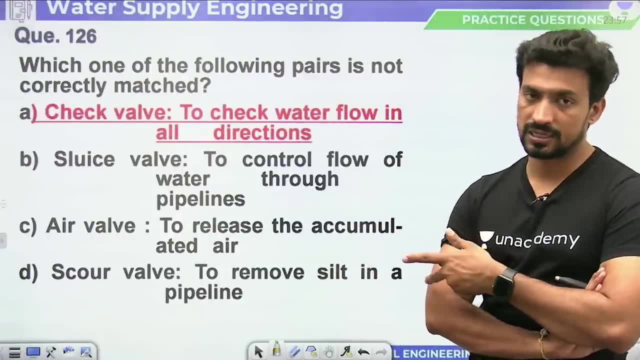 Which out of the following pair is not correctly matched? So check wall will allow the flow of water in one direction. Sluice wall or gate wall: It regulates the flow, Where to let the water go or not. Air valve is used to release the air. 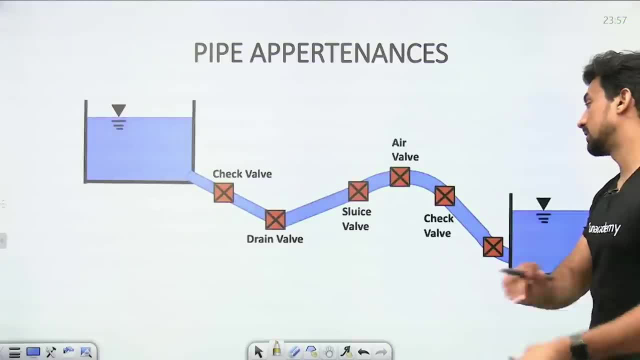 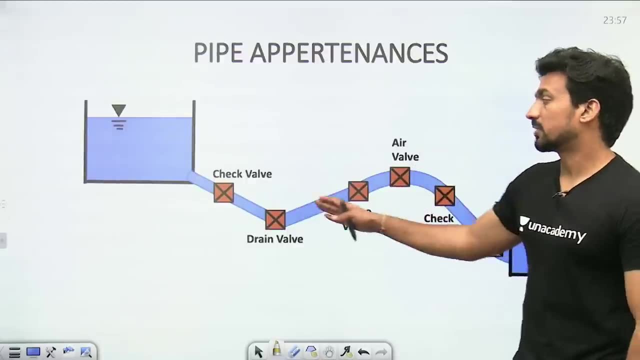 Scouring wall. If silt is accumulated somewhere, Sediments are accumulated, So it is below Drain, or scouring wall will be removed from here. If air is accumulated, then it will be here. It will be removed from here. Check wall will also ensure that the water goes only in this direction. 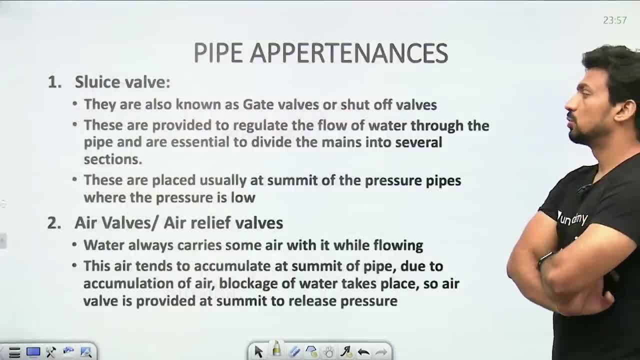 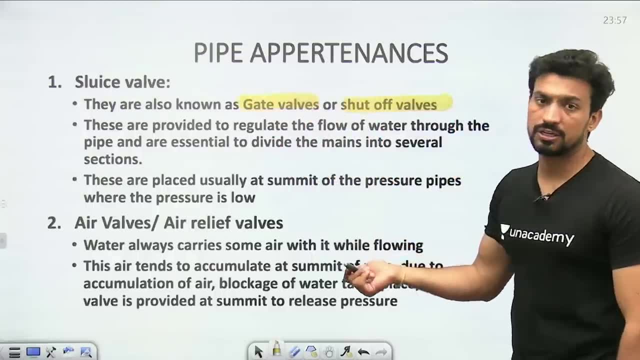 Do not go back this way. Next come Sluice wall. Their name, Gate walls or shut off walls are also called Air valves, are used to release the air. Whatever blockages come, they are removed from here. Check wall, reflux wall or non-returning wall. 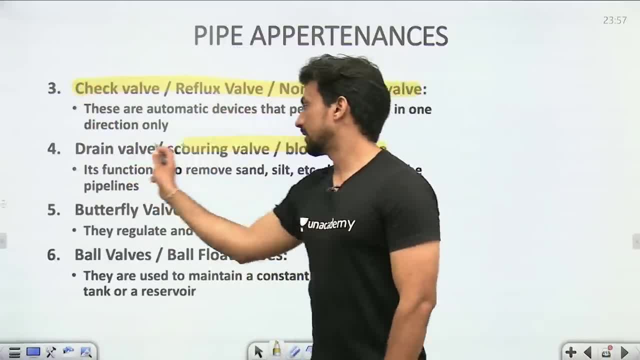 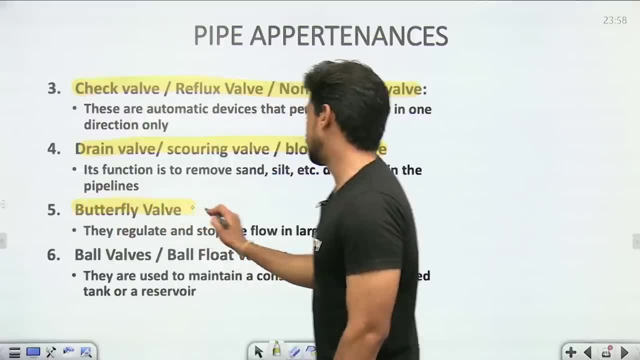 Water flows in the same direction. For this, Skull walls, scouring or blow up walls are used. They are used to remove the particles that have settled. Butterfly walls are used in large-sized pipes. Ball walls Like in the cooler You must have seen in the desert cooler. 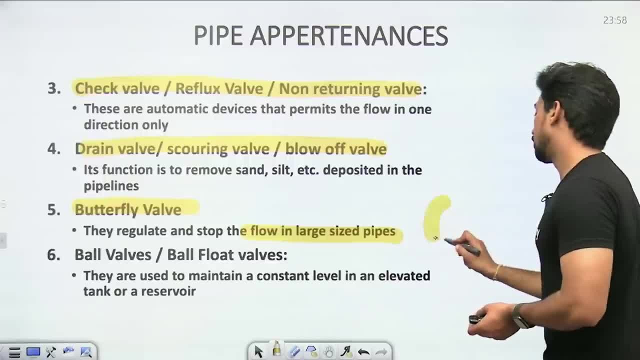 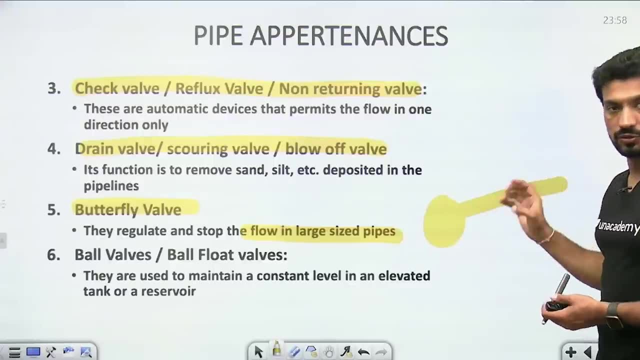 Balls are used in the tanks. on the roof There is a ball And here it is joined like this: As the water keeps flowing, it rises like this From here. the valve closes, So reservoir and tanks are used. Pressure relief walls. 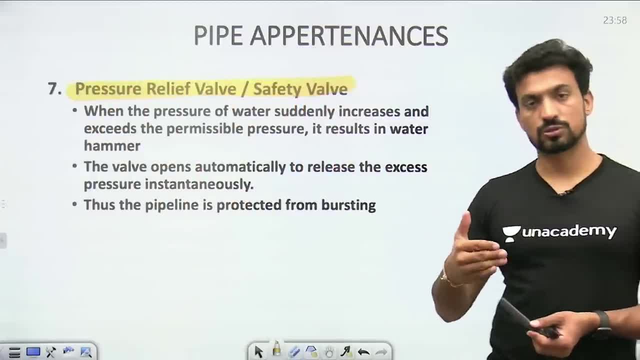 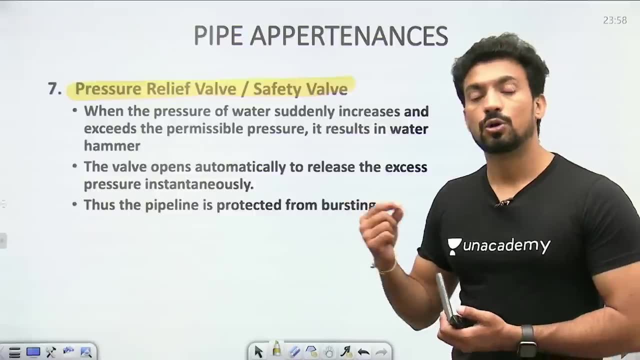 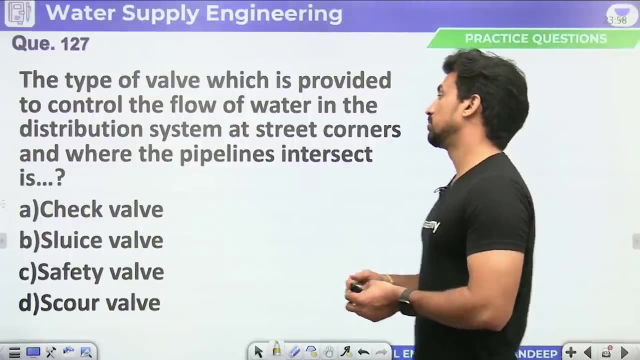 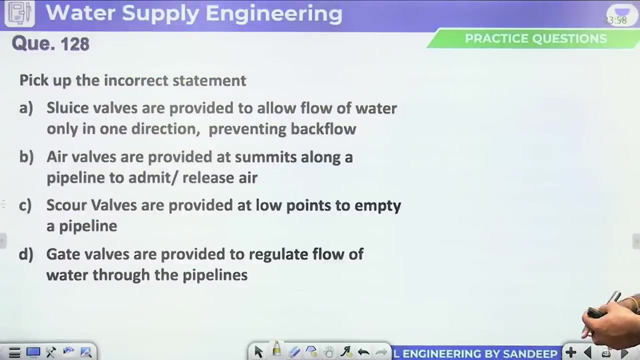 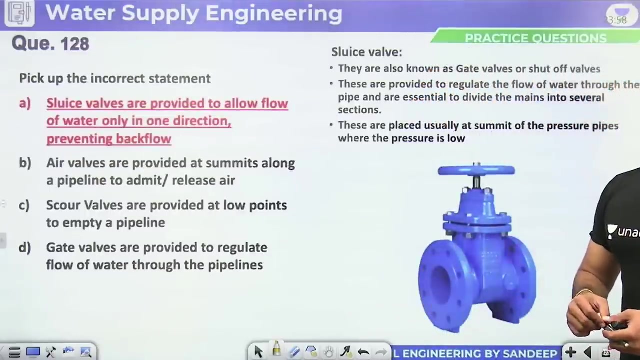 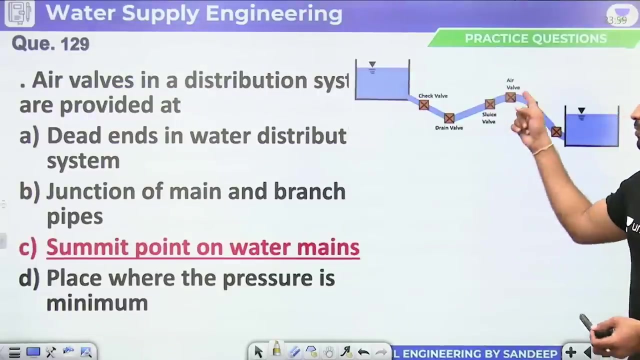 the type of wall which is provided to control the flow of water in the distribution system at street corners and where the pipelines intersect is sluice wall. pick up the incorrect statement. sluice walls are allowed to flow water in only one direction. air walls in distribution system are provided at summit and air vessel is provided at summit. 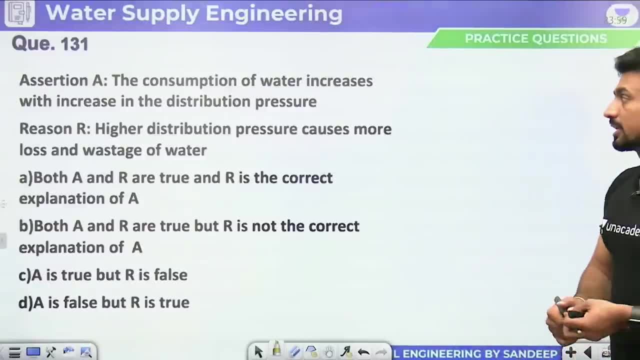 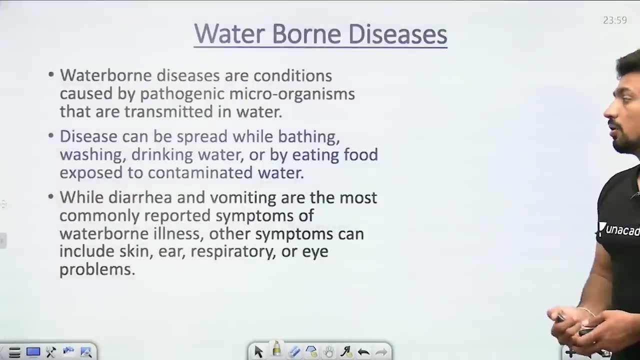 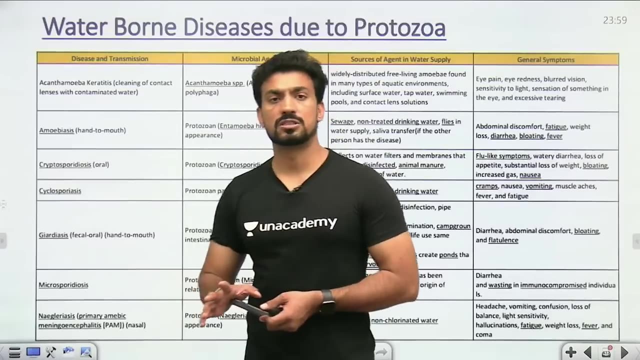 in siphon to avoid interruption in the flow. the consumption of water increases with the increase in distribution pressure. this question is repeated. if we talk about water borne diseases, then you have some set of diseases: bacteria, virus, protozoa- all these diseases. you can go through them.